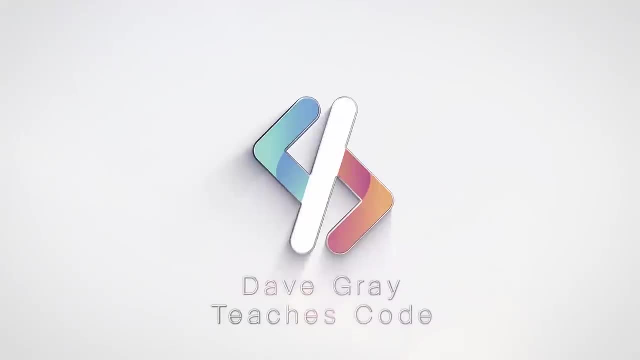 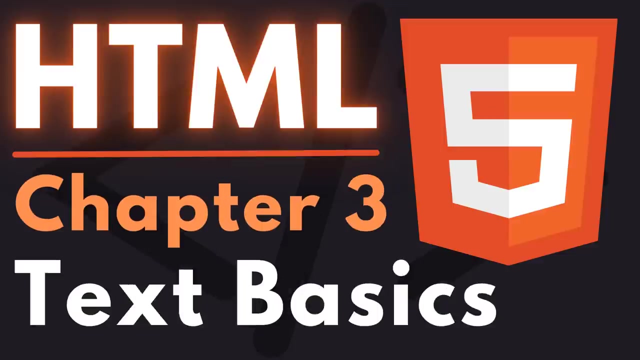 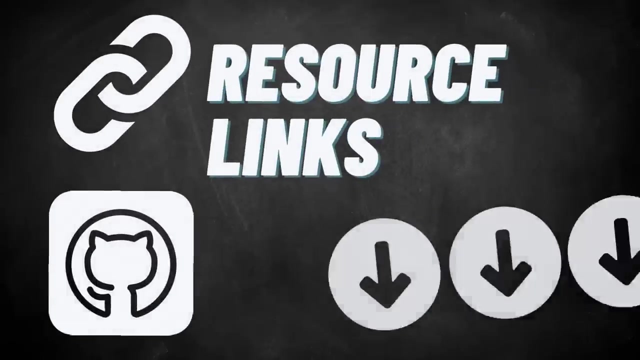 Hello and welcome to Four Hours of HTML Tutorials and Instruction. This video is made up of ten tutorials for learning HTML that build upon each other much like the chapters of a book. Throughout the lessons in this video, I will mention links being available in the. 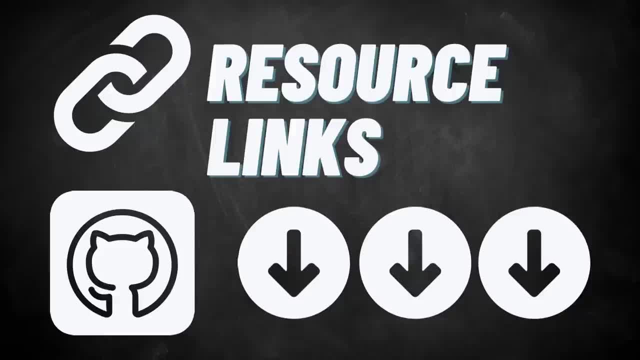 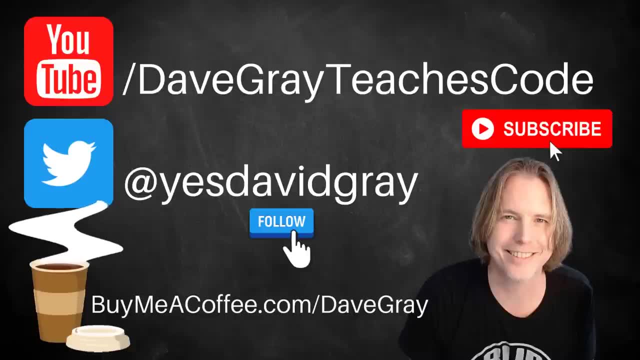 description below. I've compiled all of these links into one GitHub resource that you will find in the description. Hi, I'm Dave Gray and I'm the creator of these HTML tutorials. You can subscribe to my YouTube channel for more tutorials like this one. You can also. 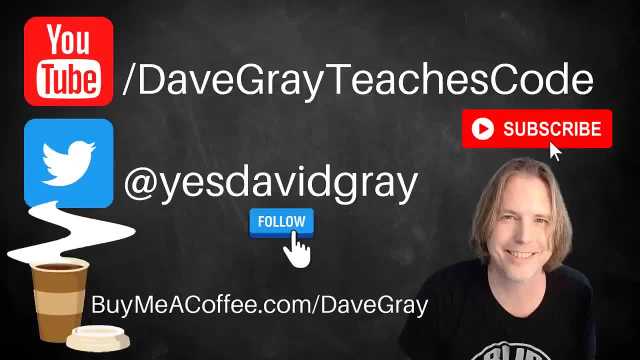 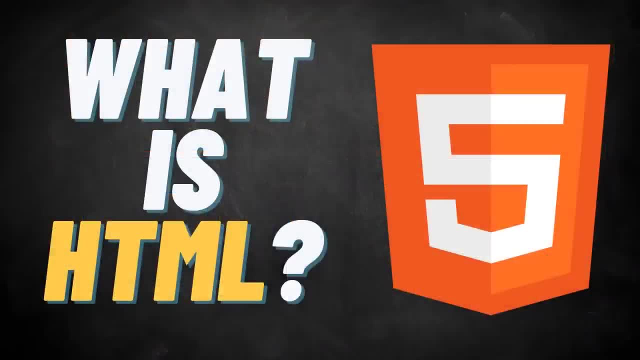 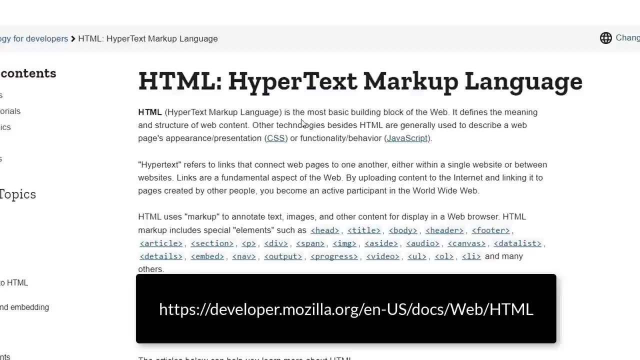 follow me on Twitter and if you're feeling generous, you can even buy me a cup of coffee. Let's get started learning HTML with Chapter 1.. What is HTML? HTML is an acronym that stands for Hypertext, Markup Language And Hypertext. 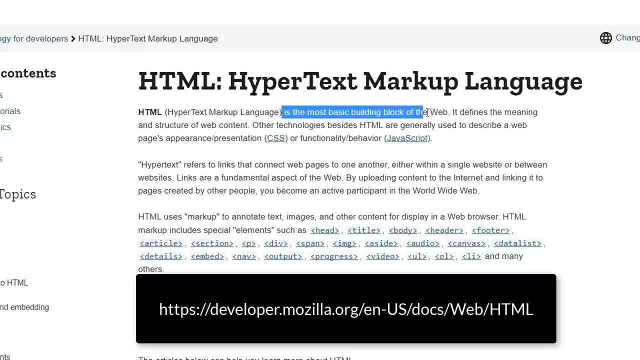 Markup Language. HTML is an acronym that stands for Hypertext Markup Language, And HTML is the most basic building block of the web. It defines the meaning and structure of web content, And hypertext refers to links that connect web pages to each other. And 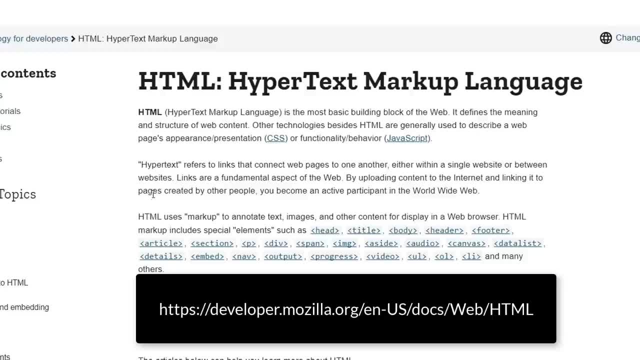 that can be within a single website or from one website to another. Overall, HTML uses markup to annotate text, images and other content for display in a web browser, And you can see an example of some of these markup elements here. But before we begin creating, 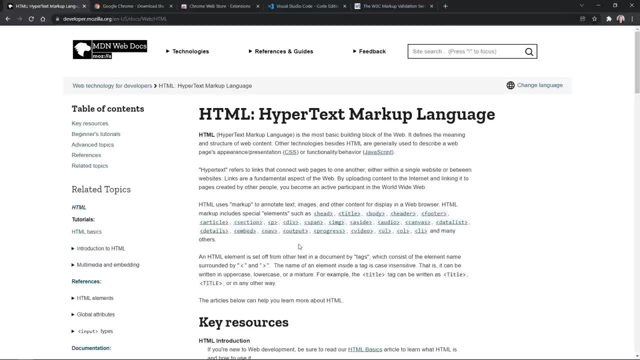 a web page and using it. I want to give you a little bit of an overview of what HTML is. To start using these markup elements, we need to get the necessary tools, So let's start with a web browser. If you don't have one, or if you're curious what I will be using, 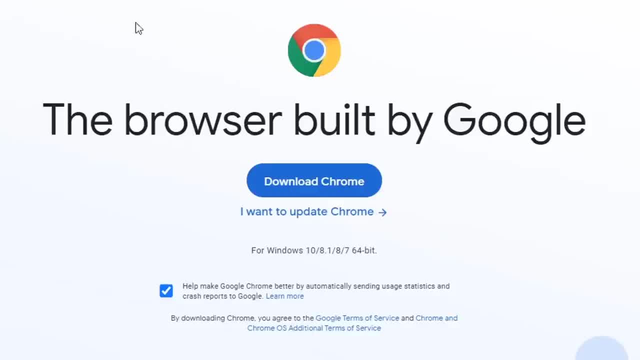 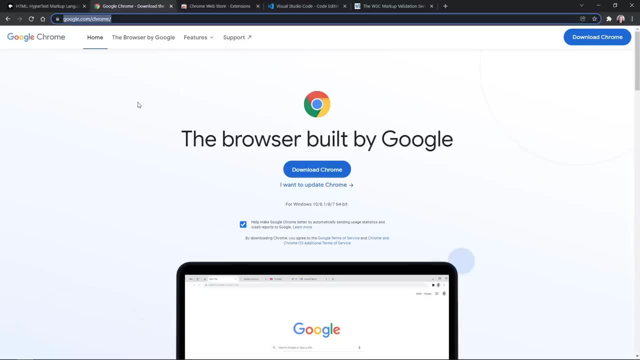 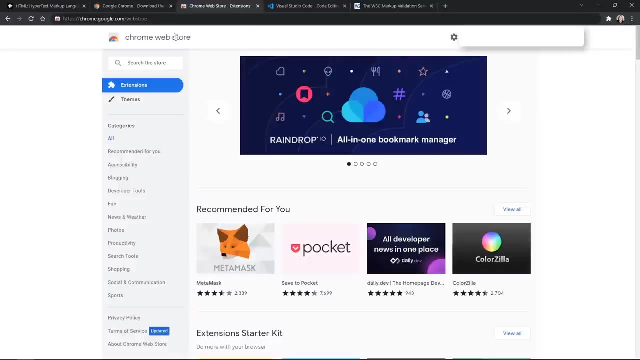 in this series I'll be using the Google Chrome browser And you can download that at googlecom slash chrome. So if you don't have that and want to use that, go ahead and download and install now and then come back to the tutorial. Also, I will be using an extension and we 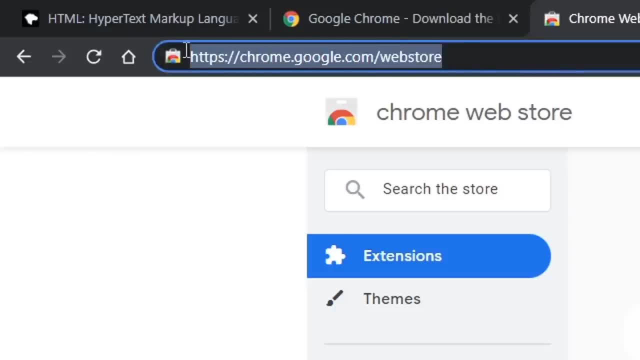 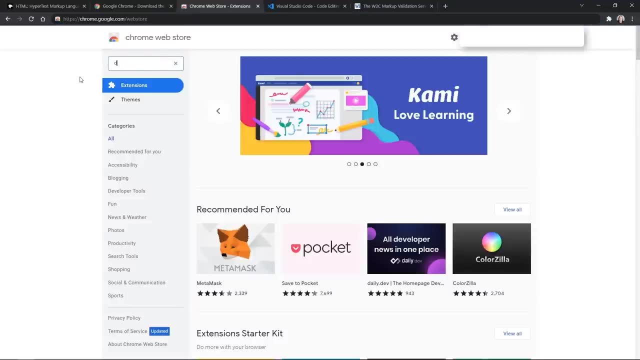 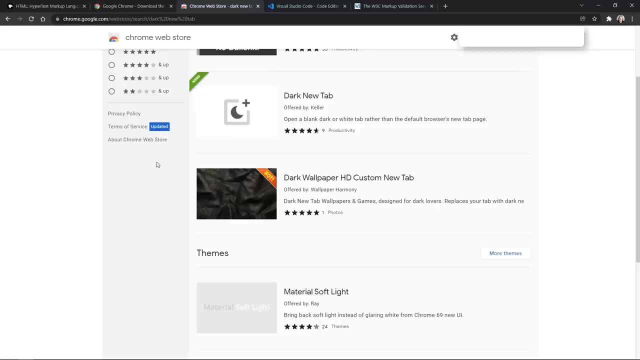 go to chromegooglecom And there, if you want to use the extension that I'm going to use, it's called darknewtab And you can press enter to search for that And once you've completed your search, you'll see darknewtab, offered by Keller, which is the one that I have added, And you can see. 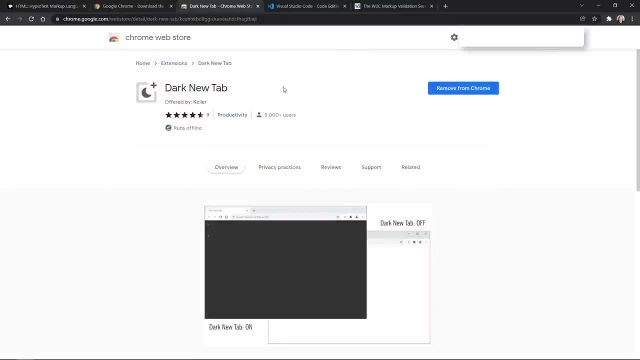 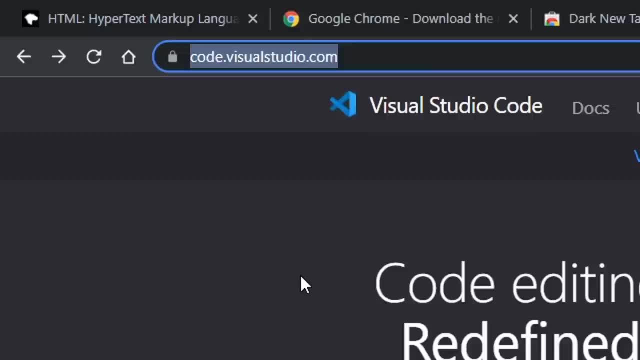 you should have an install button here, Since I already have it installed. this is now installed. you'll be able to download Visual Studio Code for free And there you can download for Windows- if you're on Windows like I am, or you can click other platforms. 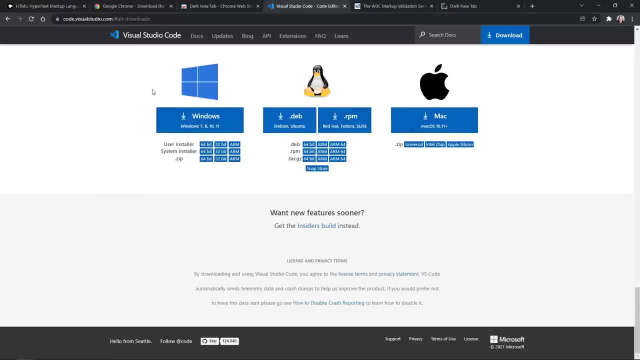 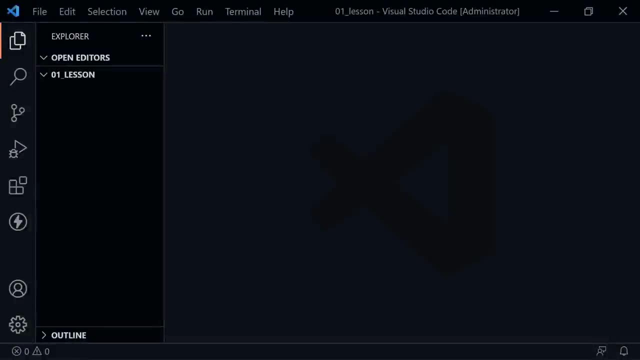 And it's also available for Linux and Mac OS. So now would be a good time to go ahead and download Visual Studio Code and install your code editor and go ahead and open that up and then come back to the video. Okay, I am now assuming you have installed Visual Studio Code. 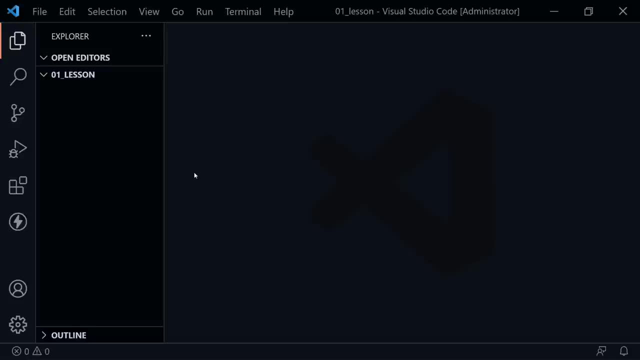 and have opened it up and you may see something like this or you may see a welcome screen. What you need to do is create a folder on your computer and we will put our files inside that folder. So if I go to the file menu and choose open folder, 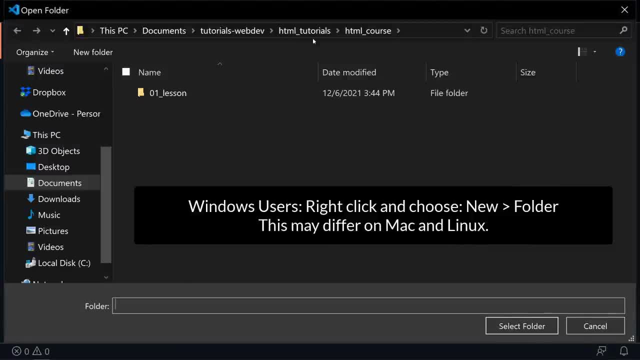 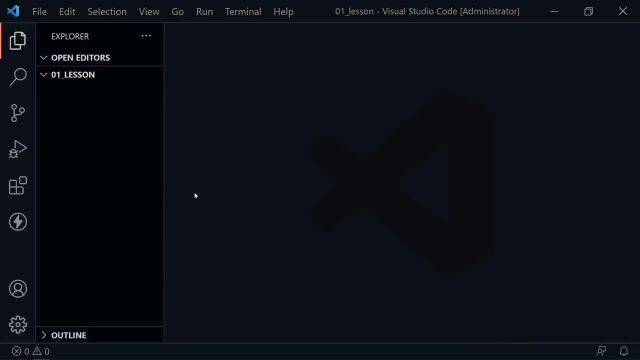 you can see once this pops up what folder I am in the HTML course folder in Windows and then I've created an 01 underscore lesson folder. So if I highlight that and select the folder, I am now inside that folder and ready to create my first HTML file. 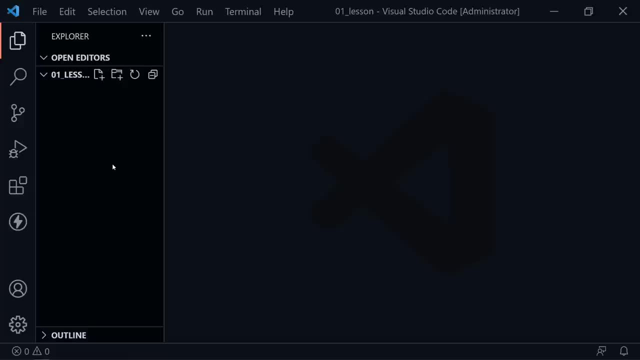 So if you see the file tree over here on the left and it's currently empty, if you don't click this icon in the top left, which is the file explorer and that will hide or show this file explorer, we're going to create the plus button. 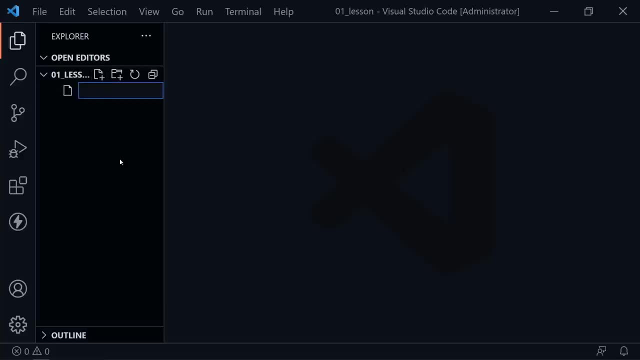 or click the plus button here for new file and create a new file. Now we'll type indexhtml, as that is always, and we'll create a new file name. that is expected to launch a website And you always want to keep your file names lowercase. 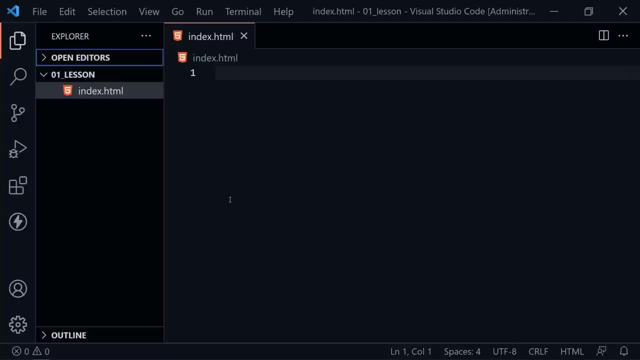 and with no spaces. Now, Windows will not complain if you put a space or use upper or lowercase. However, when we host our files on a web server, a web server will differentiate many times and that can cause problems. So the naming convention is to always use lowercase. 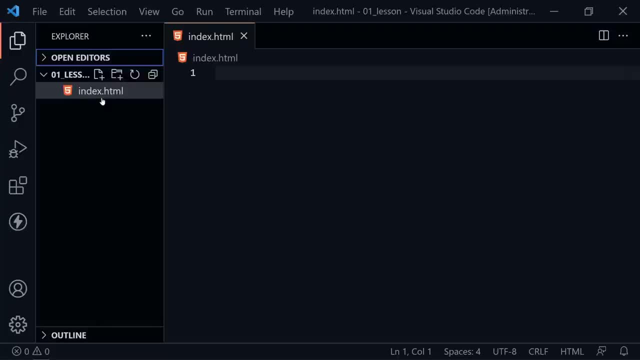 no spaces. You can use hyphens, dashes, and then end each file in html. Okay, we have an empty indexhtml file. Let's create our first HTML element And, as you might guess, the first HTML element we'll create is HTML. 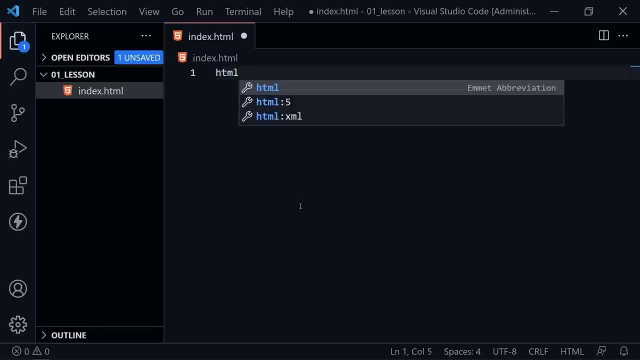 So if we type HTML all lowercase and press Tab in Visual Studio Code, it creates the tags And by tags that is often interchanged as a word with element. However, the element consists of the starting and ending tag and everything in between. 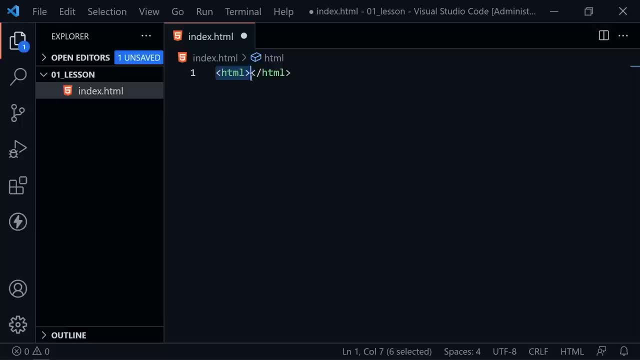 But here we might just be referring to the starting, also called the opening tag, or the ending, also called the closing tag. So we refer to HTML tags, But every page starts and ends with the HTML opening and closing tags And everything else on the page goes between those tags. 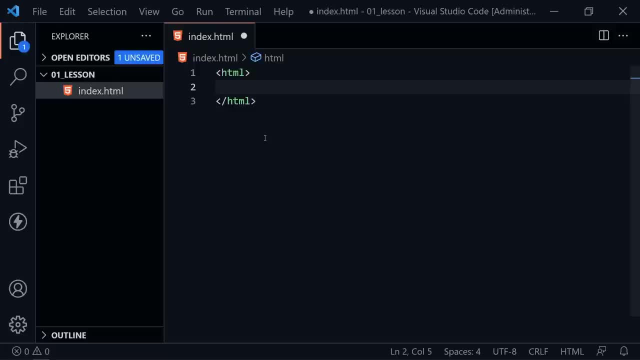 After creating our HTML element. HTML pages are a very important element. HTML pages are a very important element. HTML pages are a very important element. HTML pages have two main areas, And one area contains data that is not seen on the page but is considered to be metadata about the page. 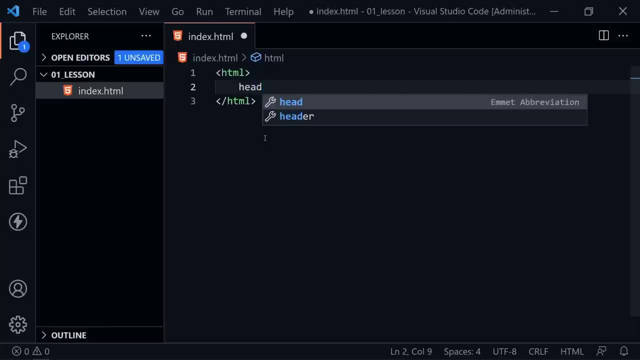 And that is the head area. So just type head- not header but head- and press Tab And now we have our head element And we will put metadata about the page inside this area. But the next area is the part of the page. 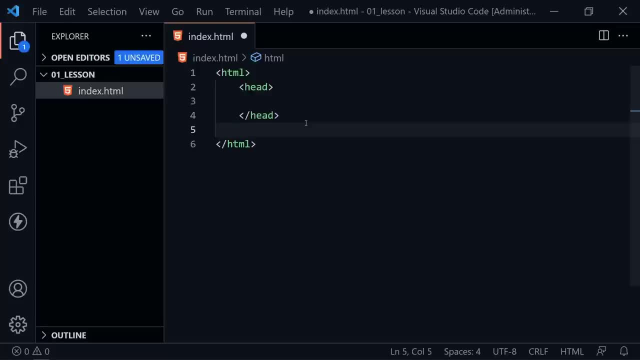 that everybody sees in the browser And that is held within the body element. So type body and press Tab. And now we have our two major sections of our page that are both inside of the HTML element. We have a head section and a body section. 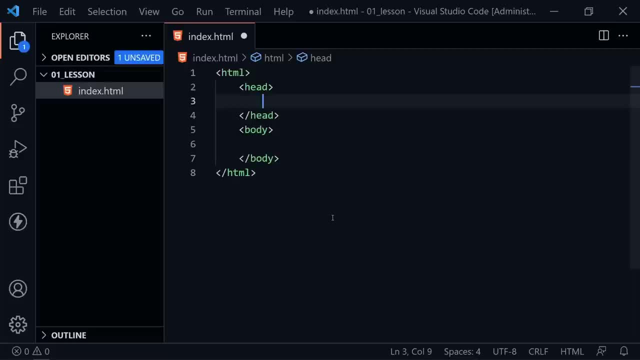 Now inside the head. we'll just put one piece of metadata today, And it really won't start with the word meta. We'll come back to that word in the future. We're going to create a title element and give our page a title. 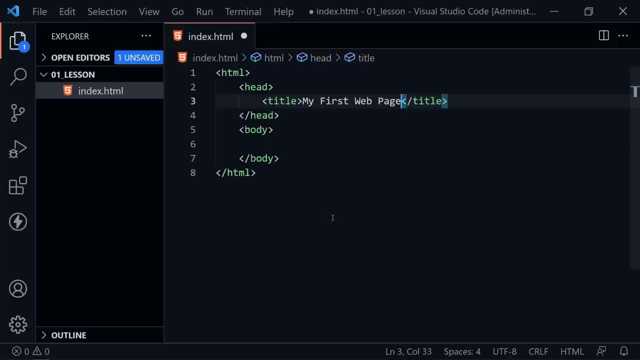 Let's just call this a title. Let's call this my first web page, And this will stay inside of the HTML document. Now I just pressed Control S, which saved the document. You otherwise would see a dot up here by the indexhtml. 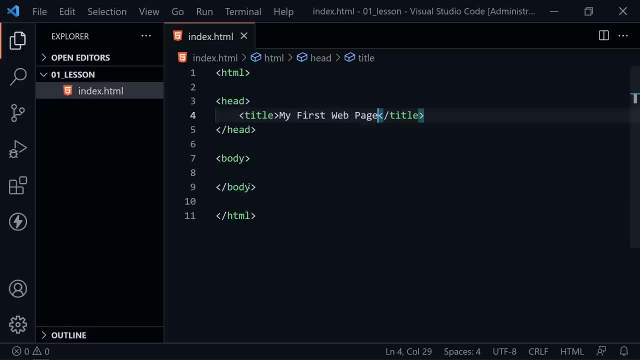 So I saved that and I am using an auto formatter. Visual Studio Code may or may not do that for you when you save your file. If you want that, you can go to the extension icon over here and search for a Prettier extension. 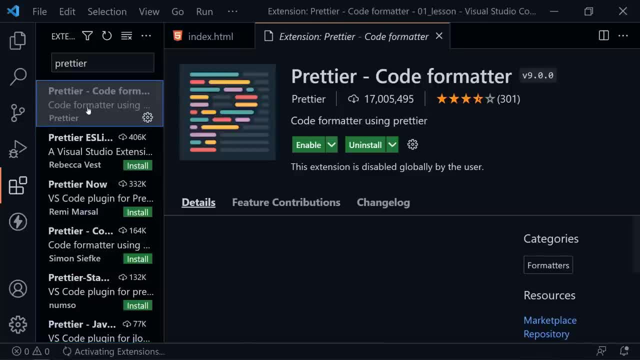 And I'm not sure if mine is enabled or I'm using something else right now. We'll have to check. Now mine is disabled, but I do recommend this one. Prettier is a code formatter that will auto format your code, But Visual Studio Code may do some of that as well. 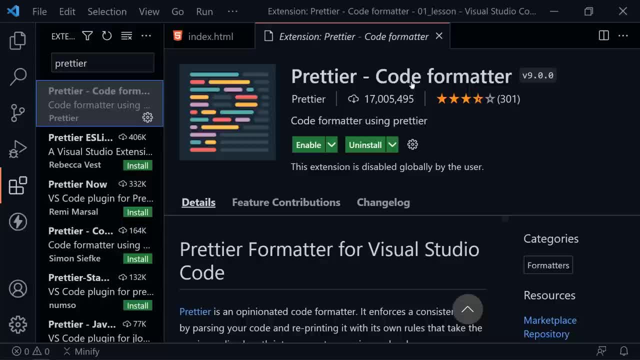 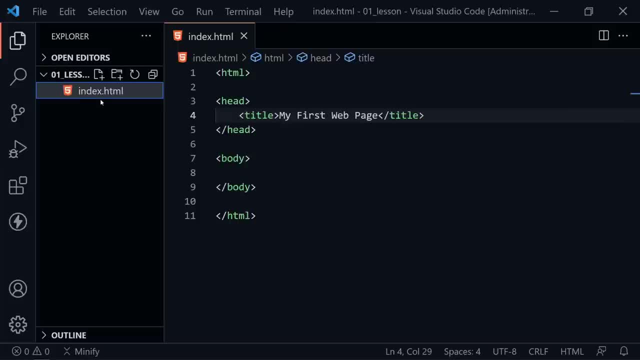 But if you want to use Prettier, go ahead and click Install and you can use that as well. So I'll close out that Prettier tab. go back to the File Explorer. here We see our indexhtml on the left instead of the extensions. 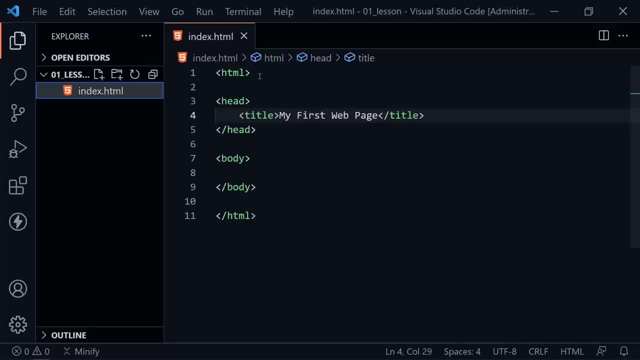 And now we can see our HTML is formatted in a very easy to read manner. We have our HTML element and then the head element, and then the body element And they're separated by spaces- Very easy to read- And we have a title inside of the head. 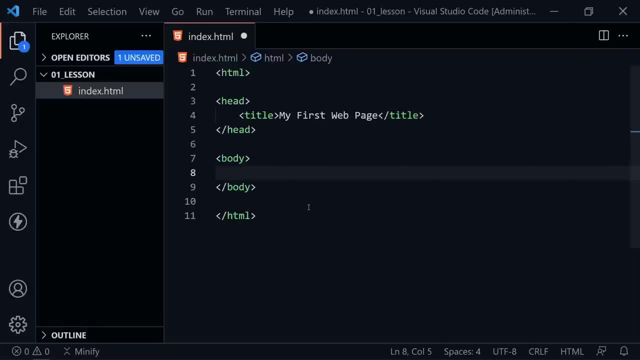 Again, the title will not be seen inside of the browser, in the body of the page, But I will show you very shortly where we do see it. Inside of the body element, though, let's put an H1 element, which stands for a heading. 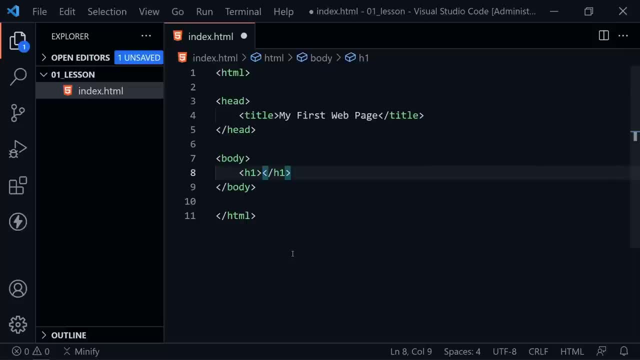 And it is the biggest heading we could put. You only put one H1 element per page And that should be saying what your page is about. It doesn't necessarily have to be the same text that is in the title, But here we're just going to put hello world. 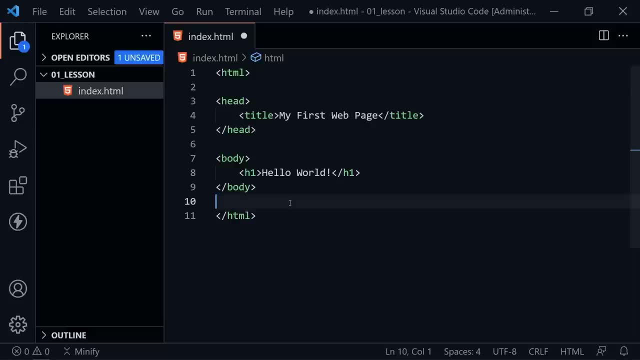 as is the tradition for creating your first file in any language you're learning. And so we have hello world On the page And we have my first web page in the head section. Let's add one more element in the body of the page. 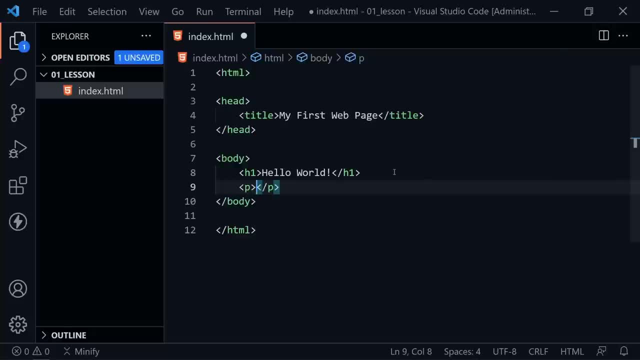 And this is a paragraph element that starts and ends just with the letter P. But notice, each of our tags, of course, start with this less than and then end with a greater than, And then the ending tag, you'll notice, has a slash. 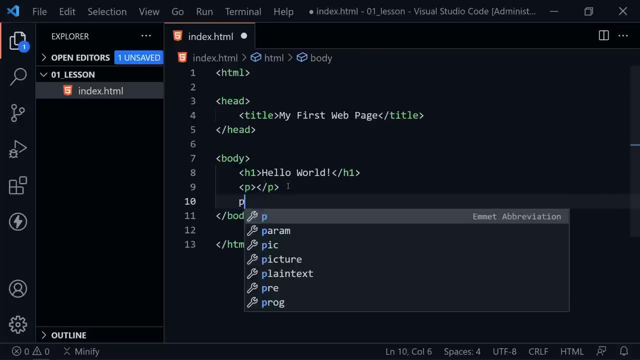 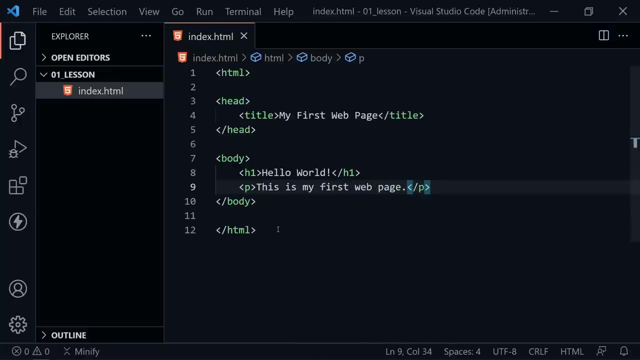 But all we have to do in Visual Studio Code is type P and press Tab And it creates both. So we're going to put some text inside of our paragraph And here we'll just put- this is my first web page with a period in the sentence and save. 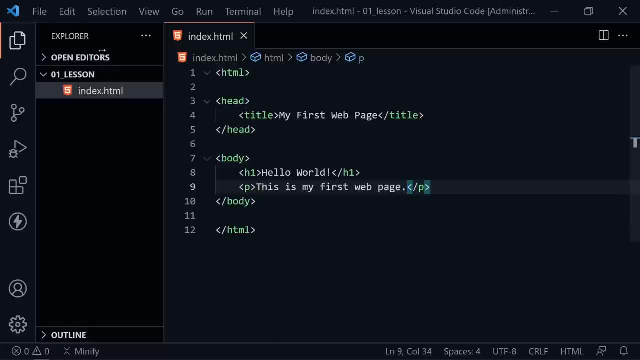 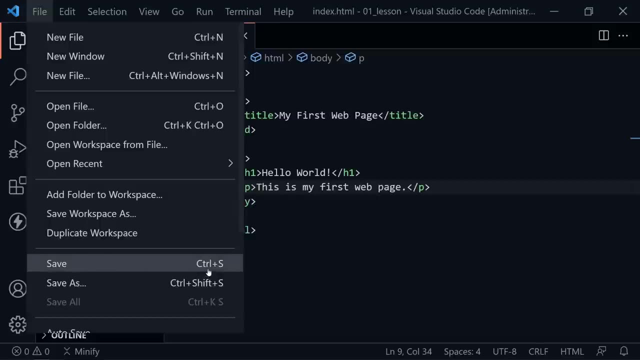 Once again I'm pressing Control S on the keyboard to save. You can go to the File menu And from there you can also choose Save. But you'll notice the shortcut is Control and the letter S. We're almost ready to view our web page. 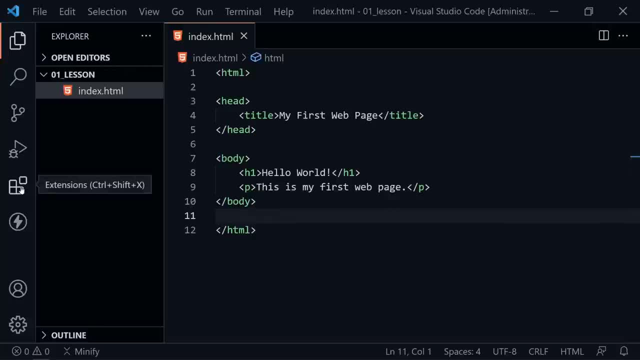 But before we do Remember the extensions we went to, I want to show you just a few, if you want your Visual Studio Code to look like mine. One thing to draw your attention to is when I created an indexhtml file, I have the little icon for HTML5 beside it. 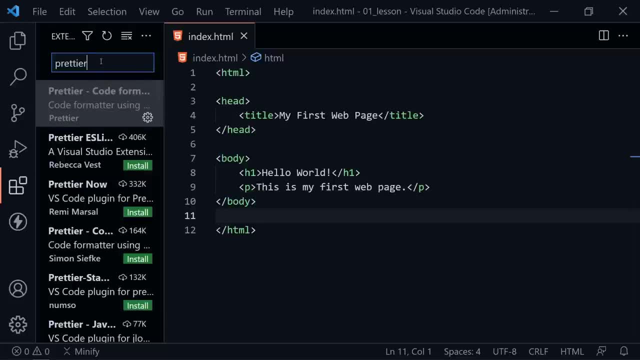 You may not have that, But if we click on Extensions and then we can delete Prettier, that I searched for before- type VS Code: dash icons, there you'll find the extension that will add that to your VS Code as well, So you can install. 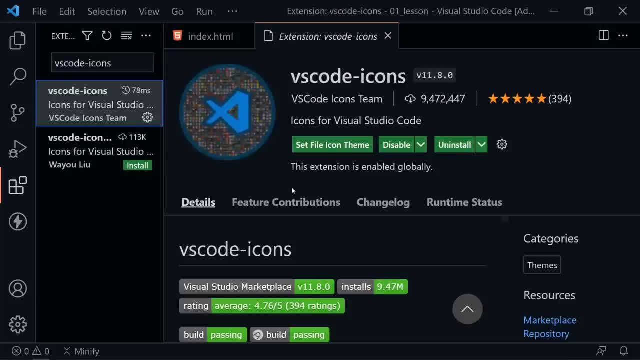 I already have it installed. So mine says Uninstall And that will add icons as you create files And it might add the icon up here as well in the tab. And that's how you see the icon here beside my indexhtml in the File Explorer. 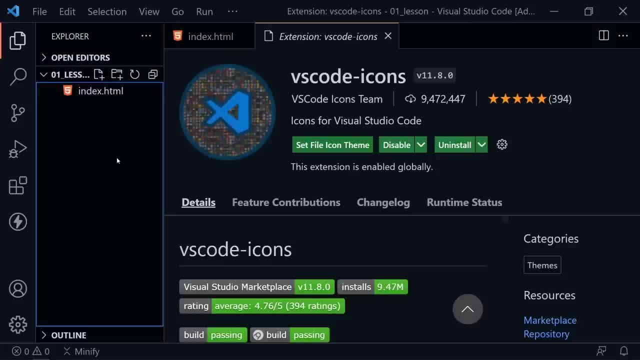 So visually it helps you see what type of file you're working with quickly, without even reading everything. After that extension, let's go ahead and click the Extensions icon again And then search for the file. Let's go below. So it's going to protect this. 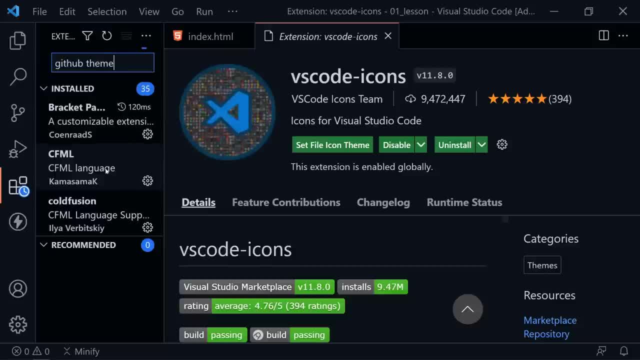 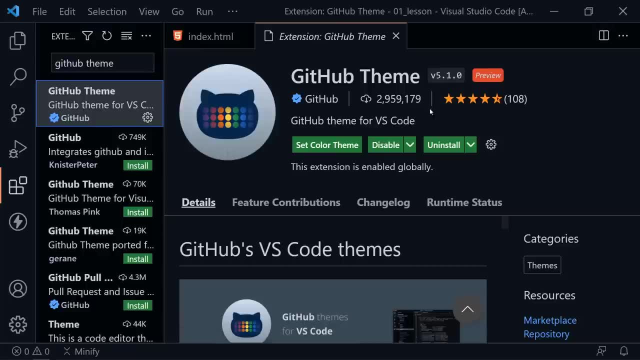 And then I'm going to go to Export And I'm going to click the Export for GitHub theme. I am using a specific theme which I prefer- dark mode in everything that I do. So I am using the GitHub theme extension and it has light and dark themes. 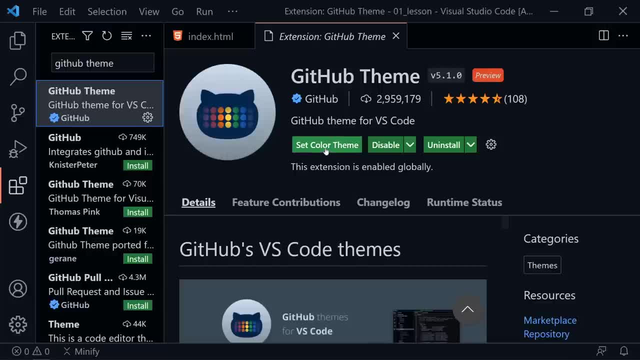 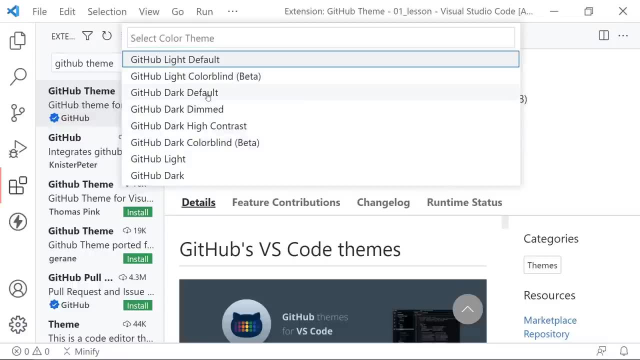 I believe I'm using the default dark theme. This might be bright for a second, but I'll click set color theme And, yes, it switched back to light. but I choose GitHub dark default And then yours will look much like mine. 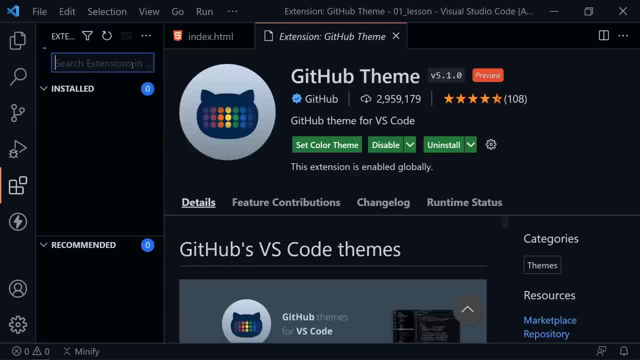 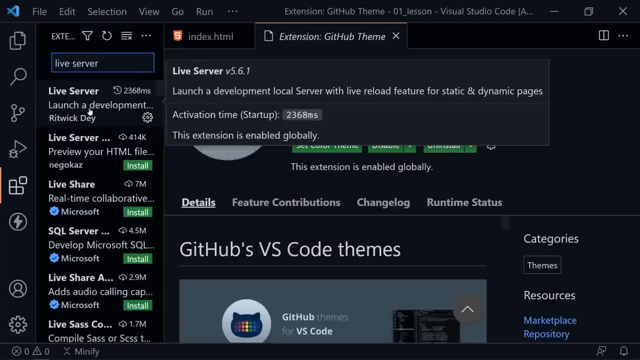 Now, these previous extensions have been optional, but one that I say is a must for you to install is called Live Server. So let's pull up Live Server by Rytwick Day. I'll click on that And you want to install Live Server? 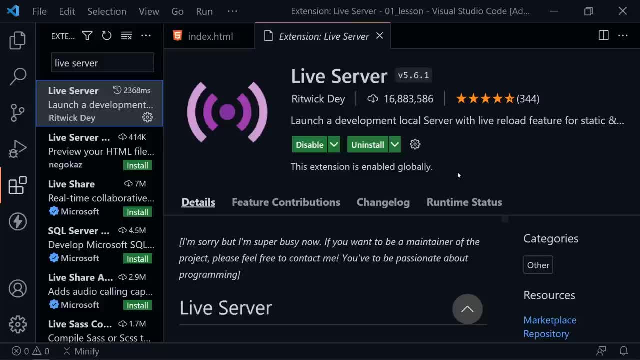 because it's going to help us view our webpages. So go ahead and install Live Server And after you have it installed, we'll go ahead and take a look at the webpage we've created. Okay, with that installed, I'm going to close that tab. 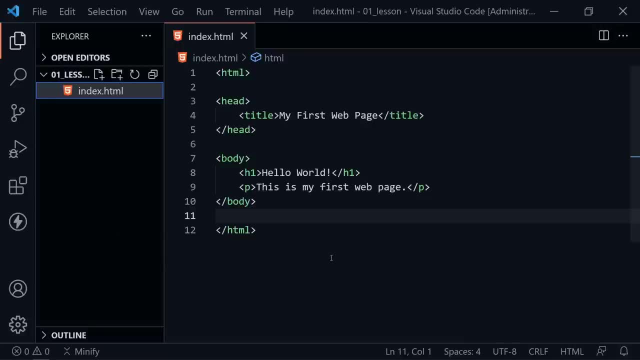 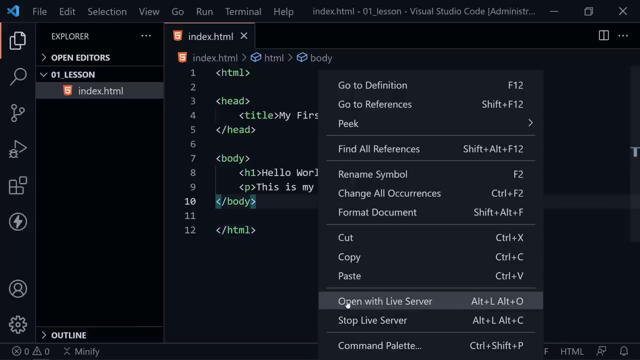 I'll come back to the file explorer here to show the file. And now, if you have Live Server installed, you should be able to right click and open with Live Server. And once we choose open with Live Server, it opens our browser and we can see our webpage. 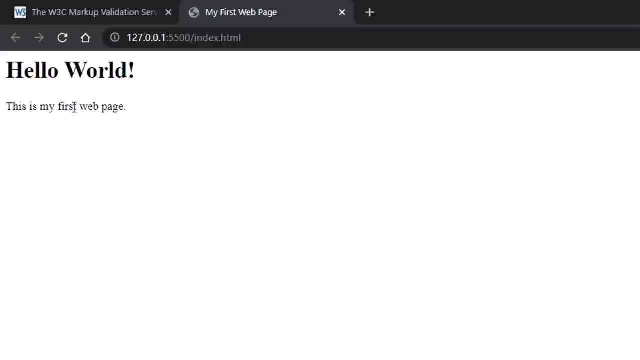 It says hello world, this is my first webpage. In addition, in the tab at the top it says my first webpage. So that is where the title goes, the very top of the browser, in the tab. Now this is very bright. 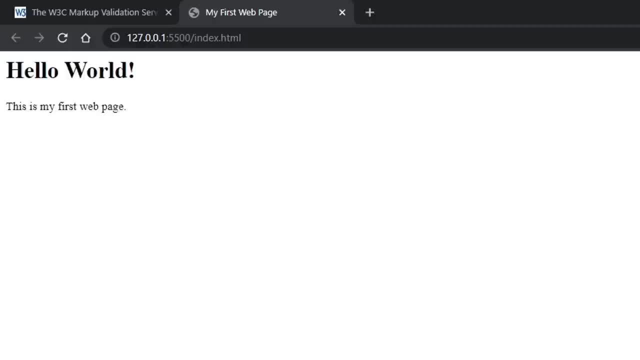 and I have mentioned that I prefer dark mode. So let's go back to Visual Studio Code and I'm just going to paste in some quick styling that is actually CSS. Once again, this is optional, but it will save my eyes and possibly yours. 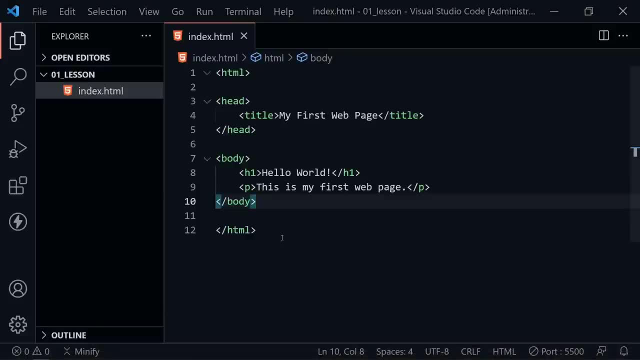 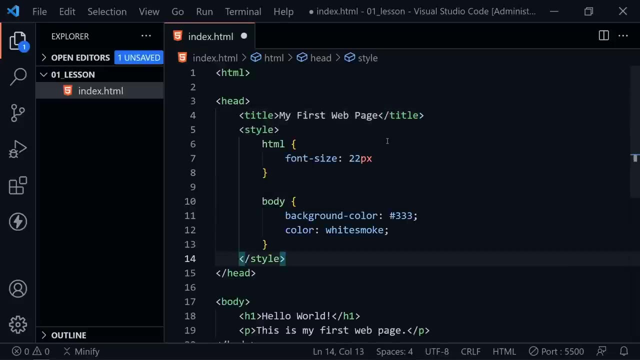 as we work through this tutorial. So once we're back in Visual Studio Code, just underneath the title in the head section, I'm going to paste this in. I'll quickly describe it. I put in a style element And that allows me to put in some quick CSS. 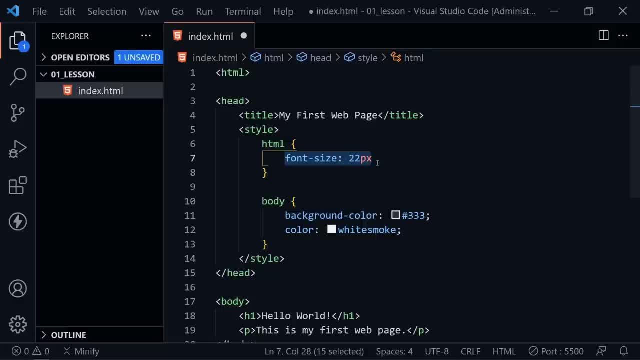 And I changed the font size to make it just a little larger, And then I changed the background color to a dark color And I changed the font color to an off-white color called white smoke, And that's all I did. We're not really learning CSS here. 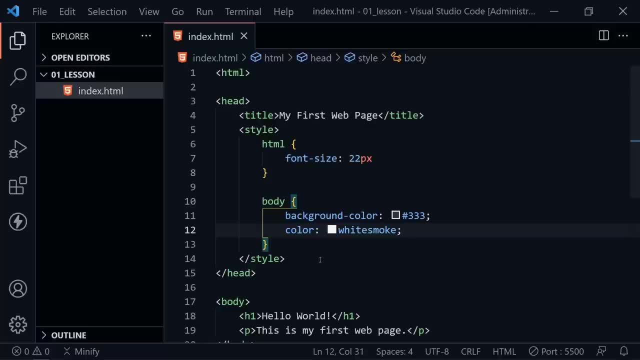 but this will save our eyes going forward. if you want to make these changes, If you prefer the white with dark text, that is fine too, But now that I've saved this, the beauty of Live Server is that it automatically reloads our page for us in the browser. 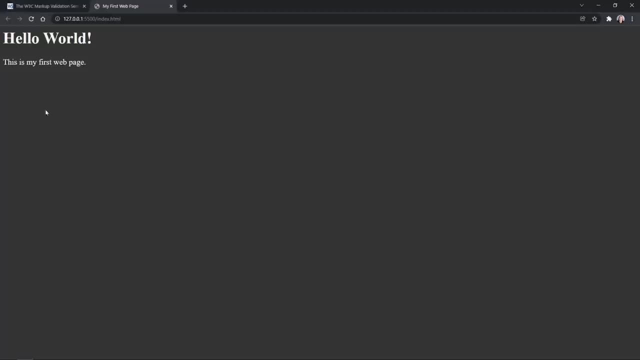 So let's go back to the browser and look at our update, And now you can see our web page is in dark mode And we have a little bit larger text here as well. It did not change our title from the head, because that just goes into the tab of the browser. 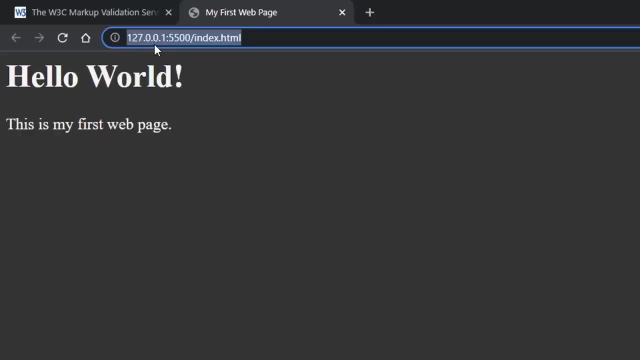 Also notice the address. This is an IP address, And then we have a colon And this is a port number. But this is on your own computer. This is not on mine. I can't go onto the web and see your page that we just created. 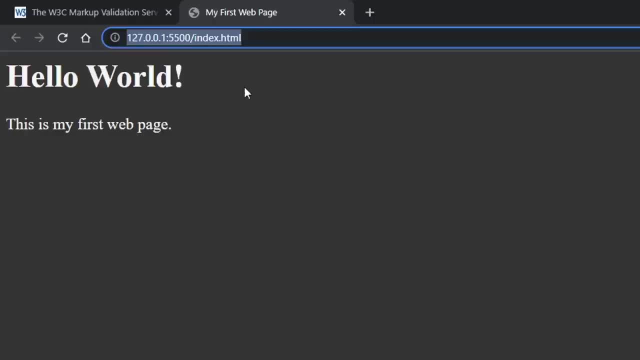 We haven't loaded it to the web, It is just running on your computer. But this is the way to view web pages as we create them, which creates your own local server. It's what's called a dev environment, And that is preferred. 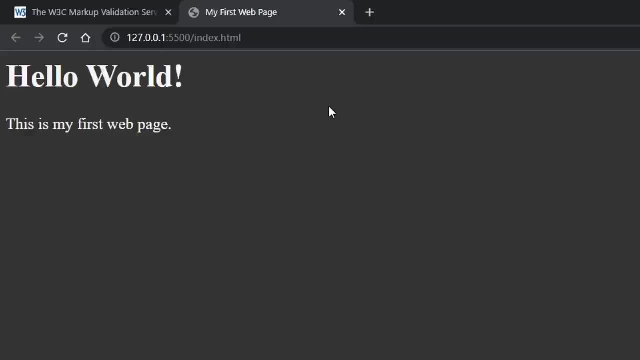 What you don't want to do in Chrome is try to open a file like you would in Word or some other document browser or even Visual Studio Code. how we open files. That's not how you want to view a web page. You want to use a development server. 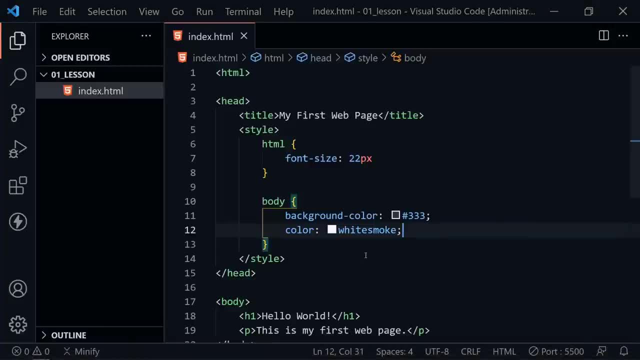 And that's what we're doing with Live Server in Visual Studio Code. Now, if you ever want to stop the server down here in the bottom you can see the port number 5500.. And it says click to close server. So I can just click that. 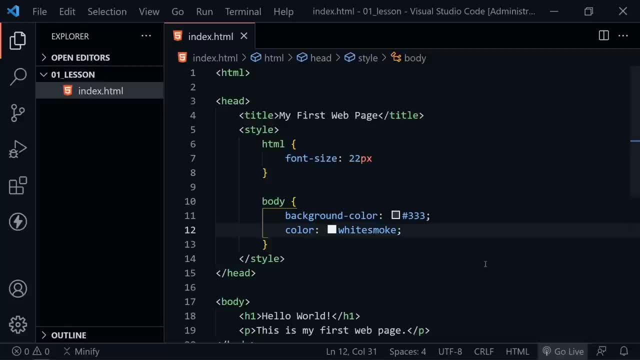 It says disposing, And now we have a Go Live button which you can also use. You can also right click on your document and choose Stop or Open with Live Server. Now we would once again, Since we stopped, that we would need. 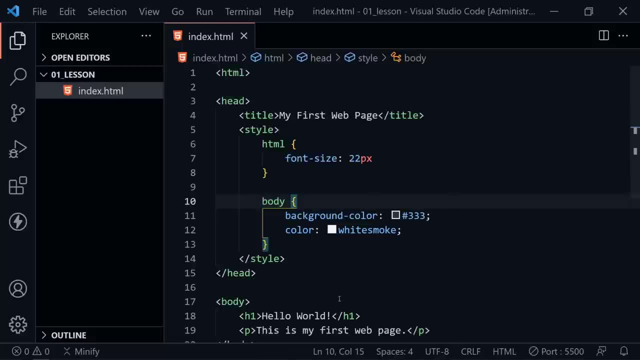 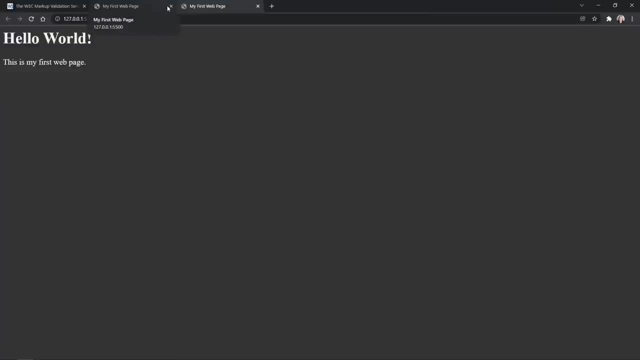 to open with Live Server, to have a live web page that responds to changes we make, And notice how it opened a new tab here instead of our old tab, Our old tab. the server for that page closed, So we close that out And now we're using this one because this: 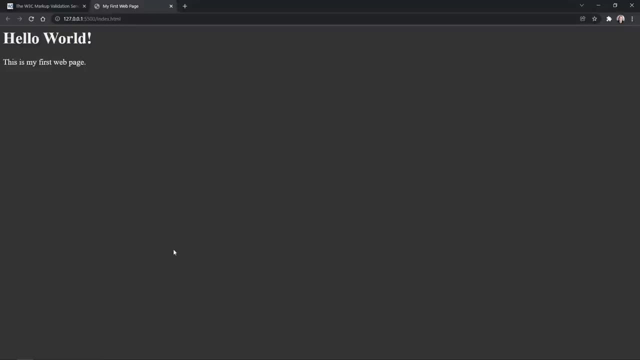 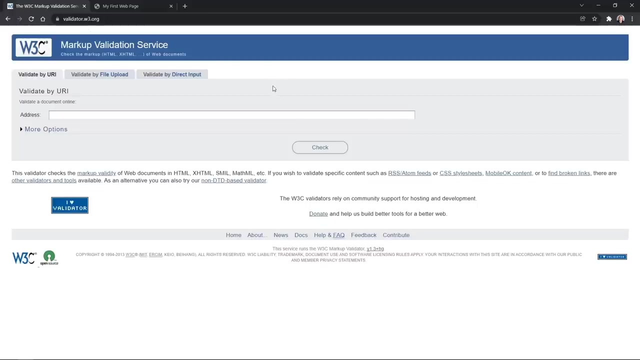 is going to show our most recent changes. Now, after we've created a web page, how do we know if we have errors or not? Well, that's where a validation service comes into play, And this is the W3C Markup Validation Service. 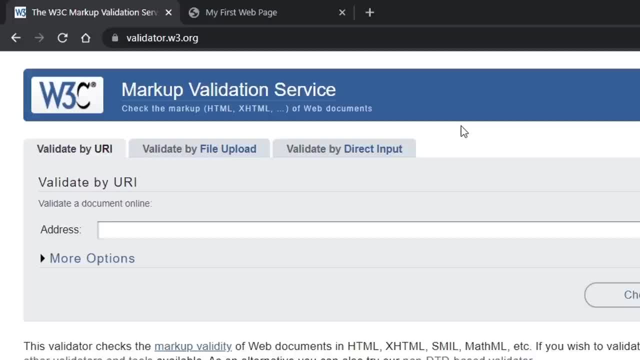 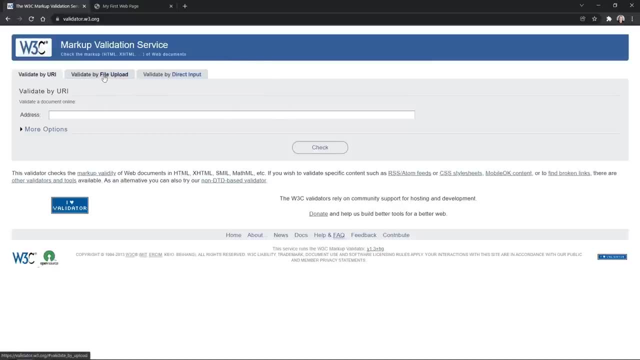 W3C stands for the World Wide Web Consortium. that really makes the standards for the web overall. What we want to do to check our page is click File Upload Because, remember, our web page is really not on the web, It's just on our computer. 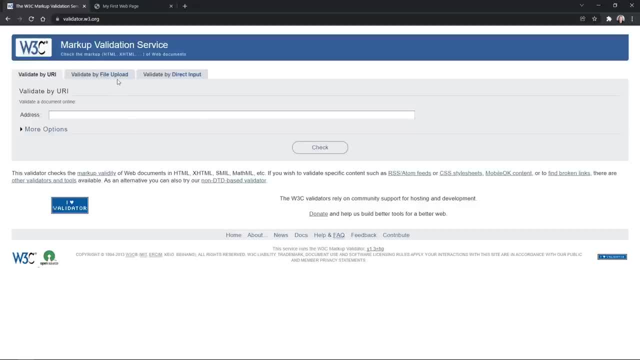 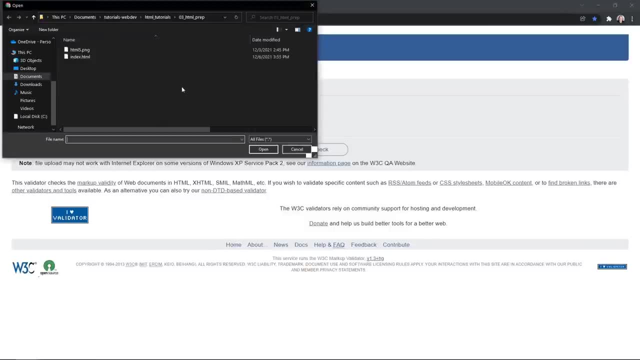 Your web page is on your computer and mine is on my computer. So let's click File Upload And from here we're going to choose the file that we want to upload to our web page. So if we click File Upload, we're. 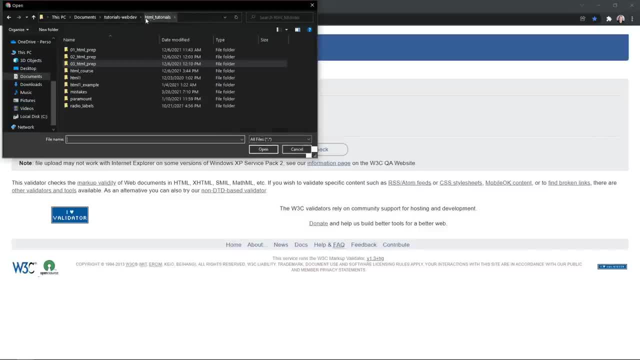 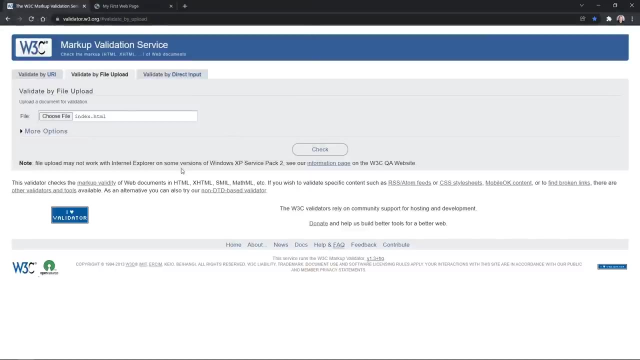 going to see. we've got our web page here. It's on our computer And we get a browse window And now I'm going to click HTML Tutorials And then I have an HTML course folder and then the zero lesson one folder that we just created. 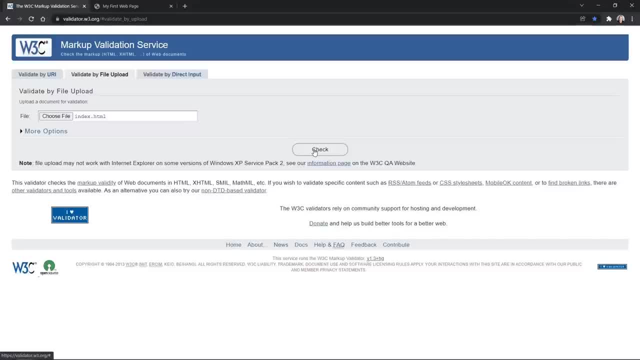 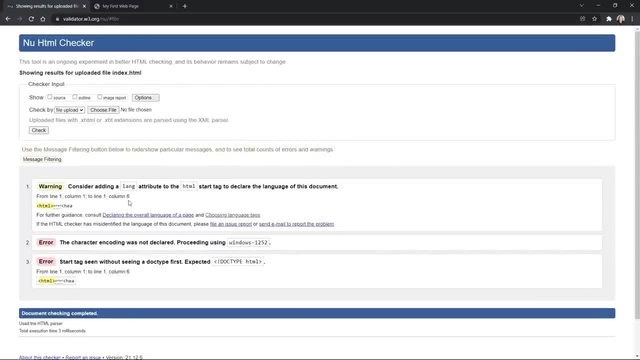 And there is the indexhtml file we've been working with. So I'll click Open And now that it's here, we can click Check And we're going to get some errors and we'll go over those Now that we have checked our page. 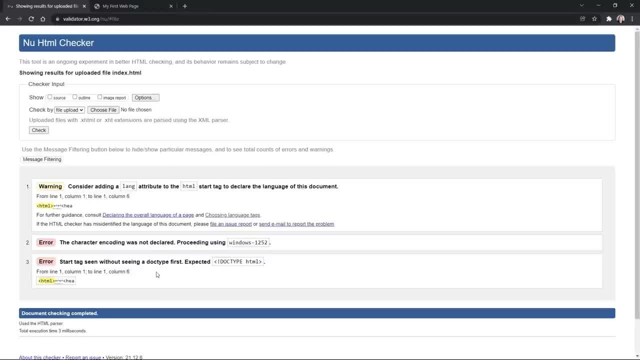 we have got a warning and a couple of errors, So there are things we need to fix in our HTML file. Let's address these in order with. the first warning says: consider adding a lang attribute to the HTML start tag to declare the language of the document. 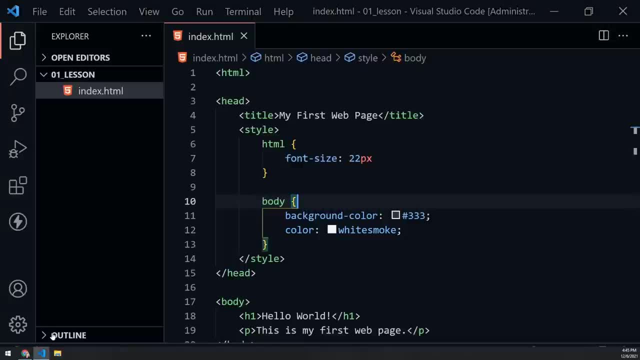 So that is something we should do. Now we're going to go to the HTML tag and we can add what is called an attribute, And this is the lang attribute, And I'm going to set it equal to EN, which is the abbreviation for English in general. 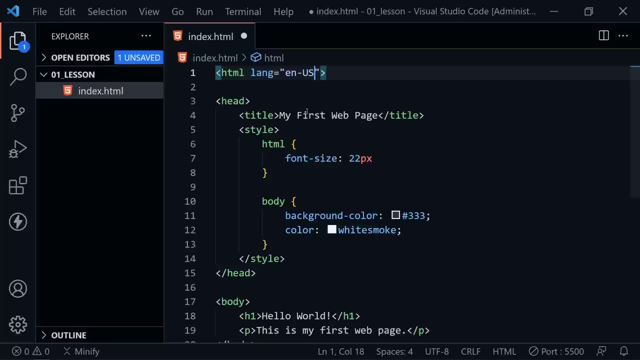 You can supply a dialect like this: dash US or I believe the other would be GB, but I don't usually do that, So I'm just putting EN for English. You might have another language you prefer to put there and you can find a list of those. 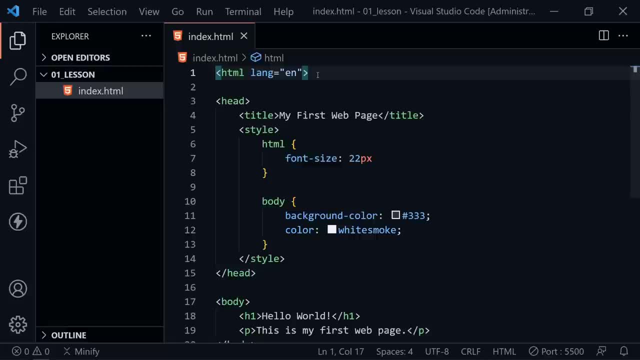 at the MDN network as well, And that's the page where we were looking for the definition of HTML at the beginning of this tutorial. So I will link to MDN, the Mozilla Developer Network, in the description, Now that we've added the language attribute. 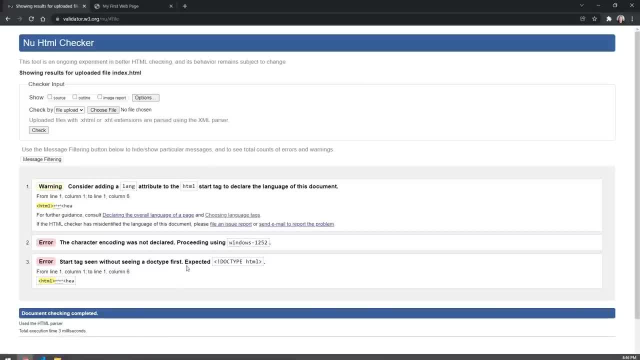 let's go look at the other errors we had and see what else we need to fix. It says the character encoding was not declared, So we also need to handle that. Let's go back to Visual Studio Code. And now inside the head. 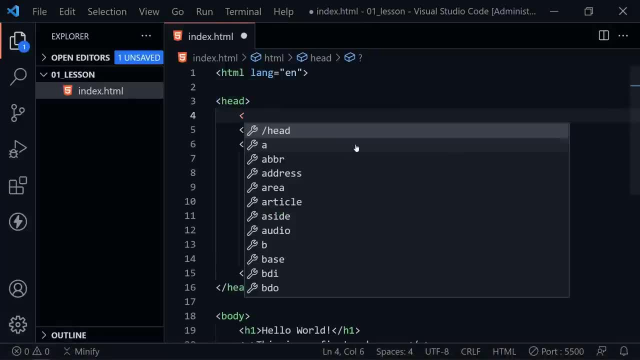 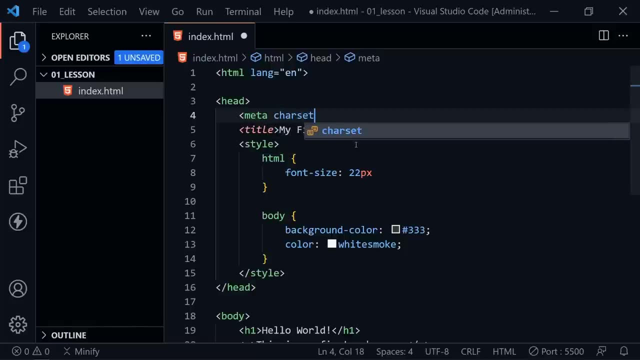 there is an element called meta. Earlier I said, the head stores metadata. Let me keep it all lowercase here. And here we can set what is called the character set attribute inside of a meta element, And from here I'll put UTF-8,. 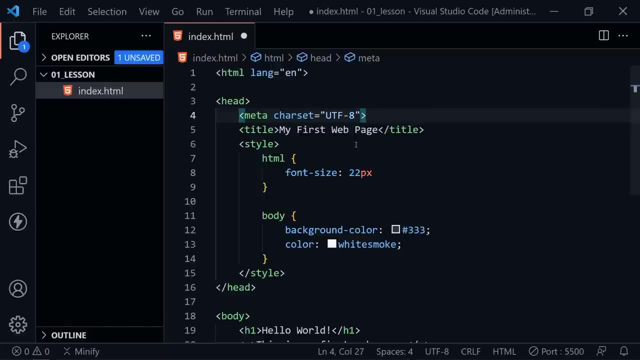 which is the standard for all web pages that I have worked on. There are other character sets, but this is the typical value you would see in there, So I'm going to save this And in the future we'll cover more meta tag values. 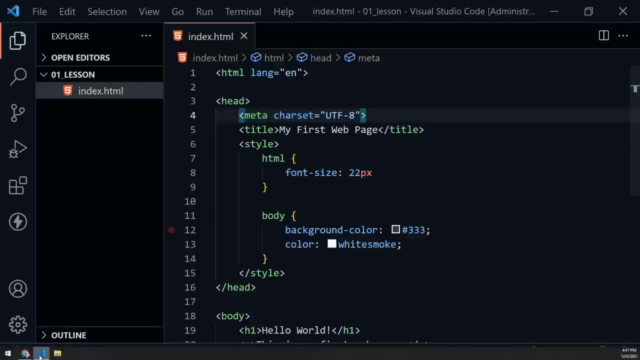 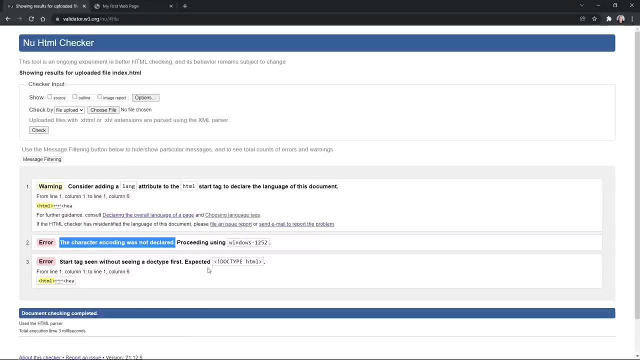 that we'll have inside of the head. Now let's go back and look at that last error that we got from the validation service And that said start tag seen without seeing a doc type first Expected, and it shows you exactly what it wants. 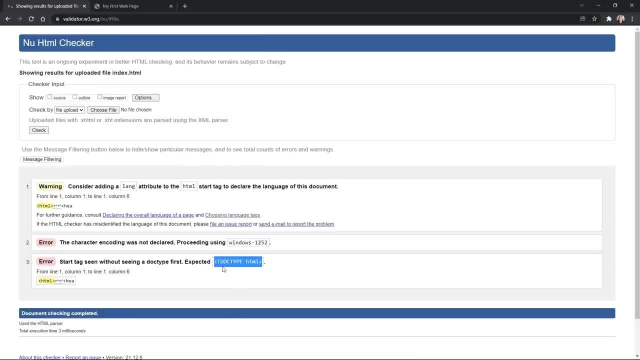 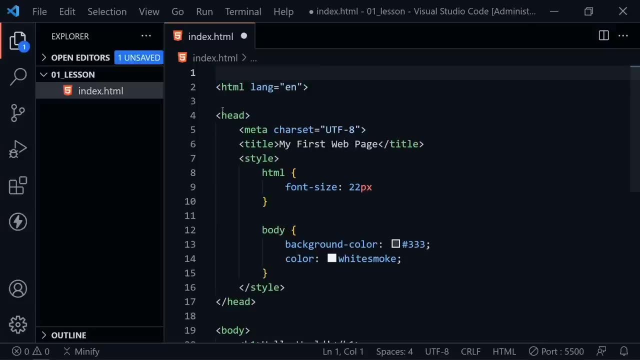 Doc type: HTML. And that is a document type declaration that should be on the very first line of your page. So let's go back to our HTML file, Go to the very top and we'll press return And we'll paste in exactly what they had there. 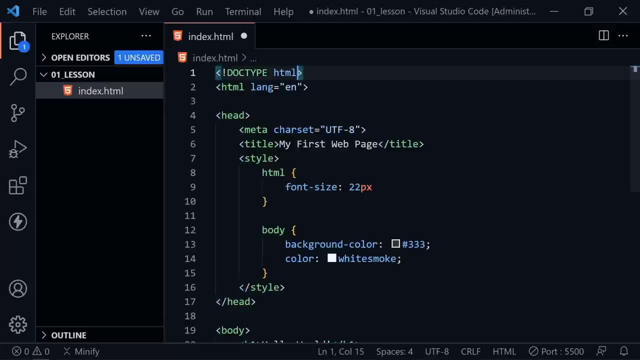 So you see, once again it starts with the less than and the greater than symbol. But this is not really an HTML element or tag. This is just a doc type declaration that you should have in every HTML file at the very beginning. So now I'll put that in and save as well. 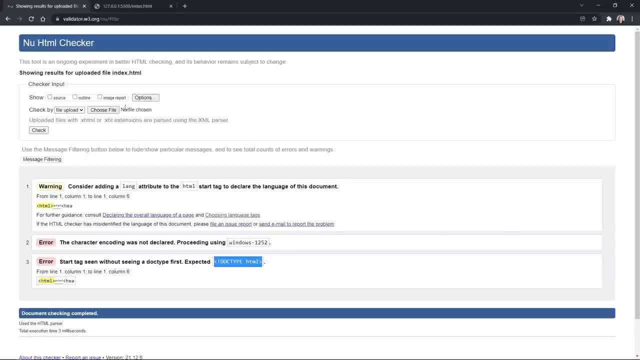 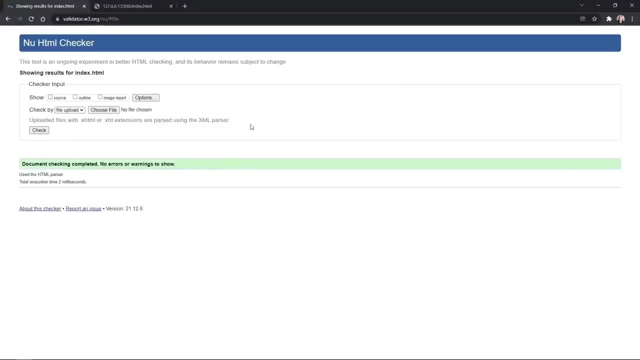 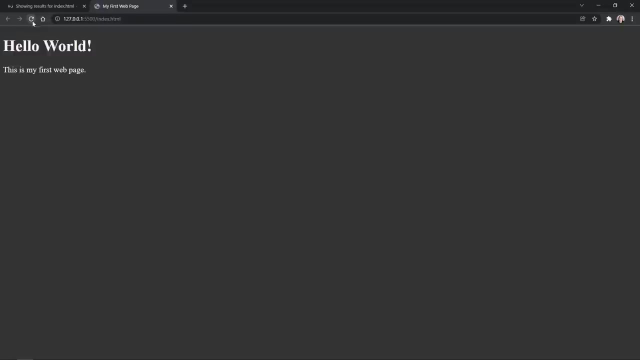 Let's look at the validator file- All right, first, and let's choose the file again. and now i've selected the indexhtml to upload with our changes and we'll click check. document checking completed: no errors or warnings. so our document is just fine. let's go to the tab with our page and let's reload the page. and once we reloaded, 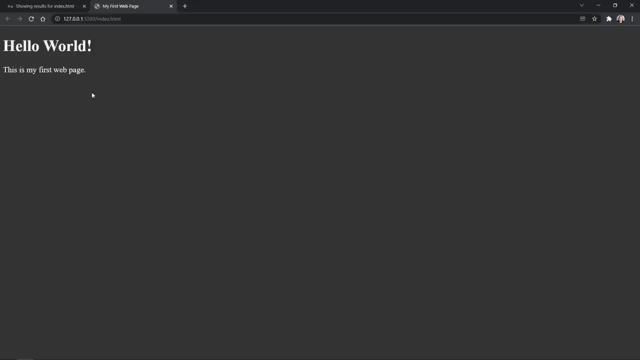 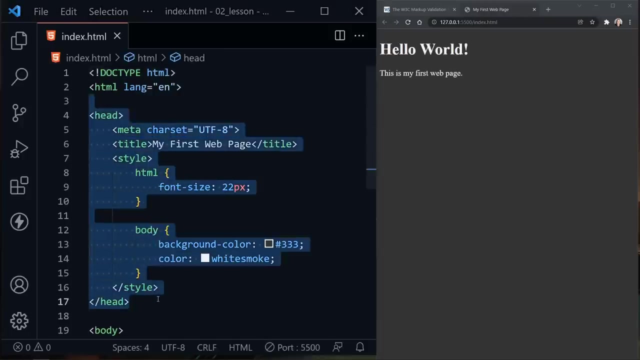 everything looked great. so we've got hello world. this is my first web page and we still have my first web page in the tab at the top for the title and we have passed all validation checks. let's move on to what else might go inside of our head element and remember everything inside of the 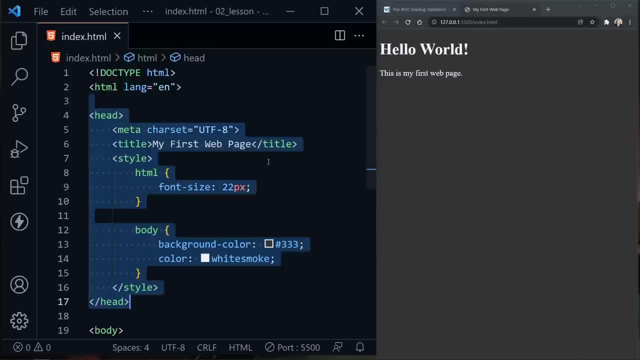 head element is not seen on the web page and, with that said, i've dragged the visual studio code window to a little smaller size on the left and chrome to a little smaller size on the right, but i'm just going to expand visual studio code window to a little smaller size on the right. 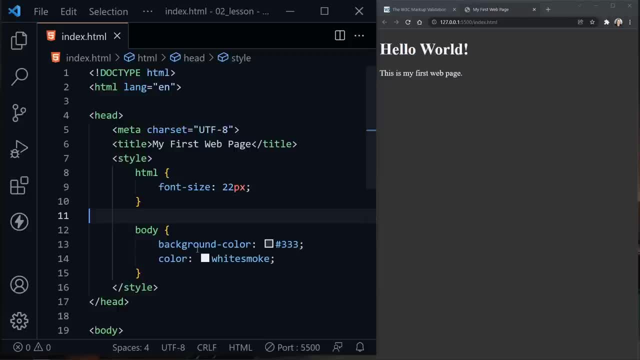 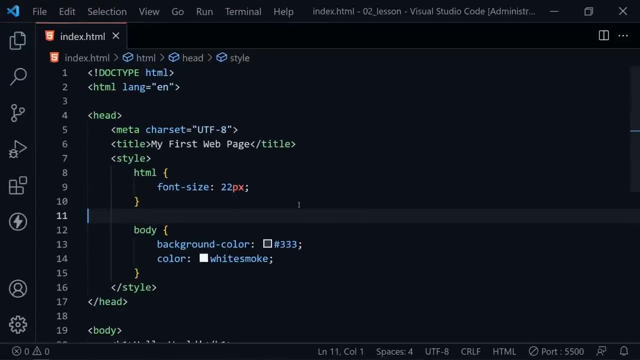 because anything we change inside of the head element will not be seen on the web page anyway. so i'll click the expand button and we'll just see our code now. i had mentioned that we could store more metadata inside of the head element, and that is definitely some of what we see. so 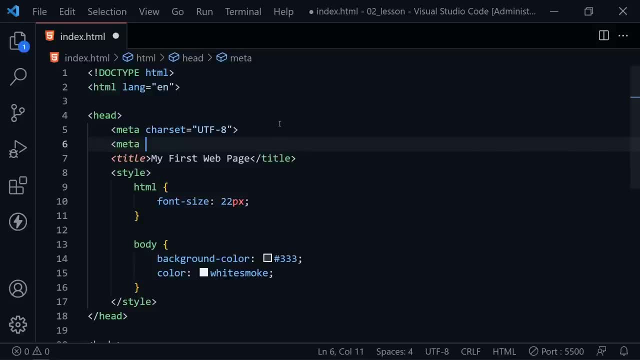 let's add a couple of typical meta tags that have metadata that you would commonly see, the first being for the author of the page. so we'll say name: the attribute name is equal to author, because that's what type of meta tag this will be, and then we'll have a content. 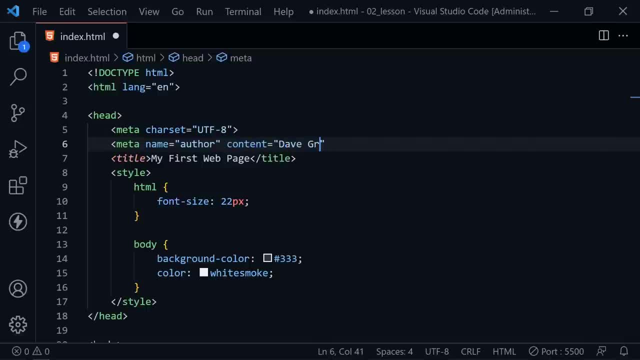 attribute and this is where you can put your name. i'll put my name for now, since i'm the author of the page, and then let's add another meta tag and let's give it a name as well, and here we'll put a description. this will describe the web page in a little bit more detail than possibly the title. 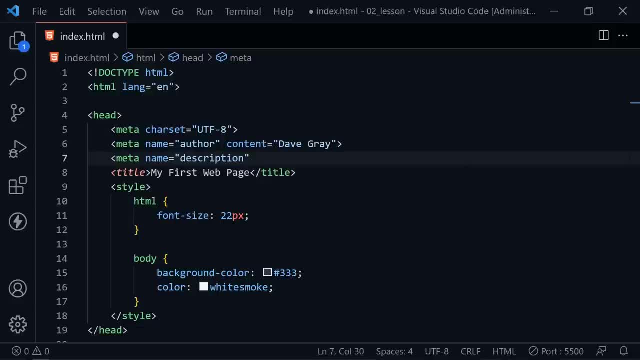 would. so here we can put more of a sentence, and once again we need the content attribute to do that. let's say, this page contains all the things i am learning how- if i could spell how to- and it looks like i'm extending the page. so in visual studio code i'm going to press alt z in windows to make. 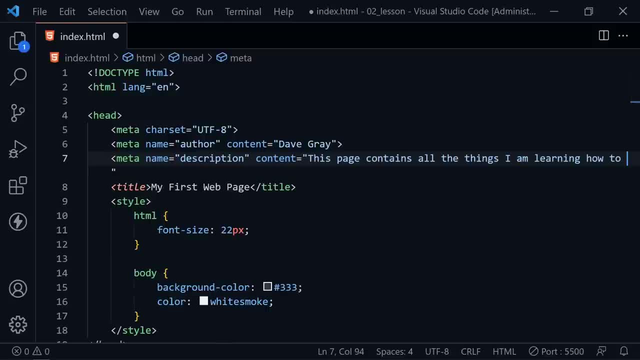 sure the text continues to wrap, and then i'll say all the things i am or i am learning how to create as i learn html. there we go now. after that, of course, you still need to close the meta tag and ctrl s to save. and again i got the words to wrap. let's go to the view menu. if you scroll all, 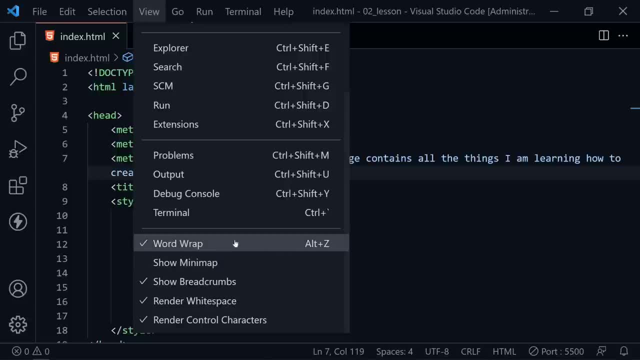 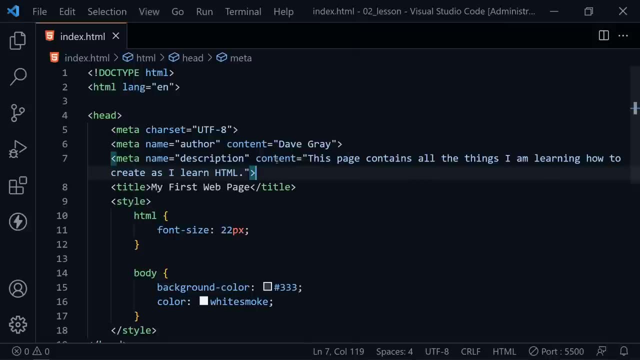 the way down. you can see word wrap is alt z. it may be something different if you're on mac or linux, so you might want to check the view menu under word wrap if you want your words to wrap and not just extend forever to the right here. now we've added more description about our page now. 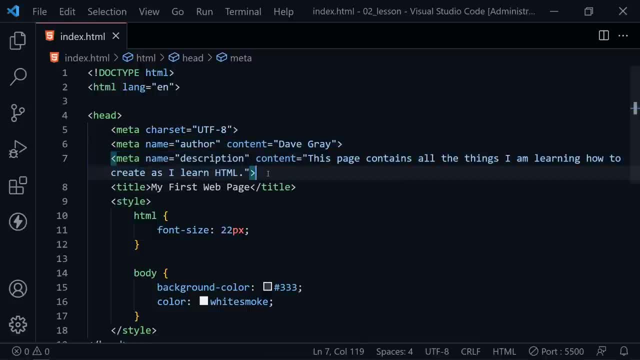 this is the page that we're going to be using for our page, so we're going to go ahead and add a link element to our page and this information could be picked up in a search engine or some other service that wants to learn more about our web page. however, let's go ahead and put something in. 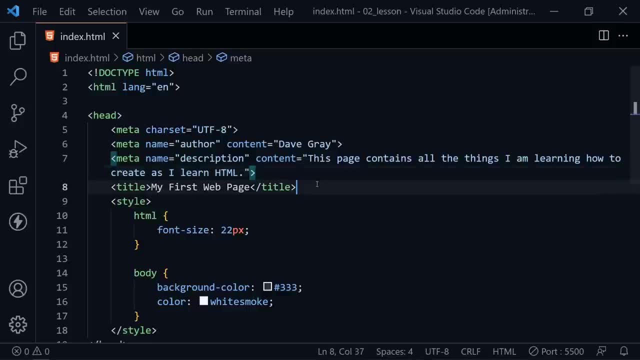 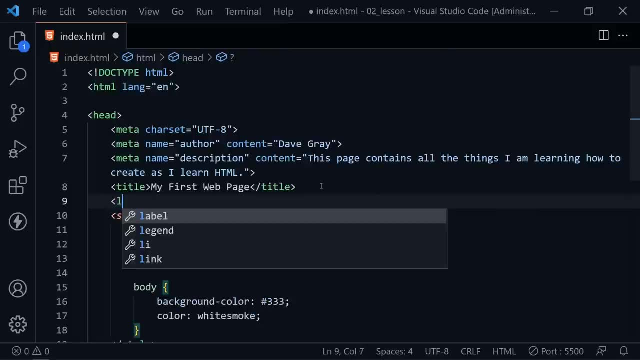 the head, where we will notice the change when we go back to the browser, and that is to add what is called a fav icon, and we can do that with a link element- let me use lowercase once again- and inside of the link element we'll have several attributes. one is the rel, which stands for relate or relation. 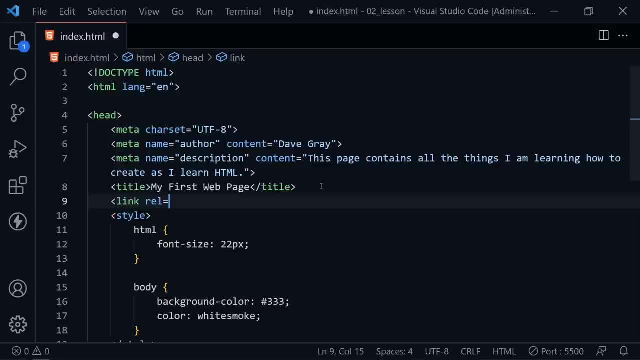 how does this relate to the web page, and here we're going to provide an icon. after that, we need an href. this refers back to html that stands for hypertext. this is a hypertext reference, so we're referencing a resource, and here we're going to reference a file that i have now put inside of. 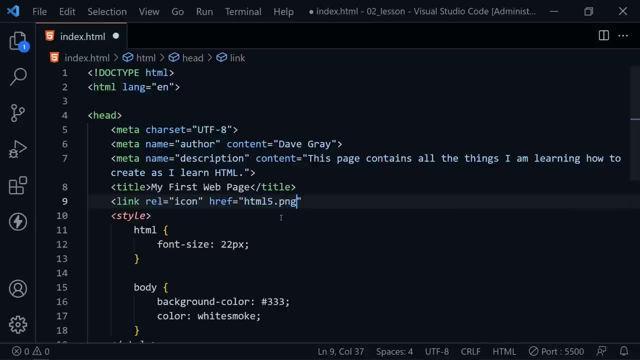 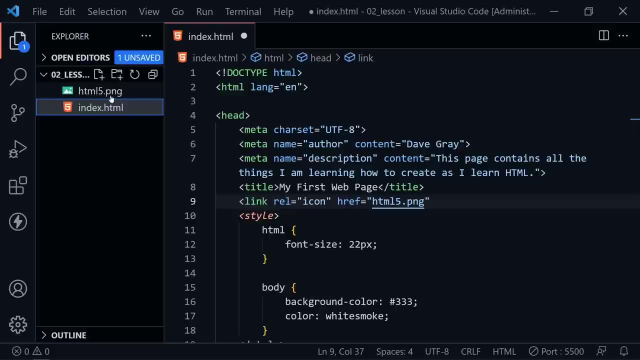 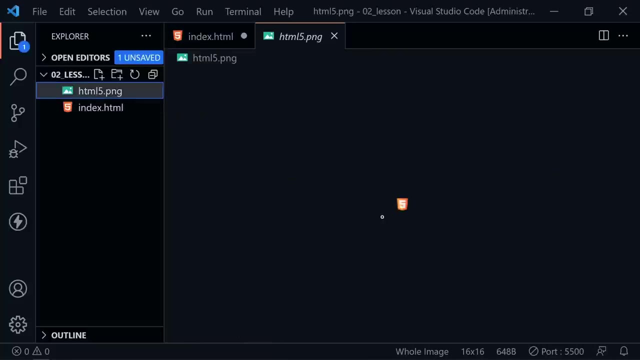 our folder that is called html5.png, and if i click the file explorer over here, you can see i've now added an image file that's a dot png file, html5.png, and you can download this image from the resources and you can see it's a small little icon for the html5 logo. so i'll close. 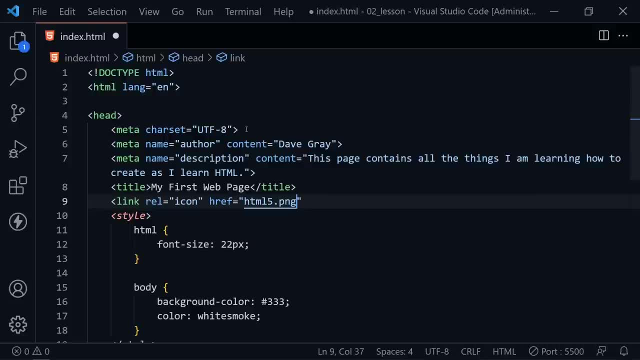 that i'm going to click the file browser to have that disappear again. so we see this. now we have one more attribute to add, and that is the type: what type of resource is this? and here we'll say image x icon? and now we can save this and i'm going to go ahead and minimize the code window. and now, if we 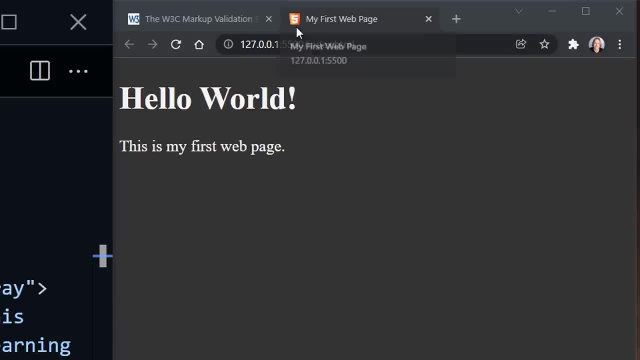 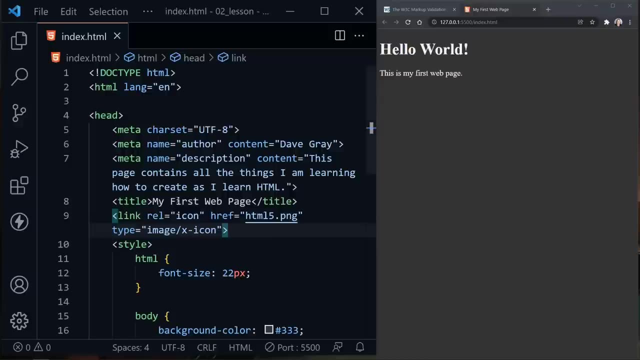 look at our web page in the browser notice we have an icon up here. my first web page now has our little fav icon beside the title and that's what we added here in the head by adding the fav icon with a link element. now we won't add any more here today, but this is the same area where we would. 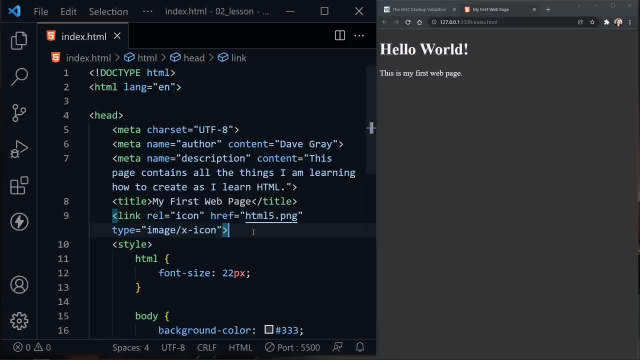 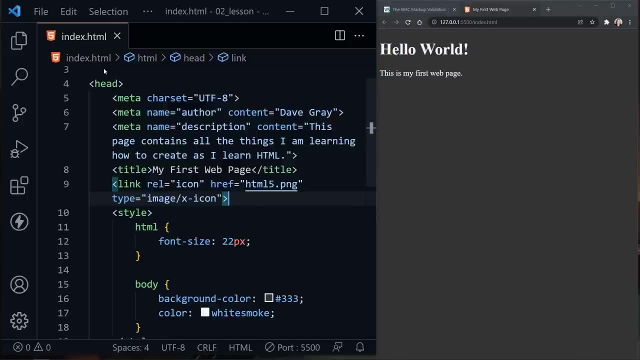 link to css files or even the code itself, and we'll look at a review and see if this is files and even JavaScript files and other resources that we pull in from the web. So the head is a very important part of the page, even though we don't see the content of the head. 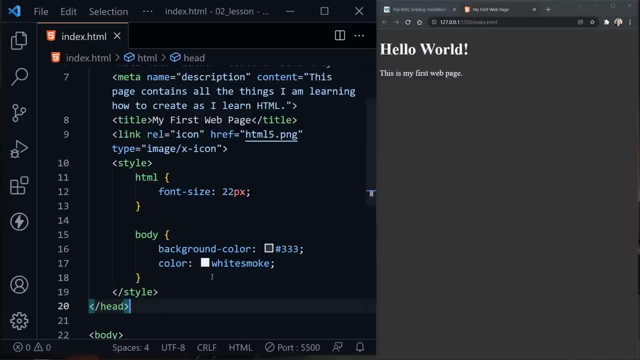 inside the body of the page And I said we wouldn't link to anything else here today. But since we do have this default CSS to make our page a dark mode, if you added this- and once again, this was optional- if you prefer the white page with dark text, you didn't need to add this. 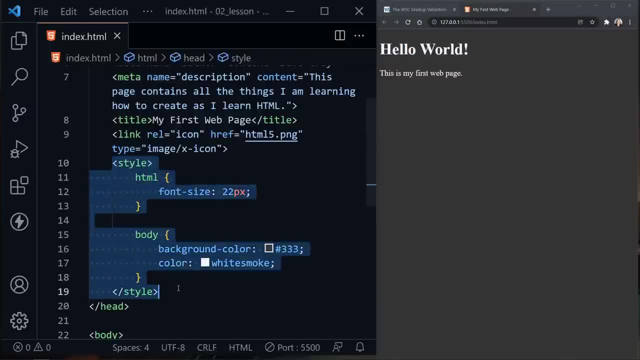 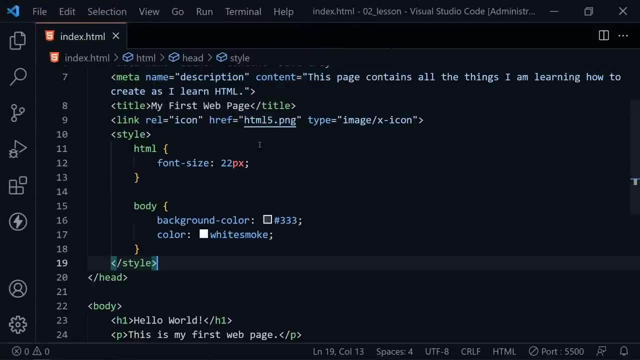 And we had this style element here to hold the CSS in the head, But that's not usually where you would find it for a page, So let's go ahead and do that. I'll expand Visual Studio Code again. click the File Explorer And over here inside the file tree I want to create a new file. 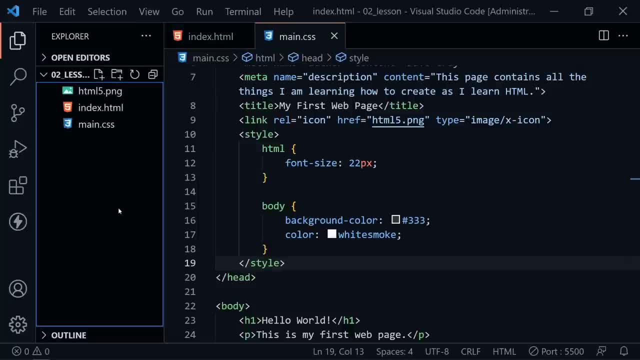 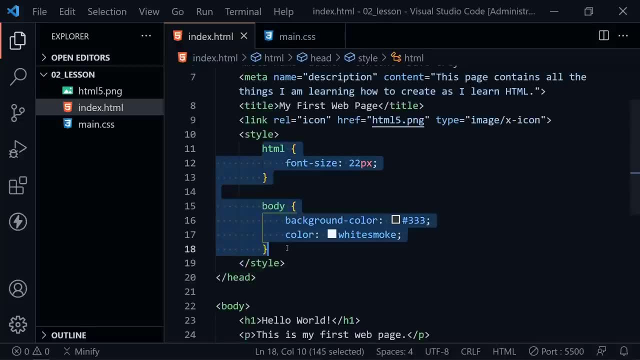 I'm going to call this maincss And I have an empty CSS file. All we need to do now is go back to the index, select the CSS that we put here for the HTML, the body, not the style tags. just select the CSS. that's between the style tags I'm going to press. 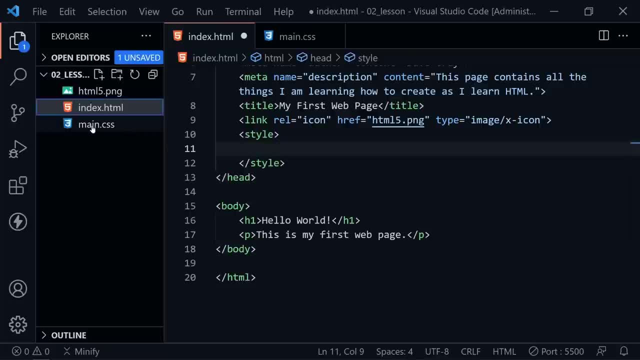 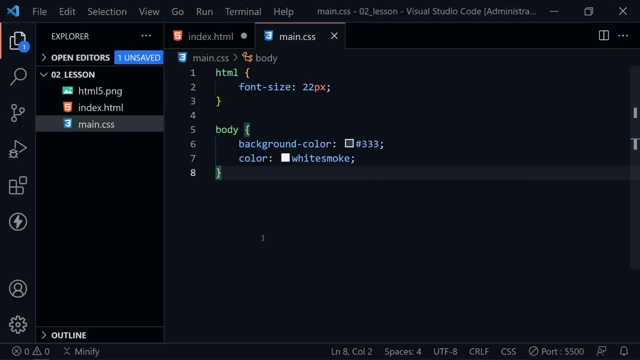 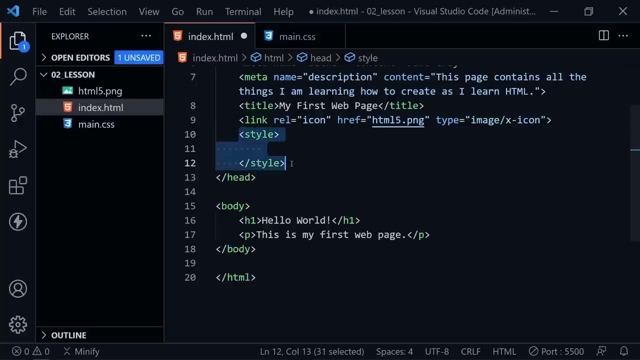 Ctrl X to cut it out of the page. go to the CSS file and Ctrl V to paste it into the CSS file, Ctrl S to save that file. Now, back in the HTML, I'm going to remove the style element. I'm going to add another link And here for the rel, not ref but rel. 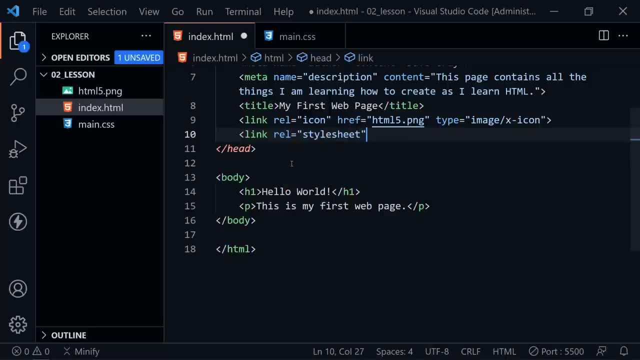 we have a style sheet. because we're adding a CSS style sheet, Our href will now point to our CSS maincss specifically and our type, which isn't actually required anymore. But since we have it, let's go ahead and add text slash CSS, But our browser should know what it is. 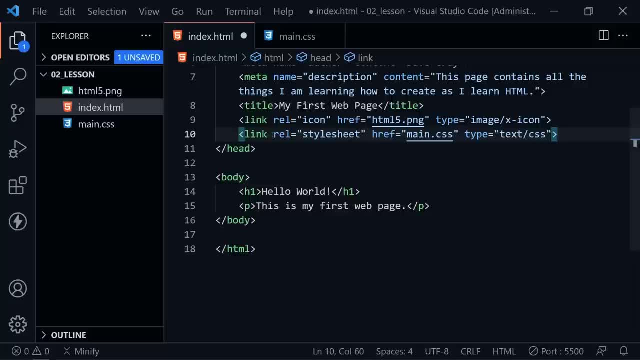 even if we didn't add that at this point, because that's really the only type of style sheet there is- is a CSS. Now that we've made these changes, let's save the file And let's go ahead and click the button. 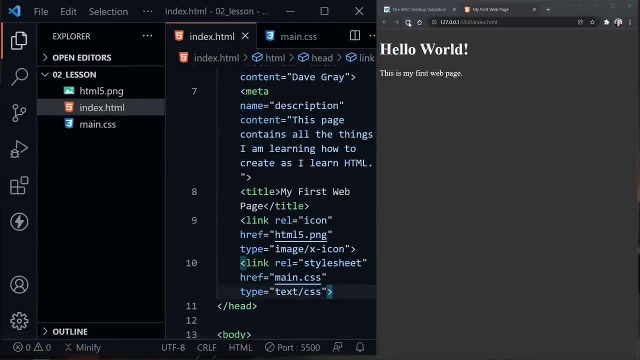 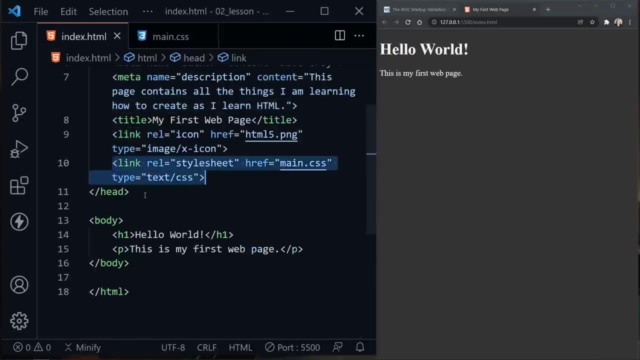 again to make our code shrink back down. and look at our page- We can reload, just to make sure it has reloaded And everything looks the same. That's because we are pulling in our code. I'm going to go ahead and hide the file tree here. We are pulling in our CSS code using our link tag. 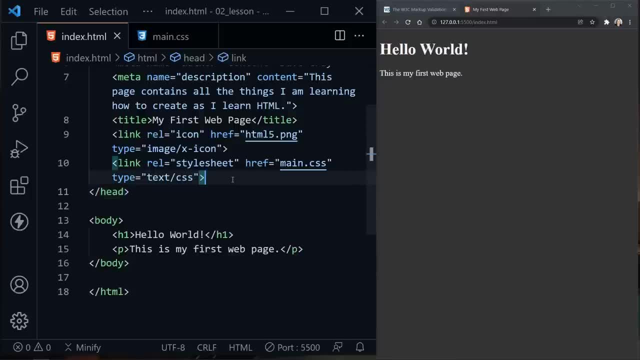 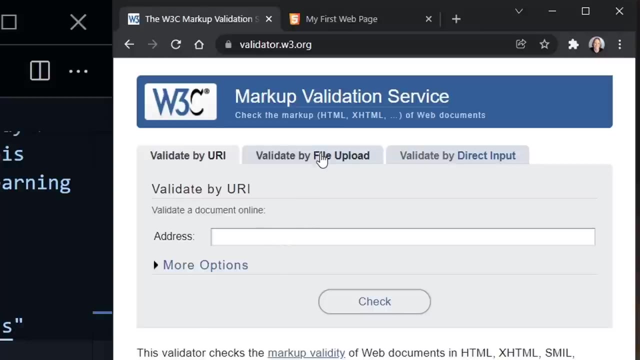 inside of the head element. Now, finally, I'm going to create an error on purpose by deleting the symbol at the end of this link tag and saving the file with control S. Now, why would I create an error on purpose? Because we want to validate our file again And this will let us know that. yes, 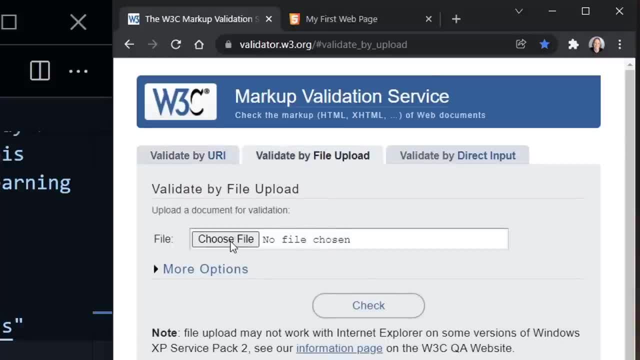 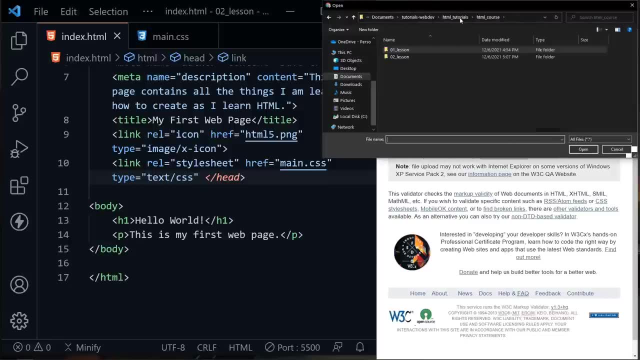 we've got the right file and we expect one error there. You don't, of course, have to create an error on purpose, but that's what I'm doing to make sure I'm selecting the correct file out of the correct lesson folder, because I'm in lesson two Now you might be working on the same file. 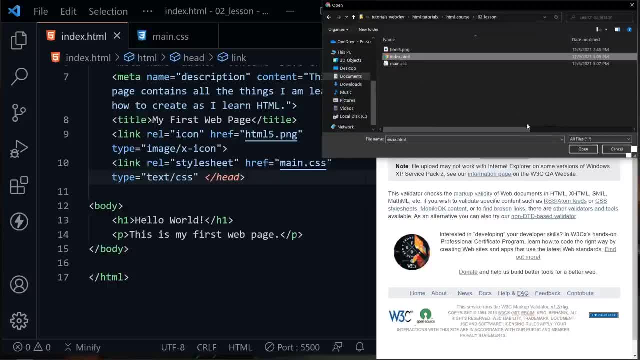 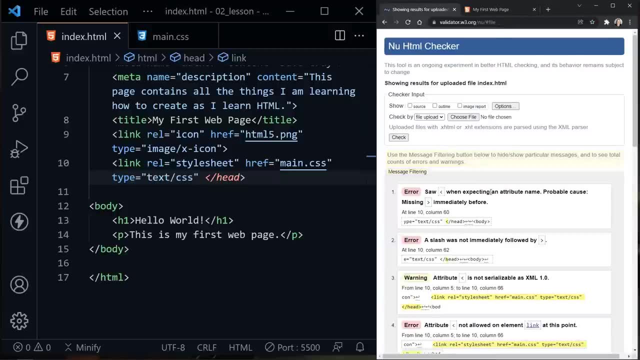 we started with. There's the CSS file and the image file. I'll select the indexhtml and check, And I should have at least one, if not more, errors because of that. Yes, I created several errors on the page just by leaving out that one. closing- 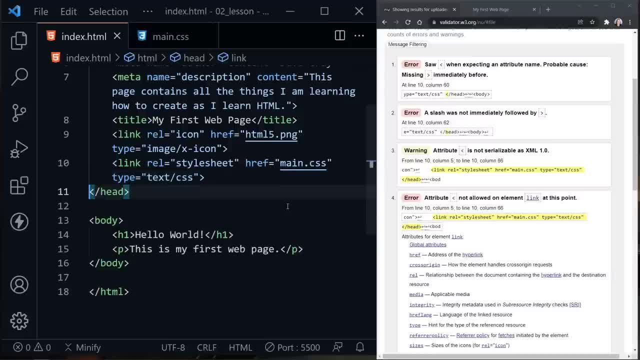 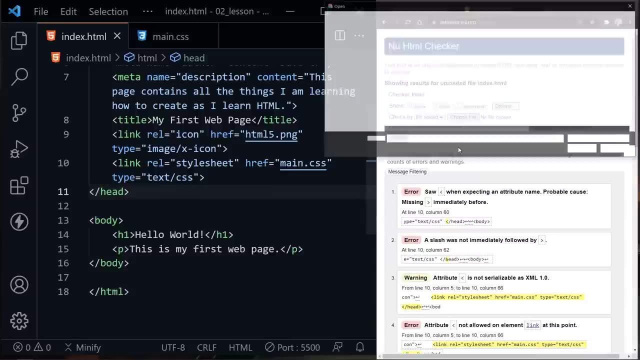 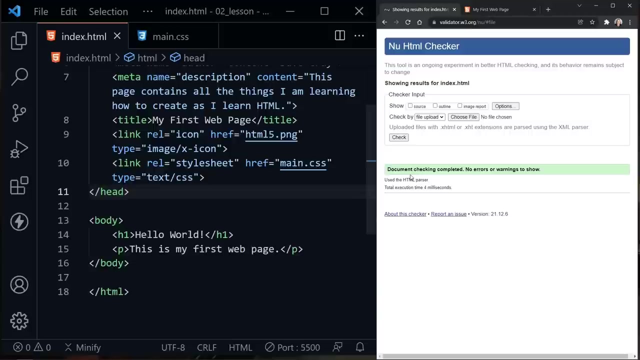 greater than symbol for the link tag. So now, if I save again, Visual Studio Code formats our code correctly instead of trying to pull the closing head tag up here, And I'm going to go ahead and load the file to check it. So we choose indexhtml. Now I'll click check And document checking. 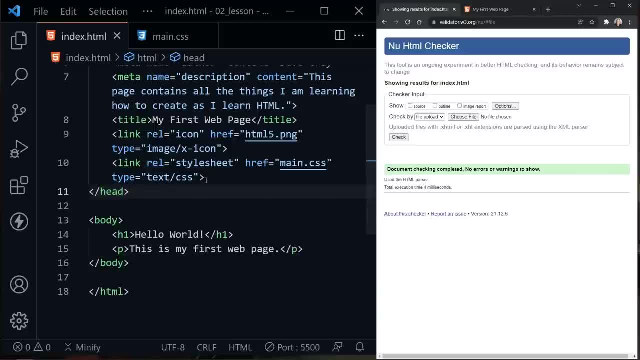 completed. No errors or warnings to show. So just by missing one little thing in our page, we could have a whole list of errors. So follow the prompts from Visual Studio Code. Notice how, if I leave that out here in my theme, this turns red or pink. It doesn't look quite right. Visual. 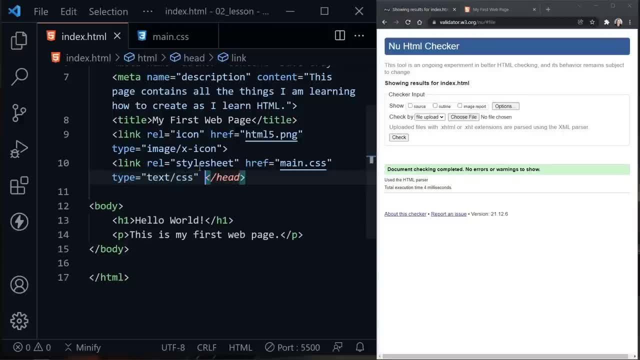 Studio Code wants to check that, So I'm going to go ahead and click check. And now I'm going to format it differently. if I save the file And it pulls that up here instead of putting the closing tag, There's several cues to show you that you have an error in the file, And so follow. 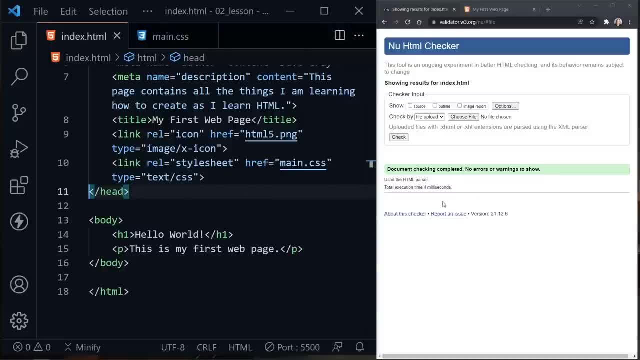 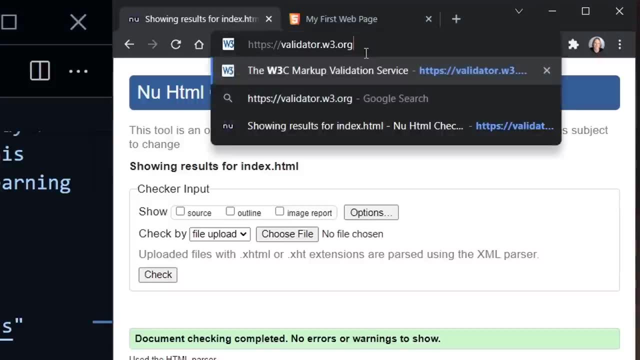 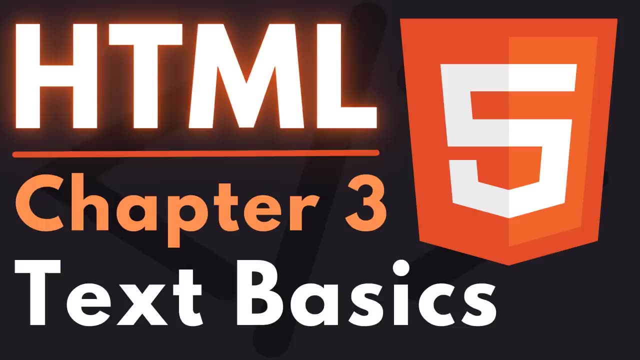 those prompts in Visual Studio Code. And then remember to always validate your page, And we always do that at validatorw3.org. I'll get rid of everything at the end of that And here you can pull it up. And then we choose file upload. Let's look at the basics of 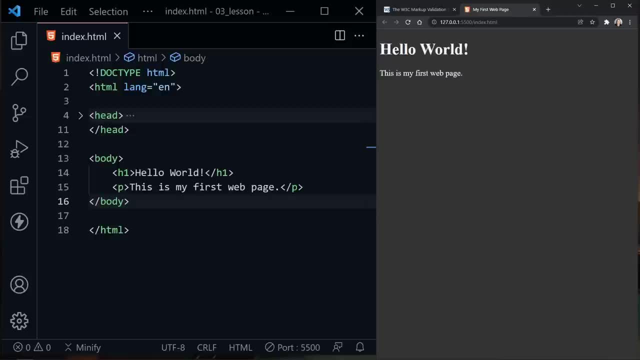 creating text content on a web page. Now, web pages are a lot like essays or even a newspaper, where they have headings and usually paragraphs of text or at least a sentence or two of text describing something afterwards. So we see our paragraph element here and our H1 heading here. 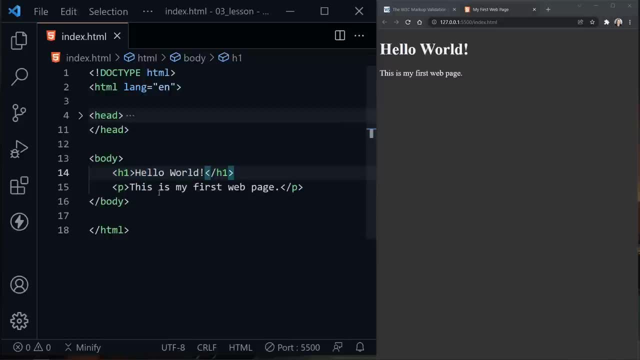 Much of the text content on a web page will be made up of headings and paragraphs. Now, headings have a hierarchy And that means we'll start out with only one heading And then we'll start out with one H1 on the page, And each page should only have one H1. But after that we can have subtopics. 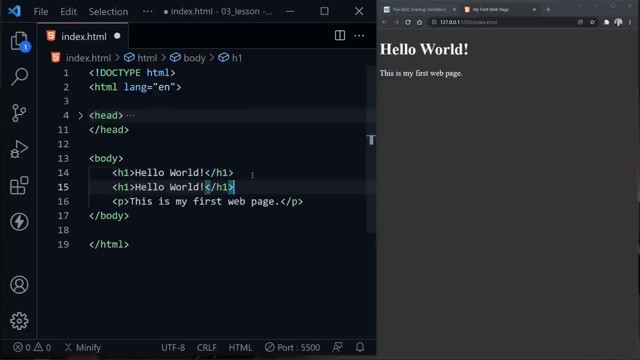 So here I'm going to press shift, alt and the down arrow. Again, I'm using Windows. It may be different for you on Mac or Linux, But I just copied a line down. So now I have two H1s, But I'm going to change this by typing H2 over that H1.. And notice how the ending tag immediately. 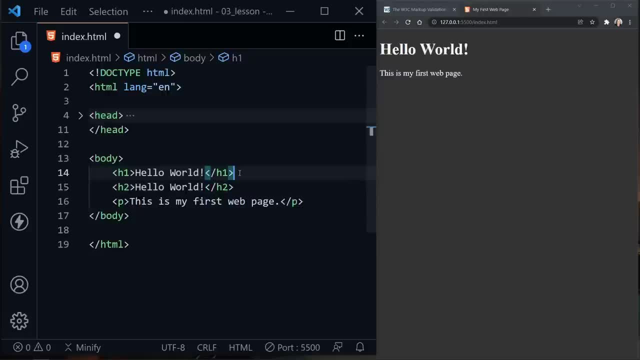 changed here in Visual Studio Code as well, So that's helpful. Now this is a subtopic for the page, So imagine this being the title of your essay or the big headline in a newspaper, And then we have subtopics. So for H2, I'm going to type something. 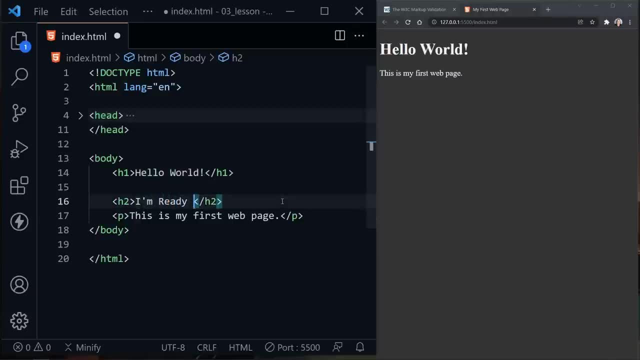 different. Let's go with. I'm ready to learn HTML And now we can have a paragraph about that, And so we do. at least we have a sentence. This is my first web page. Now I'm going to highlight this subheading H2 and the paragraph, And once again I'm going to press shift, alt and the down arrow. 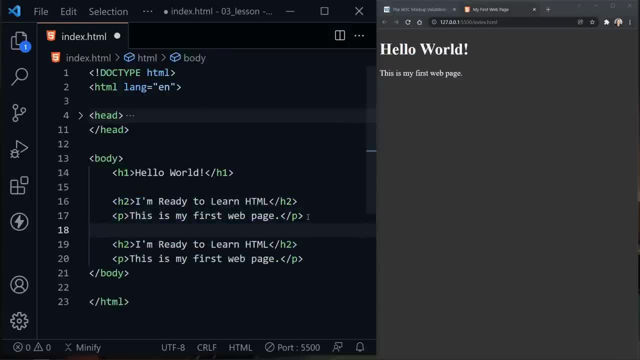 And it copies both lines down for me And I'll add an extra blank line here And I'm going to change this second H2 into an H3.. Now we- I'll use lowercase. There we go. Now we could have more than one H2 on the page, But I wanted to show how you could have a subtopic under our subtopic. So 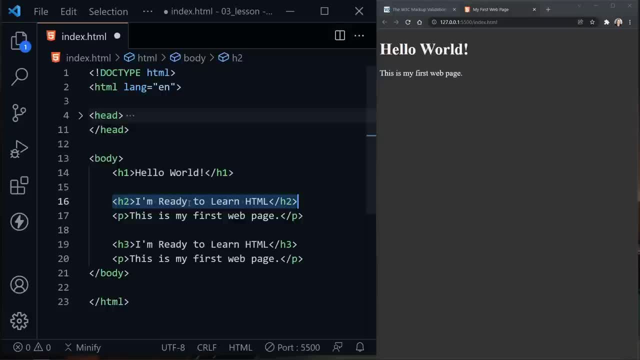 we have an area of discussion that we've added an H2 as the heading for, And now under this area of discussion, we could have further subtopics, And this is how we now have an H3.. So now, instead of my first web page or I'm ready to learn HTML, let's change this to my daily schedule. So this: 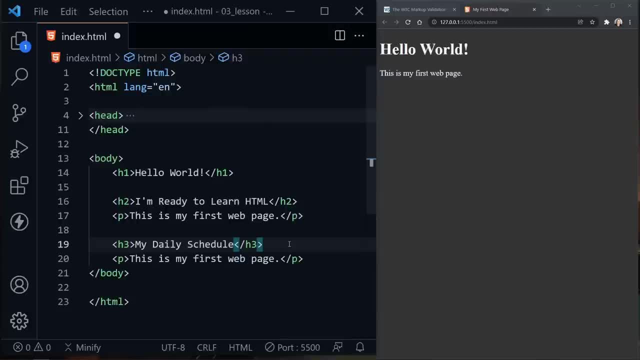 will discuss our schedule for learning HTML And then we can just say something about I'm going to, or let me tell you how I and I'll just put some dots there for now. We'll expand on that later if we want to. But really what I'm showing is this hierarchy, And it's also important, not just 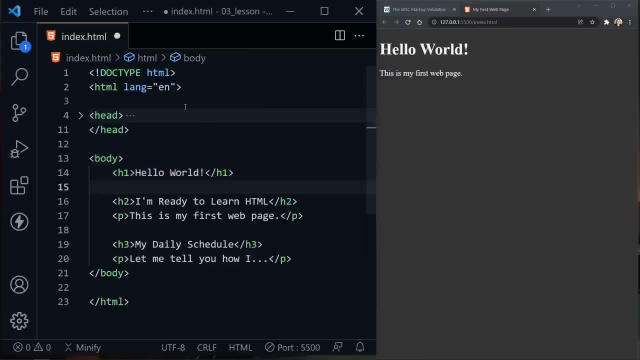 visually. Let me go ahead and save this by pressing control S Or remember. you can go to the file menu and choose save Visually we see that it's naturally formatted larger on the page with the H1 than it is the H2.. 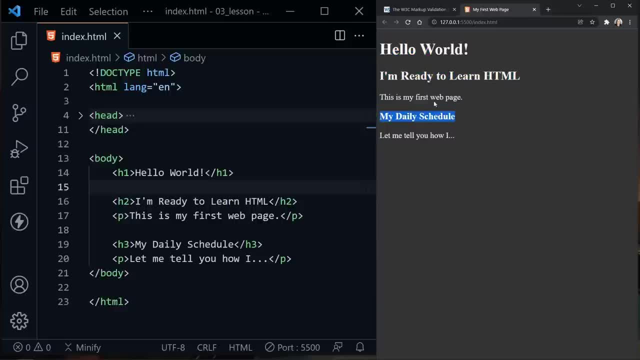 And then the H3 is even smaller than the H2.. But we can change all of that with CSS. in the future, CSS will really style how our web page looks. But what is important is we can quickly visually tell the headers apart right now, And when a screen reader or other assistive technology looks at our code, then it can navigate. 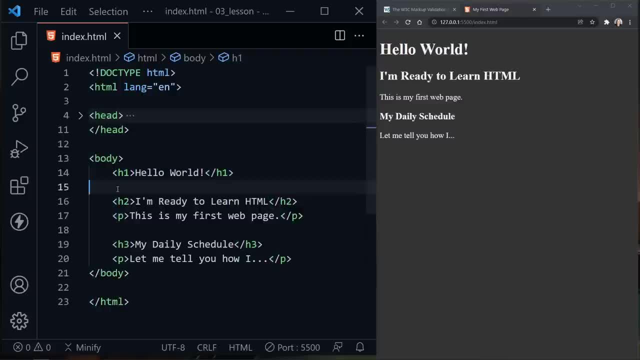 the code through the headers of what is important here, The header hierarchy, And that's why it's so important to organize your page. The headers actually give semantic meaning, saying this is the main topic, This is a subtopic under the main topic And this is a subtopic under the higher subtopic in. 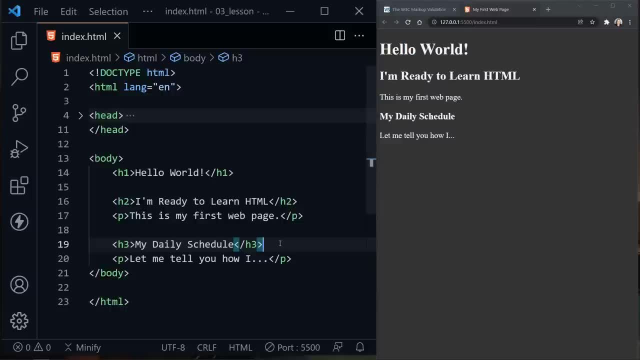 the hierarchy. So headers do have semantic importance, And that means giving meaning to our content, And of course then our paragraphs can just have whatever details we want to add about those subtopics as well. Now, even though we've created a little separation in our code, when we look at our page we just see line space, line space. 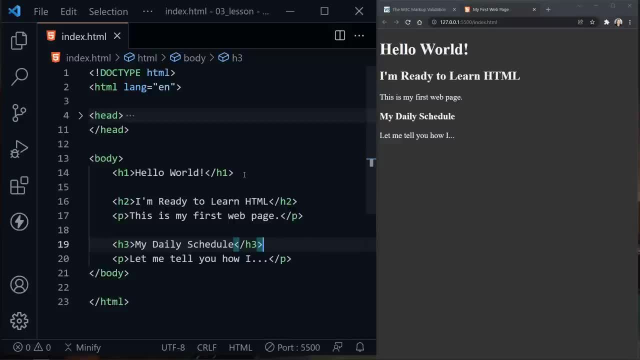 and we don't have a good visual separation, I'm going to add an element that doesn't really provide any semantic meaning but visually it helps us on the page, And that is a horizontal rule element And it's just added like this: 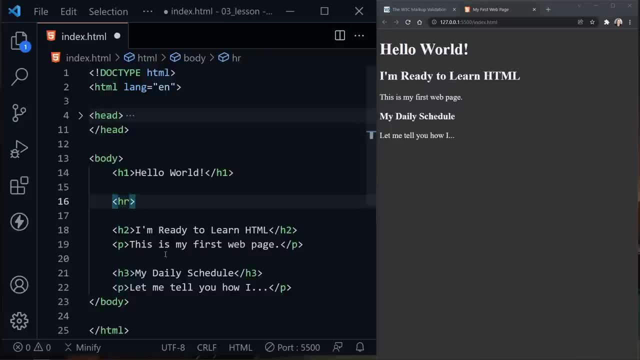 There is no closing tag for the horizontal rule, And then I'm going to add another one after our final subtopic Discussion here, so we can add something else underneath that. And so now let's save and look what the horizontal rule adds to the. 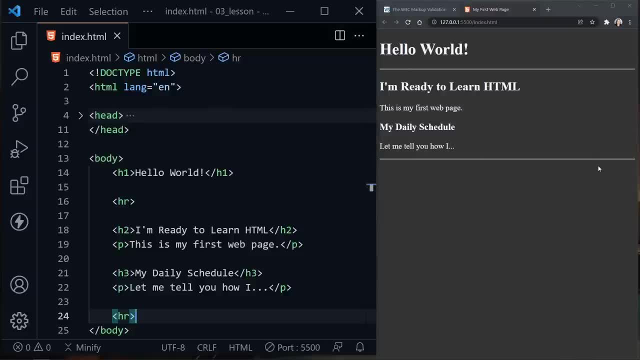 page. Now we have lines going across the page And those are called horizontal rules. So we have our main heading And now we have our subtopic, And I left the H3 in here because it's a subtopic of this topic. So now we can go ahead and I'm going to. 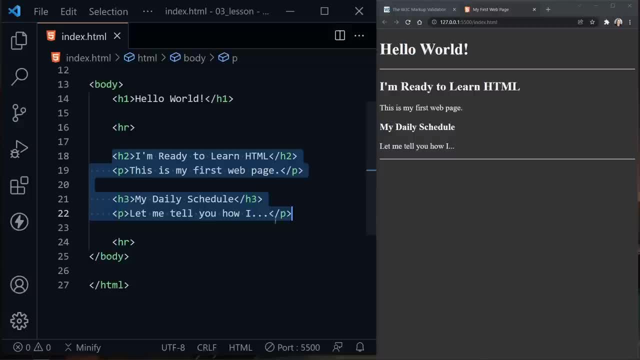 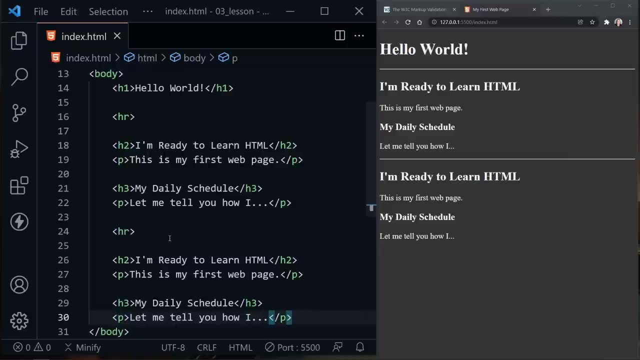 highlight the H2 and the H3.. Control C to copy. Come down further on the page and paste and I'll save, just so we can see what happens. Now we have two different subtopic sections and we still have our top hello world. so you could picture this more like an essay page And of course, these could be. 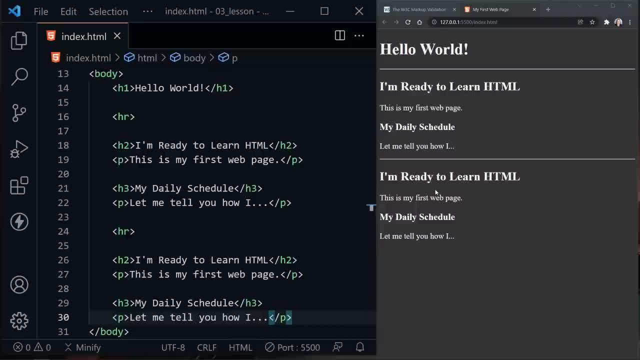 paragraphs that have more text, or you could picture this more like a newspaper, and then we would have an article here and an article here and our heading at the top. This is also a good time to discuss. What is the meaning of this. What is it about? 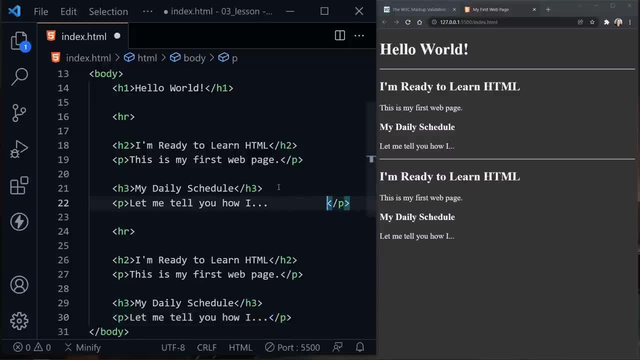 What is the meaning of this? What does it mean? white space- So if I just press the space bar and add all these extra spaces to the page, if I say, Visual Studio Code is already going to probably reformat this, but what is important to 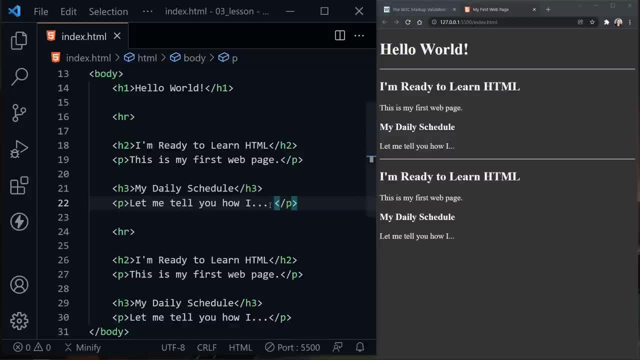 know when I save, you'll see. yes, it changed and it just went back. it only left one space. is web pages or HTML. do not honor all those spaces you might add with a space bar. It's called white space collapsing, and so we can space many lines, but it won't really be represented on the page. 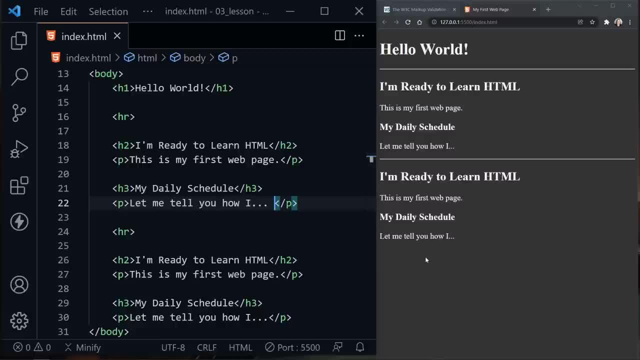 that is not how we add extra space in HTML. So again, recognize white space collapsing that it will not last. Now something we can do is what's called a line break and that can be inserted inside a paragraph element. So now I'll put: let me tell you how, and then I'm going to return. 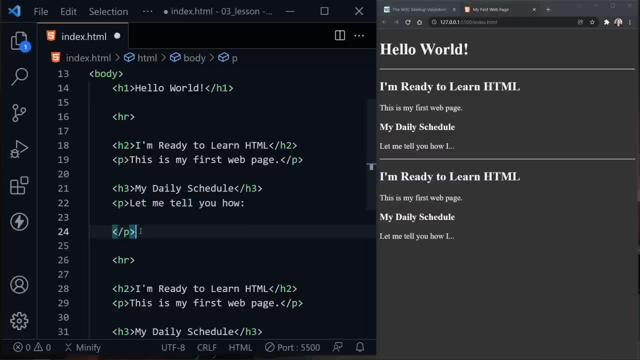 remember we don't have to have the open paragraph, opening and closing tags on the same line for an element. we can nest other elements inside of an element. so I'm going to put a break, and that stands for line break, and then I'll put three. 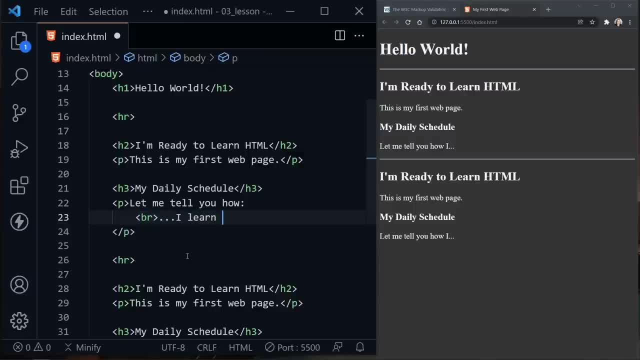 dots and I'll say: let me tell you how I learn more about web dev and a period that looks good. and now we can put another break. and I'll just put three more dots and say I plan out my schedule and one more line break. the three dots, of course, are not required, it's just what I'm adding here. 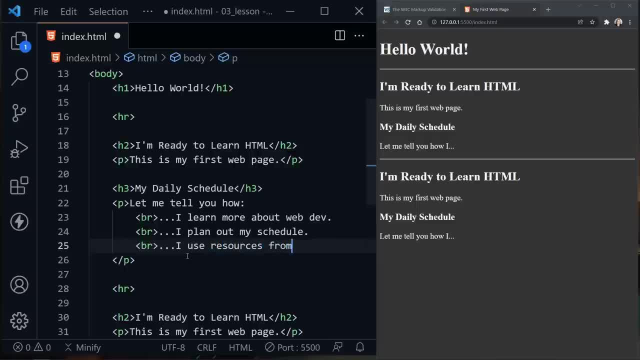 and then I'll say: I use resources from MDN, which previously we discussed, and when I showed the definition of HTML, we were looking at the Mozilla developer network and that's what MDN is. so now, if we save this file, you can see we've got line breaks and we're showing each of these details. 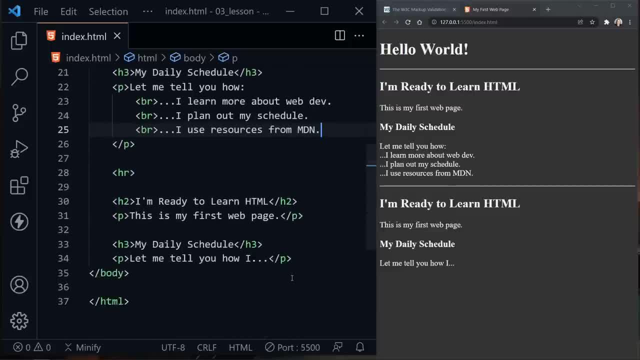 on separate lines. Okay, Let's scroll down and change some of our second topic now. so instead of I'm ready to learn HTML, let's change our second subtopic to I am. let me capitalize that I am also planning a vacation, and now we can put some details about that vacation in the paragraph underneath this subtopic. 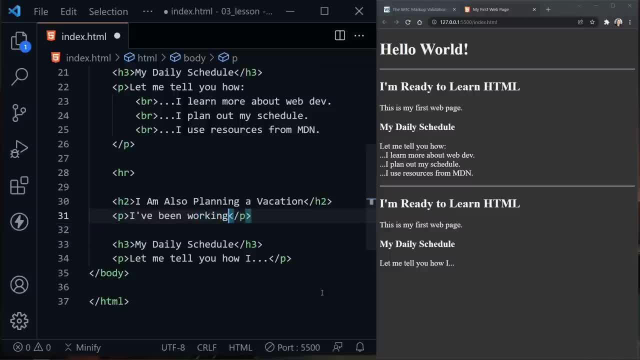 and I'll say: I've been working hard and really need a getaway period and let's see if we want to add anything underneath that. Yep, let's add one more sentence and what I'm going to do once again is shift, alt and the down arrow. 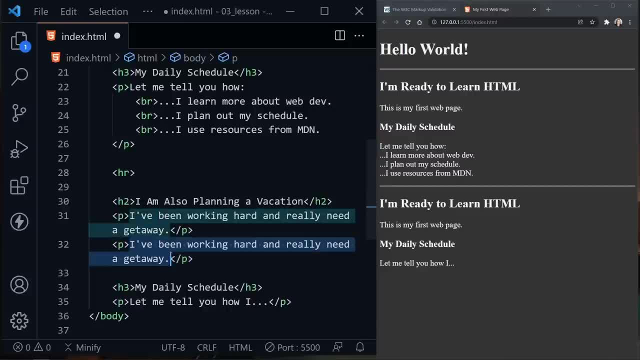 and Visual Studio Code will copy that line down. so now we can just change the sentence here and I'll say: I live in Kansas, so I want to visit a beach. Kansas is nowhere near the ocean, so that sounds pretty good. Okay, So let's save that. 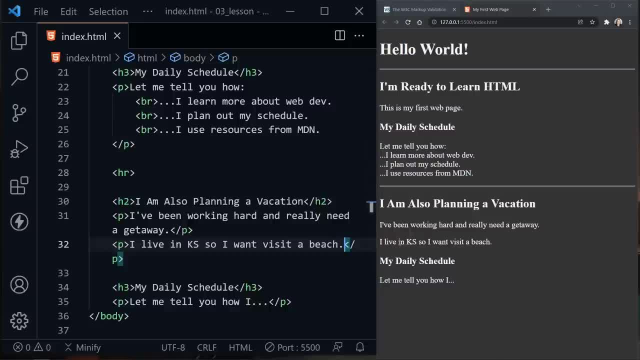 And now we can see our subtopic care changed and we have a couple of sentences about planning a vacation. Now let's change the my daily schedule subtopic at the H3 to places I'd like to visit, and I guess I could capitalize that tell unlike. 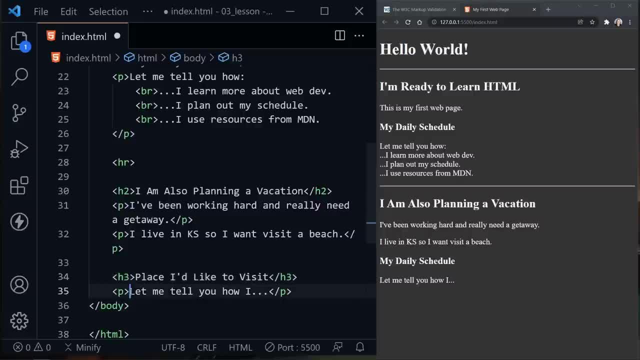 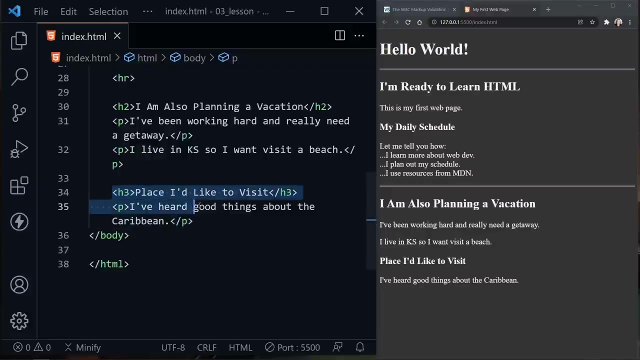 There we go, Places I'd like to visit, and now I'll highlight that paragraph and say I've heard good, Okay, save, Okay, good things about the Caribbean. Sounds like they have warm water and fun islands to visit, Okay. so now we've got some extra details here And we can have more than one subtopic here. 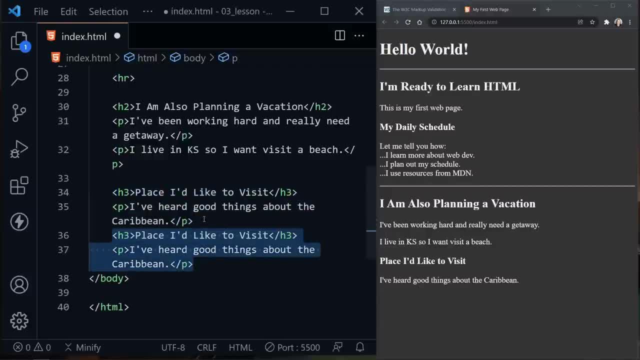 So let's go ahead and do that Again: shift alt and the down arrow to copy that. And places I want to avoid could be our next one. So places I want to avoid And here we can put anywhere cold, No way with an exclamation mark. 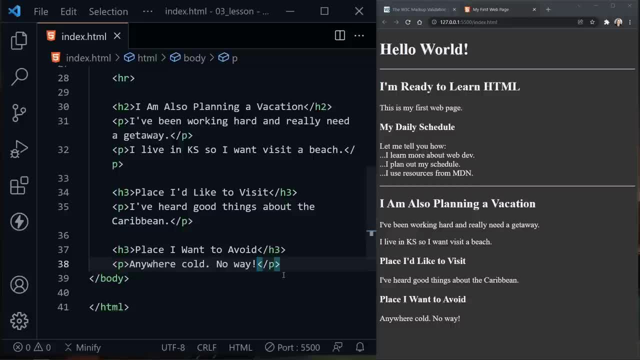 Okay, so now we've got some extra detail here in our second area, And this will allow me to go ahead and show you the difference between block level elements and inline elements. What we've been working with here are block level elements. Notice, with every paragraph and every heading, they start on a new line. 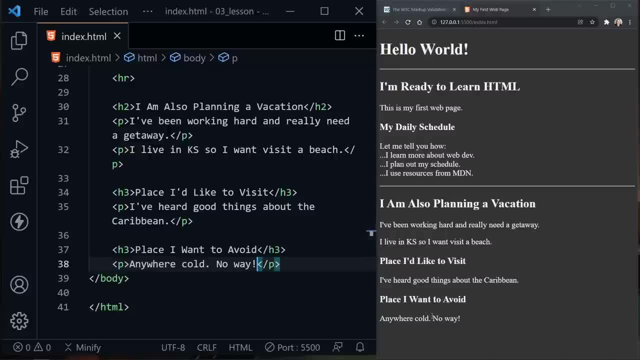 That is a block level element. It creates space around it, which of course can be formatted in the future with CSS, But it does not allow you to put another paragraph inside of a header or a paragraph without creating that new line, that space. 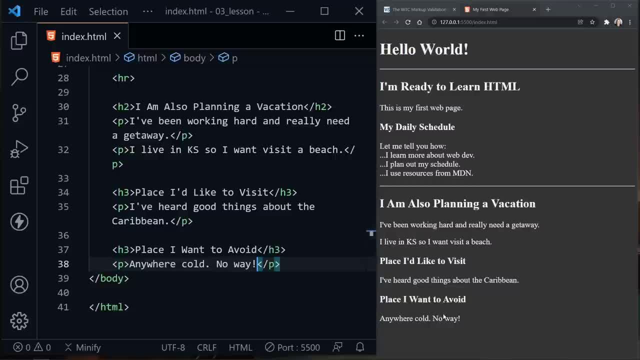 So there will be a return essentially in your content when you're using the block level elements. So there will be a return essentially in your content when you're using the block level elements. So there will be a return essentially in your content when you're using the block level elements. 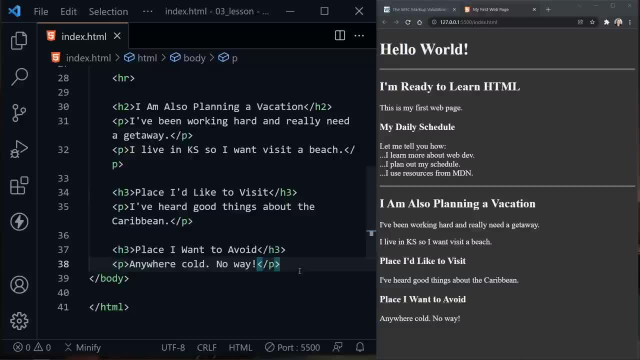 But when you use an inline element, that doesn't happen. So let's look at a couple of these. First of all, we can say: I've been working really hard and I've been working hard and really need a getaway. Let's emphasize that: really need a getaway. 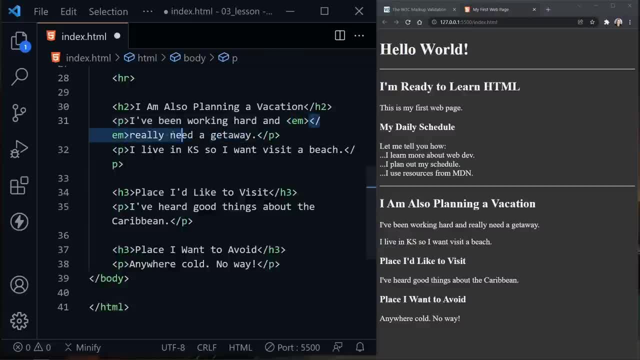 And one inline element that we can do that with is EM, And that stands for emphasis. That provides some semantic meaning once again. So now a screen reader Or other assistive technology Or just our browser overall knows we're emphasizing this, really need a getaway. 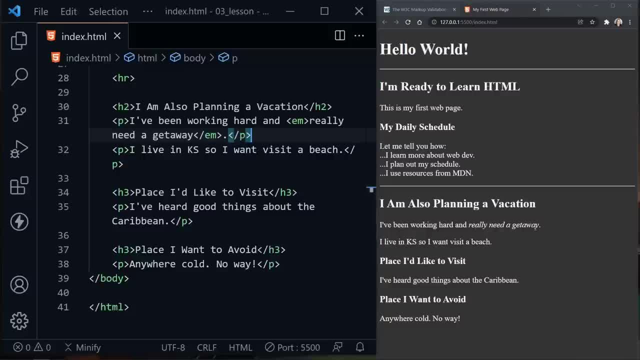 So let's save And notice: really need a getaway is italicized. Now. we're not using it for the italicized text. Again, the formatting will come later with CSS, But that is just the natural behavior of using the emphasis element as we wrap our text. 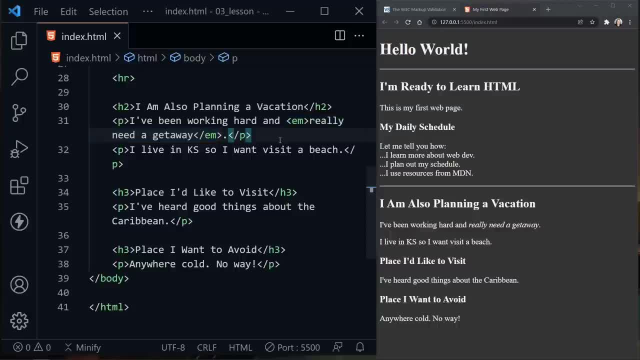 But it provides that meaning. Now, what if we really want to emphasize That text? it has a strong meaning to us. like our no way here, We don't want to go anywhere cold. Well, there is a strong element we can use for that. 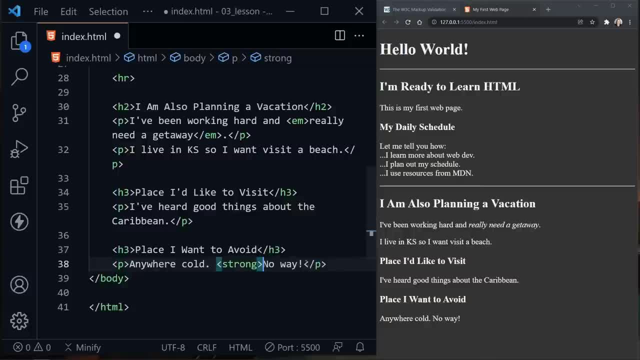 And here let me grab the ending tag and put it at the end of our no way, And now I'll save and notice it got just a little bit bigger and bolder here as far as the natural formatting of the strong element. But again, this is an inline element. 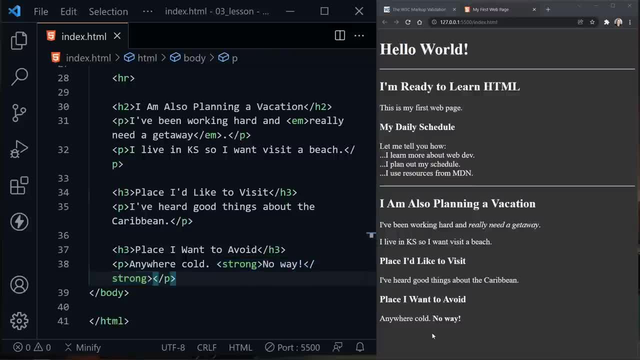 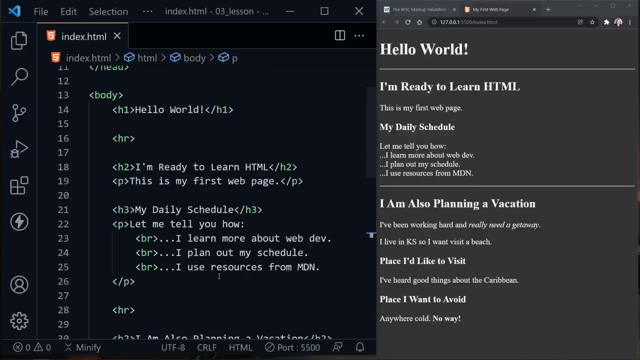 It's inside the paragraph. It did not create a text, It did not create a break in the line, It did not create any extra space around it. So these are inline level elements, And the other elements, such as the header and the paragraph we've been working with, are block level elements. 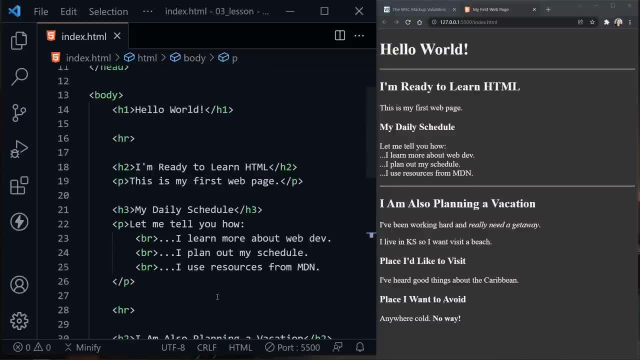 Another type of content we can add to our page are HTML entities, So they are things that are not really the normal text we would type out. What, for example, if we wanted to show a less than or a greater than Symbol on our page? right now, HTML interprets those as we're starting or ending a tag. 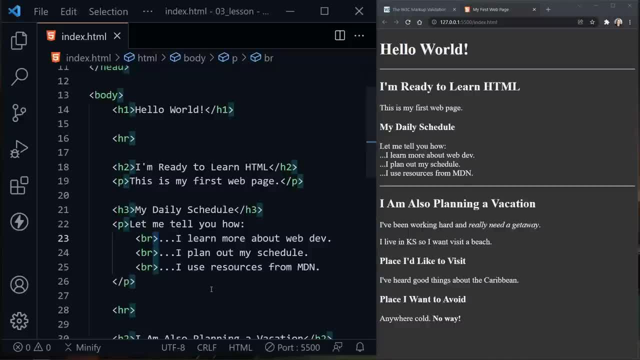 So we can't just easily put one of those on the page. Likewise, there are some other symbols, Or remember when I talked about white space collapsing? if we need a little bit of extra space, there's an HTML entity for that. So I want to indent these three lines with a little bit of space and I can use the HTML entity. 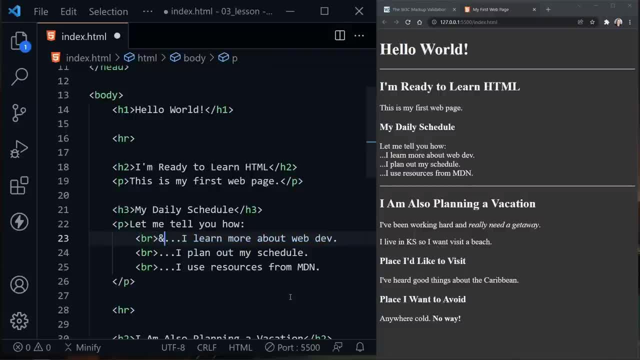 I still need the closing there. Here we go, And ampersand is usually What starts out: an HTML entity. And now I'll type NBSP and a semicolon Notice. Visual Studio Code recognizes that right away And, if I save, I have spaced this line over just a little bit. 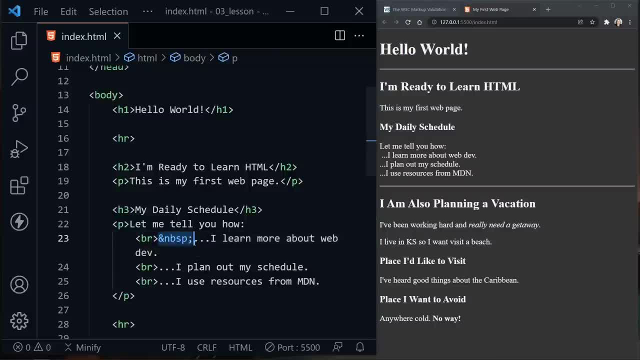 Now I can add more than one of those if I want. So I'm going to copy that and I'm going to add two more And now save, And our line is over even a little further. So I will go ahead and select all three of these. 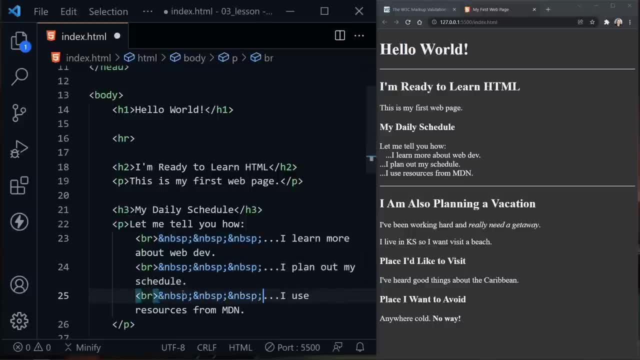 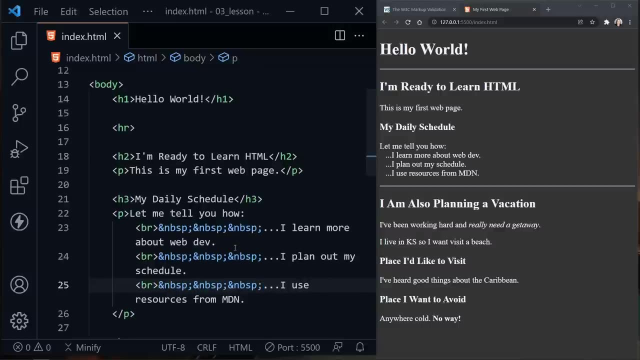 And I'm I'm going to paste them right after the line break on each line and save, And now we have indented with some extra space all three of these lines with these HTML entities that create space. But, as I mentioned, there are other HTML entities as well. 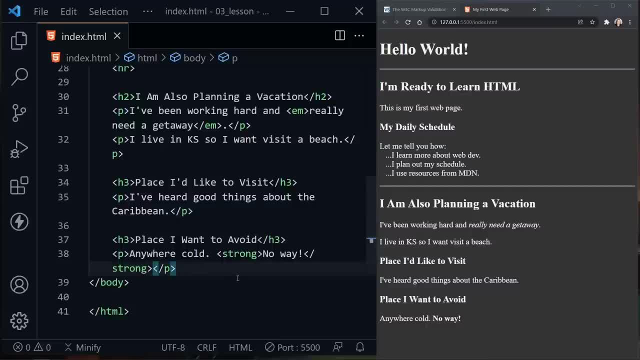 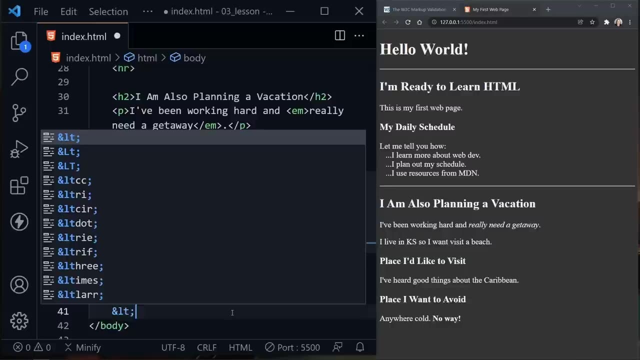 So let's scroll down here to the bottom of our page And after this last topic let's add another HR, and now we'll type and LT And a semicolon, and that stands for less than. So if we save now, look, we have a less than symbol underneath the final horizontal rule here at the bottom of the page. 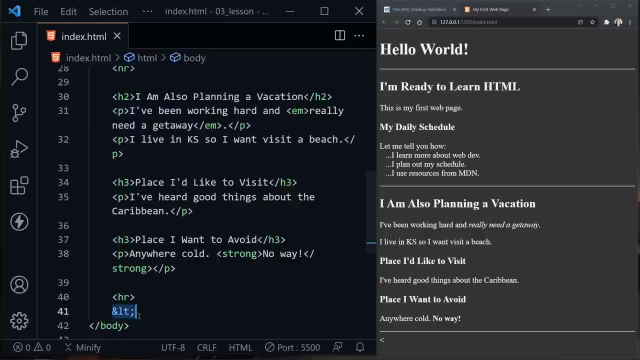 I'm going to go ahead and copy that and paste two more and then I'm going to add ampersand copy with a semicolon and that will be the copyright symbol. Then I'll just put my name, You can put yours, And then I'm going to add ampersand GT for greater than and a semicolon. 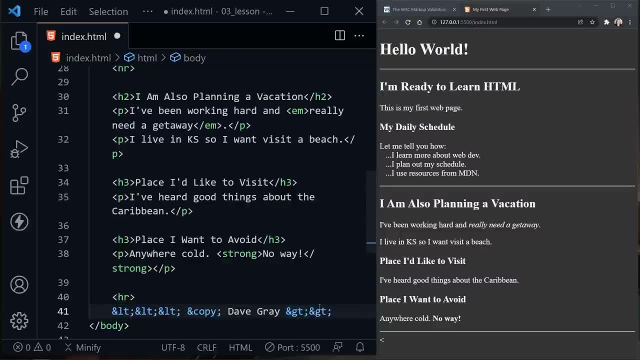 And once again I'll copy that and paste two more. Now, if we save, you can see we've got our three less than symbols. We've got a copyright symbol, then your name or my name, and then three greater than symbols. 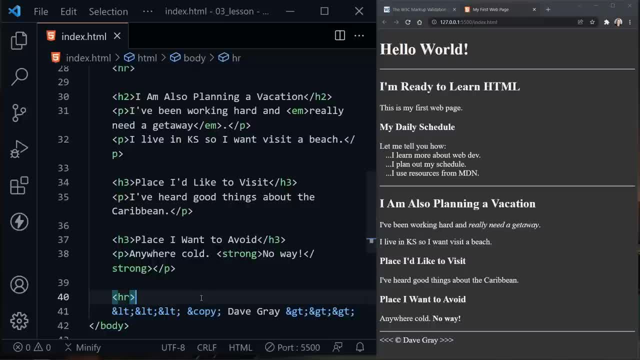 And we're using HTML entities to create those. I'll provide a link to a list of HTML entity codes In the Resources for this tutorial. you may have noticed we've got a couple of abbreviations on our page. We have the abbreviation for Kansas, which is KS, and we also have the acronym or abbreviation for the Mozilla Developer Network here on our page. 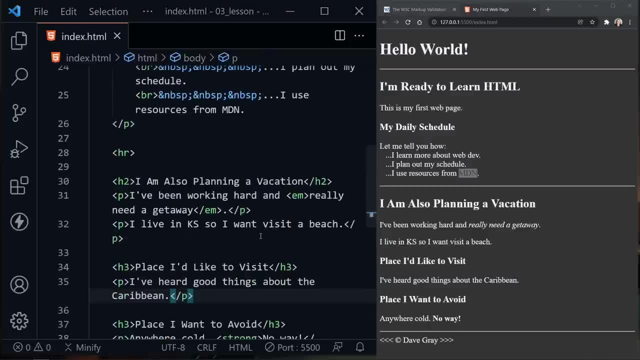 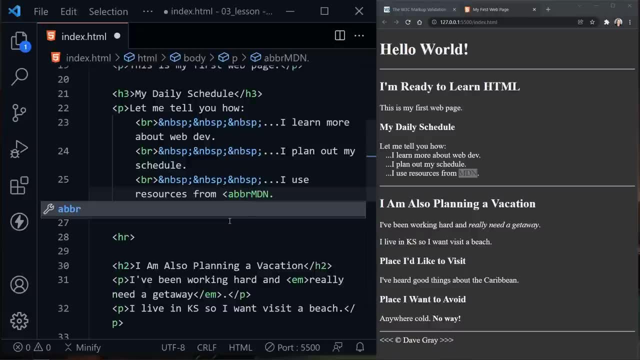 So let's go ahead and add another inline level element and that can help us with our abbreviations, And that is ABBR. but it doesn't really do it by itself. I'm going to go ahead And select MDN, cut it and paste it here in the middle of the element. 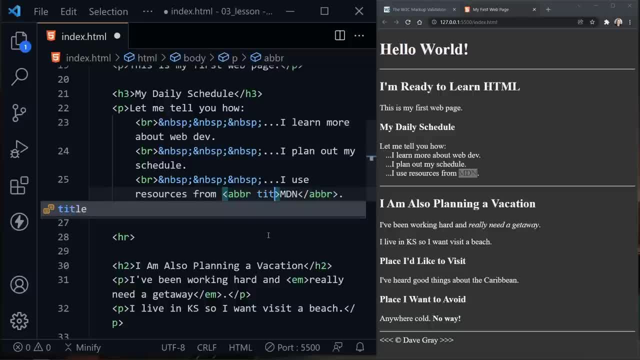 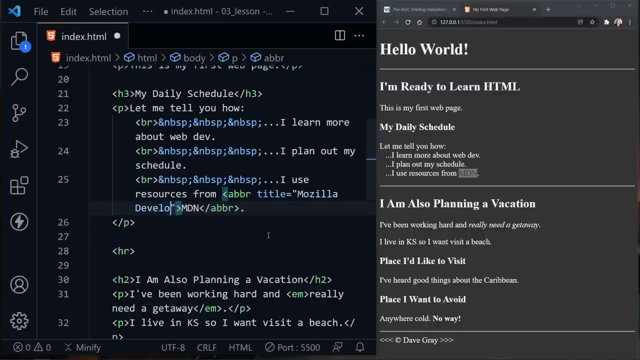 And this won't really provide anything. We also need to add the attribute title. here I can put the full text Mozilla Developer Network and save. And now when we look at our page, it has some dots underneath MDN. If we mouse over, we get a tool tip that says Mozilla Developer Network. 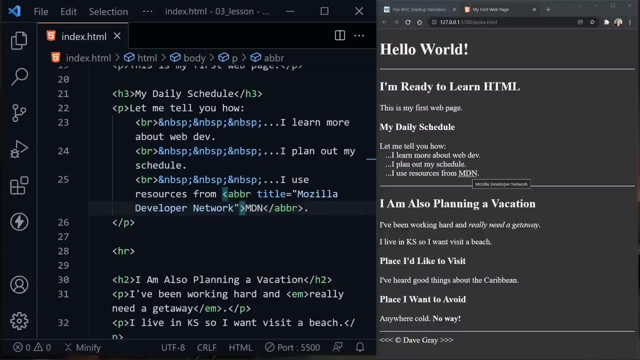 Now it's important to realize this Tool Tip will not really be available to screen reader and assistive technology, So we don't want anything super important for the understanding of the meaning of the page to be in there. So if we are using abbreviation, it's a nice thing to have, but it is really not accessible to all assistive technology. 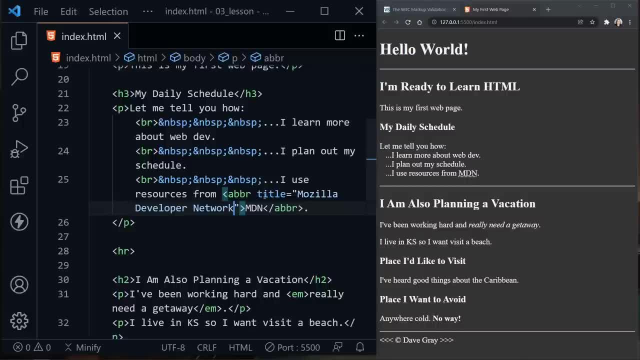 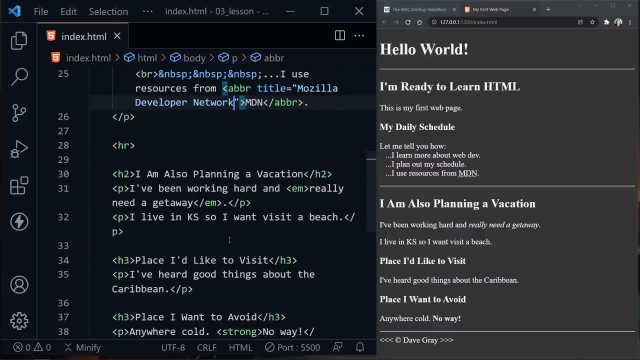 So it's you can't have anything in there that the page really depends on, because some of the people accessing the page may not be able to read or see the information that you provide here inside the title attribute of the abbreviation element. Let's go ahead and add that abbreviation element for Kansas as well. 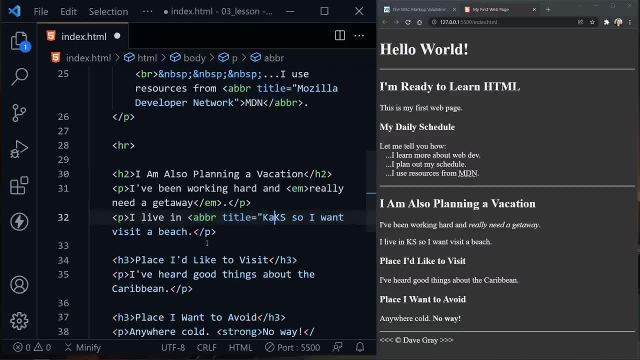 So ABBR, and then title, and I'll spell the state name Kansas, And then I can go ahead and double click on Kansas, control X, to cut, and I'm going to paste it with control V right inside the element Save. And now dots are under the KS here on the page. 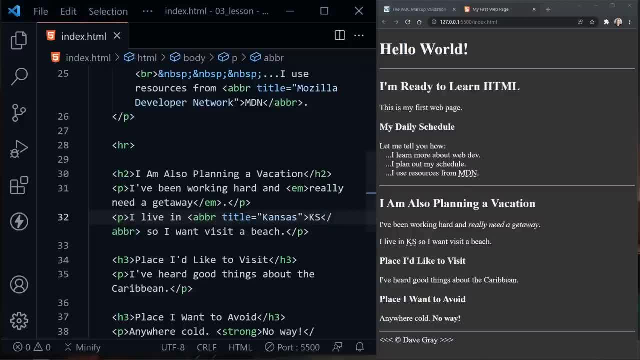 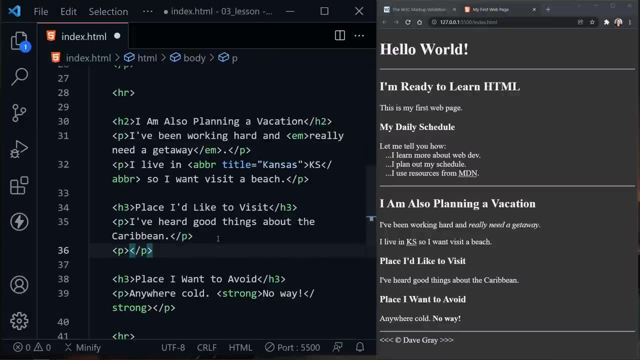 And if I mouse over, we get a tool tip that says Kansas. Let's put another paragraph under places I'd like to visit and I'll put. I can just type P and press tab as well. There we go, And now I'll type: I've heard good things about going here with a colon. 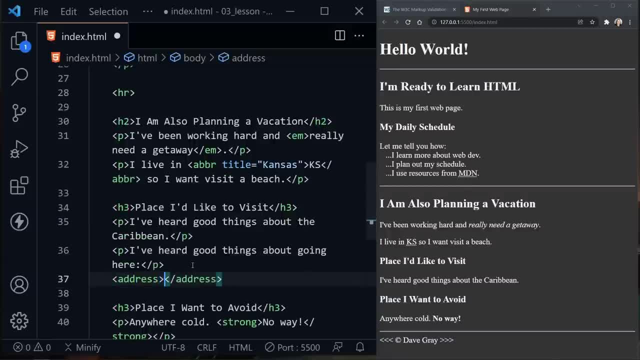 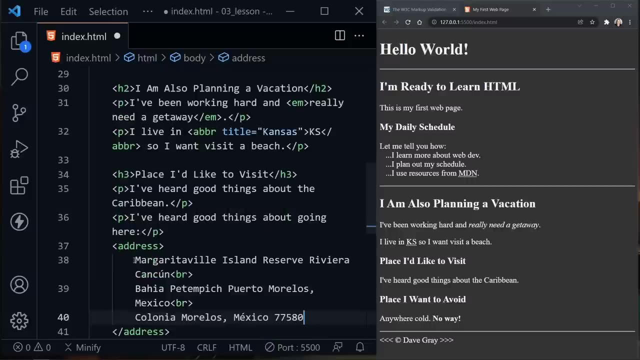 And now I'm going to add an address element and we can put a location Inside of this address element and it tells the browser that this is an address or a specific location. So I'm just going to paste this in, because you don't need to see me type all of this and I might easily have a typo here. 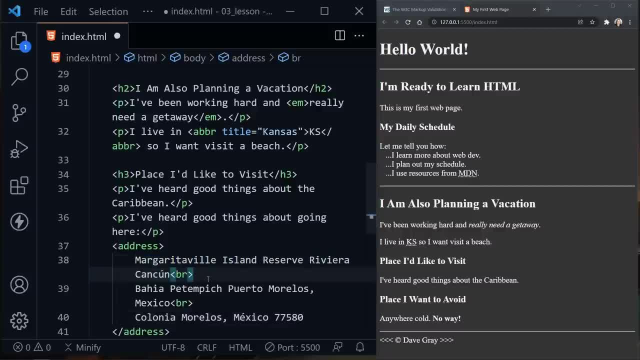 This is Margaritaville Island in Cancun. It sounds like a great place for a vacation. Notice, we've got a line break element after each line, except the last line, And if we save this and look at the page, you can see how the browser handles this. 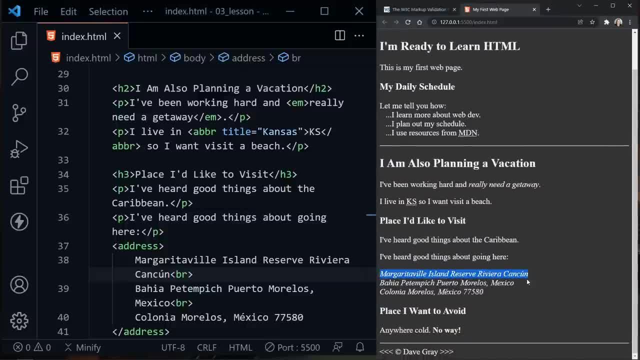 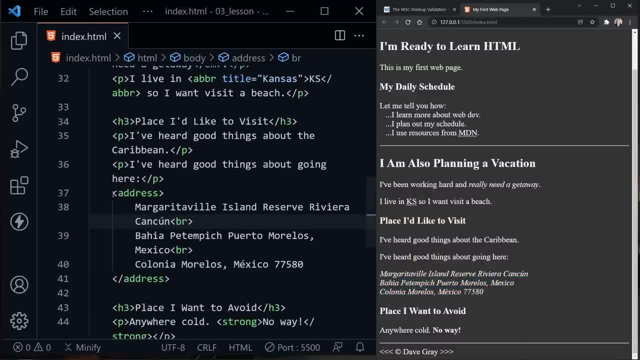 It is just three lines of text. It is all italicized by default and the browser knows that this is an address And once again, so would assistive technology. So an address element does provide some semantic meaning as well to the content within it. 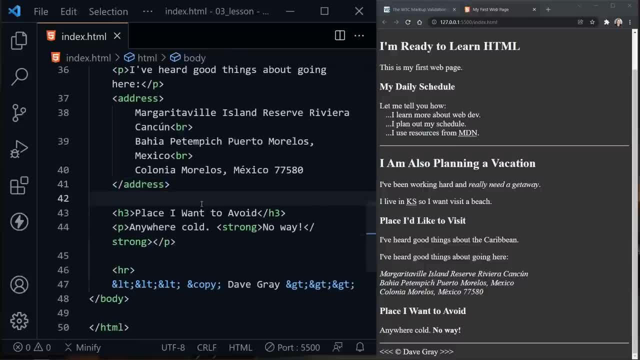 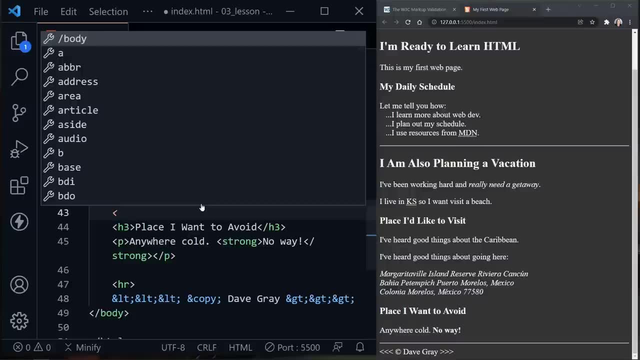 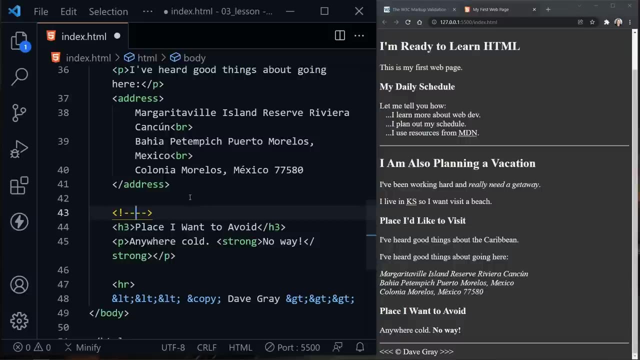 Now, before we finish this lesson about content, there's one other thing we can add to our code. Now we won't see it on the page, but it is important to us, And this is an HTML comment, And so now you can see Visual Studio Code colored this differently, at least with the theme that I'm using. 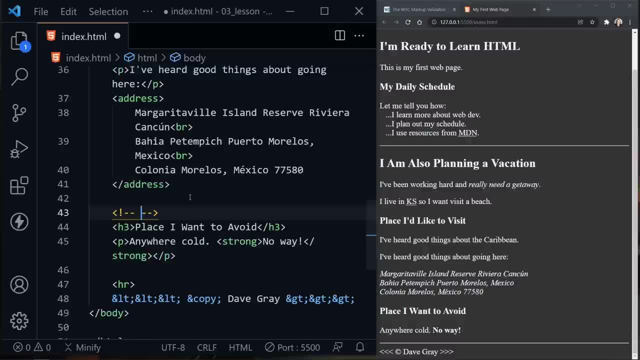 And we can leave a note for ourselves inside of our code. Now, notice: this will not be on the page, but I will show you how the public can see it, So you don't want to put anything in here that you don't expect the public to be able to read. 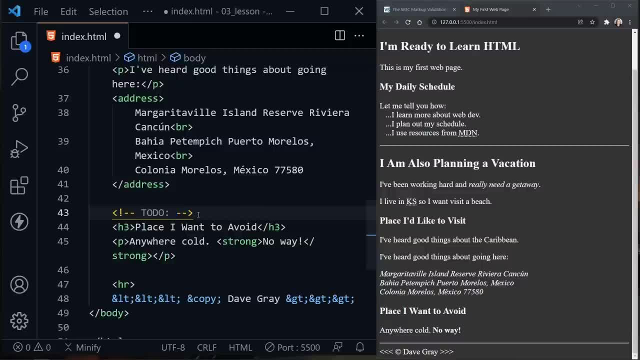 I'll put a to-do, which is a common use, and I'll just put add more places. So it's a reminder to me to add more places to the list of places I want to avoid And we save that And it doesn't show on the page. 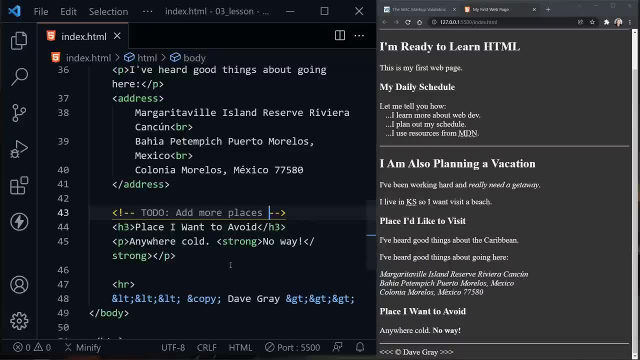 It's just a reminder in the code or a note to yourself inside of the code, But I will show you how the public can see this. If we right click and choose inspect, that works, Or you can also press control U. Either way will show your source code. 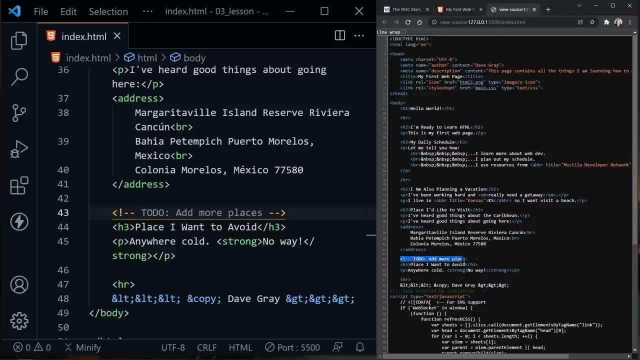 Now notice we've got a comment in here that says add more places. It's not visible on the web page itself, but it is visible on the page, But it is visible in the source code. Again, you can press control U to view this. 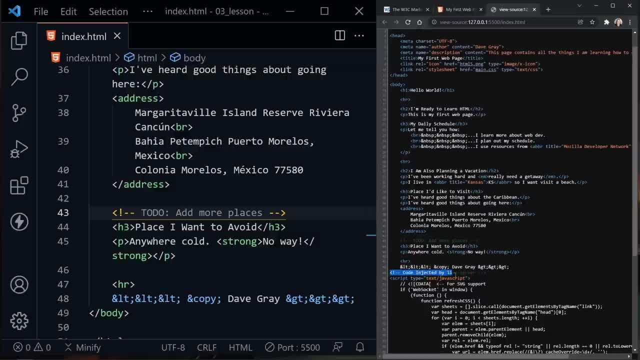 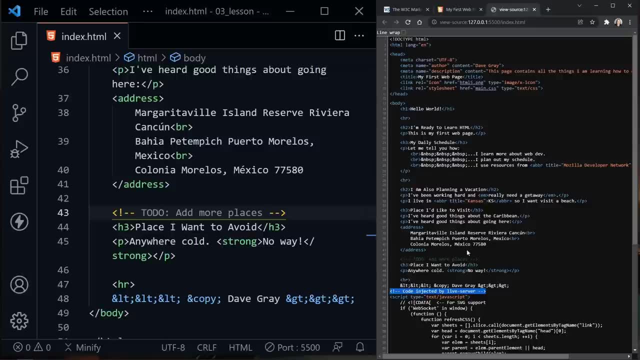 Now notice: live server also injected a comment here and it injected some JavaScript. So when we look at the overall source code of what is live, we're seeing more than we even had. But this is a comment, once again, that is not seen on the page. 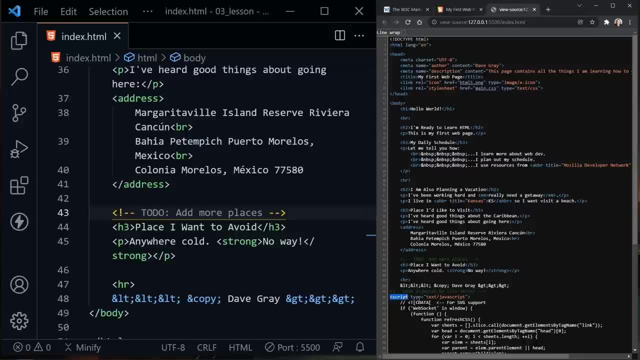 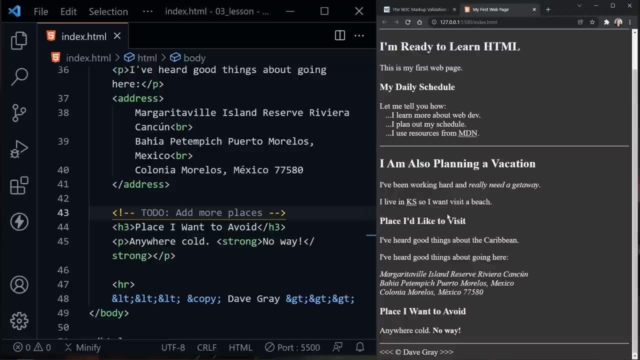 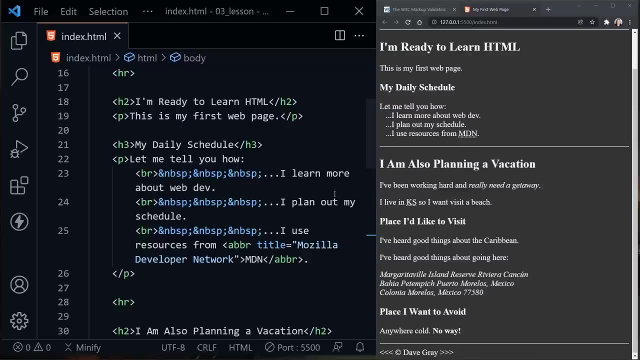 And live server is using a script element that we do not see on the page either And that can contain JavaScript, for example. So just to let you know, If you leave a note for yourself, it can be viewed by others. And finally, now that we've added all of this HTML content to our page, 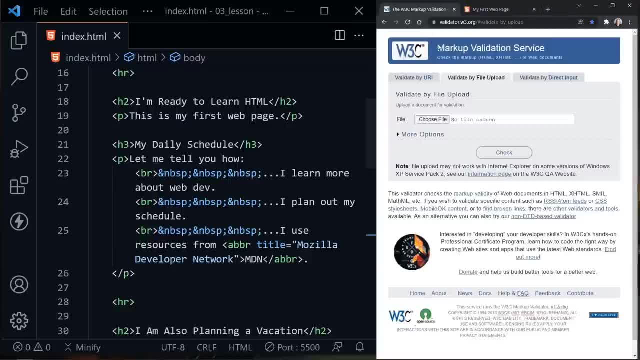 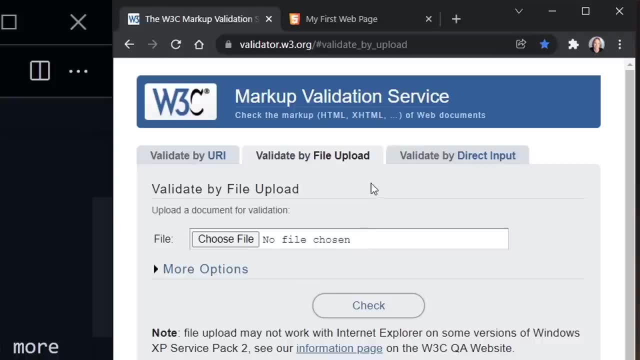 we once again should go to the validator markup validation service from W3C to check our file to see if it is valid HTML or if we have any mistakes. Choose validate by file upload And then click choose file. I'm going to have to probably go to a different folder from the one that I chose. 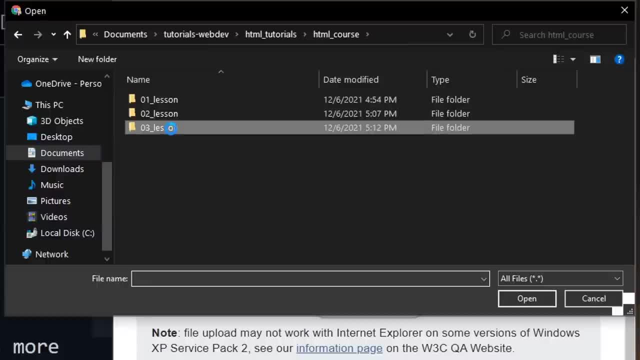 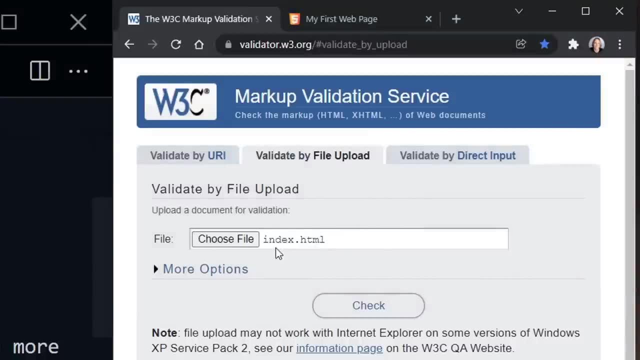 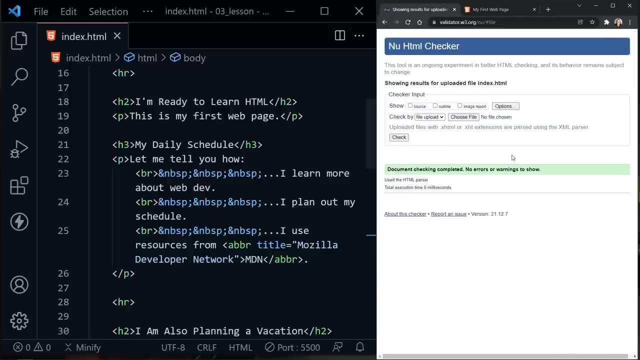 I checked last, So I'll go to HTML course lesson three, which is the file we are working with. Choose my indexhtml and open that here with the validator. Now it has the indexhtml file uploaded and we can click, check And we'll see if we have valid HTML. 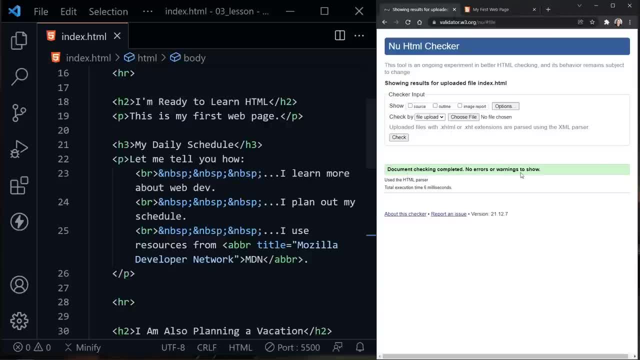 So this is valid. It's green Document. checking completed No errors or warnings. to show: If you have errors or warnings, it should point out exactly where that error is And you can fix that in your HTML. Let's look at how to create lists on a web page. 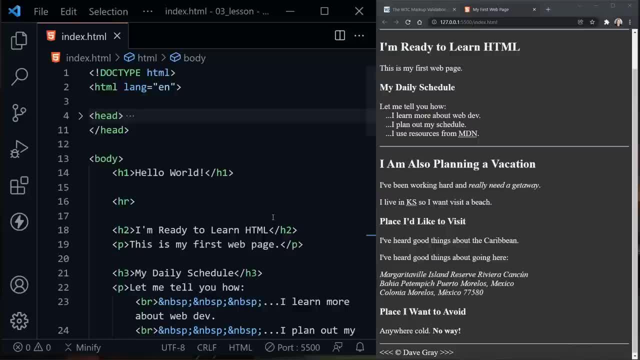 Lists are very useful and are used in many places on the web, So we have three different types of lists we're going to create today: Ordered lists, unordered lists and description lists. Let's start out with recapping. here. We've got Visual Studio Code on the left. 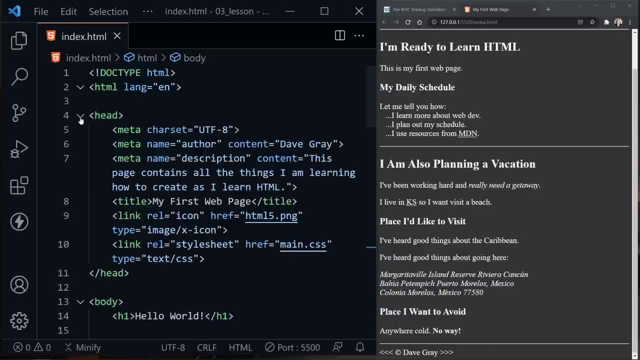 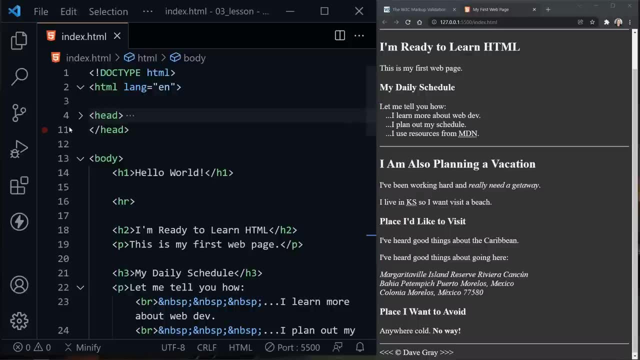 And I've got the head element collapsed So we had meta details inside of there. We can collapse that by clicking on the arrow by the line And you see lines between 4 and 11 are now collapsed. So we're working inside of the body element to add content to the page. 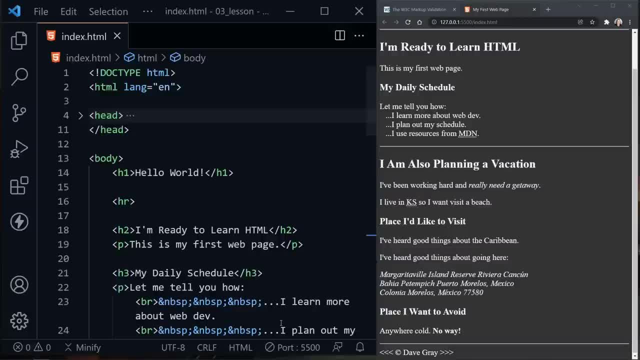 And this is Visual Studio Code and I'm running the live server extension. You can see down here. it says port 5500, click to close server. If you've installed the live server extension, it may say click to launch or something like that. 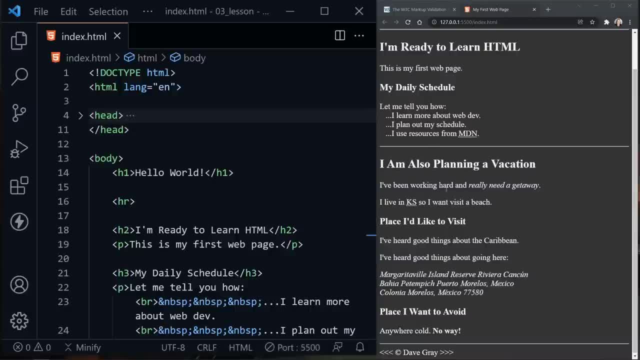 which would actually launch your web page for you, because that's how you want to view it In a development environment. You don't want to just go to file and open the file in your browser. You want to have that live server running that simulates a web server. 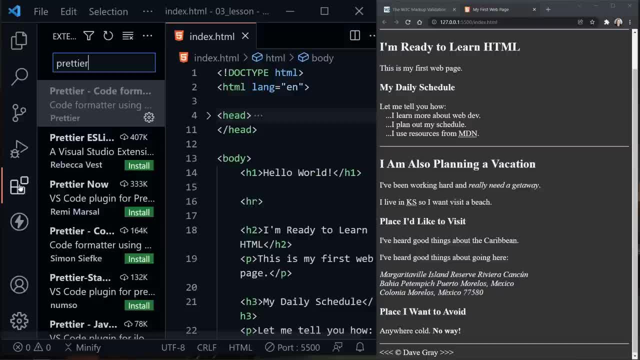 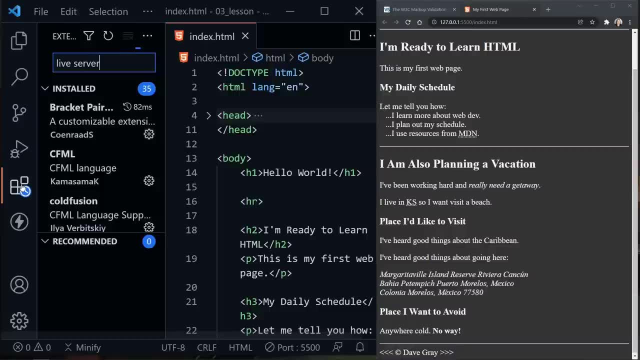 If you're not familiar with the live server extension, you can click on the extensions logo here And, instead of searching for prettier that I have in there, you can search for live server And you can install that live server extension by Ritwik Day right here. 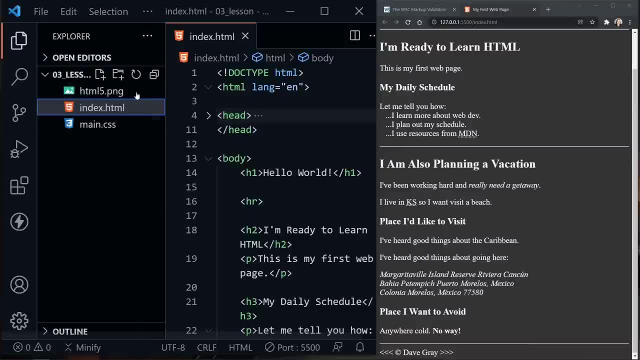 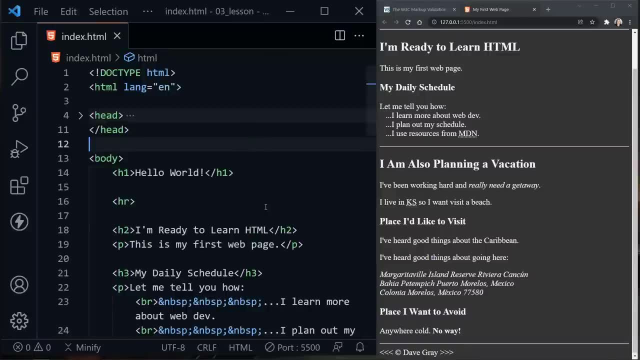 Okay, So We've recapped all of that. Here's the file tree with our files. I'm going to hide that by clicking the file explorer here so we can see more of our code, And we will add lists to our web page today. 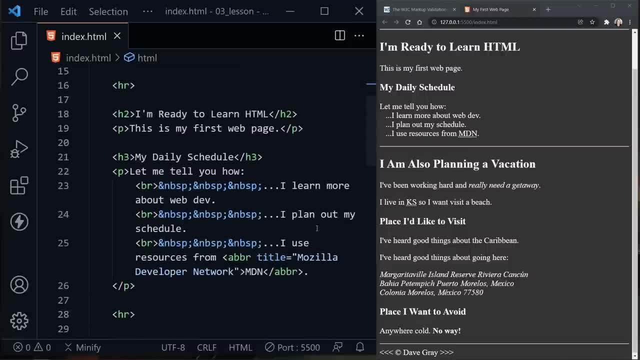 So I'll scroll down to under the subtopic of my daily schedule And notice how we had these line breaks and spaces here. Well, we're going to replace these. So I'm highlighting the first one And then I'm going to press control D. that highlights the next one. 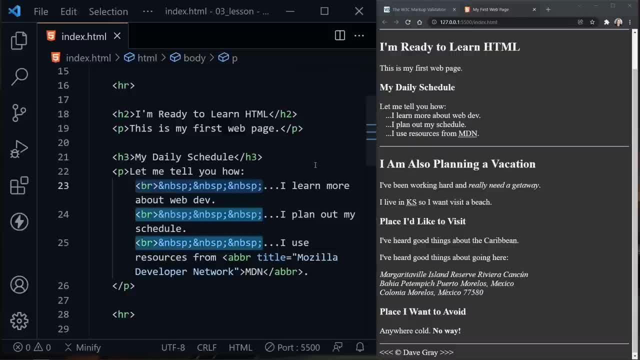 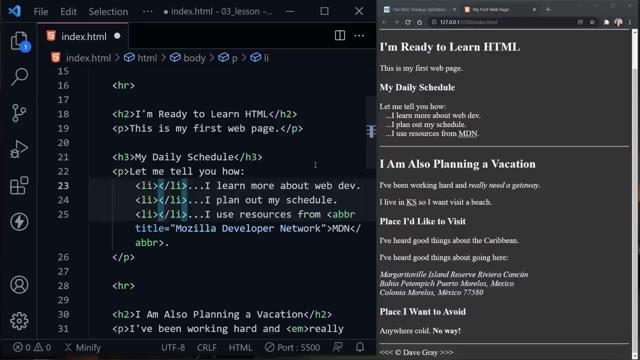 And control D again. Now it has highlighted all three of those And instead of this line break I'm going to type LI and press tab. That adds a list item. But we haven't enclosed this in a list yet And we definitely don't need the closing list items here. 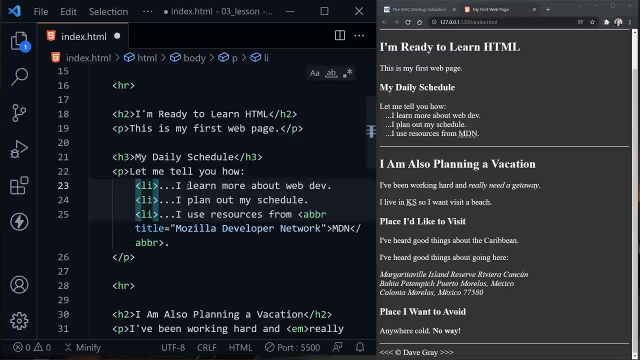 So, once again, control D, control D. So all three of these will be list items, But they need to be inside of a list too, So let's make this an ordered list by starting out with an OL And I'll press tab. 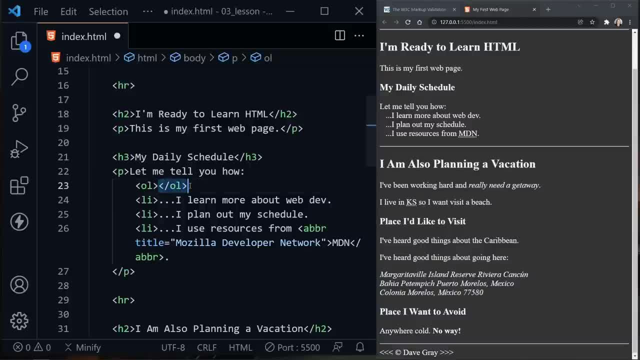 And we got the closing OL tag as well. That stands for ordered list, as you might expect, And I'm going to actually put the OL down here after the paragraph tag, The closing paragraph tag, And I'm going to cut with control X. 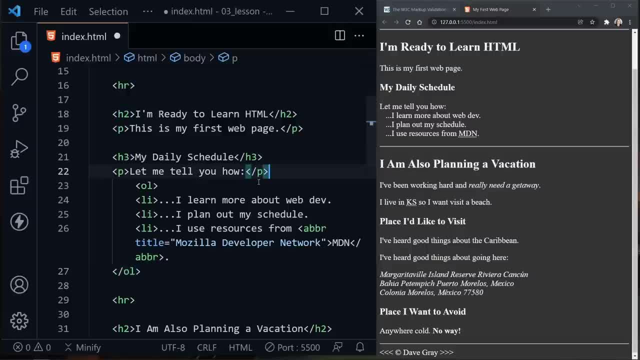 Or you could retype if you want to. And I pasted the closing paragraph tag right after the end of. let me tell you how. So this is a shortened paragraph now, And the list will not be inside of the paragraph. And now we have our ordered list. 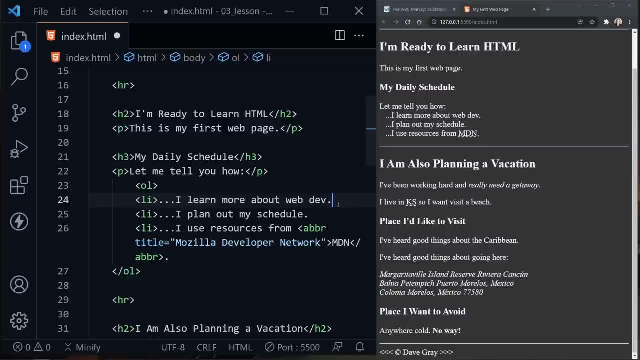 But it also needs closing LI tags. So I'm going to type the less than symbol and a slash And Visual Studio Code instantly filled in the closing- The rest of what is needed there- And I'll do that again for the second one. 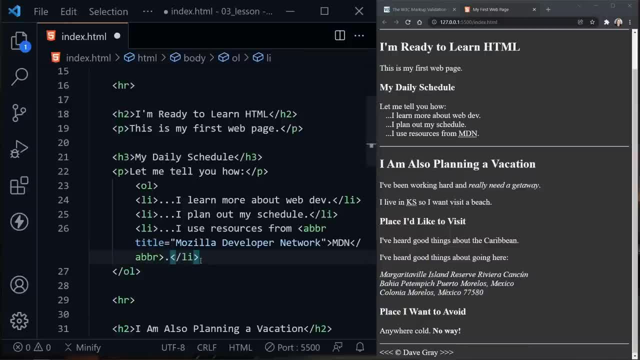 And then I'll do that here for the last one And notice we do have the abbreviation still nested inside of the list item here. So now I'm going to press control S and save And Visual Studio Code reformatted. that just a little for me. 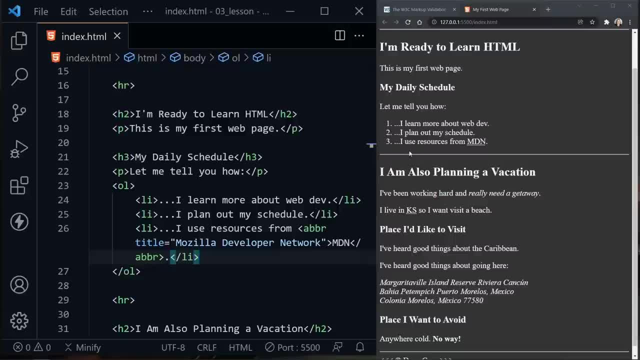 But look at our page now that we've added this list. It's an ordered list and it is numbered. That means it's in order: numerical order: one, two and three. Notice: these are not. this text is not enclosed inside of a paragraph element. 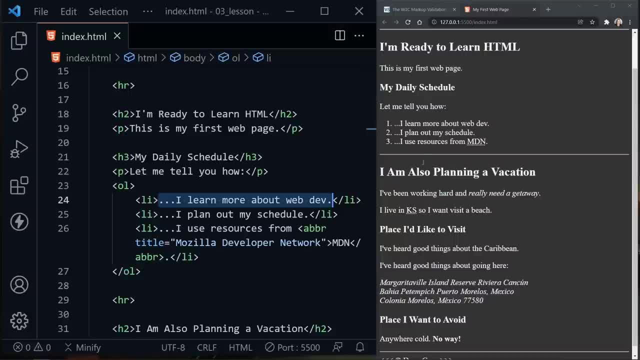 So it's not creating that extra space that a paragraph element does. They're stacked right on top of each other. There's still a little bit, A little bit of space, but not like we have between our paragraphs. So that is an ordered list. 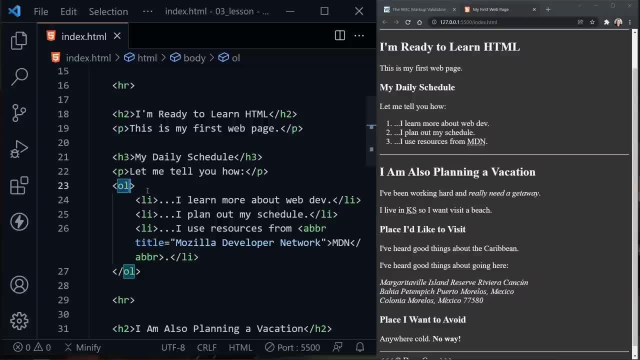 We start out with the ordered list element and then the list items go inside it And each list item is starting and then ending with the LI. Now let's scroll down and look at our vacation area. It says I'm also planning a vacation. 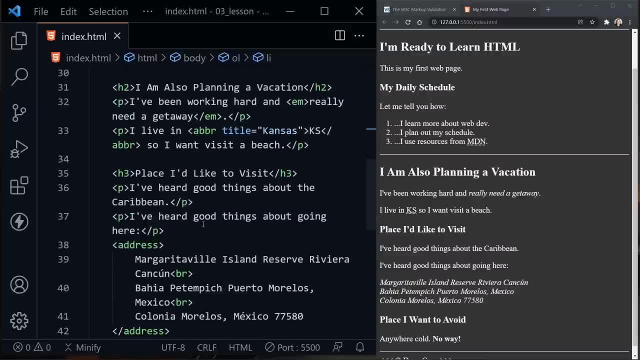 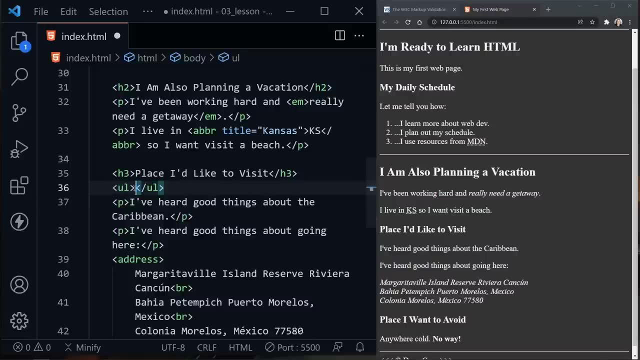 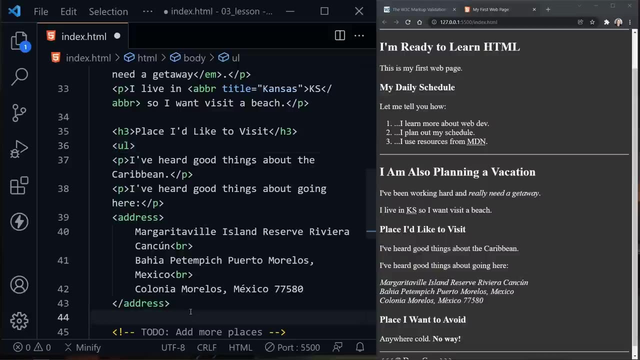 And we've got a places I would like to visit area. So after that, let's go ahead and add a UL, which, as you might guess, stands for unordered list, And we'll go ahead and cut that closing tag And I want to put it after the address here at the bottom. 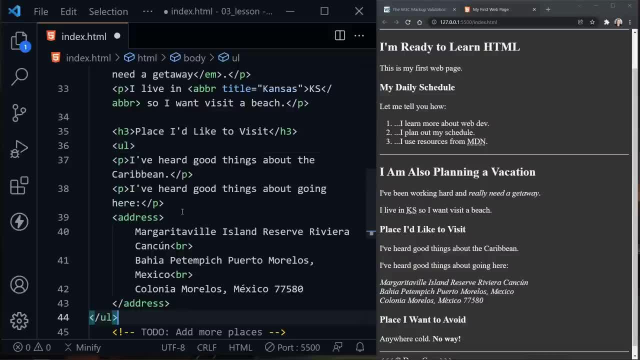 So this will be our full list. Now we need to declare list items here. In this instance I'm going to go ahead and keep the paragraph tags inside each list item, So we created an LI there And I'll use control X to cut and close that first list item. here for the first paragraph. 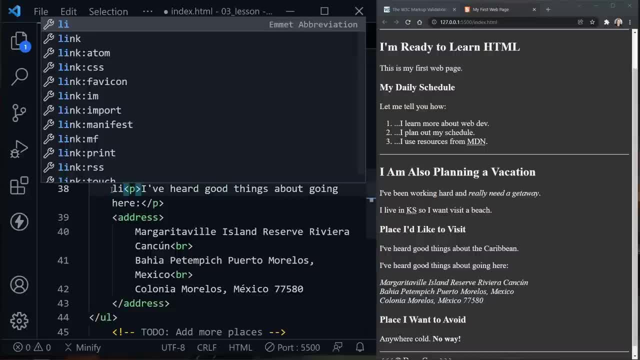 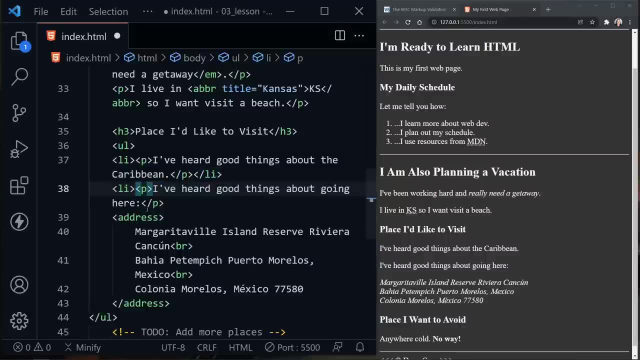 I'll do something similar here. Got an LI, but the closing one is going to be in a different spot because our list item can have these tags nested within it, just like we nested the paragraph here. I'm going to go ahead and nest the paragraph and the address inside of the list item here. 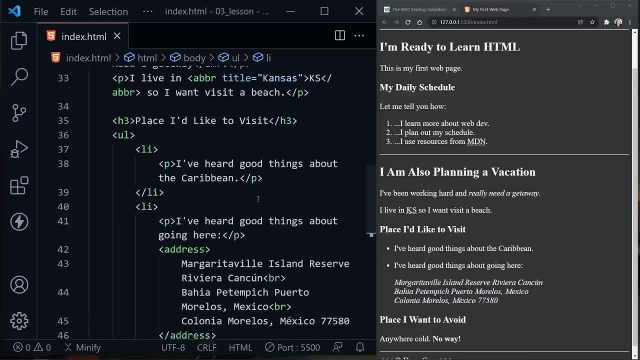 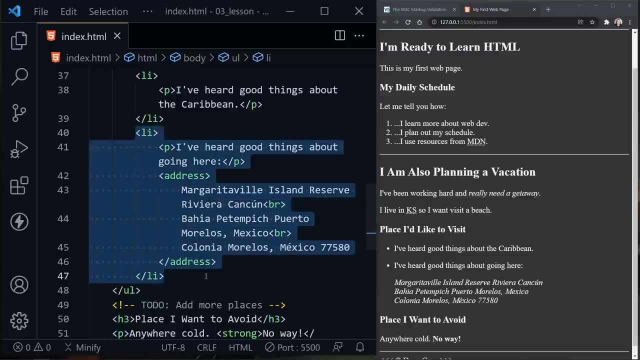 And so now if I save and Visual Studio Code reformatted my code for me, I notice here's the beginning of the list item And we're going to save it And we have the end way down here after the address. So let's look at what this unordered list looks like on our page. 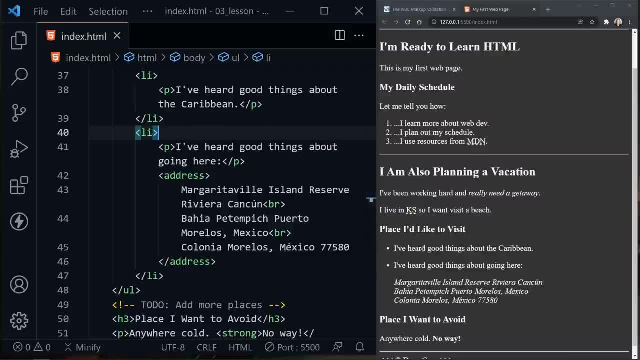 And you can see, instead of numbers it has dots. It does have the extra space created by the paragraph tags And the address element still has the content that it had before and still formatted the same. But notice, our ordered list and our unordered list are both indented. 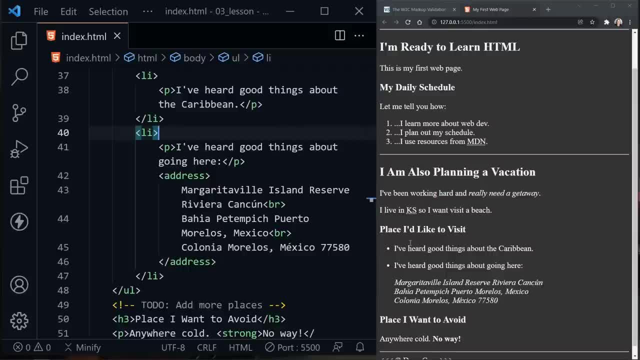 compared to being over here, flush to the left with everything else we had, Like they were before, So similar in formatting from an ordered list to an unordered list, And also realize that the really the only difference is the bullet point here in an unordered list. 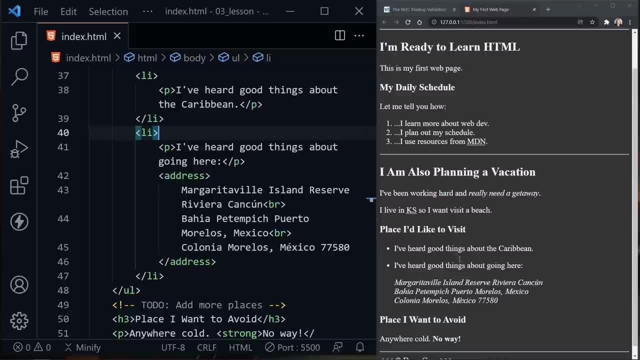 versus the number in an ordered list. The extra spaces were caused by the paragraph element inside of these unordered list items And we did not use a paragraph element on these ordered list items. So the list itself and the list items themselves and the list items did not create the extra space that was created by the paragraph elements. 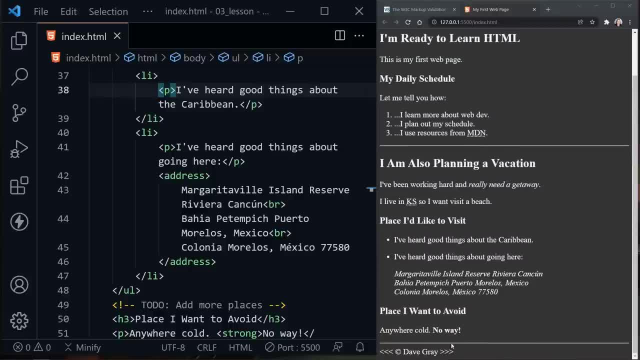 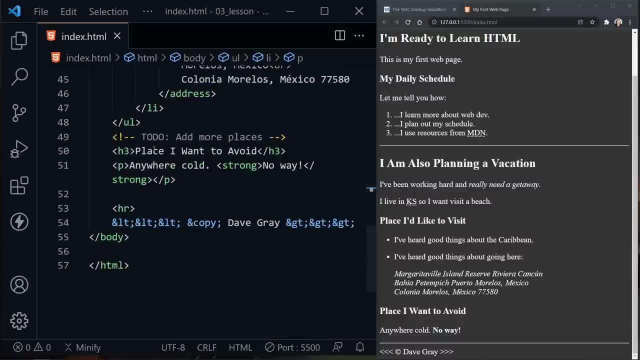 Now let's scroll our page. We've got enough content. We need to make sure we're visiting the very bottom here. We want to add more under place I want to avoid- And I'm going to change that to places I want to avoid. 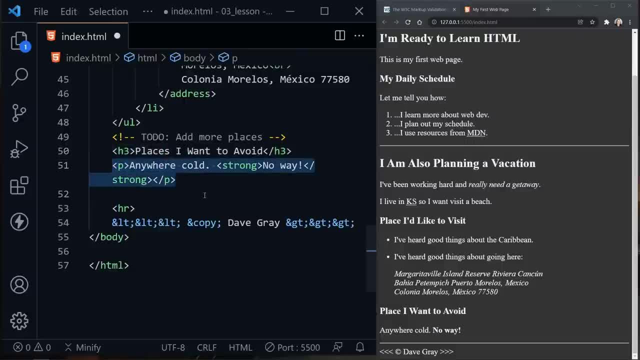 And let's go ahead and remove our paragraph that says anywhere cold, No way. And let's add a description list here. So a description list, as you might guess, starts with DL. Now, inside the description list, there are two different types of elements. 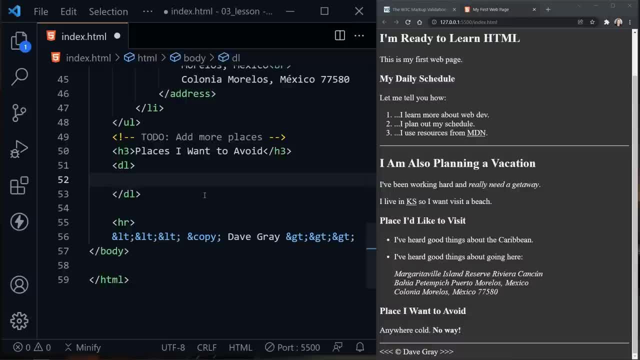 Instead of just an LI, like we had in our other lists. for a list item, we have a description term, And this description term could be the place we want to talk about, So let's say the North Pole. And now for the description term. we need to also have description details. 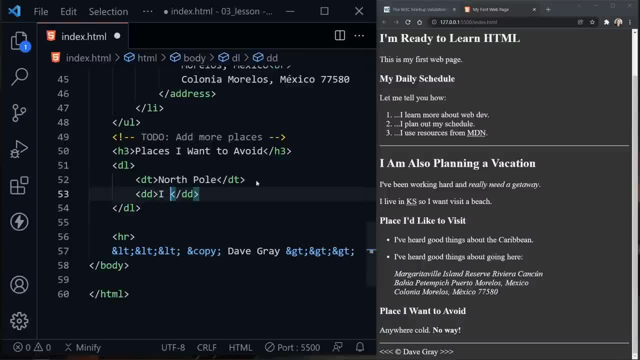 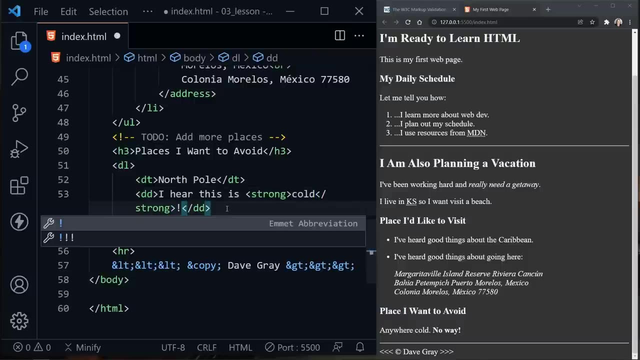 So that's DD, And here I can put. I hear this is Now let's go ahead and put our strong emphasis back here And I'll put cold And then our exclamation mark. So we have put a strong emphasis on cold. 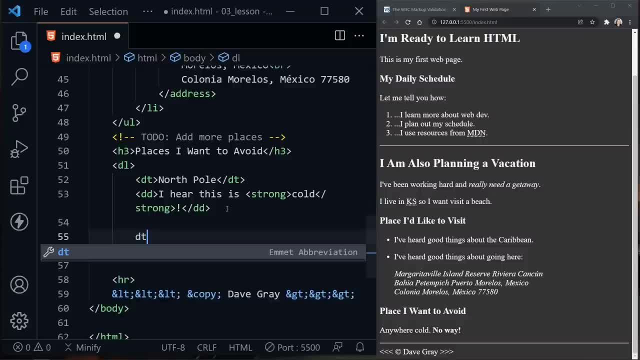 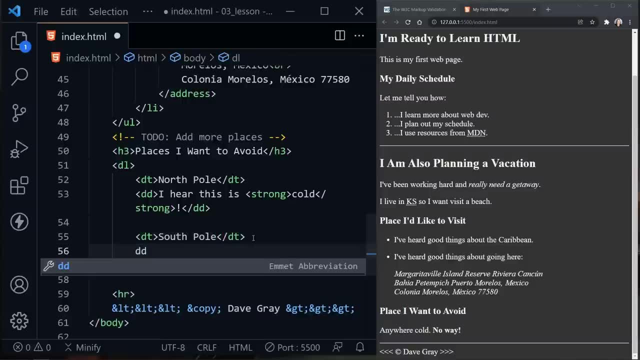 And now I'll create an extra line here just to space these apart. Another DT: I'll put the South Pole And then DD for the details, description, details, And I'll say: this is also cold, And let's add one more. 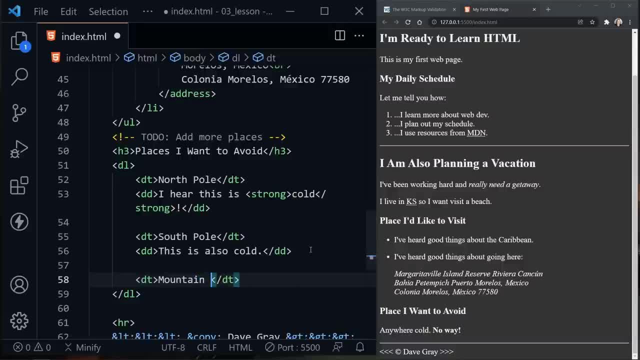 Description term, This will be mountaintops, and DD for description details, And these, if I spell these, these are also cold. Now, if we save, let's scroll just a little bit more so we can see all of our content here. 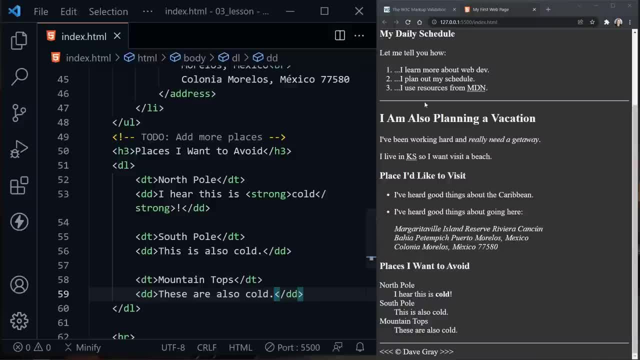 You can see our description list has a different format than the ordered list and the unordered list. Our description term is to the left And then the description details are indented to the right. But here is our full list of the North Pole, South Pole and mountaintops. 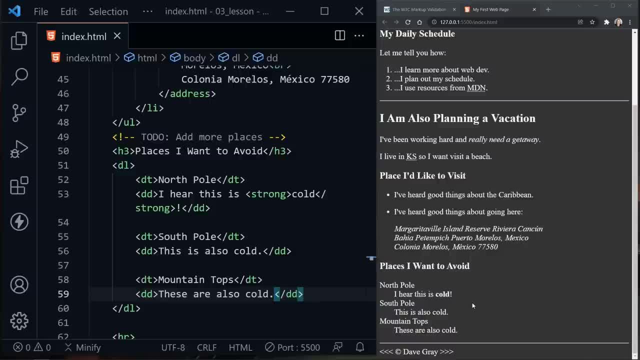 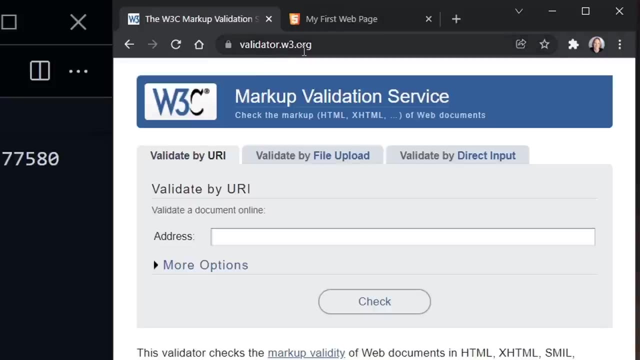 We want to avoid all of these places when we go on our vacation. With these new lists now added to our file, let's go ahead and create an error on purpose, just to see if we have an error in our page when we check it at our validatorwsuedu. 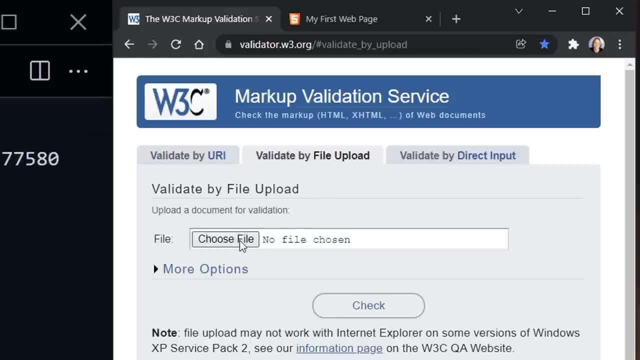 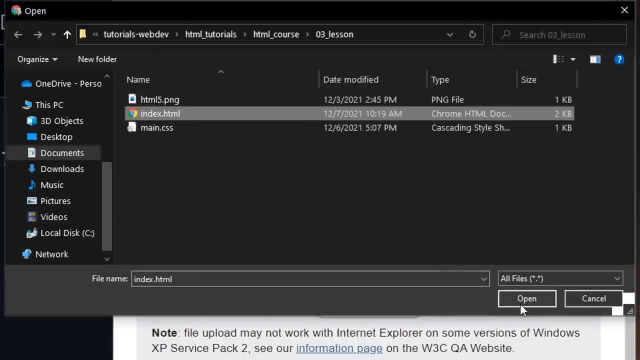 And here I'm going to choose file upload, And I may have to switch folders. Let's see. No, I'm in the right one, So I'll just choose index.3.. I think we're on lesson four and I forgot to change the file. 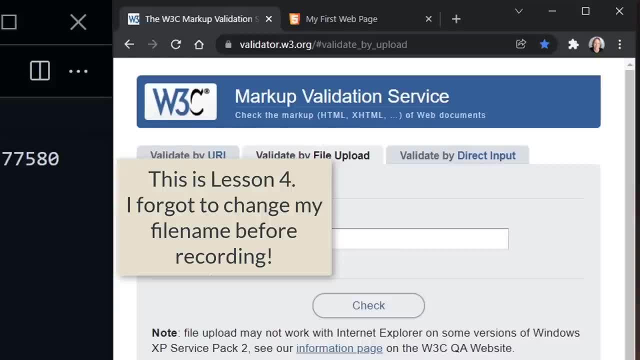 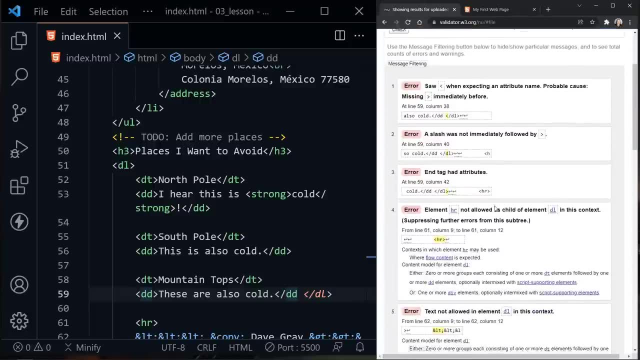 But I'll do that to make sure that the GitHub repo with all the source code is correct. So let's go ahead and check this file. And yes, we have some errors, because we created one specifically. Let's see if that's our fault. 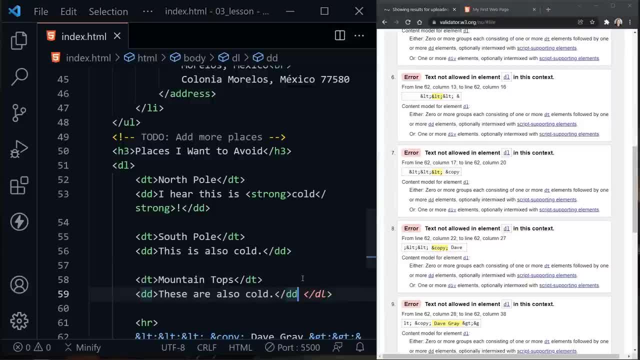 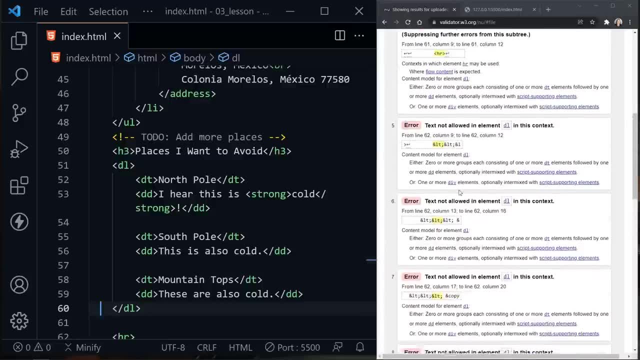 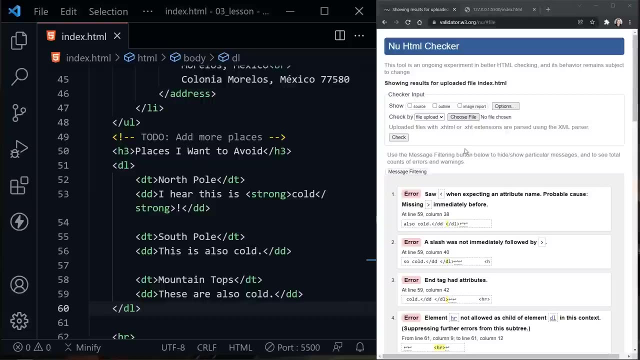 This is our only error. As we have noted in the past, one error can create a cascade or a lot of errors. So now I've formatted this correctly, Let's go ahead and load our file back up. So we'll choose file. 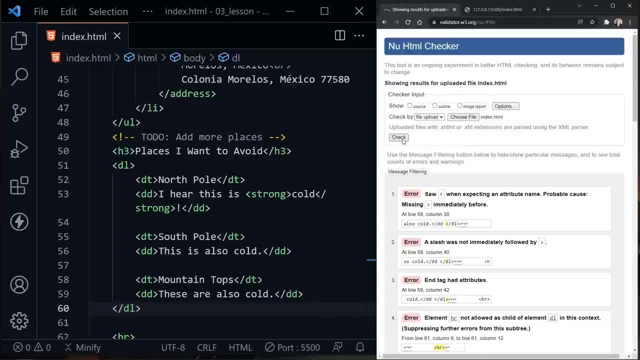 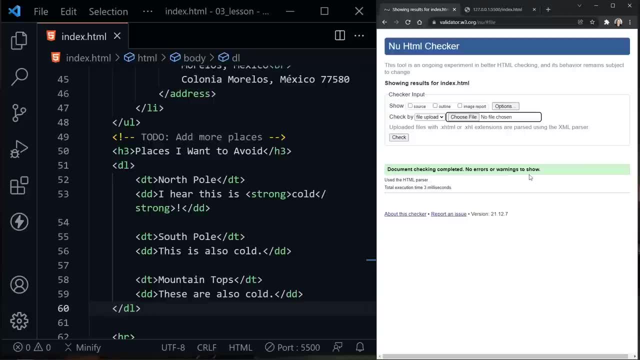 We'll choose that indexhtml file again And I'll click check. Now everything is okay. Document checking complete. No errors or warnings to show. So realize if you have an error it could just be one small syntax error that creates a cascade of errors when we're checking. 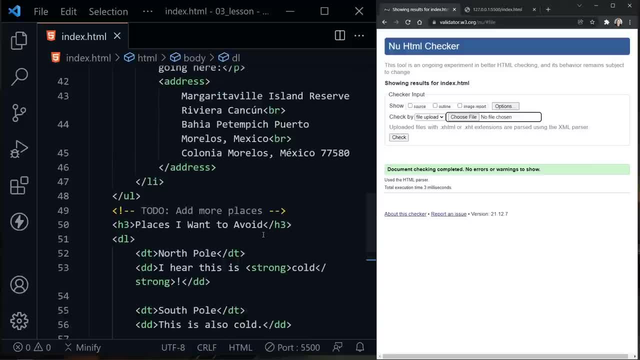 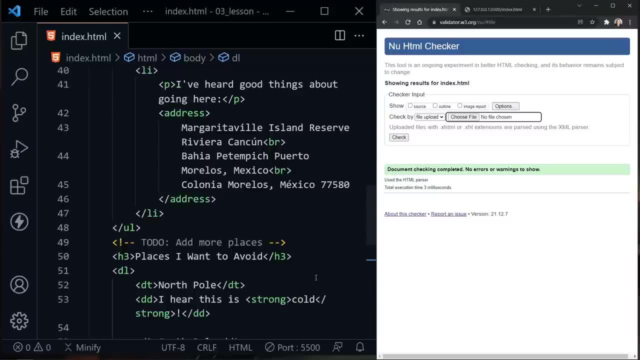 But this is a great way to learn. and, of course, look at the details of the code- And it's always a good idea to validate your code after you write it to make sure you don't have any syntax errors. Let's move on to creating links on our web page. 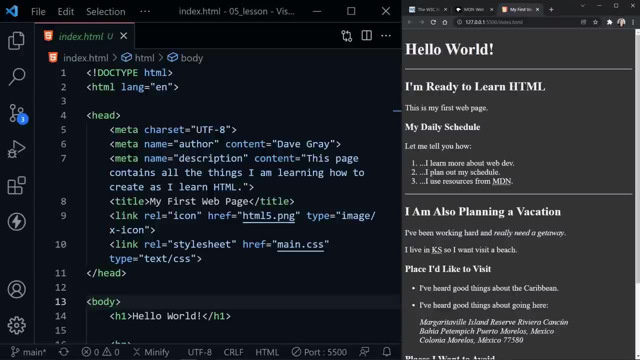 Hypertext is the HT in HTML And it's what links together everything on the web. It's really what makes the web work so well. Think about Spiderman or really any type of spider that's throwing out strands of web and linking things together. 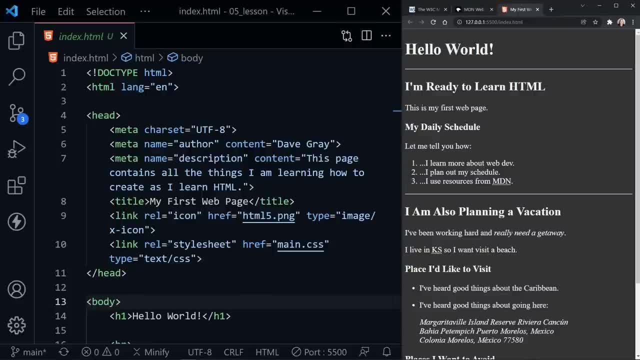 That's essentially what we're doing. when we create hypertext links, We're linking the web together. Now, as we say link, there can be some confusion Because notice here in Visual Studio Code on the left that I've got link tags that we created in the head part of the page. 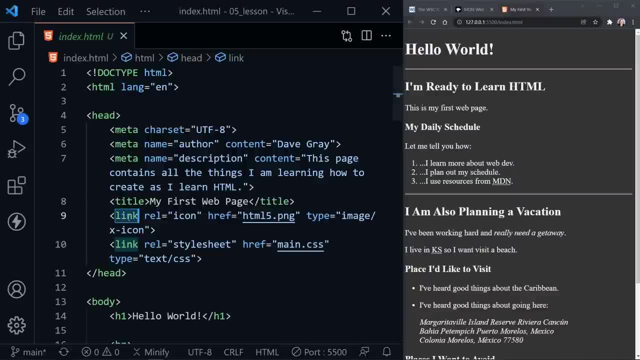 That's from lines 4 to 11.. And these link tags are pulling in resources from other parts of the web, Whether it's something we have on our server with our web page, like this fav icon, Or we could pull in something from another part of the web, like a font from Google Fonts and things like that. 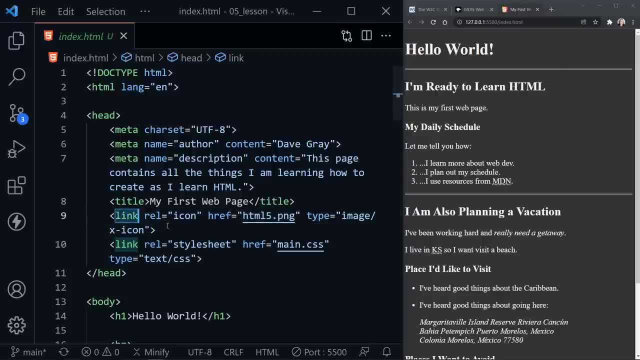 Which we haven't done yet, but it's possible with the link tag. But that's not what we use to link pages to each other. I'm going to collapse this head section by clicking OK, Clicking on the arrow over here by number 4.. 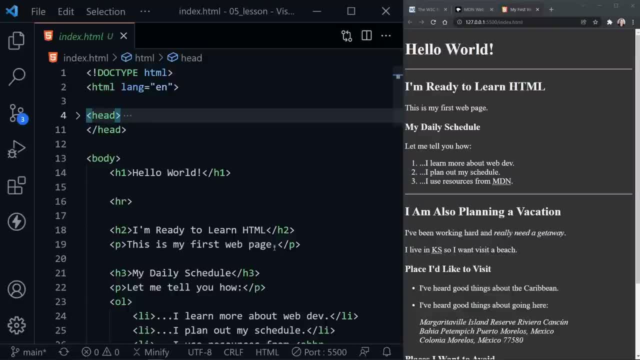 So we have a little more room And now we're looking at the body area in Visual Studio Code. By the way, I'm running the live server extension and have our page from our starter code. that's available for download at the GitHub link in the description. 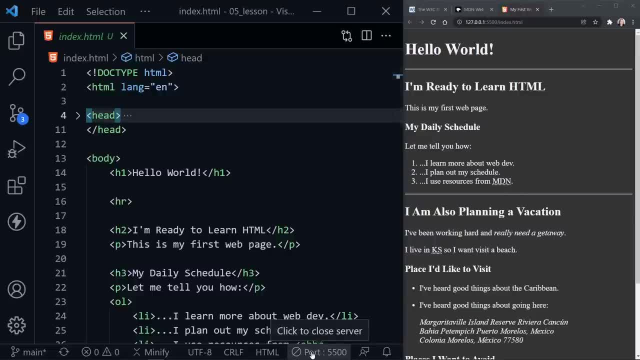 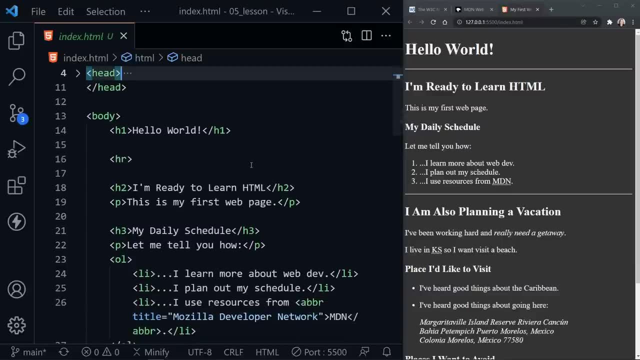 And I'm running that with the live server. You can see it running here. It says click to close. the server Shows port 5500.. OK, In Visual Studio Code let's scroll down a little bit And let's add what is called an anchor. 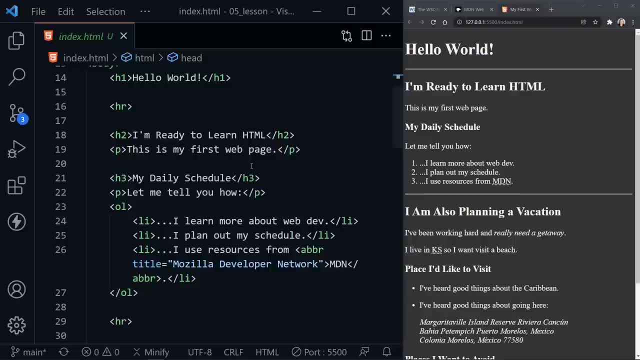 An anchor tag that will create a link to another page on the web. So in our list, where it says: let me tell you how- And we're talking about the different things we do to learn web development- We have an abbreviation for the Mozilla Developer Network. 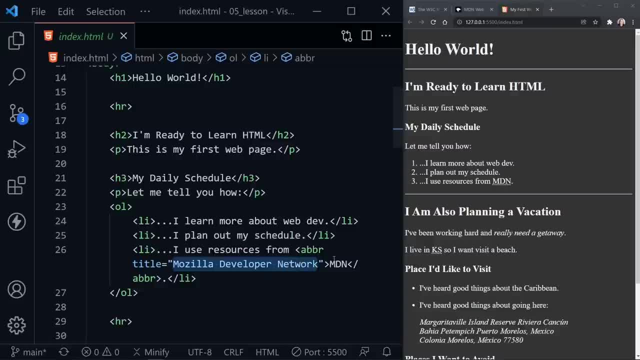 Maybe this would be a good place to go ahead and link to the Mozilla Developer Network And we can insert a link around this MDN abbreviation inside the inline element. that is the abbreviation element. So I'm going to press enter here to start a new line. 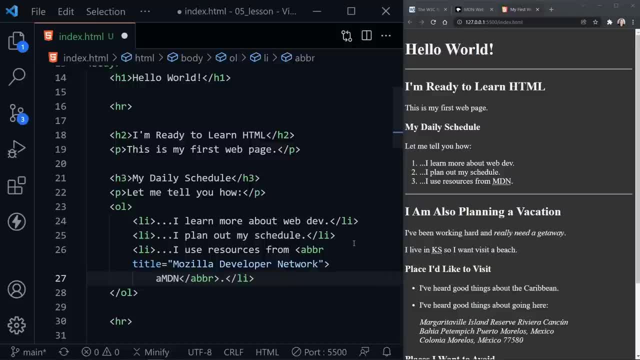 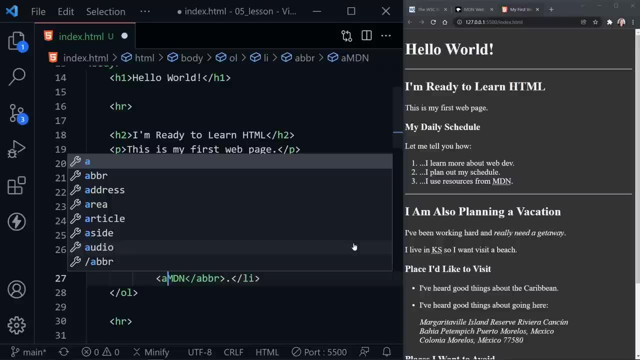 Now I'll just type A, And this is well, I guess, because it's followed by MDN. it's not doing it, So I'll start out with the less than sign and then A, And this is the anchor tag that I'm starting. 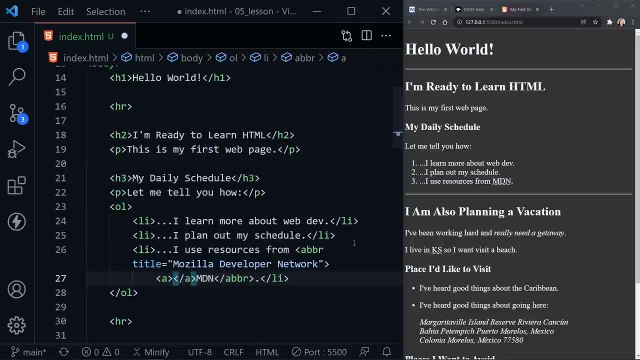 But by itself, if we just put the anchor tag, while you can do that by itself, it will not link to anything. It needs a specific attribute that tells it where to go. So I'm going to press enter here And we have it surrounded by this anchor tag. 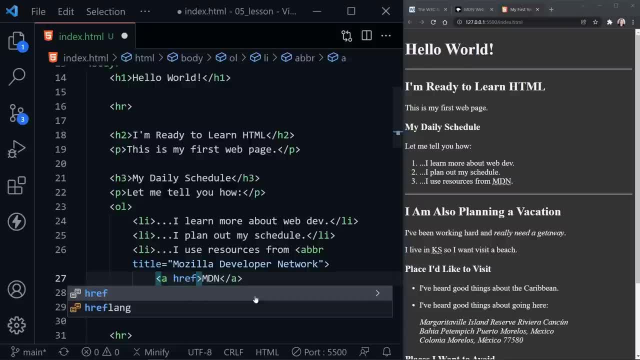 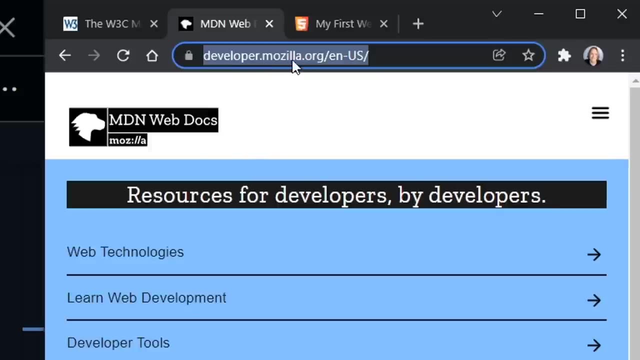 We need to add the href attribute, And now we're going to reference an address on the web, So this is where we would put that address in, Over here in the Chrome browser. I have the Mozilla Developer Network open. We can see up here at the top: it's developermozillaorg. 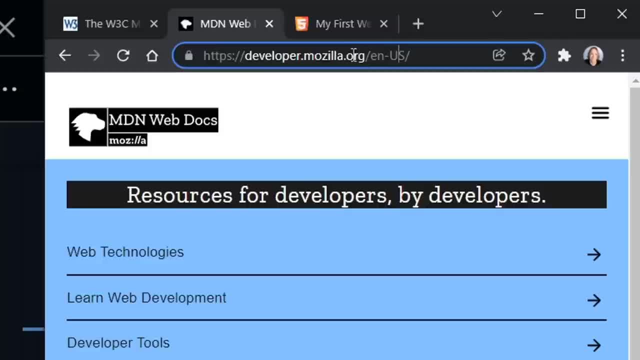 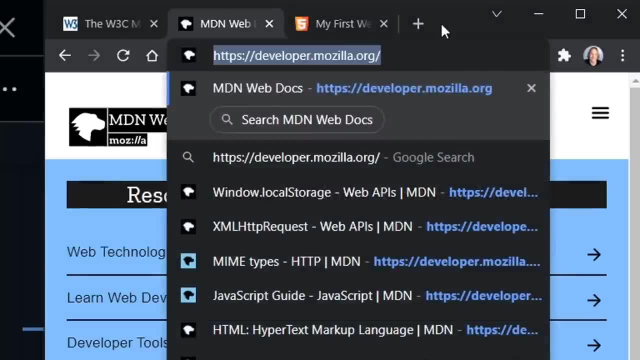 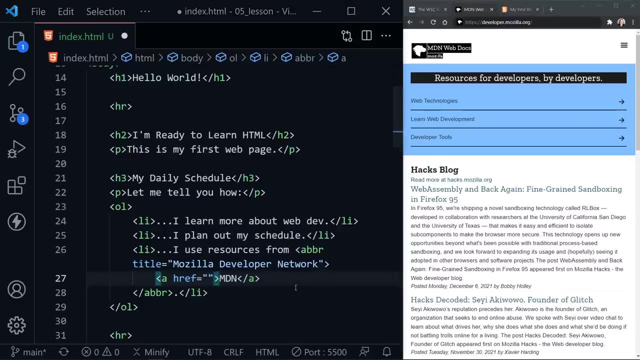 And then there's a slash after that that gives the specific language for the site. I believe it will default to the browser, So I'm going to remove that part, Go ahead and select the rest, And now that I have copied that with control C, I'm going to click here inside of Visual Studio Code and put that address right inside the href attribute. 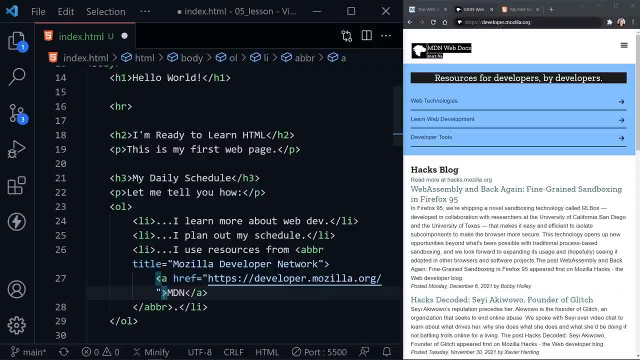 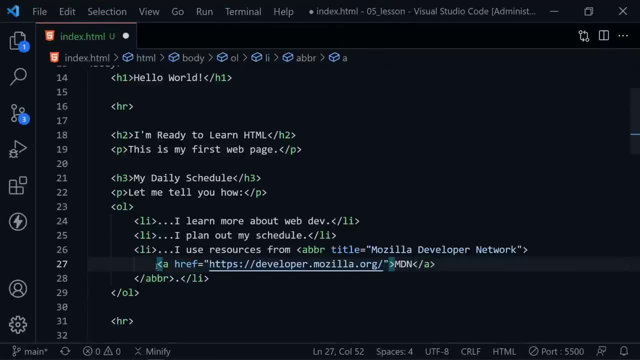 Now I am wrapping the code down to another line so you can see it all. It doesn't go off the screen. I could expand Visual Studio Code here And now you can see the full address without that line wrapping. So we're linking. 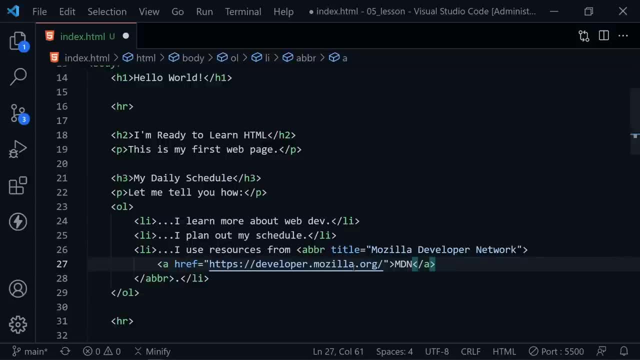 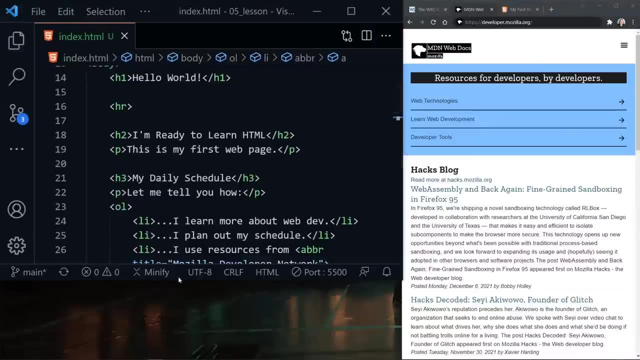 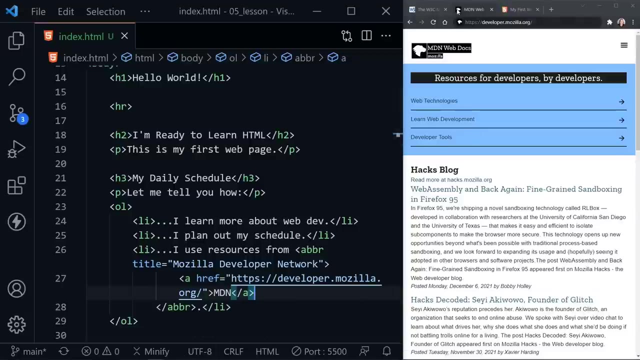 We're linking to the developermozillaorg website with this link And we can save this. And now I'm going to go ahead and bring Visual Studio Code back to the size I had it. The code lines will wrap. But if we look at our code or our page in Chrome- that should have now updated because we're using live server- you can see we have a link. 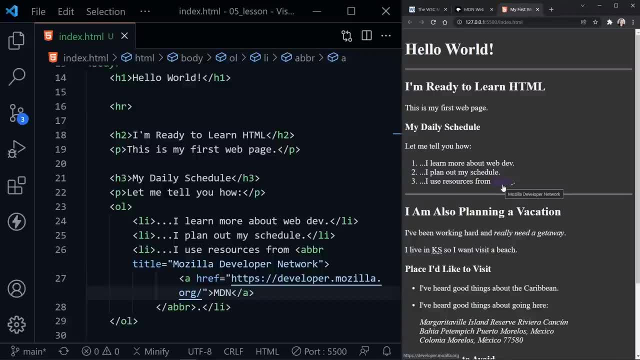 And it turned purple. It's a little hard for me to see right now, but we can change that color in just a little bit. But that purple means a visited link. If you have not visited that site, it's probably more like a royal blue or a bright blue color. 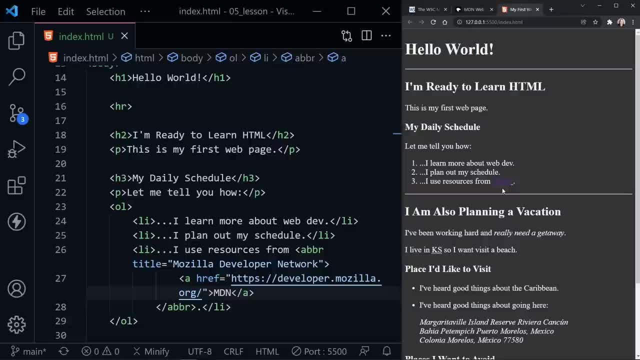 And that means it's not visited yet, And those are the default colors for links, But something about this link that we need to acknowledge. this is the full address to that website And it's a specific address. This is what you would call an absolute reference. 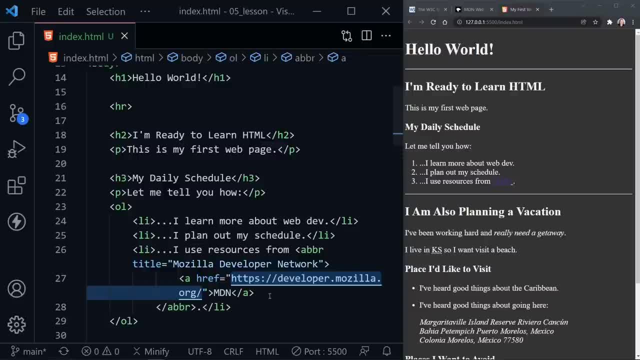 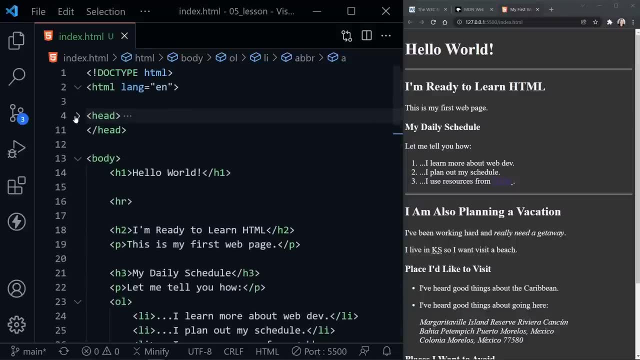 This has the full address for the web page to where we're going. But when we link to something that's already on the same server as our page, where we're hosting our website, then let's go ahead and expand this head section again. 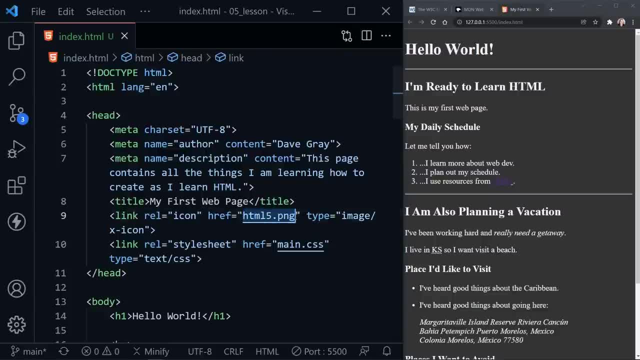 Notice we're not giving an absolute reference. We're giving what's called a relative reference. Right now we don't even have a slash here because we know this HTML5.png file is in the same folder as our indexhtml file And the same with this maincss file. 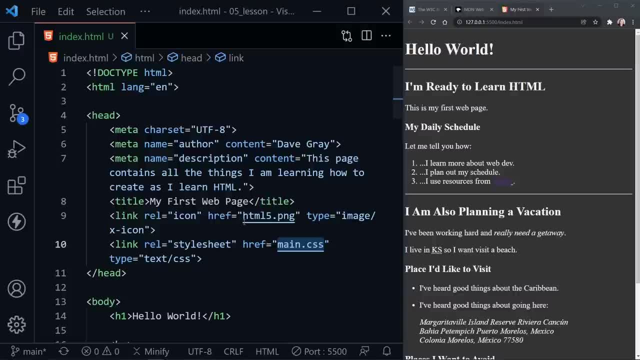 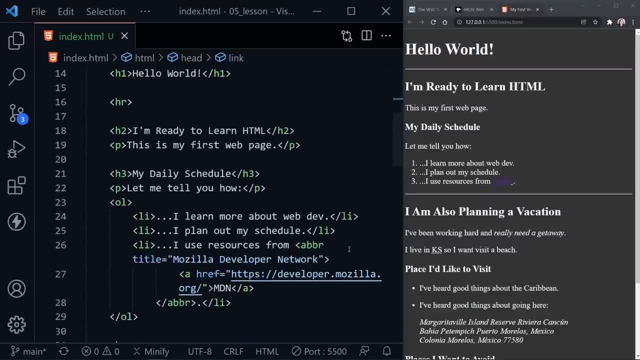 It's in the same folder, We don't even need to provide a slash. It's not in another folder, even. But it is a relative reference And that's the difference. So we have an absolute reference here to a place on the web. 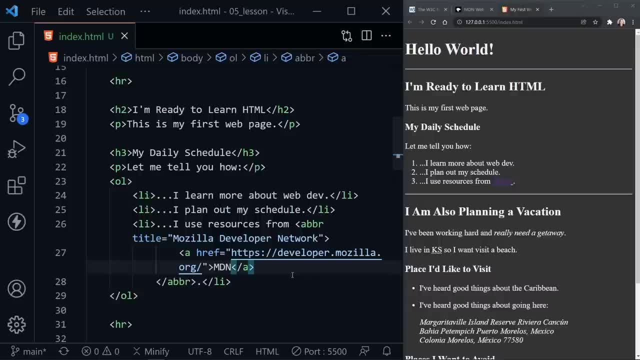 And then we can provide a relative reference to something that's on the same server that we're on. So now let's go ahead and create a relative reference to another page, And I'll scroll down to do this. We haven't created the page yet. 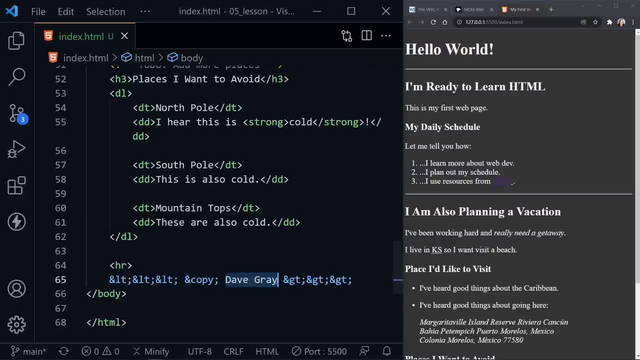 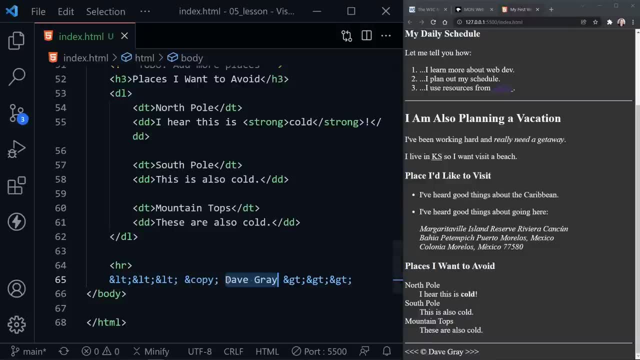 We'll do that next. But if you have your name here here at the bottom I have my name, Where we have the copyright symbol And in Chrome I can scroll down and we can see this at the very bottom. Let's go ahead and link with a relative reference. 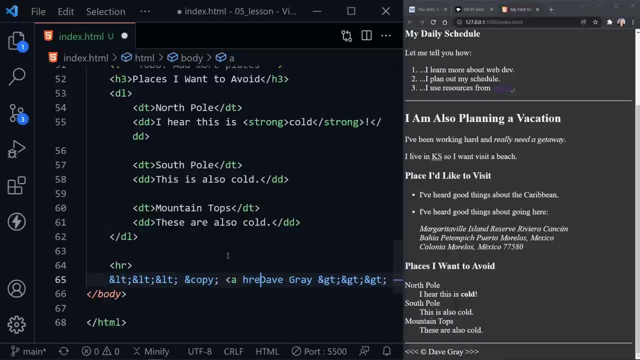 So I create that anchor tag, that a tag, And then href and equals And let's link to abouthtml And notice I'm putting quotes around that file name, just like I did for the full address in the absolute reference above. And now I want to put my name. 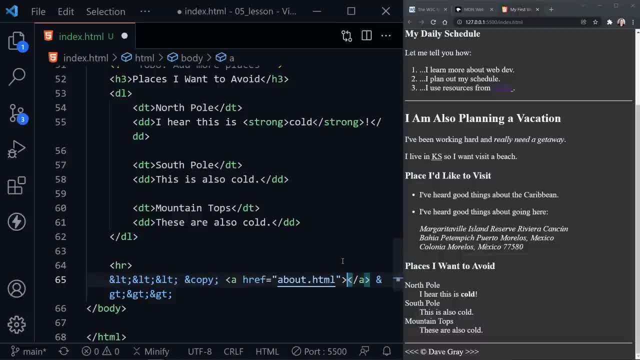 Of course, between the opening and closing anchor tag, And now that will link this to the about page that we haven't created yet. I'll save And notice now. this is that bright blue or dark blue that I was mentioning earlier, A link that has not been visited. 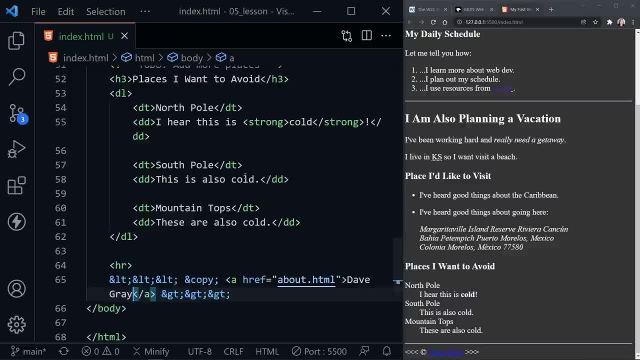 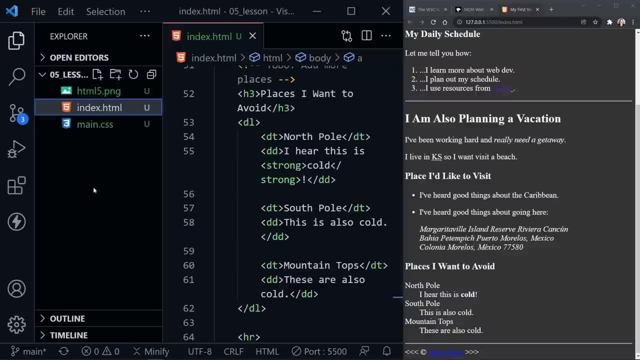 This page doesn't even exist yet, So we need to create this page. If you don't have the file explorer open in the top left of Visual Studio Code, you can click that And you'll see the files that we have here in the file tree. 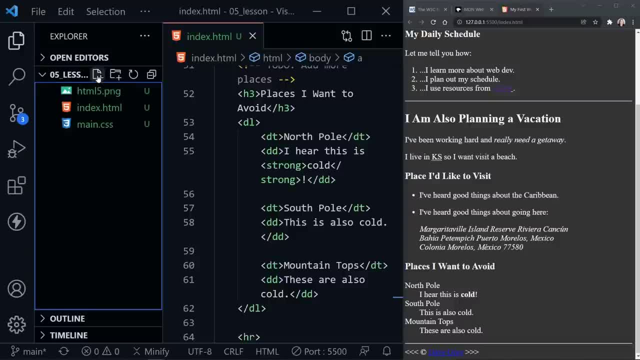 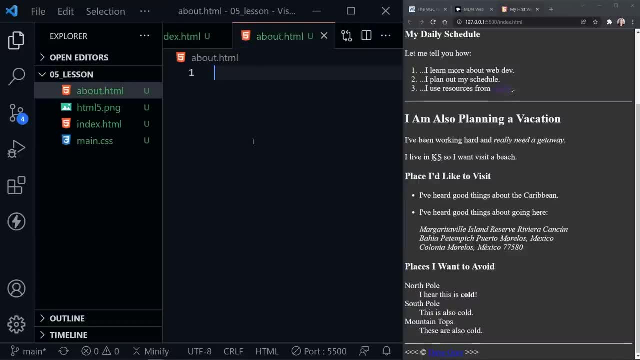 What I want you to do is click on the new file icon. Name this page abouthtml. Now, this is a good place to go ahead and pause the video. You can click on the file explorer tree over here- The file explorer- to hide the tree if you need more room. 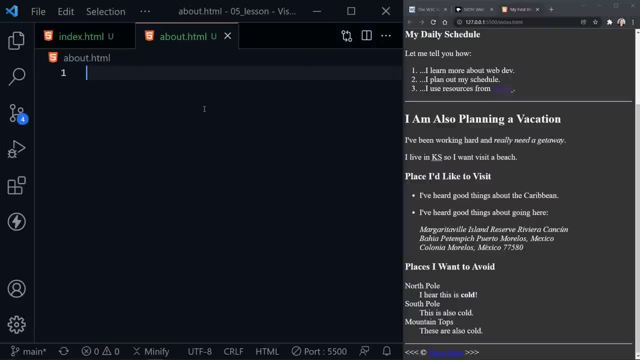 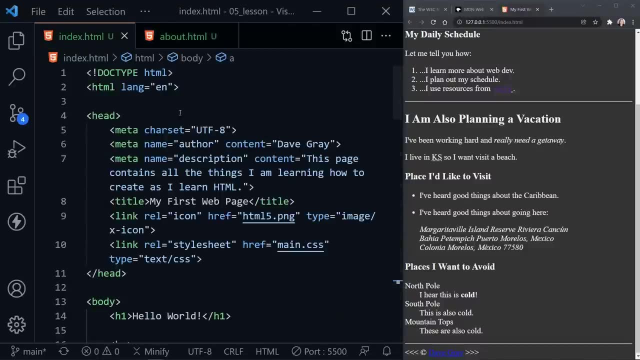 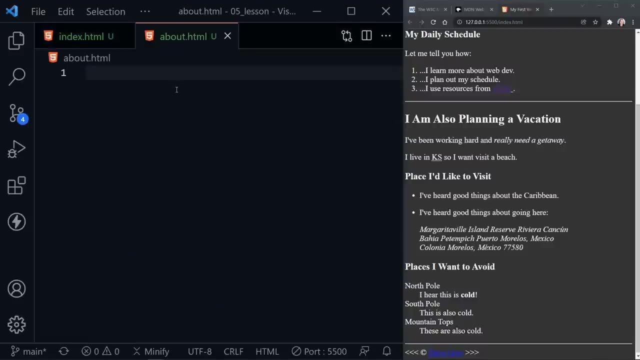 But go ahead and create an about page. You know everything we've already learned from the indexhtml page, So what I want you to do is pause the video, Create your own abouthtml And then come back and I will create one with you. 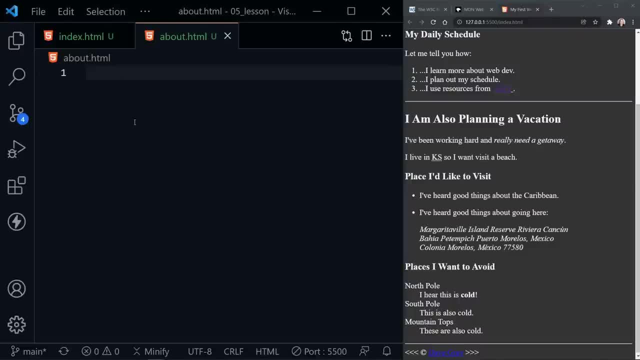 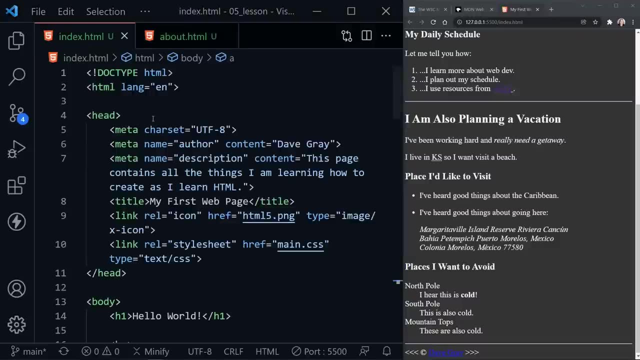 Okay, I hope that went well for you. I'm going to help you create an abouthtml page now, Or you can watch how I do it and compare to what you did Now. I've been doing this for a long time And I'm going to take a few shortcuts so you don't have to see me type everything out. 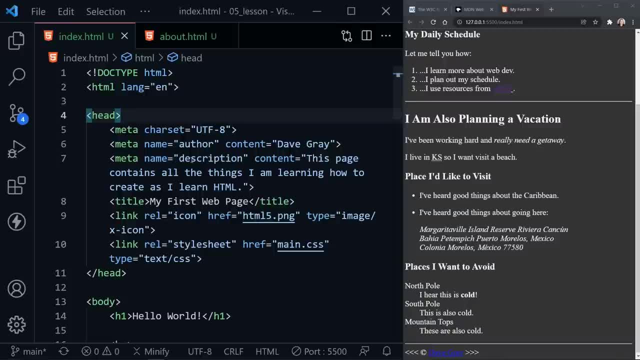 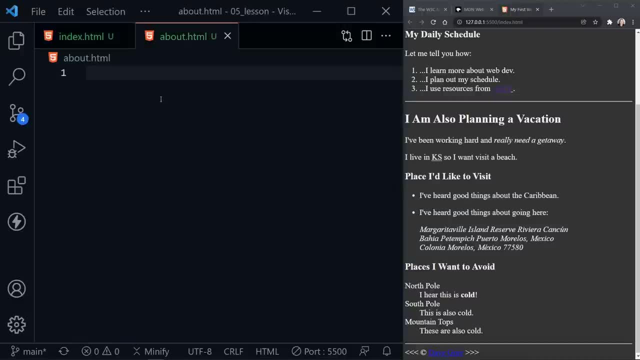 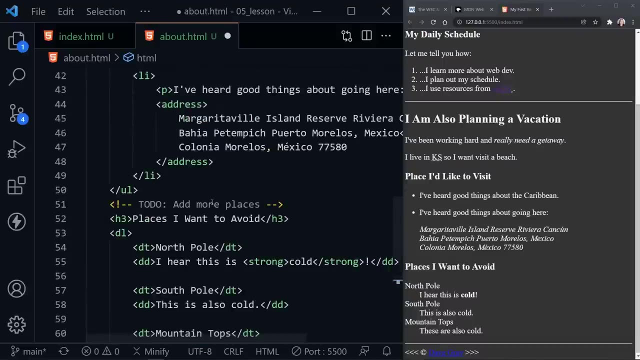 I'm at the indexhtml page. I'm going to press control A to select everything, Then control C to copy everything. Click the abouthtml page again And I'm going to paste everything in with control V. Now, as you're learning how to do this, I think it's important that you type everything. 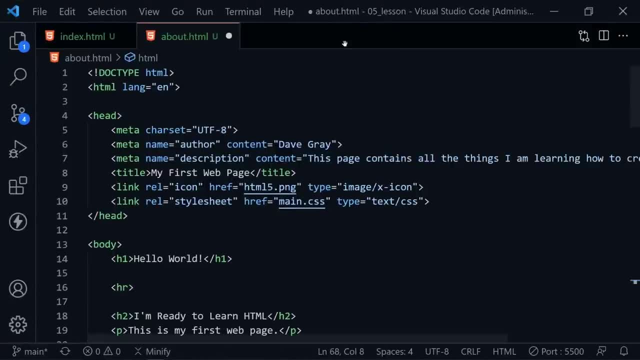 But I don't want to take up your time by having you watch me type everything out, So I'm just going to make some changes here. The doc type is the same, The HTML element is the same And, of course, we have a head section. 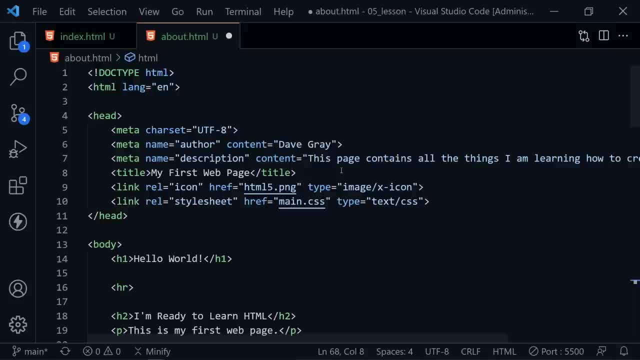 The meta tag for the character set is the same. The author is the same. Now this description meta tag Right here on line 7.. That could be just a little different. I'm also going to press alt Z to get this page to wrap lines that are longer. 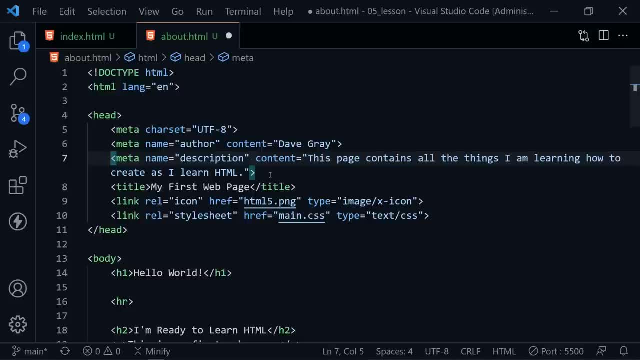 So now you can see line 7 wraps down to a second line here And we see the space to the left. Now in this description I can change this just a little bit And I'm going to say: hi, I'm Dave Gray. 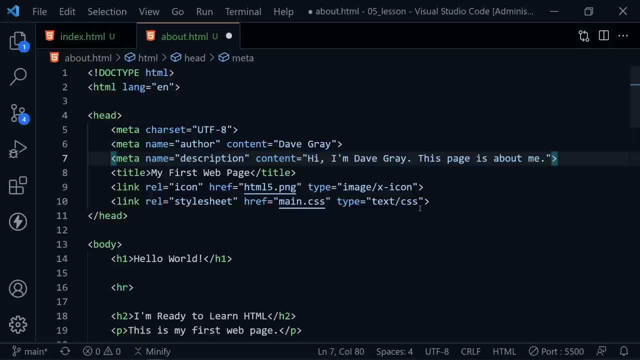 This page is about me, So we've given an accurate description for the page now And instead of my first web page in the title, I'm just going to call it about me in the title, And now we still can use the same fav icon. 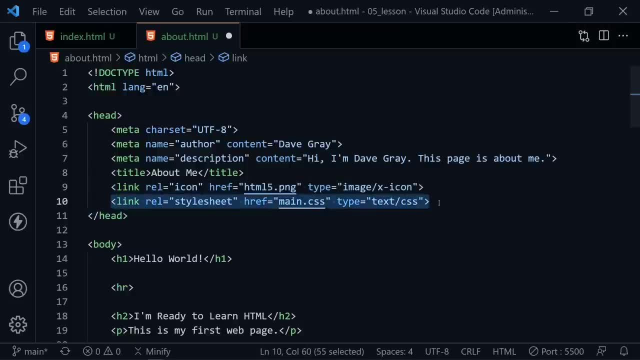 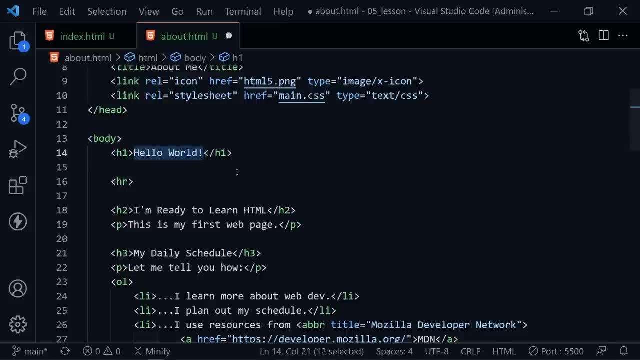 And we're going to use the same style sheet, So this page will look like the other page as far as the styles. And now we can change the heading for the page. And here I'm just going to say: hi, I'm Dave Gray. 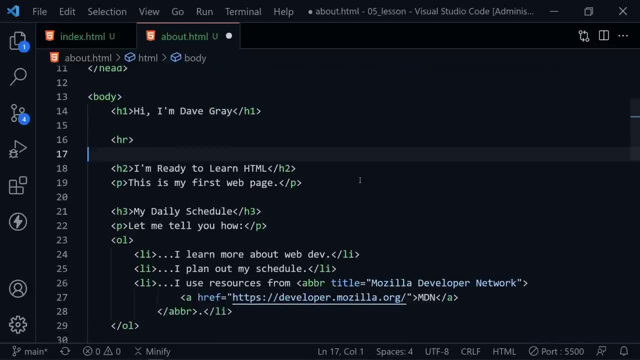 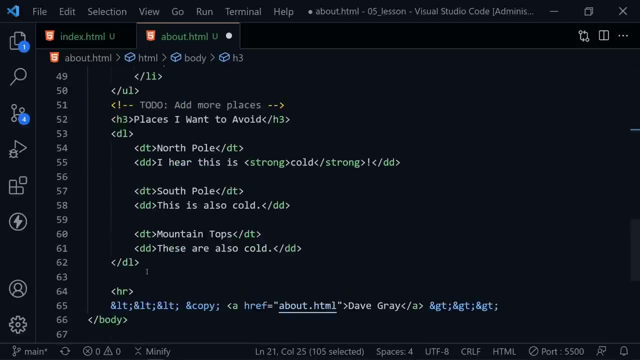 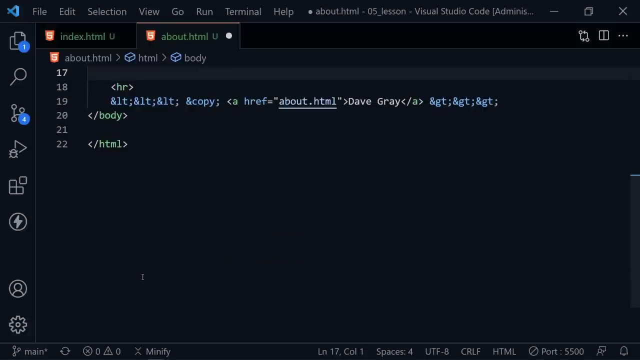 After that, I'm going to eliminate most of what we see Here on the page, So I'm going to highlight everything from line 17 all the way down to 63. I pressed shift and I clicked on my mouse there And I've selected all of that specifically. 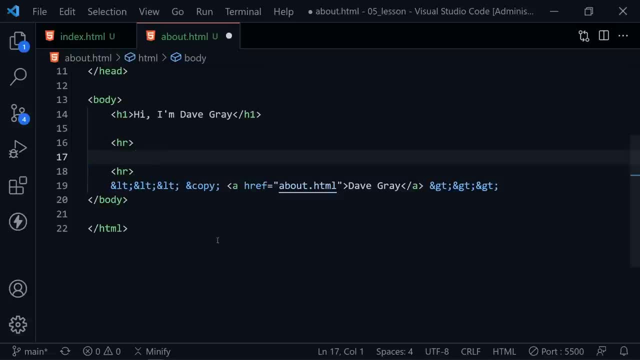 And now you can see we're left with the horizontal rules and the space in between, And so now I'm just going to put a paragraph. that's not really about me. I'm just going to create some lorem text, And I can do that with a P element. 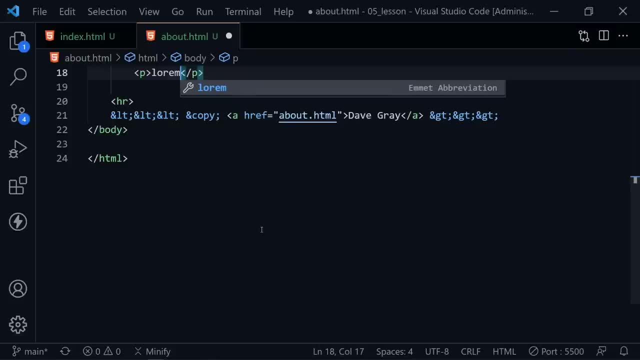 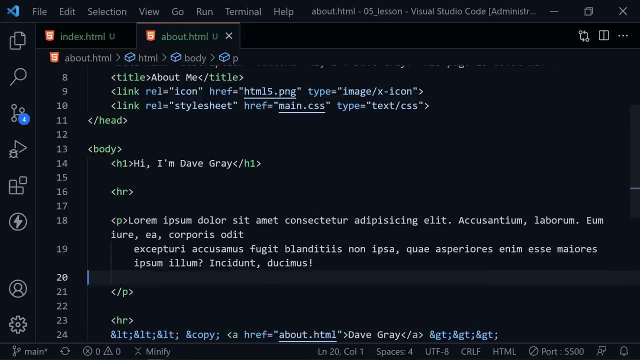 Try lorem Times one. I just want one paragraph. We'll click that. There we go- One paragraph of information. So it's still kind of formatted that strange. I'm going to go ahead and enter before and after. There we go. 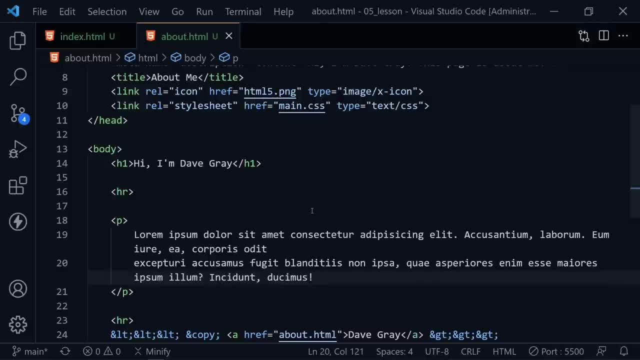 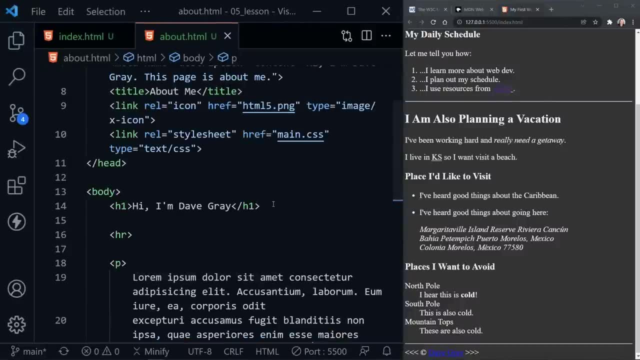 And now we've got that single paragraph here. Anyway, this is a basic abouthtml And we have linked to it, So now let's downsize Visual Studio Code Back here with the button you see right here. This is the square. 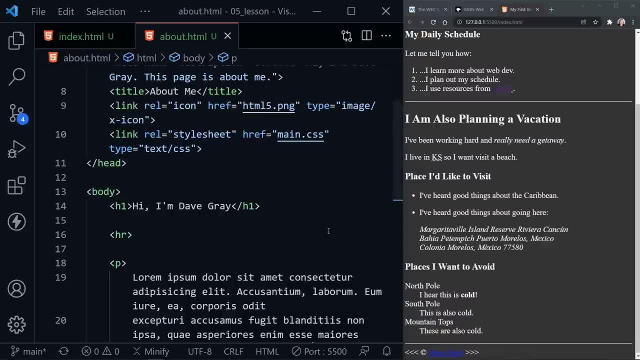 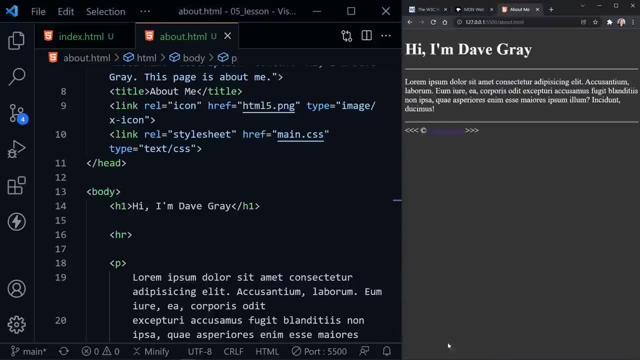 Not minimized, but downsized. It's not maximized either, And now our link to the abouthtml should work, So I'm going to click that link. And here we're on the about page. And now, notice, my name is this dark purple again. 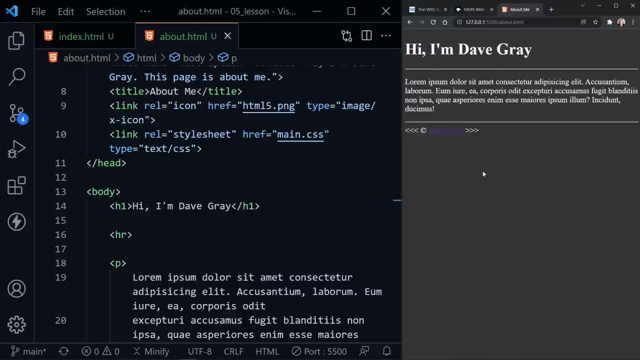 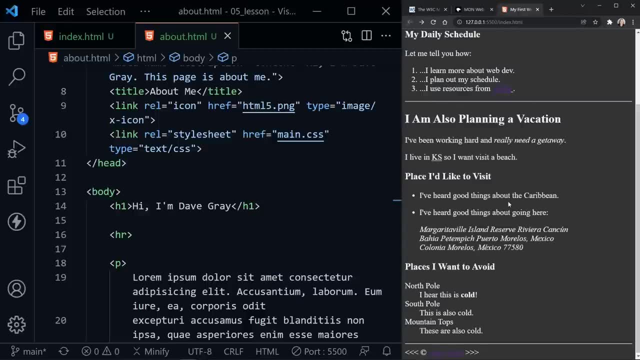 So we have gone to the about page that we just created. It says about me here in the top tab. I'm going to click the back button to go back to the original home page. here Now, back on the home page, there is a third type of link. 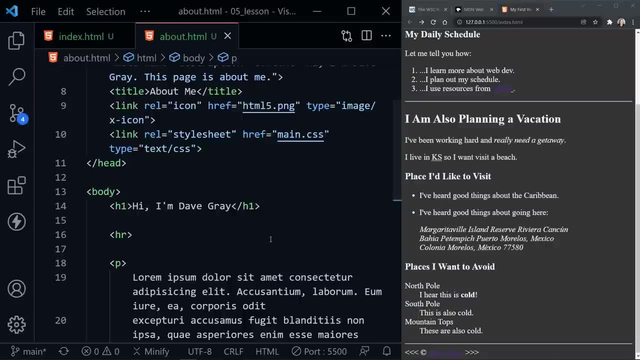 That we can create, And this is a link to an area on the same page. On the page we're already on, We can create shortcuts to different areas of the page. So we've had our absolute references, We've had our relative references. 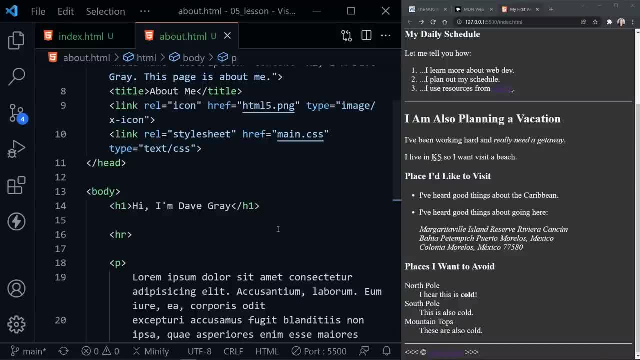 And now this is what I would call an internal reference, Or it's an anchor link directly to a portion of the page that we want to go to. In order to do this, we're going to add just a little bit more to our page. 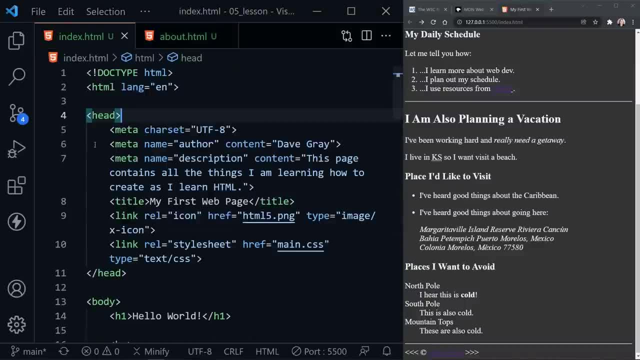 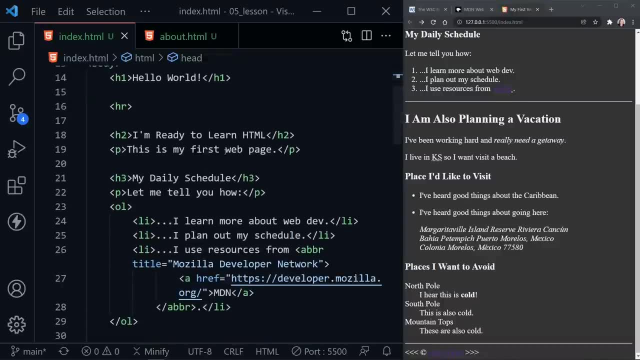 So I want to click on the input. I'm going to go to indexhtml. There we are. I'm going to go ahead and collapse the head again And we've got a couple of topic areas besides our big hello world at the top. 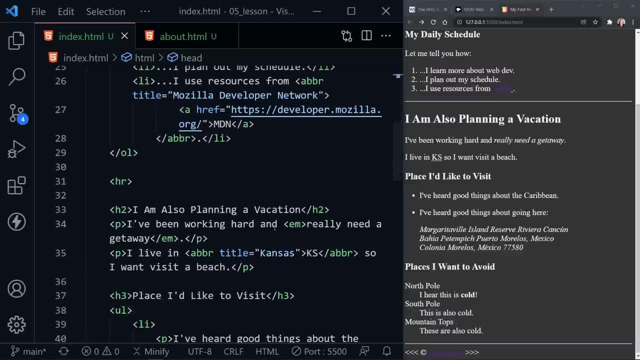 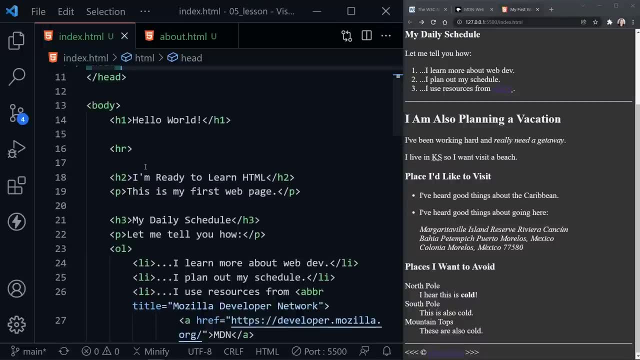 So we've got the part where we're ready to learn HTML And we've got the part that we're discussing planning a vacation. So we're going to organize this into sections And there is a semantic HTML element called sections, So I'm going to type the word section. 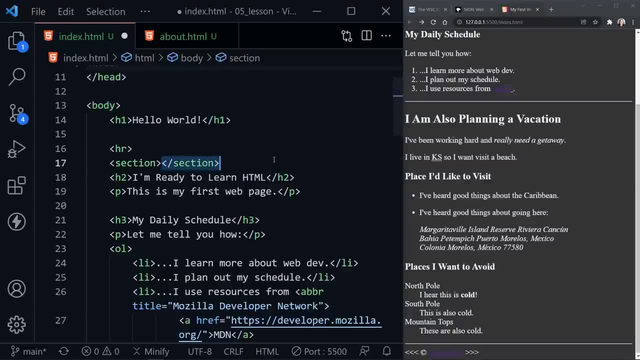 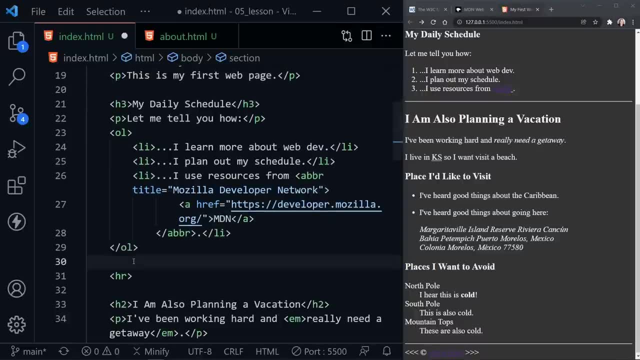 Press tab And then I'm going to highlight the closing tag of the section Control X. To go ahead and cut that out, I'll come down here before the horizontal rule we used as a divider And I'll paste that closing section tag in. 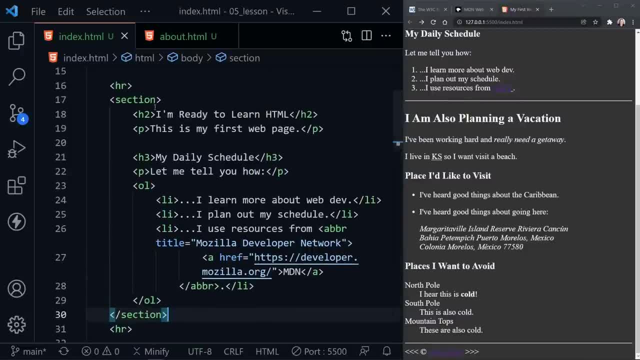 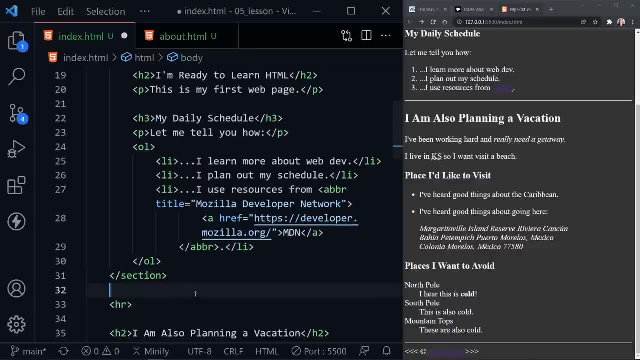 And, if I save, Yes, we've got some auto formatting there. So now we have our section separated And we've got horizontal rules in between. I'll go ahead and add a space between each of those. I'm going to do the same thing for the vacation planning area. 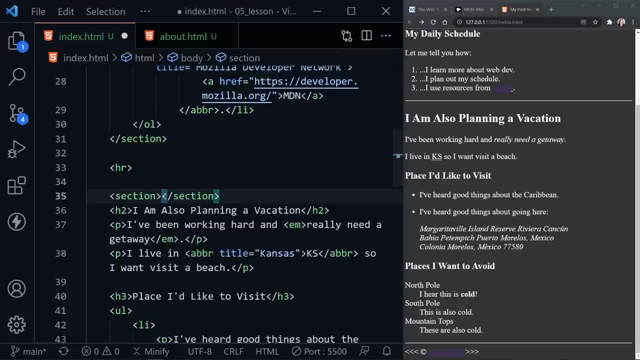 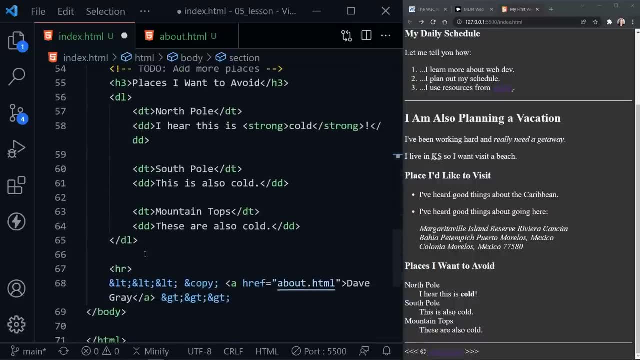 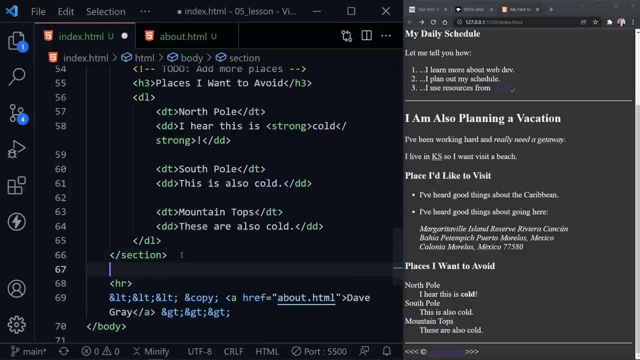 So type section: Press tab, Go ahead and highlight the closing tag, Control X, Scroll down to the bottom where we're finished discussing the vacations, And go ahead and paste in that section. Now I'll save. once again. Took advantage of the auto formatting. 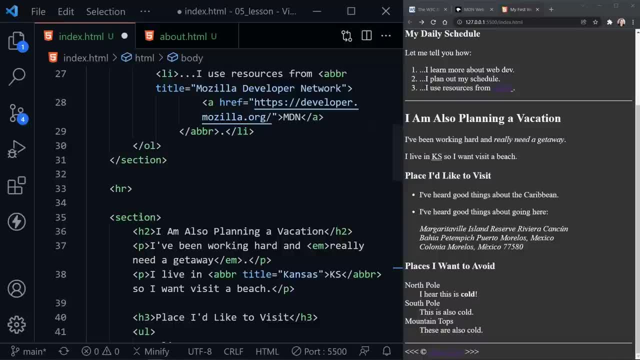 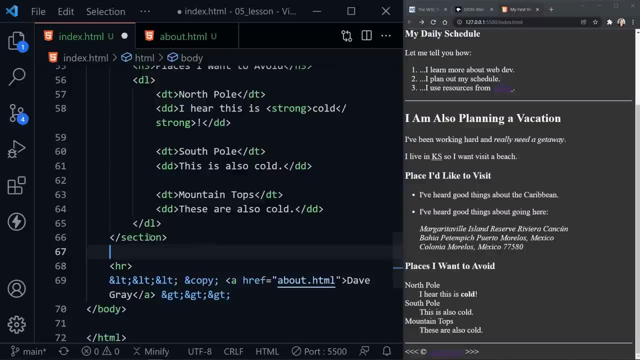 And we'll leave a space, Of course, before the section here, Between the horizontal rule and the section, And the same at the end, Just so we can see it a little better. After the closing section tag we have a space. So now we've created semantic HTML space. 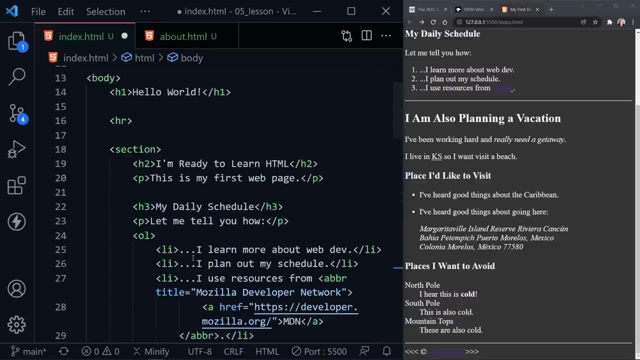 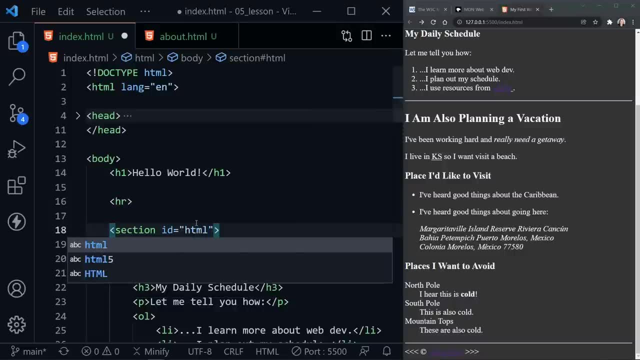 And that's not all we need. We also need to give these sections an ID attribute. So I'm just going to give the first ID value For the I'm ready to learn HTML area, An ID of HTML, And then in the next section. 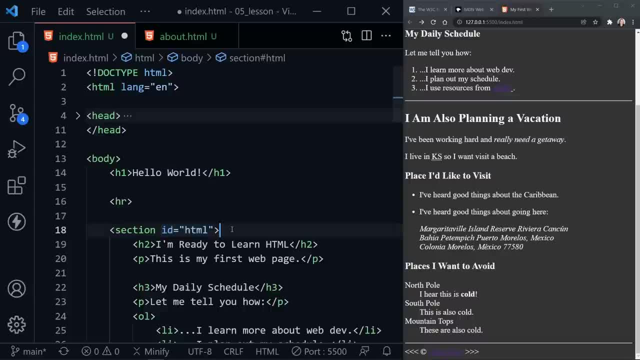 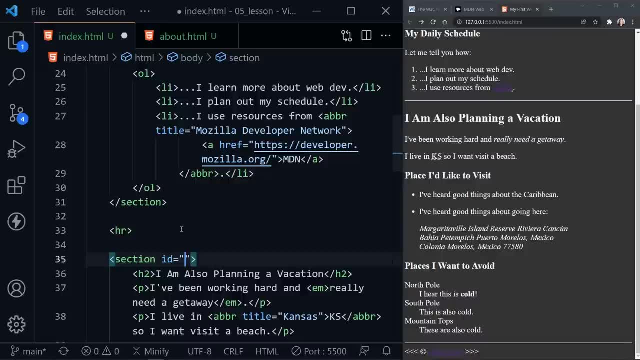 I'm going to give an ID attribute And that value is going to be vacation, And once again, Control S to save, Or you can go to the file menu And click save And then in the next section I'm going to give an ID attribute. 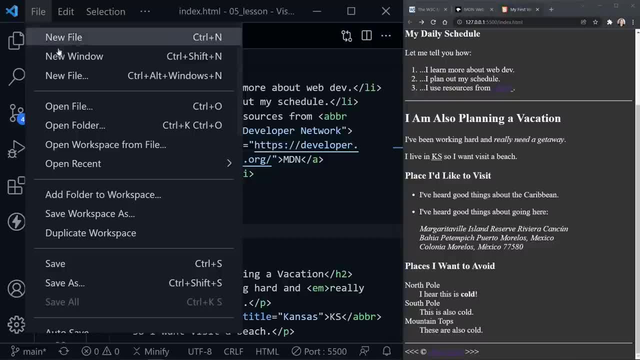 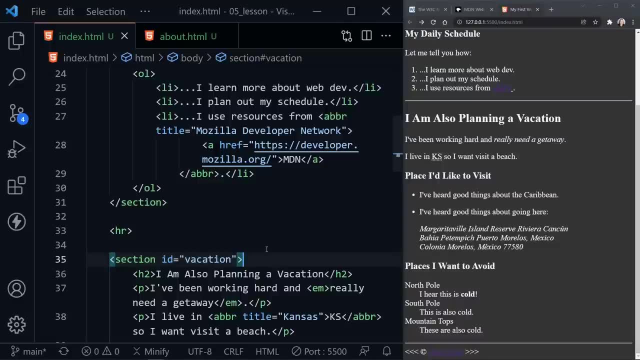 And that value is going to be vacation, And once again Go to the file menu And choose save that way as well. Now that we've done that, We still haven't created the links, But we have created the destination For each of the links that we want to create. 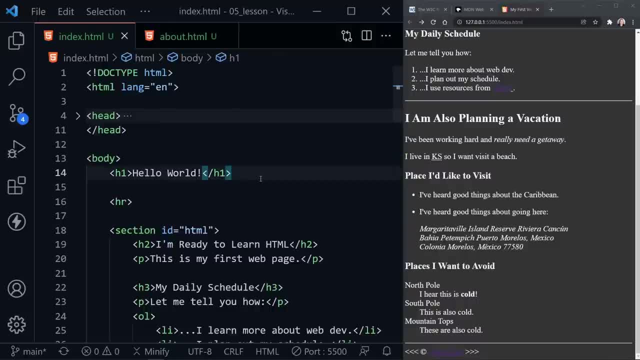 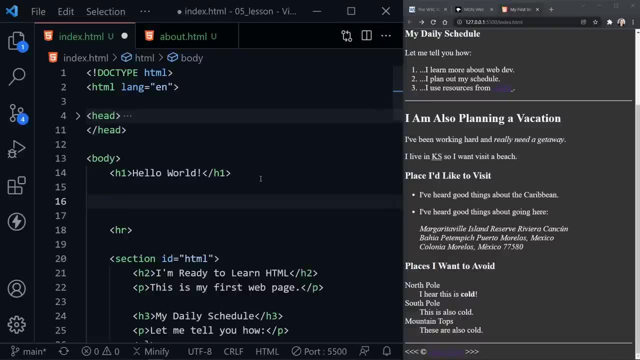 So now let's create one more semantic HTML element, And to do that, After our hello world heading, I'll go ahead and press enter to come down a couple of lines. Type HR for one more horizontal rule. And now between the horizontal rules: 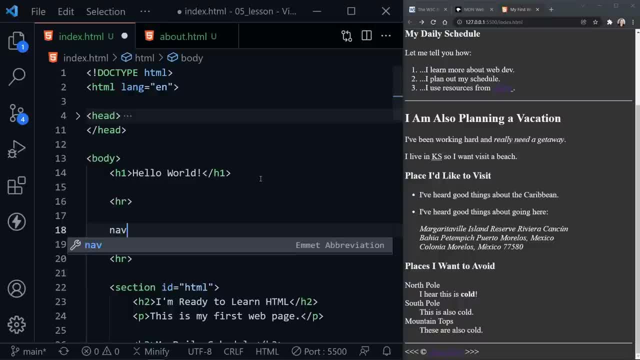 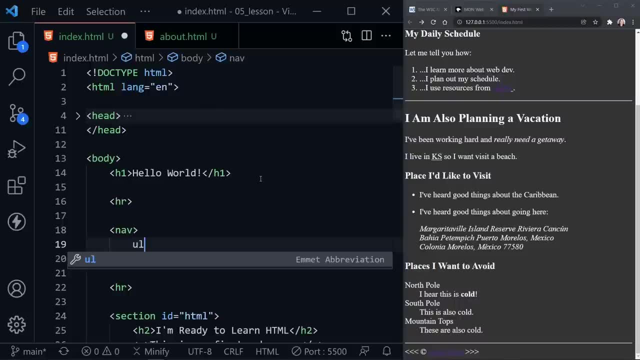 I'm going to type nav, And this is a semantic HTML element. It says we're creating a navigation area Inside the nav. I'm going to type ul. We learned how to create unordered lists already, And so now we've added an unordered list. 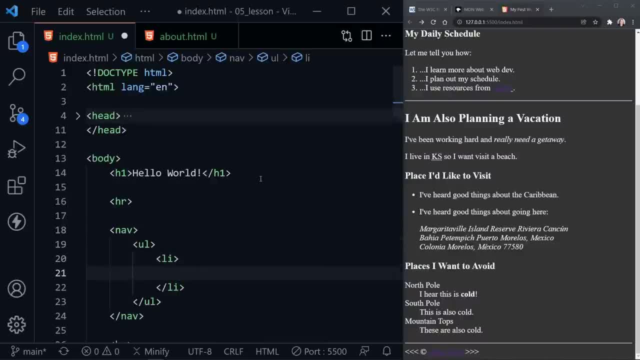 And now we can add list items, And the first list item that we're going to create Is a link, And there it absolutely. After I pressed A and tab, It knew we needed the href in Visual Studio Code, So now it's waiting for me to fill in. 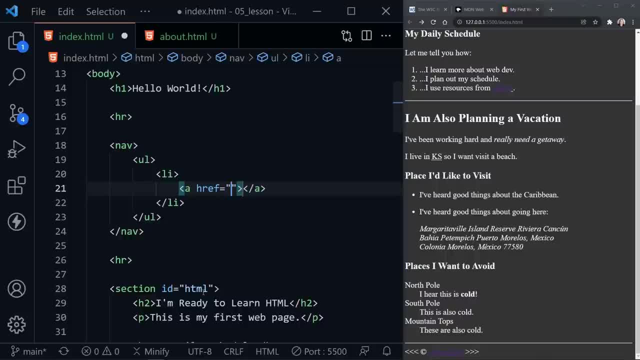 This href. Now, to link to our HTML section here on the page, We need to add the hashtag And then the ID value. So there's HTML, And so now we can put Learn HTML for this link, And then let's go ahead and add one more. 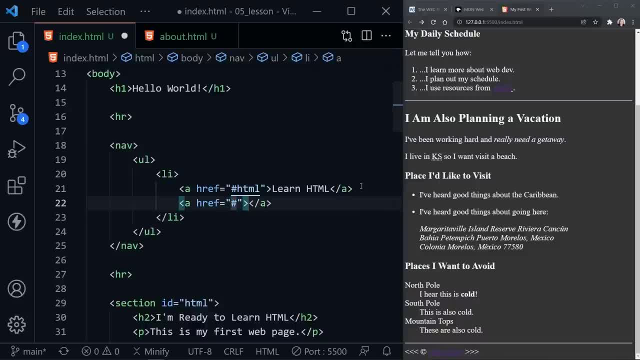 Lowercase Press tab And now hashtag Vacation, And we'll put here Planning a Vacation. As a matter of fact, Let's change this from learn HTML to learning HTML, And now at the top Instead of hello world. 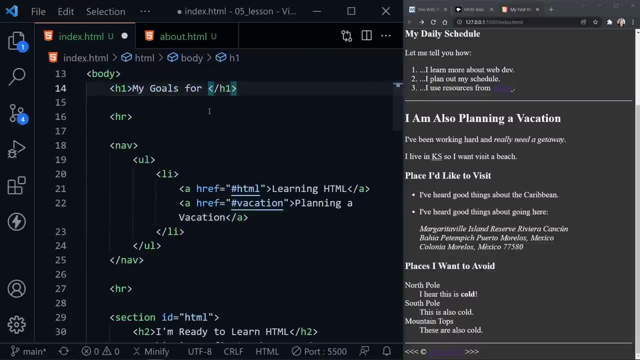 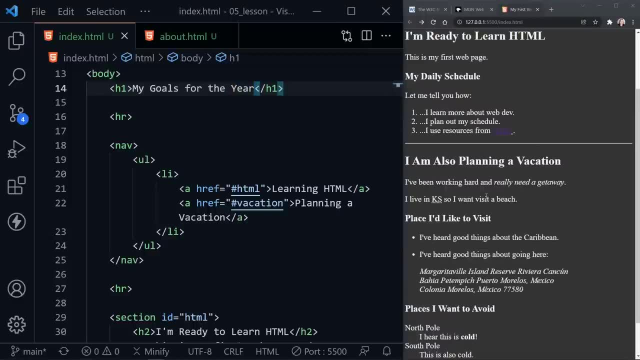 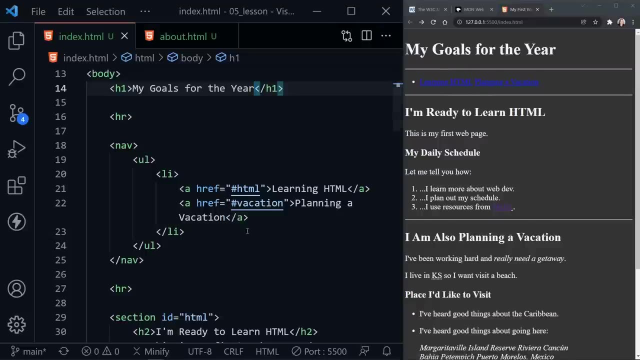 I'm going to put my Goals for The year, And now we have My goals for the year At the top And we've got learning HTML and planning a vacation, But I put them both in the same list item And that's not what we want. 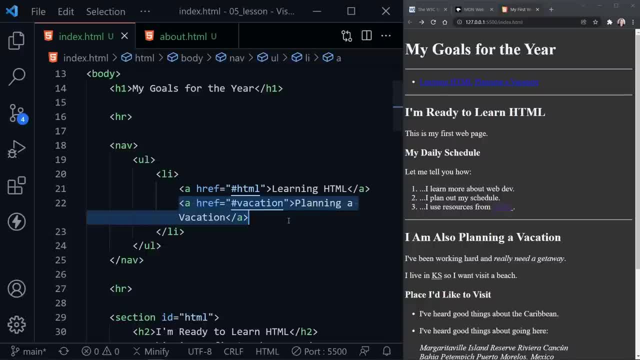 So Going to go ahead and Highlight Planning a vacation. Press control X to cut that out. And now let's put it in its own list item. So Li Press tab: We've got a new list item And we can paste that. 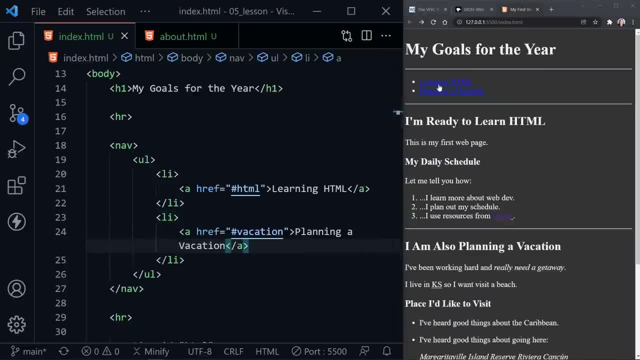 Planning a vacation If we save. that looks much better on our page, Even though the blue isn't looking great on the darker background. We'll still change that in the future. So now, if we click learning HTML on the page, It goes ahead and scrolls the page. 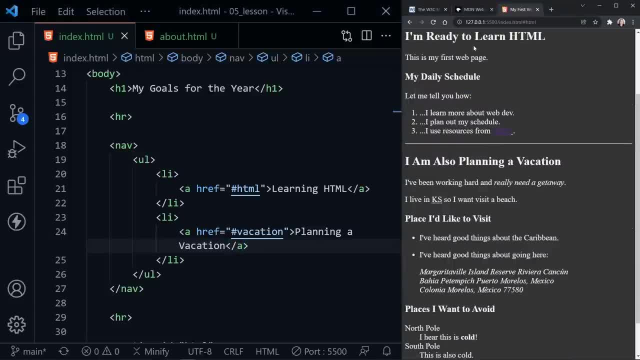 Directly up to the I'm ready to learn HTML section. We can click back and we go back to where we were. And now, if we click planning a vacation, It doesn't take us all the way to the planning A vacation area because there's no more content. 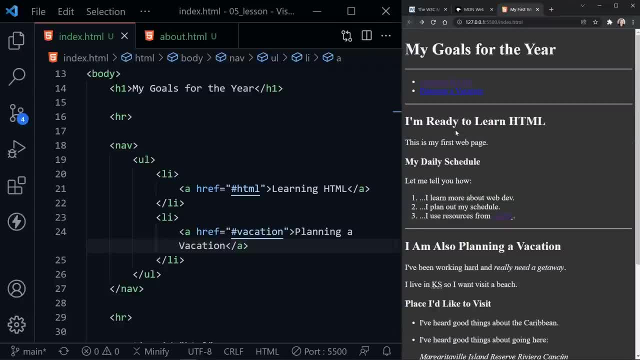 There's no more space. It can't scroll any higher, But it scrolled as far as it possibly could to take us to that area And once again we can press the back button to go back. And now we've got our H. 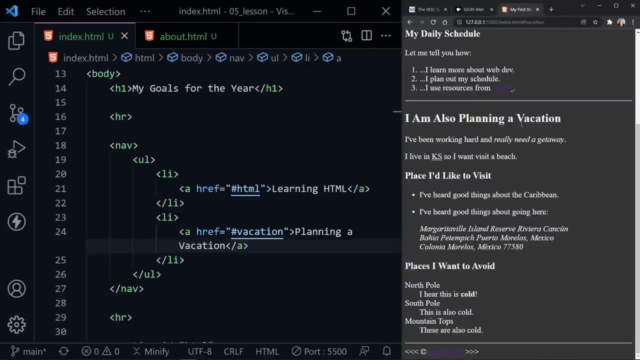 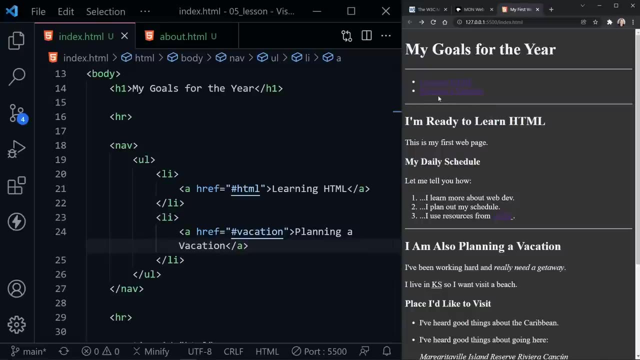 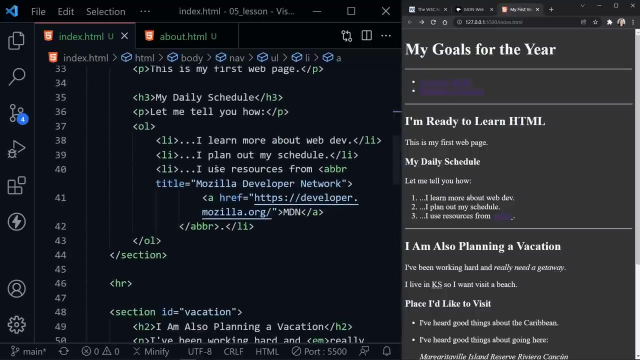 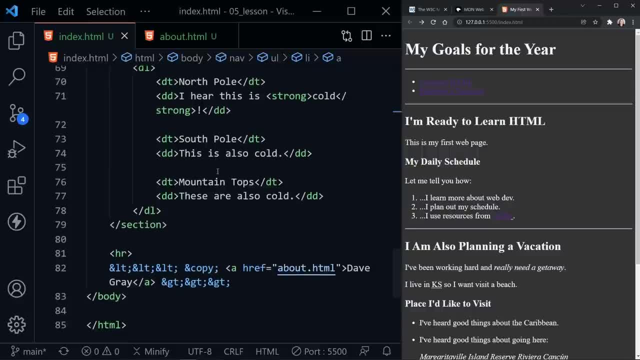 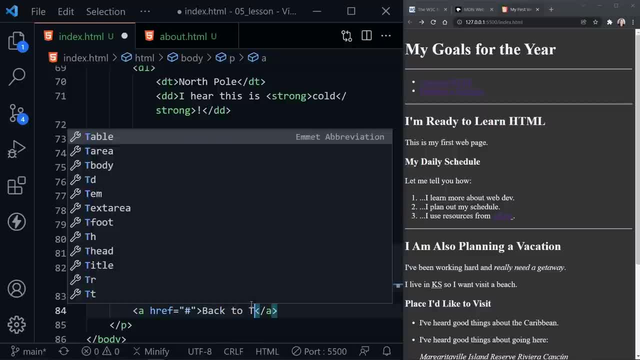 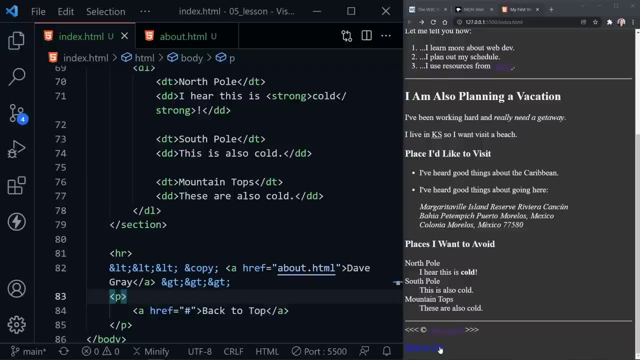 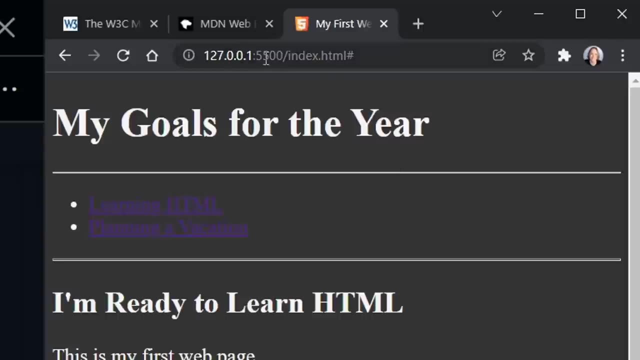 Now what we want to put in here for text is back to top and we can save. Now if we scroll down in our page here we'll see the back to top link and if I click it it loads the page and takes us back to the top. It's worth noting what we have up here in the address bar. Of course live server gives us. 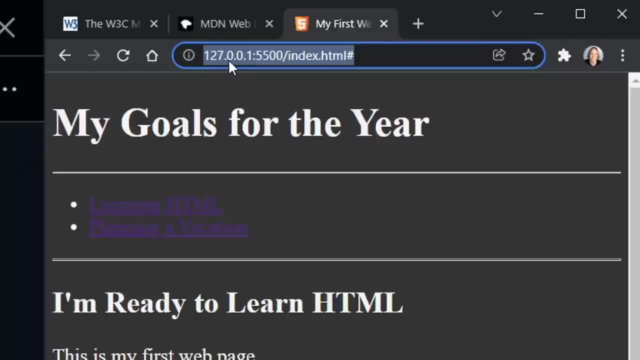 our ip address, which is our own computer: 127.0.0.1.. Nobody else on the web can see what you're seeing. This is just on your computer. and then you've got a colon and the port number 5500 where live server. 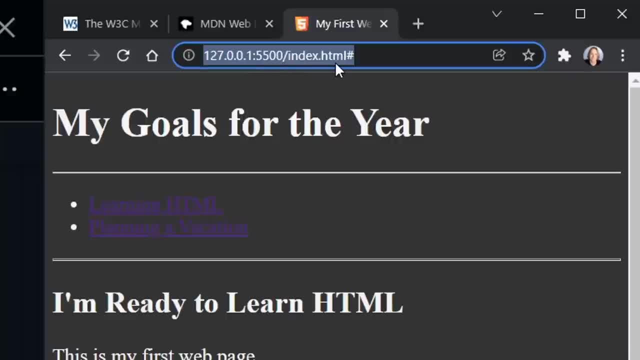 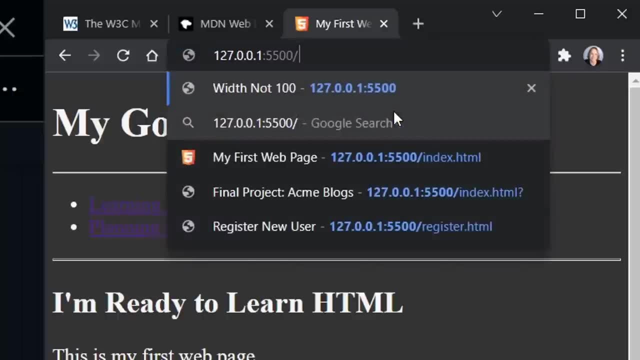 is serving your page. Then we've got our indexhtml file. Then notice, you've got the hashtag. after that We could actually remove the indexhtml and the index page will still show by default, just like you see right here. And now we've got the indexhtml and we can see that the indexhtml is still showing by default. 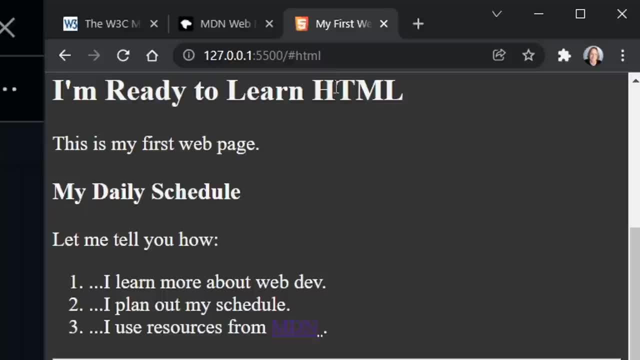 And now we've got the indexhtml and we can see that the indexhtml is still showing by default, just like you see right here. Now, once again, if we click learning HTML notice in the address we get the hashtag HTML. When we click back, it disappears. 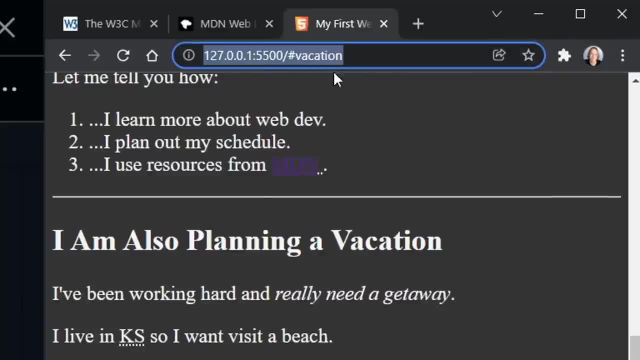 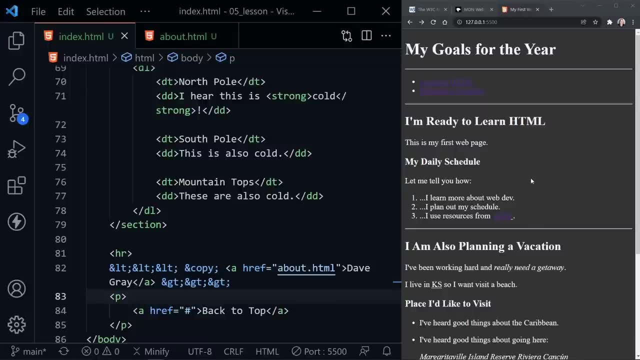 If we click planning a vacation, we get the hashtag vacation in the address bar And if we click back it disappears. In previous tutorials I had mentioned switching the theme over to this dark mode that's easier on my eyes was entirely optionable. 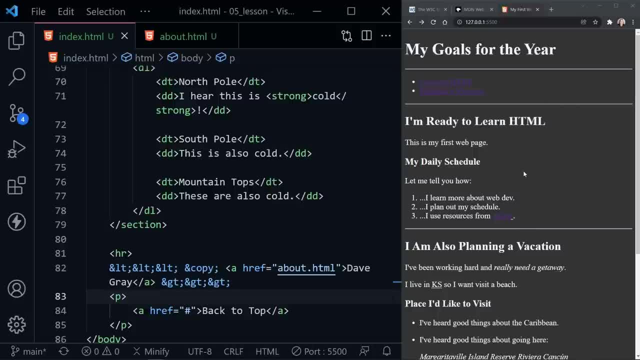 So if you're still using a white background with black lettering, probably the purple and blue links look just fine to you And you could just leave it that way. If you have switched to the dark mode theme that I have provided with some basic CSS already, let's go ahead and make those changes so the links look better as well. 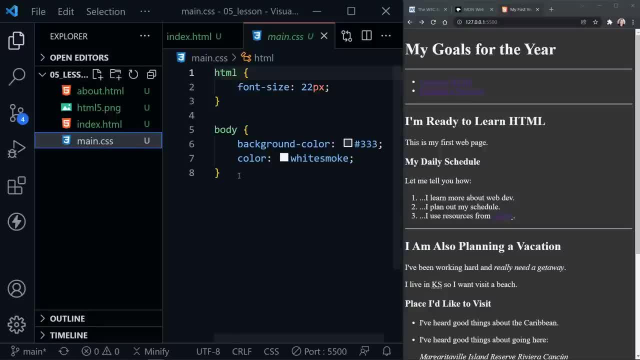 So we're here in the maincss file, now in the file explorer. So we're just going to change the color of our anchor tag And I'll switch that color to a color named Alice Blue. After that, I also want to change what the link looks like when it's been visited. 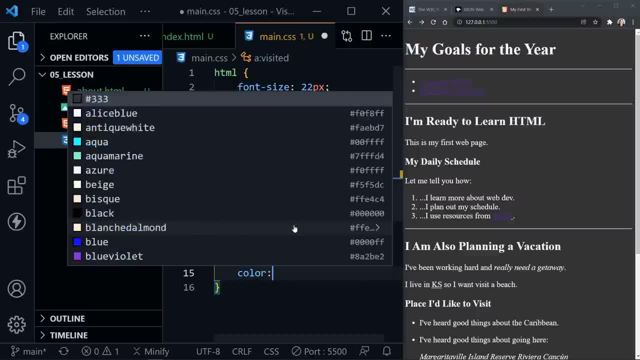 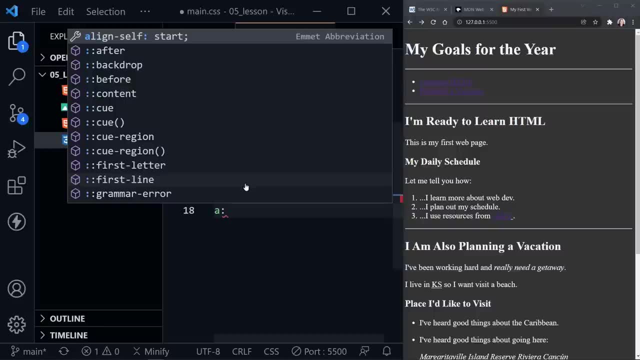 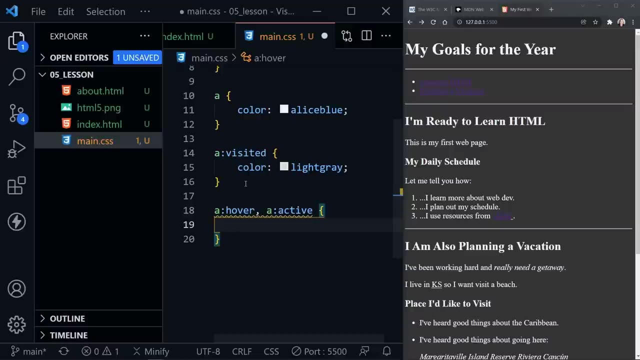 Right now it's that purple color, So I'm going to change that color to a light gray. And there's also another thing that we can change, And that is when you hover over the link, or when the link is active, And then I'm just going to change that color to. 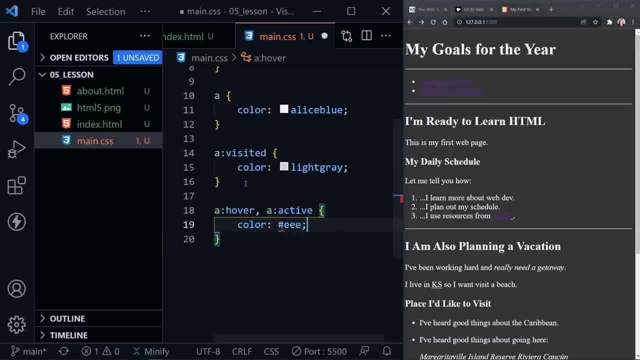 Hashtag E-E, not three E-E-E. There we go And save that, And so now it's changed the color of our links. You can see this is the light gray. We visited these links, But when I hover over it gets a little lighter. 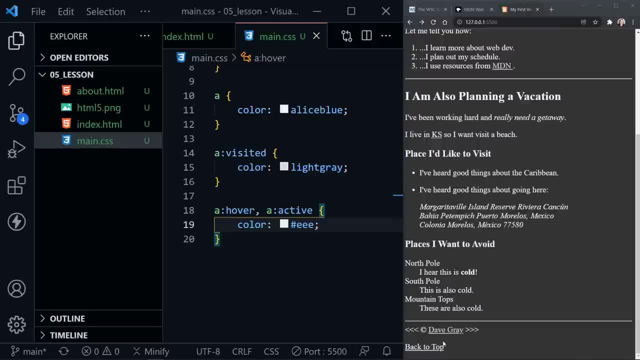 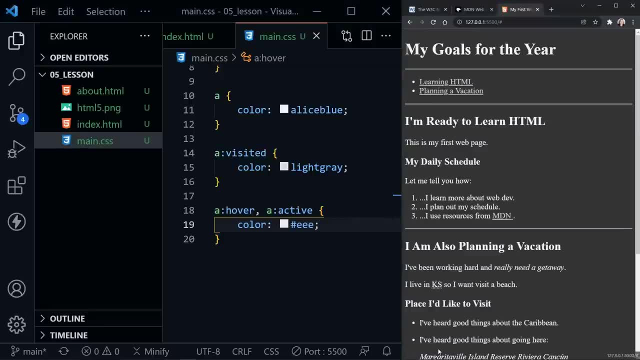 And so that looks good. I think we visited every link here. No, we haven't visited back to the top yet, So you can even see the Alice Blue color right here, And let's go ahead and visit back to the top. 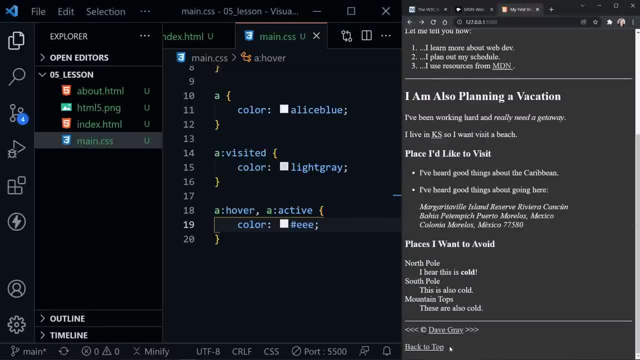 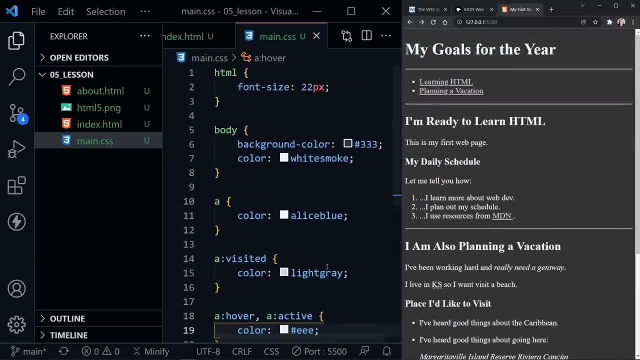 And now if we go back, You can see it's a little darker until I hover over it. So we've just changed those colors. We're not really covering CSS yet. We eventually will after we get through all of the HTML. 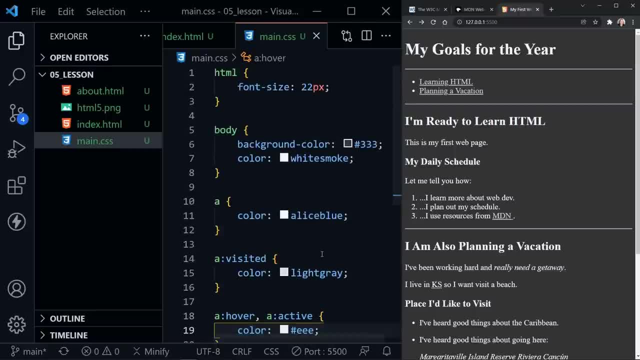 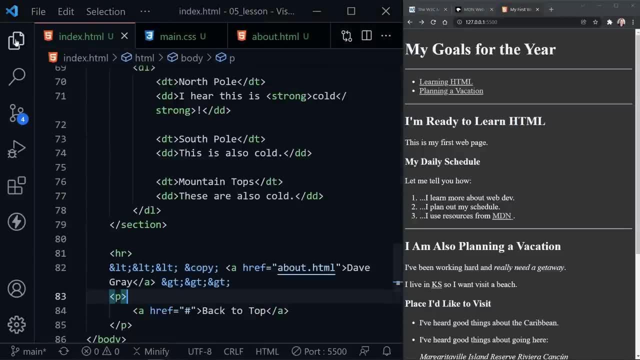 But just for now, if you want those, Of course these will be downloadable as well in the source code. Let's go back to the indexhtml file And let's hide this file explorer by clicking on the icon in the top left. 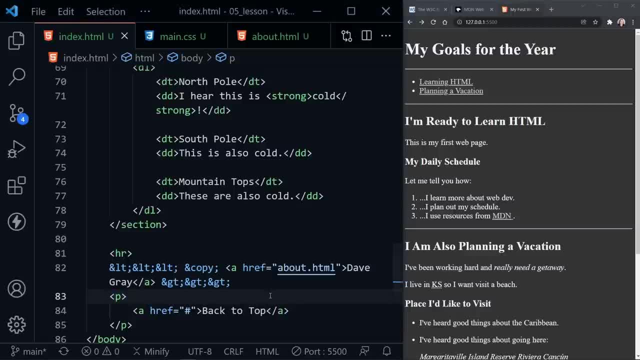 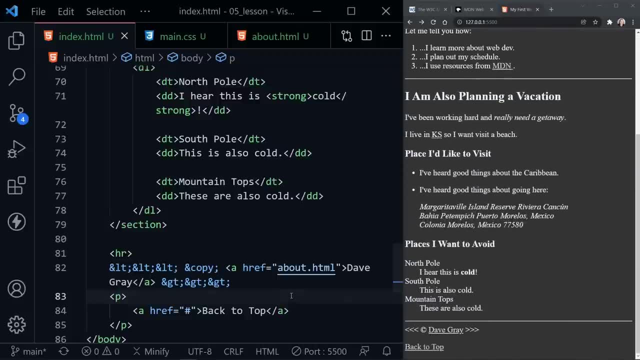 This is a good spot to talk about some link naming conventions And things you don't want to do, So for now I'm just going to use this link at the very bottom that has my name as an example And one thing you wouldn't want to do. 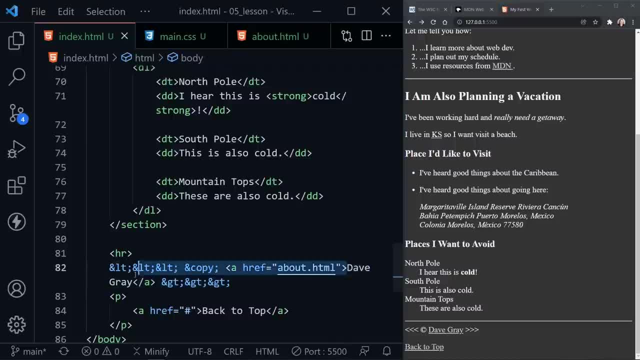 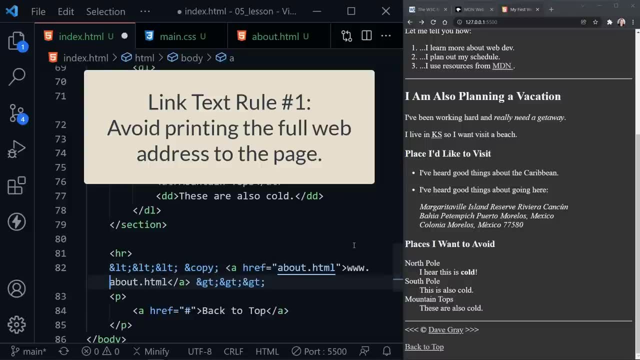 Is be. instead of my name, Just put in the file text like this: Or what would be worse would be a full URL like wwwgooglecom, slash abouthtml. And if I save this, Of course that's not to Google, That's just ugly. 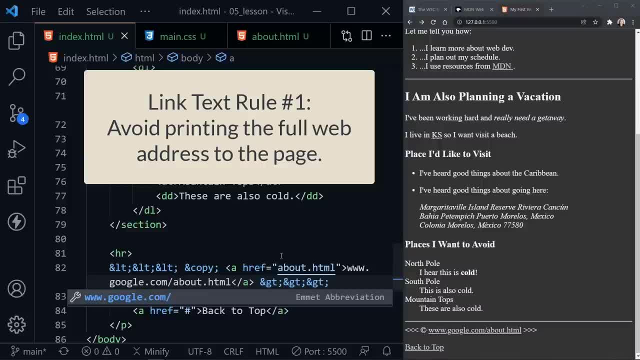 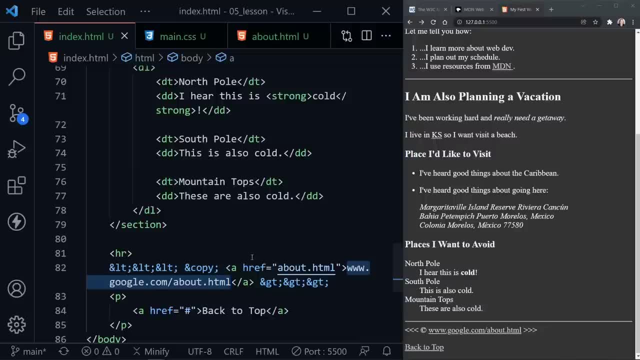 And of course you don't need all of that. You can pare that down To just Actually a short description of what is there. You don't really want the full URL there, So I'll put this back to my name And there we go. 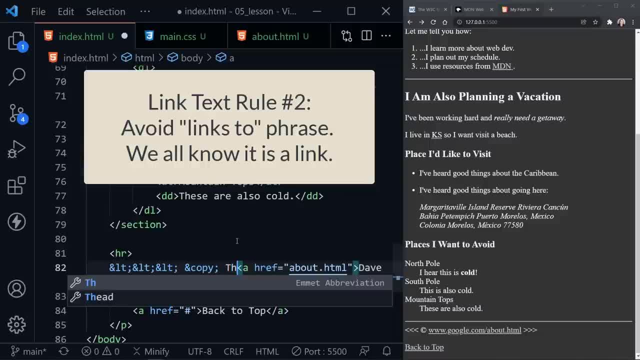 And another thing you really don't want to do is say this links to info about, Because really that's redundant. So if I save that and we go, this links to info about- And I didn't have a space there, I guess, But either way, 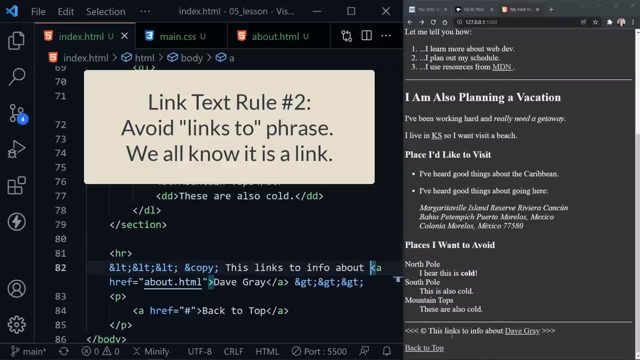 Saying this links to is really redundant. Just saying this is a link A screen reader knows it's a link, You already know it's a link when you see something underlined like that. So you don't need to say this links to or this is a link about. 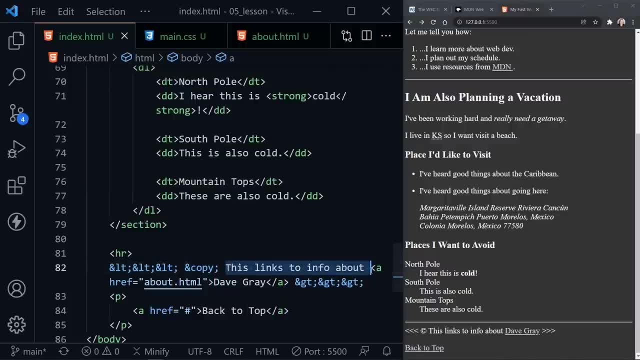 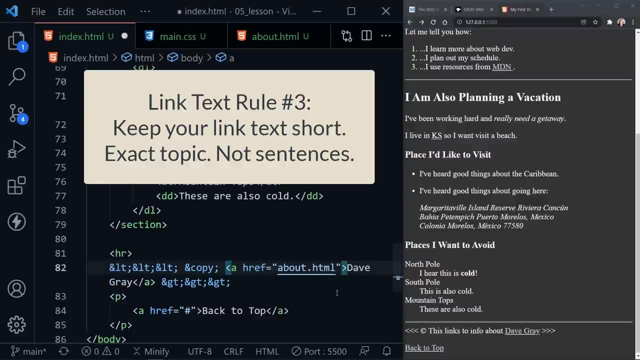 That's just unnecessary. You also want to keep your link text as short as possible, So imagine if I had that same sentence before. this links to information about Dave Gray And you just put the whole sentence in the link. That's way too long. 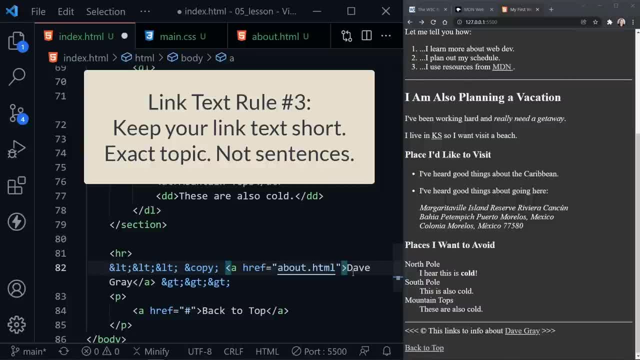 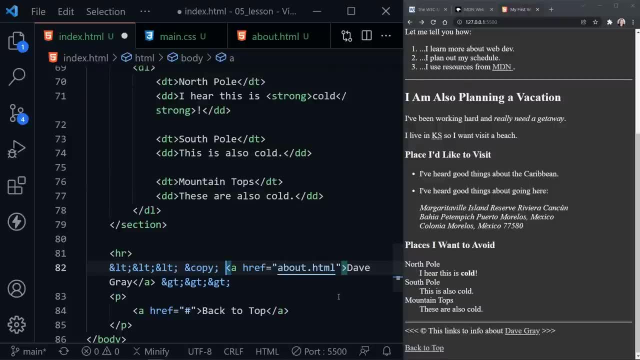 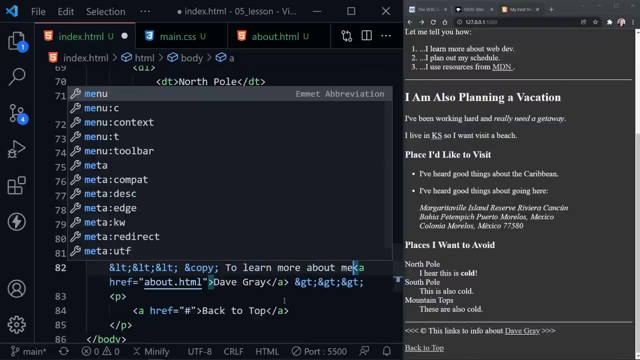 Just keep it to the Exact topic. So if the page is about you, as in our about page, just put your name in there for the link. You don't want a whole sentence about that. And now, the very worst one of all really would be to say something to learn more about me. 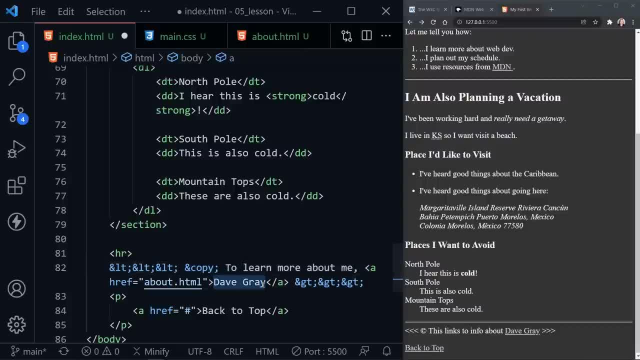 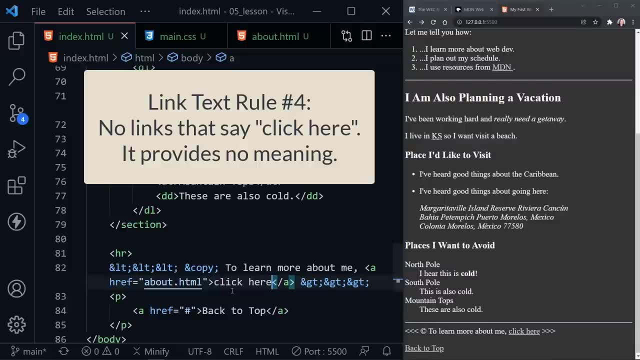 Comma and then, instead of having your name right here for the text, you put click here. We've probably all seen a link on the web that says click here. that has no description whatsoever For what's on the following page. That's not good for the context of what you're linking to. 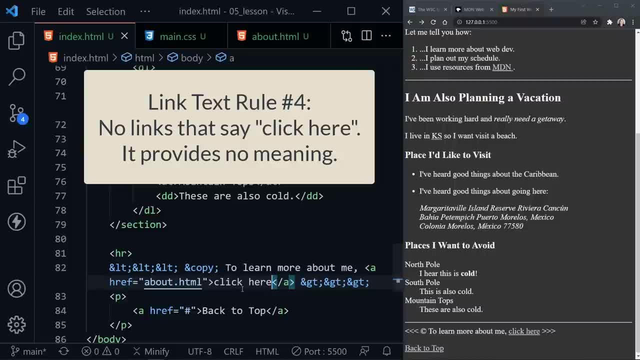 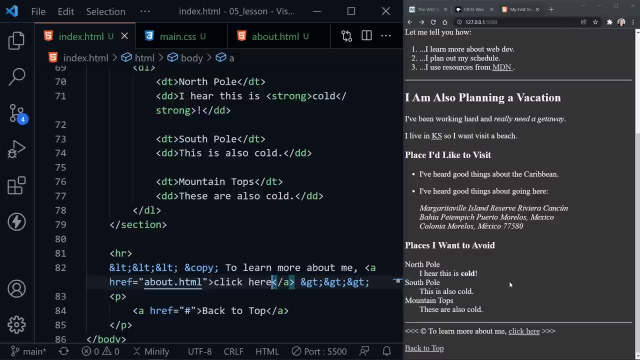 It's not good for a screen reader as it tries to get context from what the link says. So really, a link that says click here. And of course you can imagine there could be several links that say click here, all on the same page linking to different things. 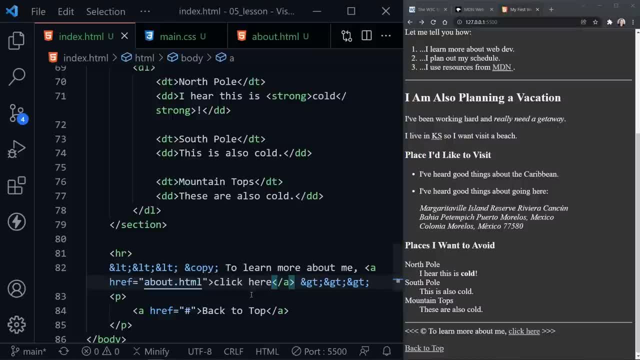 And that's just confusing. So you always want to avoid something like that that says click here. So once again, I'll remove all of this and we'll just go back And we'll put our name here at this link. But I hope those pointers give you some guidelines about namings. 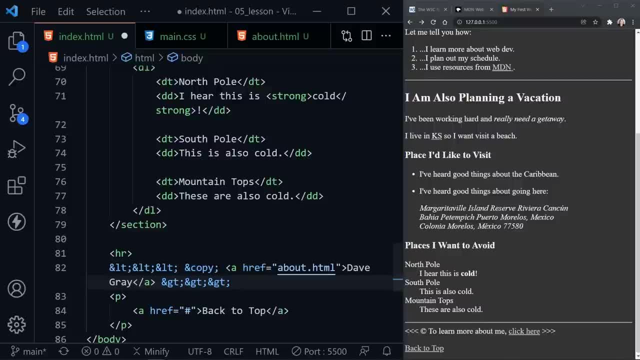 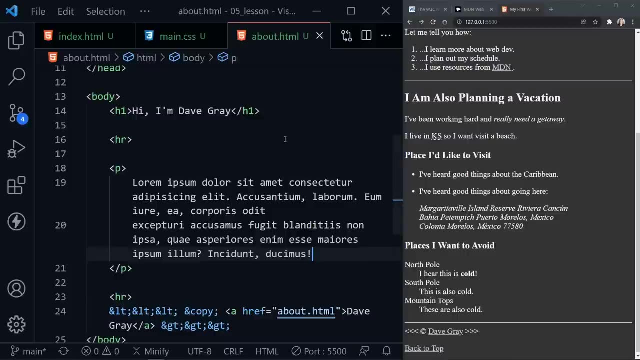 Just keep it short and, of course, say what is on the following page: A very brief description, not a full sentence and definitely not something generic like click here. Okay, I'm going to save the indexhtml and we're going to go back to the abouthtml page and we'll add a few more link types. 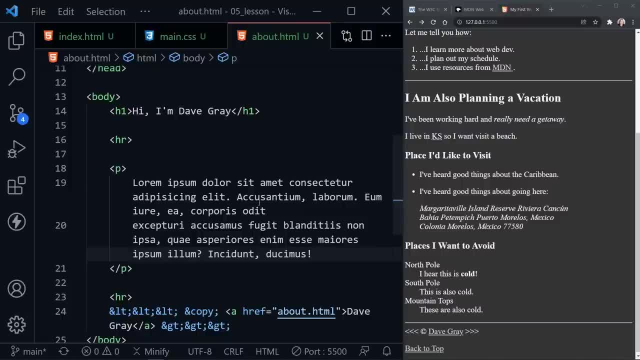 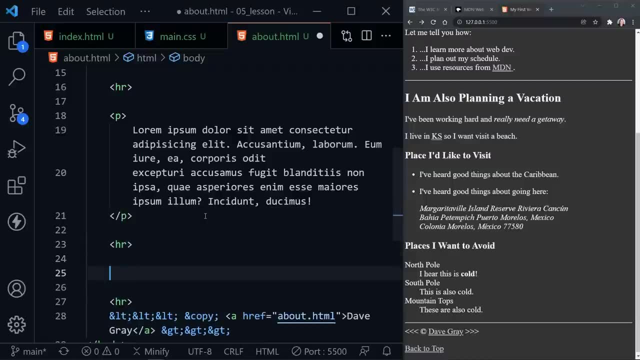 So we've got a section that we're really saying: this is about me. Let's just add one more area here so we can add another horizontal rule, Press tab, and now let's add an unordered list, And inside this unordered list we'll have list items. 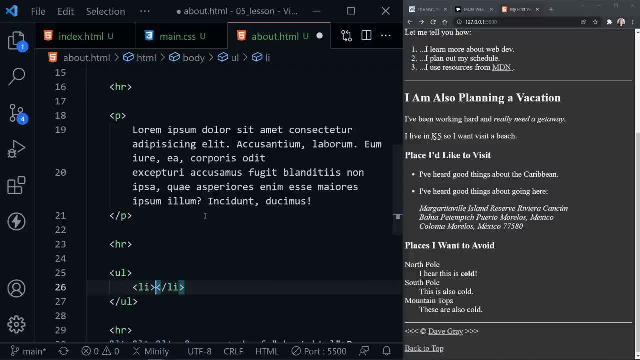 And this first list item should be a download. So we have a favicon file that we can offer for downloads. So let's say download in, and then I'll give the anchor tag, So a href equals. And now let's go back, And now let's link to that favicon file that we have. 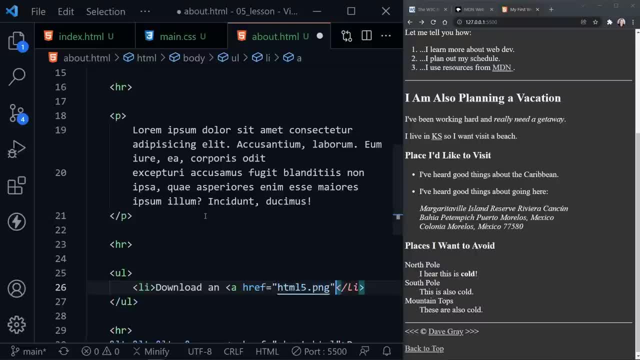 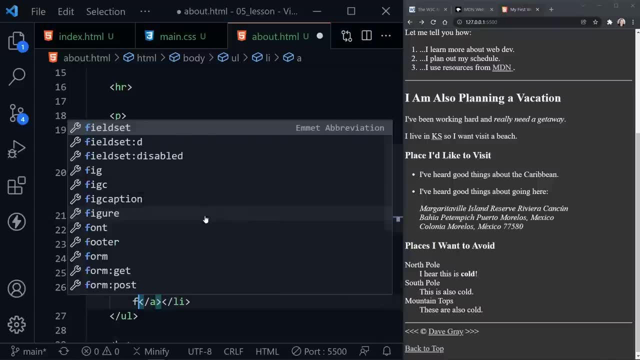 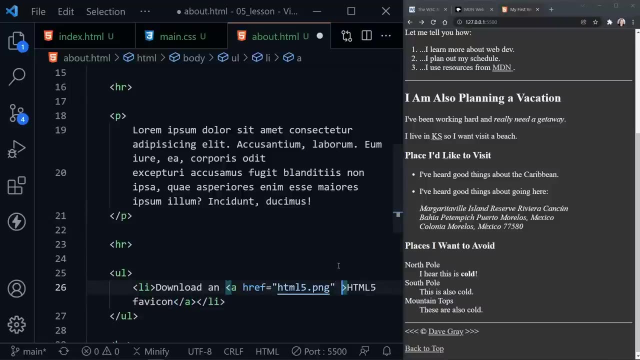 So that would be html5.png. And now inside of this, we can put our html5 favicon text, But this won't allow us to download the file yet. We need to add the download attribute, And now this is a download link. 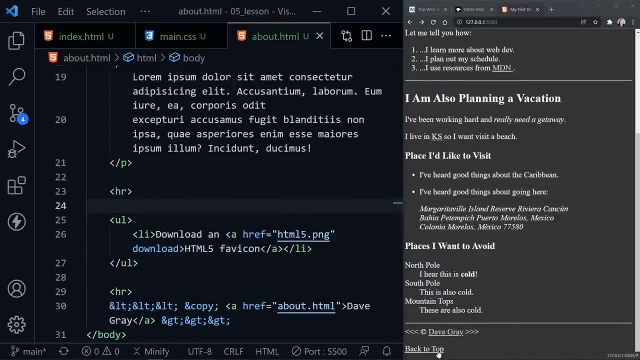 So if we save this, We go ahead, Go back to the top over here in Chrome. And well, I guess not back to the top. We need to go ahead and click your name or my name, Whatever you've got on your page. 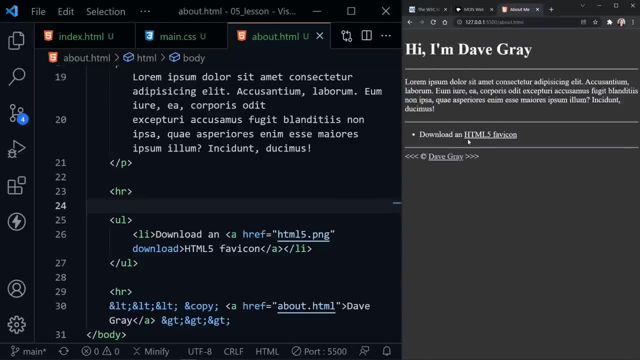 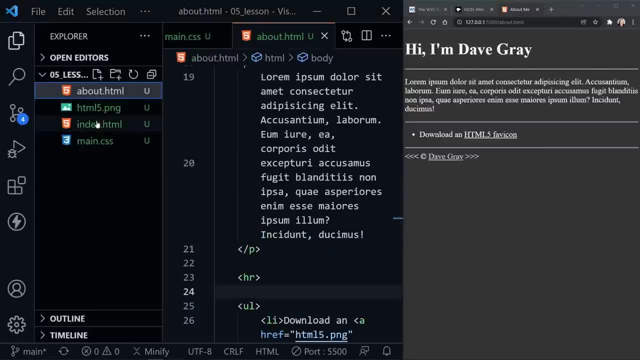 And that takes us to the about page And now we have download an html5 icon And remember, this icon is in our folder over here as I click the file explorer. So we've got html5.png And that's what we're going to download. 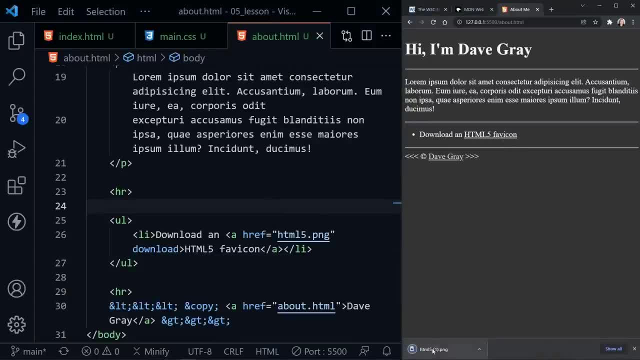 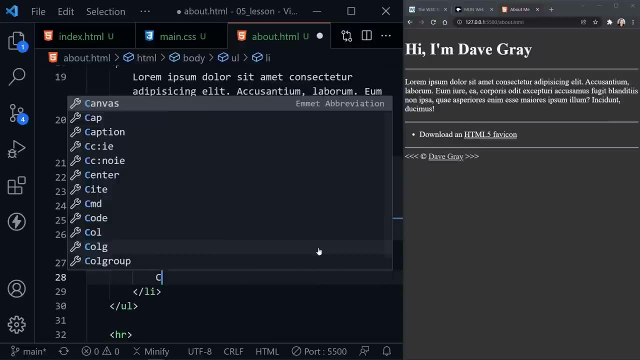 So if we click this link, We instantly get a download of that file. So that is a download link. Now let's add another type of link. So add another list item here And inside our list item. now let's say contact me at: 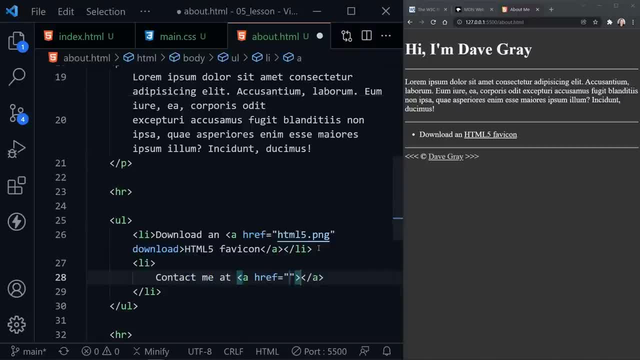 And now let's go ahead and do another anchor tag with the href And we can add an email link, Even though these are not advised. And I should say before we add this: These are not advised Because there are so many spiders out there that crawl the web. 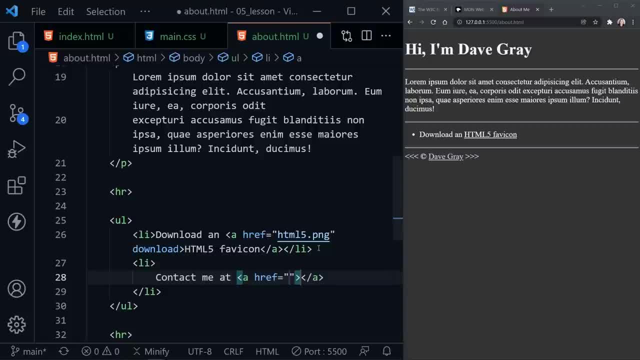 Really search spiders, if you will, And what they do could harvest these email addresses, And so these have kind of become a thing of the past. Most people add a contact form, Which we'll talk about forms in the future, Instead of just putting their email address directly in the page to be harvested. 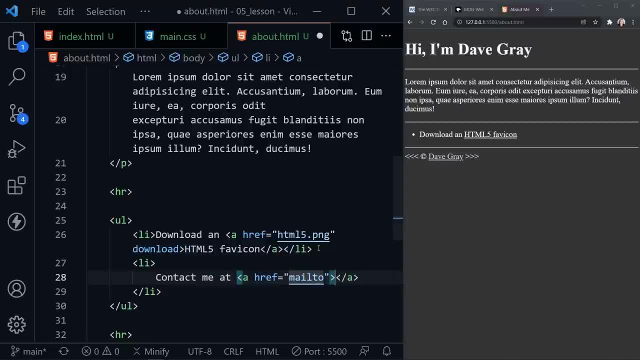 But to add an email link. you start with mail to, And after that you would just have your email address. So I'll just put random at email dot com And if that's your email address, I'm sorry but it seems random to me. 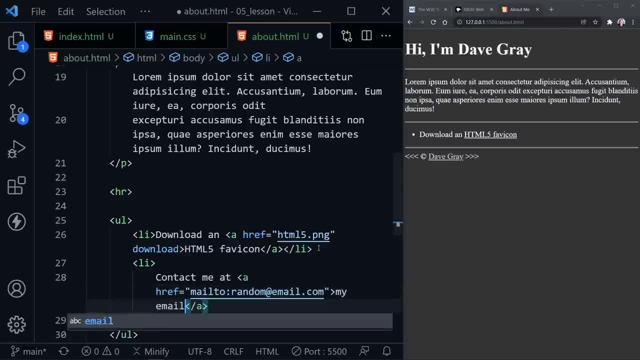 And then I can just put my email address, Which would complete the sentence rather than actually typing the email address there as well. So I like something like that. as far as being descriptive, Contact me at my email address And that's what the link is. 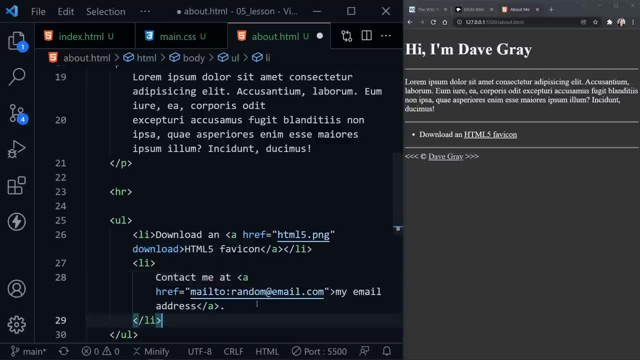 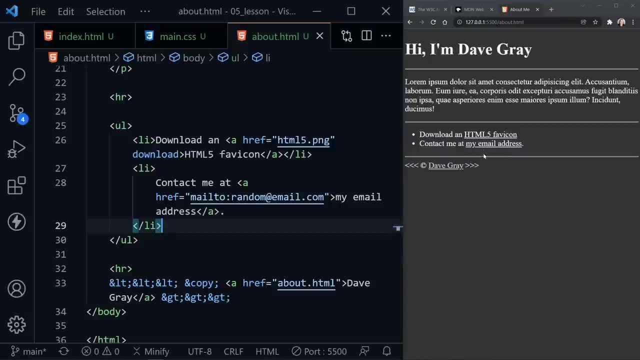 The link is describing Your email address. Okay, then there's one other type of link we can have. Oh, let me save that, by the way. And if you click this link That says my email address, It would ask you what type of email client you want to open these types of links with. 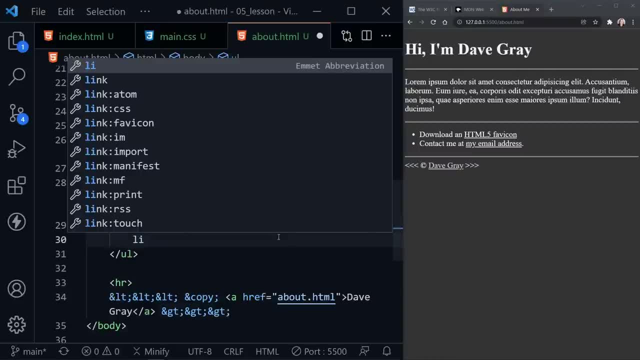 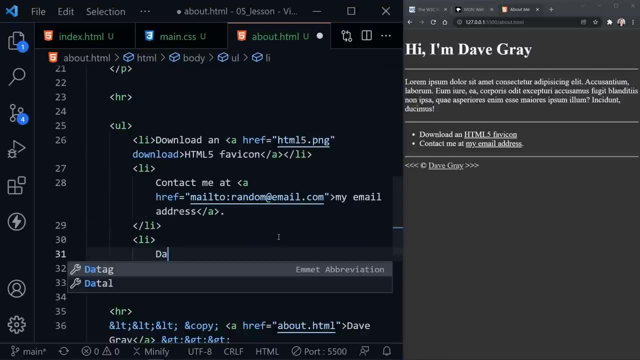 Is what it should do at least. Okay, the next link type that we have in our list item Will be dialing a telephone number. So now I'll say: Oops, Spell it right. Dial. And now let's put our anchor tag with the HREF. 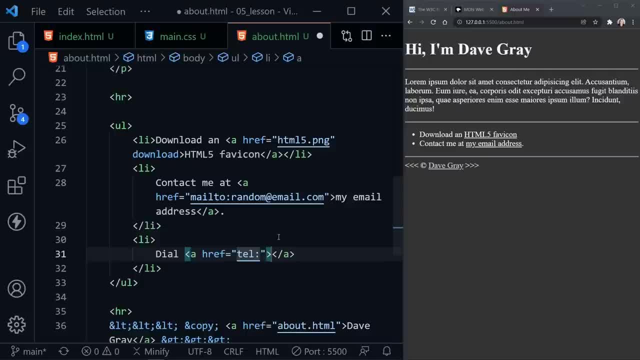 And we start out with TEL for the telephone number, And you can experiment with this. Many examples I've seen. add the plus symbol And I've also got it to work without the plus symbol. So I'll put the plus symbol here. 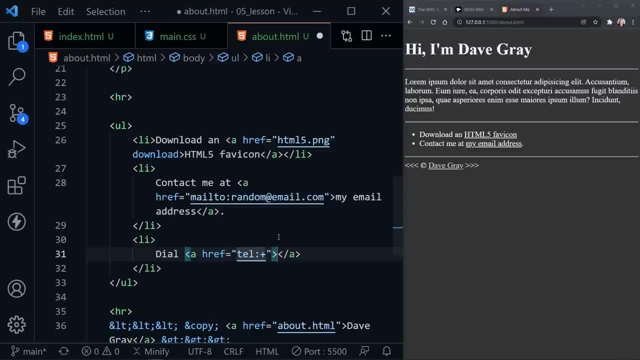 In the United States most phone numbers are ten digits, So I would have like one, two, three would be the first set of digits, Then four, five, six And the last set of digits seven, eight, nine, zero, Something like that. 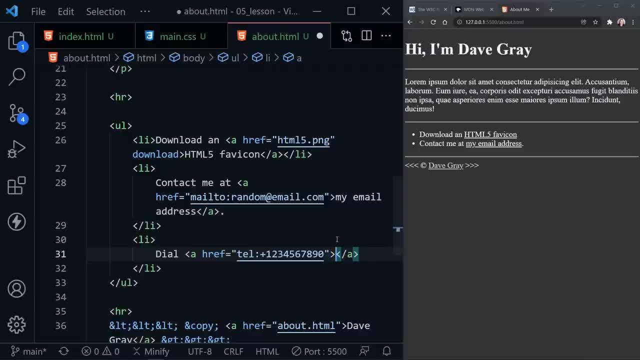 And that is a telephone link, So I could say dial And then I could just put my phone number, Just like I did with my email address. And now, especially on a mobile phone, If this was a mobile website, This would be very handy. 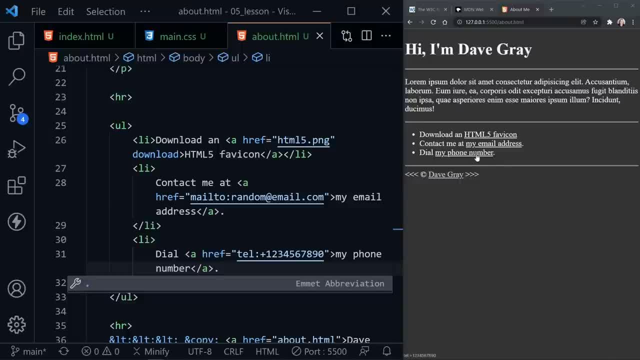 You could tap this and it should open up the dialer. If I click this link now in Chrome, It wants to make a call. It's asking me how to do it And pick an app to do it, Because I'm here on my laptop. 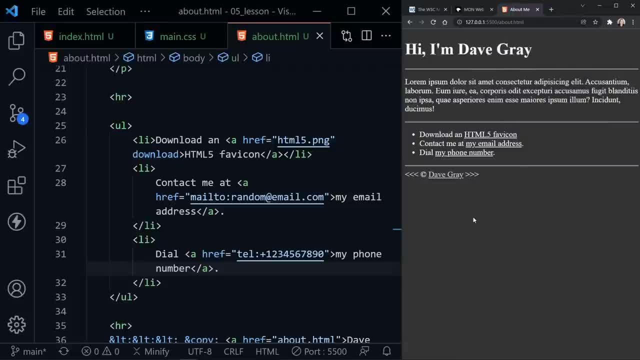 But on a mobile device, This would probably open up the dialer Right away. Now let's look at one more type of attribute here. So I'm just going to put one more list item Inside that, One more anchor tag With the href attribute. 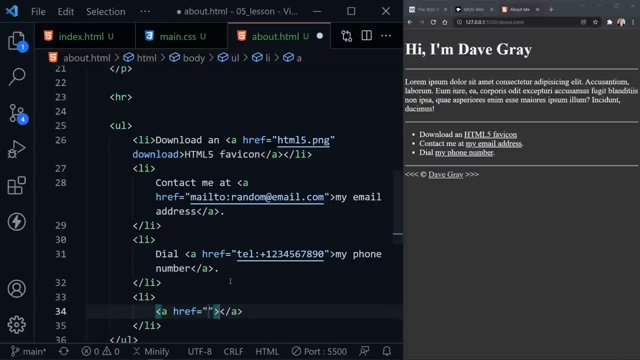 And we're going to link directly to Google, So we need an absolute reference. This would be https//wwwgooglecom, And we can put the slash if we want to as well, And this is an absolute reference, But the attribute Oh, and I haven't really put in any text. 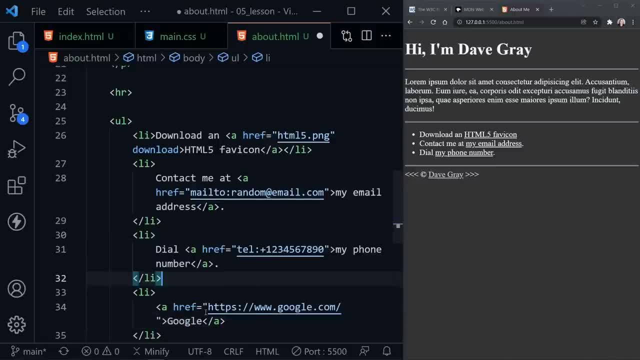 Let's go ahead and just put Google, Because we're not really adding any extra context to this. So the attribute that we need to consider, That we haven't used yet, Is target, And what I want to do Is have this open in a new tab. 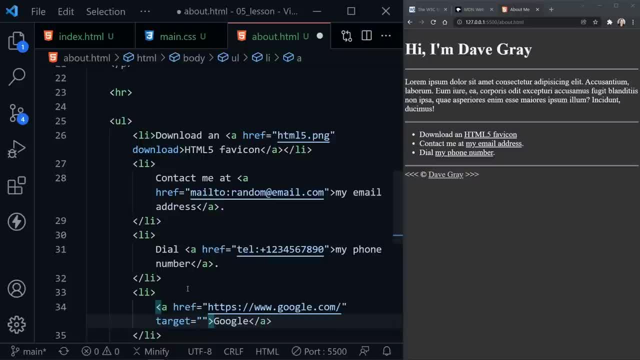 So I'm going to use quotes. Then you put underscore blank And save, And now we have a link to Google. So let me maybe add a little context here. I'll put open Google in a new tab Period. Save that. 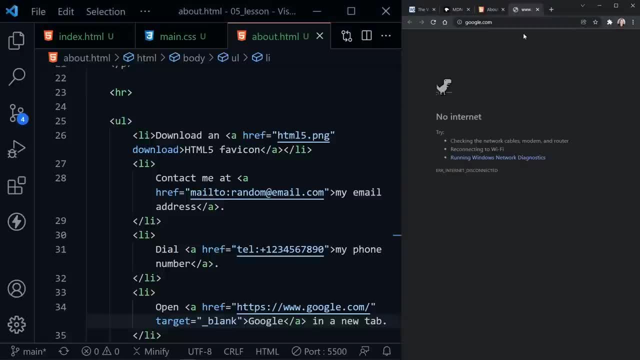 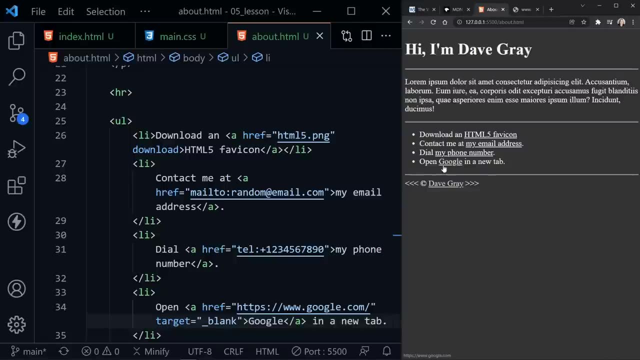 And now we've got our link to Google. If we click this, We opened up a new tab And I don't have internet right now. I guess I need to check my connection Internet's back up and running. Let's click this link again. 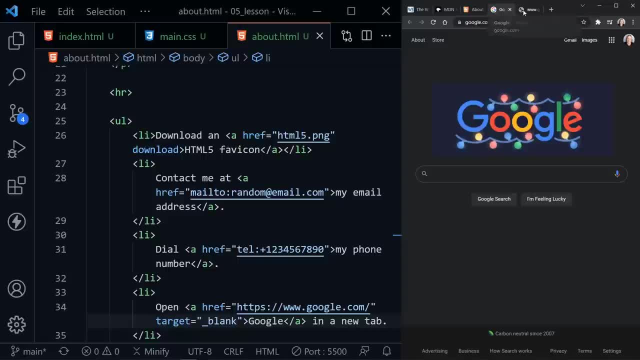 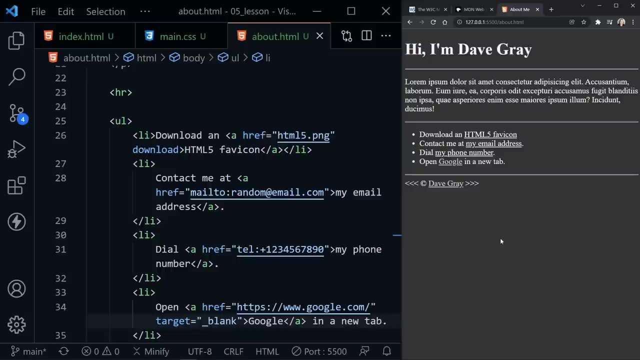 And there's Google. So we've opened it in a new tab And all is well, So I'll go ahead and close that. There's the one that didn't work, And now We're back to our page. Now there's one more type of link. 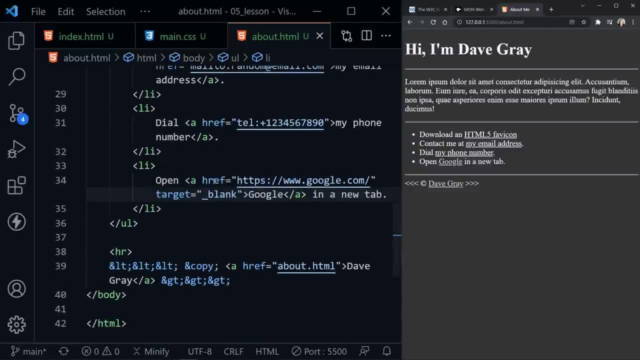 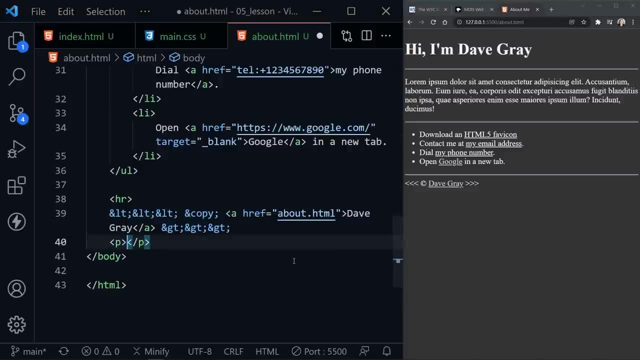 I want to add before we finish today, Let's scroll down in our abouthtml And underneath our copyright line Let's go ahead and press enter, Add a paragraph, And inside here We'll add the link that we want to add. 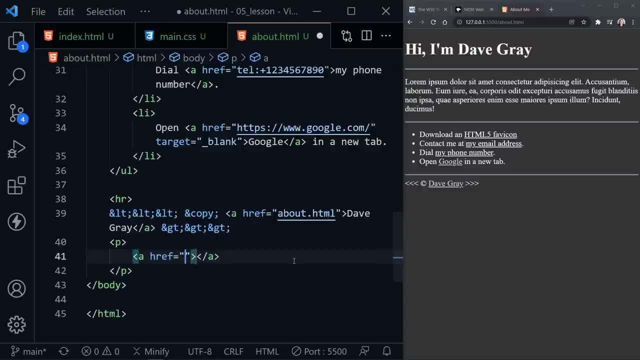 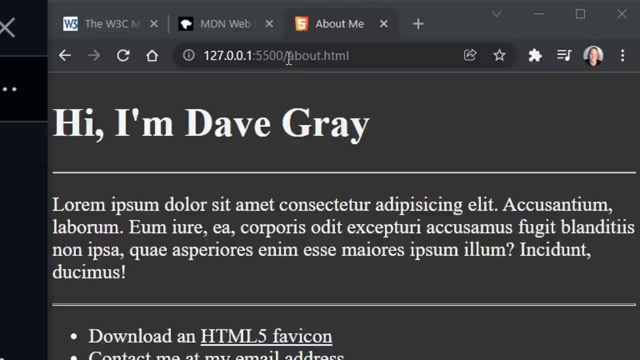 So type A for anchor, And now the href is just going to have a slash value. What this does is link back to the root of our website, And that is our indexhtml. It's the page that loads by default. Remember, I had said we don't even have to have the indexhtml up here in the address. 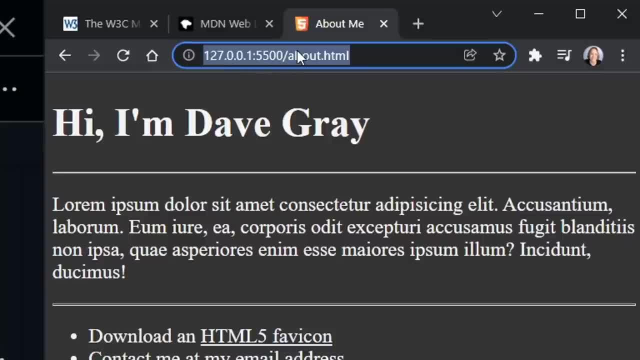 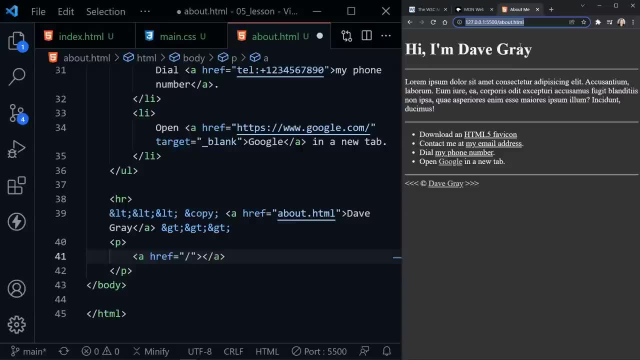 It's just the slash after the IP address and the port here on our local server. And if we had a domain name like googlecom, Well then the slash would essentially be the home. It doesn't have anything else. after the slash It loads a page by default. 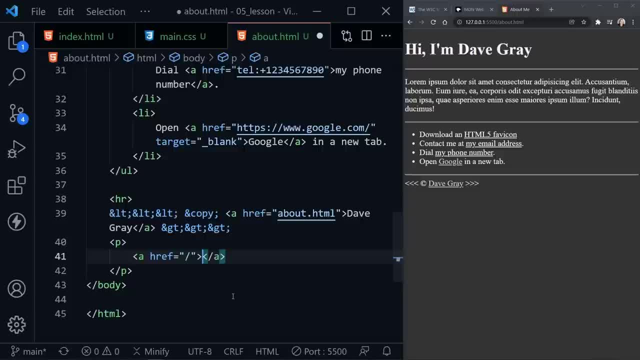 So that's the same thing we're doing for our website. So here we can just put back to home And save this, And now we have a link that will take us back to our index page. So let's click this link And we're back to our indexhtml. 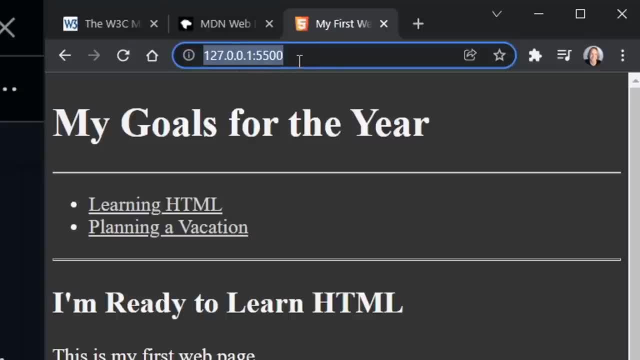 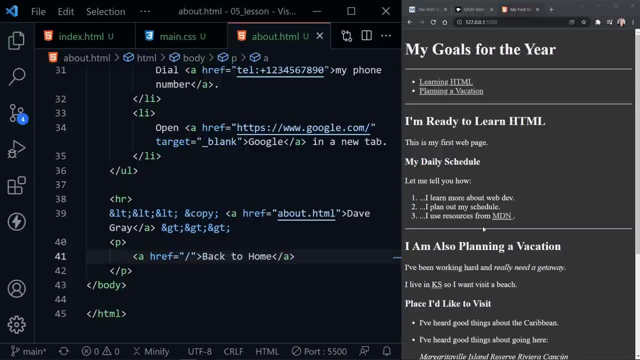 But notice in the web address It doesn't even have the indexhtml up here. It doesn't need that because it loads this page by default. This is the first page of your website, Now that we've made all of these changes to our web page. 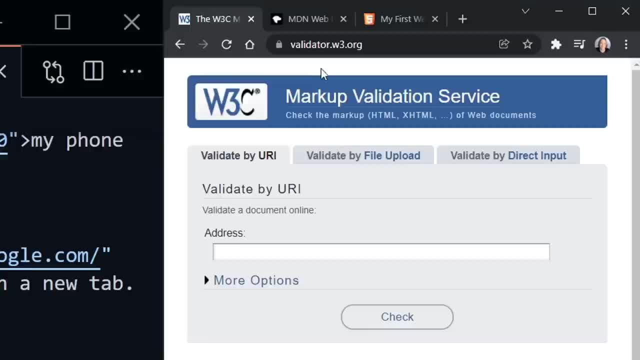 And we've actually added a second web page. Let's go To validatorw3.org And validate. Make sure that we don't have any errors In our indexhtml And our abouthtml. We're going to choose: validate by file upload. 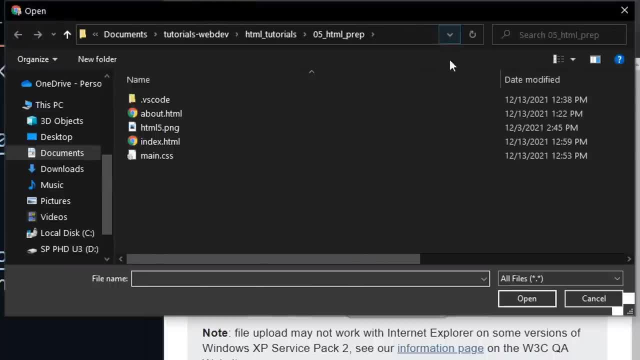 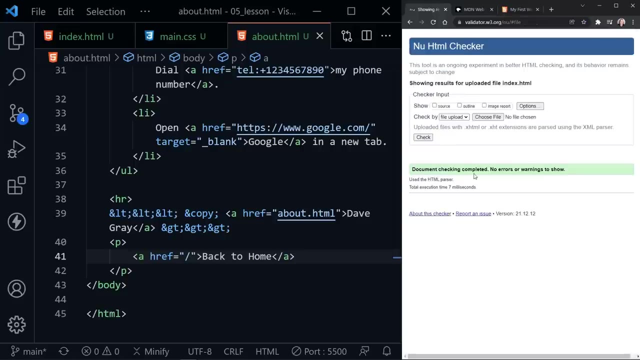 And choose file. And for me, I'm going to have to go into my html tutorials folder, Click html course And I'm in the 05 lesson here. So indexhtml, Open the file And check And document checking complete. 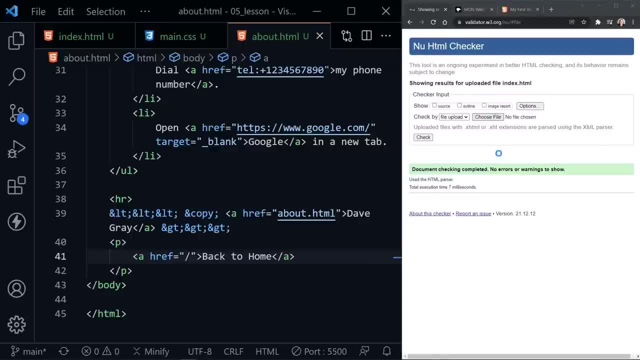 No errors or warnings to show. Now we want to do the same thing for the abouthtml And let's check that as well. And once again, Document checking completed: No errors or warnings to show. If you have errors or warnings, Of course, follow up on what it shows you here in the validator. 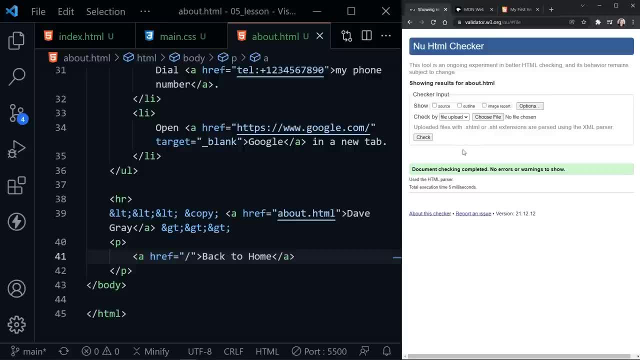 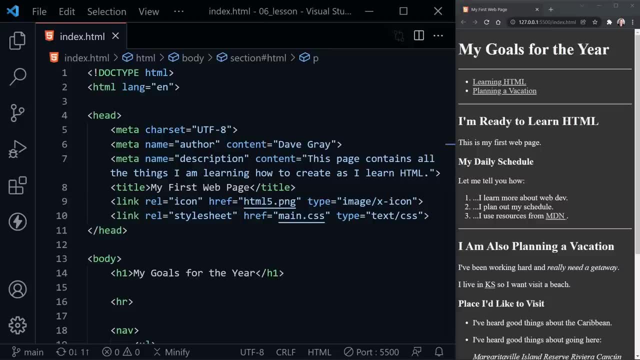 And I hope you've learned a lot about the different kinds of links You can create in your html files. Let's look at adding images to our web page. Until now, we've only worked with text, But html supports multimedia, And images are a big part of that. 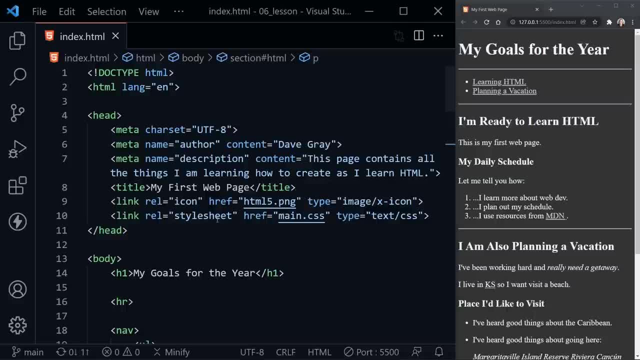 So what we want to do is go to visual studio code that I have here on the left And I have our project running here on the right And we're using live server for that. So the live server has launched down here And you can click to close the server or open the server. 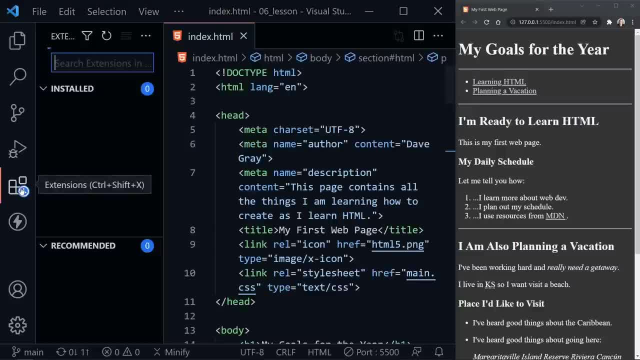 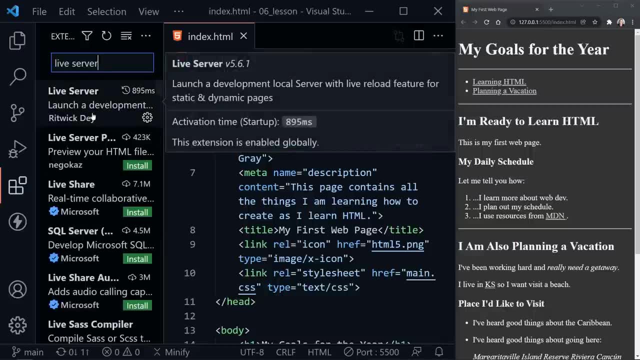 If you don't have the live server extension, Search for that here in the extensions, Find live server, And that should pull up by Ritwik day And you just want to install that And it can launch your page for you, Okay. 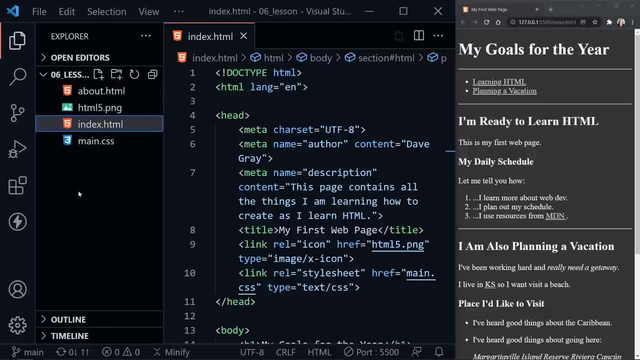 Going back to what we need. We have clicked on the file explorer in visual studio code And we need to create a folder to hold our image files. So I'll type img to name this folder. And it is a common practice to keep your images for your web page or web pages in a separate folder. 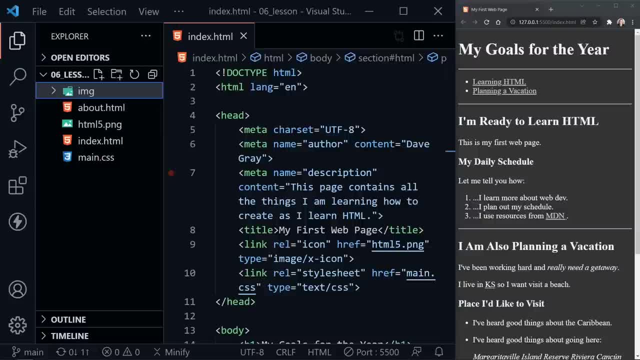 As you organize your project. Now that we've got that, I'm going to grab some images and paste those in so we can work with them. You'll be able to download these images from the files and resources that I share in the description. 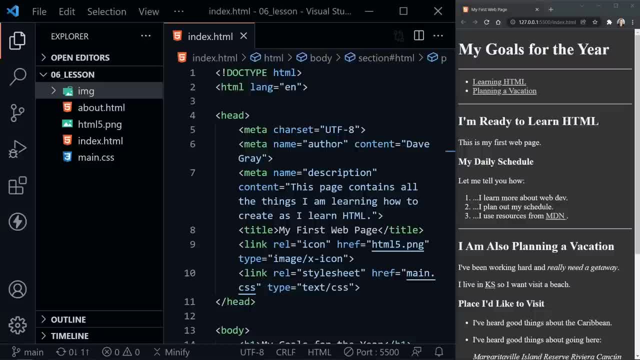 However, at the end of this tutorial, I'm also going to go over some resources where you can download your own images that are free for use. So now, inside this image folder, I'm just going to right click and choose paste And paste these images in. 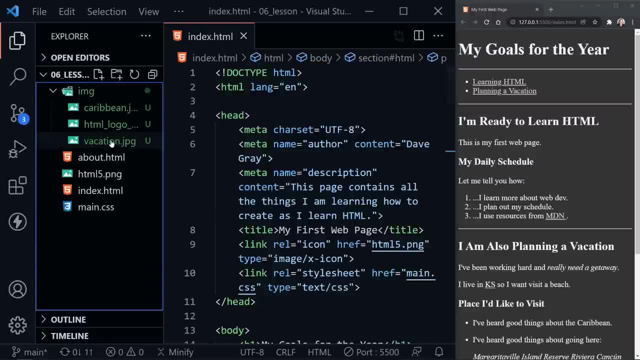 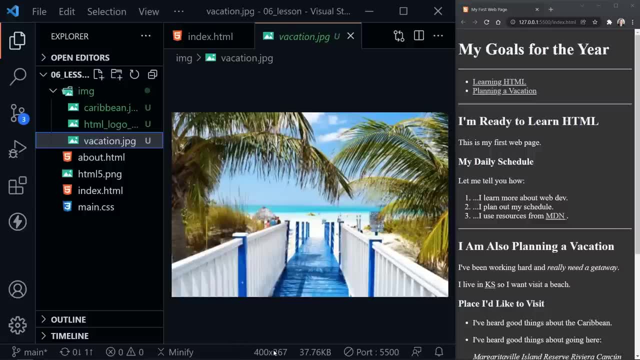 And let's look at what we've got. I can click on the vacation image And I get this vacation image here And notice at the bottom we can see the size of the image: It's 400 by 267.. Those are pixels. 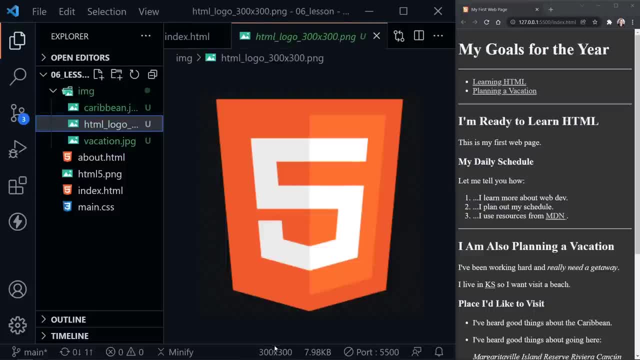 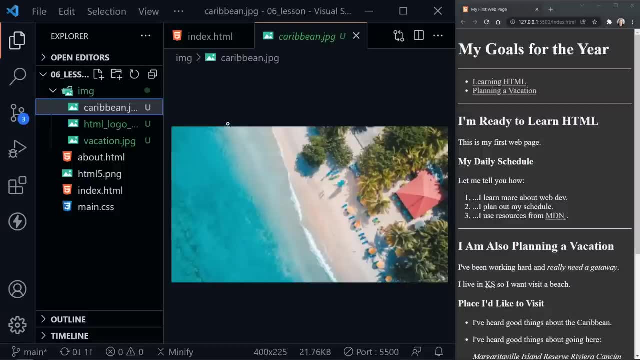 We can look at this HTML logo that we're going to use. It's 300 by 300. And we've got an image of the Caribbean as well, And it's 400 by 225.. So I'm going to collapse this now. 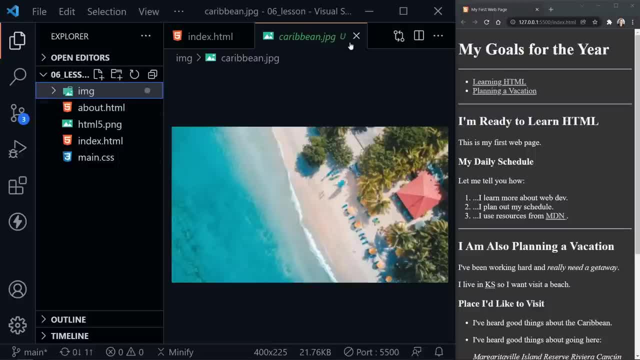 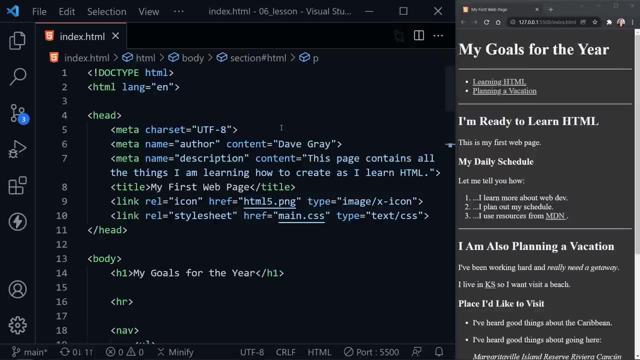 And we're going to use those, And we're going to use those in our HTML code. So now I'll click on the file explorer to hide the file tree. And this all starts with the image tag. So let's scroll down in our HTML to where we want to insert our first image in our page. 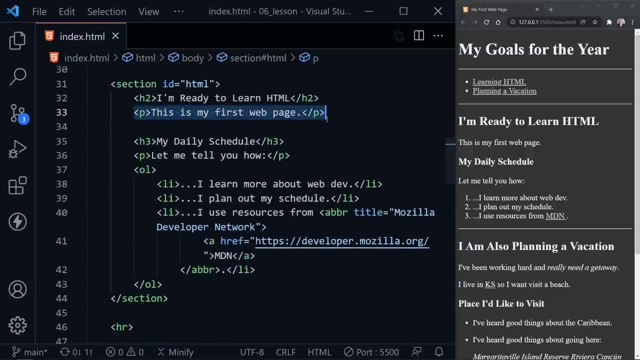 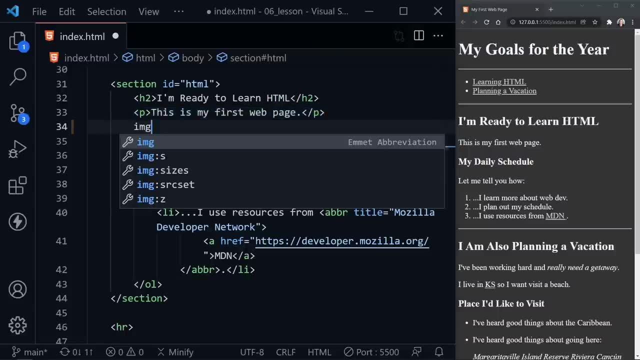 We're going to put it right below the paragraph that says: this is my first web page in the I'm ready to learn HTML section. Okay, let's start by typing img and pressing tab, And then Visual Studio Code will help us with that image. 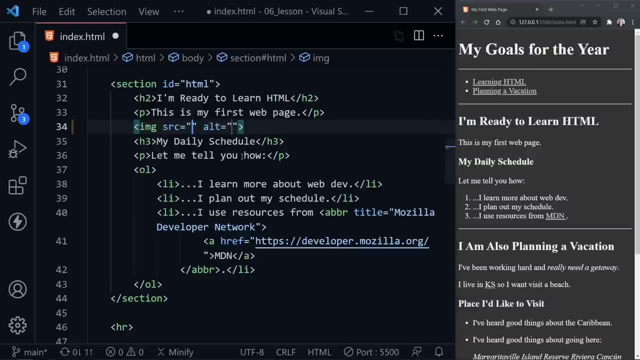 And it will automatically fill out the rest of the image element. Now notice: the image element doesn't have a closing element, like we see here with a heading or we see here with a paragraph. Sometimes you will see it with a slash like that at the end, which means it's self-closing. 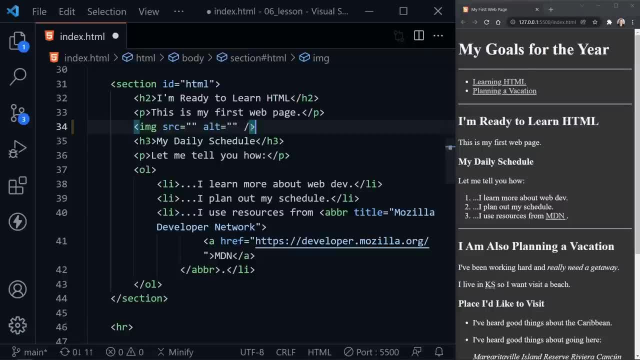 HTML does not require that, Or I should say, HTML5 does not require that. However, if you are using this in the future in something like React, it may require that. So that's just something to be aware of. Right now, I won't put that in because HTML5 does not require it. 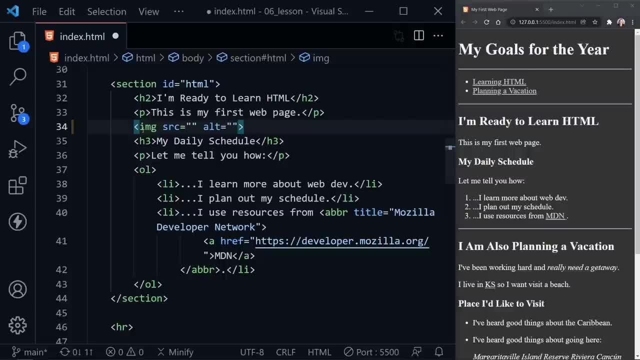 And that's what we're focusing on. Okay, notice: the image element has a source attribute and an alt attribute. automatically, The source attribute tells HTML where to grab the image we want. So we start by typing the folder name that we created, And now we see the folder here: img slash. 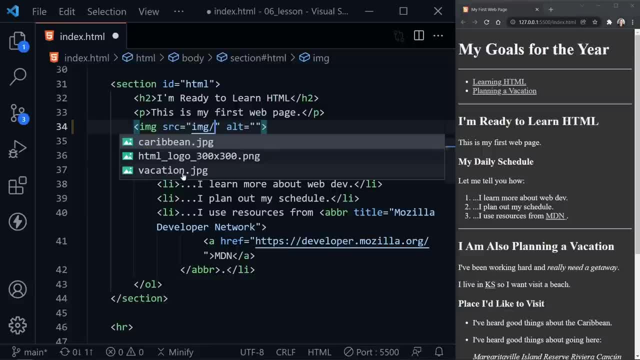 And I can click on that, And then it provides us the names of the images that we have. Well, we want the HTML logo that I saved, So I'll just click on that And there is the full relative path to our image. 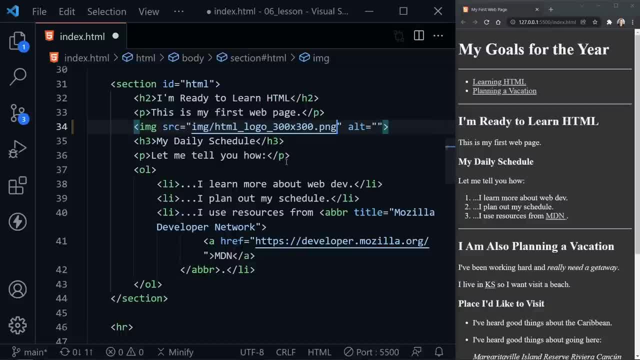 It's in the same project here And it's on our local server in this area, So we don't need that absolute URL that would grab it from somewhere else on the web. So this is once again a relative path to our folder and then to the image. 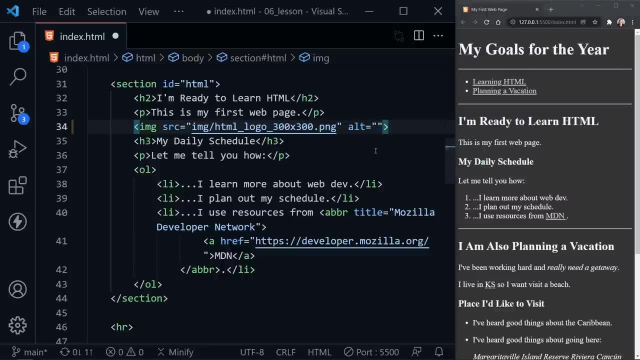 Then we have the alt attribute. Now the alt attribute has a couple of purposes. One is to help assistive technology For those that may not be able to see the image we are putting on the page. the assistive technology, like a screen reader, will read the description of the image. 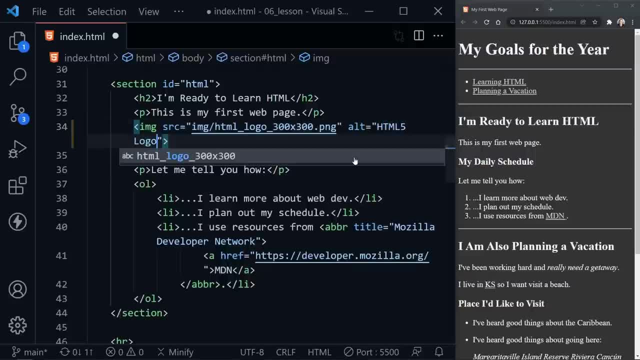 So let's put HTML5 logo as the alt text, But this also makes this alt text appear on the page if the image for some reason does not load. So first of all, let's just save our page And you'll see the logo. 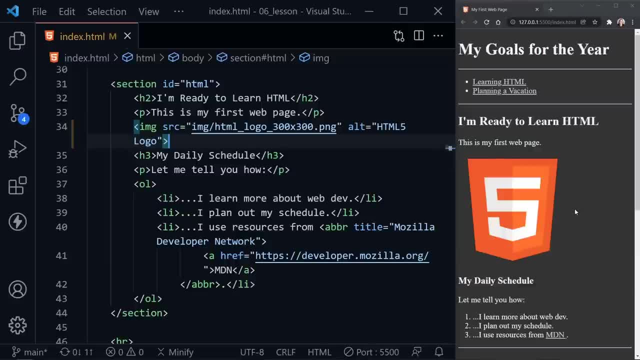 Now appear on the web page And suddenly our page got much more interesting. It's awesome putting images into our web pages. However, let's go ahead and change the file name so that it doesn't find the image, And let's see what happens on the page. 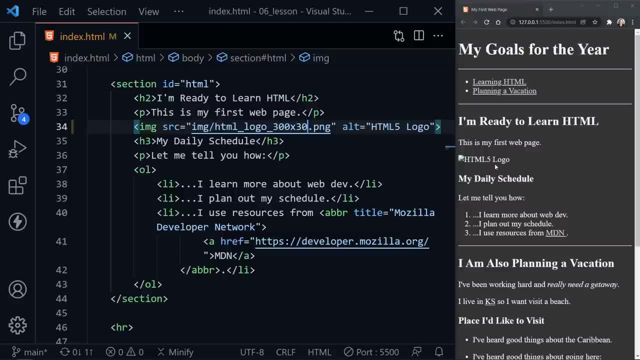 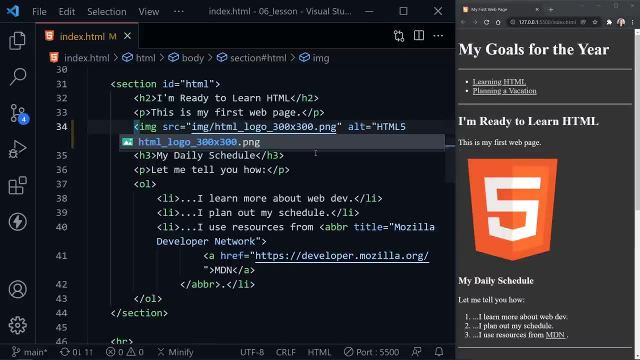 Now we have a broken image icon But notice our alt text appears- HTML5 logo. So that is another purpose of the alt attribute. I'll fix that so we get our logo back. Now there's other attributes That we can and probably should use with an image. 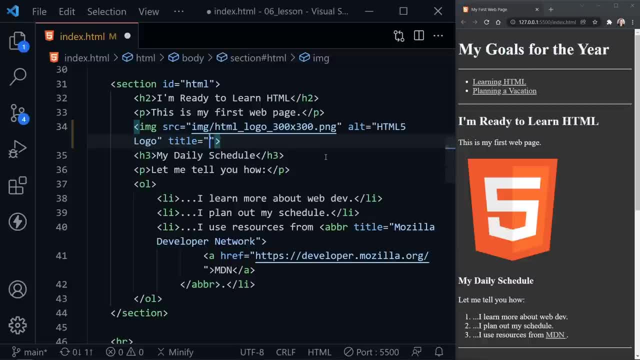 So one is title. Now we've seen the title attribute before. Remember: the title text that we provide here in the title attribute is not accessible. A screen reader will not read it, So this can't be something that is very important that everybody should know. 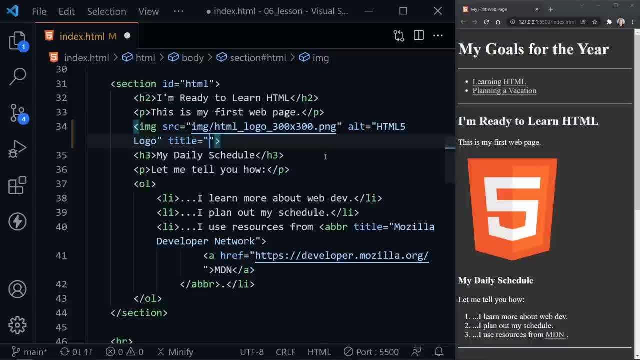 This is text that can complement our image, but it's not necessarily required. The page is complete without it, But we can add some complementary text here, So I'll just put: I am learning HTML5.. It doesn't have to be. I don't even need the period, really. 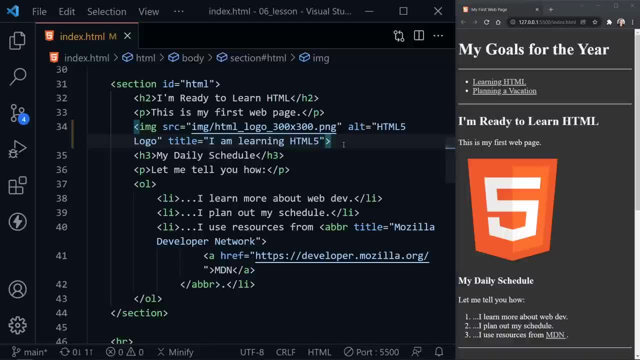 It doesn't have to be identical to the alt text at all. This should be complementary, But now if we mouse over the image, we'll see the title pop up that says I am learning HTML5. And that's complementary. A couple of other attributes. 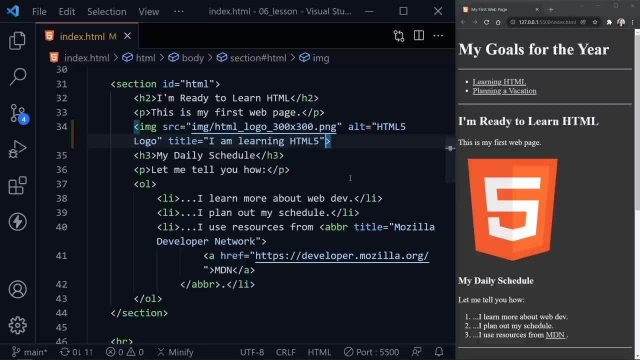 That way. back in the 1990s, These were required. However, for years these have not been required, But now they're coming back And it's width and height. So if we define a width here And we want to provide the same width of our image, 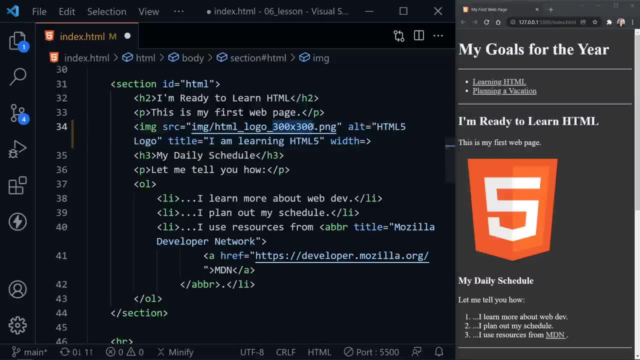 Now I saved this image with a file name that tells me, or reminds me exactly the width and the height, And it's 300 pixels by 300 pixels, So I'll just put 300.. If we just provide the width, HTML will work. 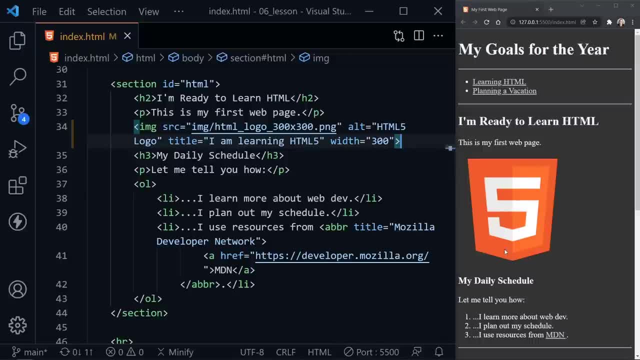 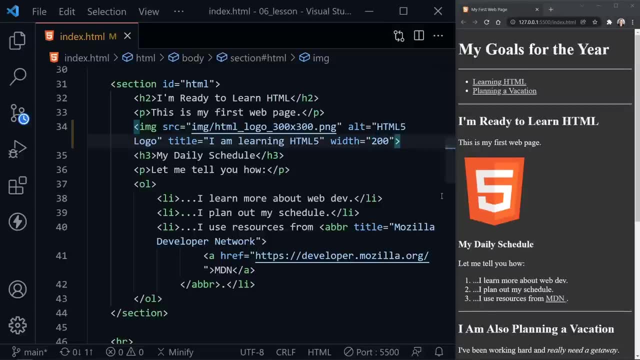 It will remember or shift the image to match, So the aspect ratio stays the same. So if I switch this to 200 and save, Notice it also adjusted the height of the image. However, we want to provide both. We want to provide the width and the height. 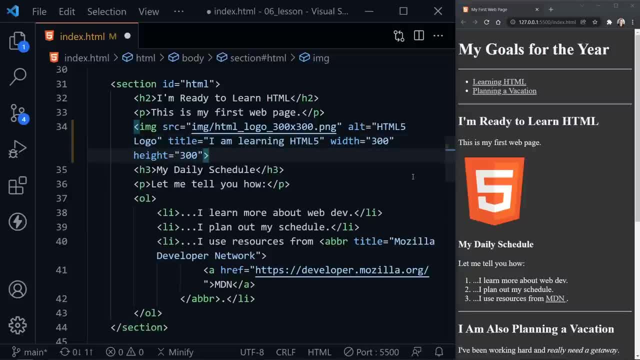 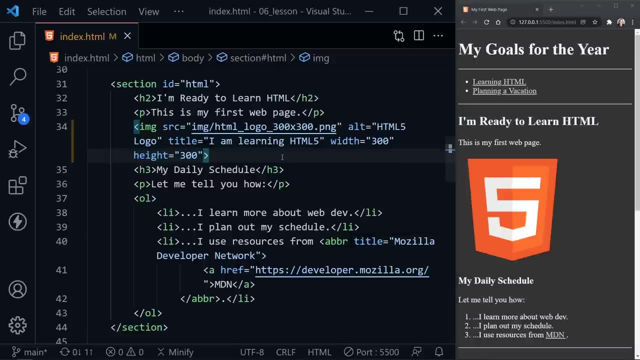 And let's provide exactly what they are. And I'll tell you why this is making a comeback And why it is now recommended to provide the width and the height, Even though we can change this in the future with CSS. So I'm saying: we provide these. 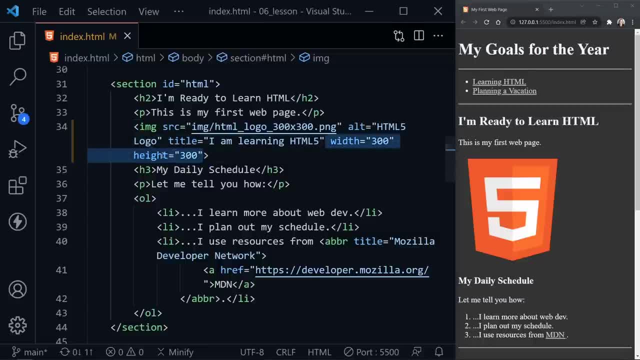 But, yes, CSS may change and override these values, So why do we provide them? Well, it's a little complicated, But it's called cumulative layout shift. If you've ever gone to a web page And you were getting ready to click on something, 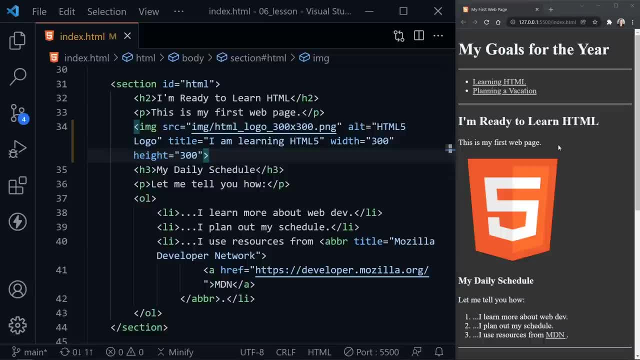 And then you saw the page shift around, Maybe a pop-up ad appeared or a banner ad And you clicked on something that you didn't intend to click, Because the button or the image that you wanted to click suddenly moved. That is cumulative layout shift. 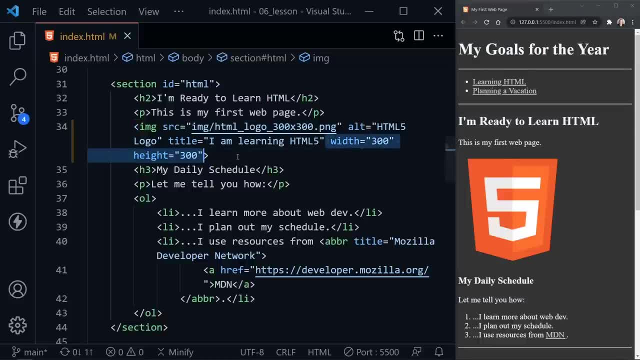 So we provide the width and the height now To tell the browser: Hey, this is going to take up some space here, And this is how much. If we don't provide that, The browser shifts everything once it figures out the size of the image. 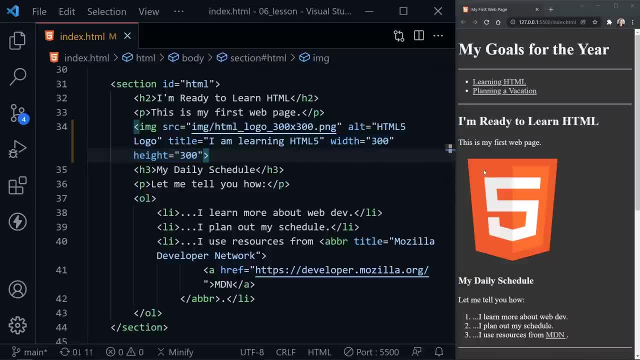 Now, once again, you can still change the size of the image, Make it responsive, Which would adapt to mobile devices And everything else with CSS. So we really provide this information with the width and the height Just to give the browser an idea. 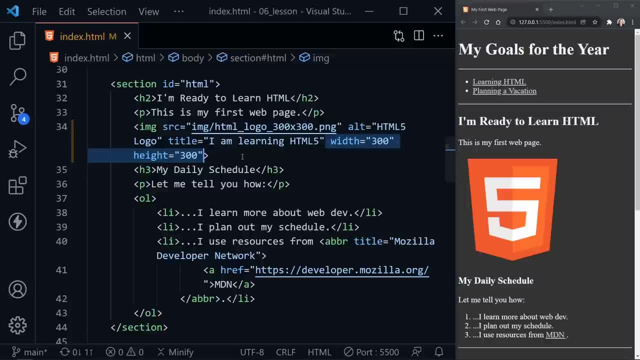 Of the size and the aspect ratio Coming in, So it just kind of prepares itself, And that helps just a little bit. It is now recommended by Google developers That we do provide the width and the height In the image element With our first image added. 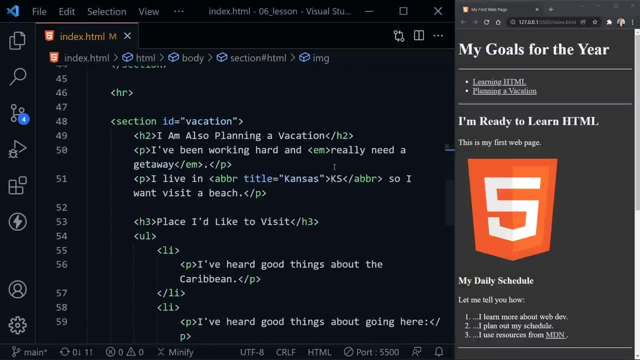 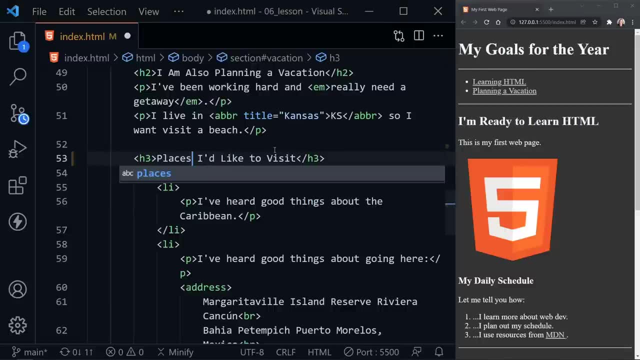 Now let's scroll down And add a second image to our page And we'll scroll down to our vacation image And we'll go to our vacation area, Place I'd like to visit. Let's change this to places I'd like to visit. 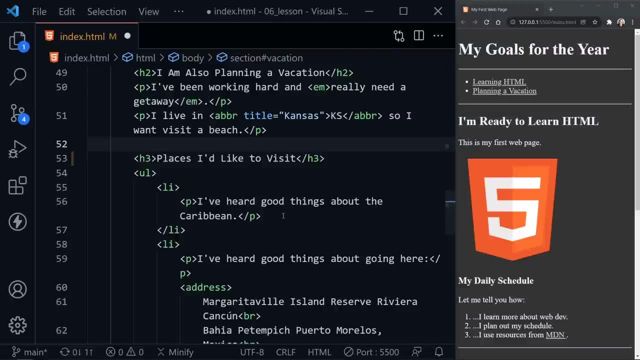 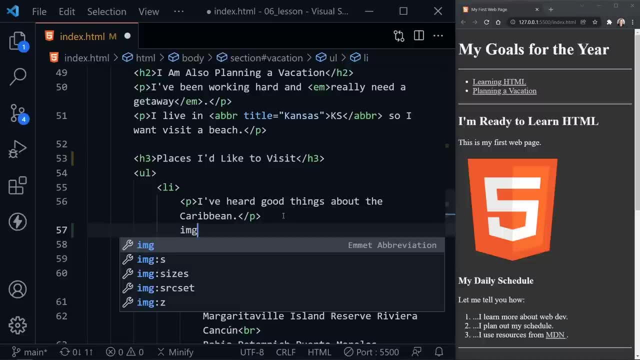 And they've got. I've heard good things about the Caribbean, So this seems like a great place to put an image of a Caribbean beach. So once again, We'll type our IMG abbreviation And press tab, And then Visual Studio Code helps us out. 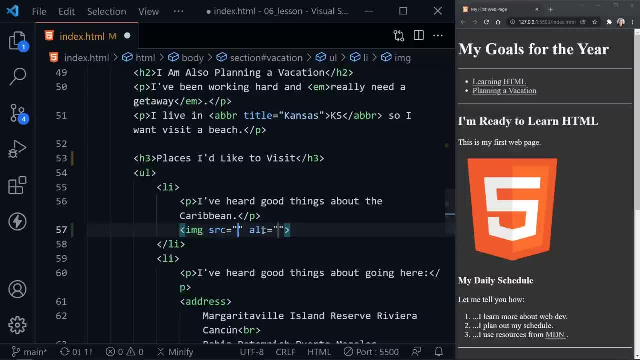 By providing the image element With the source and alt attributes ready to go. So for the source, Once again Type the name of our folder, Press slash, And now we get the names of the images we have ready. I'm going to choose Caribbean. 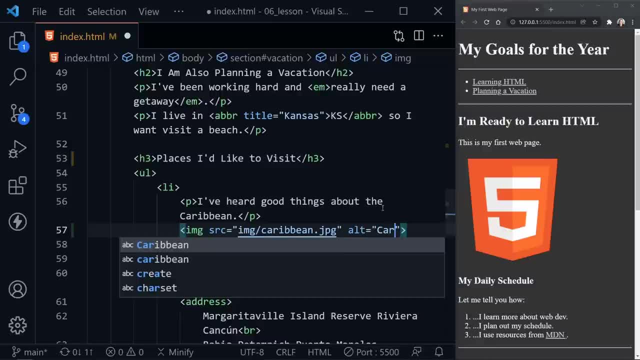 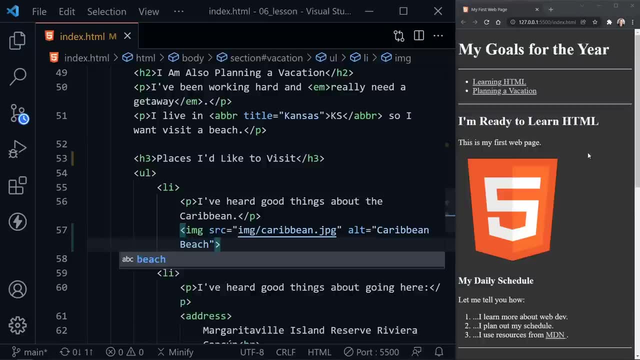 And then in the alt area I'm going to type Caribbean Beach. And now let's save And see what we get on the page When we scroll down, Because we have to scroll down a little ways to see it, And there is our Caribbean Beach image. 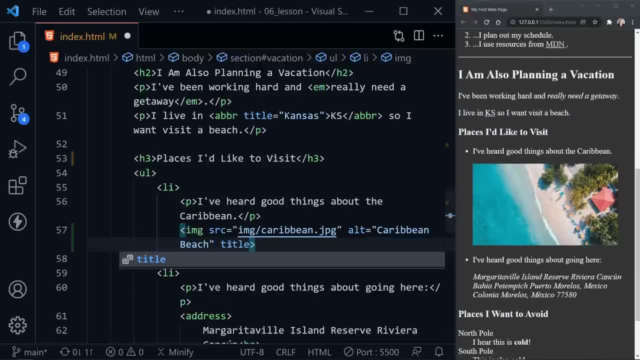 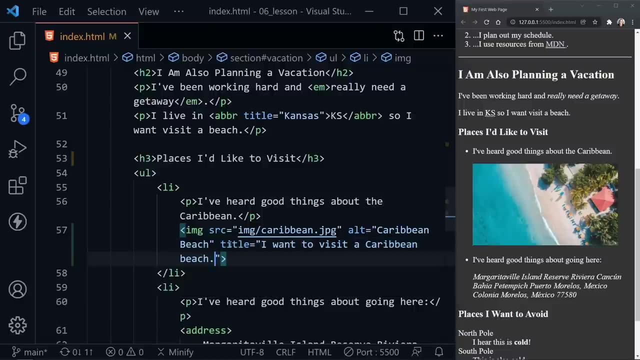 So now let's add a title attribute That's just a little different than our alt attribute, Just complimentary text, And this is: I want to visit a Caribbean beach, And we'll save that. Now we're getting closer, But remember. 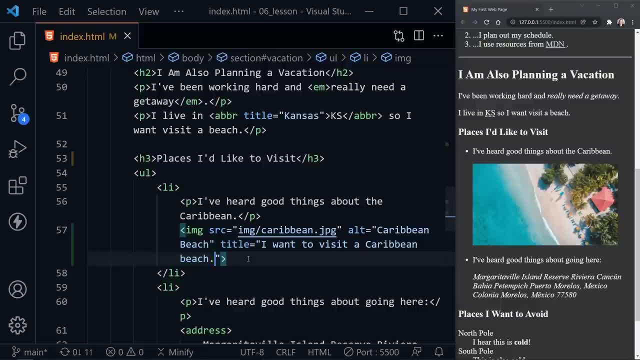 We should apply the width and the height attributes as well. So let's click on the file explorer, Because I didn't have the width and the height saved in the name of this JPEG file: Dot JPG. Notice, the other image we used was a dot PNG. 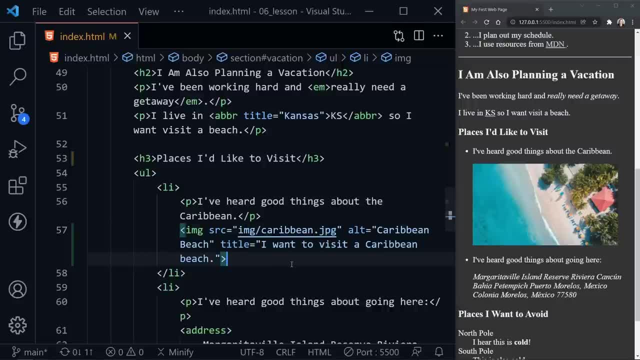 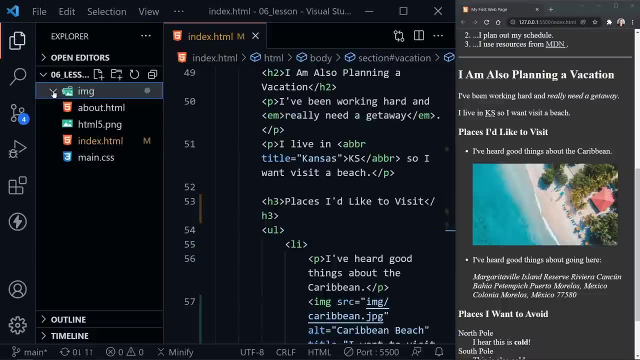 There are different image file types And those have different extensions. So now I'll click the explorer up here, We'll go back, Open the image folder And I'm going to click on the Caribbean image, And when I do that in Visual Studio Code. 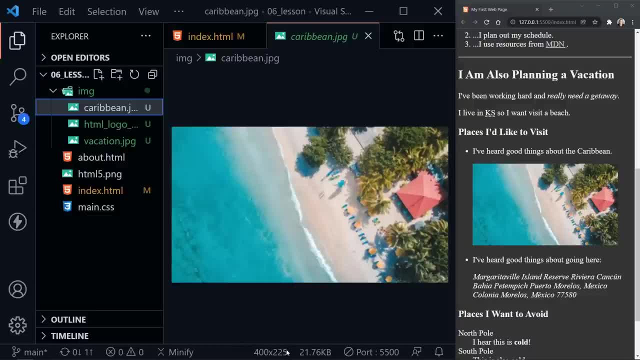 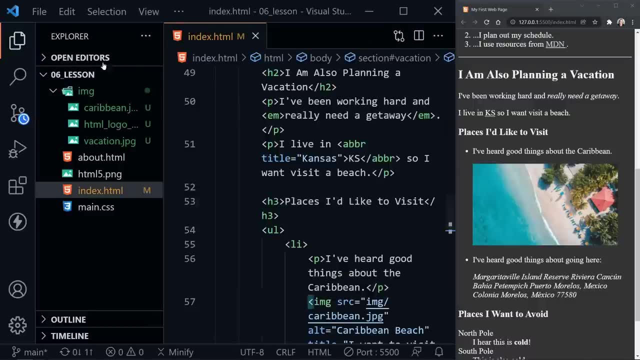 It shows the image And at the bottom I can see it is 400 pixels by 225.. The first number is the width. So I'm going to close this now. Click file explorer to hide that. So I have a little more room. 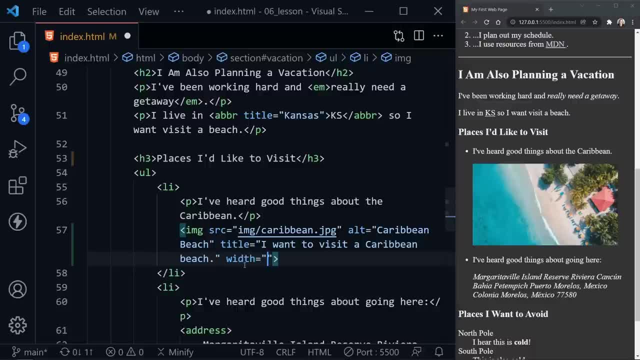 And now I can say: width equals 400.. And the height equals 225.. And if we save, Everything should remain the same. We've just provided these extra attributes. Now I've noticed that this wrapped a little strange here in Visual Studio Code. 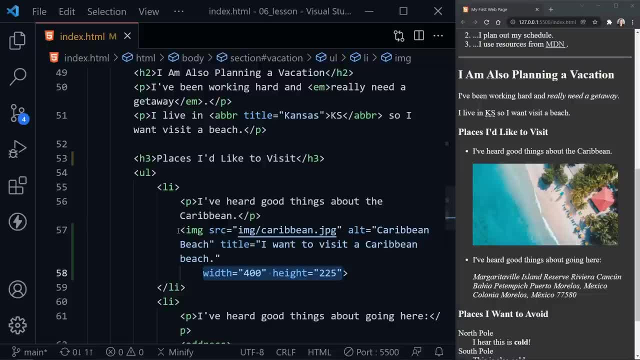 But know that the width and the height are still part of the image element that we started right here. Okay, Now that we've got that, Let's go ahead and remove the in from the jpeg, So it will not find the image, And make sure our alt text appears. 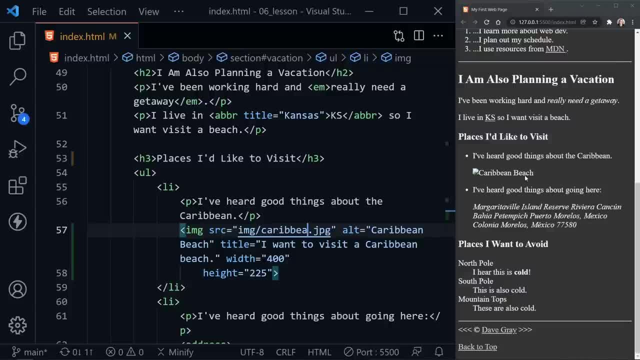 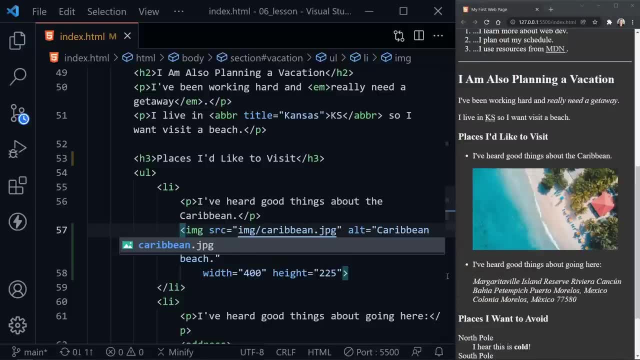 Yes, we've got a broken image icon, But it says Caribbean Beach And that is our alt text. So I'll fix that by putting the in back in the name, Spelling it correctly And the image shows up, Because now Visual Studio Code can find the file for us. 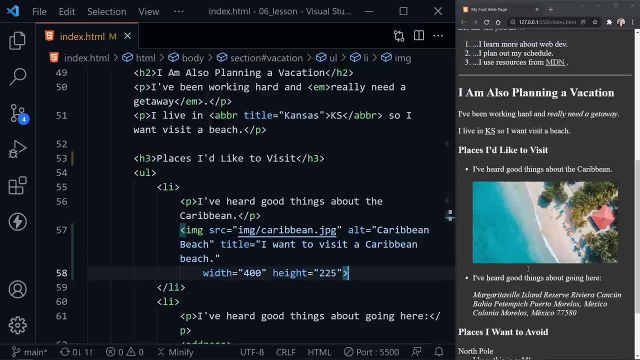 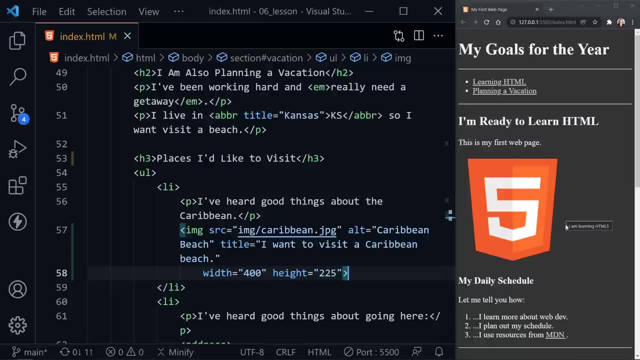 Okay, We had to scroll down to see this image Because our page is long enough that if we scroll to the top We don't see our vacation area anymore. Now, this bottom of the page here, You could call it a crease if it was a newspaper. 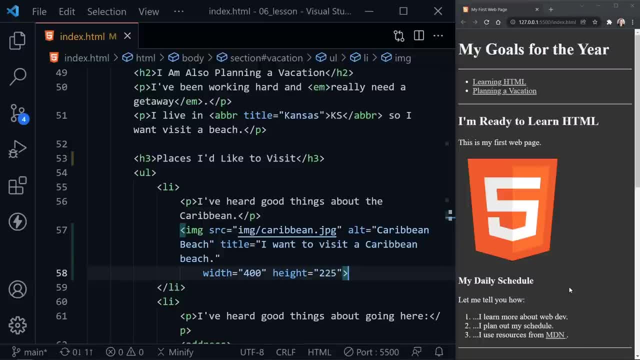 And a lot of the terminology kind of goes back to newspapers and magazines as we talk about layout And so this bottom part that defines the line That anything below that we do not see right now That's called the fold. So anything after this area that we can now see is called below the fold. 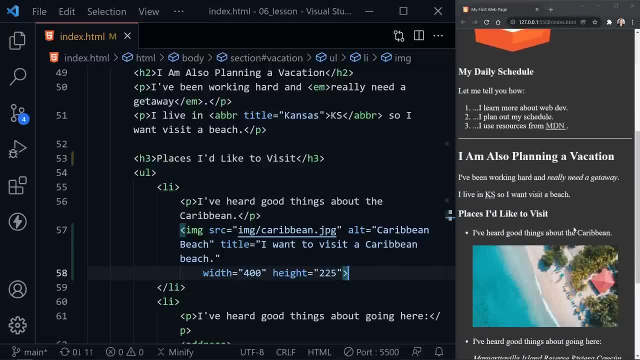 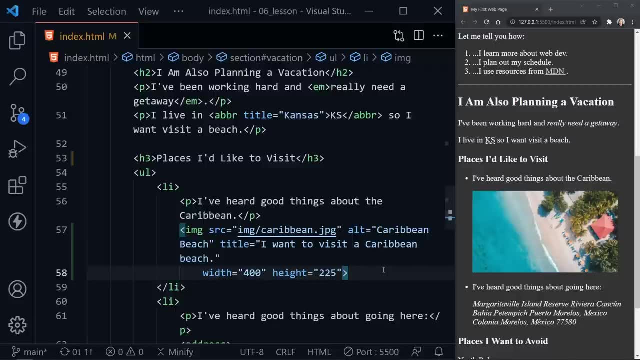 So anything below the fold We have to scroll to see. And now we scroll to see this image. Well, there's one more attribute for this image that I want to talk about, And it's the loading attribute. And if we provide loading, 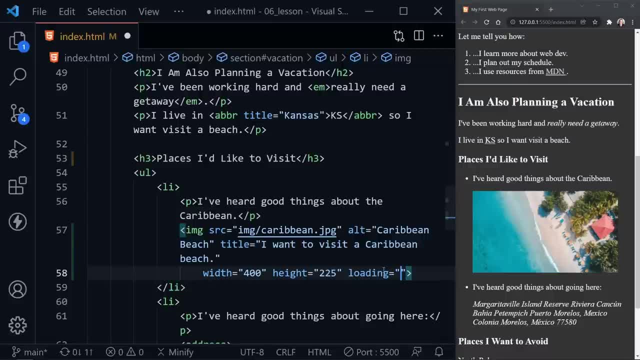 And we can set it equal to a value. And there's two possible values. The first one is eager, But we never have to provide this. This is the value by default. So if we do not provide the loading attribute, The loading attribute is always there. 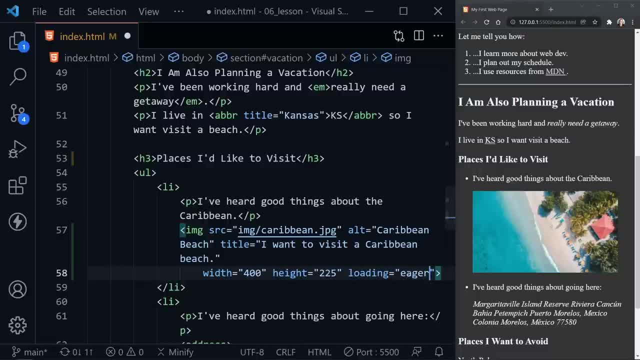 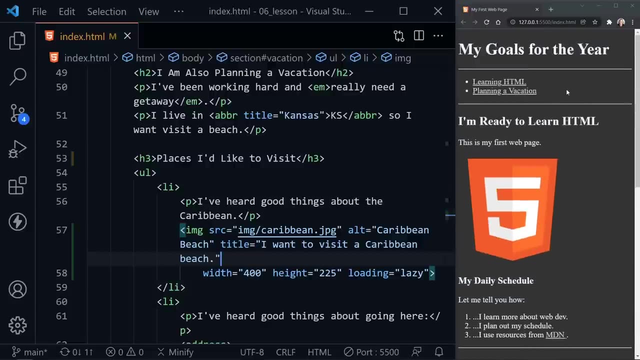 And it's just set to eager. We just don't see it. But the one that we do need to provide is called lazy, And what you want to do for performance for your web page is for any image that is below the fold, That is, one you do not currently see when the page loads. 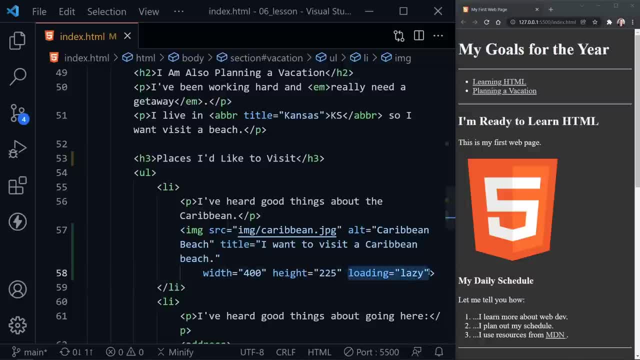 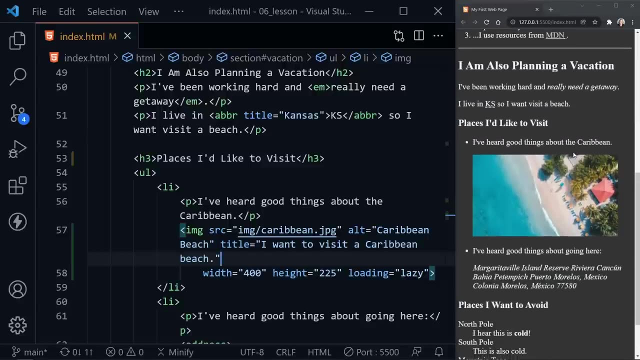 You want to set the loading attribute to lazy, And that means the browser will only load that image when it knows it is about to show it When we start to scroll. Now Firefox, the web browser, Firefox, is much easier to demonstrate this in. 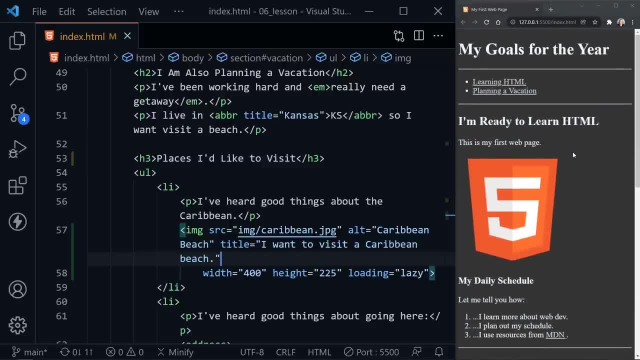 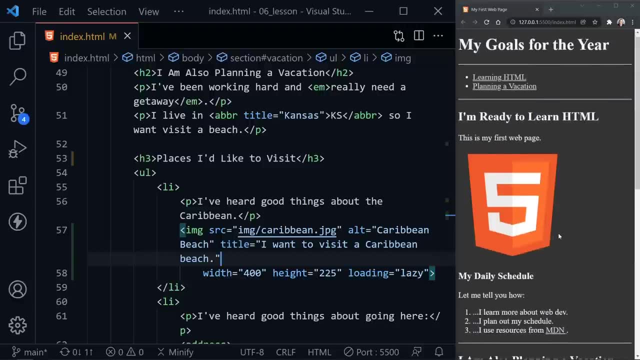 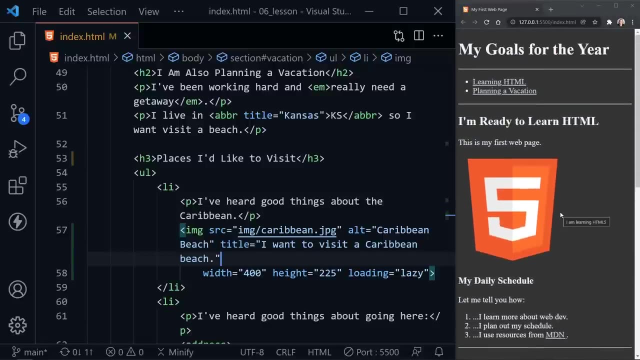 Chrome wants to display the image much earlier, So right now this image is close enough to the area that we see that it will still load this Caribbean image automatically that we have here. So I need to create some extra space And I can demonstrate this to you by using something called Chrome Dev Tools that's available in the browser. 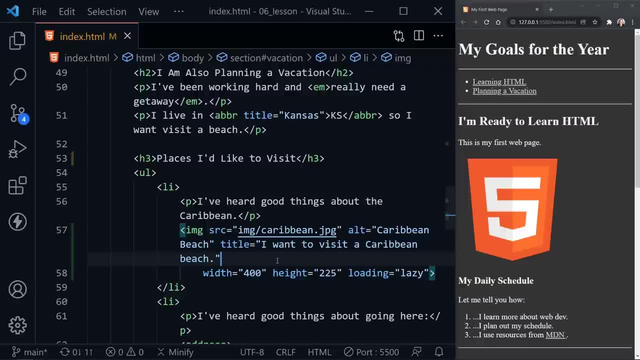 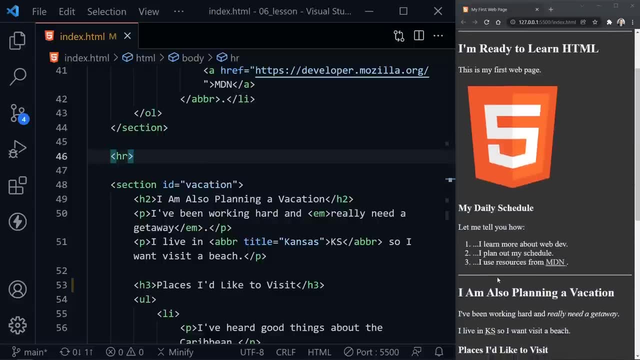 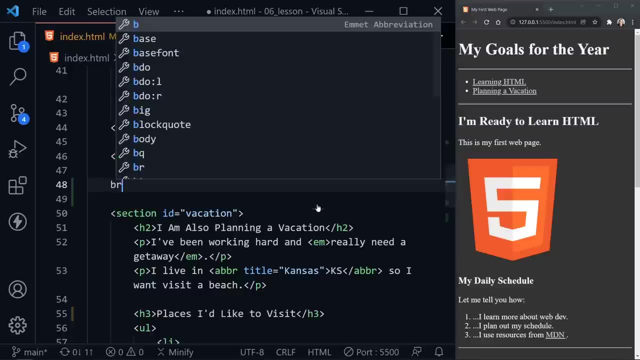 So let's do that. now. I'm going to scroll back up above places I'd like to visit, to the HR area, The horizontal rule that we have going across right here before the. I am also planning a vacation And I'll type an abbreviation- BR- for a line break. 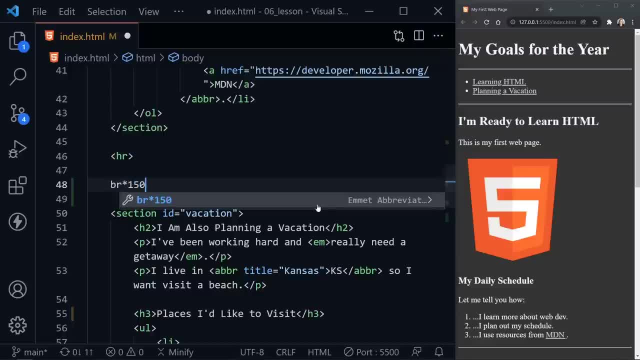 And then I'll put the asterisk for times And I'm going to put 150.. This Emmet abbreviation that Visual Studio Code supports will insert 150 line breaks- 150 line breaks- into our page. There's no way I would want to type all of those individually. 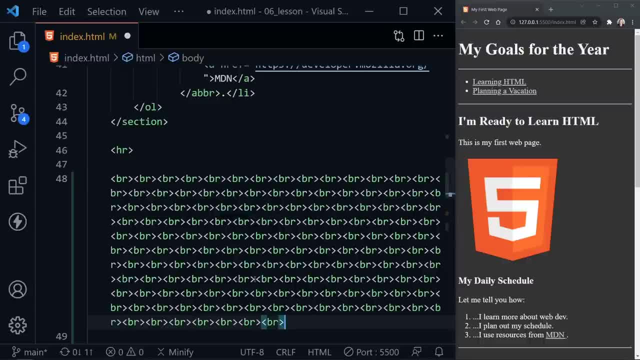 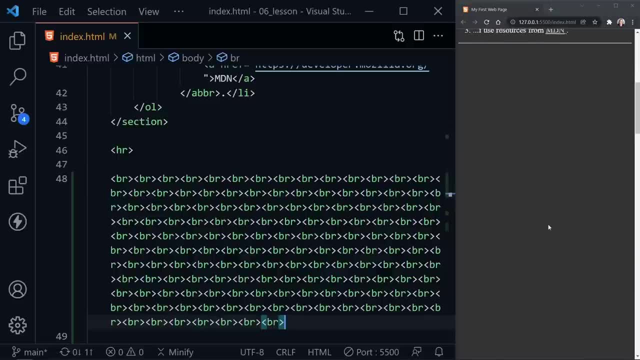 But I can do it with this abbreviation, So I'll click that And suddenly we have all of these line breaks If I save, And we don't see this change. But now there's a lot of space between the sections, And that's what I need: to demonstrate this. 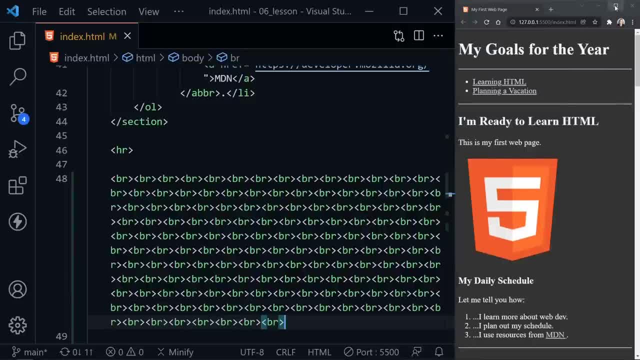 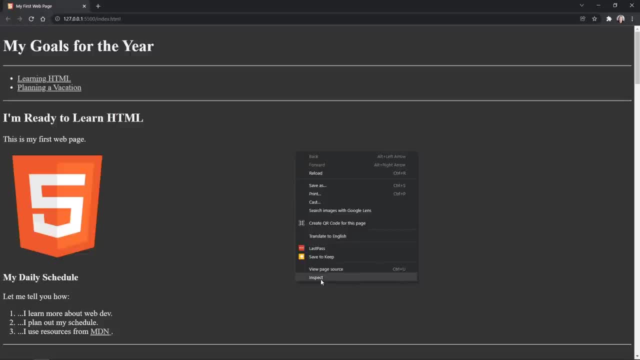 So we've changed the code. I'm going to click the maximize button here in Chrome to bring the browser all the way out. And now let's right click and choose inspect. And you could also do this with keys, And it would be control, shift and the letter I all at once. 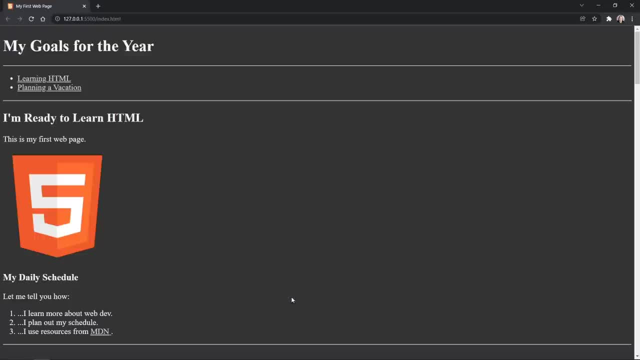 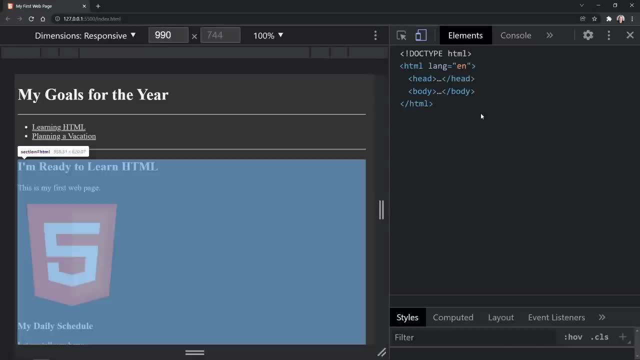 The control key, the shift key and the letter I. I'm just going to right click and choose inspect. Either way will open up the dev tools in Chrome And now that we're getting the dev tools open, it will automatically open to the elements tab. 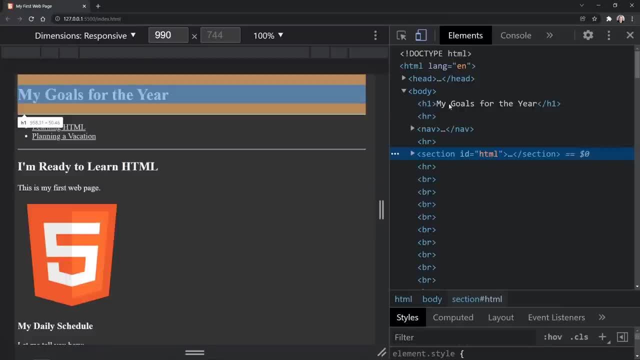 And notice how if I hover over an area in the elements now, it highlights those on the left in the browser. So here I've hovered over my goals for the year And we can see that I can hover over the section that discusses HTML. 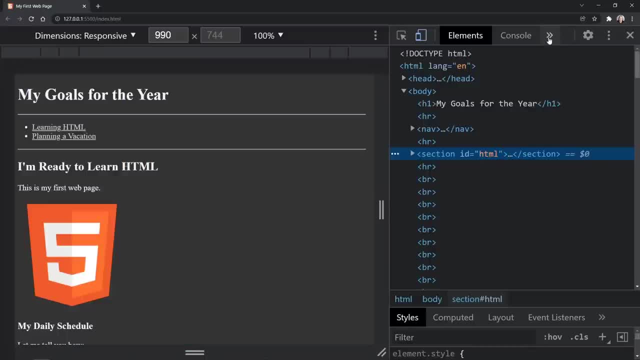 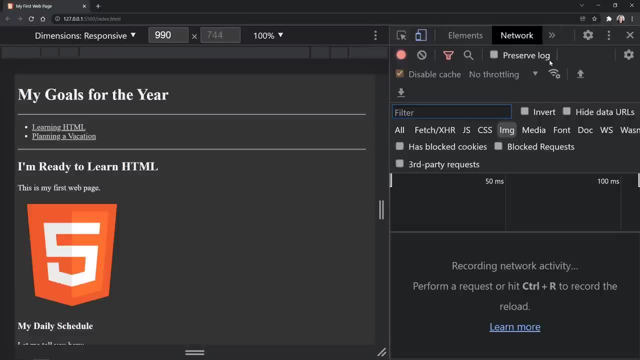 And it highlights that section. What we want to do, though, is click the two greater than symbols here at the top, And I'm going to choose the network tab. Once it shows the network tab, you'll want your disable cache to have the check mark. 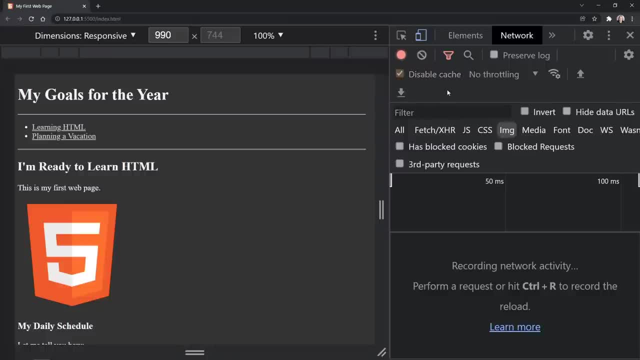 And that is because browsers know to save images after they've loaded them initially. They can reload them fast, But that is called the cache where it stores the images. That's CACHE. We want to disable that cache so we can demonstrate this Also in this area. right below the filters, you see all fetch slash XHR JS CSS. 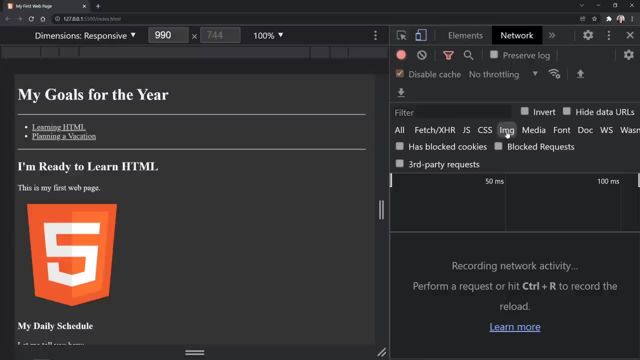 Choose the image. All we are interested in right now are the image files. We don't want to see the rest of the files. So once you've done all of that, we're going to go ahead and reload the page. So I'm going to click the reload icon up here in the browser. 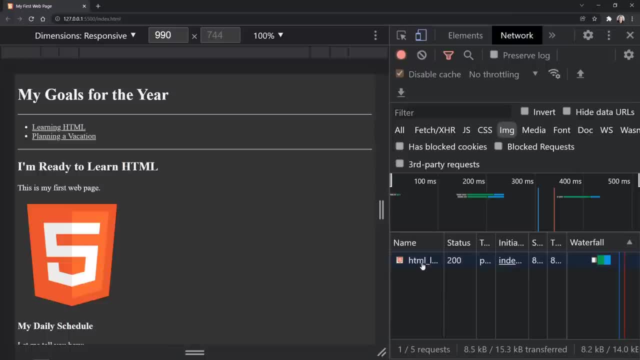 And we've reloaded And notice down here we just see the HTML logo file. That's all that has loaded right now And now as we scroll down, as we get close to the Caribbean image file, we will see it load. 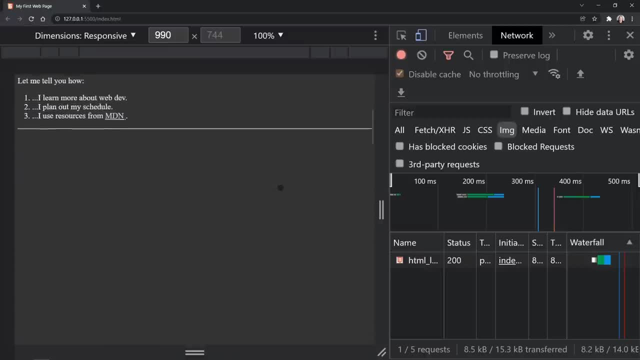 Because it has the loading attribute set to lazy. So only once we get close- And I created a lot of space here, So I'm scrolling down And fairly soon it should pop up. There it is. We don't see it on the page yet over here. 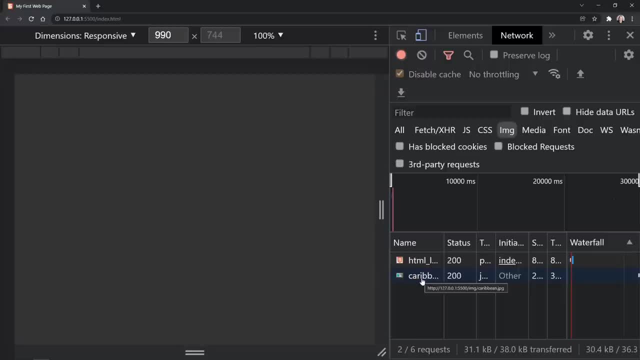 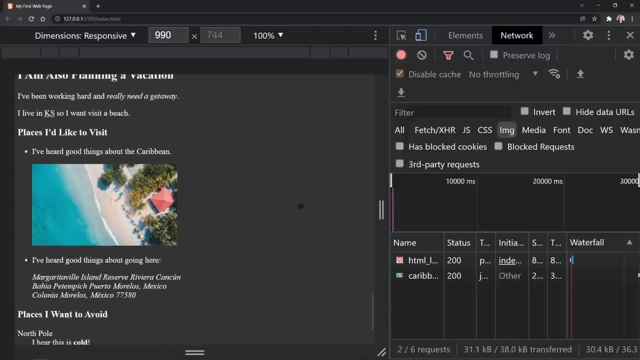 But it's getting close, So Chrome loaded it in preparation for us to see it. But what that really helps is that it did not load the image right when we loaded our page, So that made our page load faster. It only loads these images when it thinks it's going to need them. 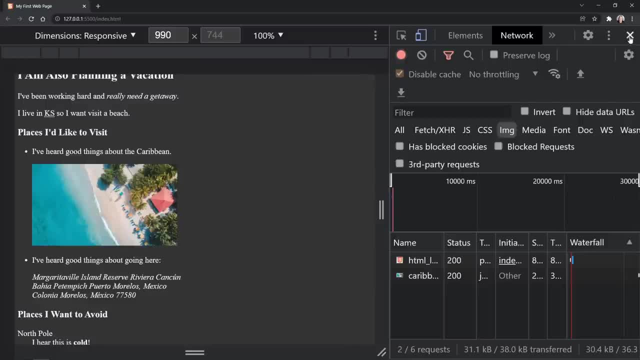 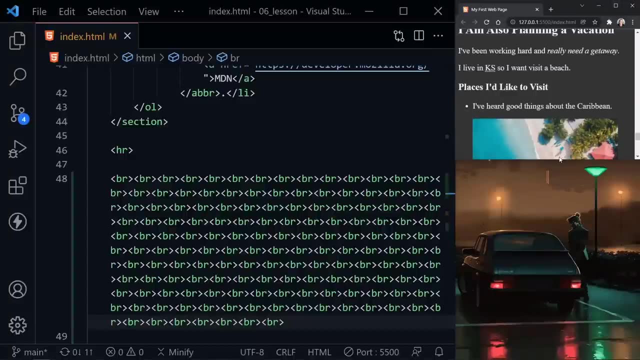 And that is lazy loading. So now you can click the X here in the top right to close the dev tools. Then I'm going to click the maximize button Again to get the browser back to the size we wanted it. I'll drag it down here so we can see everything. 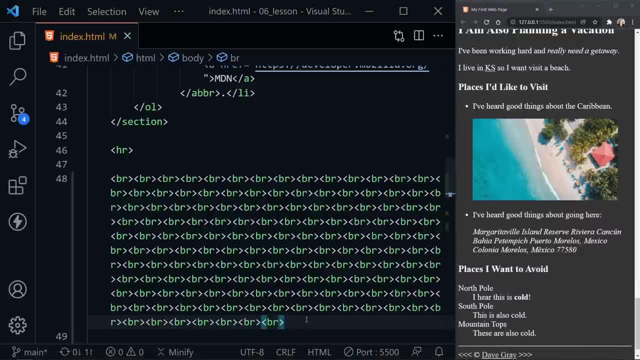 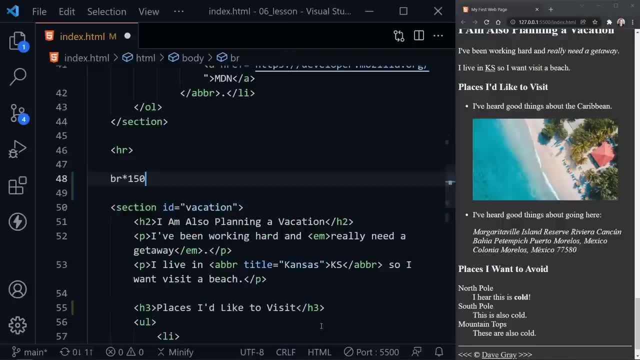 And then over in Visual Studio Code. I'm going to press control Z, which is undo. You can also go to the edit menu and choose undo, But I'll do control Z and get rid of all those line breaks. But again, if you want to demonstrate that, you can just type in BR. 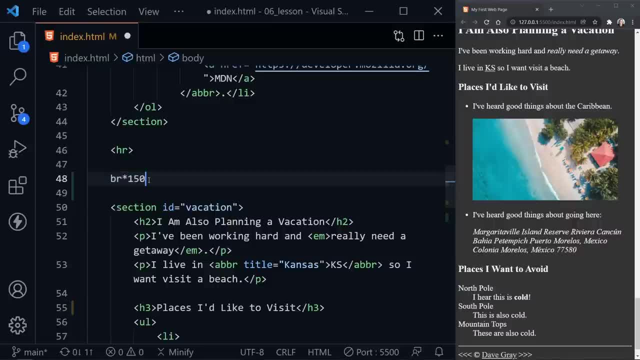 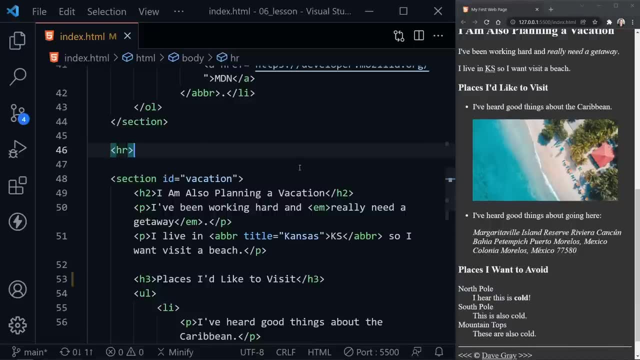 And then how many of those elements you want in Visual Studio Code will recognize that. So that is a demonstration of a lazy loading technique that helps your pages load faster. Imagine if you had a page that had a dozen or 20 or even 50 images. 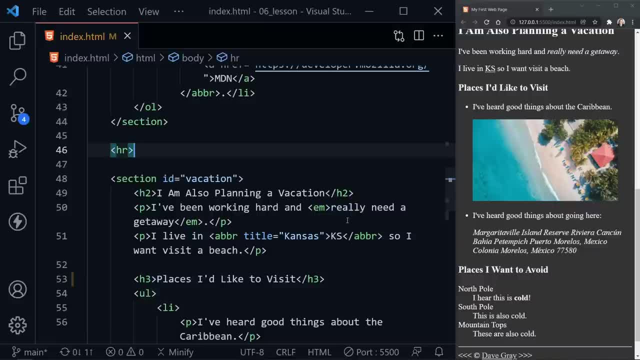 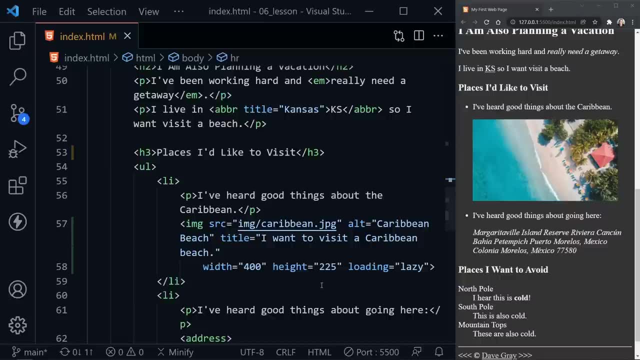 You wouldn't want the page to continue loading until it loaded all of those images. So lazy loading is a very good performance technique, especially when you're dealing with lots of images that are below the fold. Now let's add a new element to our page. 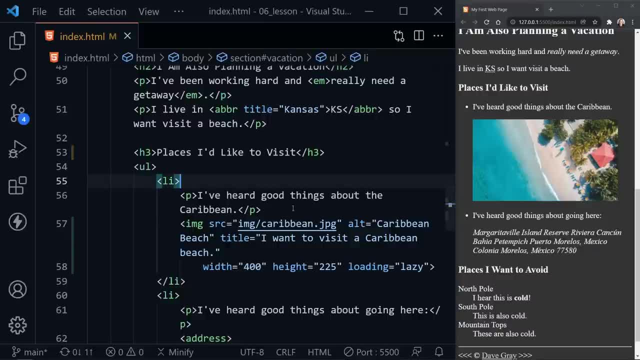 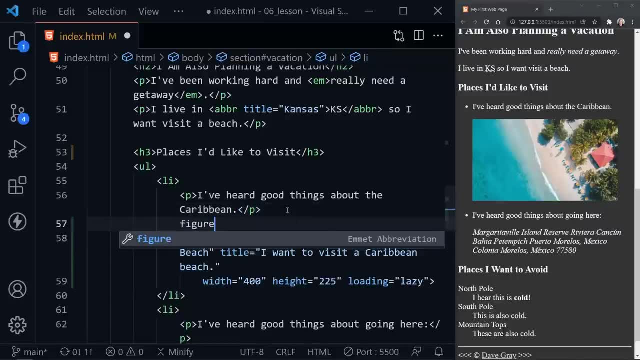 And it's something we're going to wrap this image in. So I'll put it underneath the paragraph that says I've heard good things about the Caribbean And I'm going to type the word figure And I'll press tab, because figure is an element. 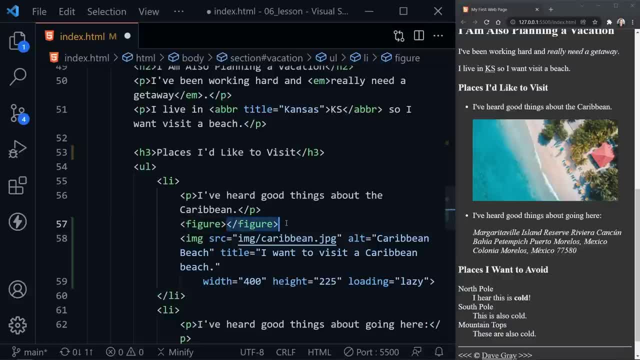 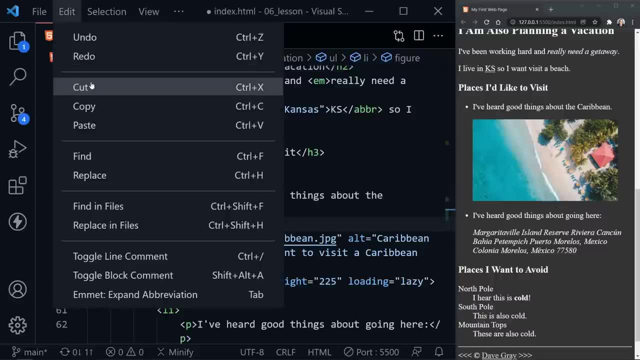 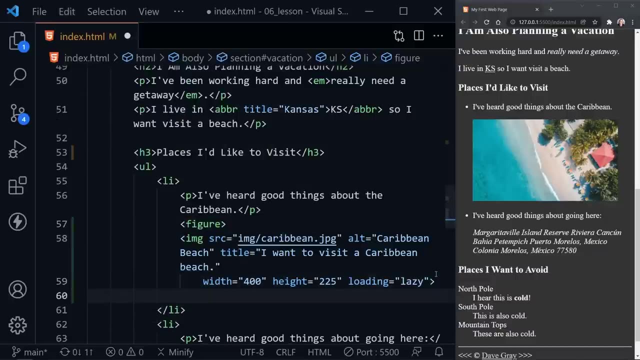 Now I'll highlight the closing tag and press control X to cut. You can also get these options that I use with the keyboard shortcuts in the edit menu. There's cut, copy and paste. So it's control X to cut. And now at the end of the image here I'm going to paste, which is control V. 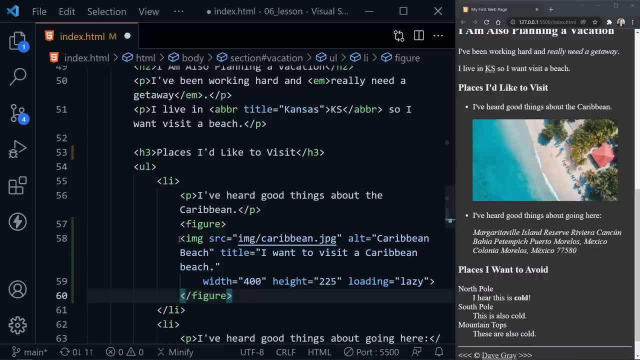 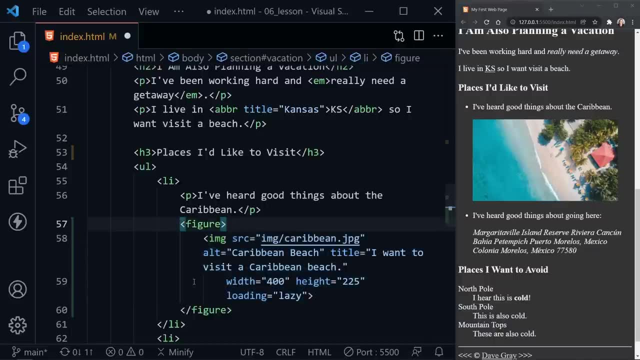 And now I've got it. I've got the opening and closing figure tags. I'll highlight the image here and just tab it in as I'm used to seeing it. So the image is inside the figure element Now. this by itself won't do much. 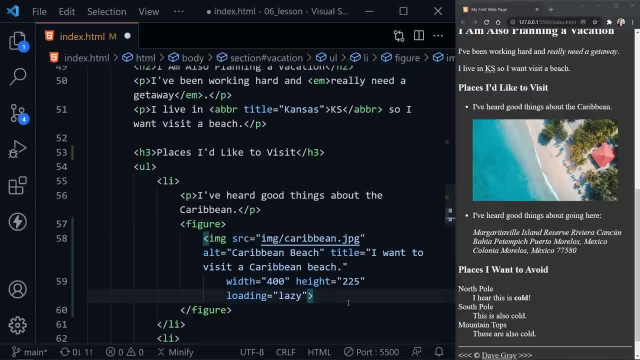 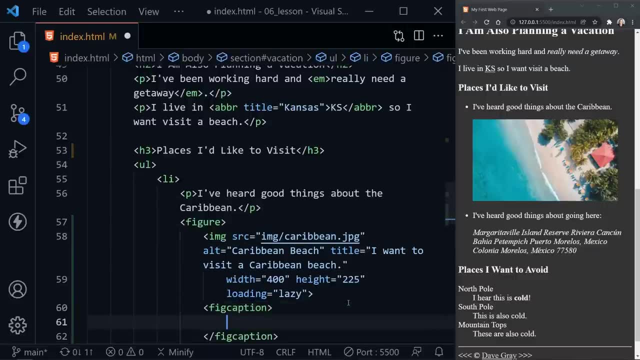 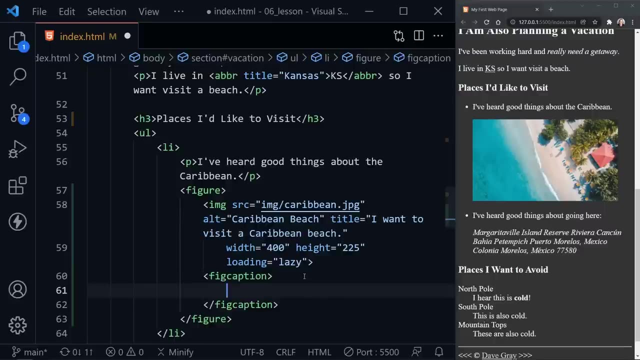 But it is saying we've got a figure with an image And we can add a caption, And it tells the browser that the caption- big caption- element is related to the image, Which is better than just putting a paragraph under there. The paragraph, while we could visually see, it's probably related to the image if it was right under the image. 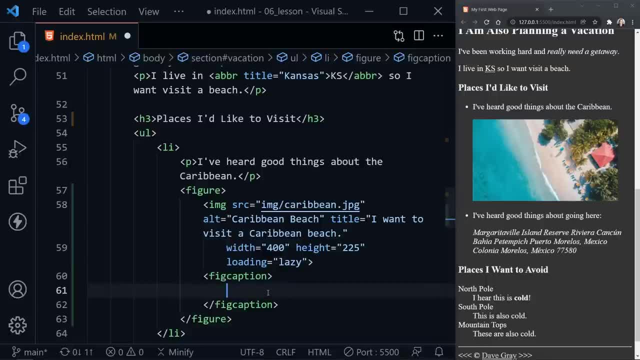 it's not telling the browser or assistive technology that it is a caption for the image. This spells it out for both the browser and assistive technology that, yes, what we put in here is directly related to this image, But it doesn't have to be identical to the alt attribute of the image. 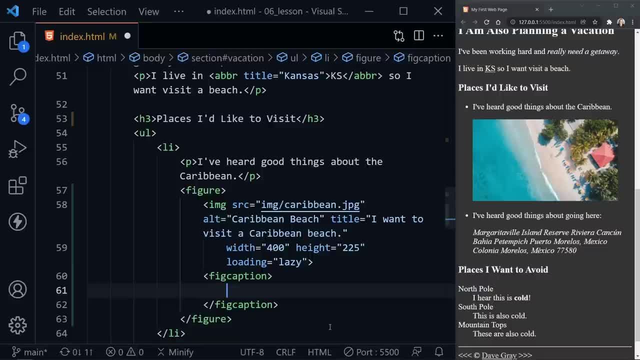 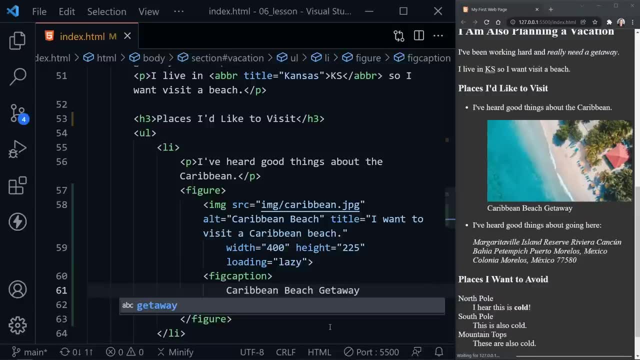 Although it should kind of be a description of the image. So I'll put Caribbean Beach Getaway here as our fig caption. And now it does show up on the page And notice the image has been indented just a little bit And once again we can change all of the layout of the page and how everything looks with CSS in the future. 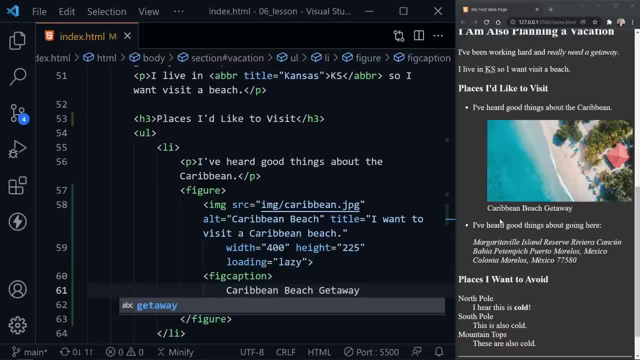 But this is just the default behavior. when we apply a figure, It's indented somewhat, So we have an image and the caption. now Let's go ahead and add our last image as well, And we want to put that underneath. Margarita Island Reserve. Riviera Cancun. 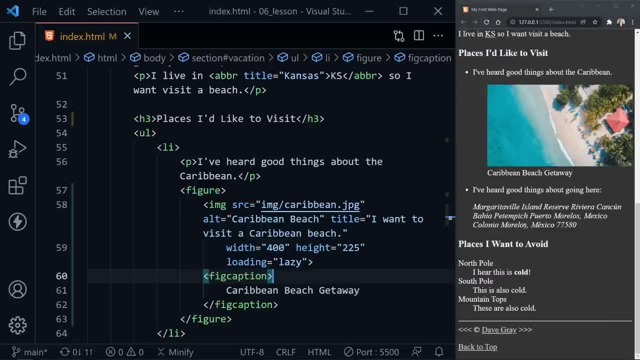 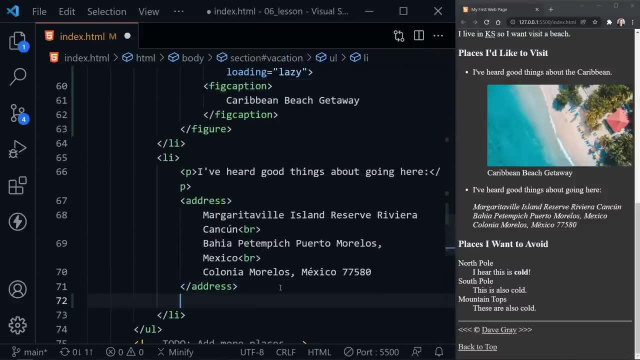 An actual resort in the Mexican Riviera, Cancun area. So we'll scroll down here And underneath the address we want to add an image of at least the Cancun area, Because that's where we're thinking about going. So, image, and we press the tab button and we get the source and alt attribute again. 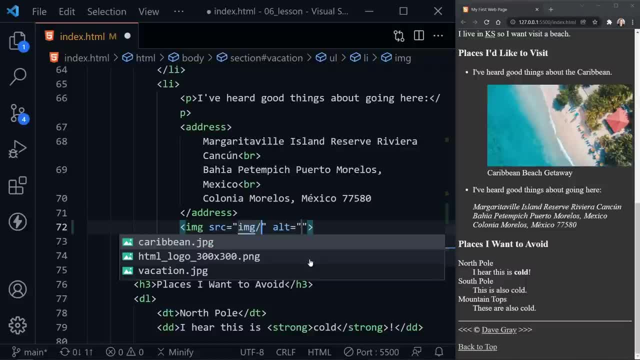 So let's type img- That's the name of our folder- And save Slash, And now we've got our vacation image And that looks good And now we can put in the alt tag the Cancun vacation for our vacation image. 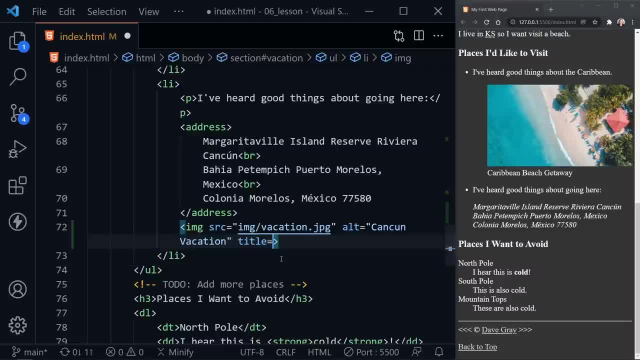 And now in the title we can put something like it's 5 o'clock somewhere- Because that's kind of related to Margaritaville and Jimmy Buffet And he's famous for that- saying: And it's 5 o'clock somewhere. 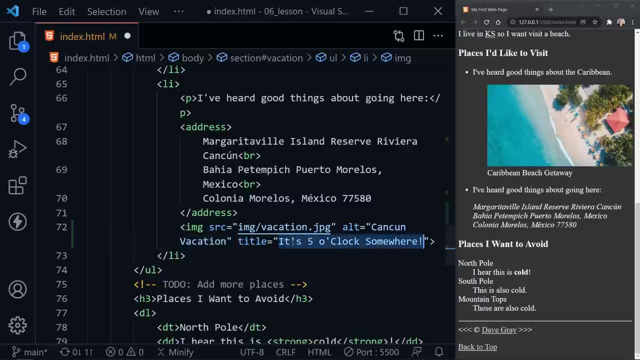 There's something worth noting about this phrase. We've got single quotations here inside of our double quotations. Now that's what's possible. If we had used single quotes out here, this would not be possible. But we can use single quotes inside of our double quotes. 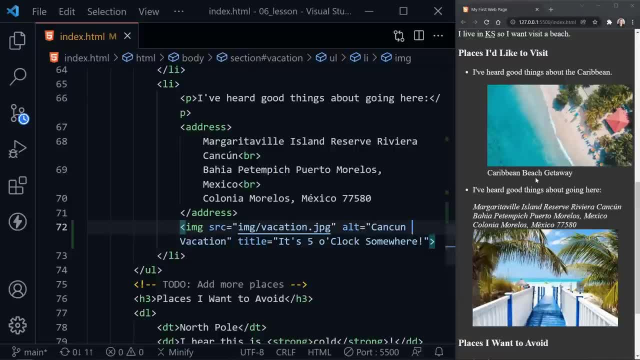 So this does work. Now let's go ahead and save And if we look at the page right underneath the address for the resort we're thinking about, We've got our Caribbean vacation image And if we mouse over, we've got the title: it's 5 o'clock somewhere. 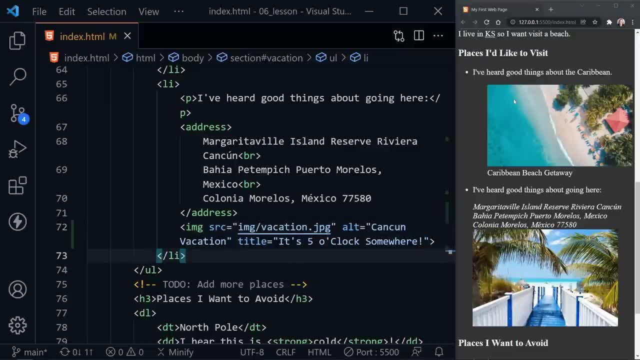 That looks good. But notice, we don't have the space or the indentation that we get from the figure element. So let's go ahead and put a figure element around this image as well. So we'll type figure Press tab. Once again. I'm going to highlight the closing tag. 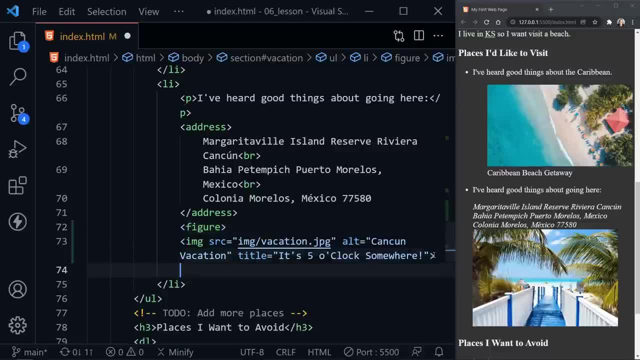 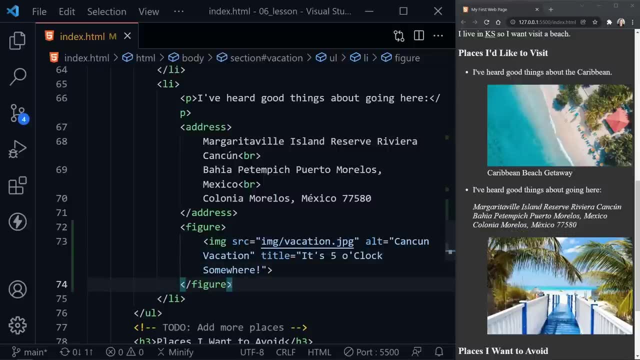 Press control x underneath the image, Control v to paste it in. And if I save I should get some auto formatting. And so now I've got the image indented inside the figure And let's add a caption here as well. Remember, it's the fig caption element. 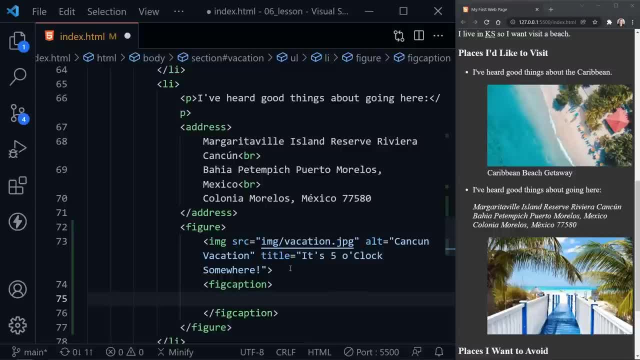 So I'll press tab. And now let's put a Caribbean vacation image. So it's not quite the same as our alt attribute, It's not the same as our title attribute, But it's a nice description of this image. Okay, we're not quite finished with our image. 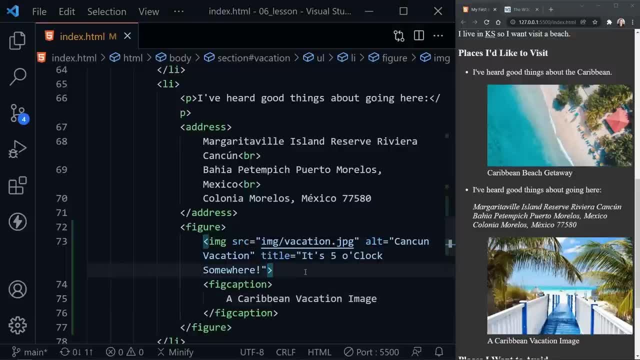 It's easy to forget some of these attributes that we might not think about applying right away. So one we know we need is the loading, because this will absolutely be below the fold. So let's set that to lazy as well and save. And now let's click on the file explorer again in the top left. 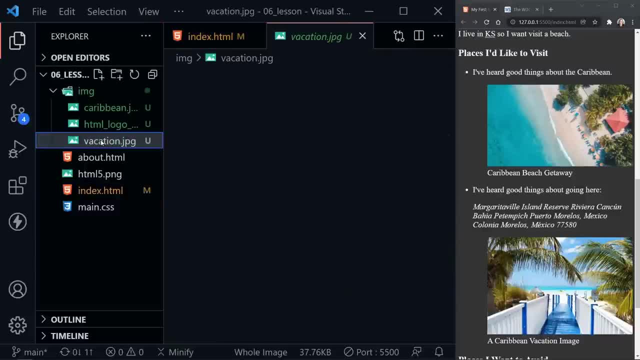 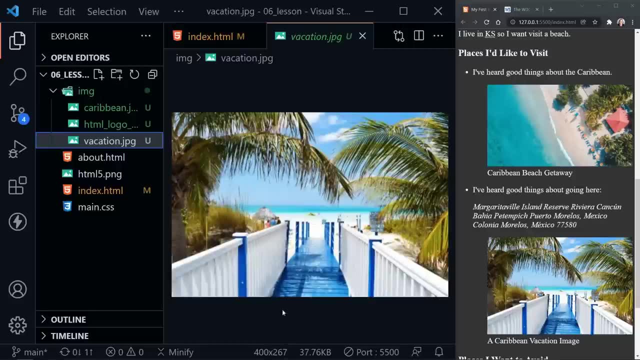 And let's look at our vacation image and find the dimensions And we can see here at the bottom it's 400 pixels. 400 pixels by 267 pixels. So now we can close that out And click on the file explorer to hide that again. 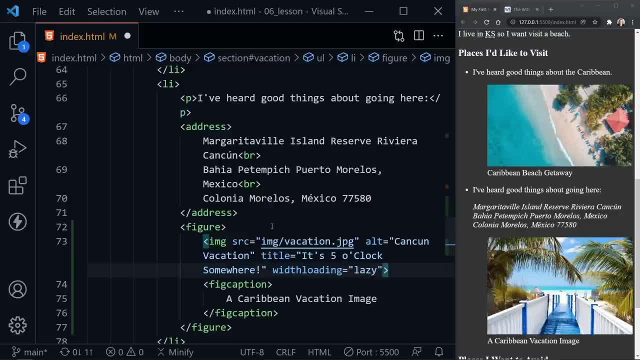 And let's provide width and height, So the width is equal to 400.. And the height is equal to 267.. So now we've provided all the correct attributes that we need for this image, And everything looks good here on the page. 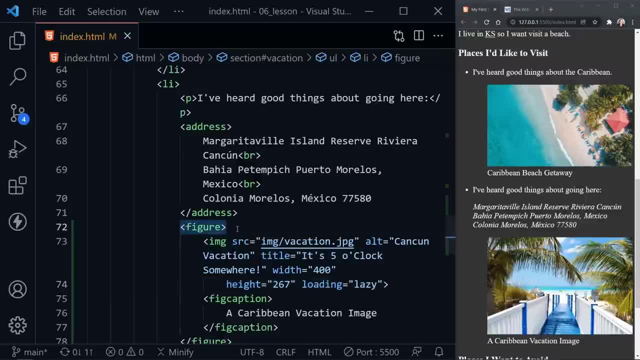 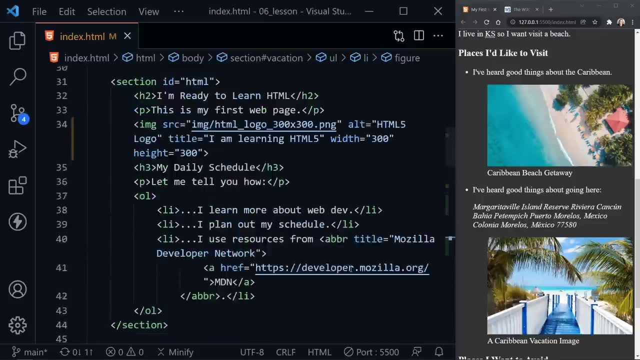 One more thing I want to add About figure. Figure is not just for images, So let's scroll up here in VS Code. back to our HTML area, And we do have our HTML logo right here underneath. This is my first web page. 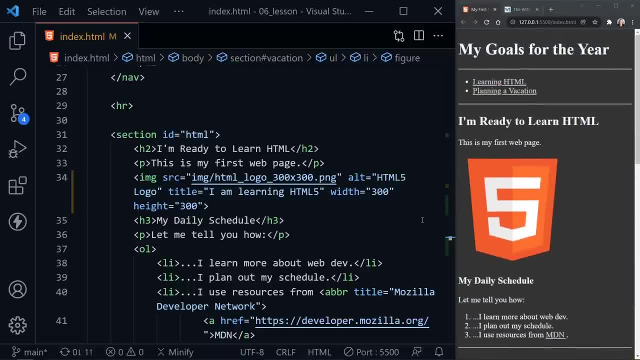 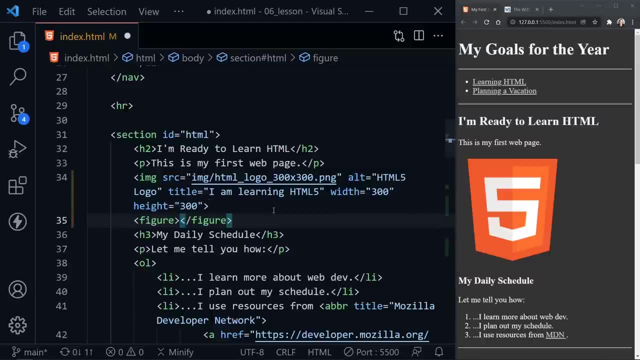 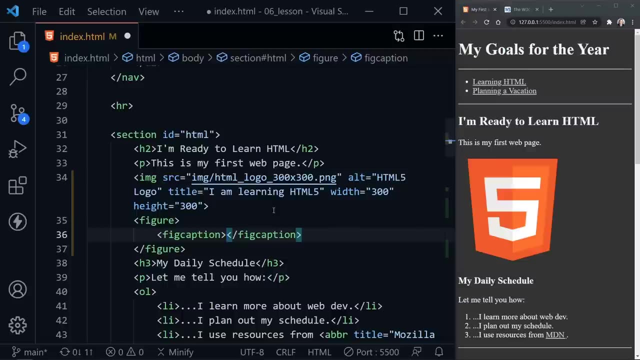 We'll scroll back up to this area here on the page as well, And now we can add a figure underneath this image. So I'll type the word figure again. And now let's add a fig caption. first, The fig caption element needs to either be the first thing inside of a figure or the last thing. 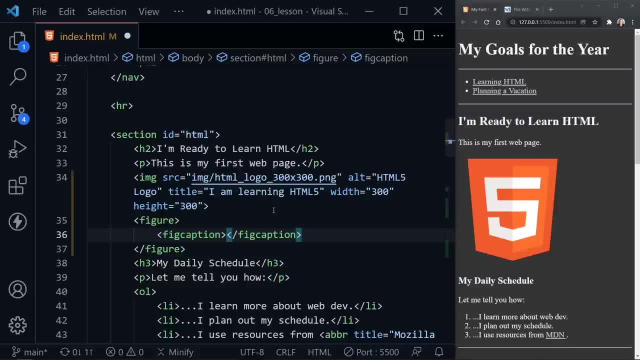 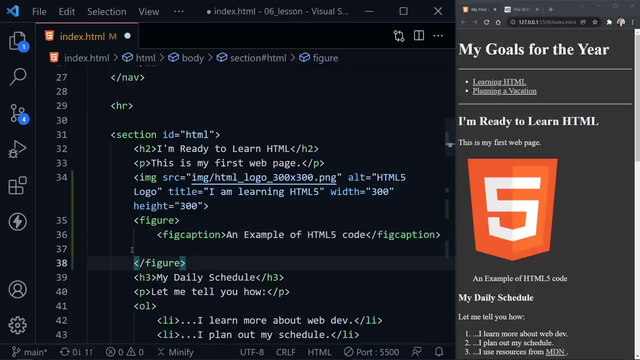 It can be either or. So here I'm going to type an example of HTML5 code And that will be our caption. So let's save that much And we see that here, But really we have no content inside of our figure yet. 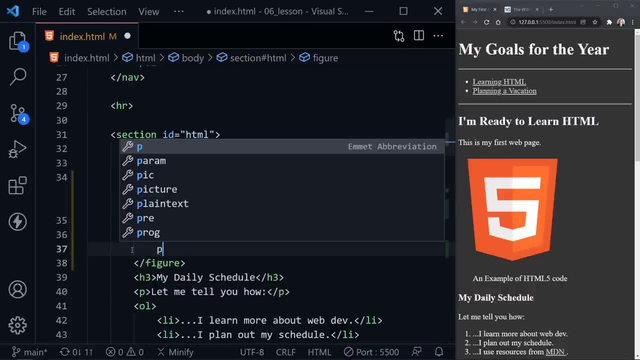 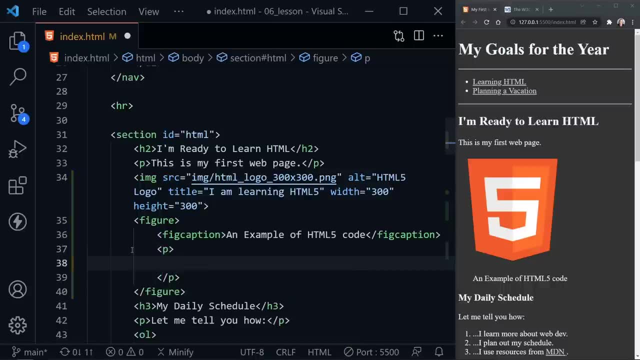 So let's go ahead and add some content And I'll add a paragraph Which is a block level element. We've discussed that in the past- Block versus inline. And now for the text of the paragraph. I want to put that inside of an inline element. 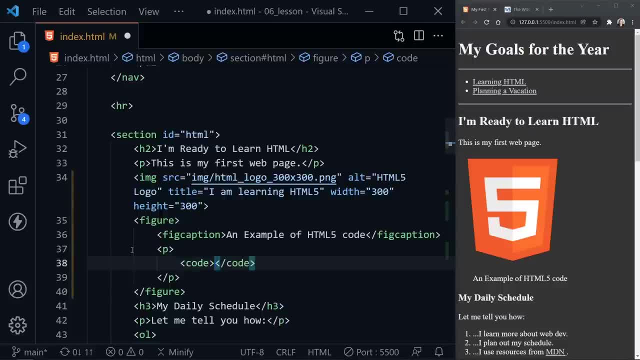 That will not create a line break, And it's a code element Code. this element code helps you actually display code. if that's what you want to use. You can use other elements inside of it though. So if I want to display HTML code, I can't simply put an H1 element. 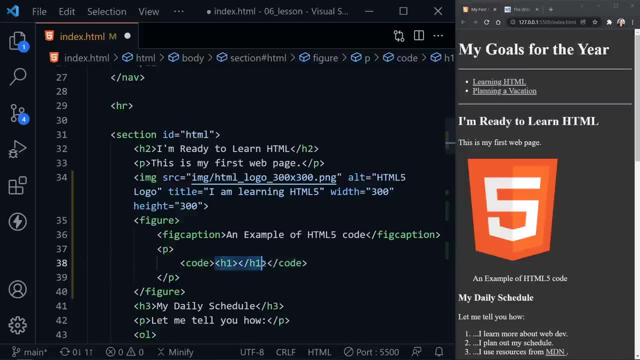 Because then it applies the code And I can't add this element to the page. We need to go back to what we learned about HTML entities to provide the less than sign, Which is ampersand LT, with a semicolon. Then I could type H1.. 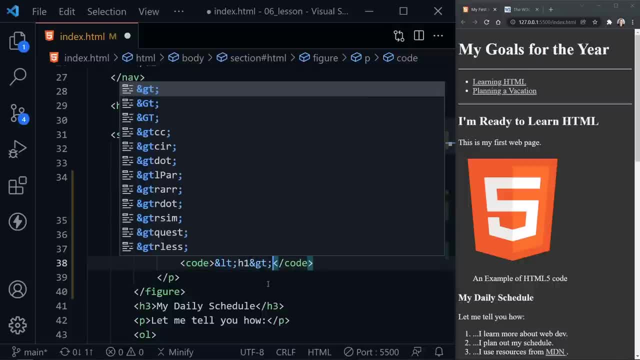 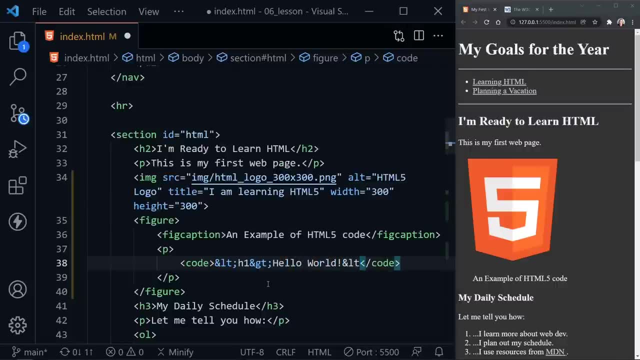 And then ampersand GT with a semicolon For the greater than symbol, And now I'll put hello world With an exclamation mark, And then I'll do the less than HTML entity again, And then a slash, H1.. And then the ampersand GT semicolon. 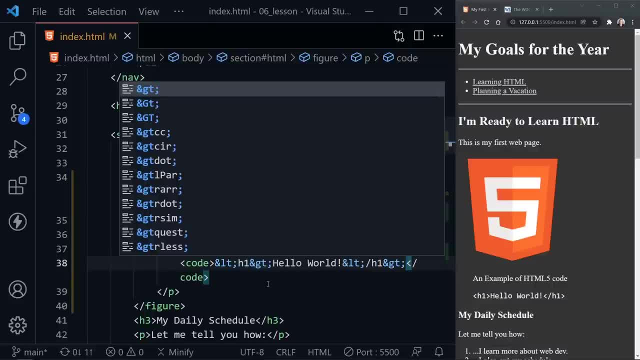 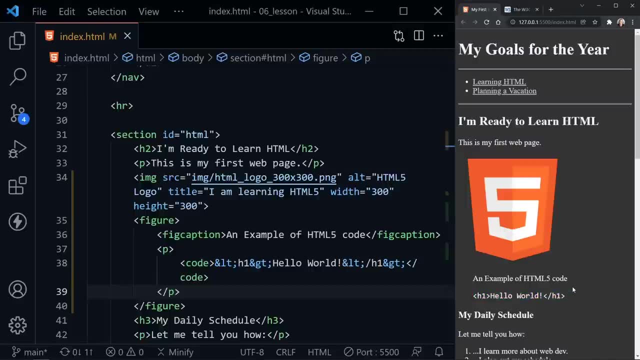 Which is greater than and a semicolon. And now if we look at the page, We have got an example of some HTML code printed directly to our web page. So this is another example of how to use a figure element. It can contain other content, such as a code sample. 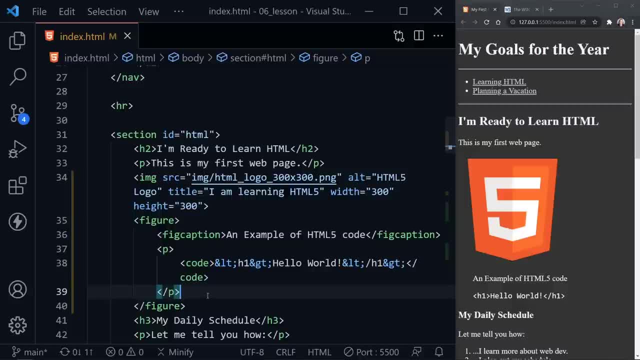 And you can have a caption at the top just as easily as you can at the bottom of the figure. Okay, our code for the lesson is complete, But I do want to show you some image resources. But before we can do that, We need to validate our code with the validator once again. 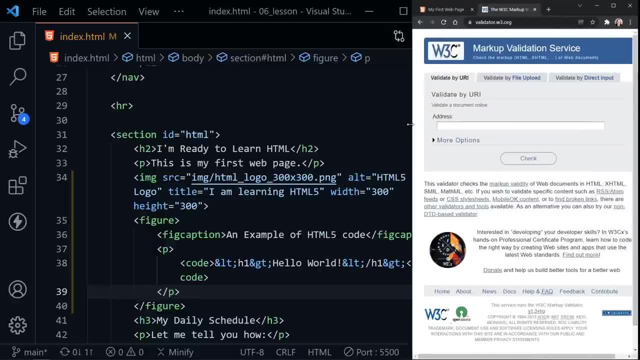 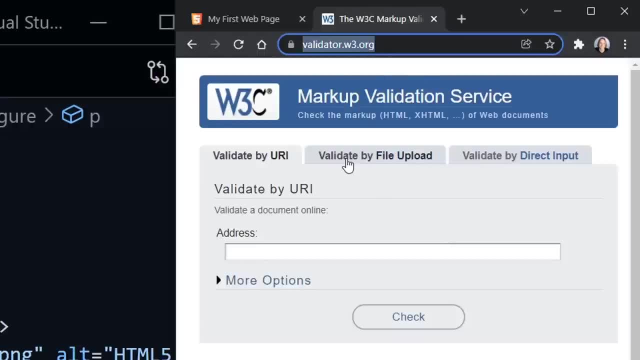 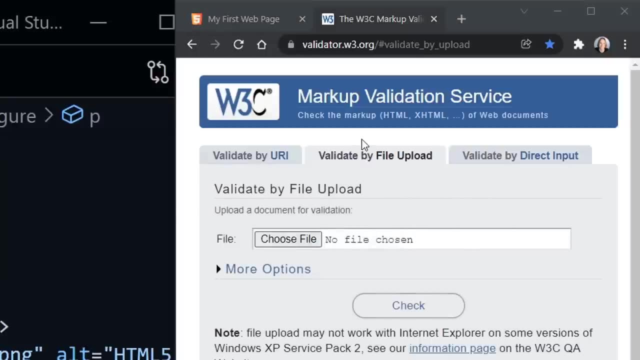 So I'm going to grab this and make it just a little wider So the validator shows up better here. Remember we're at validatorw3.org. We want to click validate by file upload. Click choose file. Make sure you're in the correct folder once this folder area opens up. 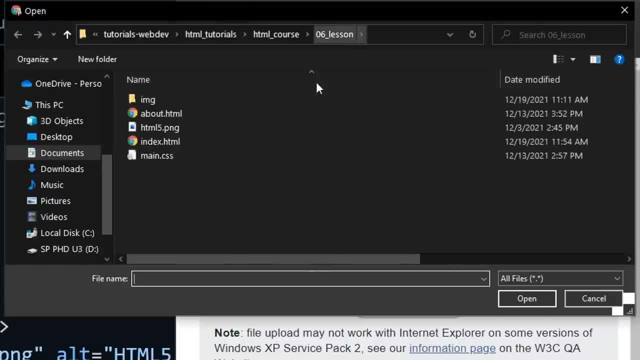 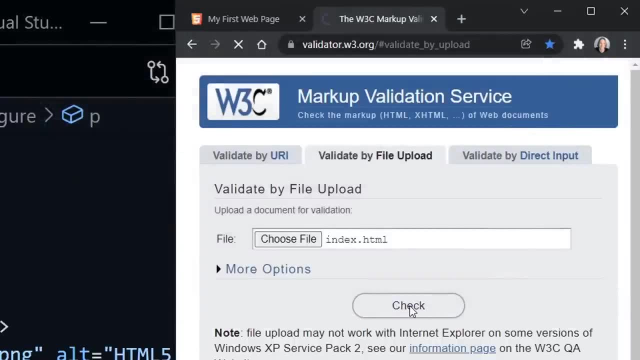 And I'm in the third folder, Lesson 6 folder, And then I'm going to choose the index file that we were working in And choose open And from there I can choose check And it should check the HTML. It says document checking completed. 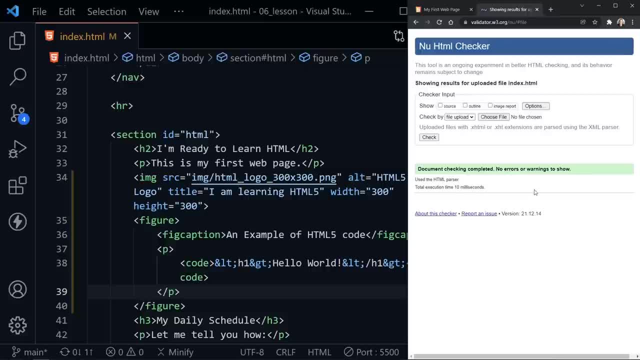 No errors or warnings to show. That's what you want. If you do get an error or warning, It should tell you what line it's on in your code And you can refer to Visual Studio Code, Find the line and fix the error that it is telling you about. 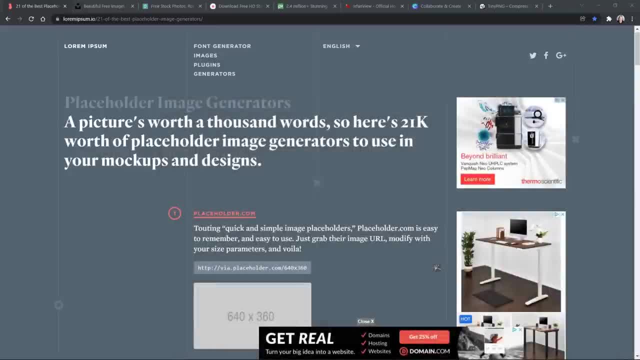 So once again, validate your code before you finish. Before finishing this image lesson, I wanted to share some resources that I use Now. there are many resources out there, So these are just a few, And I'm sure you can find others as well. 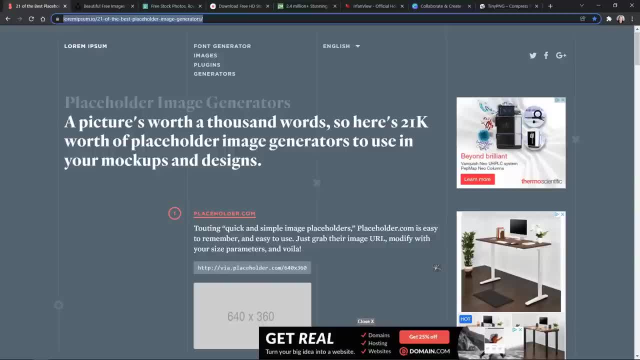 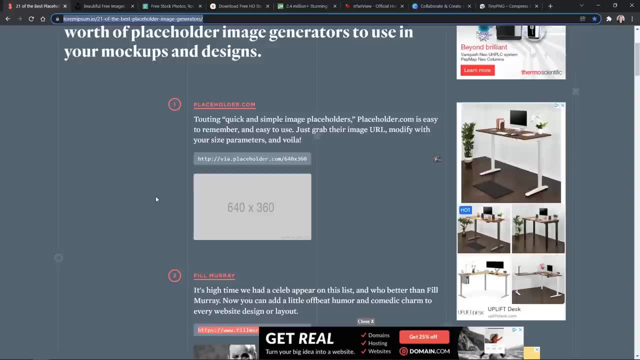 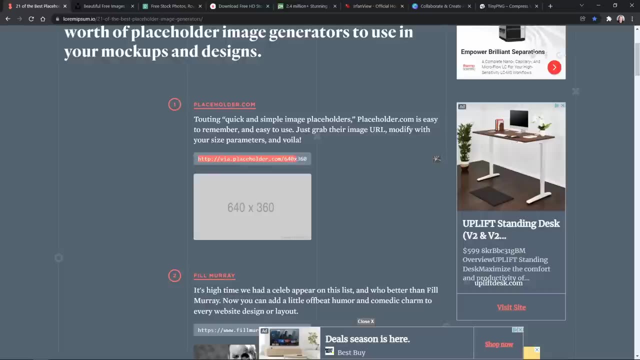 First there's this article that has 21 of the best placeholder image generators. Using placeholder images is very common practice. when you're laying out a page And you're not sure the images you want to use yet, What you can do is take a URL like this from placeholdercom. 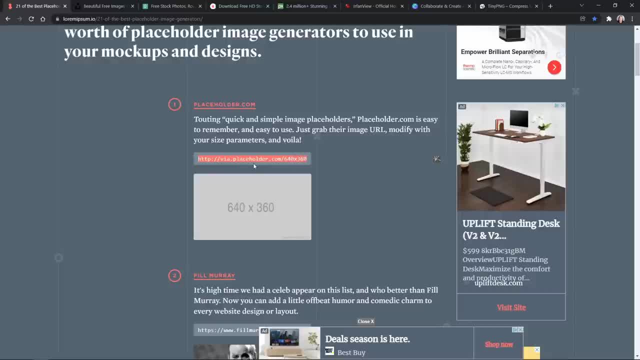 And put it in as the value of the source attribute in your HTML image tag And then it will generate a placeholder image Until you find the image you want to put there. Some of these other image generators actually provide pictures Like the second one on the list called Phil Murray. 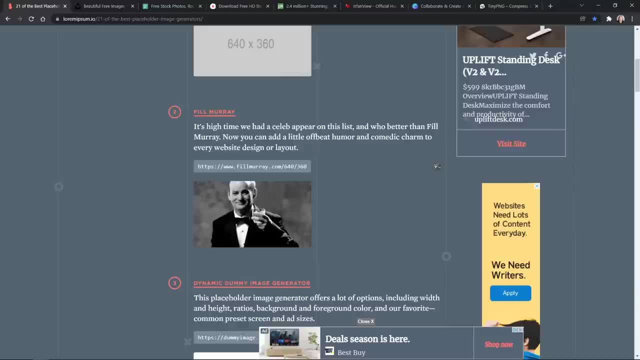 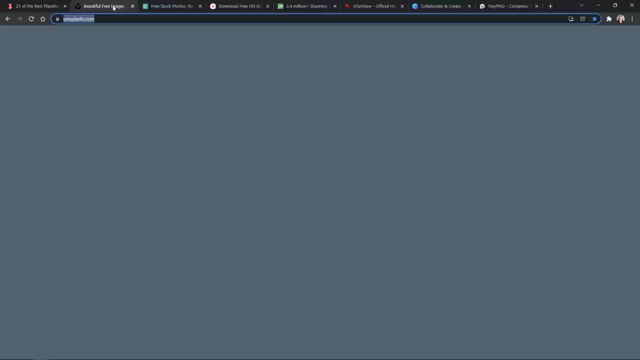 Provides random pictures of the actor Bill Murray, But it works in the same way. You put the URL in for the source attribute value in your image tag And then you will get a picture of it, Of Bill Murray, from this image generator. Okay, the next several sites are just great places to download freely usable images. 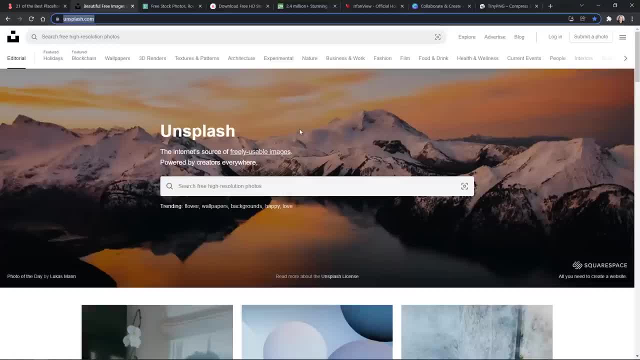 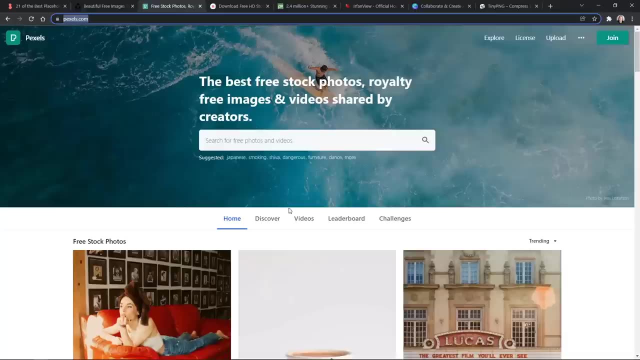 As it says right here, These are licensed for free use. It's important to download and use images that you actually have the usage rights to, So this is a good way to do that. Find them on unsplashcom is my favorite. You can also go to pexelscom, as you see here. 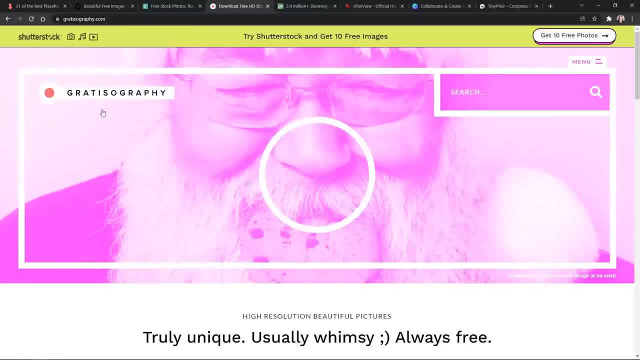 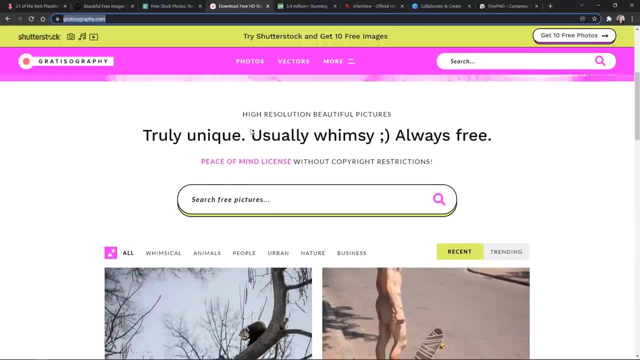 Very similar site. You can also go to gratisographycom, And this site has unique and kind of funny pictures, So that's kind of neat too, And you never know what you'll see on these. The next one is pixabaycom. 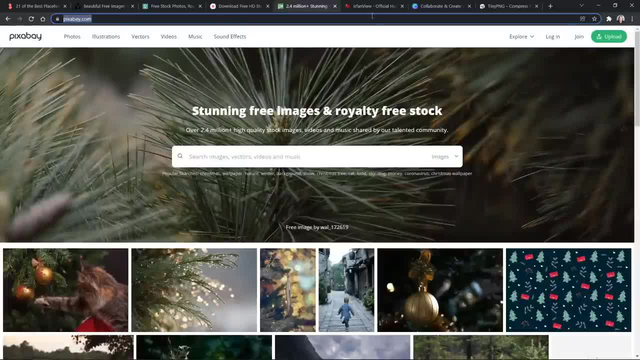 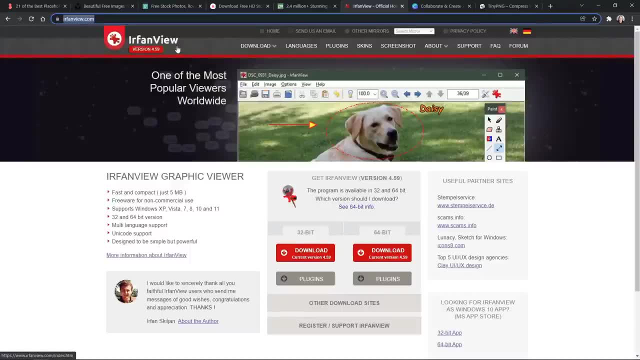 Very much like the previous ones I showed you. From there I want to suggest some free image software. It's called Earthen View. I've used this for years. It's just really lightweight software, Easy to use And you can load in there. 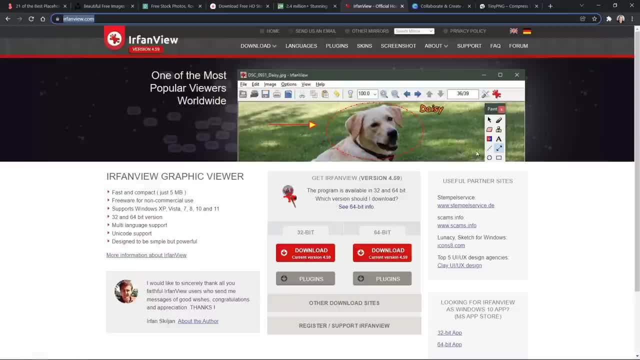 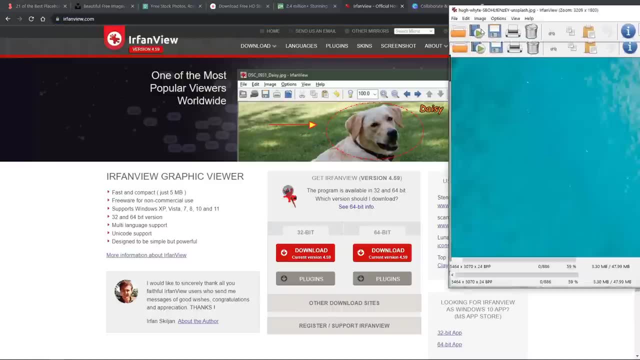 And you can load in an image and resize it, And that's what I usually use it for. You can also crop images with it. I'll pull it over here, as I have an instance of Earthen View open already. You can see I've got in this large picture of the Caribbean beach. 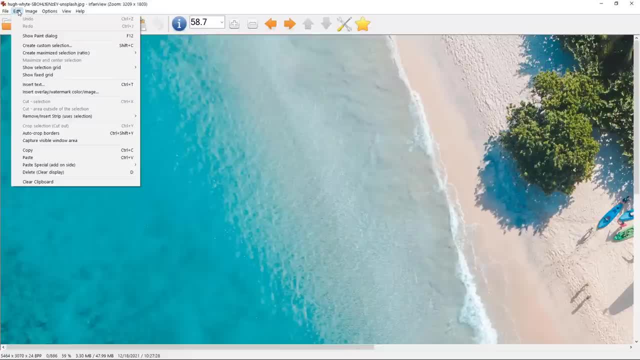 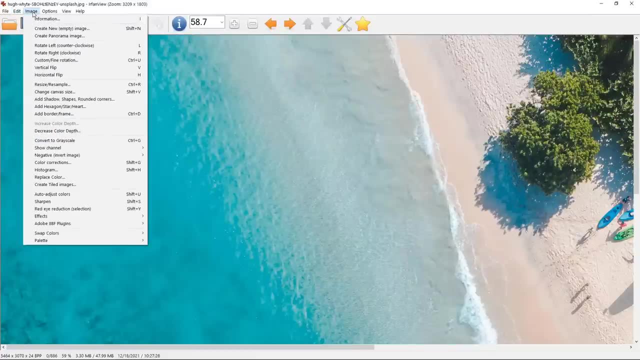 But you can go to the edit menu And you can see different options that are here, Such as the crop, And of course we'd have to select an area to do it. But in the image menu there is a resize resample And here you can see. you've got the dimensions of the image. 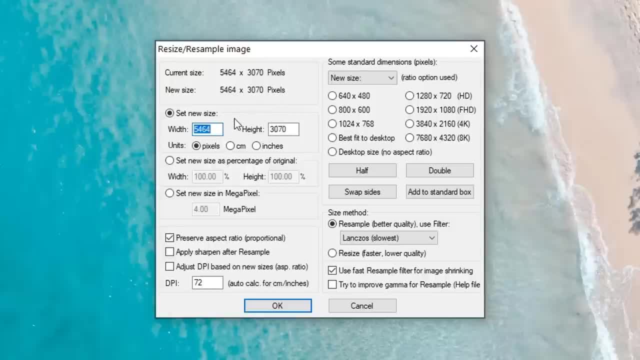 But I can resize this. It's a huge image right now 5,464 pixels wide. I'll take it to say 400 pixels, And it stays in sync So it keeps the aspect ratio And now we're at 225 for the height. 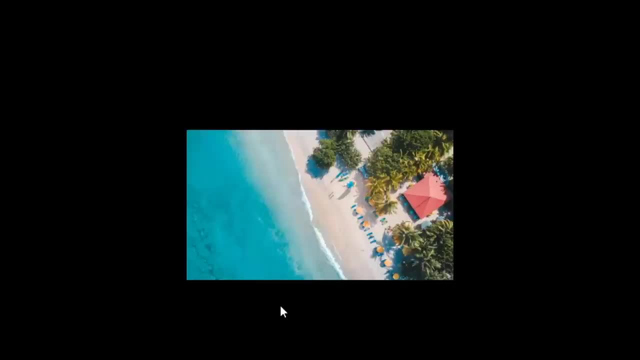 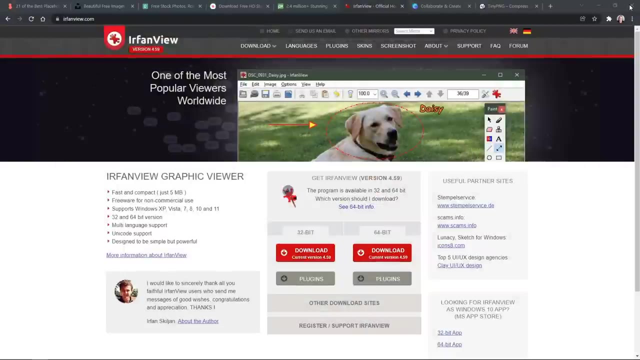 So you see the current size and then the new size. I'll click okay And it brings it down to a much smaller, nicer size, Easy to save, as well as a new size And a great little software to use From there. I also recommend Canvacom. 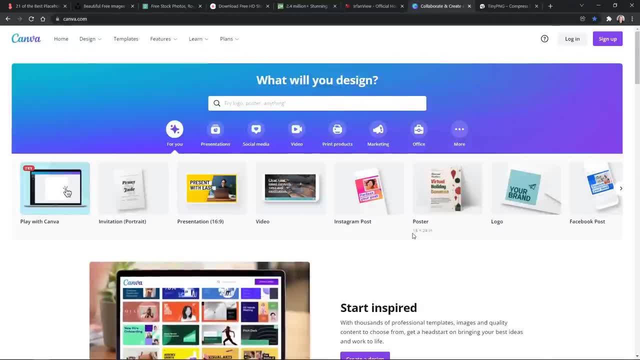 Now disclosure here. there is a paid subscription to use this site. However, I believe they have a free account that you can at least get some of the features Or try it out. So Canvacom is good After you've got your images. 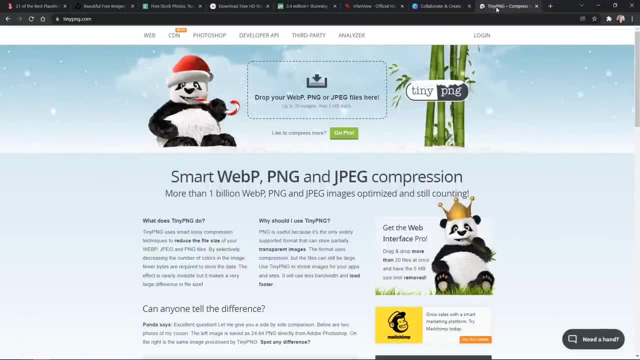 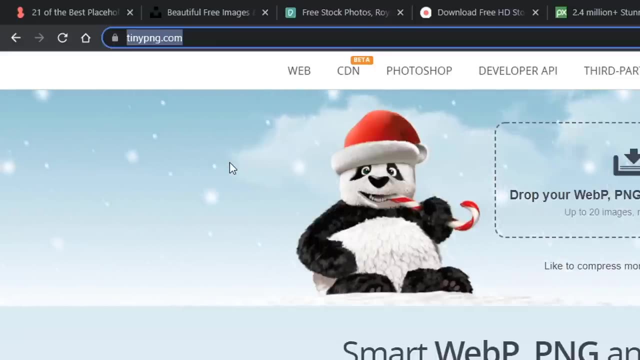 And even after you have resized your images to the smaller size that you would probably use on your site, It's also a good idea to drag and drop them into tinypngcom. I believe this also comes up if you type in tinyjpgcom. 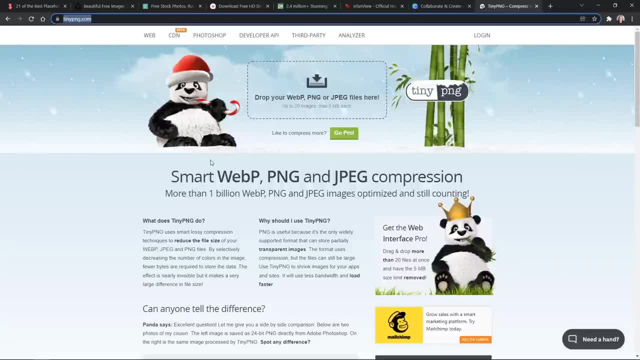 But it will compress the images And they will still look good, But they get a smaller file size So they load to that web page faster, Which is always important. So all of these resources are great And I will put links to all of them in the description below. 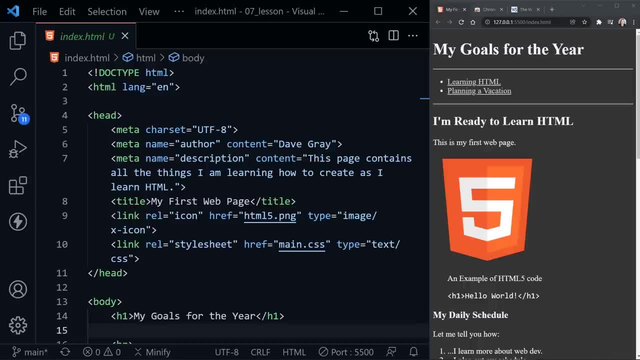 Documents need organization And our HTML files are no different. HTML achieves document organization with semantics. In this lesson we're going to improve our code with the semantic HTML layout. Let's get started. I've got Visual Studio Code here on the left with our indexhtml open. 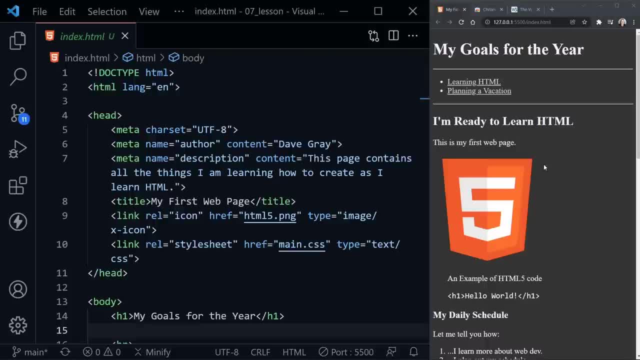 And on the right. I have got our indexhtml page displaying And we're using the live server extension for Visual Studio Code to display that page And you can see it's launched down here. You can click the close or open the server. You can search for that extension over here at the extensions icon if you do not have it. 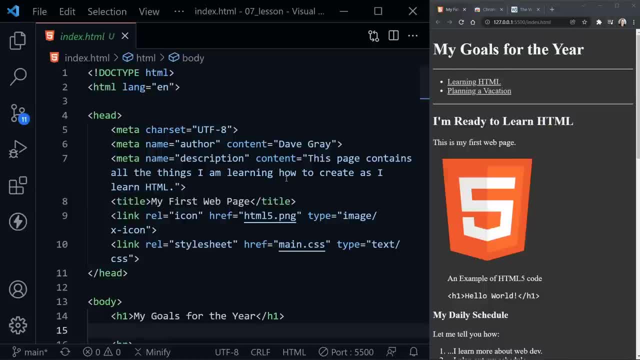 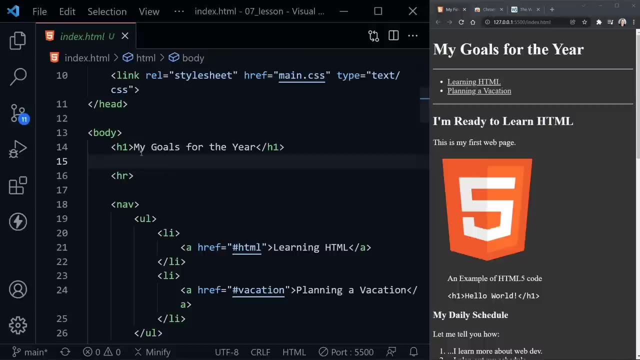 Again, it's the live server extension. Okay, So we're adding semantics to our indexhtml page. Now we've already added some, So let's highlight what we have done already, as we've built this page out over the lessons. The main thing that we have done correctly is add a hierarchy of headers. 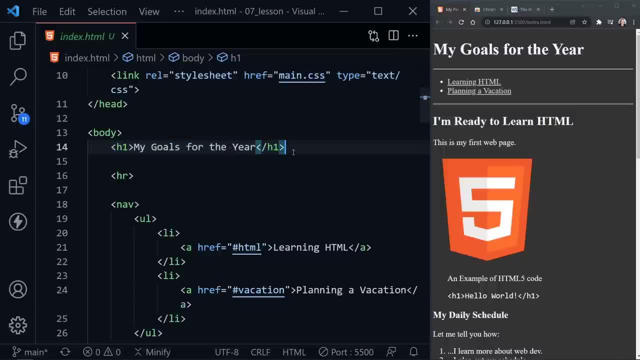 You only want one H1 per page And this should be an outline, much like you would have an outline for an essay or any type of paper topic you would write. So this is your title for the whole page, essentially, And from there you can have multiple H2 headers, which is one level down in the hierarchy. 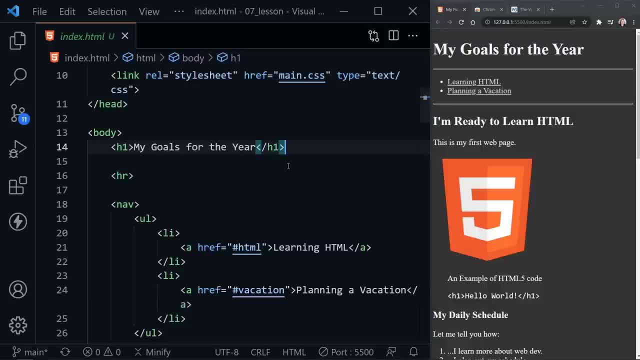 And they would define subtopics And then beneath that you could have H3 headers if there was a subtopic of a subtopic, And so on, And that continues to H6, although you really don't want any more than about three levels of headings on a page. 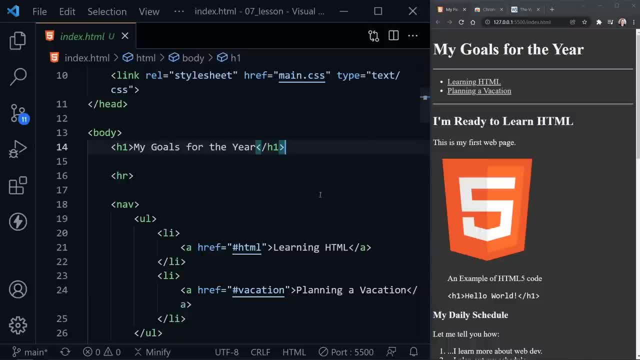 So H1, H2, H3 would be the ideal way to have a page laid out. After that, we need to consider some things about semantic HTML Writing. semantic HTML helps us quickly see or read the different sections in a web page and navigate to those sections. 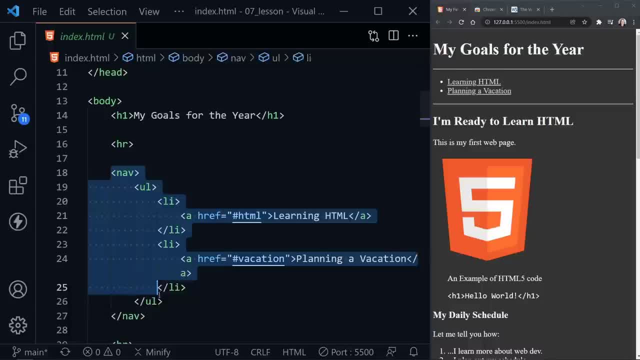 Now we've already added a nav element to our page, Okay, And nav elements are semantic elements. So this says we have a grouping of links here And we can see that on the page with learning HTML and planning a vacation. We have a grouping of links here that will help us navigate to the rest of the page. 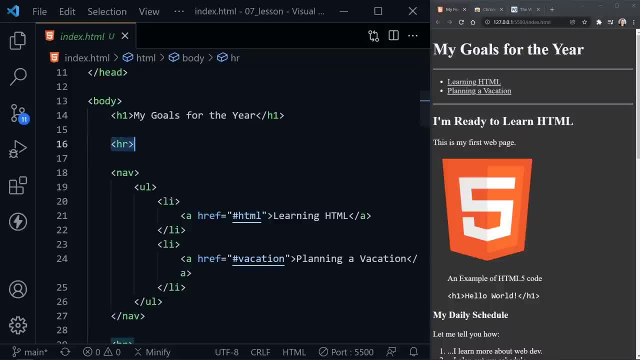 We also have an HR, which stands for horizontal rule. In the past, I believe I might have said these didn't really have a semantic meaning, But they do. They're currently viewed as semantic elements And it means that there is a topic there. 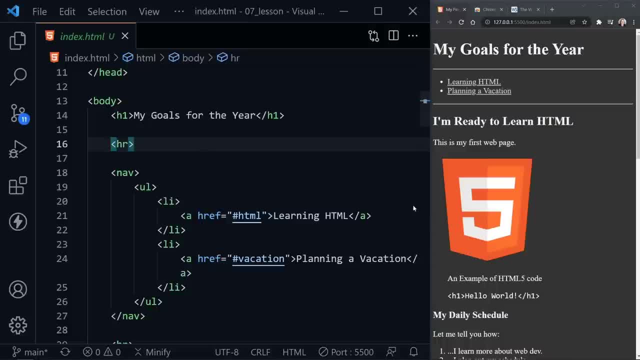 There is a topic change, So something is changing And of course we have a couple of topics on our page And we have horizontal rules between those. In the future, as we learn CSS, we may want to remove the horizontal rules we see here that divide our navigation and our heading for the page. 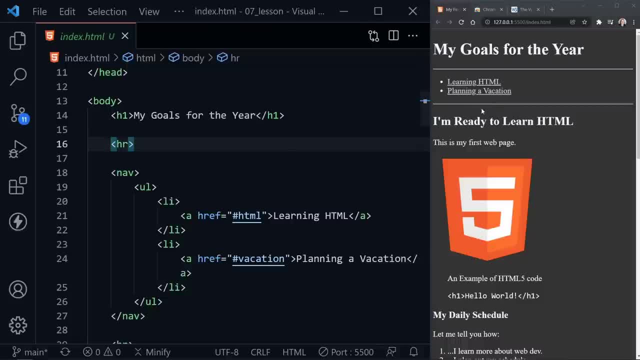 And replace those with lines that we can create with CSS, Because we're not really separating topics here, Although it doesn't hurt to have these horizontal rules in place at this time, And the main thing to convey about semantic HTML is the word semantic. 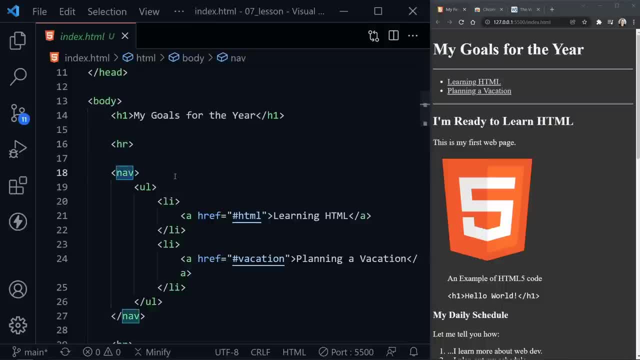 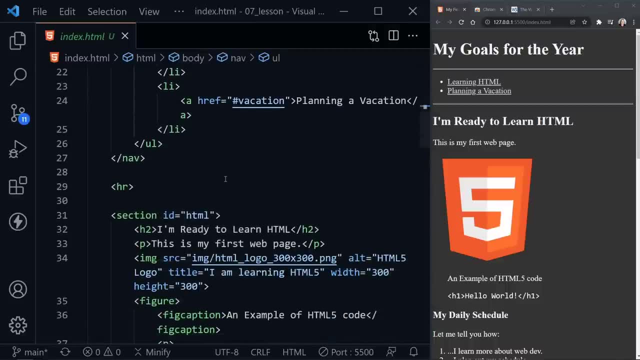 That means it provides meaning, as the nav element says, hey, this is a navigation area. Or the h1 element says, hey, this is a heading. We can also get that from other parts of the page. We added section elements that say this is a new section. 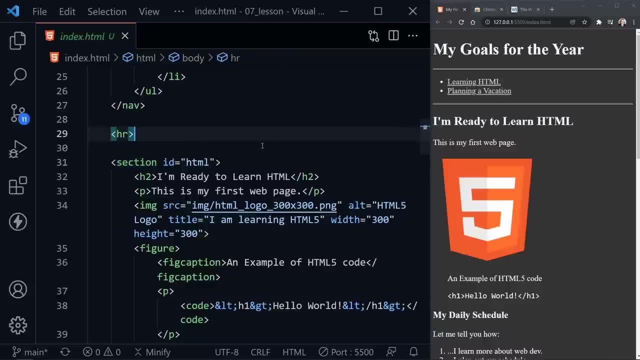 So they provide additional meaning rather than just a generic divider, And we will talk about what a generic divider is later Now. in addition, semantic HTML makes our pages accessible to screen readers and other assistive technology, And that is very important as we create pages. 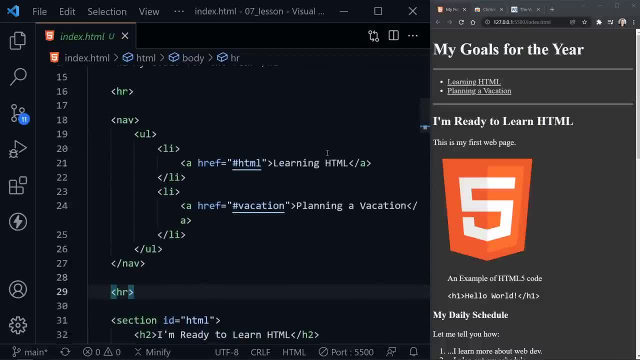 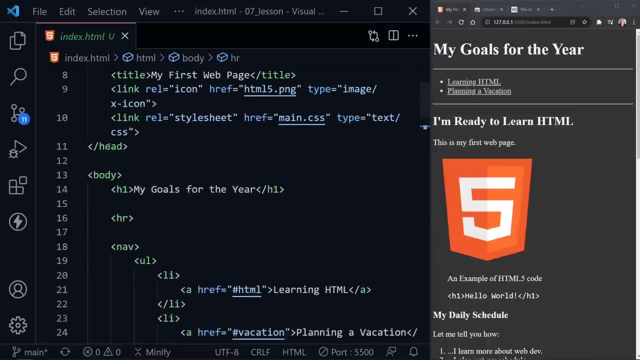 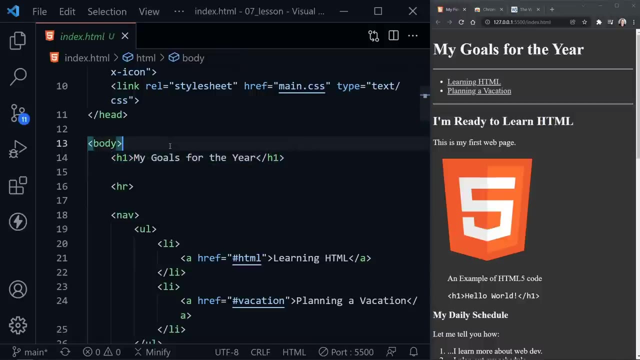 Now, while we've added some semantic HTML already, Let's add the three big areas that most consider for pages. The first is not a head section, but a header for our page. Now we have a heading which is the title of the page, But we can wrap this in a header element. 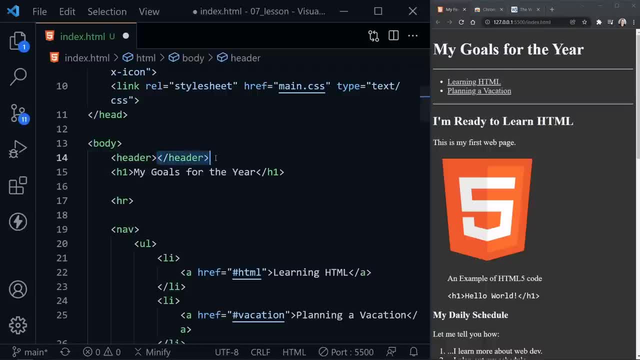 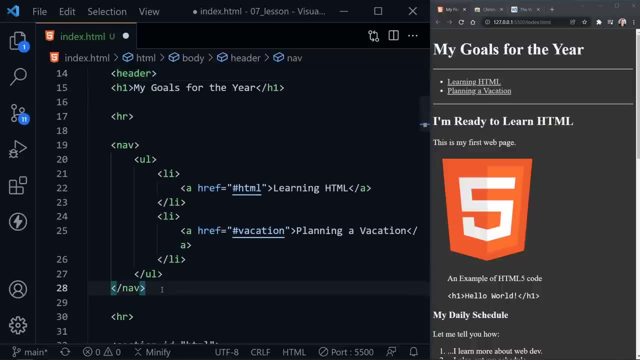 And there can be more than one header element per page. However, it needs to follow the heading hierarchy. So imagine if we had a social media site. Now every post, whether it would be a blog post or a post like Facebook or Instagram- Every post could have its own header. 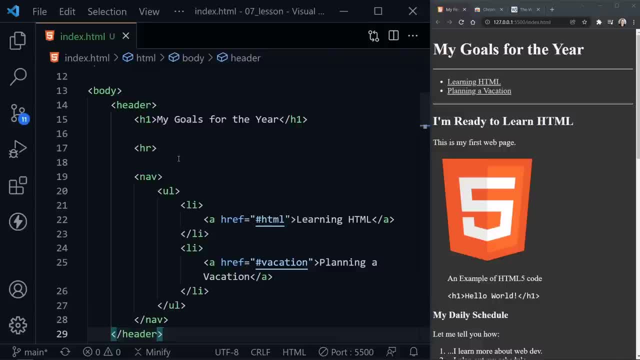 And it might have a subtitle in that post as well. But this is a header now for our full page, So this would be at the top, At the top level of our page, with the hierarchy here of H1., Which is the heading for our page. 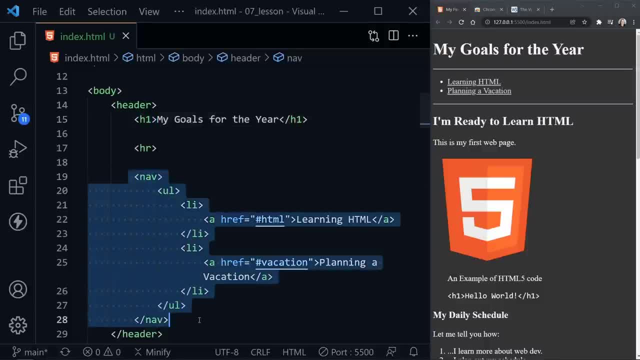 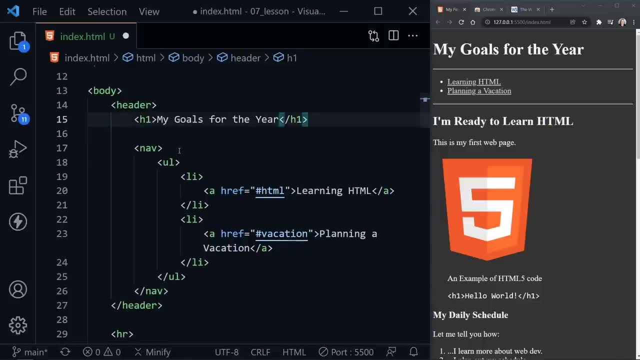 Notice. we've also included the navigation inside of our header And we can go ahead and remove this horizontal rule, And I think it will be just fine. We don't need the semantic meaning of a change topic there, And I think it's going to look okay without the line as well. 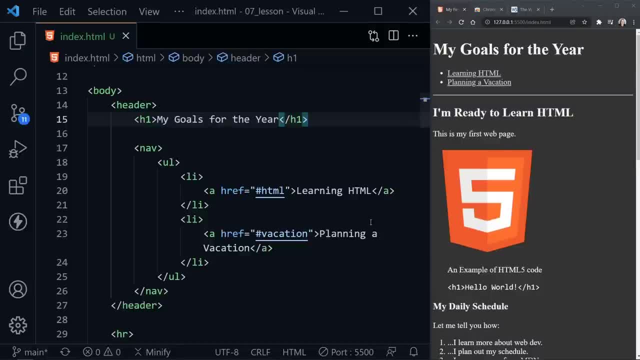 So let's save this now And we can see live server updates our page immediately. So we can see the change And really All we see visually is that our horizontal rule is removed. However, we have added some extra meaning to our HTML here now. 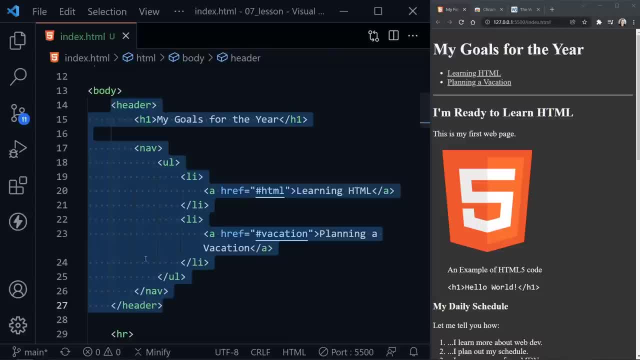 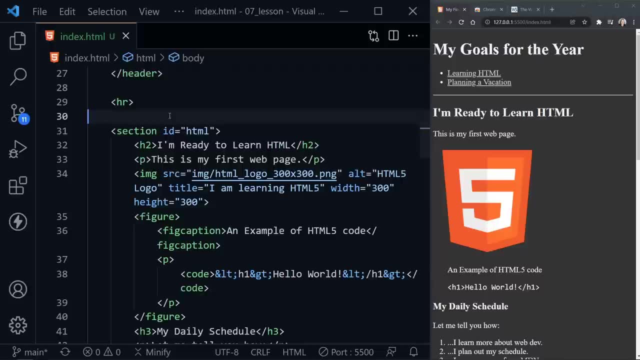 That this is the heading or the header section for our full page. Now the next element we want to add is the main element. Now there can only be one main element per page And by definition that would make sense. You can only have one main area for content per page. 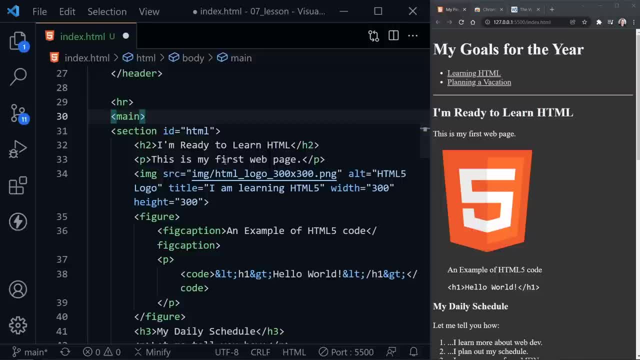 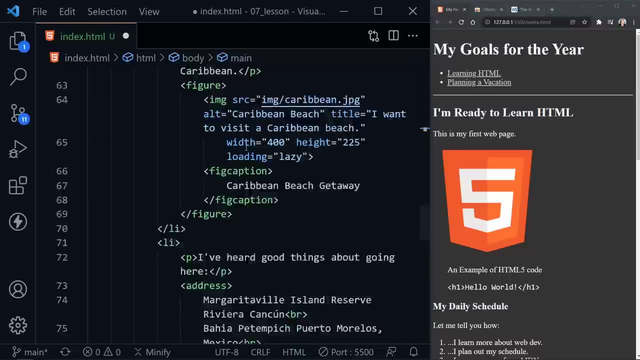 And so we'll start here, And it's going to include our sections that we've created. So I used control X to cut the closing main element tag And I'll scroll down to where our second section ends Before our area here at the end. 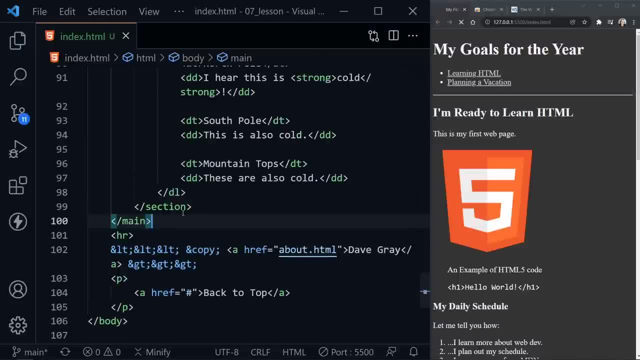 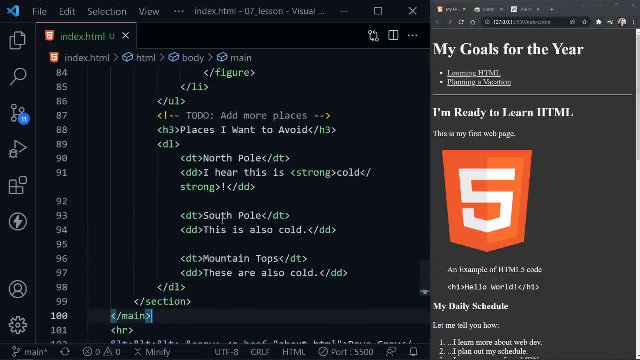 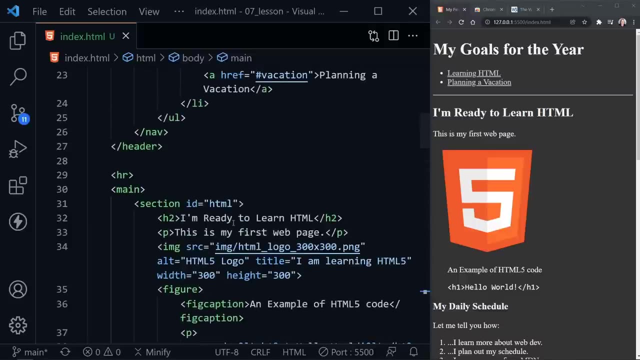 And I'll paste the closing main element And save And we can see Visual Studio Code reformatted for us. So now we've got the main element wrapping our two topic areas Of vacation and of HTML. So we've added a header and a main element. 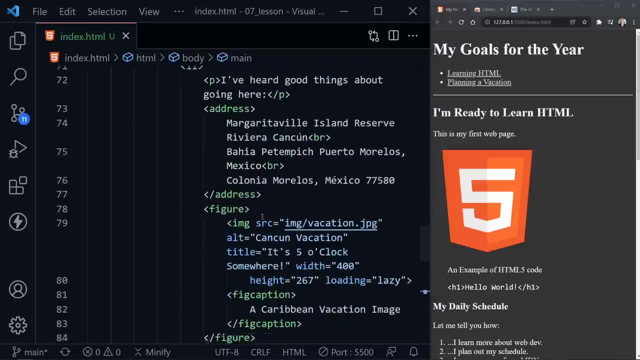 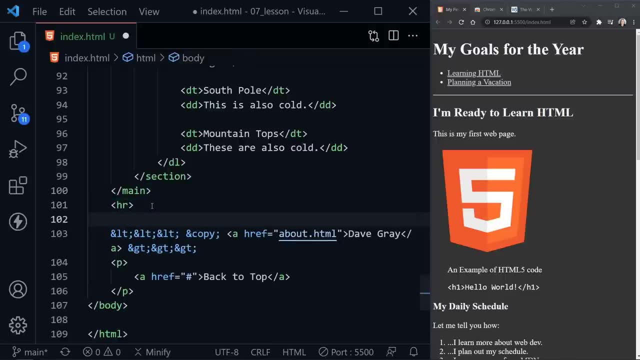 Now, one other thing we can add for our page is a footer. Now, just like the header. There can be more than one footer per page, And that might be a footer for a blog post Or a footer for a social media post, But this is the footer for our entire page. in this example, 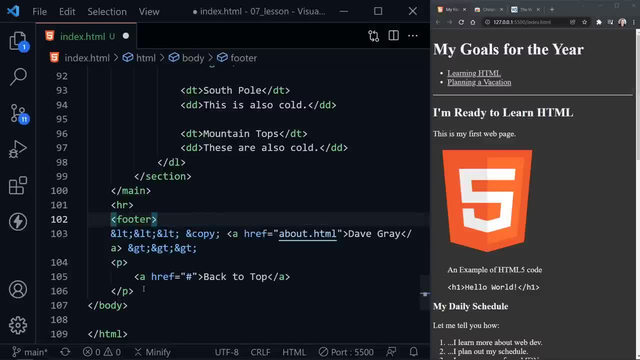 Once again control X to cut that closing tag And I'm going to wrap everything we have here at the end in the footer. One other thing I want to add, just because I didn't do it before. We've validated our page throughout the other lessons. 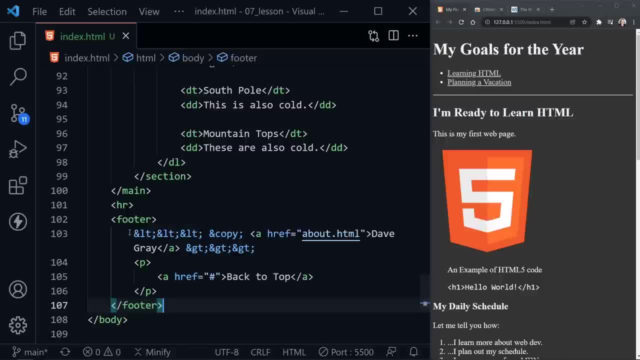 And it's not an error, It's not a problem, But I want to include this information here about the copyright. I want to include that in a paragraph element, So I'm going to make sure that's lower case. Why am I getting a capital? 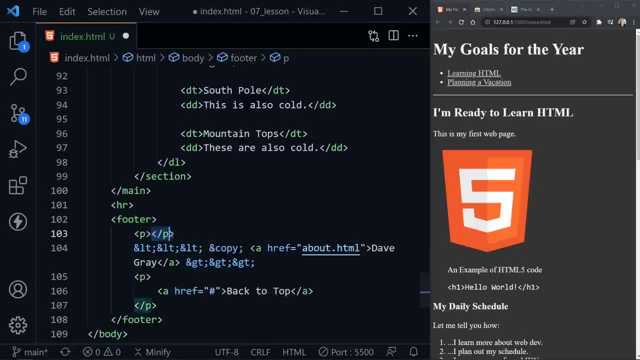 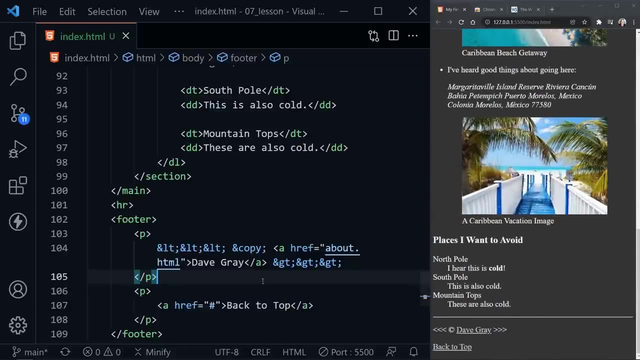 There we go, And then I'm going to once again cut the closing tag And put it after the content And save. It gets reformatted. It really doesn't change the look. I just wanted both inside that paragraph And that might help in the future when we want to format this area as well with CSS. 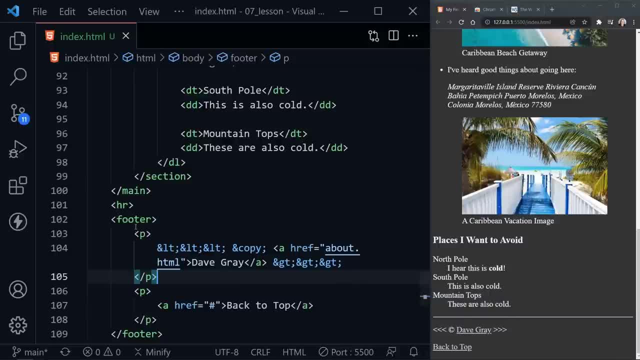 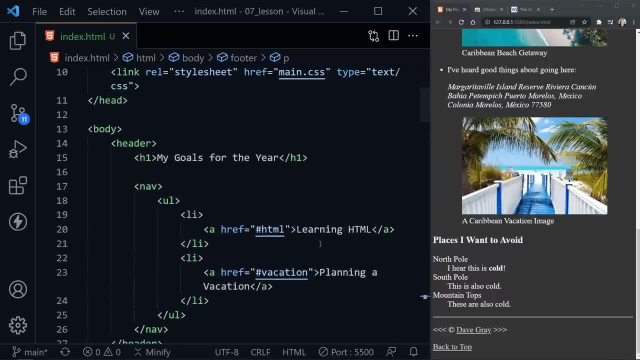 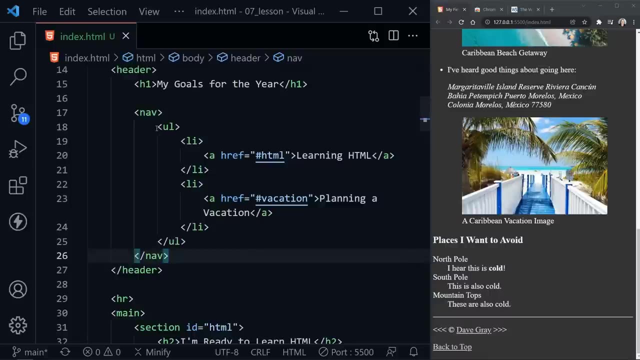 So now our document has been outlined into three major sections. We have a footer, A main area And a header, And then inside the header- we've already discussed- we have a navigation element. That is also there. Semantic HTML: Our list is also semantic HTML. 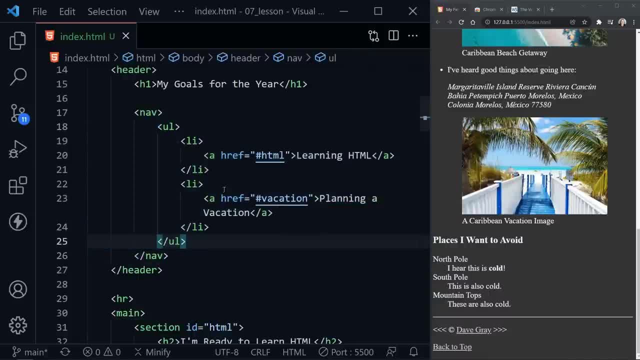 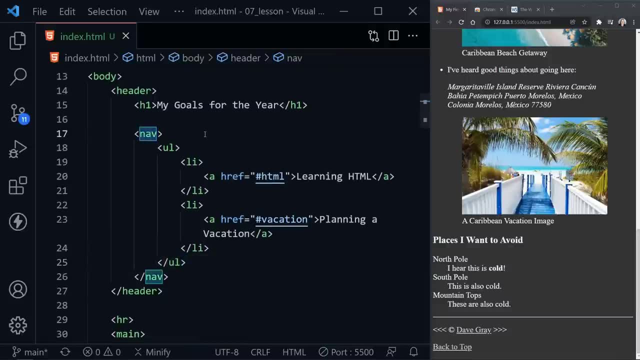 We know right away that this is providing a list, And this would be identified by assistive technology as well. Now there can be more than one nav element per page, So we might have a nav area in the footer. Footers often have links to other areas of a website. 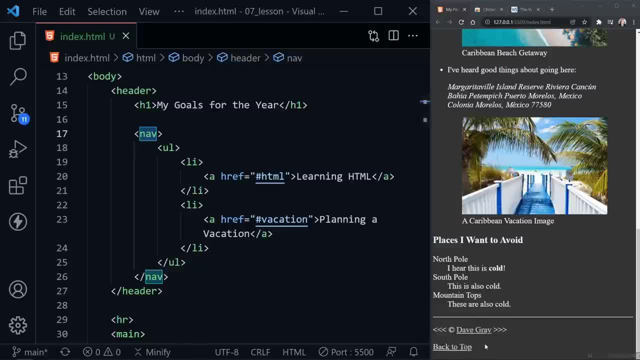 Now we've only got a couple of links in our footer, And one goes back to the top And the other does go to our about page. However, It's not a grouping of links where we would organize. If we had several other things here, I might consider a nav. 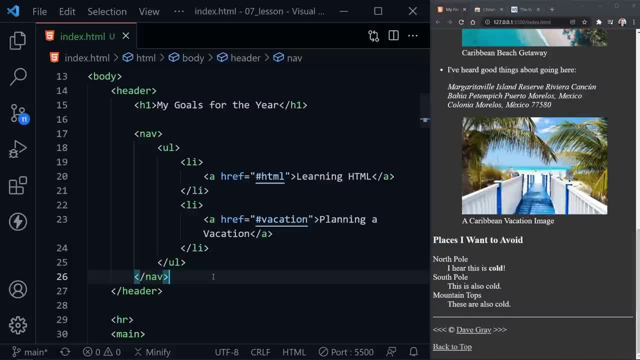 And if you do have more than one nav element per page, It's important that they are labeled, So assistive technology knows which nav is which, And here we can do that with an attribute called aria-label, And then we can set it equal to something that clearly says what it is. 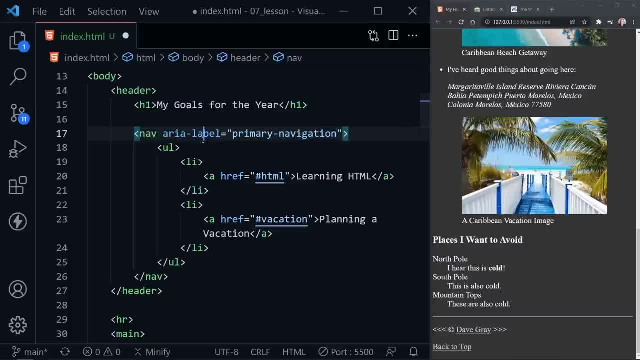 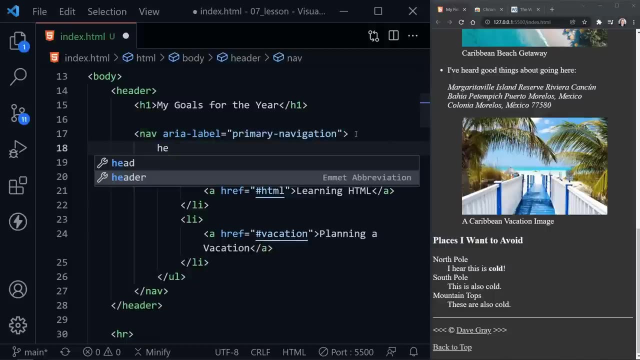 Like primary navigation And now we have labeled our nav as the primary navigation area. If you did include a heading in the nav element, Which is not required, But if you did, You could link to that So you could have an H2 here. 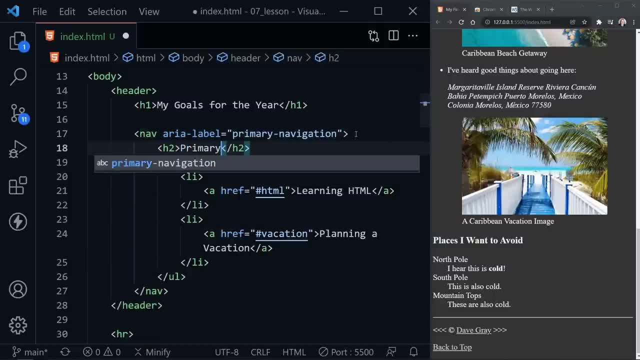 And then in the H2 we might put primary navigation, If I can spell it. There we go, And now let's give this an ID, And here we'll give the address, And here we'll give the ID, the same value: Primary navigation. 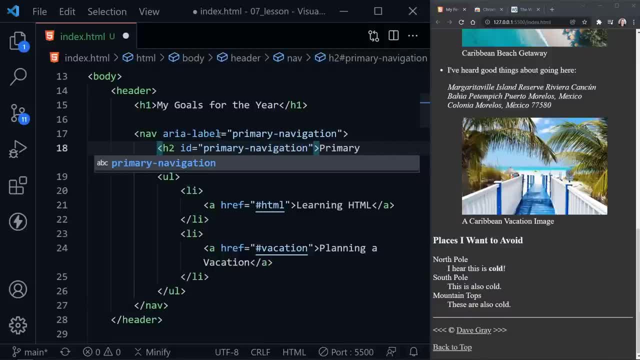 And then here, instead of aria, We would say aria labeled by is the correct attribute here. Now we're looking at our primary navigation value And it's saying, hey, it's labeled by this value that's in the H2.. So you can link these together with an aria labeled by. 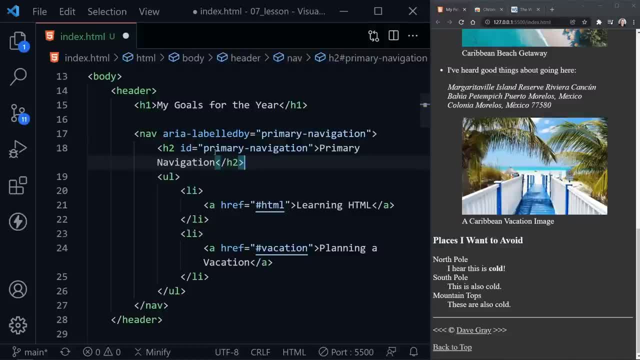 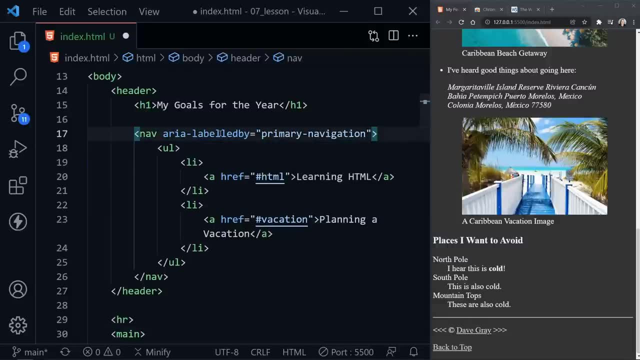 Pointing back to the ID of a heading. However, since we're not going to have an H2 in our nav, I'll go ahead and remove that And you can just choose the aria label attribute And set that equal to primary navigation. 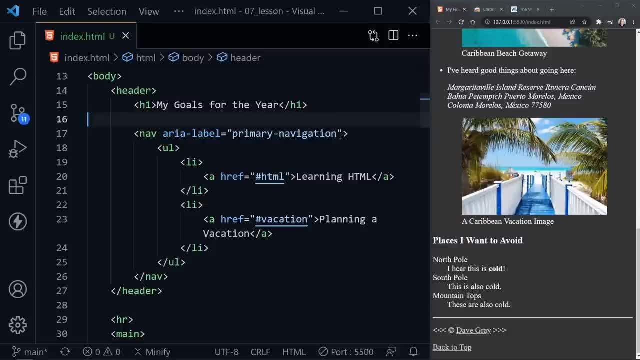 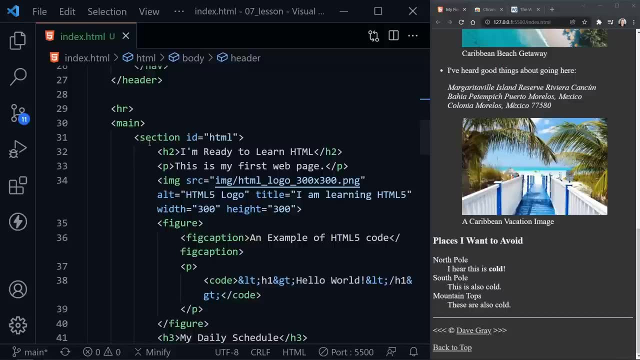 Which is equally accessible to screen readers and other technologies. Okay, let's scroll down into this main area. Previously, we broke our topics HTML and vacation Into sections, Which are semantic HTML tags. However, there is a more appropriate tag Now that we kind of have an idea of how our page is laid out. 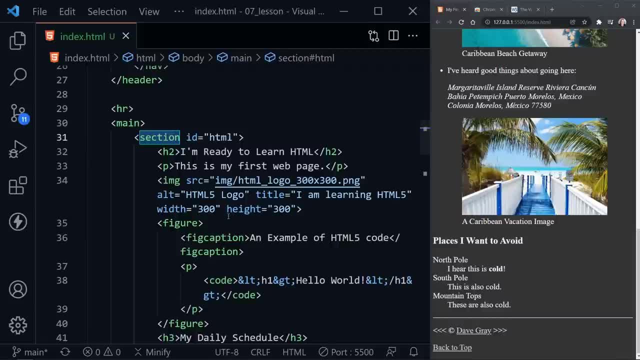 Because these are areas that could be on their own. Maybe they would each have their own page, But much like a social media post Or a blog post, Some type of article, you might think There is an article element, So I have highlighted this section. 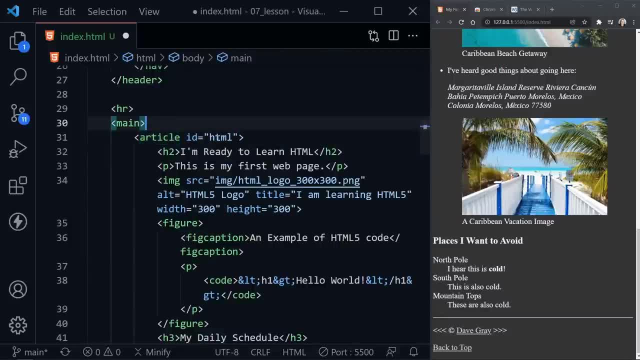 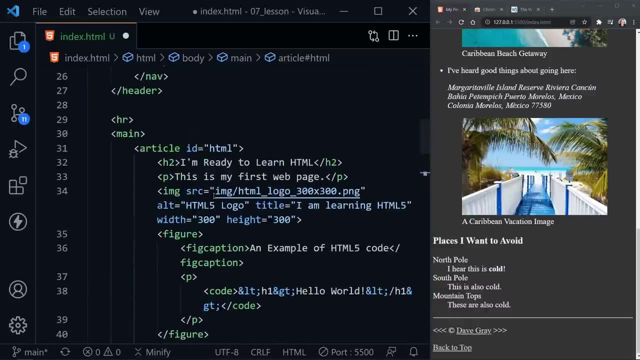 And I'm going to type article in here Instead, and I believe we'll find That VS code changes our closing tag immediately. Yes, and it was already changed to article. So instead of a section, Let's call this an article, Because it clearly has its own topic. 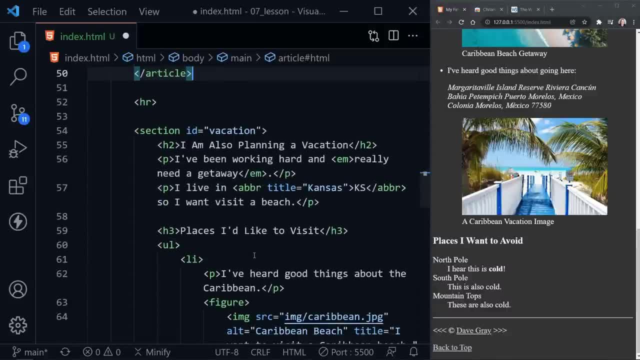 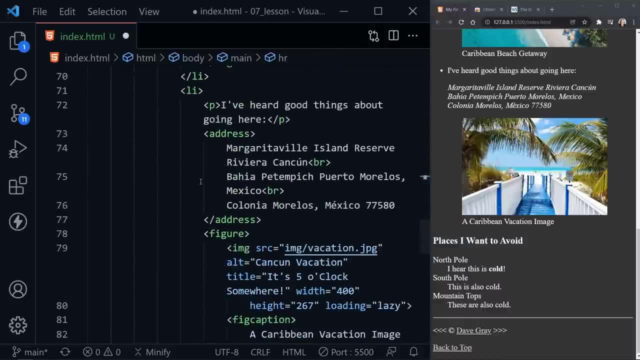 And now let's do the same for our other section, Based on vacation. So we can highlight it, Change it to article And we'll verify that the closing tag is also article. And yes, it is right here. So now we have two articles instead. 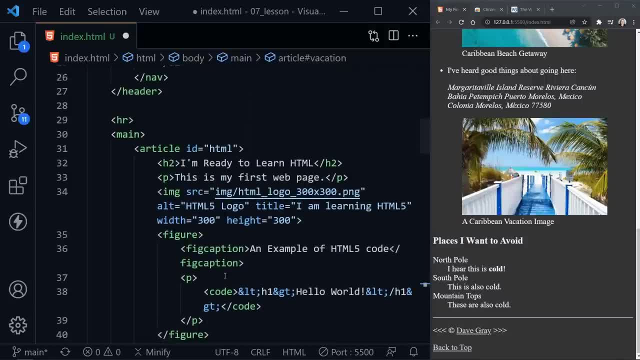 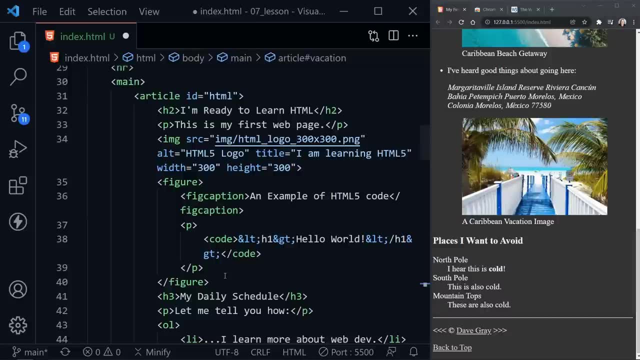 Of sections. Now there is sometimes a debate About which should be used And it's really not clearly defined. If article or section is the proper choice, They would both pass a validator check. So really, the way I look at it Is an article has a clear topic. 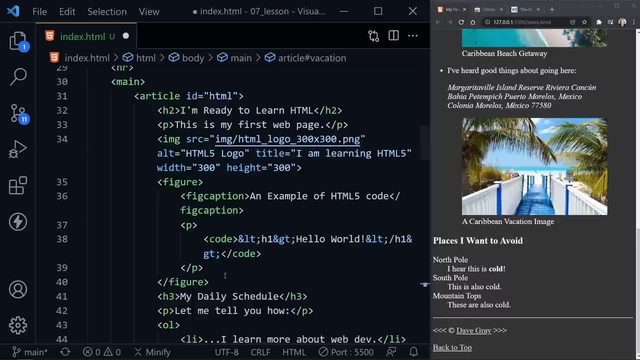 Where a section is more generic. You might use a section Just to actually create a little section In your code, Whereas an article has a clear topic That the area is about. So now, inside of the article, We could create other articles. 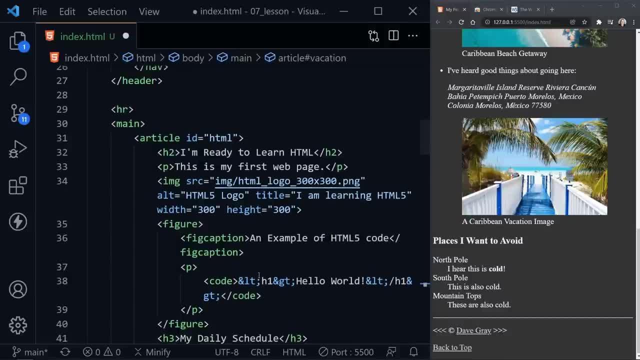 But now I want to go ahead And add a couple of sections Inside of our HTML article. So as our article begins, We've got the heading Which is H2. And it says: I'm ready to learn HTML. And then we have a paragraph saying: 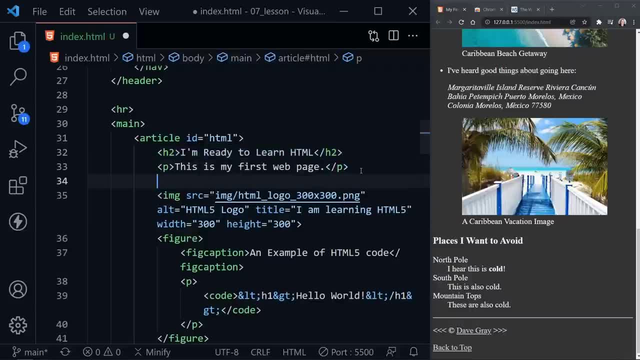 This is my first web page. That's fine. Let's go ahead and add the section After that point. And now, once again, I'll press tab To get both the opening and closing tags. I'm going to highlight the closing tag. 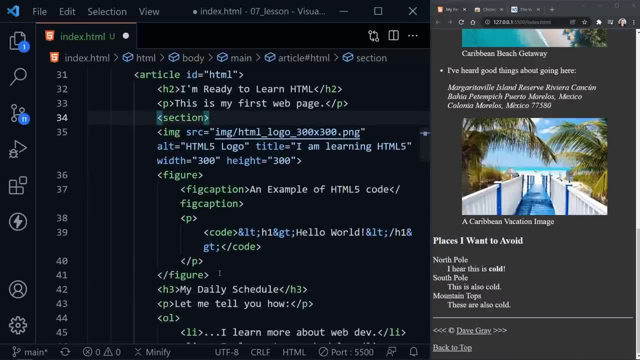 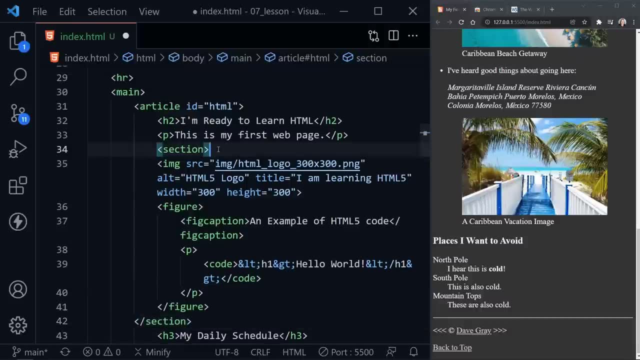 Control X to copy it, And I'm going to bring it down here To just underneath the figure. And that's where we'll end this first section. I also want to go ahead And add a subheading here, Which is an H3.. 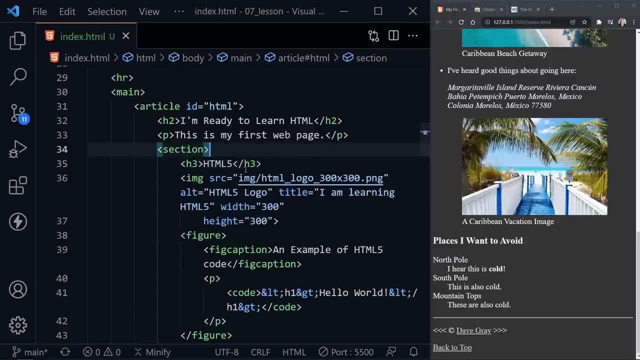 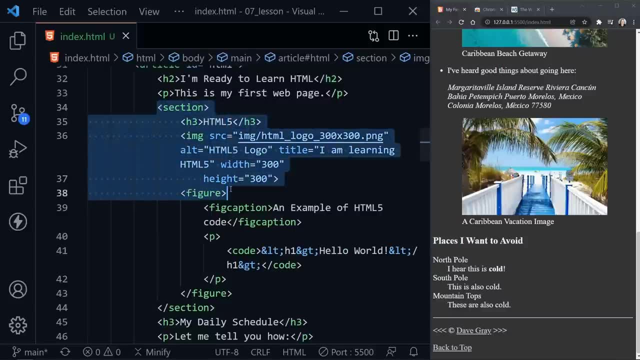 And I'll just make this HTML5. As that's what the section is about. And now our section Has the subheading HTML5.. It has the HTML5 logo And it has our figure. That has our code sample of HTML5.. 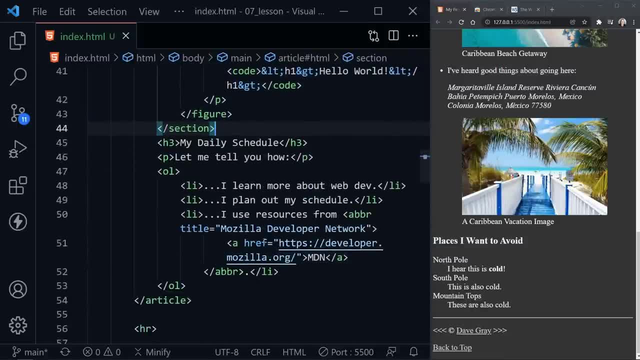 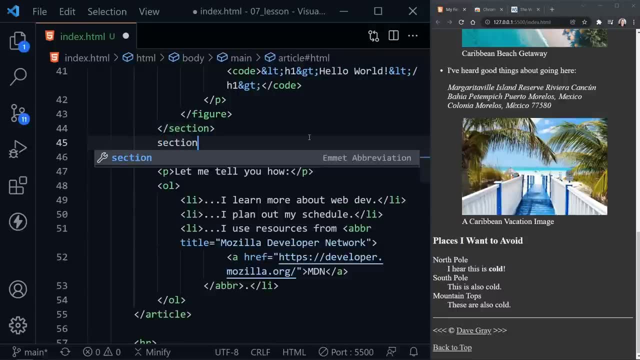 That all seems related. Now let's add another section, And this is the my daily schedule section. So Lower case again, That's what I prefer, And so we'll have section And the closing section tag. I will cut that. 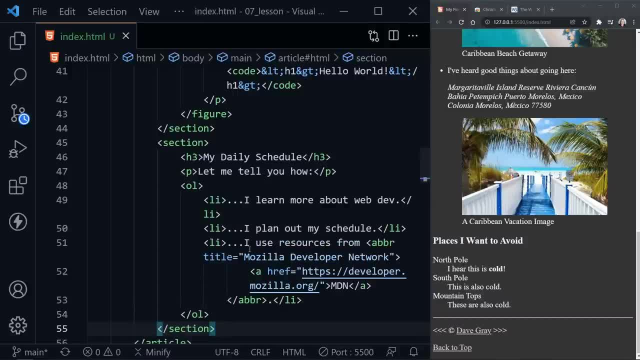 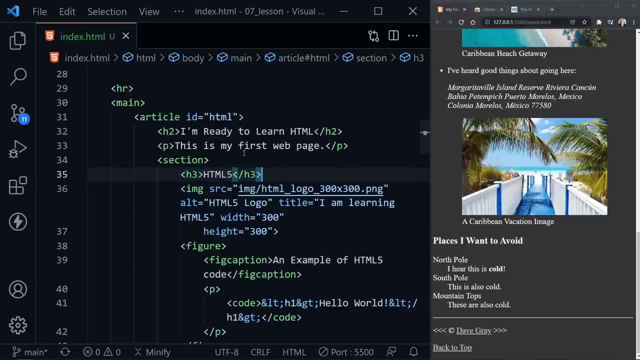 And I'll put it here at the end of the list, Before the closing article tag. So now we have two clear sections Inside of our article And they both have headings That are H3. The H1. Being the heading for the overall page. 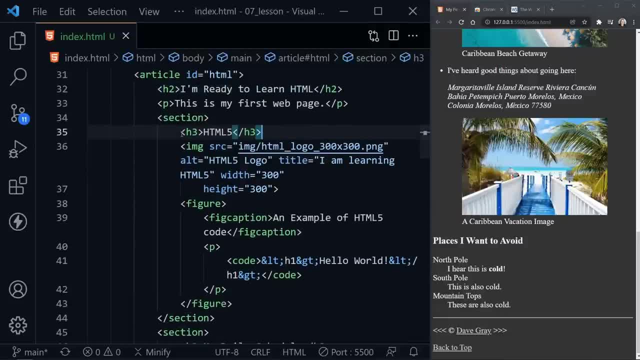 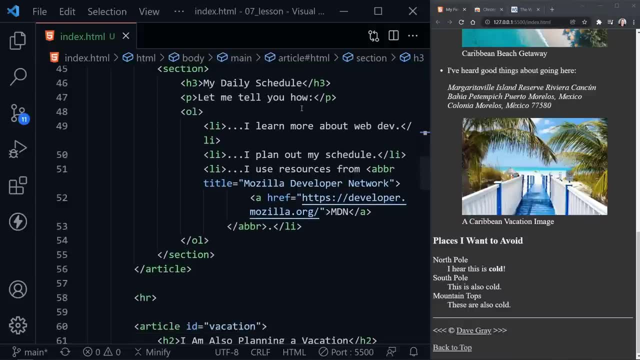 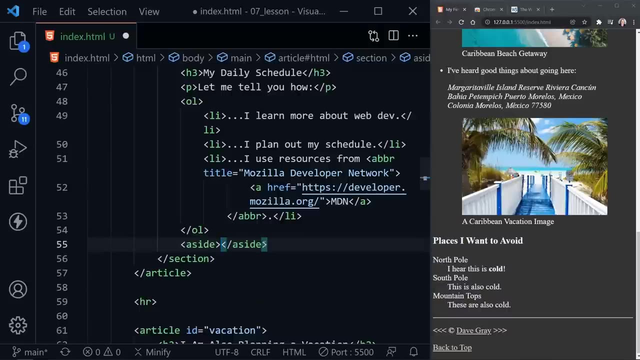 The H2. Being the heading for the article, And then the H3s Being the headings for the nested sections Within the article. So we're keeping our hierarchy in place. Underneath the list, We can add another element And just a little more content. 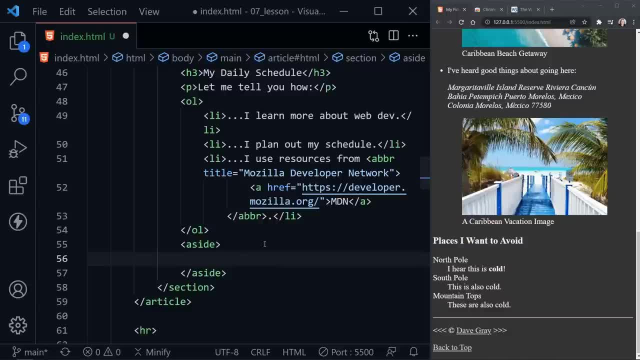 Let's call this an aside. This is a semantic element And if you think about how a web page is laid out, It's not just a bar to the page, But it could also just be another section Of complementary text That is not as important. 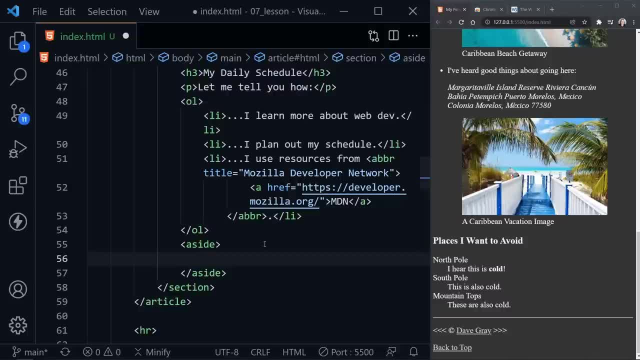 As what's in the main section Or article that you are putting it inside of, And that's what we'll do here. And then I want to use Some other semantic elements Just to demonstrate how they work. So now I'm going to add: 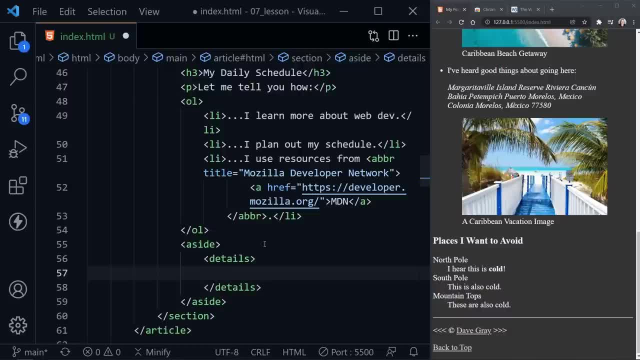 A details semantic element And inside a details element You want to add A summary element. If this was a product, We might just put warranty information In here as the summary. Here I'm going to put something that's more like a question. 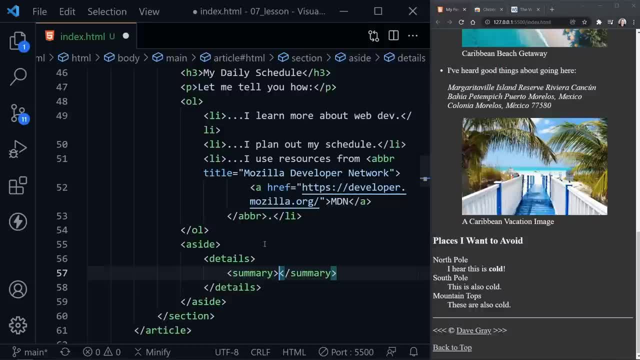 And it will display how The details and summary work. So I'm going to say: Guess the number Of hours I code Per day As our summary. Now underneath we can put the answer to this question, And now I'm going to put. 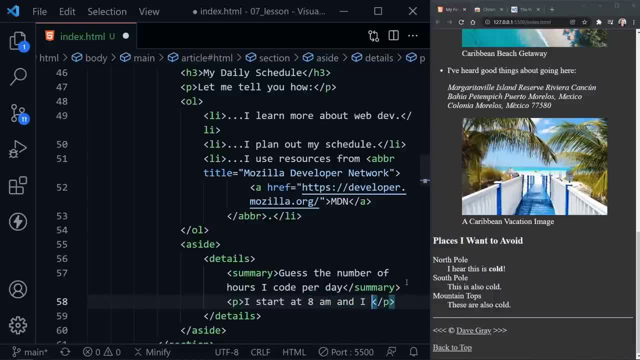 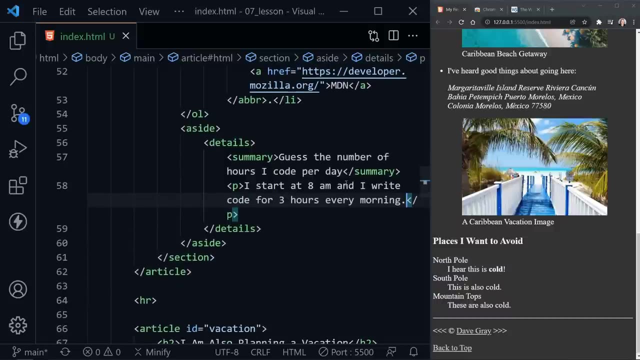 I start at 8 am And I write Code for, Let's say, 3 hours Every morning And we can save that. I'll scroll up So we have it up here Towards the middle of our page. 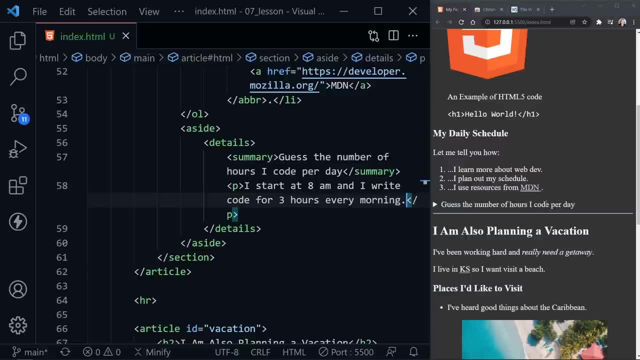 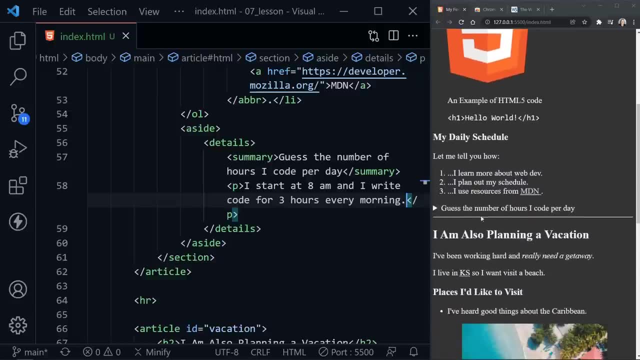 And now let's scroll up here And let's look at what we have on the page, Because the rest of our semantic changes Really didn't change the appearance here, But this Where we added this new content- Notice we're not seeing this paragraph. 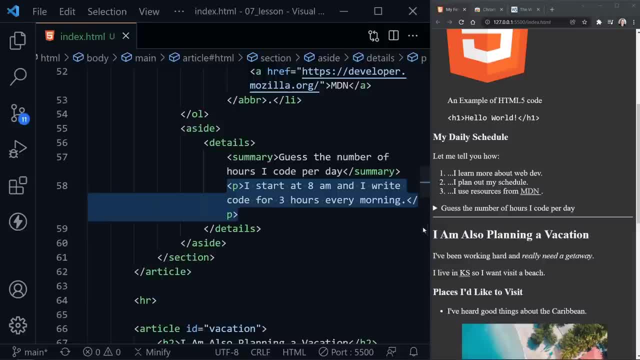 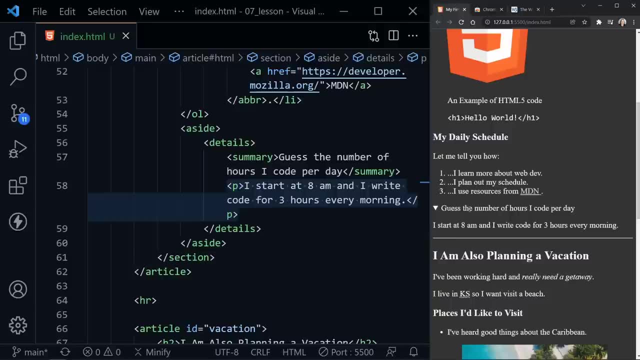 At this point We just see Guess the number of hours I code per day. But it has this little arrow next to it. If we click on this, Then we see the answer. So that's a nice little addition That this HTML element adds. 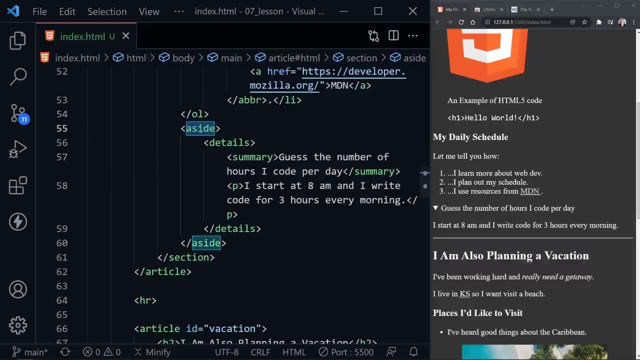 And again, These are all semantic elements, So the aside has some meaning That it's complementary text. It's not as important as what's in the rest of the article. The details, The summary work together, So this could once again. 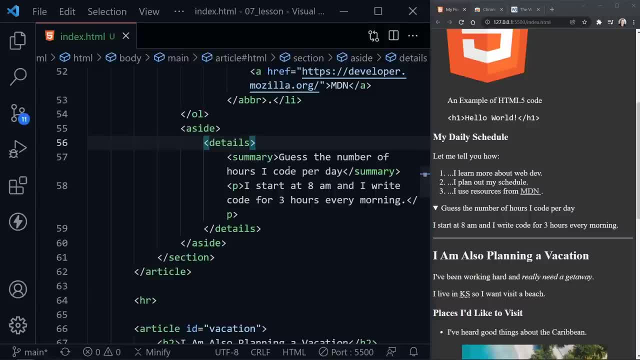 Provide details about a product, Say warranty information, Something else, A return policy, Whatever. But you could also use it kind of as a quiz here, Where you have a question And an answer. Let's go ahead and add just a couple of more semantic elements to this. 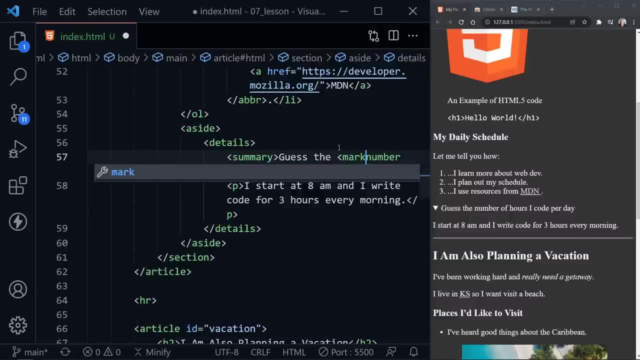 One is what we can do with a highlighter, Just like you might use a highlighter on a piece of paper. There is an element called mark, What I want to highlight here in the text And by including it in the text, You know it's an inline element. 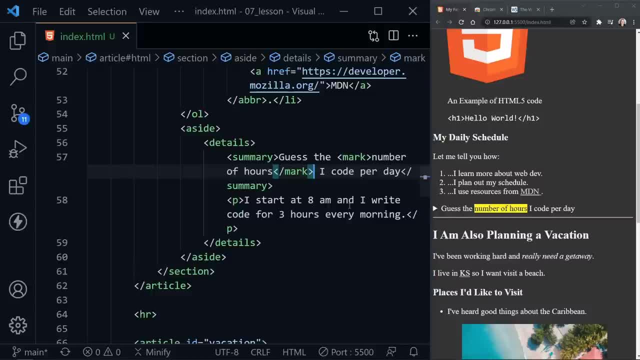 And not a block element. So now, if I save that, We have highlighted Number of hours Now inside the answer. We're looking at some time here. We have 8 am And we also have a duration of 3 hours. 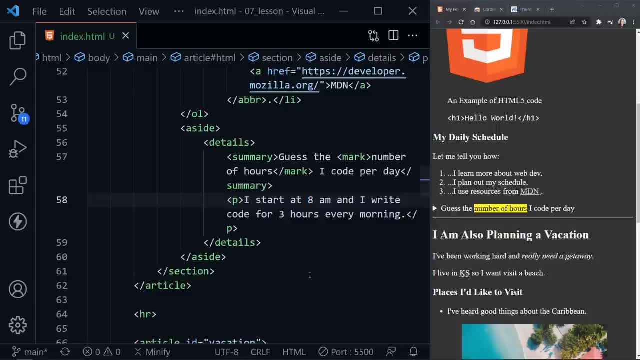 We can add some meaning to that In the text as well And we can provide a time element. Then we need a date Time attribute And for the date time attribute value I want to put in The actual hours, It accepts several values. 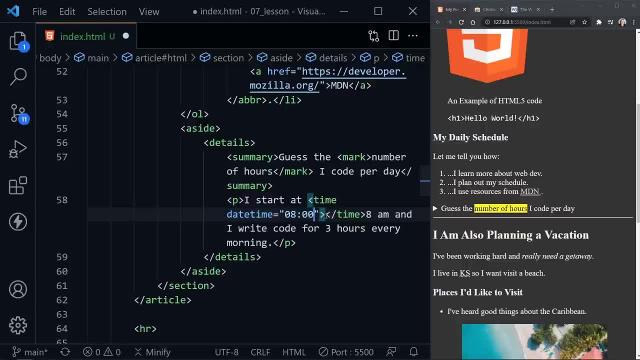 So this would be 0800 on a 24 hour clock, And now let's put the closing time element After the 8 am here And notice, If I save this right now And show this, It does not change What 8 am looks like at all. 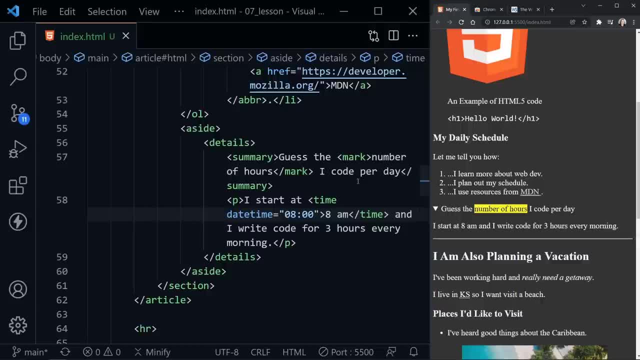 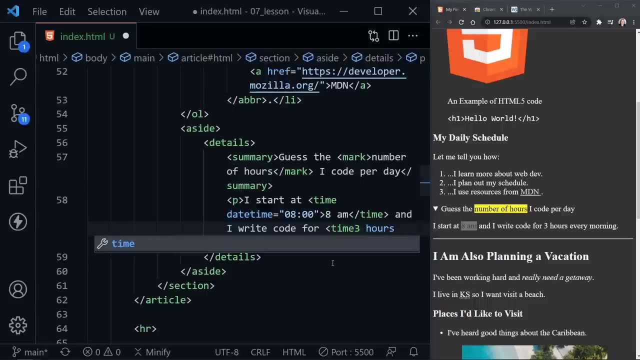 But once again, It provides meaning in our HTML When we are reading it, Especially those assistive technologies. But it could also provide some meaning For the browser itself. Now also, it says: As I write code for 3 hours, We can provide a time element. 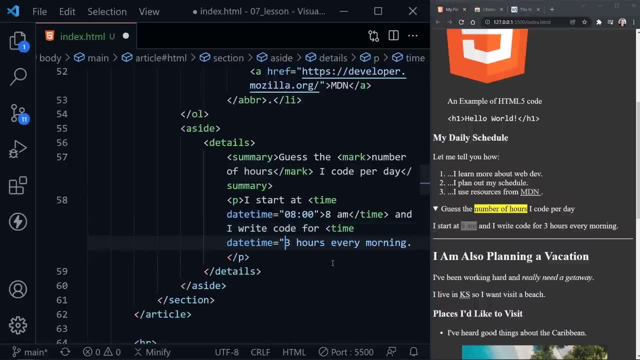 For the duration too. So we have time Once again with the date time attribute, And now we'll put in a different value, Because there is a value for duration. I'm going to put this closing Tag at the end of the 3 hours. 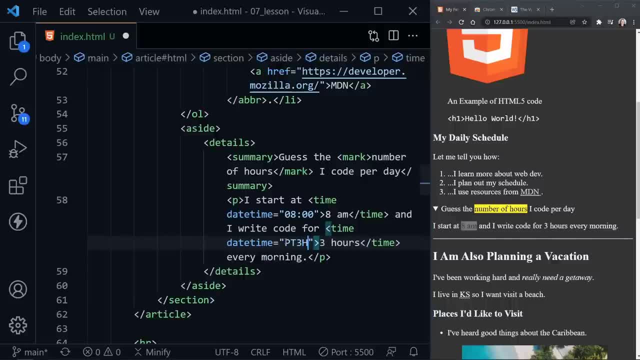 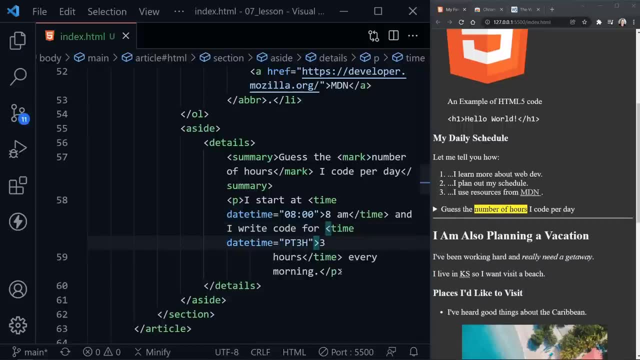 Now let's look at the value for duration PT3H And remember there is a link In all of the HTML resources That I link to in the description. There is a link That shows all of the HTML elements So you can look up, for example, 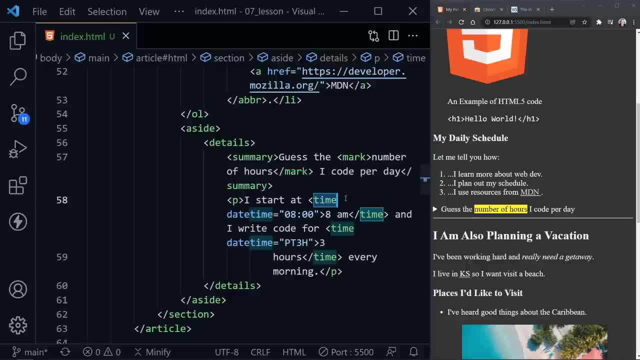 The time element on the Mozilla Developer Network. That's the MDN site And you can look at all the values That could be accepted For the date time attribute. Okay, let's save this And move down to our vacation area, Where we also want to add two sections. 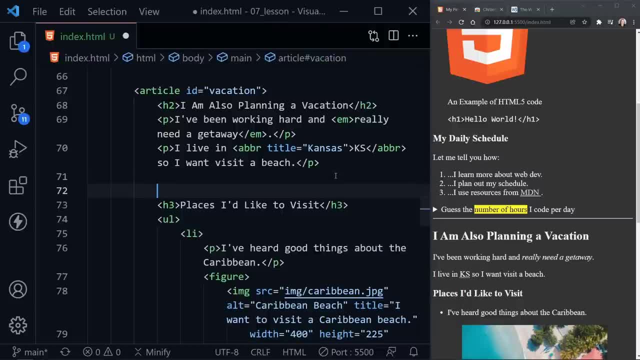 I think these are clearly defined already, Where we have subheadings For places I'd like to visit And really we have a subheading for places I don't want to visit, I believe. So here let's go ahead and add a section. 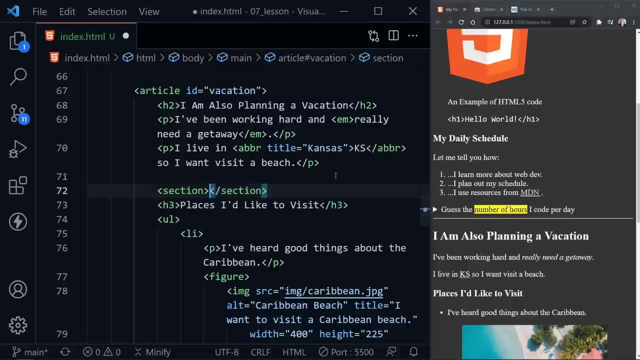 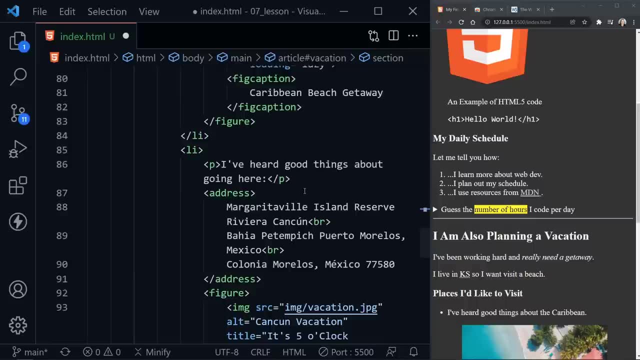 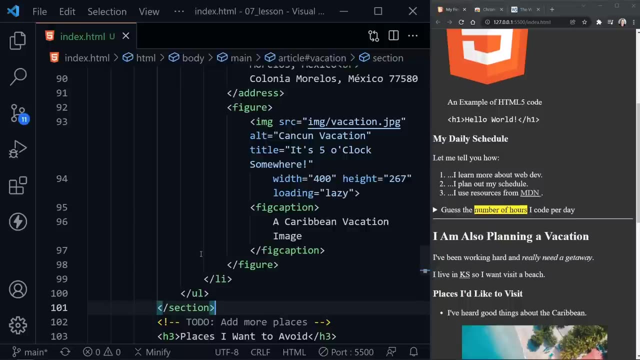 Again lower case, And I'll take that closing section tag Highlight it, Control X, to cut. I'll scroll down here And we'll add that before The next subheading. So there we go, Save that And of course it reformats again. 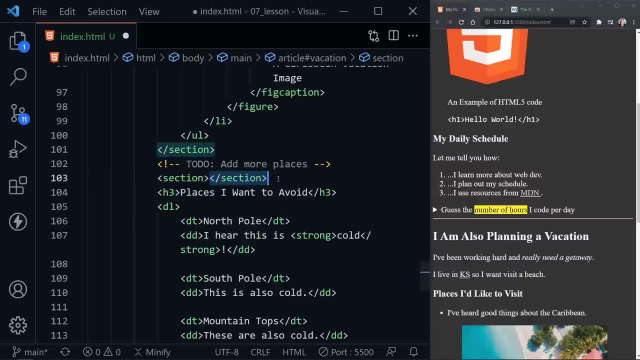 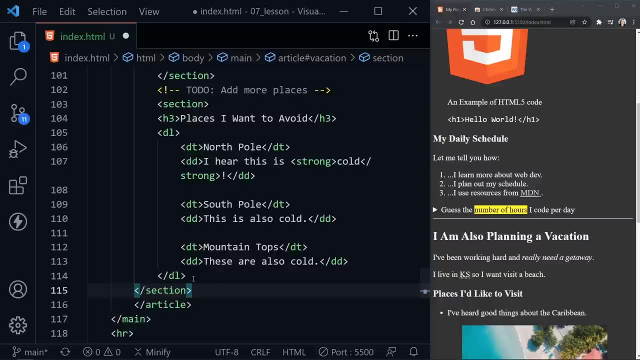 Now I'll add a section element And put the closing after We finish our places. I want to avoid Section And that would be at the end of our description list And we can save that. Now we've got two sections Inside of this article as well. 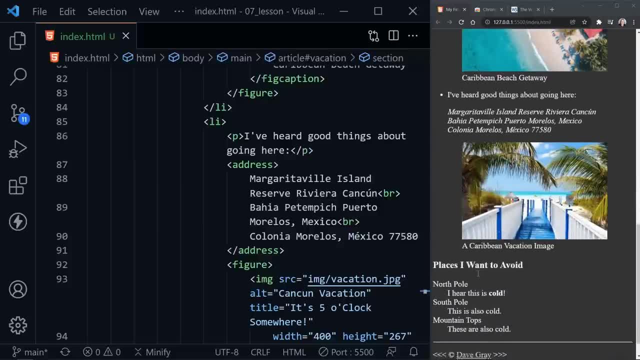 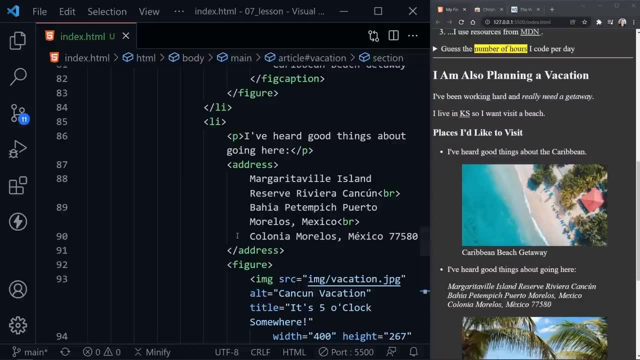 And really, once again, It doesn't change the look, But it does change how the browser interprets And it definitely adds A benefit for assistive technology. Now, before we look at our document outline With these changes, I want to quickly discuss. 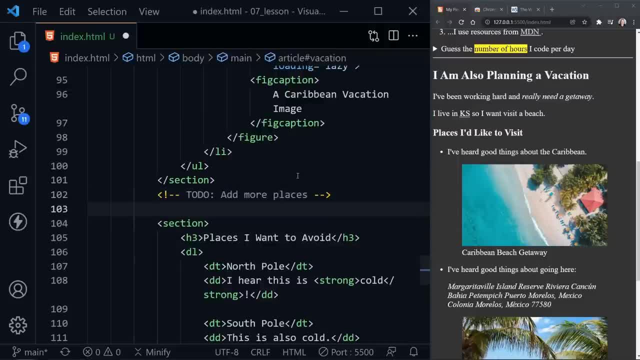 And I'll just do it here by this comment, Where it says: add more places, Two different elements That you want to avoid as you're learning HTML, And then later on You can use them as we possibly get into them with CSS. 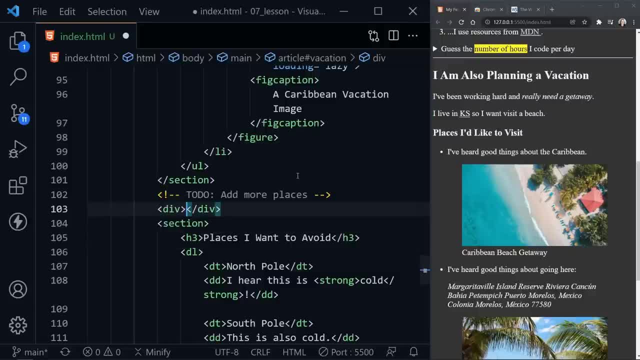 But there is a div In an older HTML code. You will see divs everywhere. Sometimes you still do, When those people that have been using divs Are used to still writing them And they just continue What they've been doing in the past. 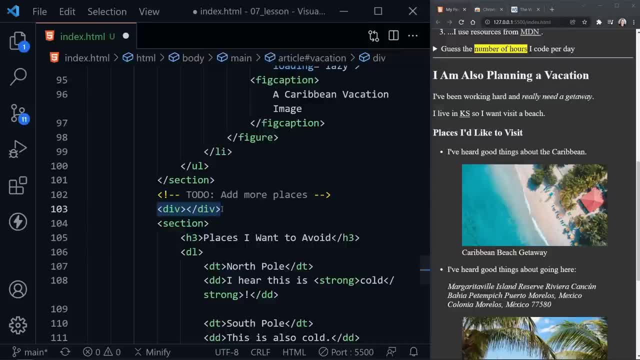 However, there is no semantic meaning to a div. Think of a div Much like a section, Without the semantic meaning. It just stands for divider And really you can put them anywhere, But if you do, You really have to do a lot of work. 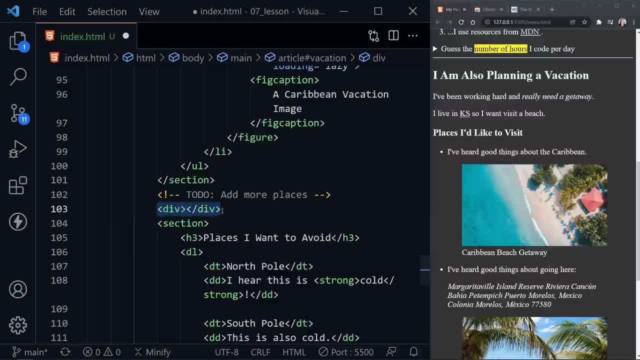 To get them to convey meaning, You have to add additional attributes That help assistive technology Interpret these elements, Because they have no meaning. They are block elements. So a very similar element That is an inline element. If we just wanted to wrap a word or two, 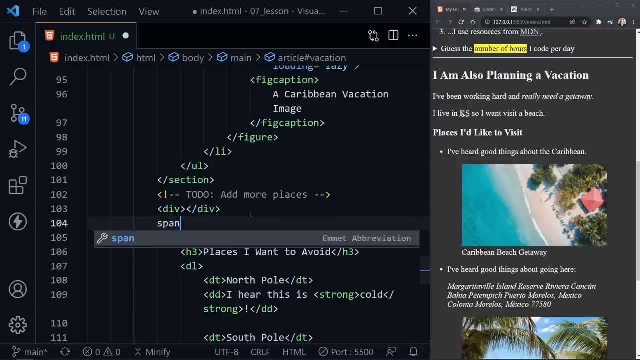 In a paragraph, In an element, Is span. We'll definitely use some spans As we learn CSS. However, once again, They have no meaning whatsoever By themselves. They don't change or add any value To your code, So we really want to avoid. 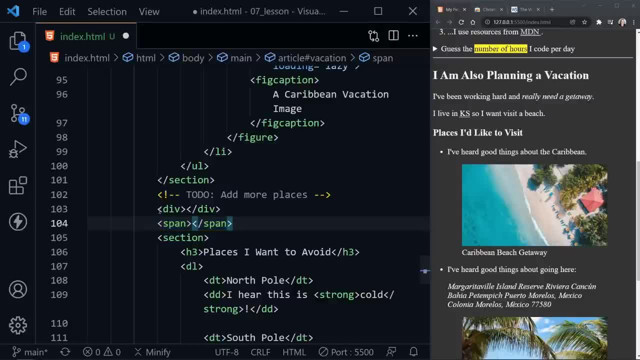 Both of these elements. As you learn HTML, Really work on using semantic elements And then, When you understand What semantic elements are And how to use them, And then occasionally, When just no semantic element Is the correct choice, That is the time. 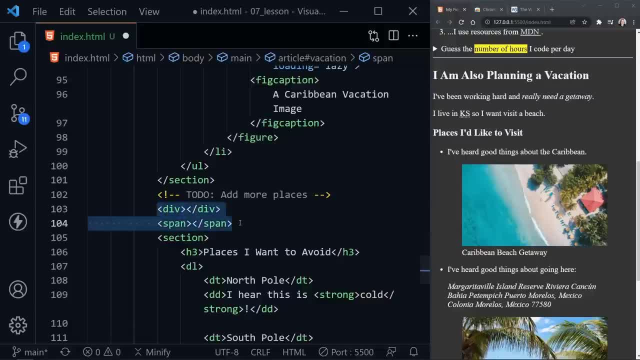 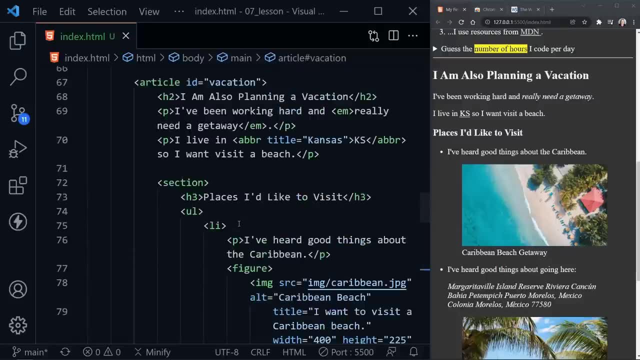 That we actually should use divs And spans, So I'm going to delete those for now And save our document. And now I'll just scroll our code Up to the very top, And I'm going to do the same for our page. 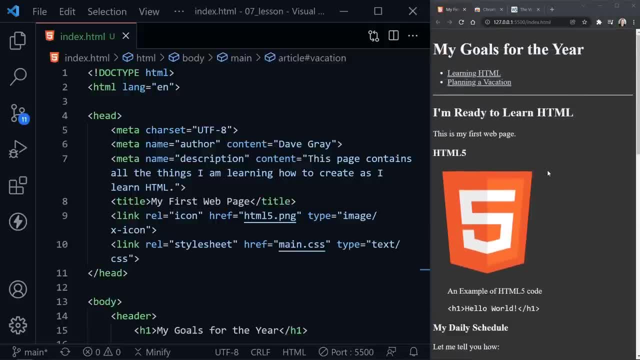 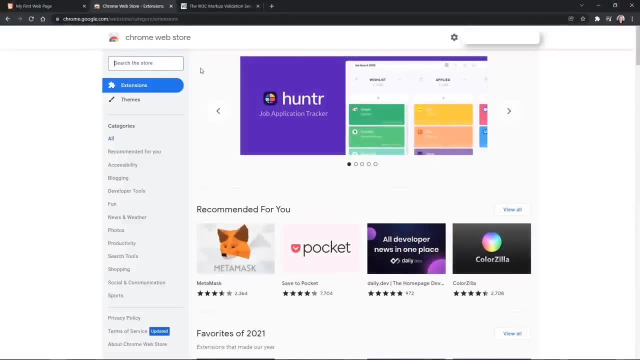 Over here on the right Now what I want to bring your attention to. I'm going to maximize the browser And we're going to go to the Chrome web store And look at an extension we can add, And that extension is: 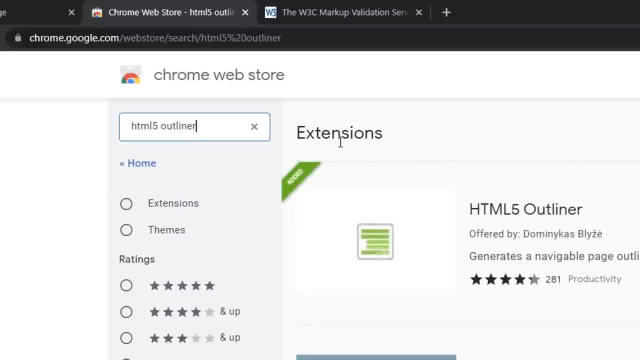 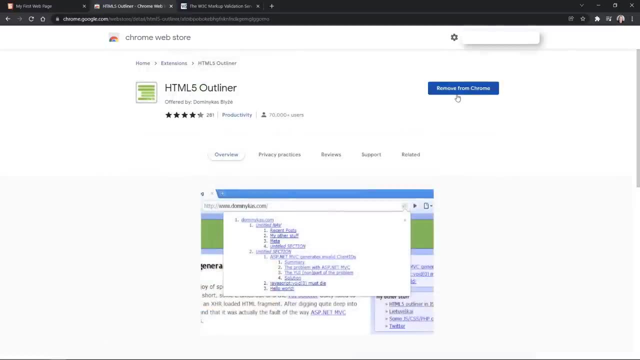 HTML5 outliner. So search for that. You'll find HTML5 outliner. You can click on that And I've got it installed already. So mine says remove from chrome. Yours would probably say install here And it will look at our. 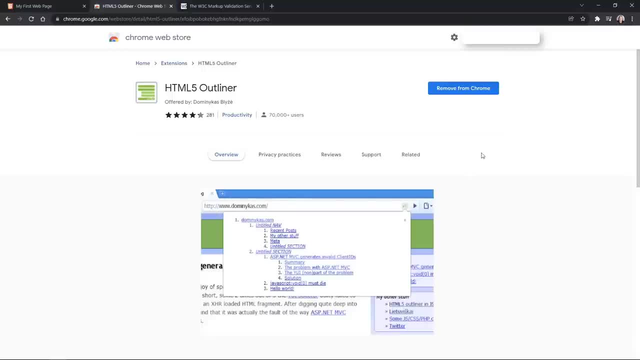 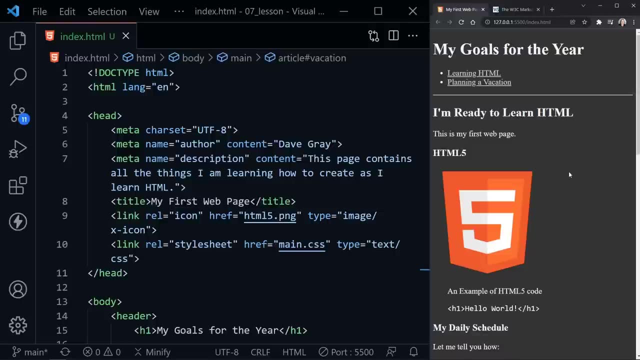 Semantic elements And make an outline of our page. So let's check that out. Okay, I'm going to bring our page back down to the size we had it Down here to the bottom Now, once you've got that extension installed. 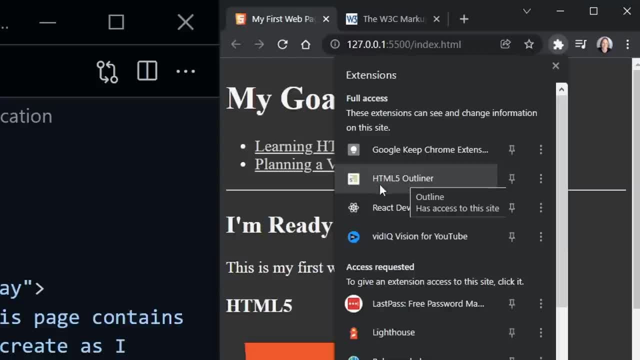 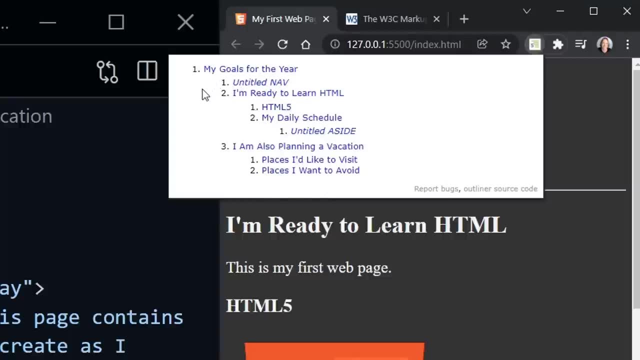 You may have to restart your Version of chrome to get it to work, But here we go. Click on HTML5 outliner And here we go. We've got our heading hierarchy correct With my goals for the year. An untitled nav. 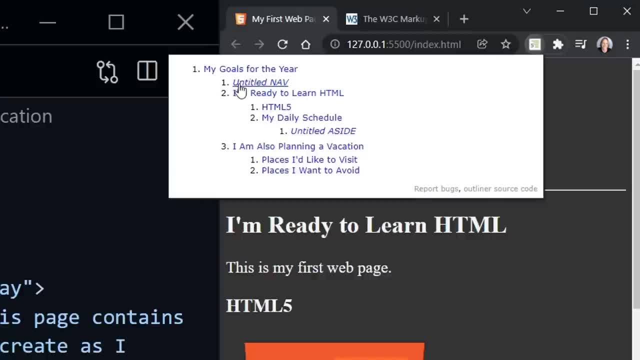 That's okay. We didn't put a heading in there. Like I said, we could have put an H2.. It's just saying we didn't have one, But a nav doesn't require one. But remember, if you do have more than one nav element. 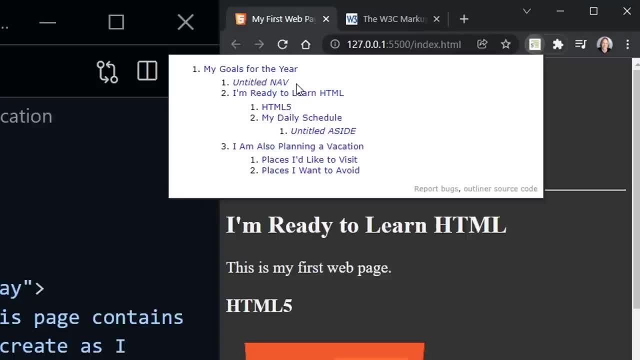 Per page, Then you do need to at least appropriately label that For assistive technology. Okay, now we've got another section. This is our article. We're in HTML and that's our H2 heading Inside the article. Remember, we have two sections. 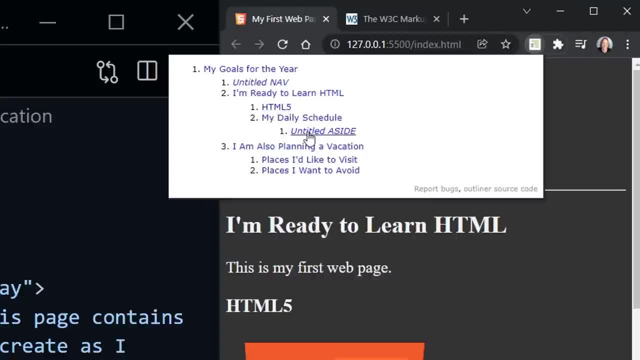 We have the HTML5 and my daily schedule, And then we have an aside, And this aside was inside The second section. It's also untitled, Which is okay. An aside does not have to have a heading, But it just notes that. 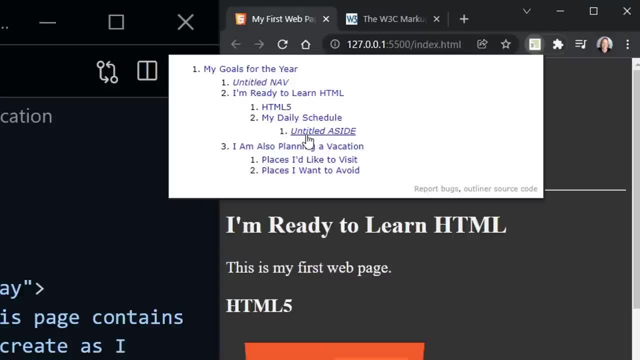 As it's untitled here. If you added a heading inside of the aside, Say an H4. Then it would of course appear there. Now we've got our other section, Our other article. actually, I am also planning a vacation. That was an H2.. 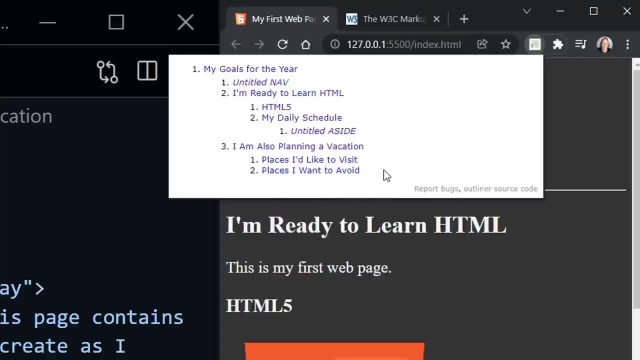 And then these are H3 headings, So you can see how important the headings are. The heading hierarchy- If you don't get any other semantics correct In your page, That's the one thing to really understand- Is the heading hierarchy of a page. 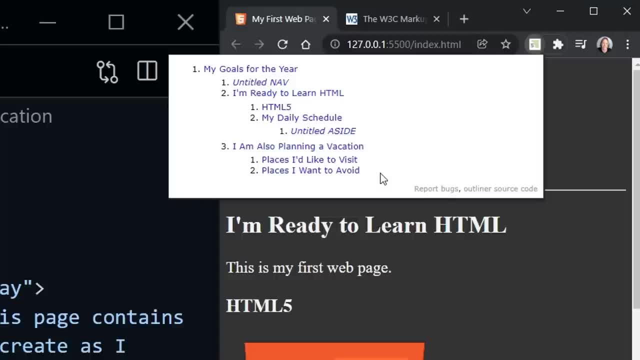 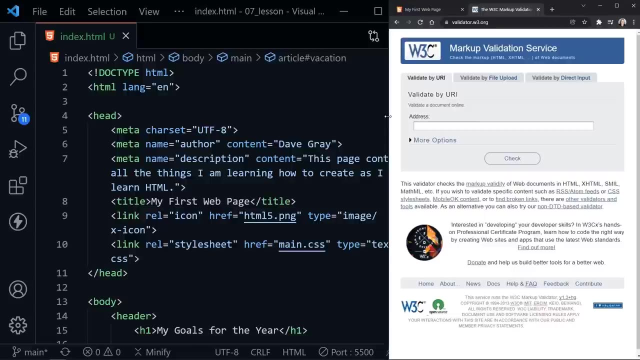 But all of these other semantic elements Definitely help outline your page And add meaning To your page, And that's the biggest mistake You can possibly make As you are constructing an HTML page. Okay, Now that we've looked at our outline, 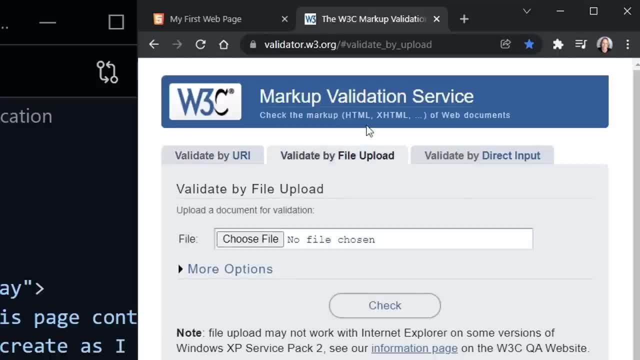 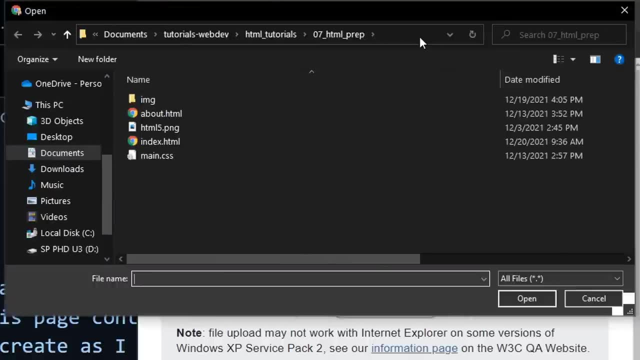 Let's once again validate our page. I'll pull this over Just so we see a little bit better. I'll click file upload. We're at validatorw3.org And I'm going to click choose file. I have to make sure I'm in the right lesson folder. 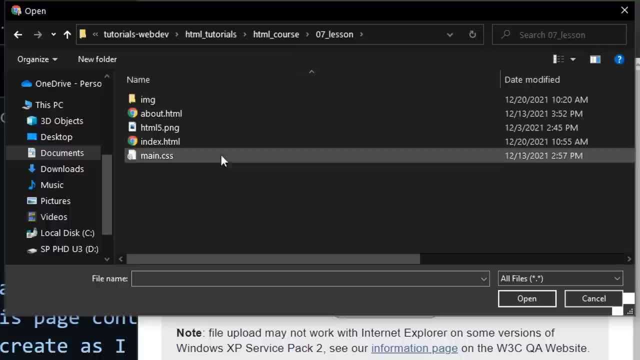 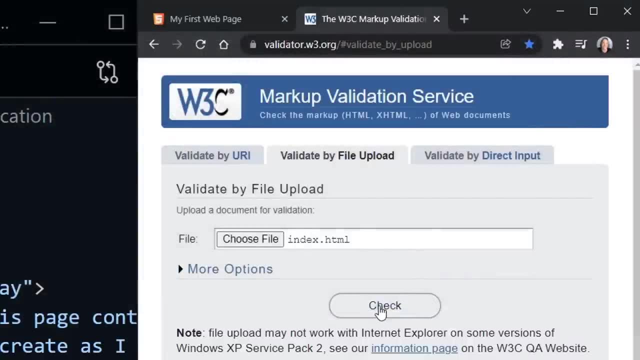 I am not, So I need to go into HTML course And I'm going to go to indexhtml. Just make sure you upload the indexhtml You were working on for this lesson. Click check And we'll see if we have any problems. 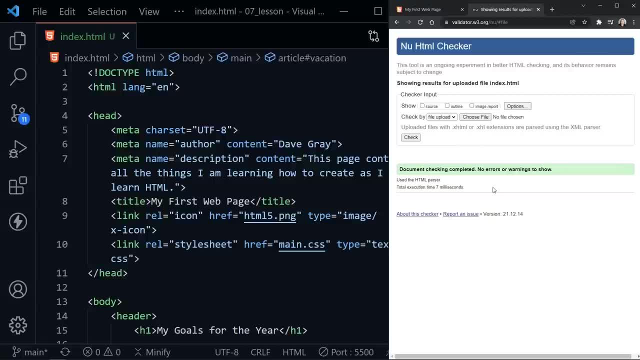 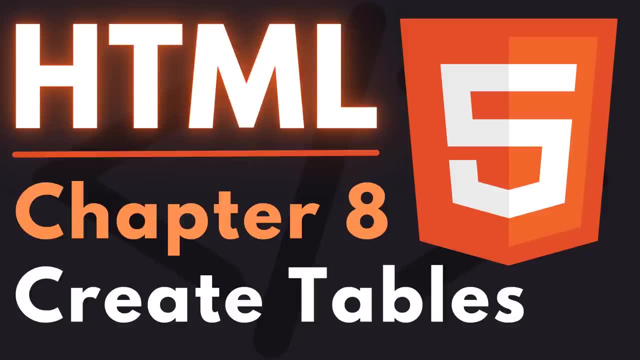 If you have a problem, It will show here. It should tell you what line and what the problem is. But we're good to go. Document checking completed. No errors or warnings to show. Let's add a table to our web page. 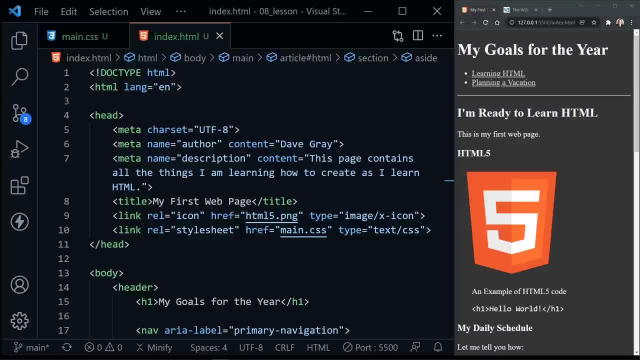 Tables structure, tabular data, That is, data that's made up of rows and columns. We often see this with schedules, Statistics in sports And many different types of data- Flight schedules, for example- And what we don't want to use tables for. 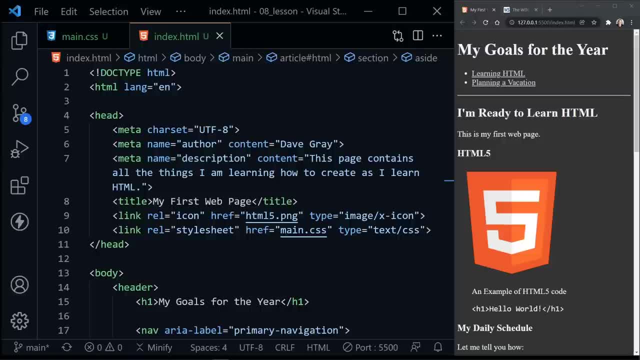 Are an entire page layout. Back in the 90s and early 2000s It was very common to use a table to structure your entire HTML page. So you may see some old code that does that, But we do not want to do that. 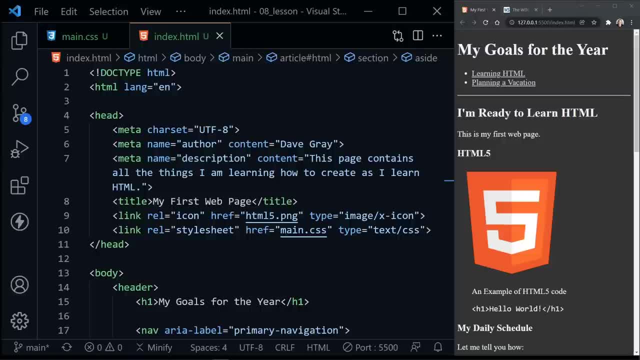 We want to stick with semantic HTML And in the future you'll learn CSS And we'll design our page layouts with semantic HTML and CSS, Not tables. Okay, Tables do really need a little bit of CSS To look kind of accurate. 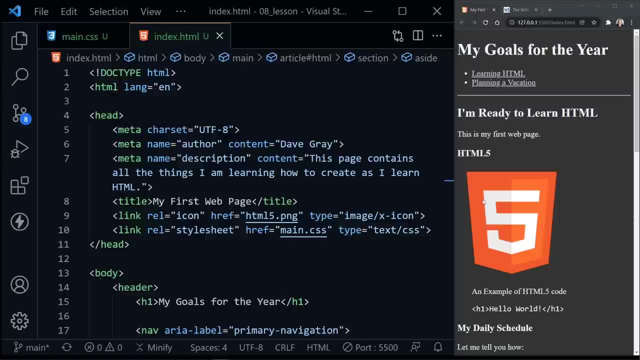 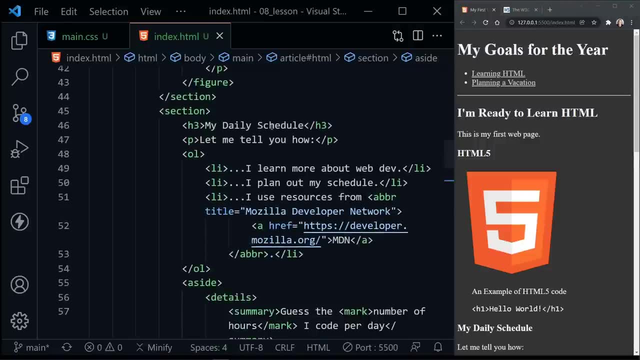 However, We can start creating a table without CSS, So let's do that. now I'm going to scroll down in our HTML file And we want to get to this section that says my daily schedule, The subsection, And then we describe the daily schedule a little bit. 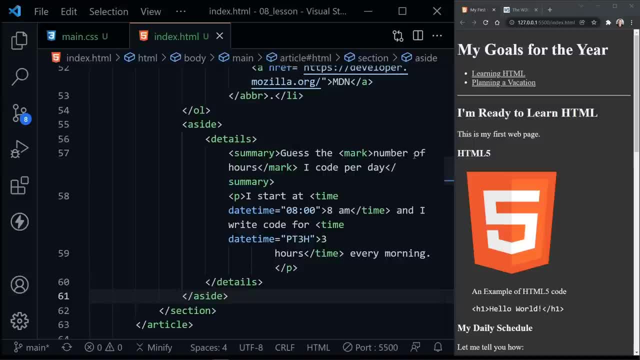 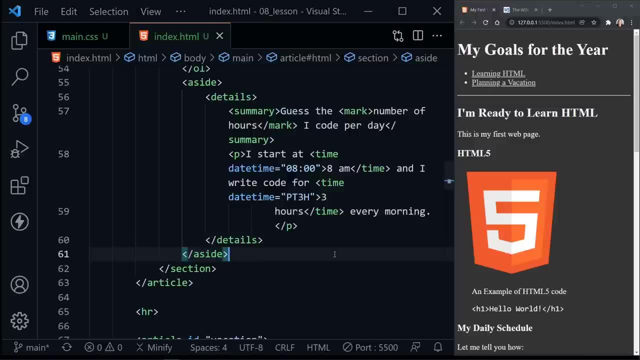 And we even have the aside here that says: guess the number of hours I code per day. So we want to put some of this in a chart Or a table if we will, But really a chart I guess. So Here we go with a line break. 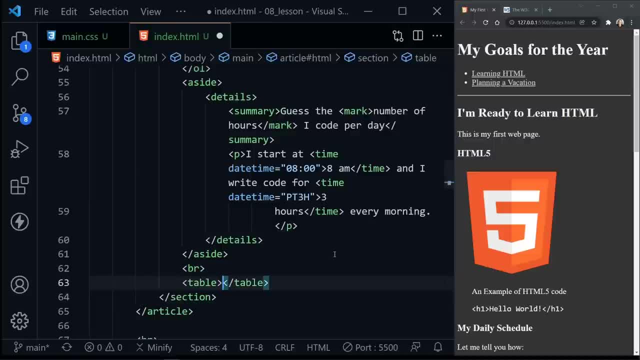 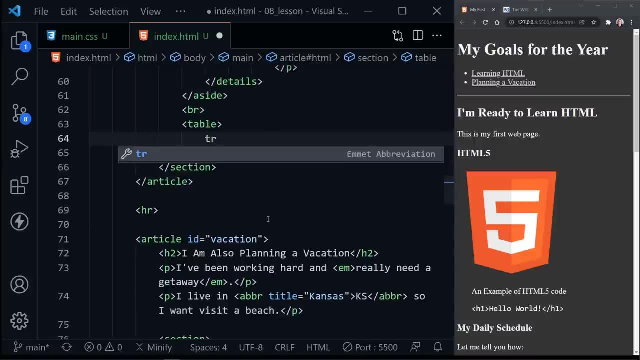 And underneath this break We'll put a table element. Inside the table element I want to scroll up just a little bit So we can see this better. Inside the table element I'm going to type a tr element Which stands for table row. 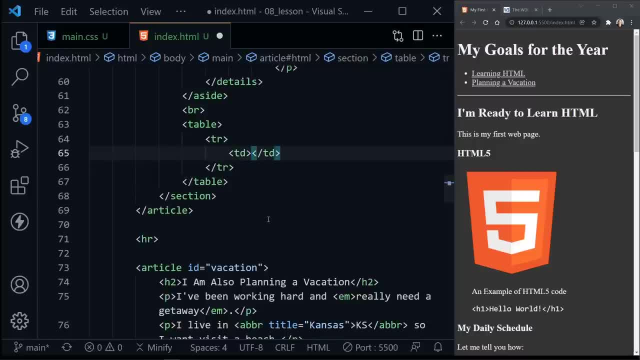 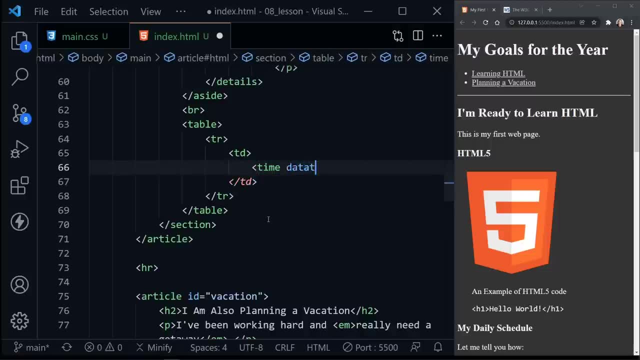 And inside the table row we put our data cells And those use td elements, Which stands for table data. Okay, So we have a time element Which is going to have a date time attribute. We'll set that equal to 8 am. 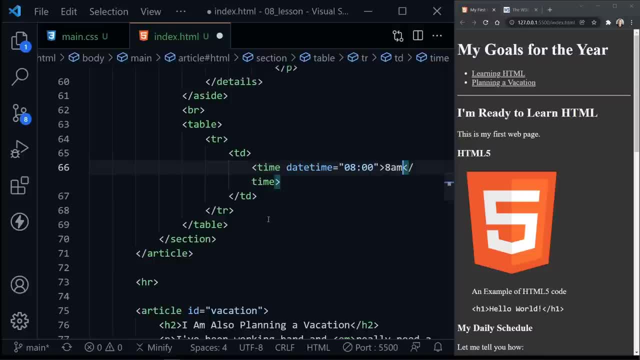 And inside this We'll put 8 am. Notice I've pressed alt z already, Which has my code wrapping down to the next line. If it would extend further. So if your code is extending outside of the window here in Visual Studio Code. 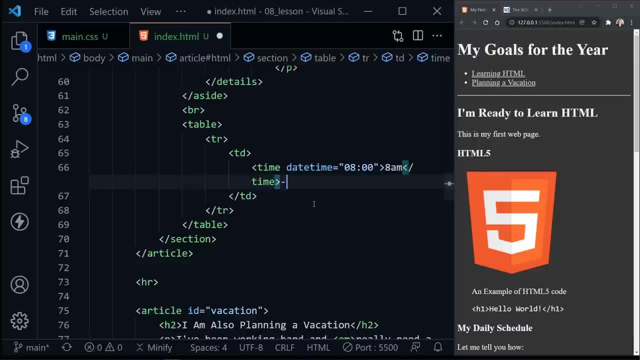 Just press alt z And it will wrap to the next line. I'll put a hyphen here. Another time element With a date time attribute. I'm going to set that equal to 11 am And I'll put 11 am here. 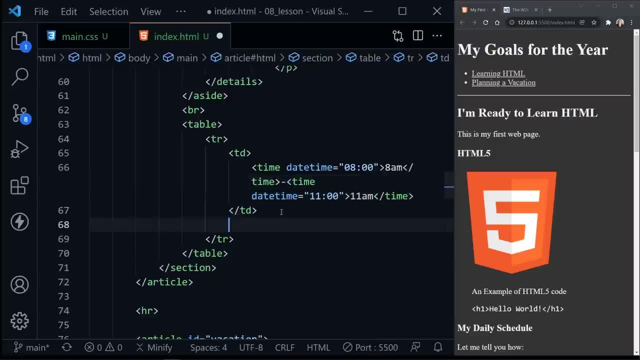 So now we have 8 am to 11 am In our first data cell And then I'll put the activity In the next data cell And here we'll put write code. Now I'm going to highlight this Full row. 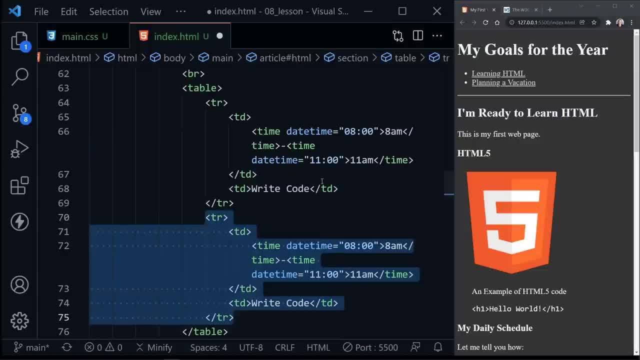 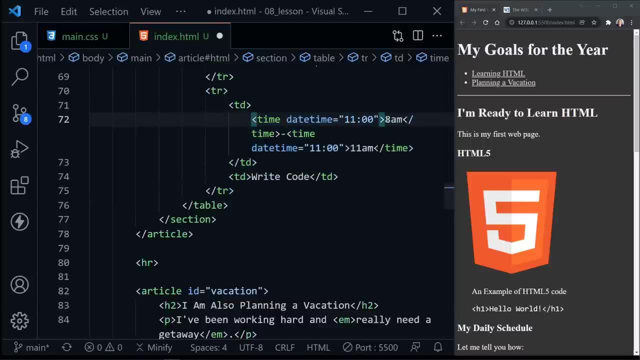 And then press shift, alt and the down arrow And it will copy that down. So I've created another row quickly So we can just edit Some of the information here. So now I'll start at 11 am And then I'll switch. 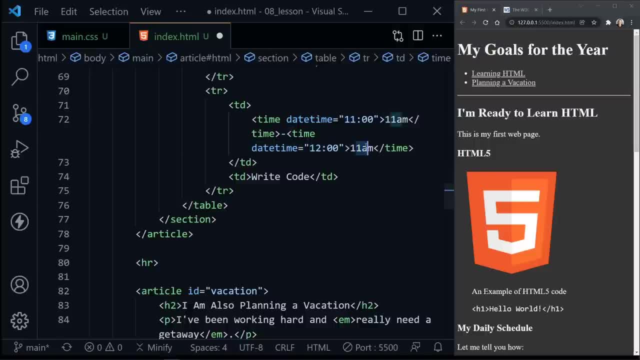 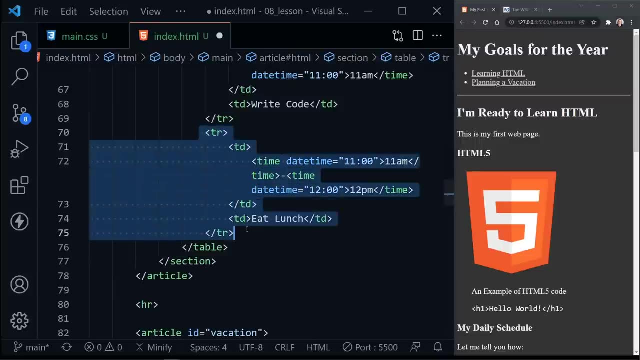 The next one to 12 pm, And so there's Our one hour for lunch. So here we can put Eat lunch. Now let's do this One more time, Or I'll highlight the row And then press shift, alt and the down arrow. 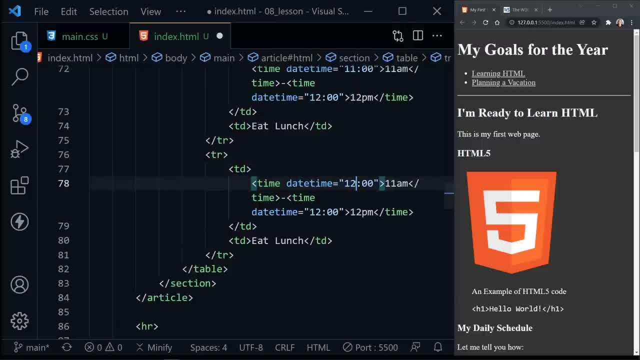 And now we'll have our afternoon time here. So this is a 24 hour clock That we need to be aware of as well. So we'll start at 12 pm, And now this will be 17.. And this would be. 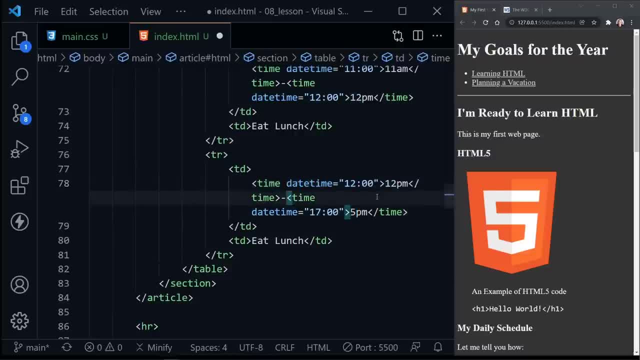 5 pm over here. So now from 12 pm To 5 pm We can put in another activity And I'll just say study for Other courses And we'll save. Now let's scroll down over here in our 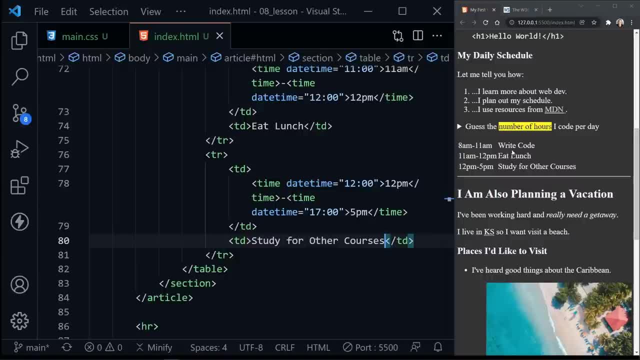 HTML and look at the table. We've applied no CSS So we can see the columns With the times on the left And the activities on the right, But it is a little hard to make out That this is a table, So I want to add just a little bit of CSS. 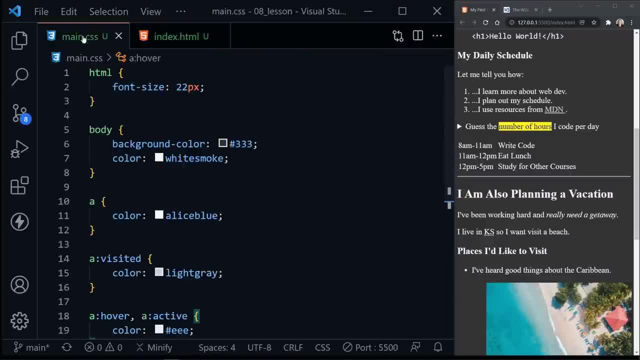 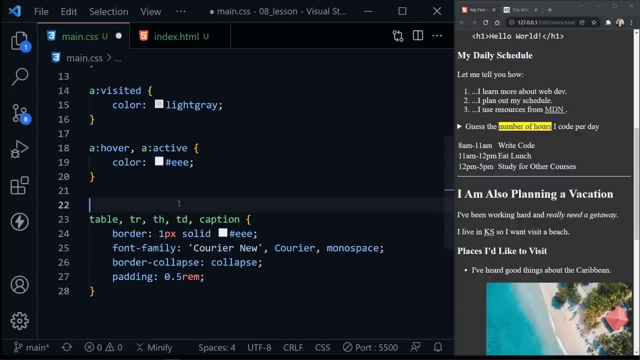 To help our page out, I'm going to click on the CSS file That we've linked to our project. Scroll down to the bottom And just paste in Just a little bit of CSS. for now, This will be available in the files. 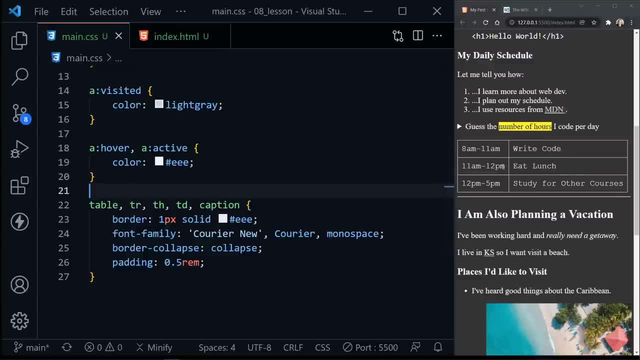 And once I save that We can quickly see how it applies to the table. This looks much more like a table. 8 am to 11 am: write code And we can see clearly Each time, block And each activity. I'm going to go back to the HTML file. 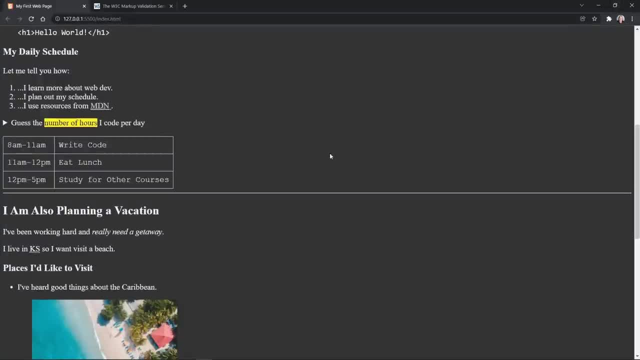 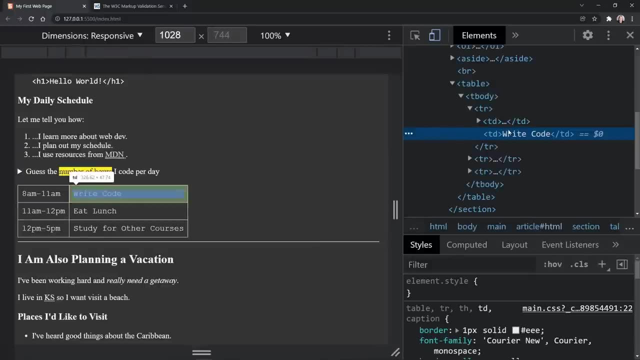 But I also want to expand the browser. To highlight something that happens here in the code. I'm going to right click on the table And click inspect. This will open dev tools And it should be showing the elements Now if we highlight the table over here, 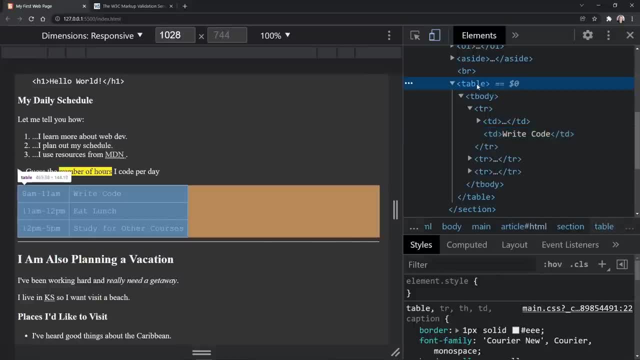 In the elements tab in dev tools You can see it's highlighted on the page. Notice all the orange to the right. That is margin. That is not table. So the table doesn't expand to the width of the page, It only expands. 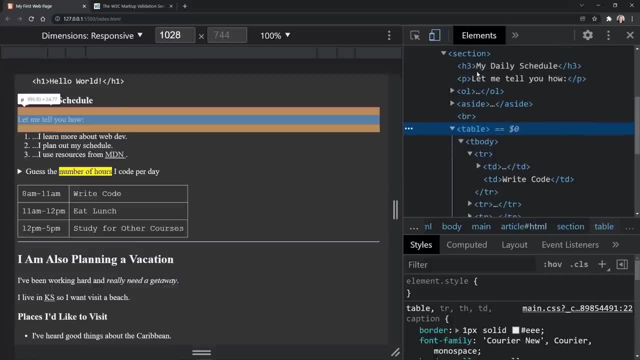 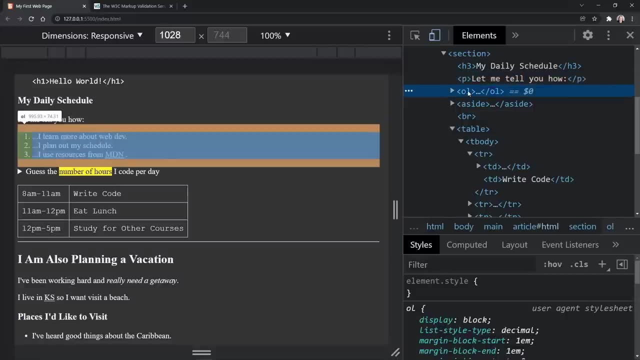 Based on the content inside the table. That is different from some other elements, Like the paragraph element- Notice how it expands for the full width of the page- Or the ordered list element That we have here: It expands for the full width of the page. 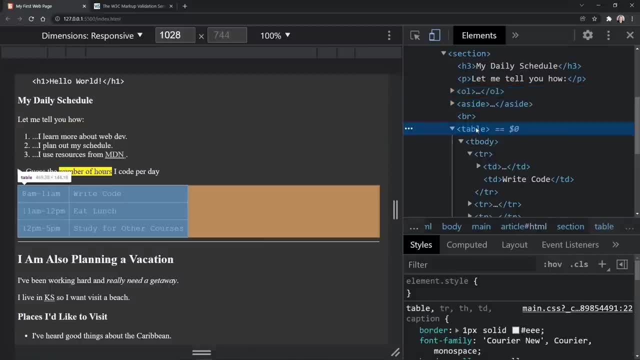 The same with the aside element, So it's worth noting that the table is different From a lot of other elements That automatically take up the full width of the page. The table element only expands To contain the content That is within the table. 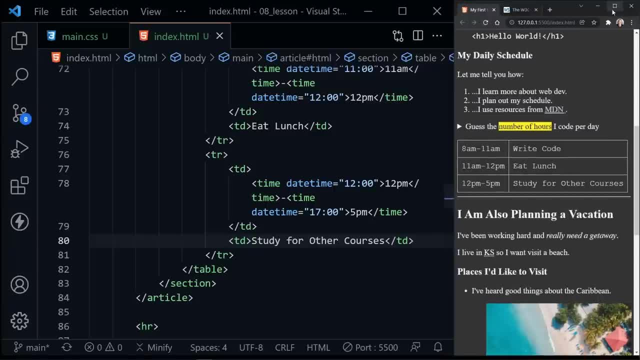 Okay, I'm going to close. dev tools Resize chrome once again, So we can see our code here on the left, And what we are missing from a table Are headers for our columns. We clearly have a time column And an activity column. 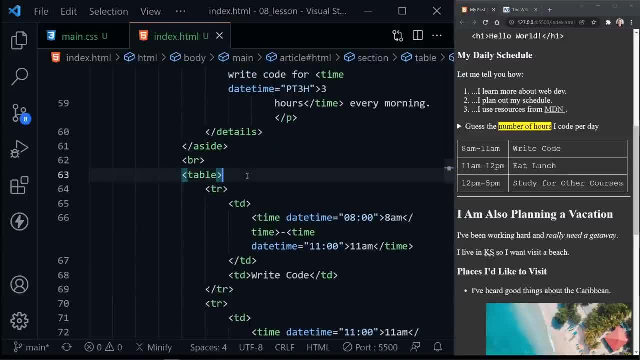 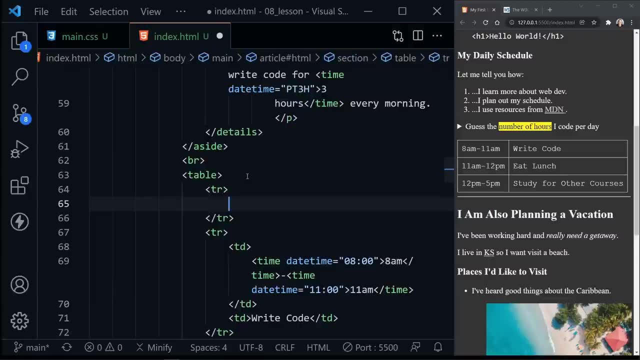 So let's add that By adding a row at the top of the table, We'll start with the T element, again TR element, And then inside, Instead of TD for table data, We have TH elements For table header, So we'll have time. 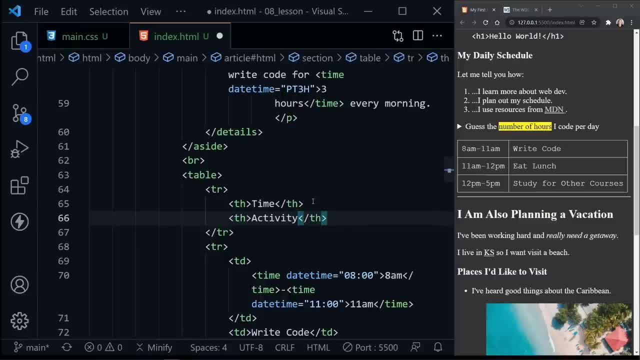 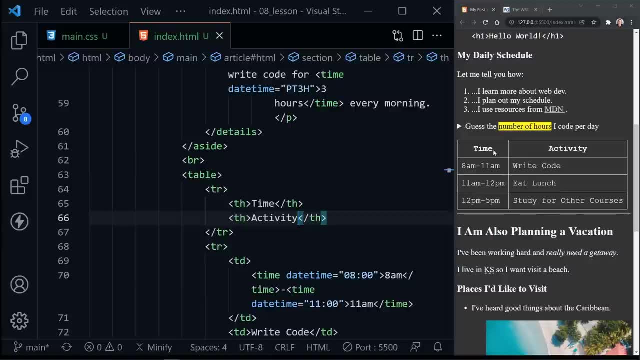 And then we'll also have Activity. And now, if we save that, Notice that the time and activity Are formatted just a little differently, And I did not do anything different For these headings In the CSS. What we have is a centered heading. 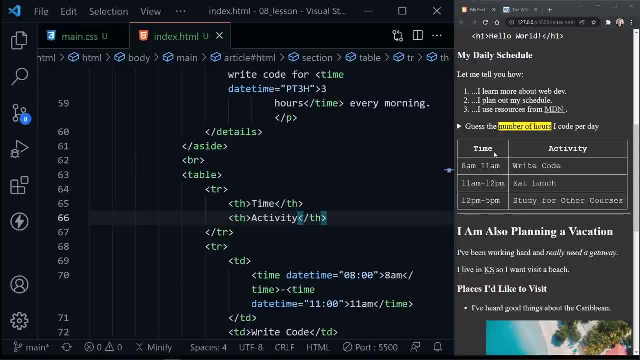 And it is in bold, And that is the default styling That is applied to table headings. Now, what if we had some data That needed to take up two columns In our table? So, in other words, one cell Would span the width of both columns. 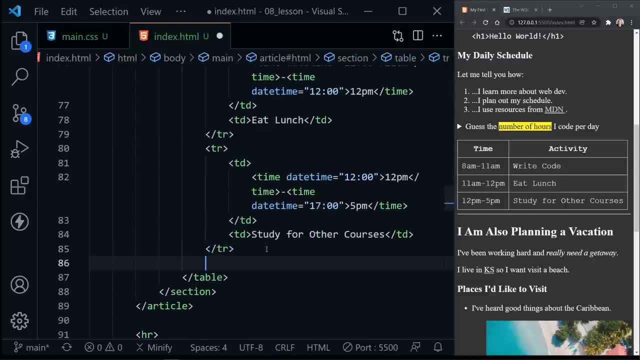 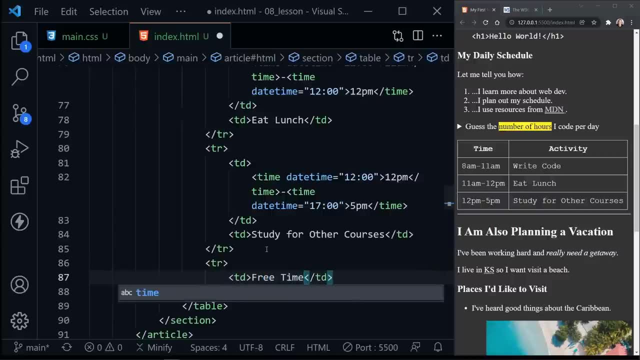 We can do that. So let's add a row at the bottom And inside the row We'll put one data cell And I'm going to put free time Inside here for data. But there is an attribute Called call span. 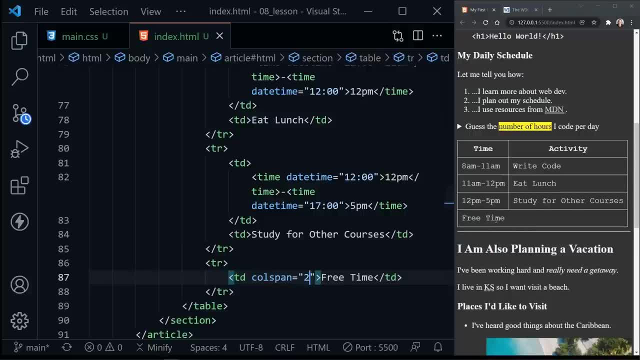 That's equal to two, And this will take up the width Of both columns. Okay, now I'm going to remove this call span And let's put A data cell before free time here, And here we'll say: Inside of this data cell. 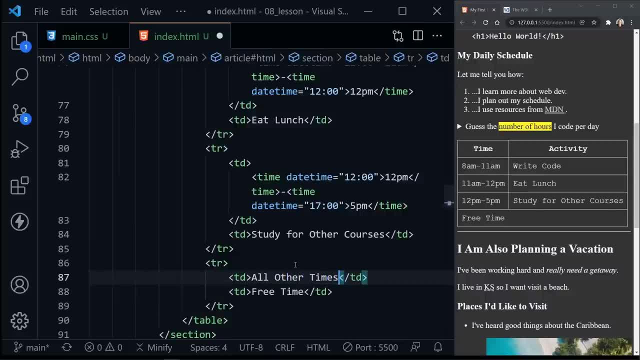 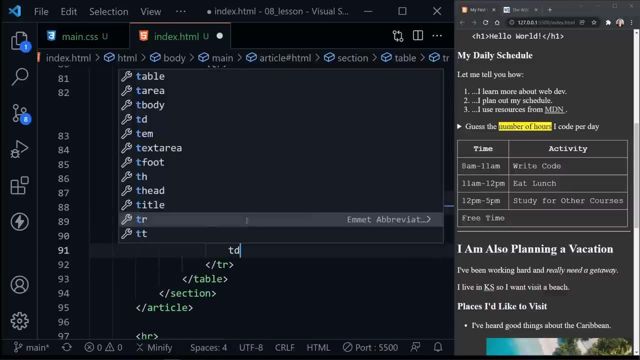 Let's put all Other Times, But for the attribute on this cell, Let's put a row span, Which also exists, And we'll have this. take up two rows Underneath And in this row we'll only have one data cell. 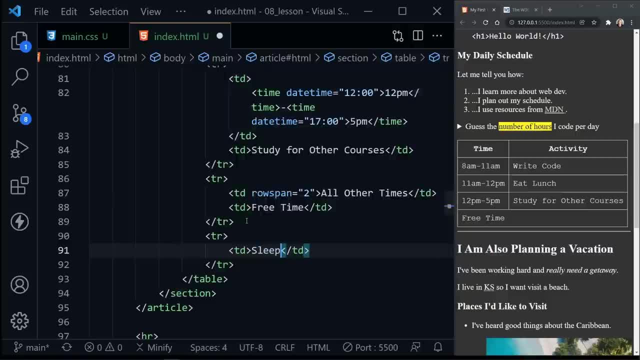 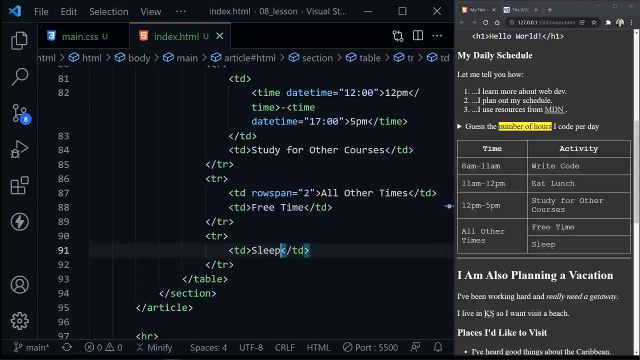 And here we can put Sleep Now. if we save, You can see our all other times Is taking up two rows And now we have free time and sleep On the right Now. our previous lesson covered HTML semantics, Which definitely 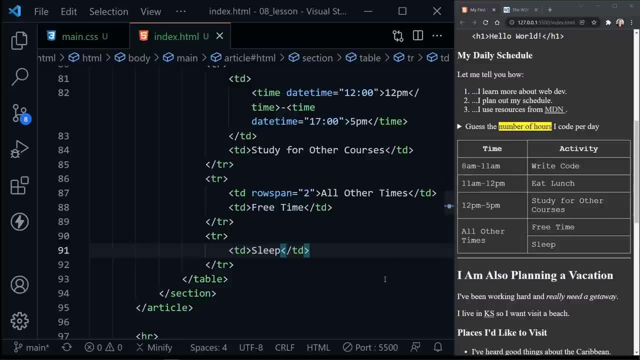 Helps structure a page And tell the browser what the page is about, And it also helps assistive technology Like screen readers Navigate a page For those that do not use a mouse, For example, to navigate the page. So let's scroll up. 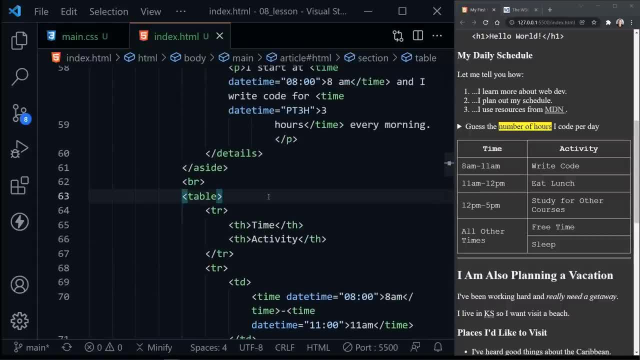 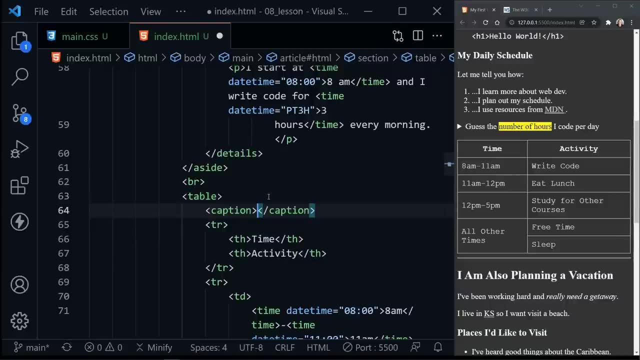 And start adding some semantics to our tables, Because that is also possible Underneath the table. The first element we want to add Is a caption. So we add the caption And we can say what the table is about, And that would help someone navigating with a screen reader. 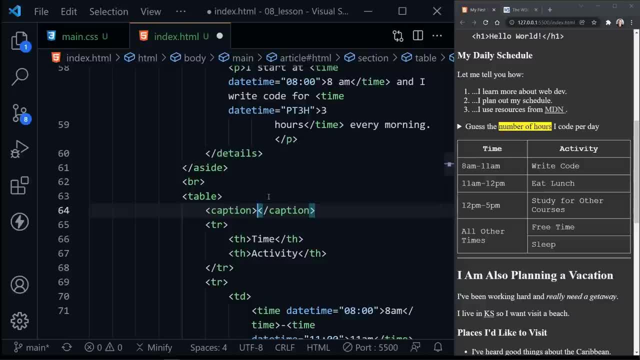 Decide if they really want to navigate the rest of the table Or just skip over it And Start visually. So let's just put in my daily schedule Like the same title we have for the subsection Above in the H3. And as soon as I save that, 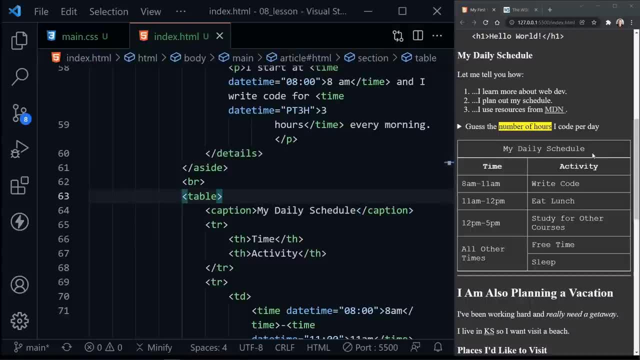 You can see now the caption Spans both columns already And is centered, And we didn't have to add a column span for that to happen. That automatically happens with the caption. After that We can clearly define sections Of a table. 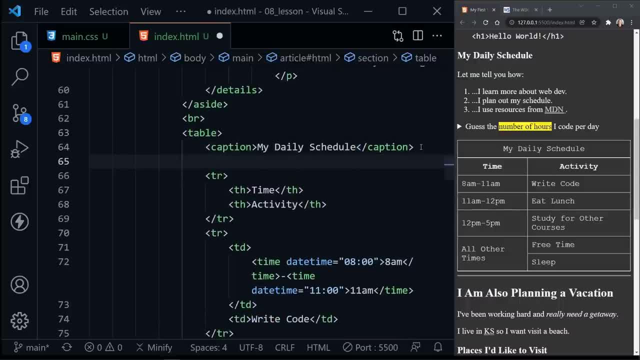 Much like we do sections of a page. So let's start out with the header, And this is the T Head, Which stands for table head. Now I'm going to go ahead and highlight the closing tag. Press control X To cut. 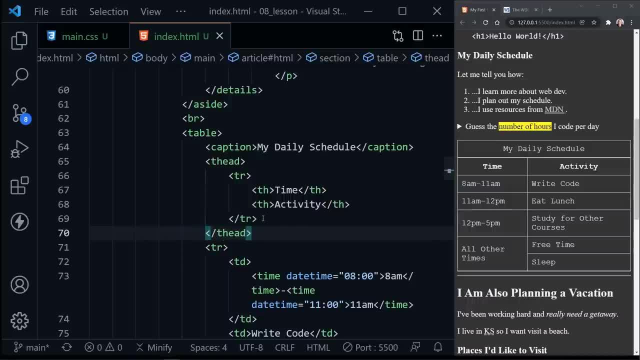 And add it underneath the end of the row And we can save. And here you see The full table head, clearly defined. It doesn't change the appearance at all, But it adds semantics to our table. Likewise, there is a T body element. 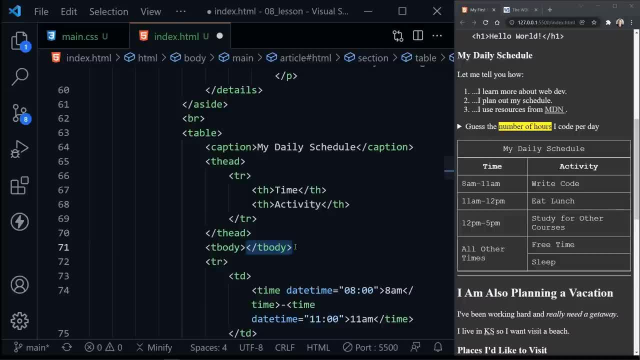 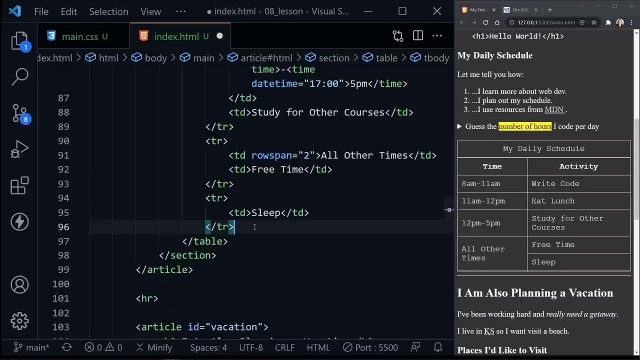 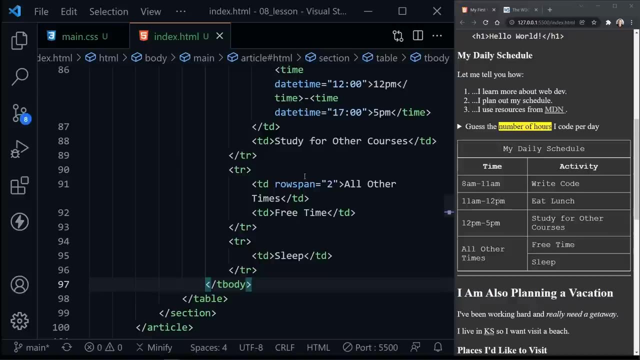 For the table body. So I'm going to once again Add the closing tag. Press control X To cut. Scroll all the way down to the end of our table, The last row, But before the closing tag of the table, And paste the T body tag. 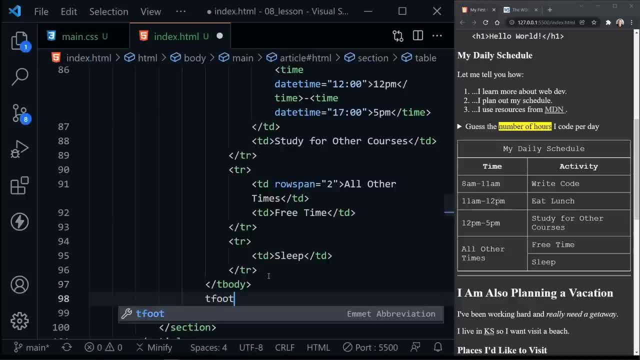 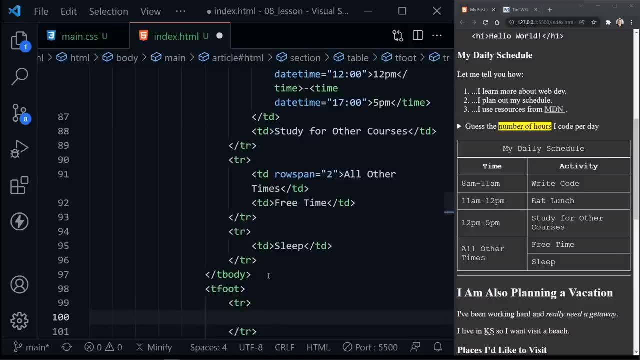 So now we've got a head and body section For our table. We can also add a T foot section. So now inside of the footer I'm going to put another row And inside the row I'll put a data cell. 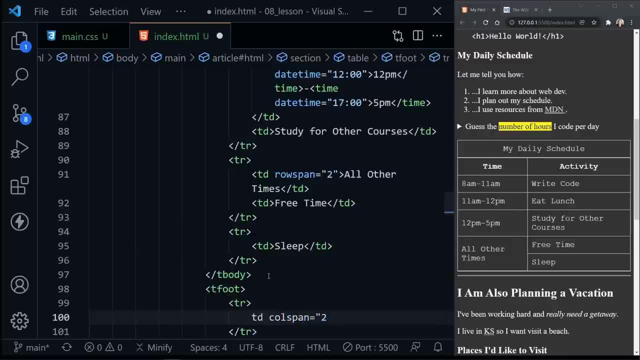 Column span equal to 2.. Well, I didn't get the data cell started. There we go. Now we go. Column span equal to 2.. And inside of here I'm just going to put a statement, But you could put something in the footer. 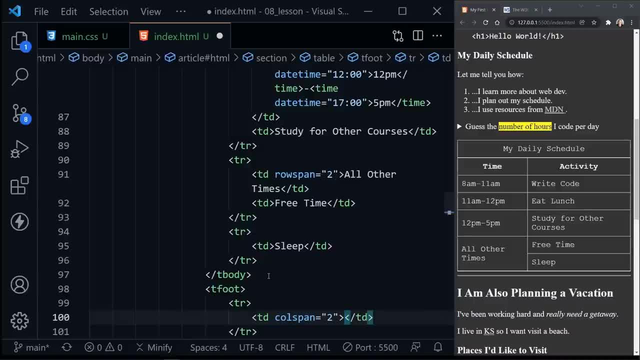 That say totals up all of the columns. If you had a ledger That was tracking account numbers Or expenses, Or say you had sports stats Or something like that Or anything else that would need totaled up, That would be a good place to put it. 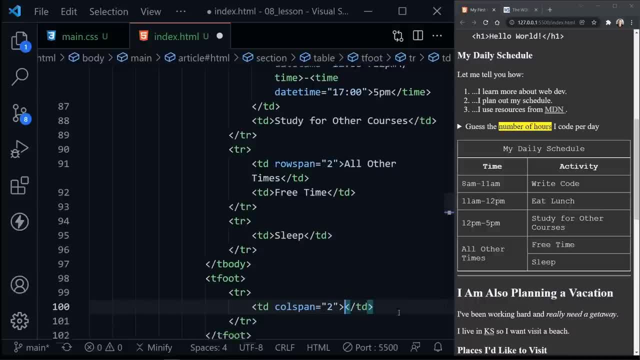 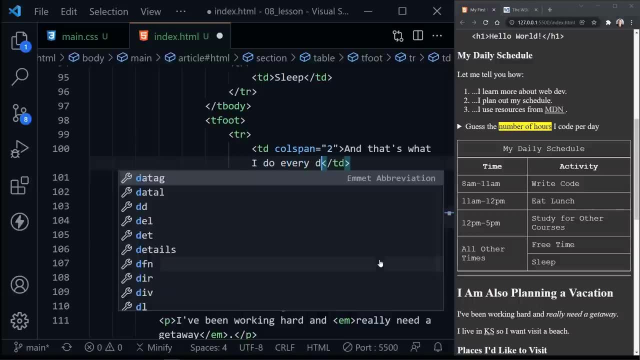 Is inside the footer. I'm just going to put a statement about our schedule. I'm going to scroll up before I add the statement, But here I'm just going to put- And that's what I do Every day- comma: Five days a week. 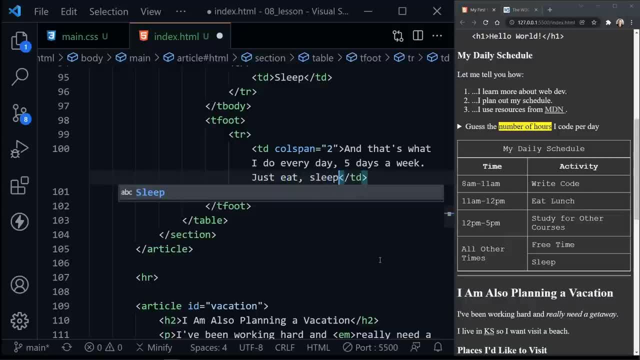 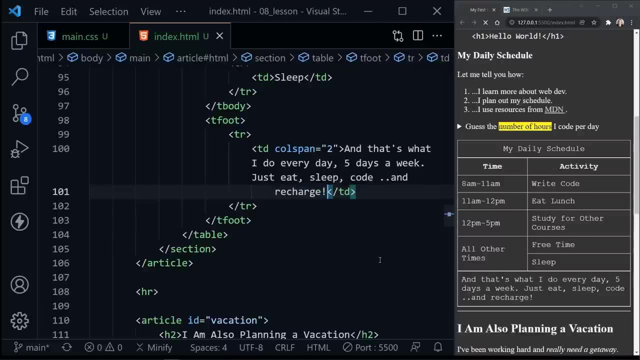 Period: Just eat, Sleep, Code And recharge And I'll save. And now we can see Both columns And we've clearly defined the semantics for our table now With a header, A body And a footer. Now another question you might think of: 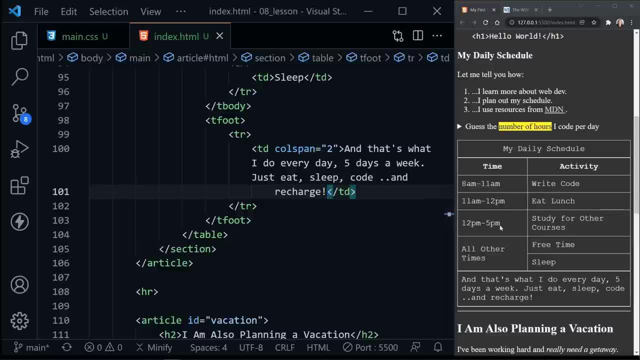 Is what if the row needs a header as well? It needs some definitions. So if we can have a heading for our column, What if we need another kind of official title For each row as well? Well, we can do that as well. 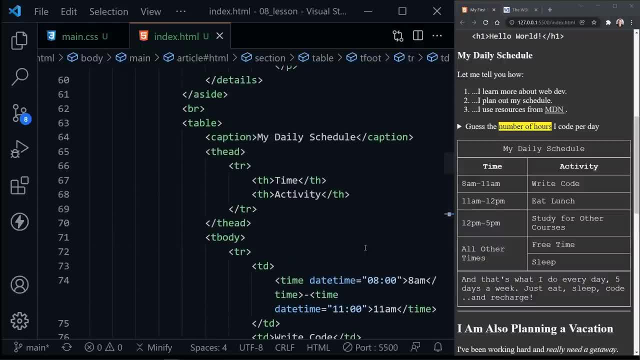 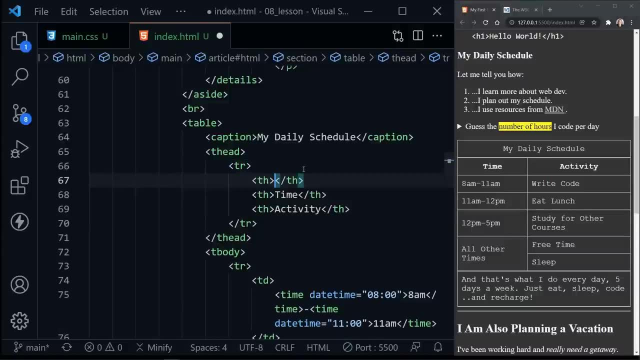 So let's scroll up here to the top And in our header We'll need to put an empty Or an empty cell, And we can do that. We'll just add another th And inside of here we need to put Ampersand mbsp with a semicolon. 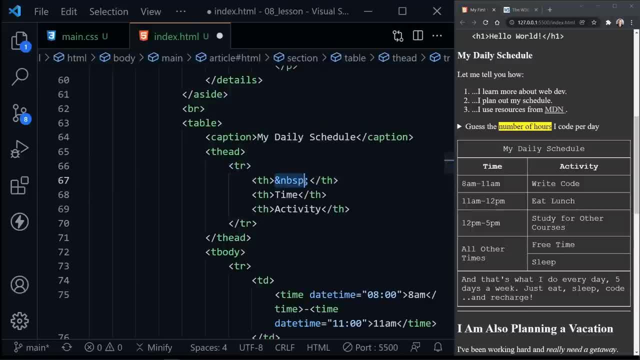 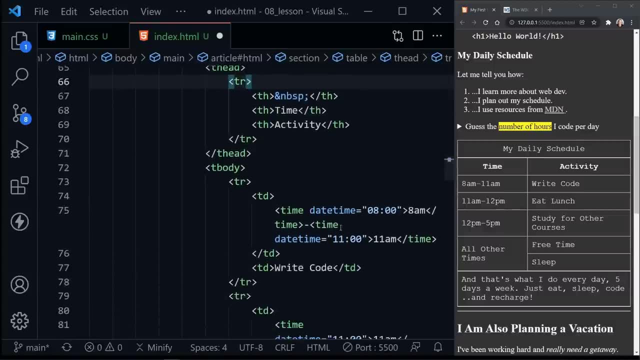 This is an html entity, If you remember when we covered html entities In a past lesson- And that just puts a little small space Inside of the cell. Now that we've added that, We can add headings to each of the other rows. 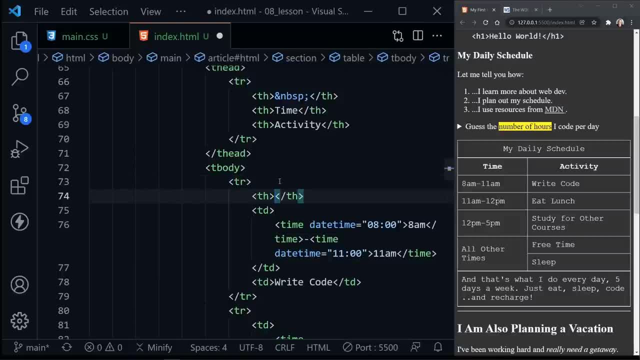 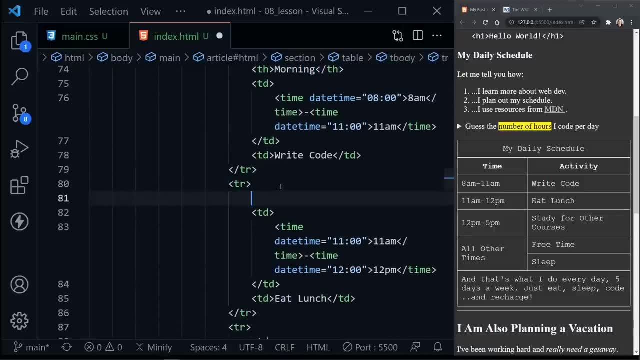 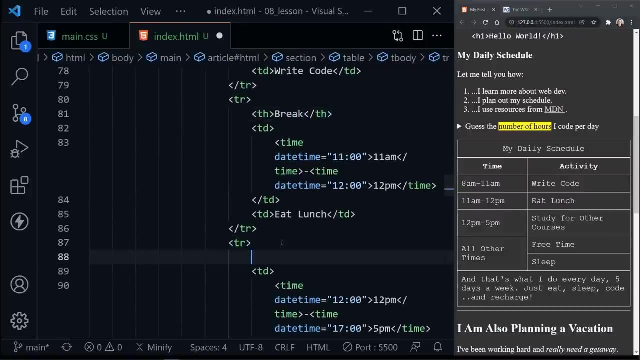 So we'll have a th here For the first row And I'm going to put Morning, And then in the next row We'll add another th And I'm going to put Break, And in the next row, Th. 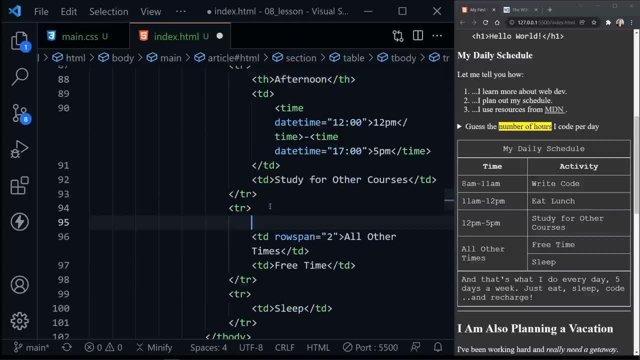 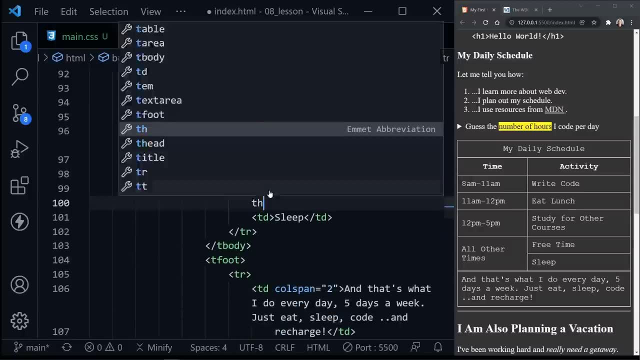 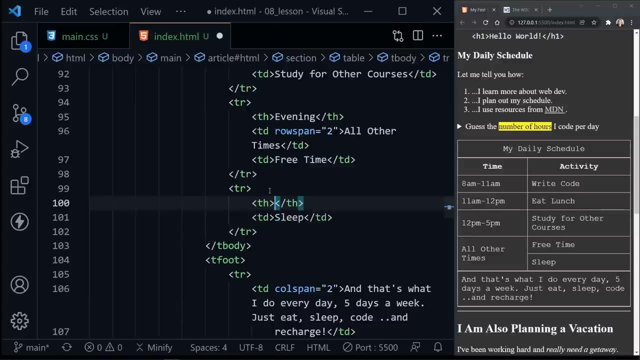 And I'm going to put afternoon. Next row Th And this is evening, And in the final row- Well, I guess not the final row, That would be the footer, But this would be the final row And I'm going to put. 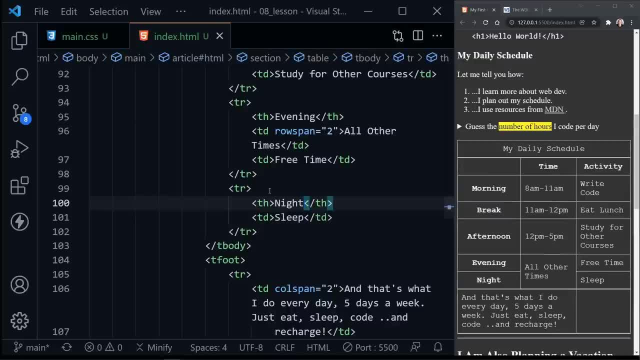 Night. So if we save this, We can really see how our table has changed. But notice, We didn't change the call span yet for the footer, So we've got an empty square here as well. Here's the empty square we defined. 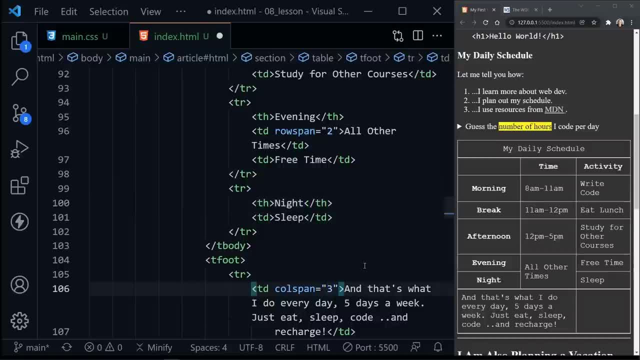 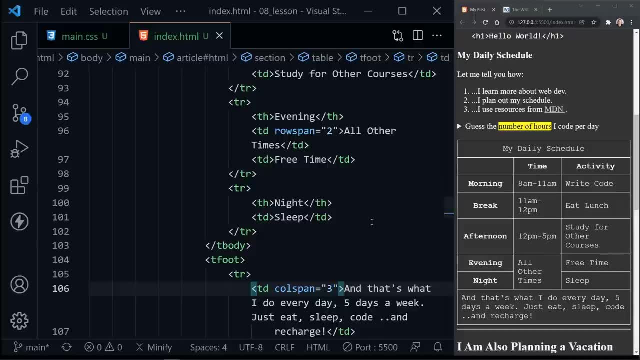 But we didn't plan on this. So we better change our call span for the footer To three, Because we now have three columns And if we save That looks much more like it. So if we go to row span And we came down to this final row, 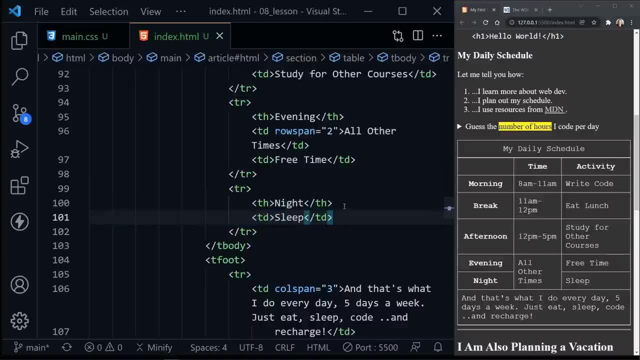 And we only added a first And a third column. We didn't have to specify That this was the first And this was the third. It automatically knew that Because the second column in the row above Is the one that had the row span of two. 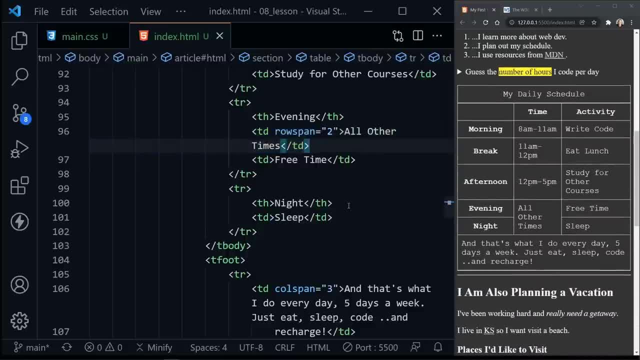 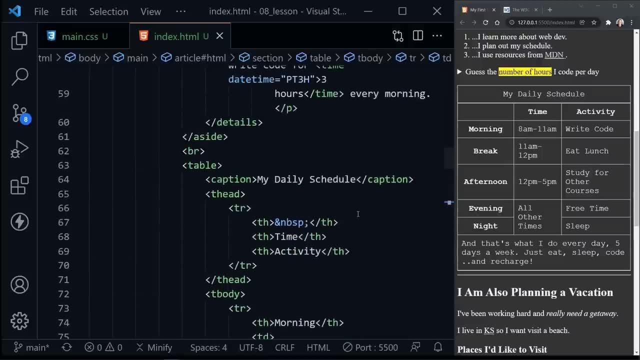 Now our page is looking pretty good over here As far as the table goes, But we need to add just a little bit more for semantics And we need to go back And start at the header. So I'll scroll back up And here we are. 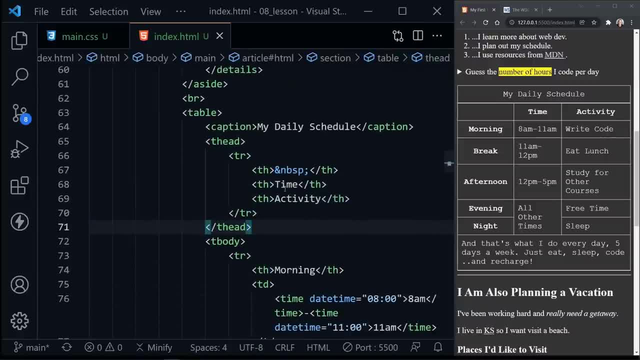 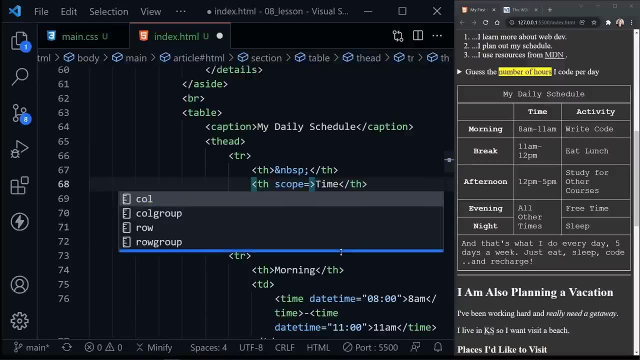 In the T head area of the table And for each heading that we have on the page- Each th except this one That has a space in it- We need to provide a scope And that says how it relates to the table. So this would be. 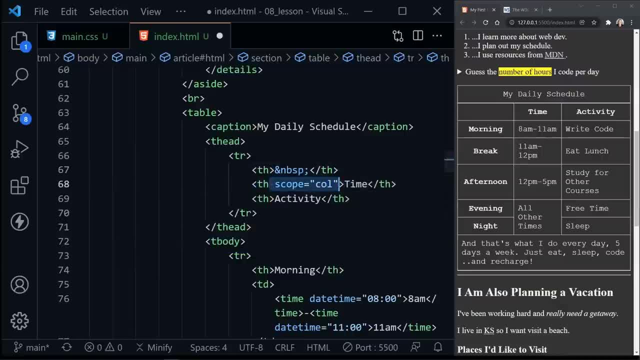 Scope equals to call, Which stands for column, And I'm just going to copy that Because we need to add that to the next one. And so time and activity both apply to the columns. So, as you might guess, When we get down to the next part in the body, 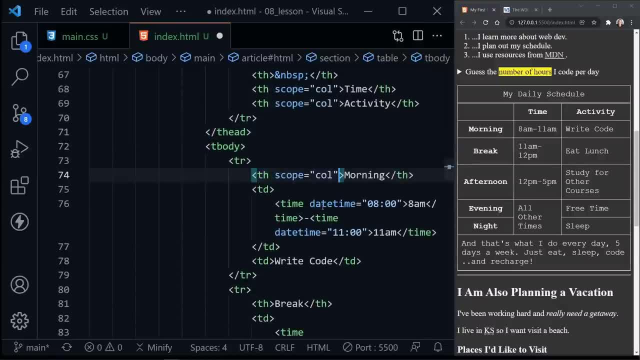 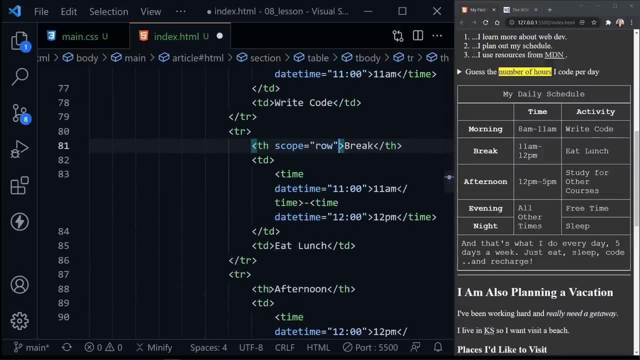 Where we get to the row headings. I can paste this in, But I need to change column To row And I'll copy this And we need to apply this to each one of the row headings. So now At break. And then we had 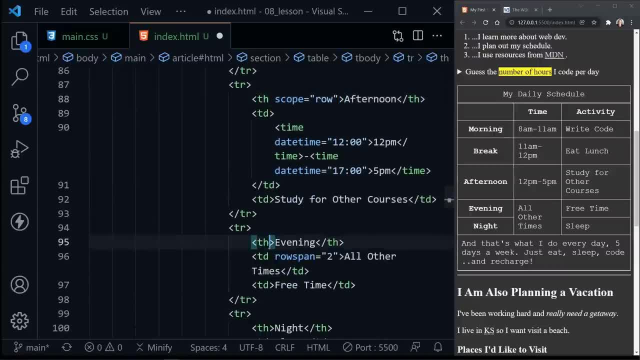 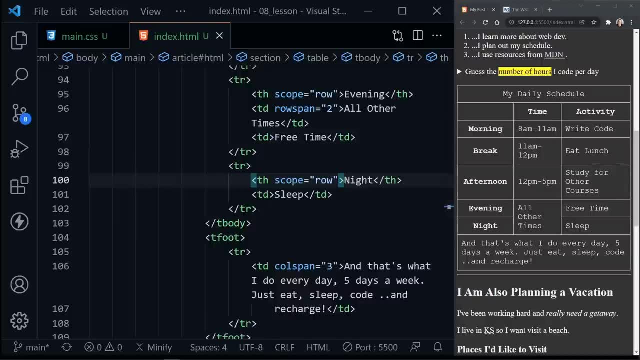 Afternoon, Evening And finally Night. And if we save that, Don't change the look On the page, But we have really helped assistive technology Navigate our table. Now this is the easier way to do that with scope. 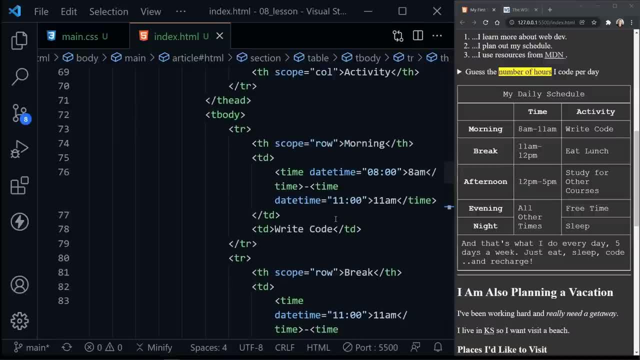 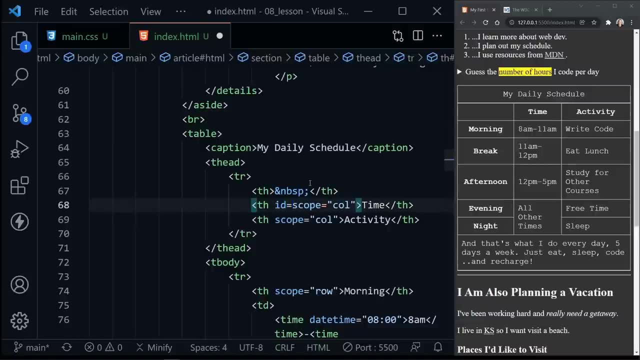 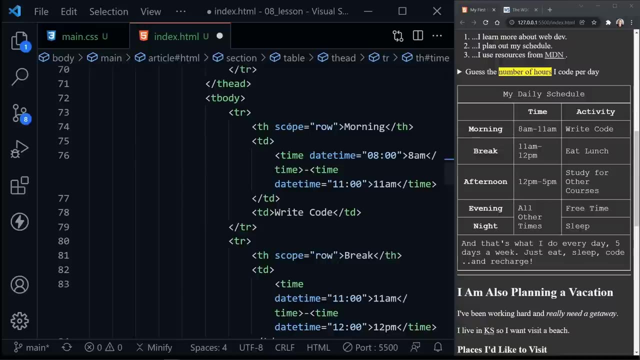 However, You may see that accomplished in another way, And that is providing an ID For each header. So if we had an ID And set that equal to time, And then we had an ID, Let's say in this row Or this row up here with morning. 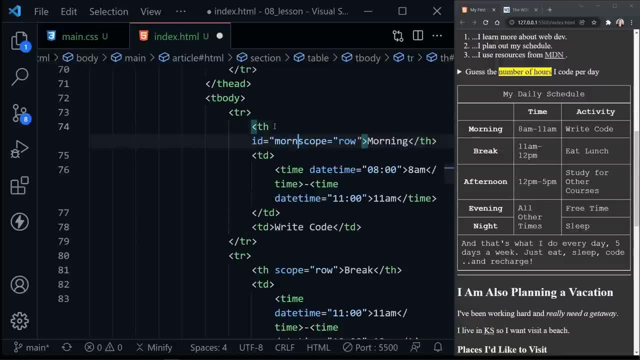 And we set it equal to morning, Then In the TD We would have to give the Headers attribute And specify both, So we would say time And morning. I find it much easier to just provide the scope Instead of IDs. 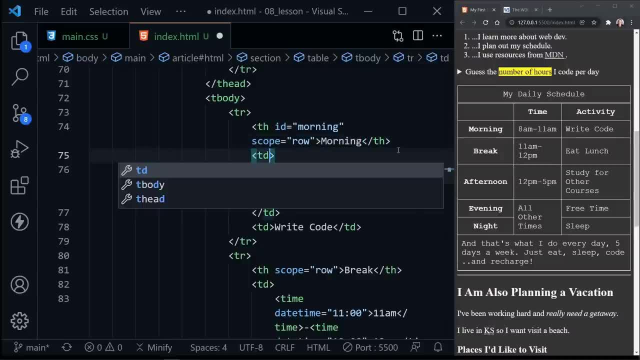 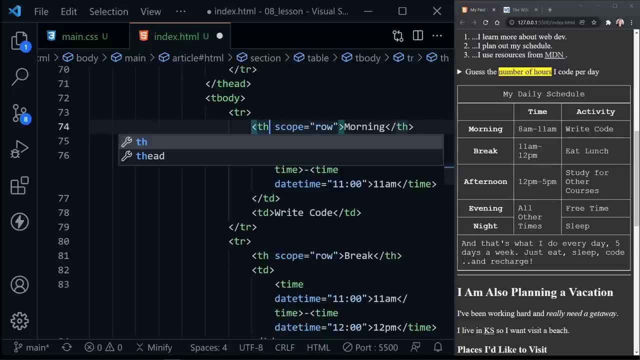 And then having to add a headers attribute To each data cell as well. So we'll just leave it at that. I'll go ahead and remove these examples That gave the IDs And we'll stick with scope Up above here. So there we go. 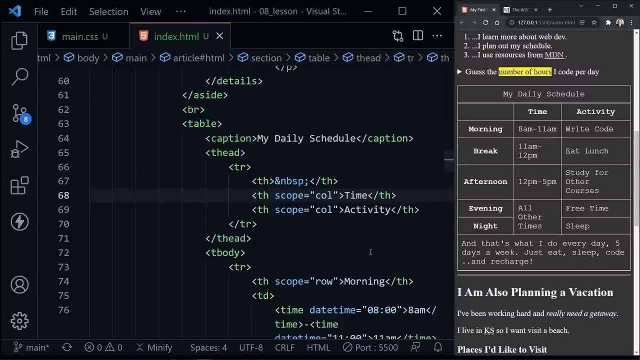 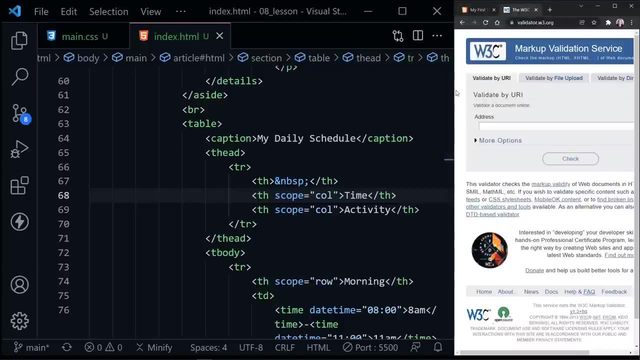 I just wanted to quickly discuss that, That there is another way to do it. Now that we've completed adding the semantics to our page And we're finished with our table, Let's validate our code. I'm going to go to validatorw3.org. 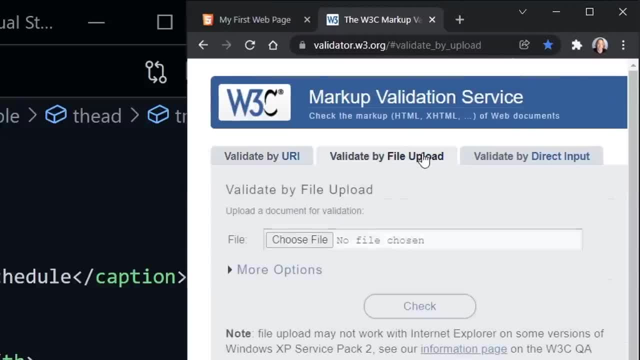 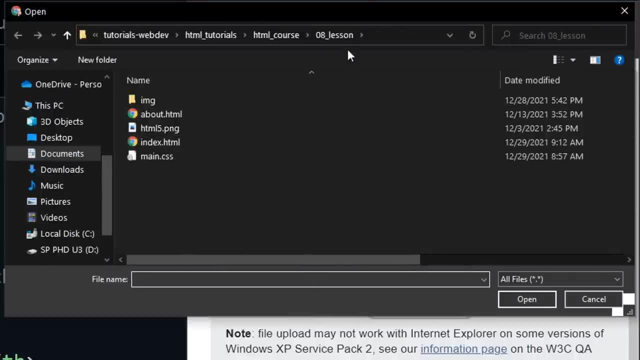 I'm going to drag the page over just a little bit. Click file Upload And now, when you click choose file, Make sure you're grabbing the correct file, That you're in the correct folder. I'm in the 08 lesson here. 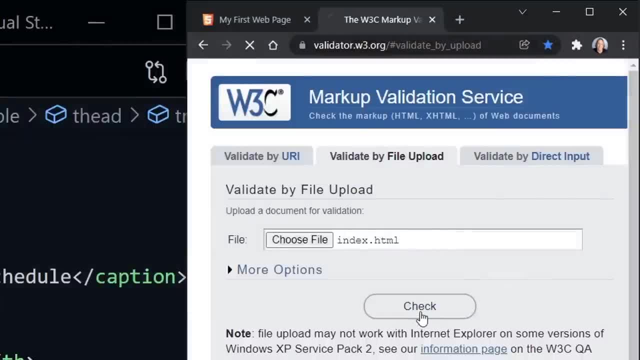 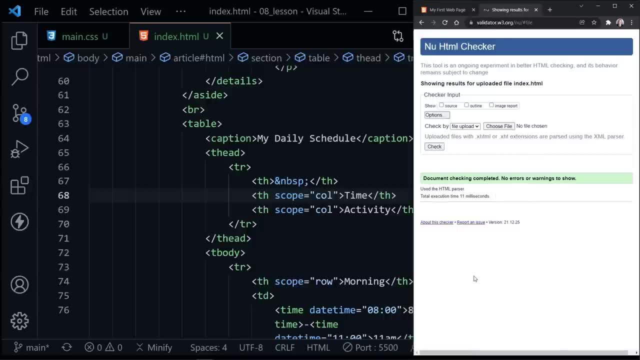 This is the folder that I want And I choose the index HTML And click check And document checking completed: No errors or warnings to show. If you have any errors, It should show down here And tell you which line they're on. 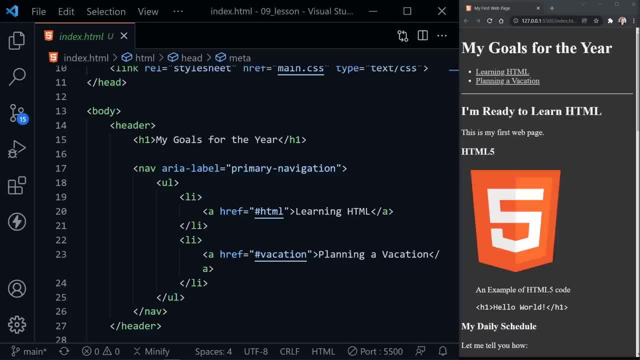 And give you some information about correcting those. So far, the HTML we have created Has resulted in one way: communication. But in this lesson We're going to add a form to our HTML page Which will allow users to send information back to us. 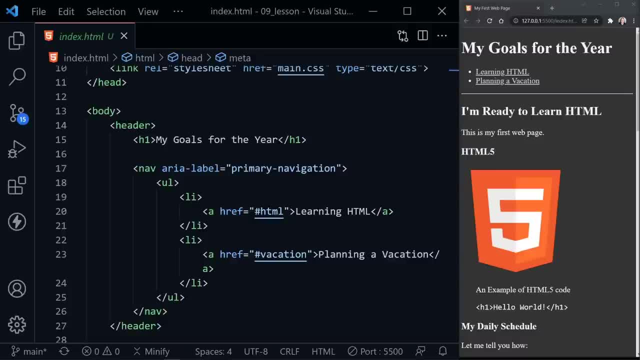 And that way That makes our HTML interactive. I've got Visual Studio Code open here on the left With the starter code for the lesson, And on the right We're displaying that starter code in the Chrome browser And I'm using the live server extension. 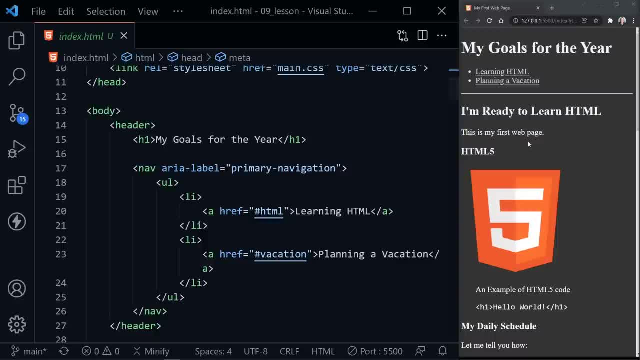 To do that. Live server also immediately updates the browser With any changes we make in the code. Adding a form to a web page Allows us to gather information from our users And, more specifically, It allows our users to send us information. 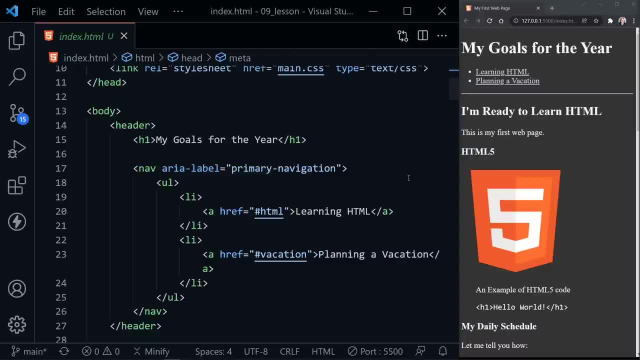 If they choose to. This is exemplified Throughout the web With contact forms, So let's add one to our page. Notice I'm near the top of the page, Around line 13. Where the body element starts, And if we come down just a little ways, 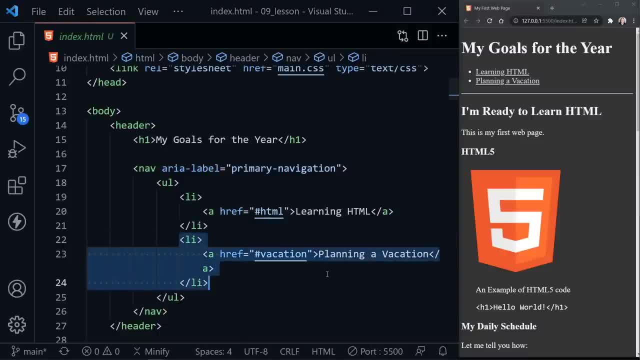 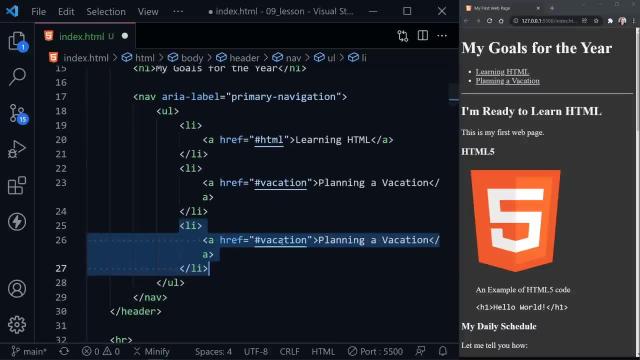 We find our nav element on line 17.. Now here I'm going to highlight the last list item In our unordered list That has planning a vacation, And I'm going to press shift, alt and the down arrow To just make a copy of that below. 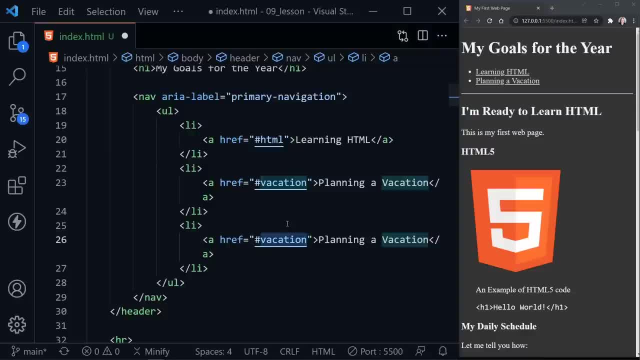 Here I'm going to add another anchor And remember This is the page I'm just going to change vacation to contact In our new link And I'll highlight the planning a vacation And change that to contact me. So now we have made a link. 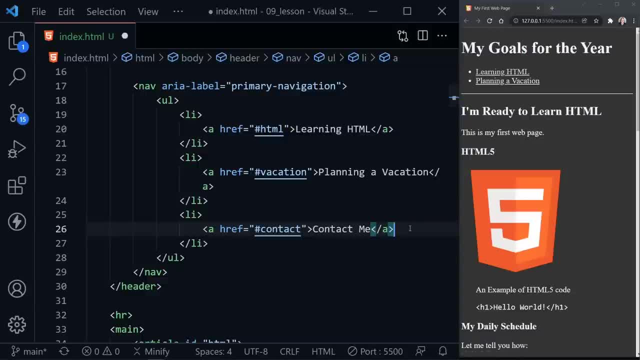 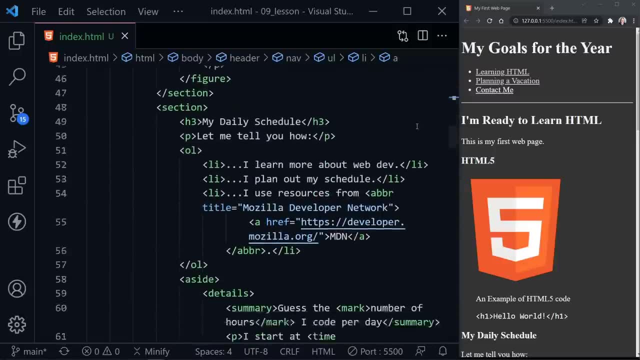 That should show up here by our learning HTML And planning a vacation. So I'm going to press control s to save And there is our new link. And now we'll want to scroll in visual studio code All the way to the bottom. 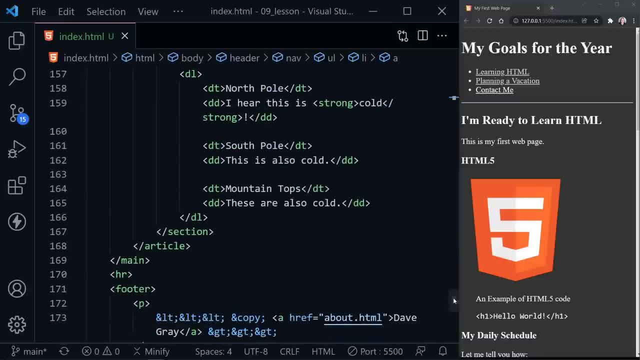 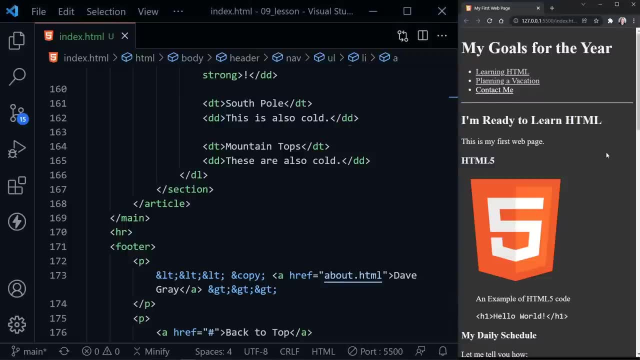 And maybe I can just grab the bar here And go a little faster. So we have our last article That has the places we do not want to visit on vacation, And we can see that in the browser as well If I scroll that down. 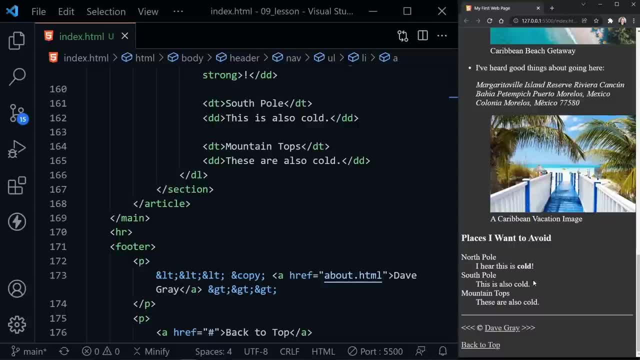 It may take just a second to get there. But here we are, Places I want to avoid. We want to add our contact form Underneath this, But above the footer as well. So underneath this last article, But before the main element. closing tag. 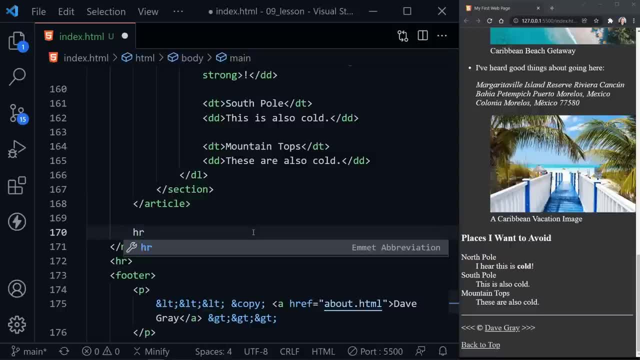 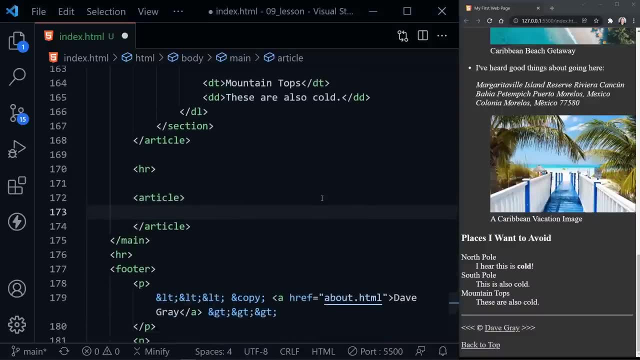 So I'm on line 170 right now, Going to add another HR, A horizontal rule divider, And from there We can start with our article element. I'm going to scroll up just a little To get this closer to the center of the page. 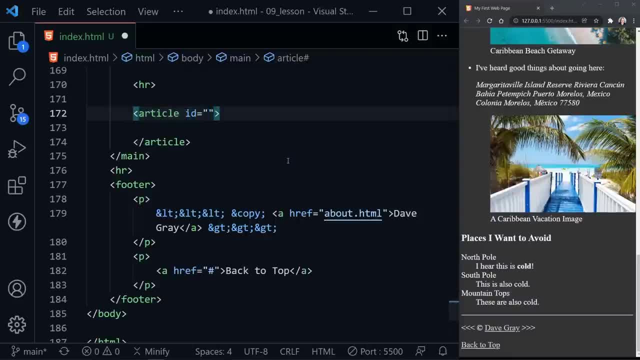 Or a little higher, And then we're going to go ahead and add that ID To the article element, And here we'll need this to match what we put in the anchor link above. So it needs to say contact. From there, let's go ahead and add our header. 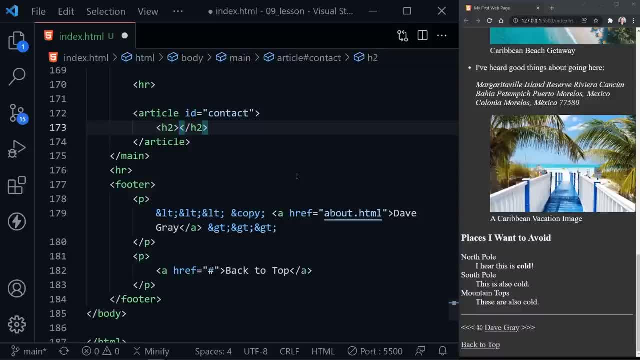 For the heading hierarchy, And this should be an H2.. As it's a new article area of our page, So it matches the other article areas And here I'll put Contact me for the title. Now let's put a paragraph. 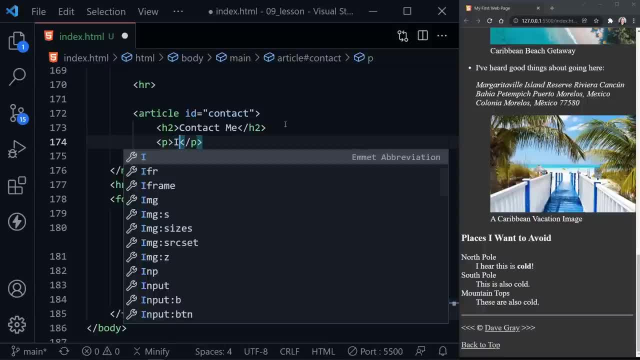 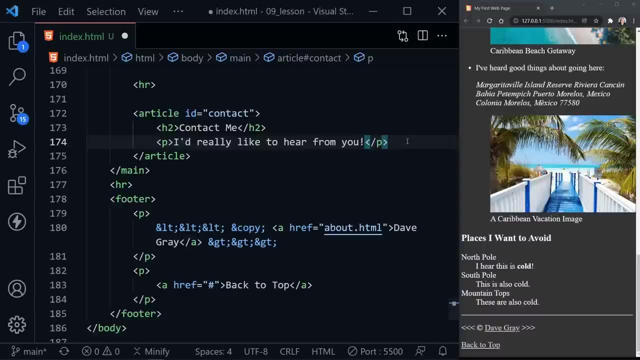 With a little description underneath. And so in the paragraph I'll just put: I'd really Like to hear from you. There we go, And now we have a title, And we have a bit of a description, And now we're ready to add. 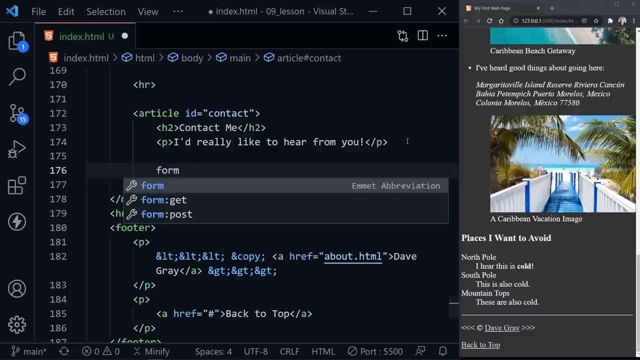 Our form to the article. So let's start out by typing form And pressing tab Notice. an action attribute is automatically added to the form tag And what we want to put here Is where we're sending the information. Usually, this would be to our own server. 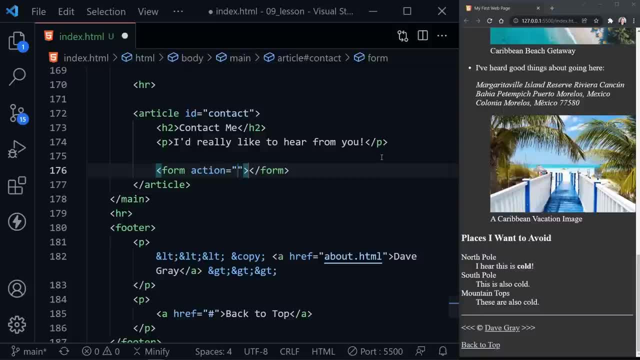 But for this tutorial And just to demonstrate what a form does, We're going to send it to a website That will display The information that we have sent with the form. So let's type HTTPS colon, slash, slash. HTTP bin. 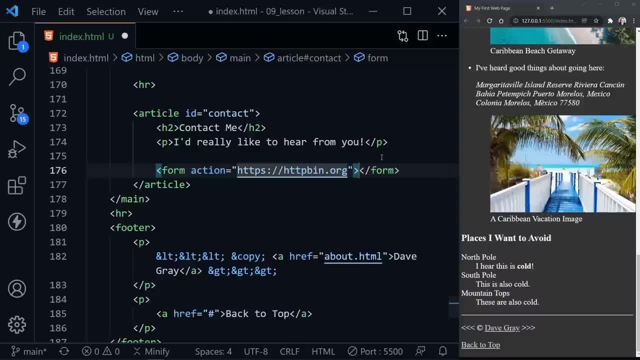 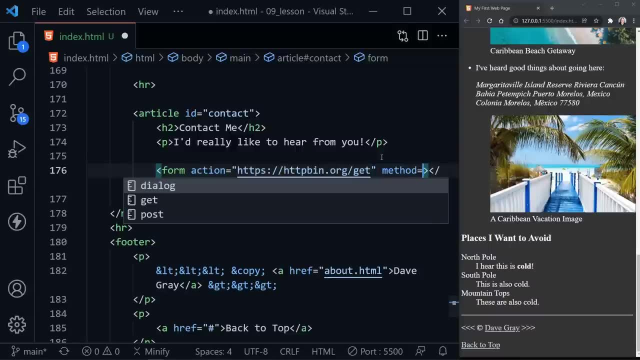 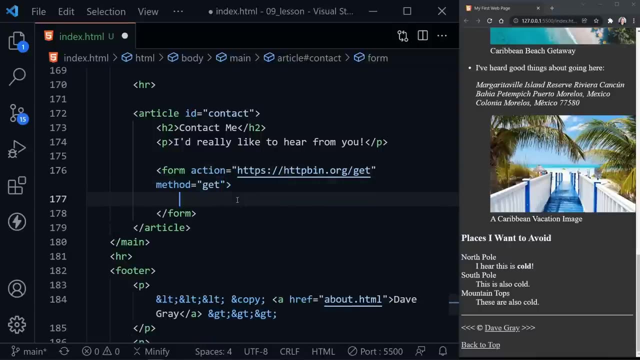 B-I-N Dot org. And then slash git. Now that last part, slash git, Refers to the method we're going to use, The attribute that we need to add to our form. So method equals git. Likewise, Method is often post as well. 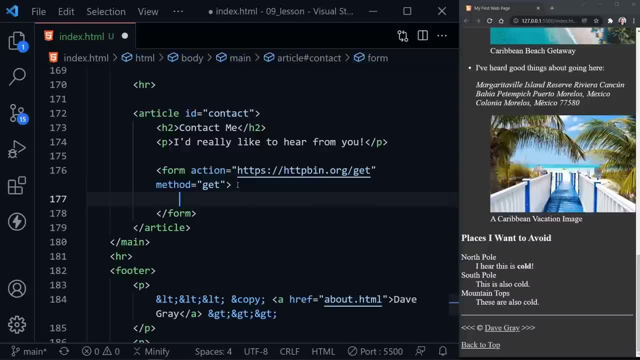 There can be other values And we'll see the difference, Because we will try both of those out before we're finished. Now, the contents of forms Are mostly labels and inputs, And every input should have a label. So let's start. 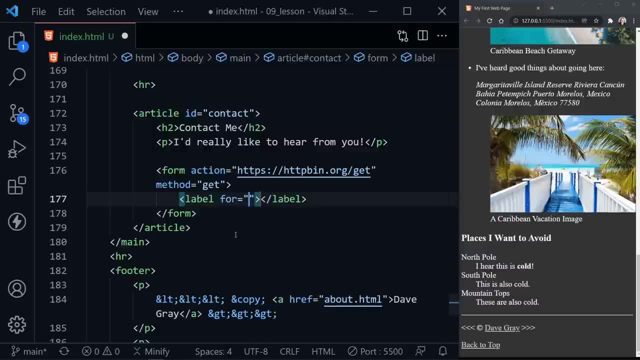 With a label element And notice it instantly has a for attribute. That for attribute value Should match the ID value Of the input. So here we're going to put first name, Because that's what we expect, And then for the label. 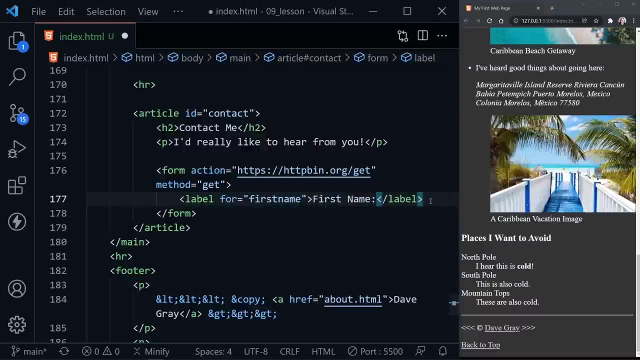 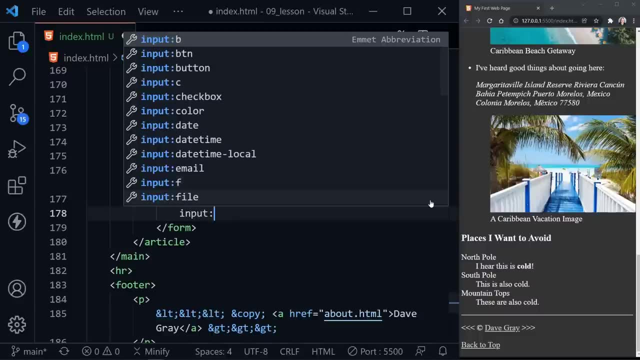 This is the part that will show on the page. We also want to put first name And then I'll put a colon After that. let's go ahead and create an input And you can also type a colon After the input And type T-E-X-T. 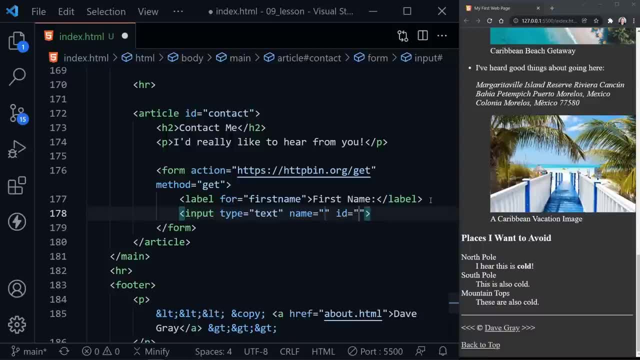 To get a text input And then press tab And notice we automatically have the type For the input filled out And now we have a name attribute And an ID attribute, And these you really want to match. So I'm going to put first name. 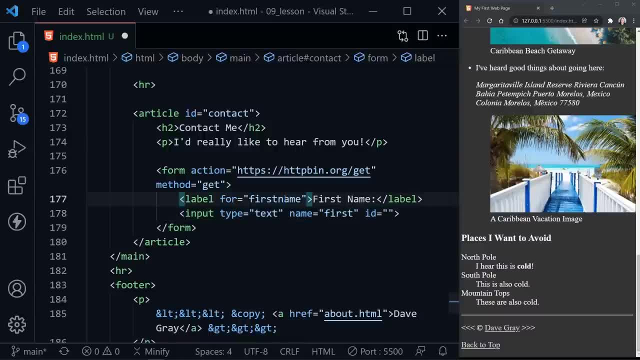 And I forgot to put camel case Here for the label, But I like to use that on these, So let's go first name. And by camel case that means the second word Has a capital, So first name with a capital, N. 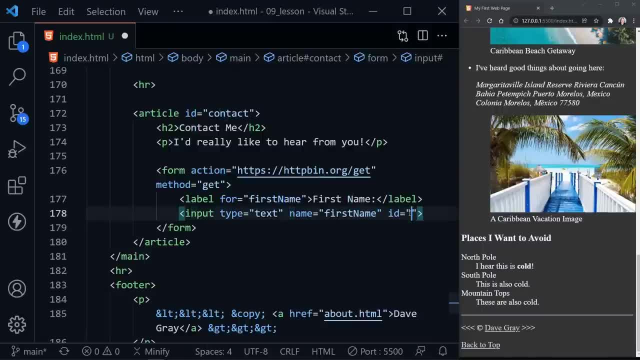 And then for the name value, We'll also put first name that matches, And let's do the same with the ID. Now, remember: the ID Absolutely needs to match The value of the for in the label. This name attribute, though, Is how it is identified. 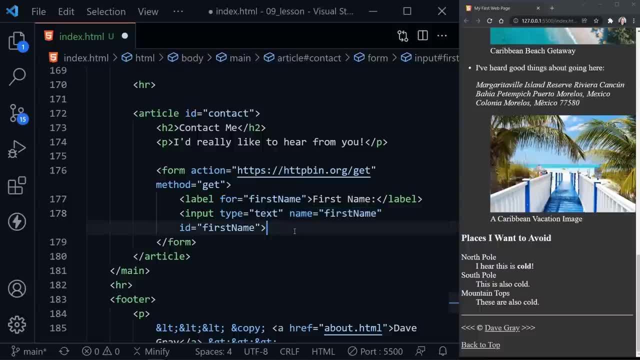 At the server level. So when we send this information onto the server, The information that is in this input Will be labeled with the value That we put in the name attribute. So let's go ahead and save this much And see what we get on our page. 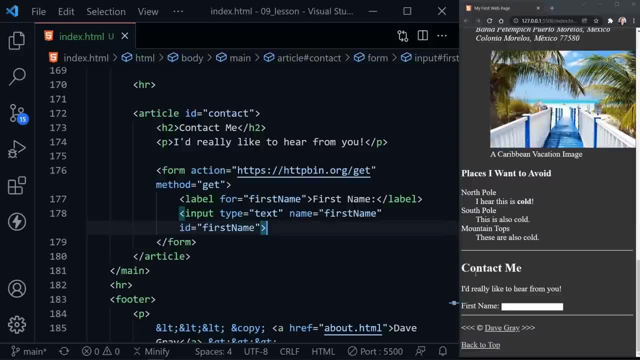 We can scroll down and look at our form. It's very basic right now, But you can see the title: Contact me, Let me hear from you, And then we have our first name label And our input Where the user can type information. 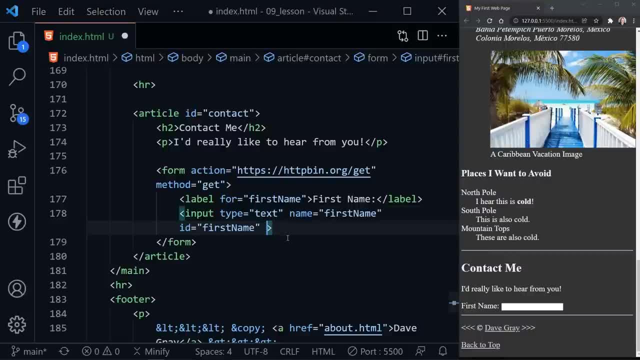 In this text input, But there are a few more attributes that we can add, So let's add one called a placeholder. Now, this lets us display text, But it's not the same as the value, Which would actually be what the user enters. 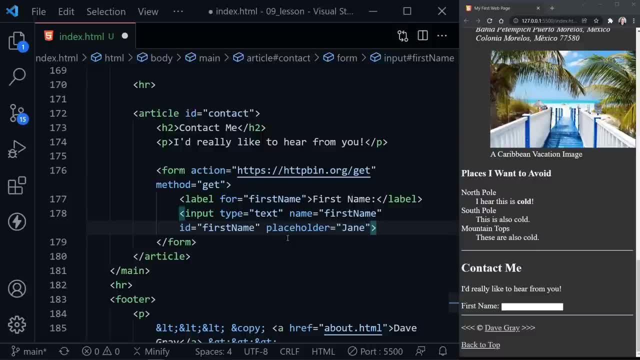 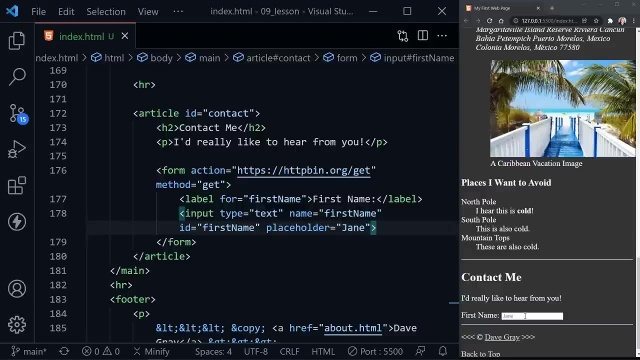 So this could just be an example. I'll type the name Jane And save, And now we see Jane in the text input, But it will not be sent with the form If we click in that input And then start to type. 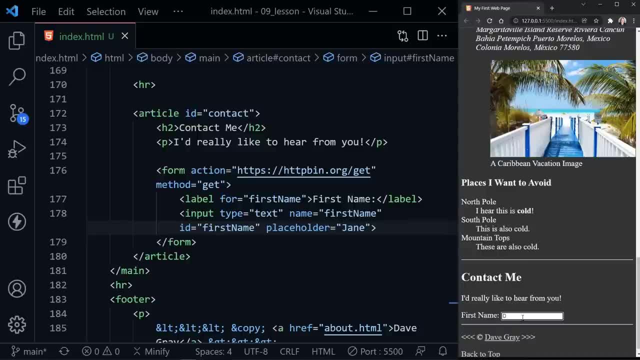 Jane disappears And now we have a value, An actual value, entered, But as soon as I delete the last letter, Jane will reappear. So placeholder is just exactly that: It is holding the place of whatever value will be put in So often times. 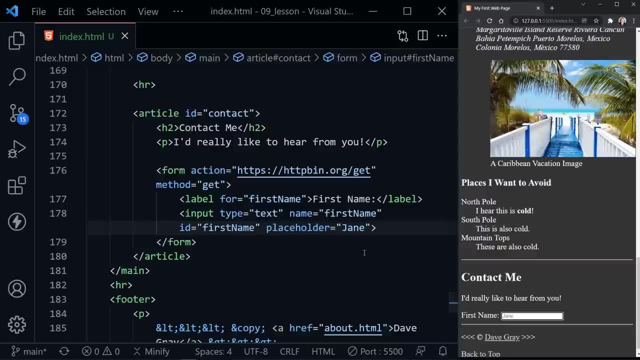 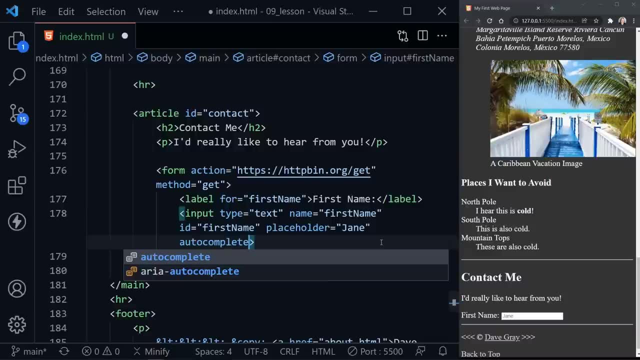 There is example data in there Just to show the user what is expected. We can also add another attribute Called autocomplete, And autocomplete Doesn't expect a yes or no Or true or false, Like others often do with attributes. As far as that goes, 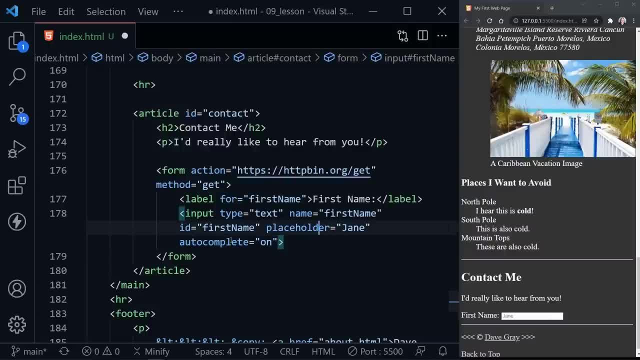 This is expecting an on or off, So we're going to turn the autocomplete on And that means It will remember other inputs That have been entered into this field And suggest those. So if we were to submit the form And then fill it out again later, 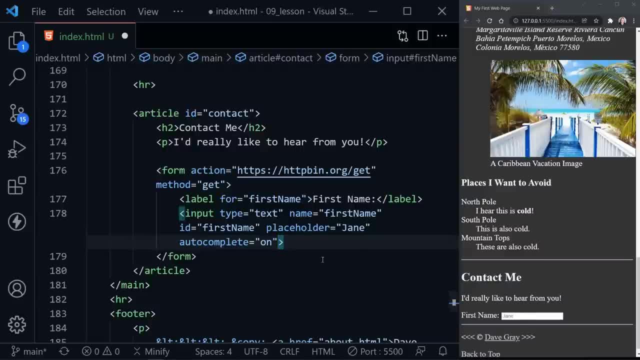 It might suggest What we previously put in. So that's a preference thing. So autocomplete on or off, Then we can put required, And this will require this field To have information from the user Before the form can be submitted. Now notice I said 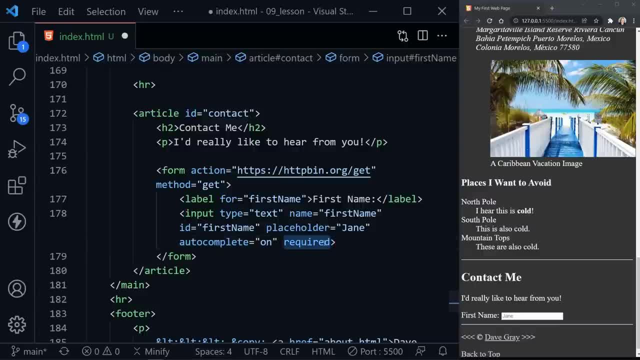 Autocomplete didn't use true or false Or yes or no, Required does. But we don't really have to set it equal to true like this. We can just say required, Because if we put required there It equals true. And then if we don't have required there, 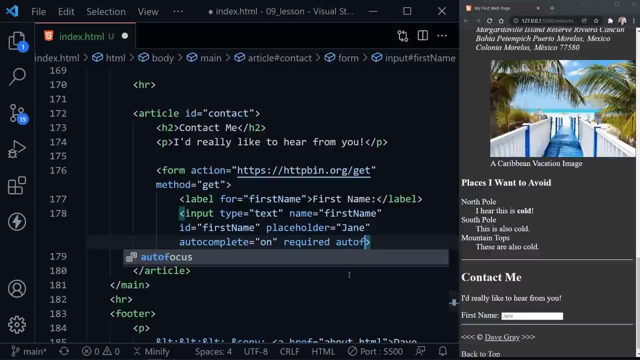 It's obviously false. So I'm going to give this: input Is autofocus. Now, only one element in the form Or on the page Can actually have autofocus, Because it can't focus on more than one at once. This will put the focus in that input. 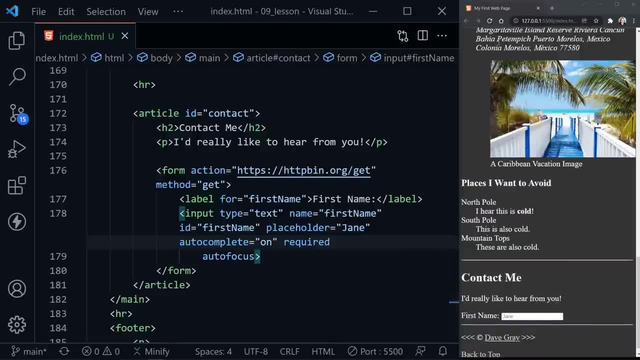 When the page loads. So I'm going to save And then, if we reload the page, We should see The flashing cursor here- There's focus in there- immediately When the page loads So we can start typing instantly. I'm going to leave the autofocus here. 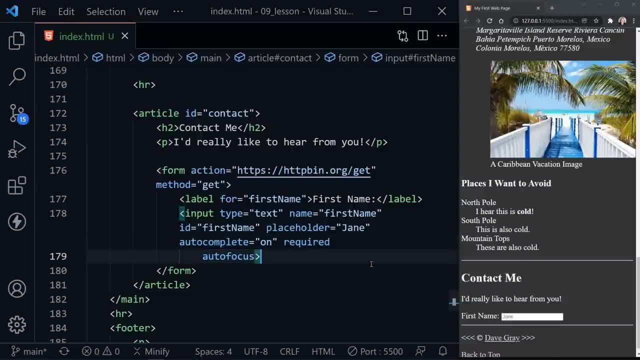 To have it in the source code for you For the lesson. However, with the contact us page Being at the bottom of the page, It may not be where you'd really want to have autofocus If you were creating a form. Okay, and that completes our first label. 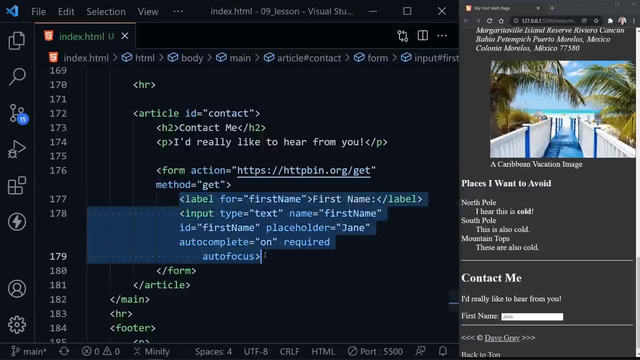 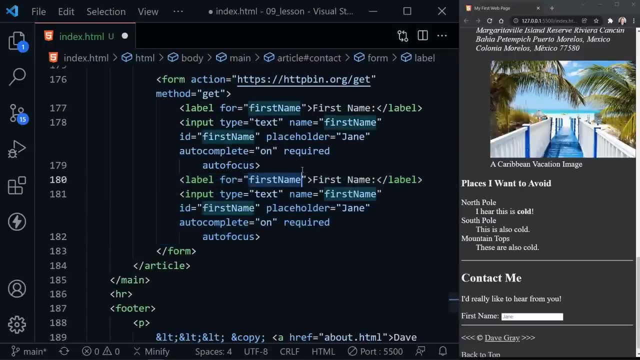 And input combination for our form. Now I'm going to highlight both of these And press shift, alt and the down arrow So I can copy this down, And I'm going to change first name. I'll press control D To highlight every instance of first name. 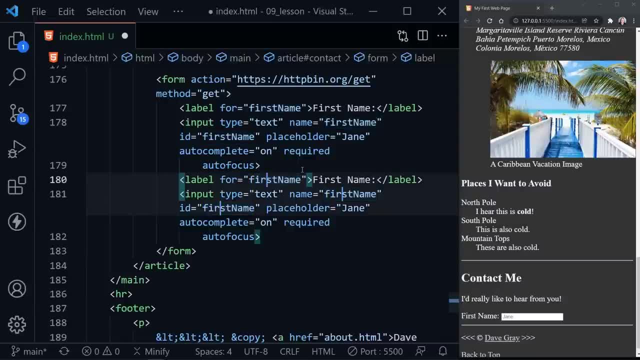 So we have three And then arrow to the front of it And then go three letters in And just switch it to last name, So we can change all of those at once Again. that's control D, And it will let you select more than one at a time. 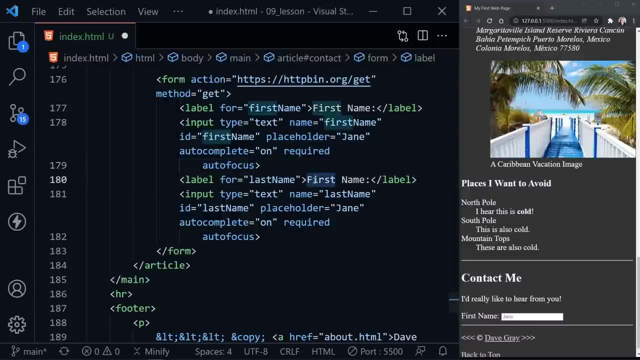 For each time you press control D. Okay, so now we have last name We need to change here. That didn't change this instance of it Because we had a space between it, So it was not the same as the others And we don't want to placeholder Jane for last name. 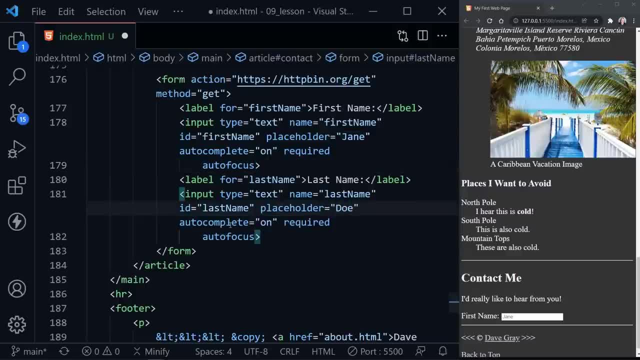 So we'll just put Doe And then auto complete on. I guess we did it for the other one. That's okay, But remember, only one element or one input Can have auto focus on a page, So we need to remove that. 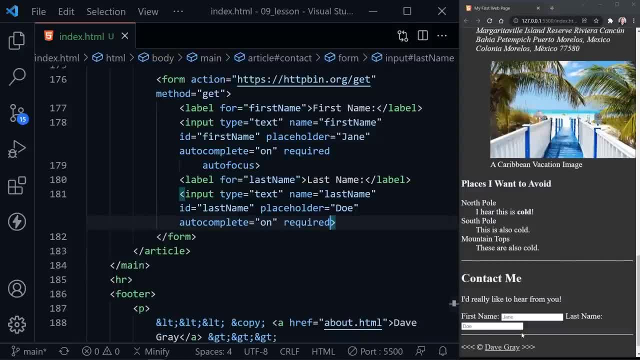 Now let's go ahead and save, And you can see. Our form has both inputs and labels. It doesn't look too great though, does it? They're just all running along one line And then wrapping to the next When it runs out of room. 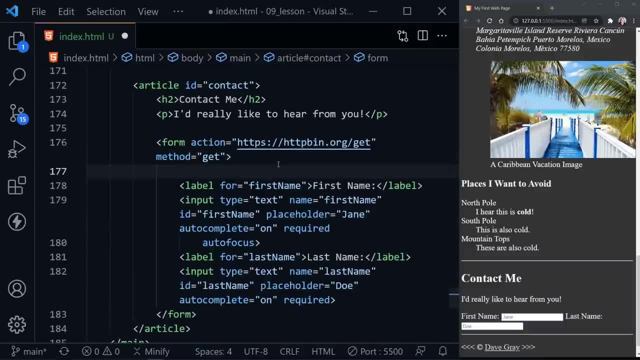 And with that problem We wrap our label and input In a block element That creates that line break. So let's use a paragraph. That once again, Better than using a div. A paragraph has just a little more meaning Than an empty div. 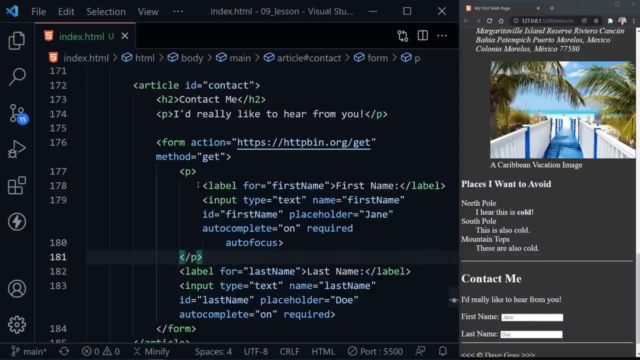 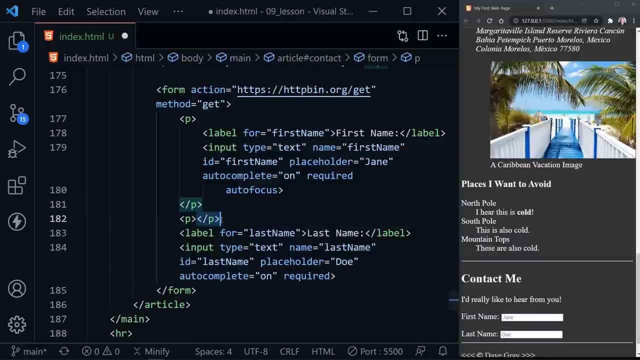 Although almost the same in this instance, And you will see some use divs here Instead of paragraphs, So we've got a paragraph there. Now let's wrap the label and input For the last name In another paragraph And save. 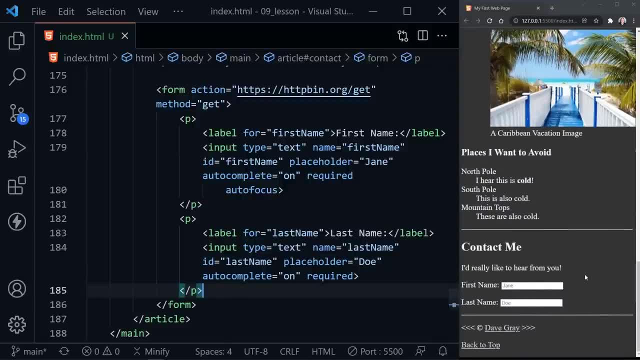 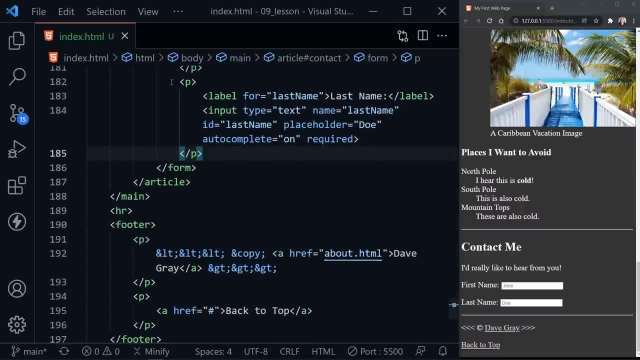 And now let's look at our form. It has a little more space here. This looks a little bit better than before. Okay, let's keep adding to our form. I'm going to scroll up again. We'll get the last name towards the top of the page. 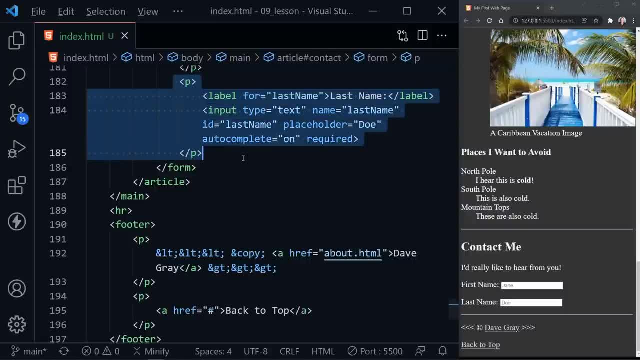 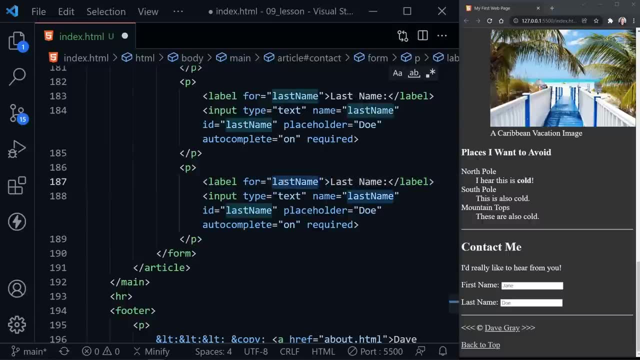 I'll highlight the paragraph And everything inside of it And shift alt and the down arrow once again, And now we'll change last name To password. So control D to select Every instance of last name again, And I'm going to type password. 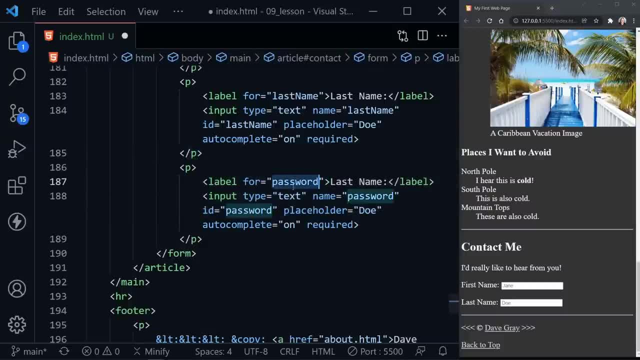 So now we've got A for attribute in the label And then the name and the ID Are password. So let's change our last name here To a password. Value for label And type text also needs to be changed To password. 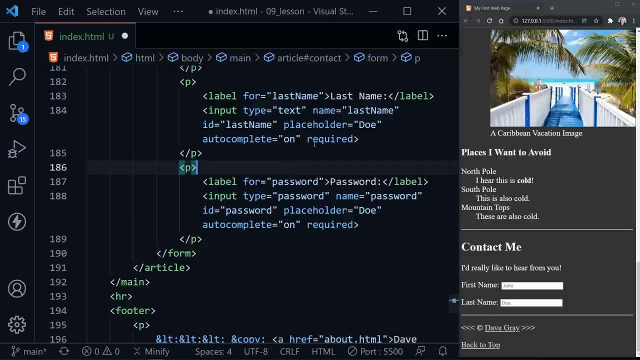 So this is a different type of input Than we used for first name and last name. For placeholder, I'm going to put your secret, And auto complete Is not supported on a password, So we can remove that, But we do want to go ahead. 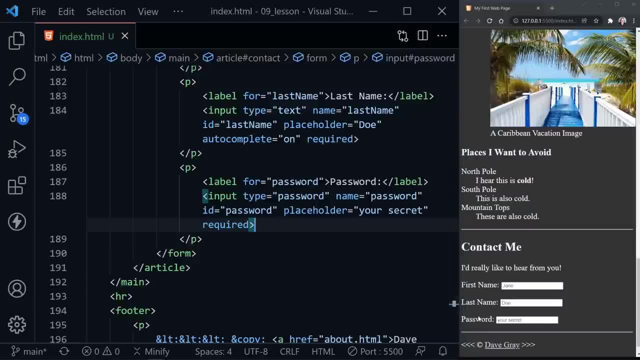 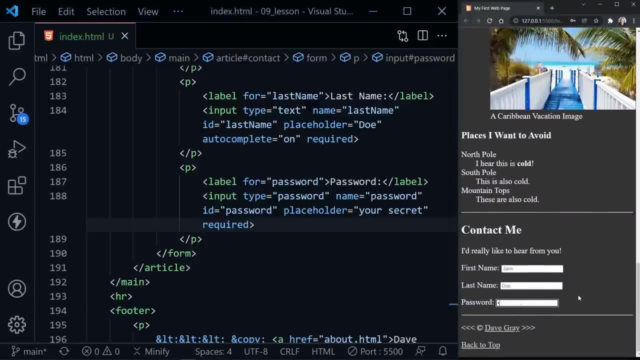 And require a password. So now let's save And we see our new input down here That says password And that's your secret for a placeholder. But now, when I start to type into this input, Notice it has little dots Instead of the text. 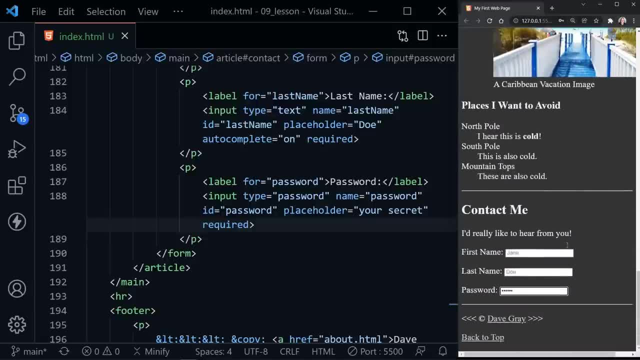 And actually let me see if I can just Enlarge this a little bit So we can see these better. There we go. So now we have our input And that is what a password field does, So it doesn't let the user see. 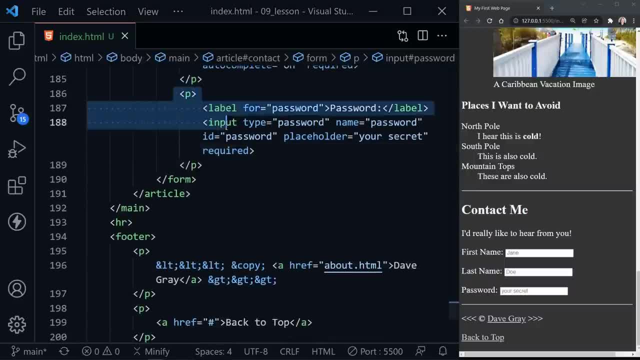 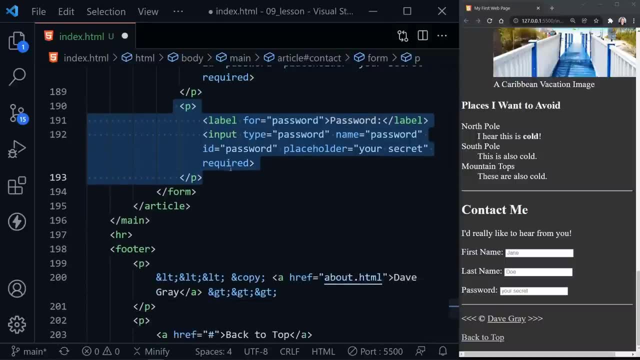 What is being typed in. Okay, let's scroll up again And I will highlight the last paragraph With the label and input Shift, alt and the down arrow to copy. And now we're going to change this one To something different. Let's say: this is a phone number. 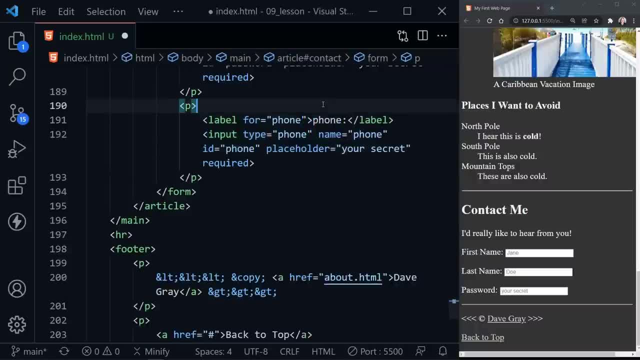 So I'll once again select. Well, I just wanted the three, But it's going to change five now Because we had password in there so many times, So I'm going to add a capital P. This is not a type phone, though. 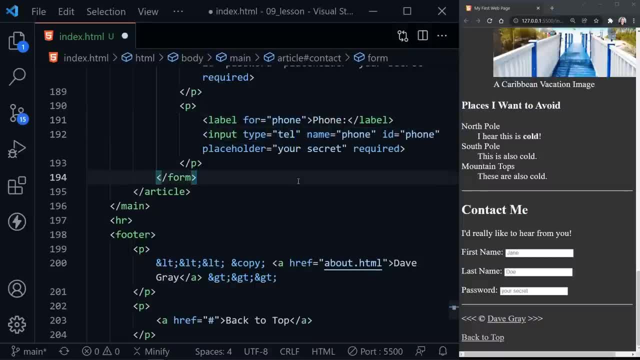 That doesn't exist. However, type tell does, Which is short for telephone. So we'll leave the for attribute on the label, The name attribute And the ID attribute values All to phone, all lower case For placeholder. let's give an example here. 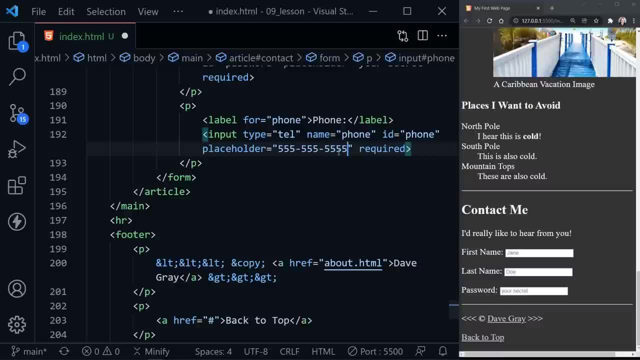 And I'm going to put 555-555-5555.. And if we wanted to leave it required, We could. But we can add another attribute here too, And that is- And I'm going to press enter Just to come down a line for this- 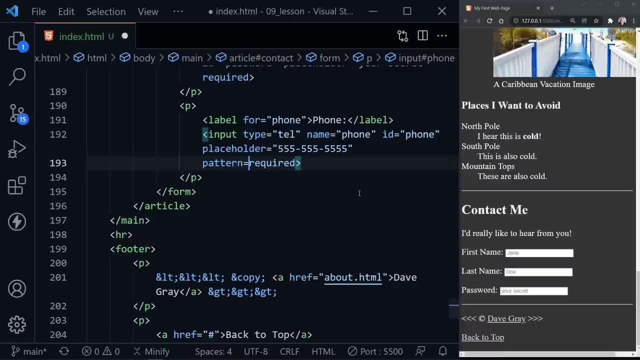 It is the pattern attribute. Now, the pattern attribute Supports regular expression patterns, And that's almost like Learning another programming language. If you're not familiar, I'll at least show you this one That will give a pattern for a phone number. 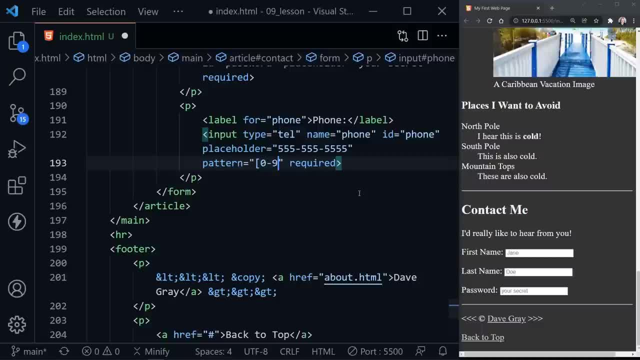 Like we have shown in the placeholder. So we're saying Zero to nine, So this must only be numerical digits, And then we'll use a curly brace To put the number three, So it should be three numerical digits. Then we'll put the dash. 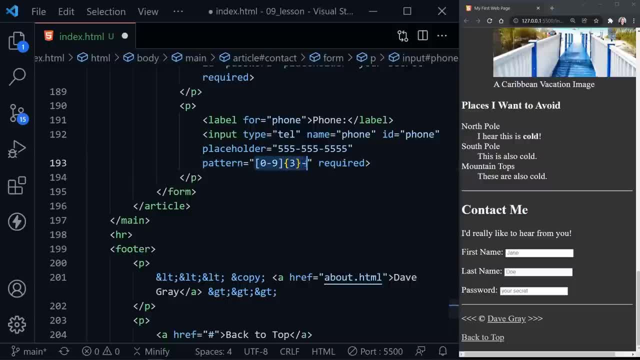 And now I'm going to put the same pattern again, Because we had three more And another dash, And then finally, It's going to be the same pattern again, Because we want all numbers And only numbers. But this last one should be four. 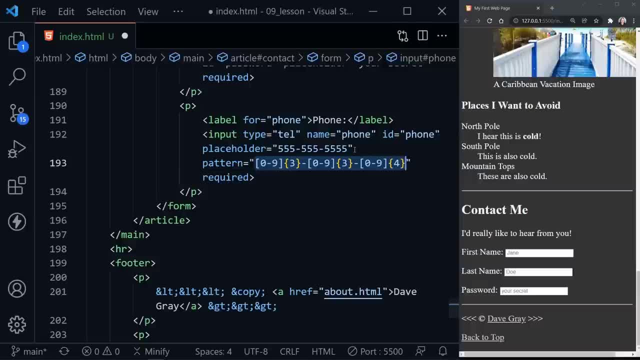 And so that is a regular expression pattern That would match what you see here. For the example. Why else would we put the type tell Instead of type text Or type number? Well, type number has a little different display, And it actually provides arrows. 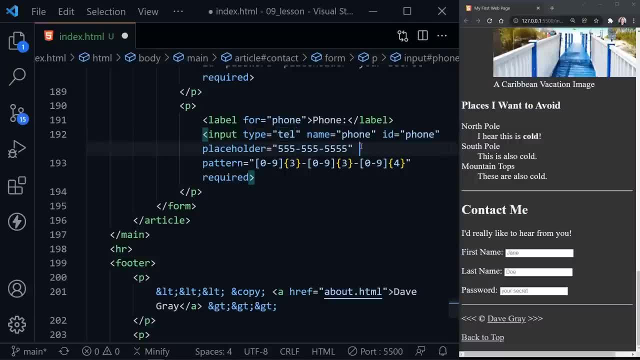 That would have you click up and down And we don't want that. But type tell, also on mobile devices, Should bring up a numeric keypad on the screen Instead of an alphanumeric, Essentially with letters. It should just bring up what you would say. 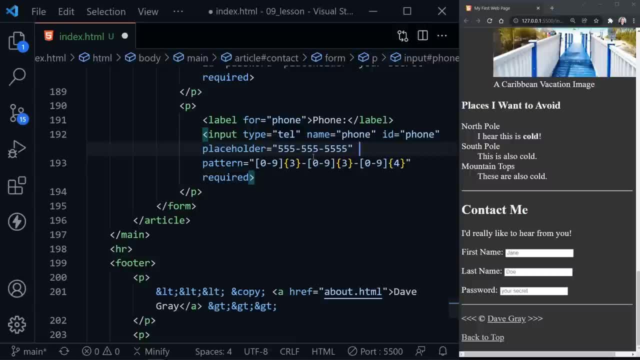 Dial for a phone number, And now that I'm thinking about that, The hyphen might not be available. So let's just make it simpler And go with all numbers here And remove those hyphens from our pattern too, So it can still match. 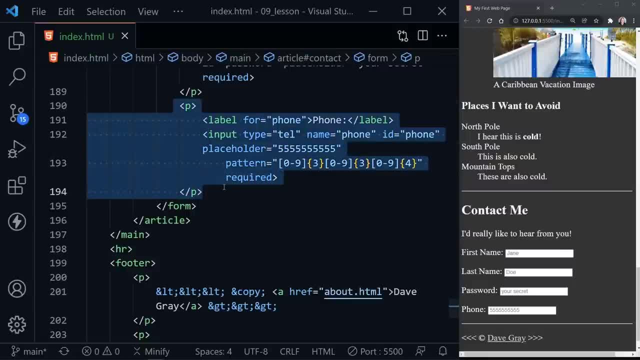 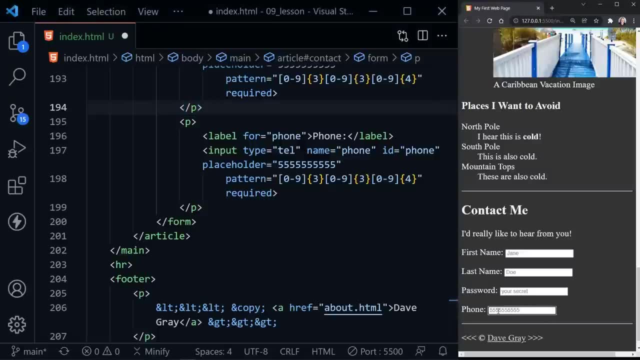 So let's save this, And now I'll go ahead and copy this down, But we'll look at an example of a number input So we can definitely see the difference. Right now we see the phone input And it's input type tell. 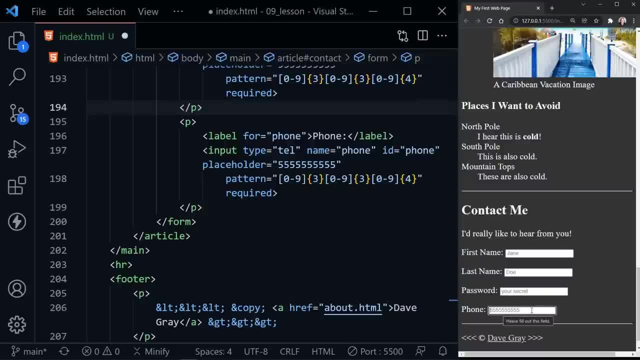 And really we don't see anything Any different here Besides that, Because it still allows you to type a hyphen Or an underscore That you want in this input, But we're just expecting numbers And it will have to match this pattern. 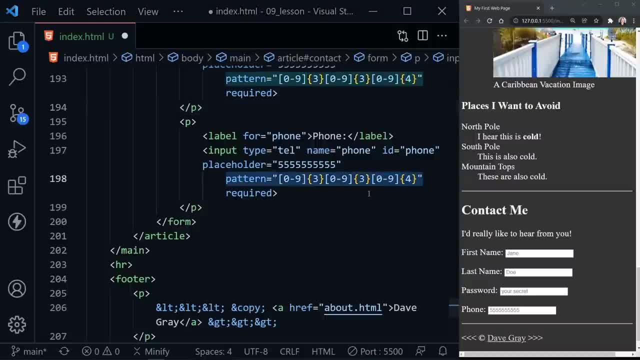 To allow the form to be submitted. So the pattern does enforce What should be entered into that input. And now let's go ahead and highlight phone. I'll press control D again And I'm going to change this value To decade. 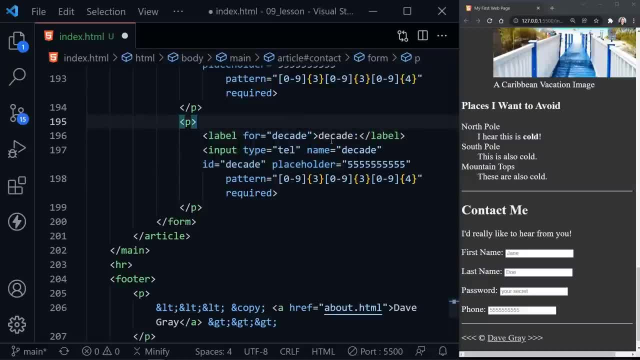 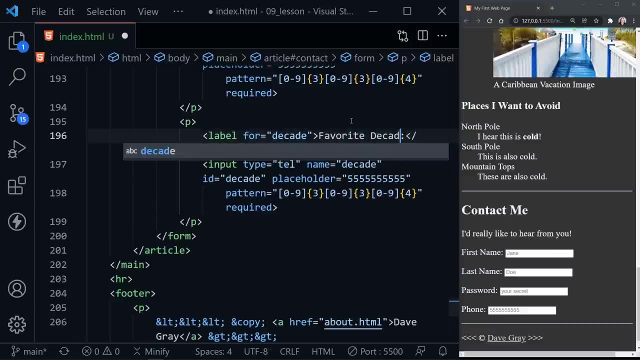 And we've changed the for attribute, The name attribute And the ID attribute, But the label here that we want the user to see Is going to be favorite decade. Now Let's change the input type To number. Let's go ahead and just remove. 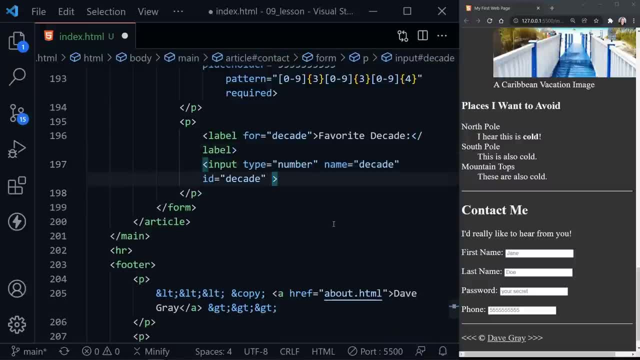 All of these attributes- Placeholder, pattern and required. And now let's add a minimum, So we'll set the min to 1950.. This is where the range will start. Let's set the max To 2020.. And then there is an attribute called step. 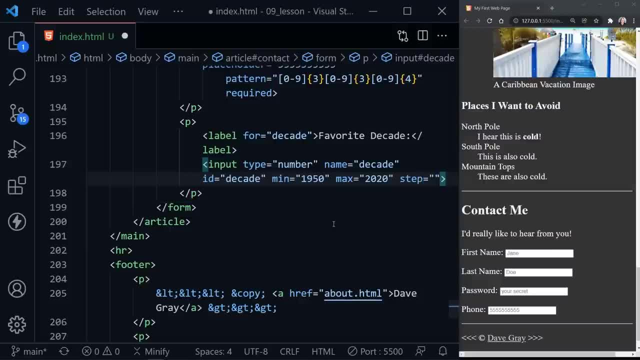 And that means The interval in between- Essentially How many years? in this case, Will we be switching between values, And so we'll just move Decade by decade, Which is 10 years, And then the starting value. So what we want to display, 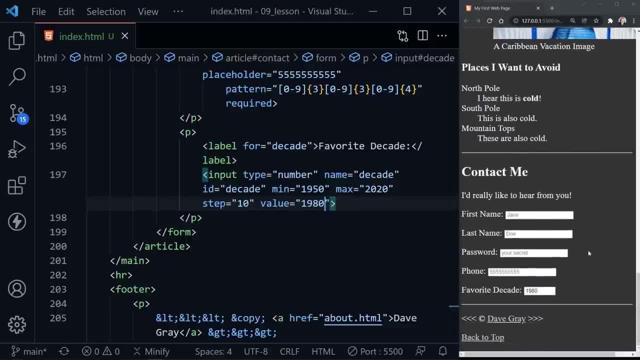 And we'll start with 1980.. So let's save this. And now we see our favorite decade input here at the bottom, And when I mouse over, Notice a couple of arrows appear. Let me enlarge this one more time. Oh. 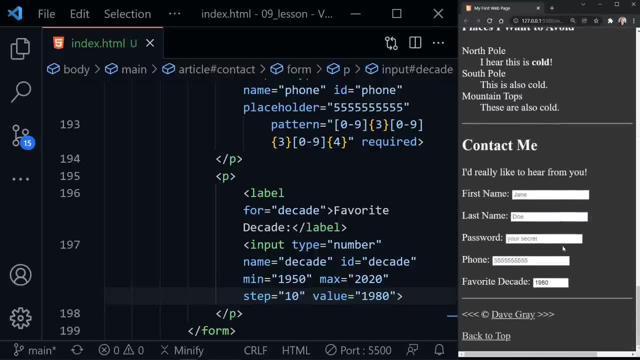 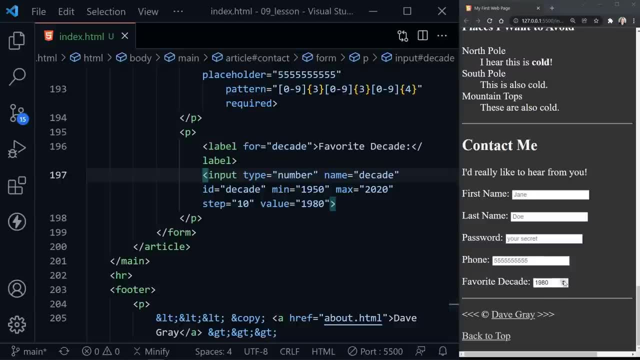 I enlarged the code instead. Let's go to the next page one more time, Scroll up and look at this form. I'll shrink the code. There we go, And so when I mouse over, We see 1980 displayed, But we get these arrows. 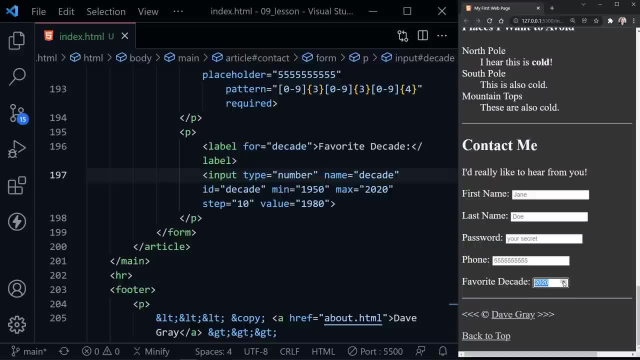 So we can arrow down to 1970.. All the way to 1950. Then I can't go any further. Likewise, I can go up to 2020.. And can't go any higher. So our step interval is working And our min and max are also working. 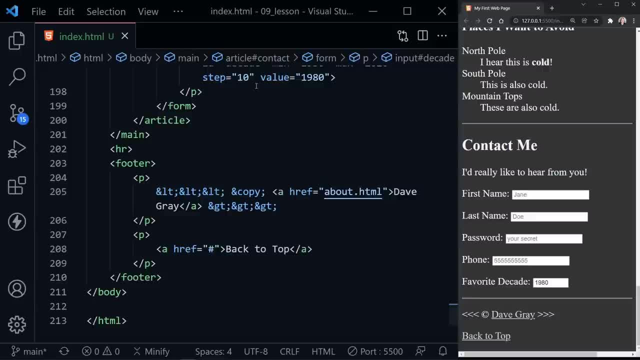 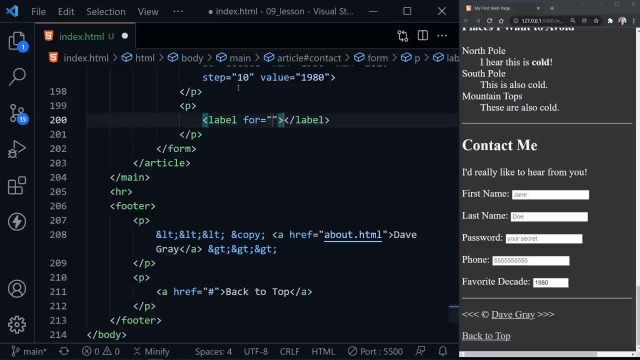 And it's displaying numbers. So I'll zoom over And I won't copy everything down, But I will start with a paragraph element. again, Inside the paragraph element We will have a label And it has a for value. I'll put for coffee. 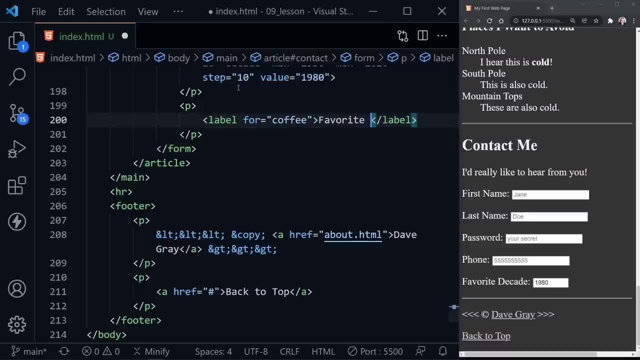 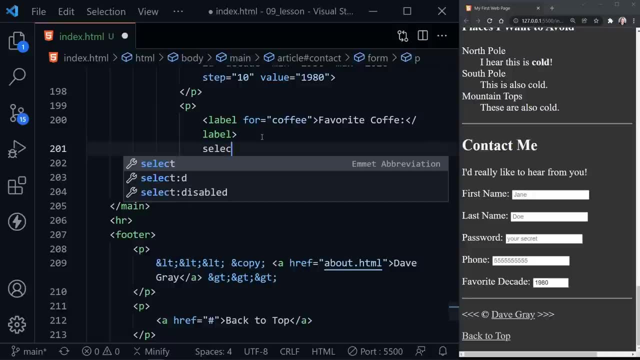 Because we'll ask what the user's favorite coffee is. So we'll say favorite coffee With a colon, And now, underneath that, Instead of an input element, We're going to add what is called a select element. Now notice, it still has a name. 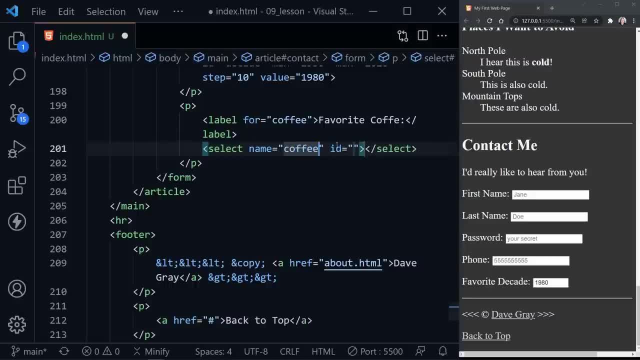 And ID, Or we'll assign the values coffee To both of these as well. The ID here still needs to match the for For the label And we'll still have the same name For the input As it's received at the server as well. 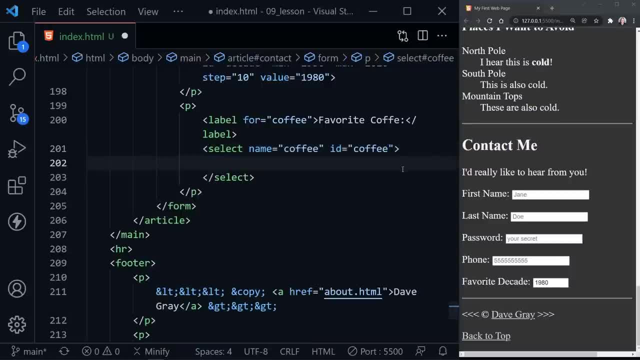 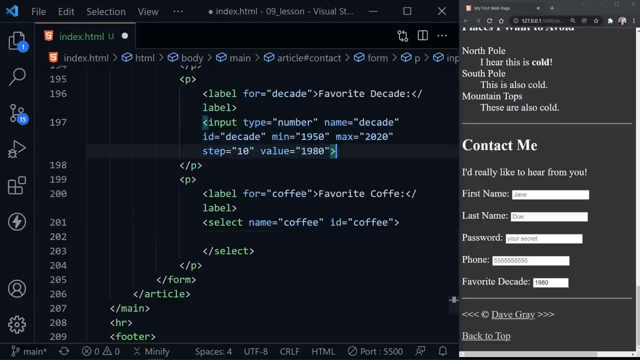 Now notice we do have a closing select element And so with that closing select element- Notice that's already different than the input That does not have a closing tag For the element. But inside of select We need to put options. So let's say: 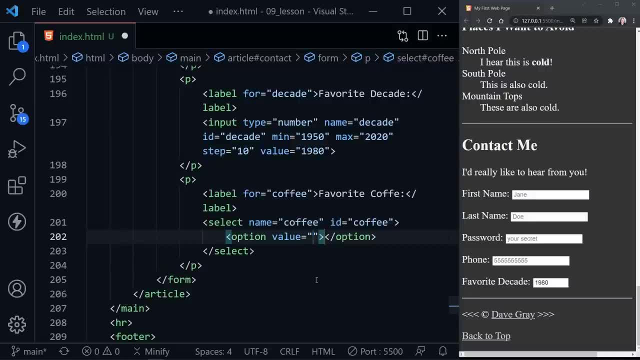 Let's give our first option element here And it has a value And we'll set this to Regular coffee. But now that's not what the user sees. The user is going to see what we put Between the opening option And closing option tags. 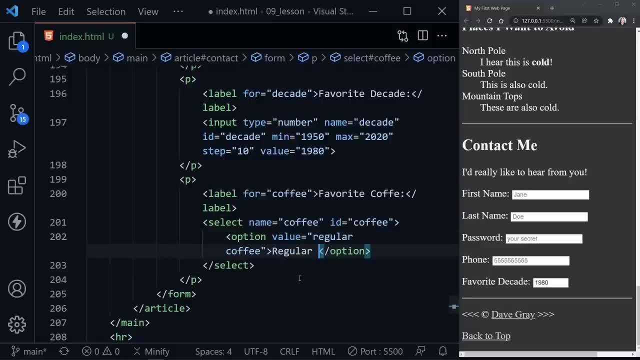 So here I'm just going to put Regular coffee With caps Instead of all lower case. And now for the next option. Let's put Iced coffee And do the same thing As far as what the user sees. There we go. 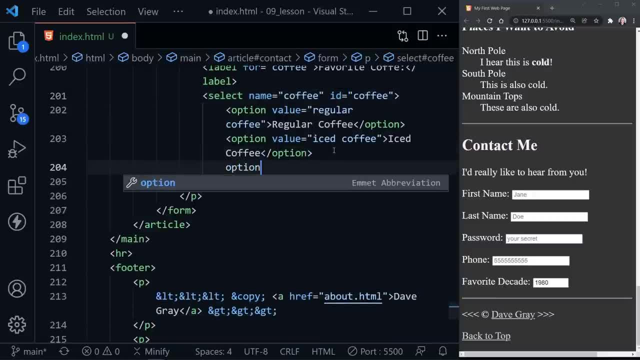 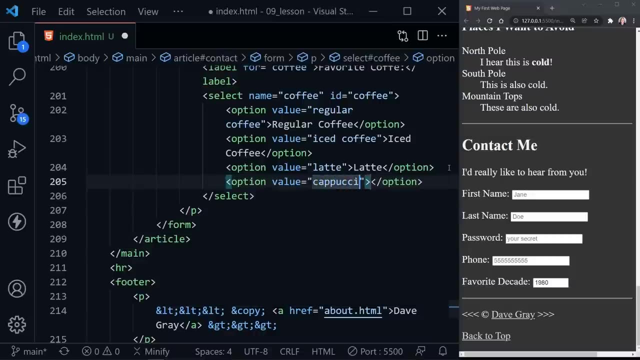 I need to scroll up just a little more. And let's look at our next option. Let's say this is a Latte. I hope I spelled that right. And let's give Another option. Let's call this Cappuccino. 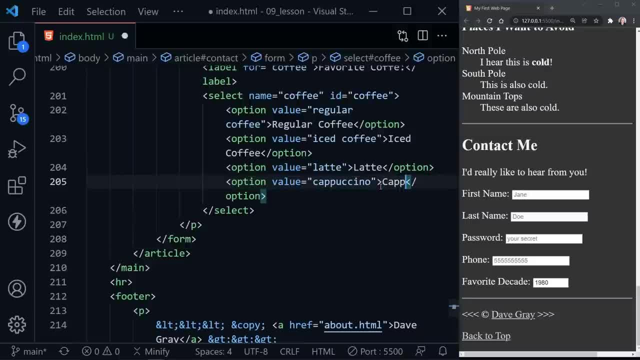 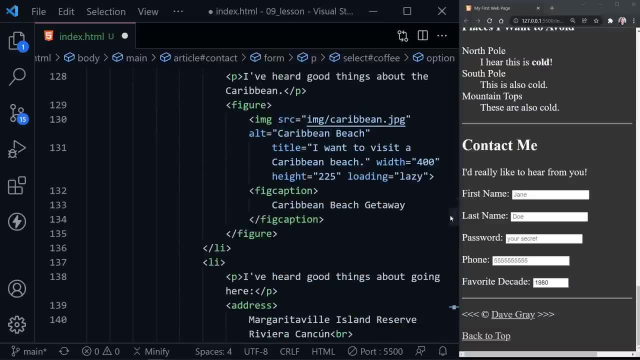 Cappuccino C-A-P-P-U-C-C-I-N-O. There we go. That's a little One I don't think about every day. Whoa, I scrolled because I clicked Just a little too far to the right. 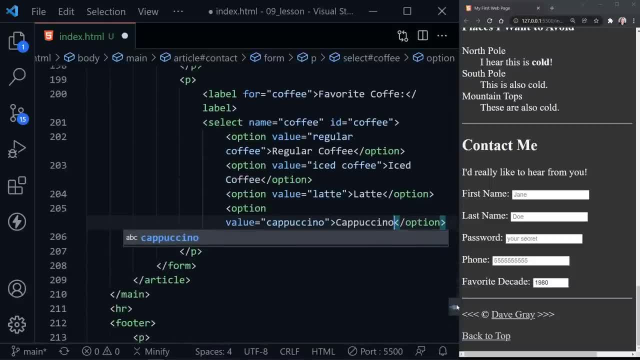 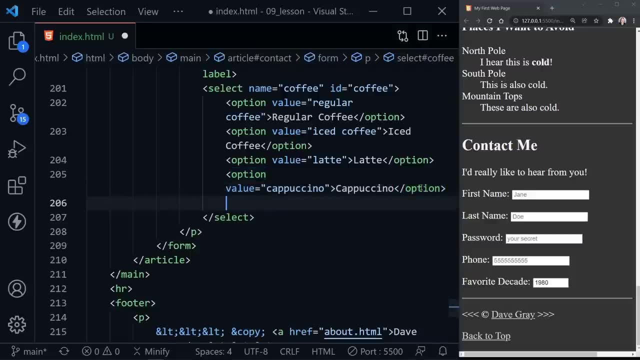 Sorry about that. Scrolling back down to our cappuccino, There it is. I scrolled way up by mistake. Get to the end of that line, Press enter. Add one more option here, Maybe two Cappuccino. 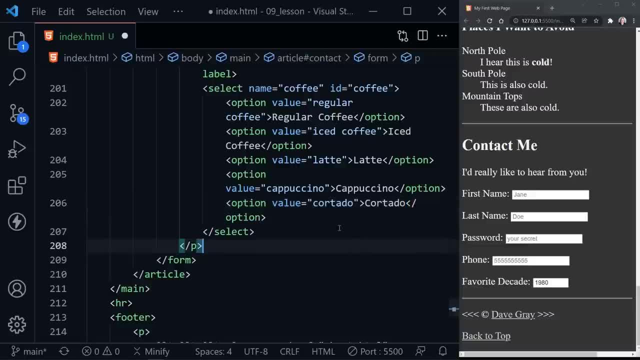 And what else could we put? Oh, yes, What I like to drink, Which is An Americano, So we've got several coffee drinks now In our list And maybe we should put Other- Other is always good- there, Because there could be something we didn't think of. 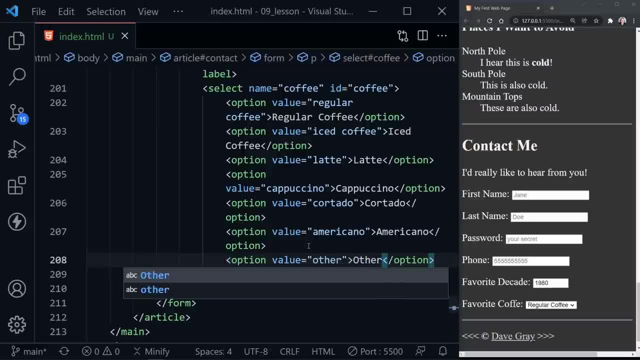 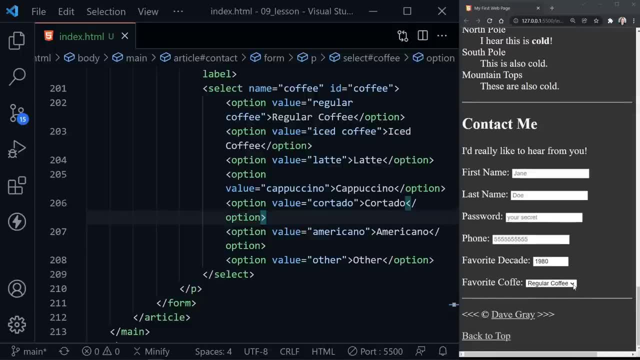 So let's just put an other selection too And save. And now if we look at our form Over here, We can see the favorite coffee is here With the select menu And we have to click on the arrow And then all of our options show. 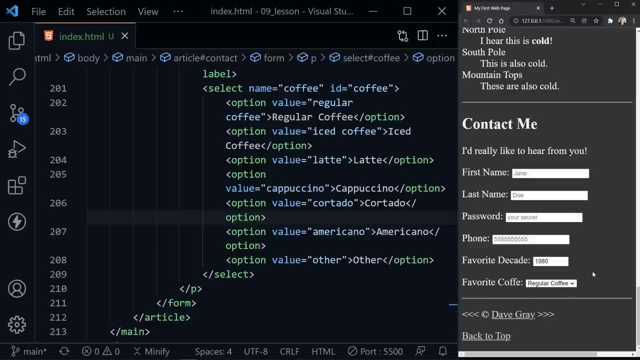 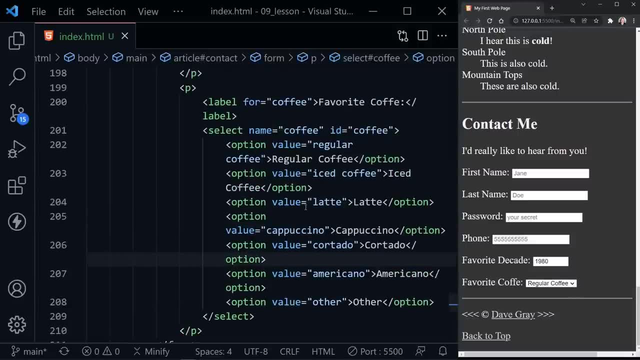 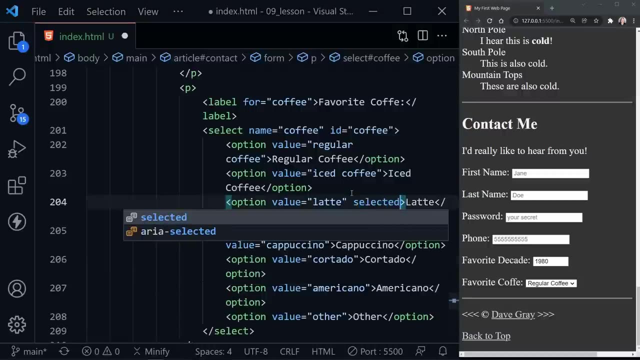 And we can choose, Like I would choose Americano, We could choose other. Any one of these options, And the top one Is what is showing, But we could decide to show a different one If we set it as selected So in the options. 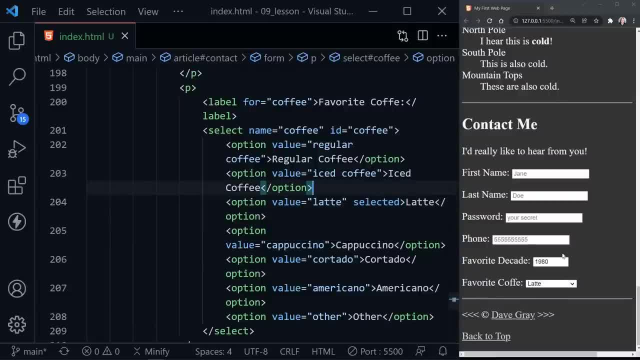 We would put selected here In the option And if we save Now it displays latte by default, So you can choose which one displays Instead of just the top one. Our code is looking a little messy here As things started to wrap lines. 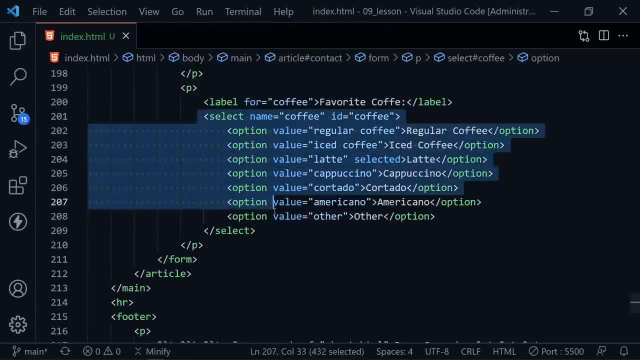 So let me just expand Visual Studio Code for a little bit And you can see how this looks much more organized When the lines are not wrapping. Now there's another element we can put in here To help organize our selections, So let's do that. 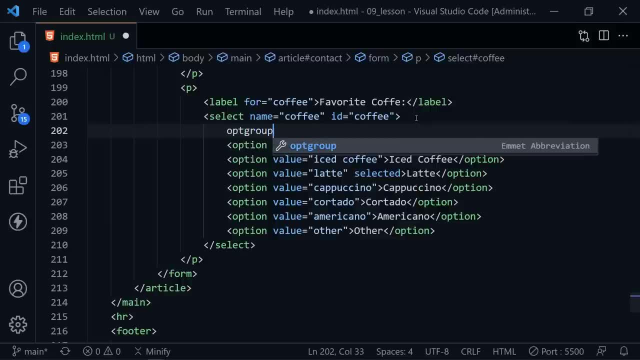 And it's called an option group, OPT group. So once I tab over It gives us the closing tag too. I'm going to highlight And control: X to cut And out of the coffees That we're going to have. 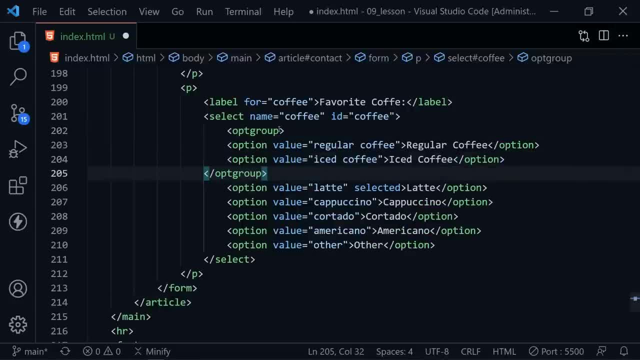 Because this first group will be coffees. It's just the first two options, So let's close this here. It will reformat as soon as I save. But we also need to put a label attribute Which is different than a label element. 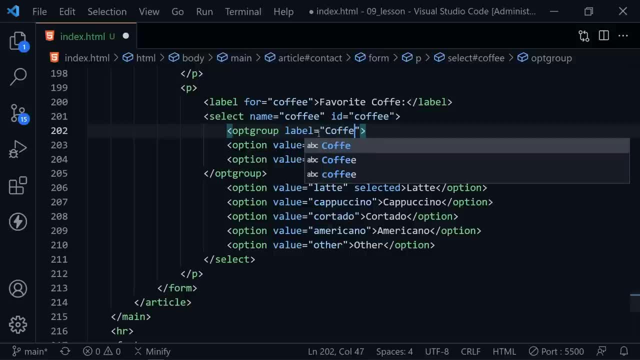 So this label attribute on the option group, Let's put Coffees With a capital C, Because you will find out, The user will see this value. So now let's save this, And we're not going to look back at the web page yet. 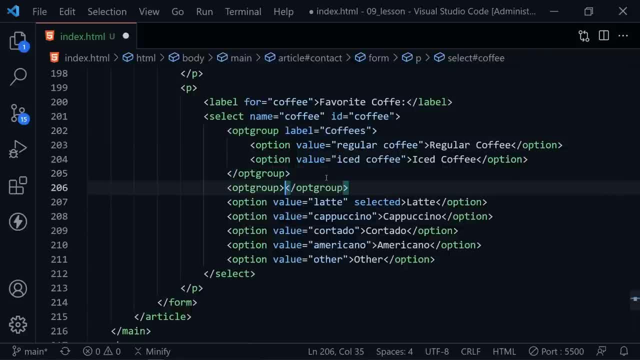 Because we need to put another opt group here For the other coffees. So now that we have that, I'll select the closing tag And I'm going to put it after Americano. Other doesn't belong to a group And that's okay too. 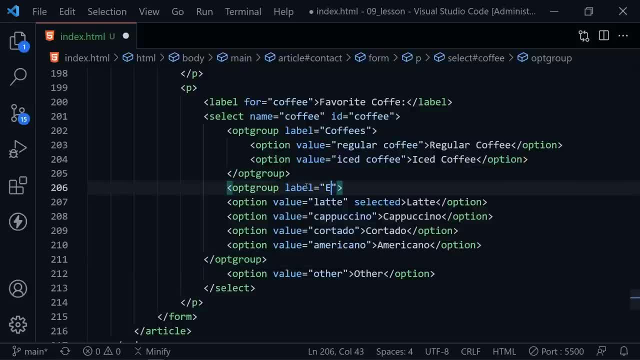 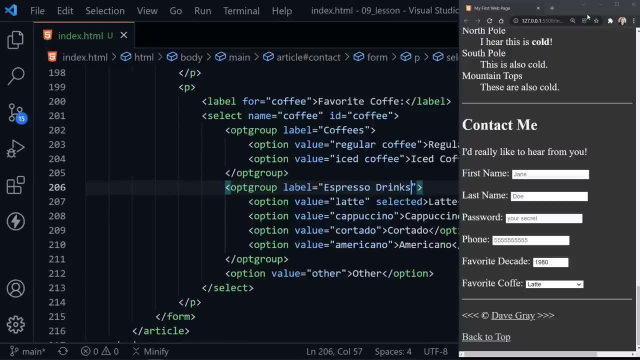 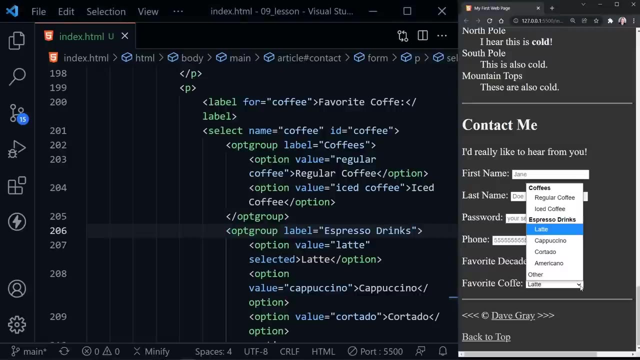 But let's give another label here For this group With a capital C: Espresso drinks And save. Now I'll resize visual studio code And we can look We still have our latte Selected as the default choice. But now, if we expand this, 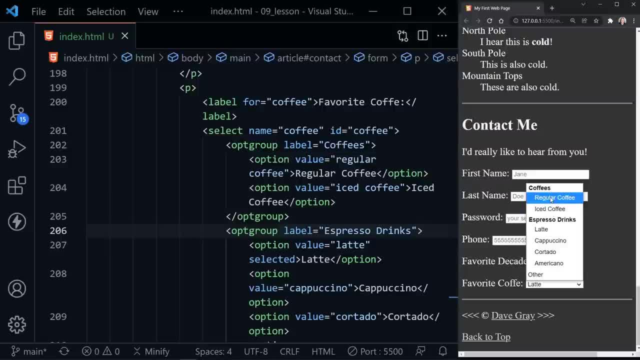 You can see, coffees is in bold. We can't choose coffees. I can't choose espresso drinks, But I can choose regular coffee, Iced coffee, Latte, cappuccino, cortado, Americano Or other. 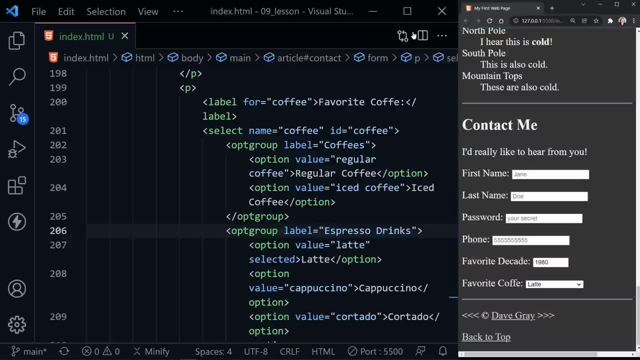 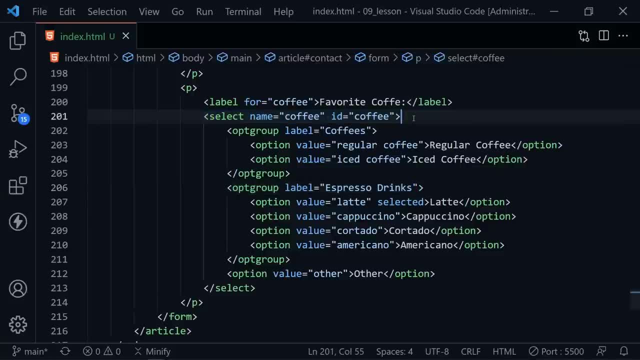 And those option groups. We can make a couple of other changes too. So let's go back And just look at the code again, And these other changes are actually attributes That we'll add back to this parent select element. So one is multiple. 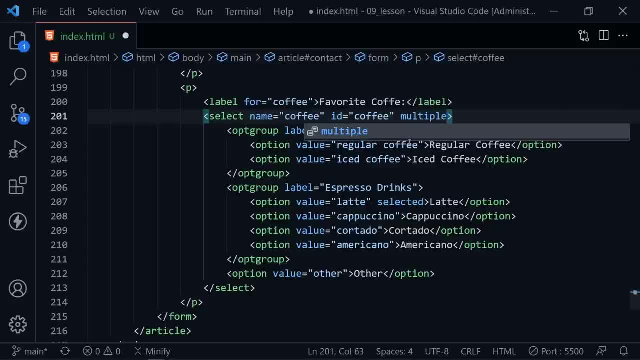 And that means We will be able to select more than one choice, So we could select Iced coffee and Americanos. And then we want to put a size value, And this size Says how many from the list Will display. 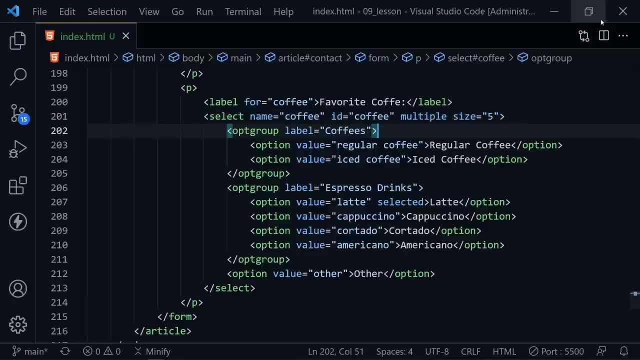 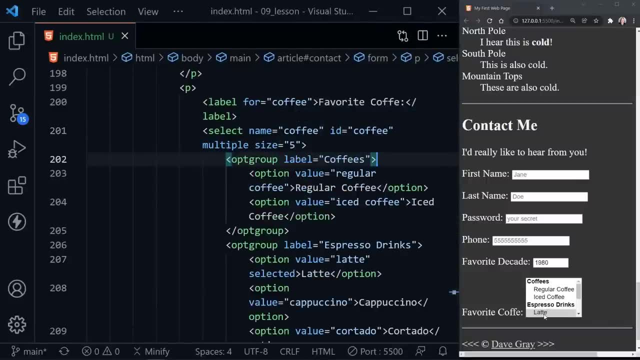 On the page at once. So if we save that, You'll see what I mean by size. Now notice we have five values Automatically displaying on the page And notice latte is already selected, Because we told it to select latte. 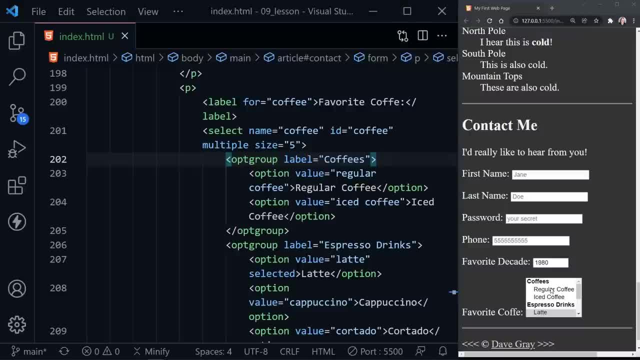 But we could also hold down The control button And click regular coffee, And now we have two selected at once, And I just noticed my typo In the label Where I only have one E in coffee, So I better fix that. 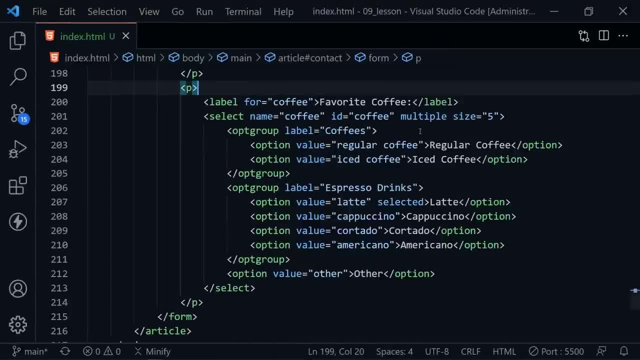 So I'm going to go to the word And save. Okay, I'm going to expand visual studio code once again. Now, this looks nice on our page And it allows us to select more than one coffee, And that's great. But I want to show another input. 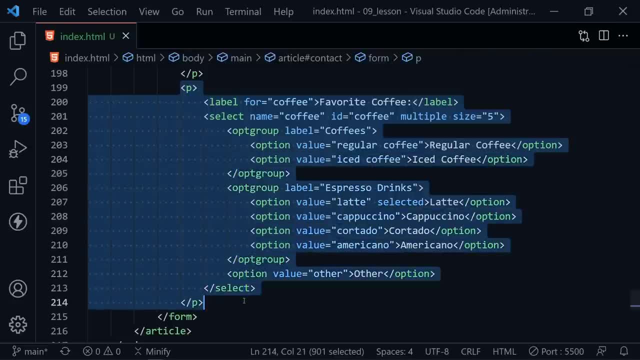 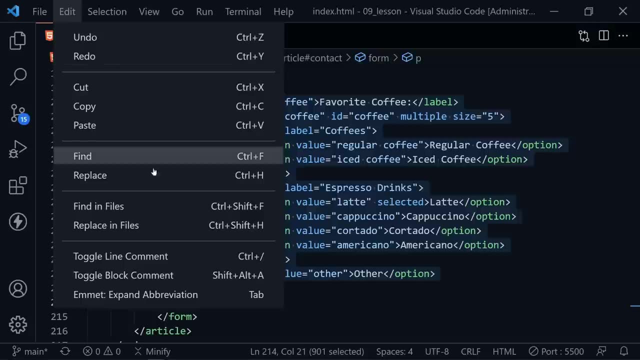 That we could use for this same type of data. So right now, starting on line 199.. I'm going to highlight everything down To 214.. Now, from the edit menu, I believe there is yes, Toggle a blocked comment, And I do this with shift alt. 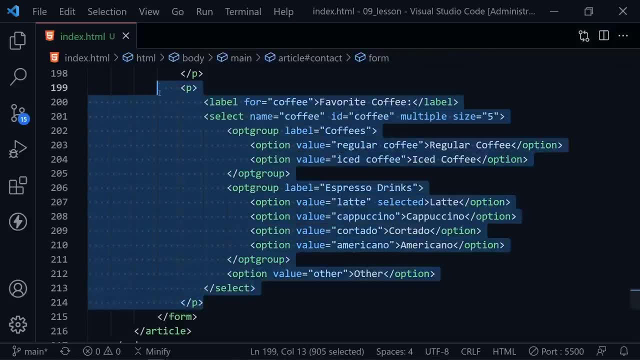 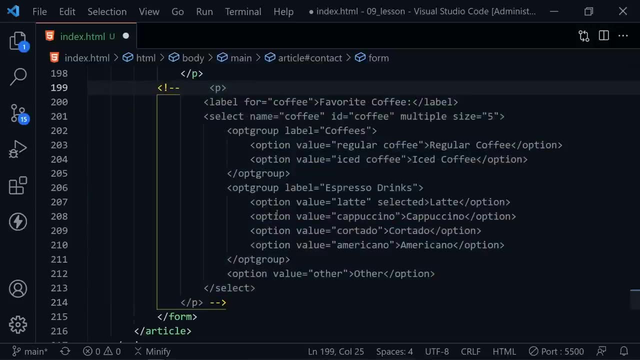 So I'm going to select all this once again, This paragraph, And press shift, alt and the letter A, And when I do that, Notice it comments everything out. So I've kept the code If we want to go back to that. 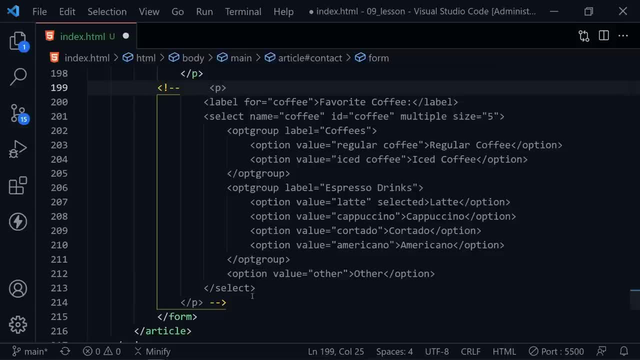 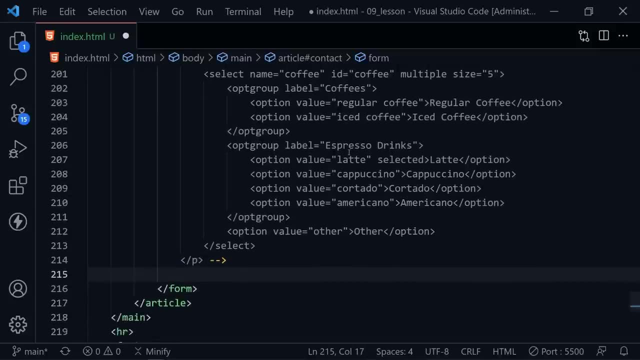 But this is an HTML comment That we have previously gone over In a past lesson And it just comments the code out for now. So I'm going to paste in another way That we could use this same information And present it to the user. 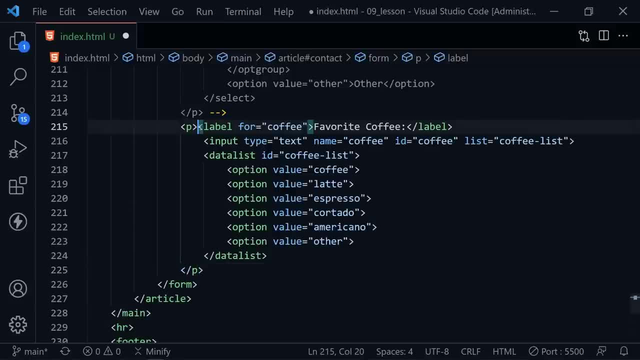 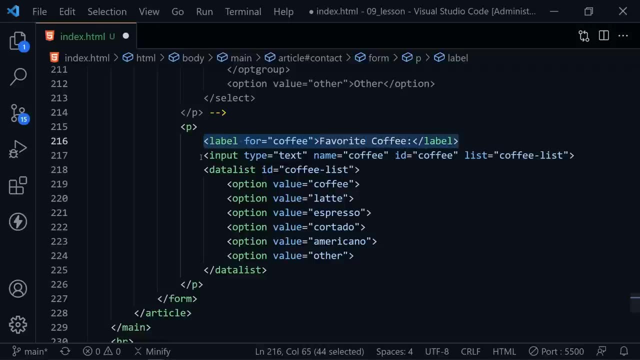 So here's the paste And let me go ahead and return there. So we have the paragraph on a separate line. But notice, we have a label. It's for coffee. It says favorite coffee. Now we don't have a select, We have an input type. 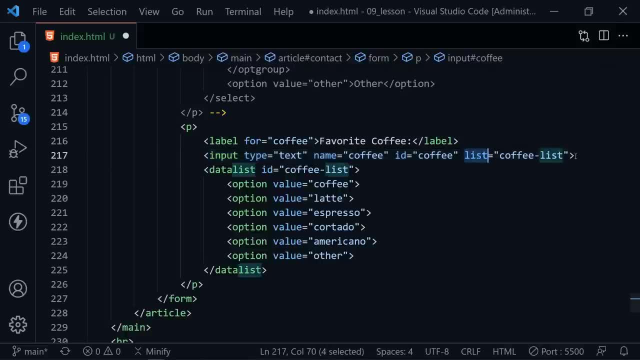 And it's a text type And then it has a list attribute And it says the list Is the coffee dash list. Then notice we have a data list element And that ID matches the list attribute of the input: Coffee dash list. 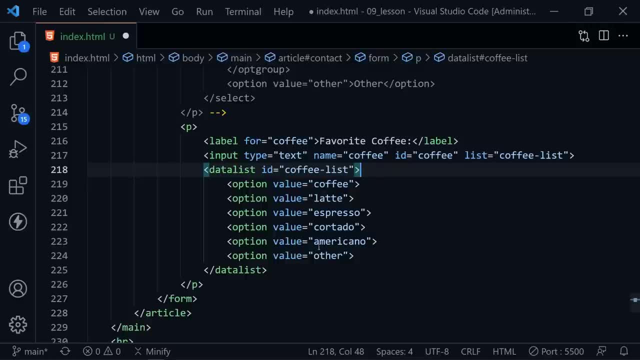 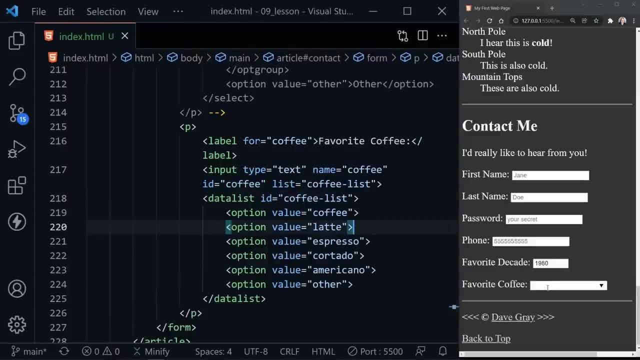 Then I've got some values here That we saw in our select menu. So this is just another example. Now let's save this And go back and look at our page And see what we've got. It looks like a text input now. 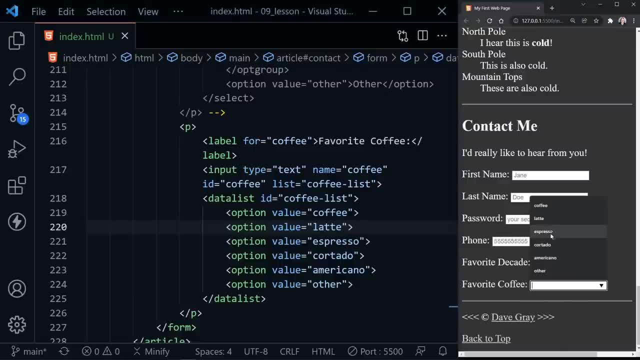 When I mouse over Notice the arrow, And if I click the arrow There's our choices that we're getting from the data list. But what is nice about this? If I just click in there, They pop up And I can start typing. 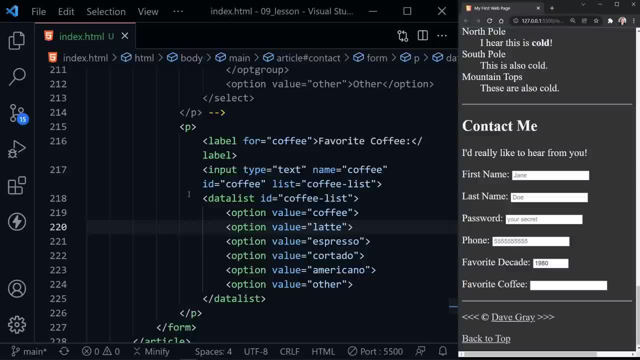 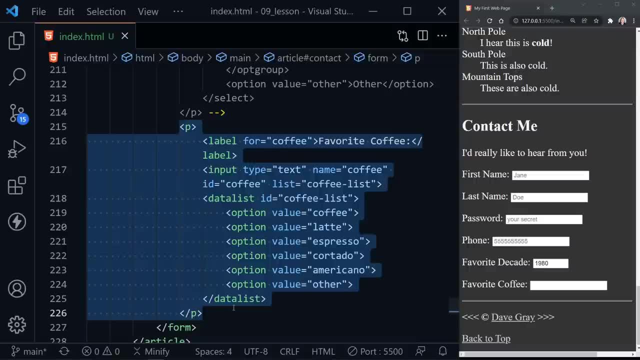 And then it just narrows it down. So it's just another type of input That can handle very similar data presentation. So, okay, What I'm going to do now Is highlight that data list, Leave it in the code for you. 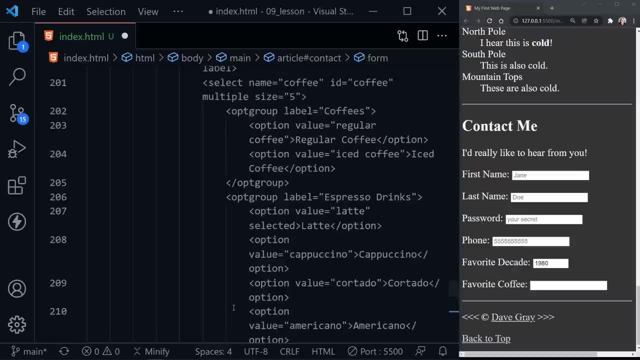 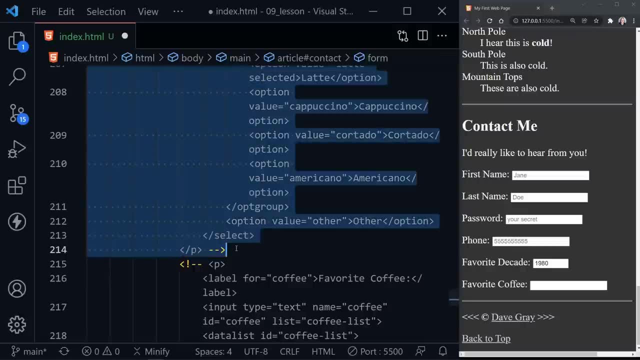 But comment it out Again. I pressed shift, alt and the letter A to do that And I can reverse this comment By doing the same thing. So again, line 199. All the way down to 214.. Shift, alt and the letter A. 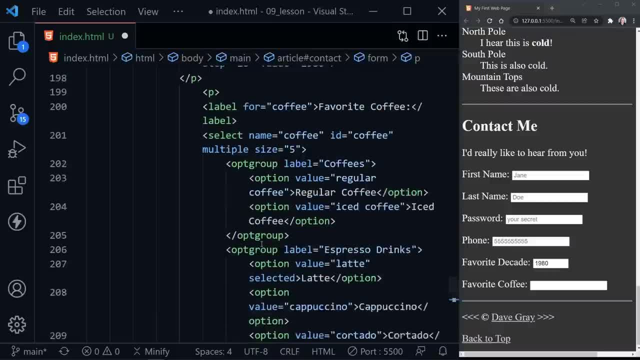 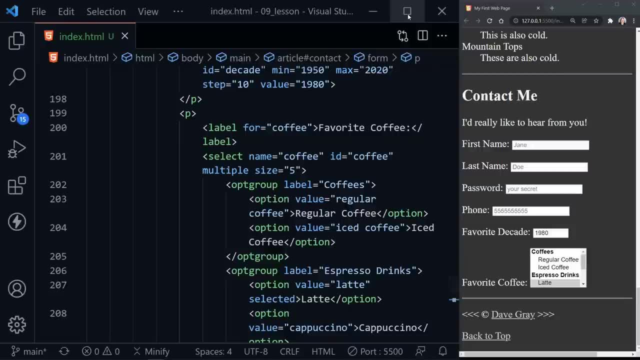 And now it is uncommented, And so we've got our original List back with the select And I'll save that And you can see that now on our page over here on the right. Okay, I'm going to expand Visual Studio Code again. 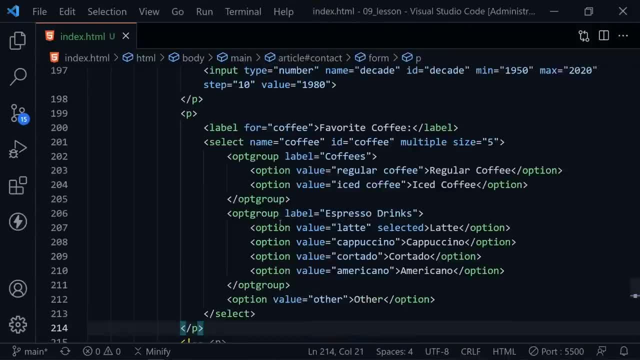 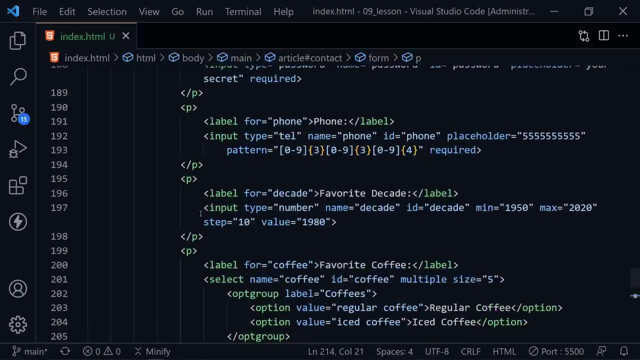 And now so far We have got fairly good semantics for our form, Because we are applying a label With the proper for attribute For every type of input that we have, And that's good. But when a form gets large Sometimes it's good to organize it. 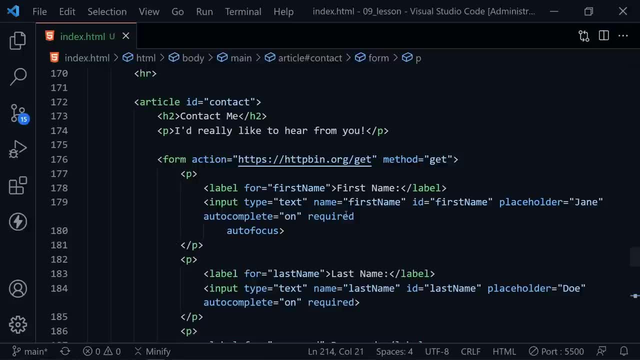 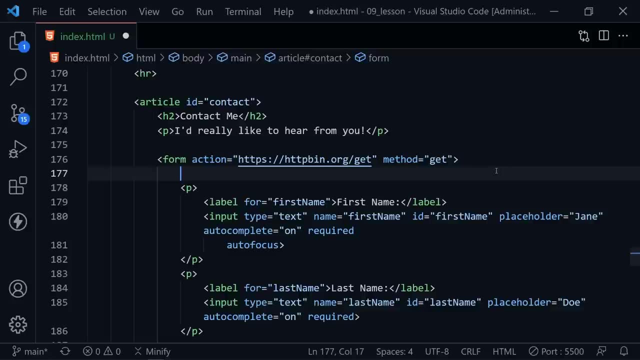 Into different sections, Sections that say What each part of the form is about. So underneath our form element, The opening tag, here I'm going to type a new tag Called field set. And now I'm going to go ahead And copy that closing tag for the field set. 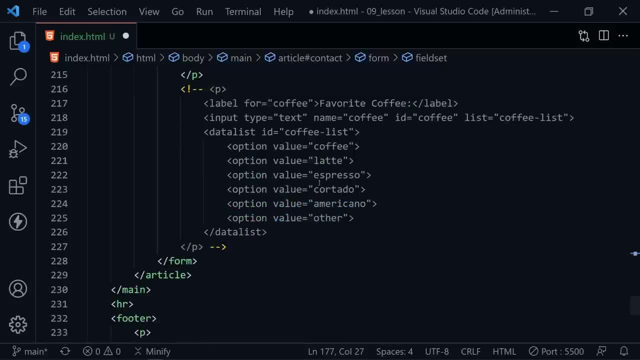 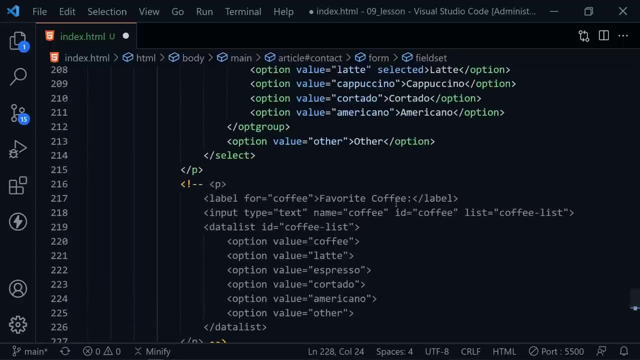 And come all the way down To just above our closing Of the form as well, Because this will be a section Where we've asked about the different information, Such as the name and your favorite coffee, And so on. And now, inside of this field, set 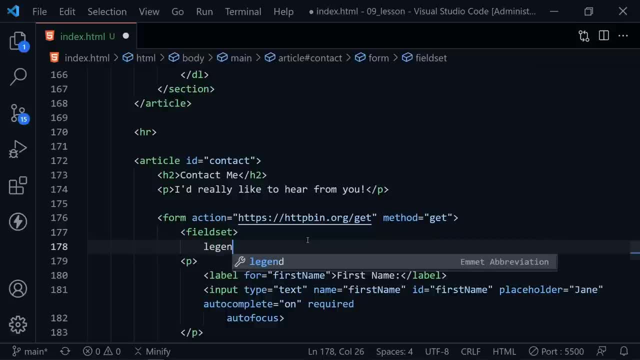 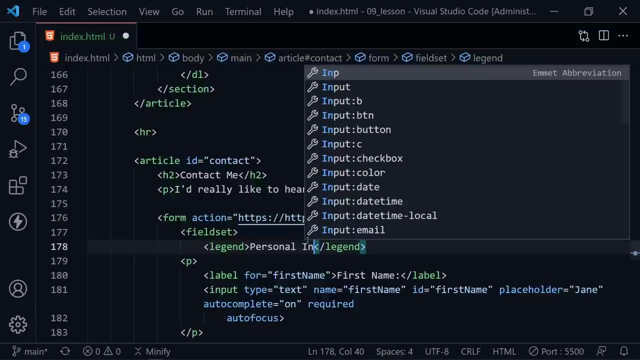 We can specify What we're requesting, And this is called legend. It's a lot like a caption And this is just saying What we're requesting in this section of the form, And I'll put personal info here And then we can save. 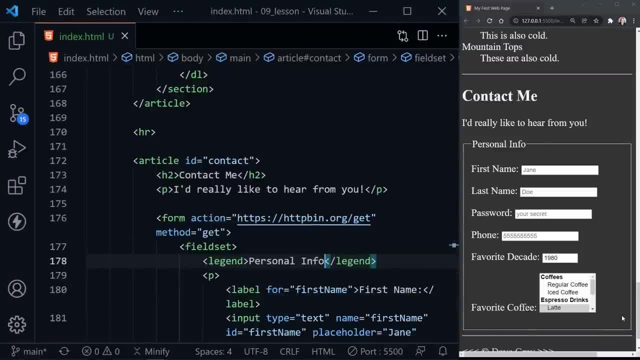 Now let's go back and look at our form again And you can see It's surrounded, This section of the form, Because we're going to add more to it yet. So we just sectioned off part of our form. essentially It's got a square around it. 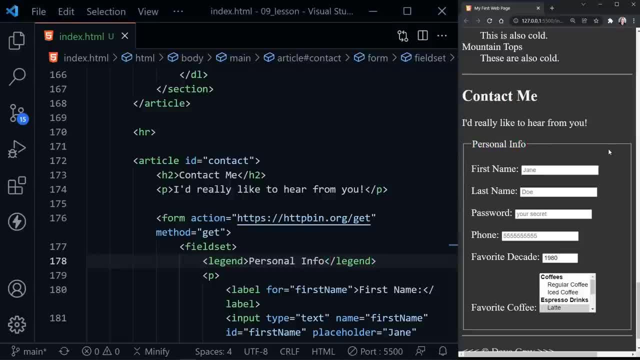 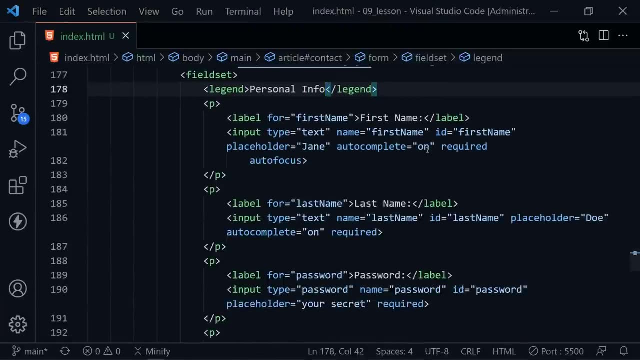 Is part of that frame, Of this section of the form, And clearly this does give some more Semantic meaning, Actually conveys meaning in our structure As we define part of the form And what it's about. Okay, Let's continue to add to our form now. 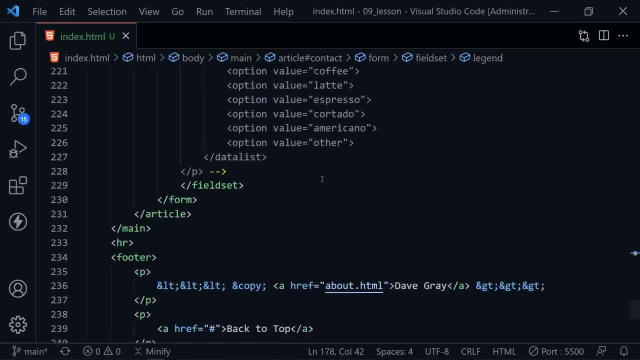 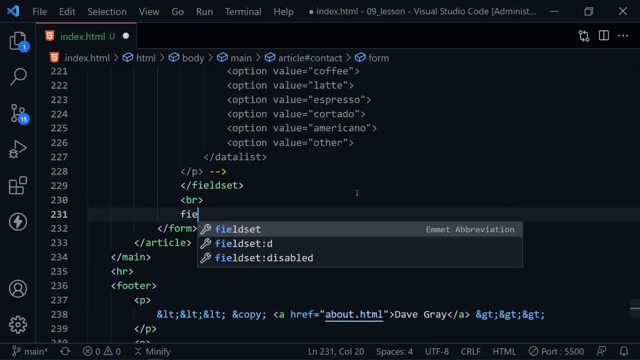 Because there's some other types of inputs We want to cover. So let's scroll all the way down By our field set And now, after the field set, We'll put in a break. So inside this field set We can add another legend element. 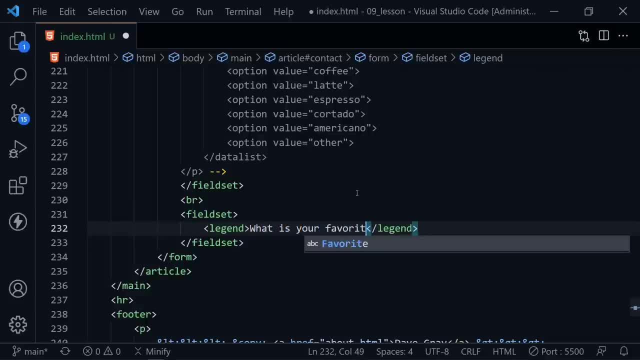 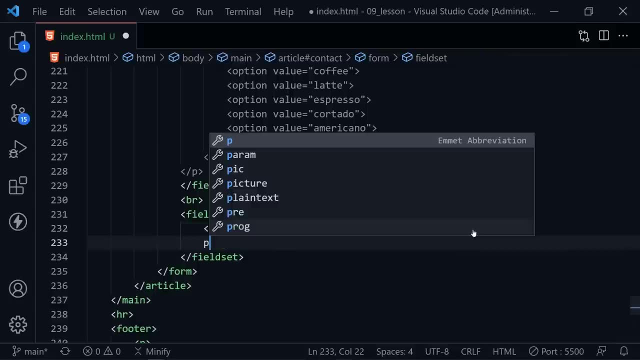 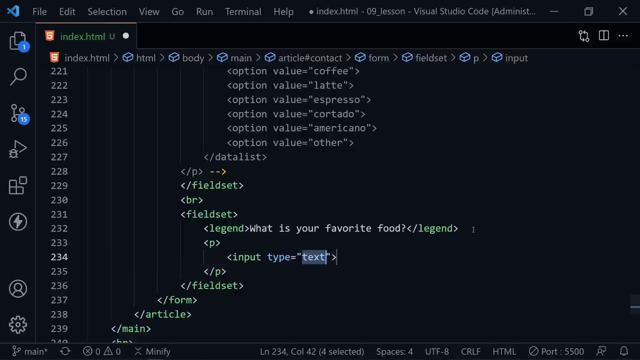 And we're going to say What is your Favorite food. So this section of the form Is all about choosing a favorite food. We'll start with a paragraph Inside this paragraph, Let's have an input before the label This time. 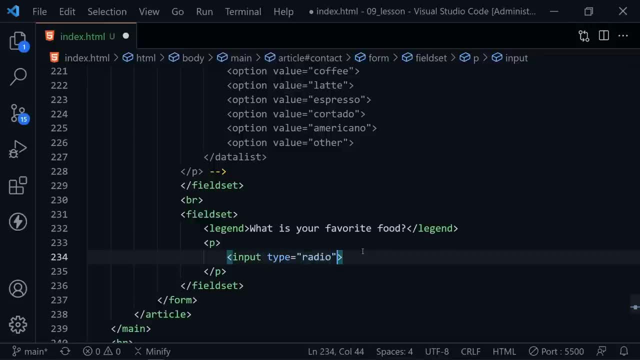 And this is going to be type radio. Radio inputs are a little different, But let's give it a name attribute And this will be for food. And now the ID attribute Is going to be different than the name this time, So we're going to say tacos. 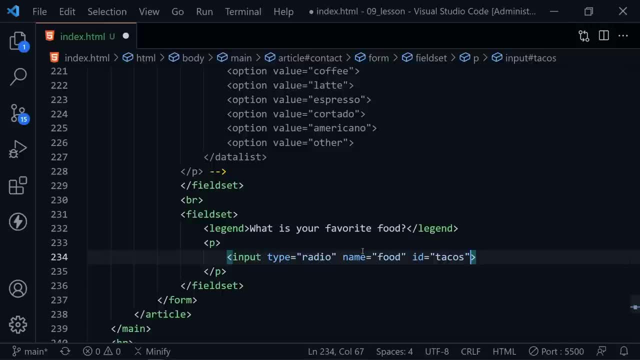 This is going to actually be more like What the value of the input is, And we'll assign the value attribute, And here we'll say tacos as well. So now that we've done that, Let's go ahead and put the label. 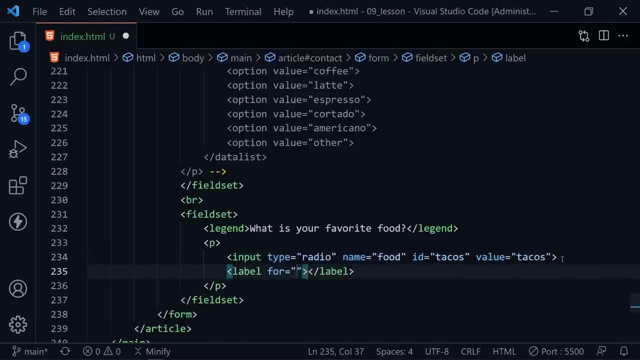 Underneath, And there we can have the, for Which it should still match the ID, Which is tacos. And then what do we want to show in the label? Well, of course, Tacos Capital T. Okay, now that we've done that, 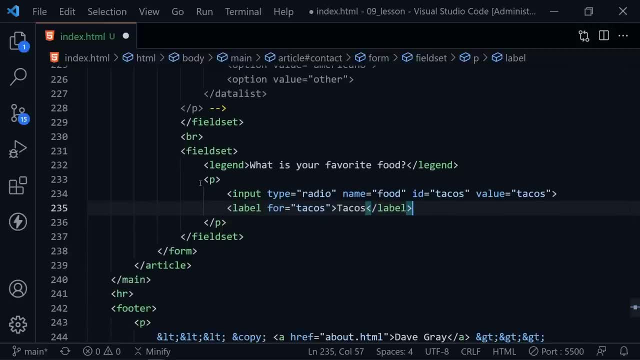 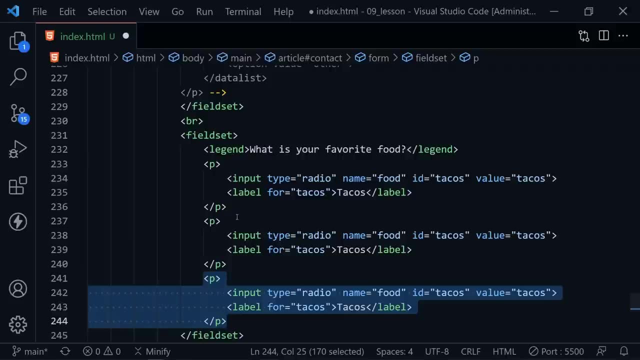 We've created one radio button So we need to do a couple more So we have other food choices. I know tacos is the proper choice, But we should have a couple of other choices here. So going to just do shift, alt and the down arrow twice. 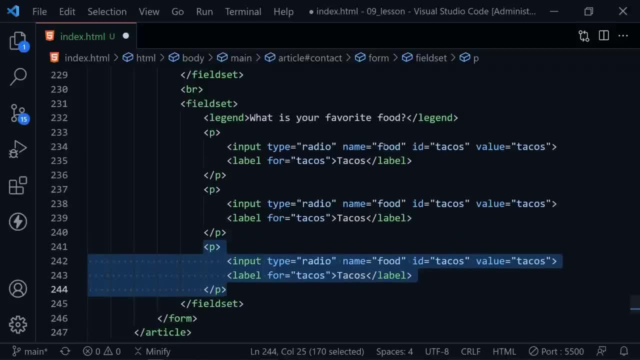 We've copied those down. We're going to leave the name attribute Food on all of these, And that's because You should only be able to select one of these. So when we select one, The other choice should Be selected. 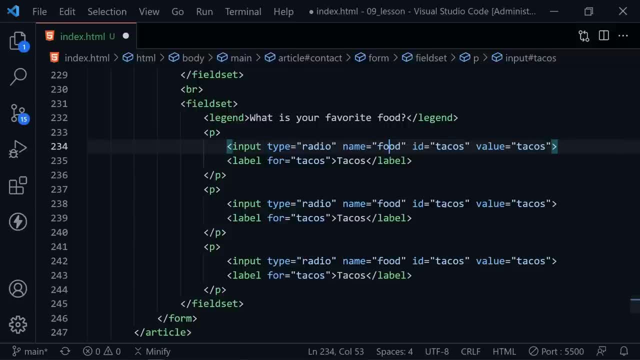 And that's what we achieve By giving them all the same name for the input. But as far as tacos for the ID And the value, We can change that to pizza And we of course should change Pizza here. Oh, and I should have changed the four here to pizza as well. 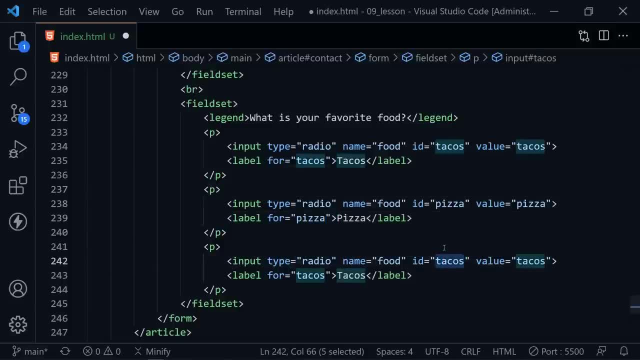 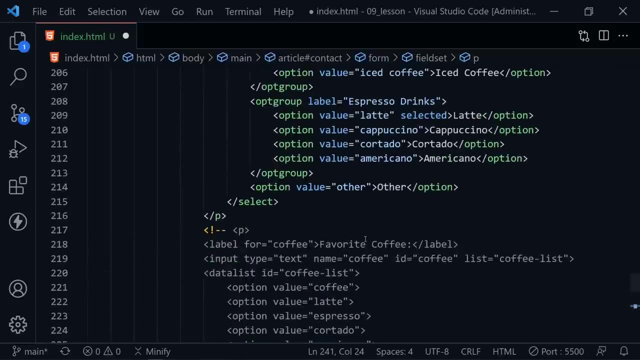 So there should be three. Now this last one, Let's go ahead and select all three tacos, Change it to other, And then Here we'll say other as well. I should note That if we had an ID of other, We didn't with our option up here. 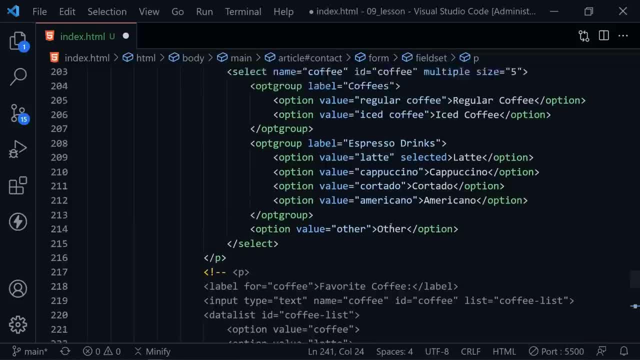 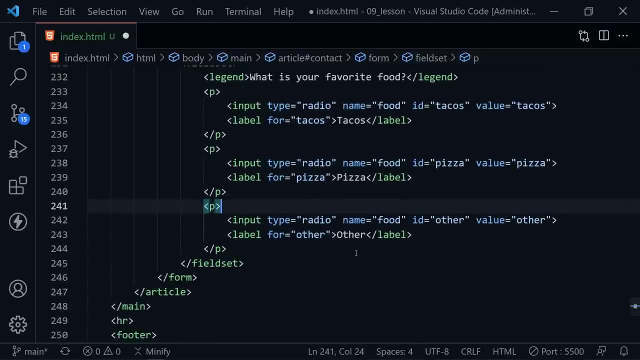 That was separate, That had just the value of other As far as the option and name, And the ID was coffee. So we're good, But you don't want to double up. You want to make sure you have individual or unique IDs. 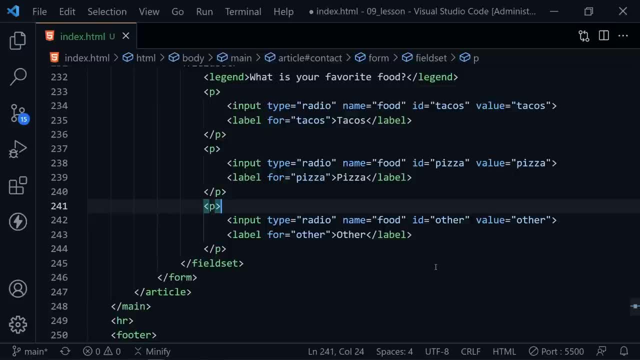 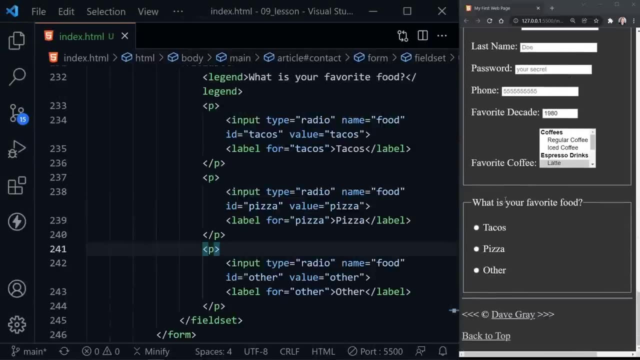 For each input in your form. Okay, now that we've added our new field set With the choices for our favorite foods, Let's take a look at that back on our page. So if we scroll up, We've got what is your favorite food. 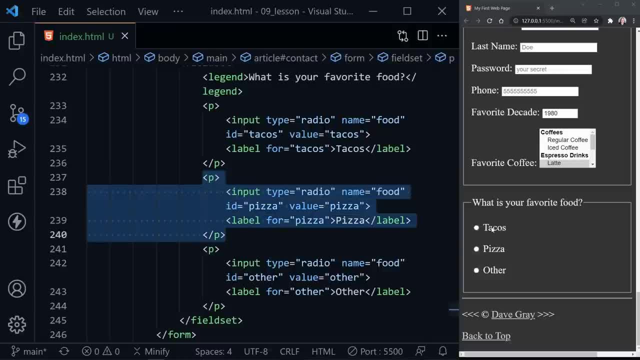 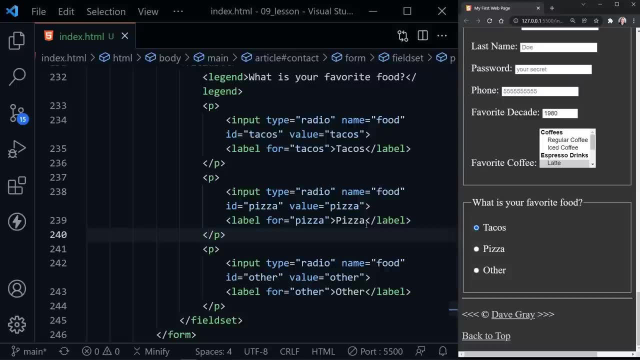 And since they're all in paragraphs Which are their own block elements, They're each on their own line Inside of our field set, So we can choose tacos, But then because they all have the same name, food, If I choose pizza, 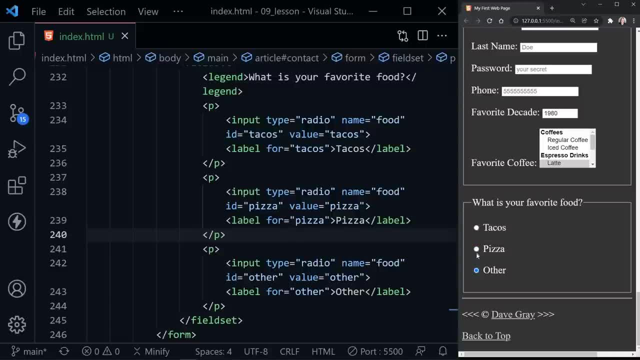 Tacos is no longer selected And it's only pizza. So you want to make sure Out of the radio buttons They all have the same value for the name attribute. Okay, let's scroll down a little more And let's add another field set. 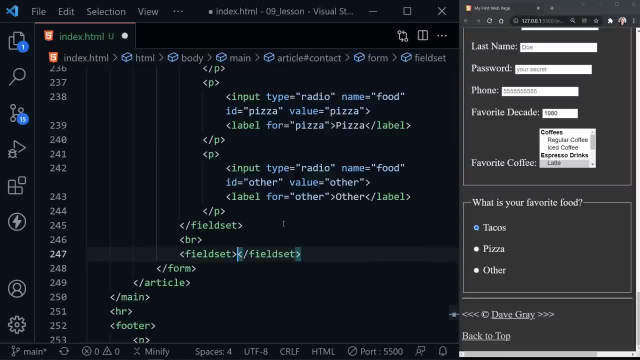 And we'll look at another type of input Inside this field set. We'll have a legend as well, And here we're going to say: Do you have pets With a question mark? And now For our inputs. They're very similar to radio buttons. 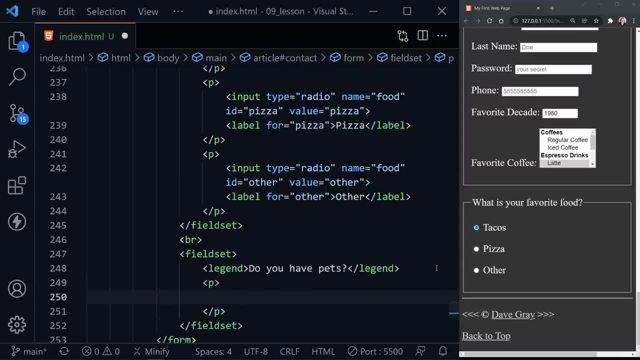 But not quite the same. So I'll start out with a paragraph Input, And the type is not text, It is checkbox, And then, once again, We'll set this equal to pets And the id Is going to be equal to dog. 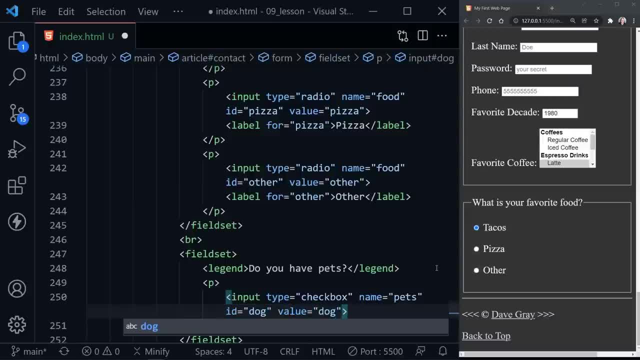 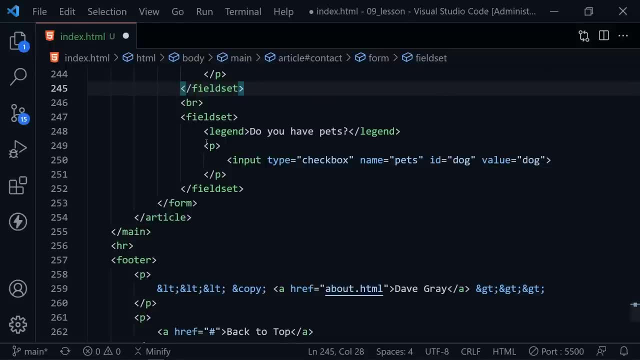 And then the value Is equal to dog. So you can see. the pattern is much like When we were adding radio buttons. Let me expand visual studio code So this will be a little easier, And now we'll go ahead and add a label after that. 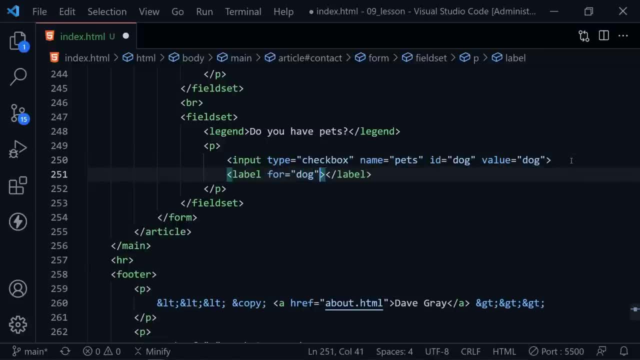 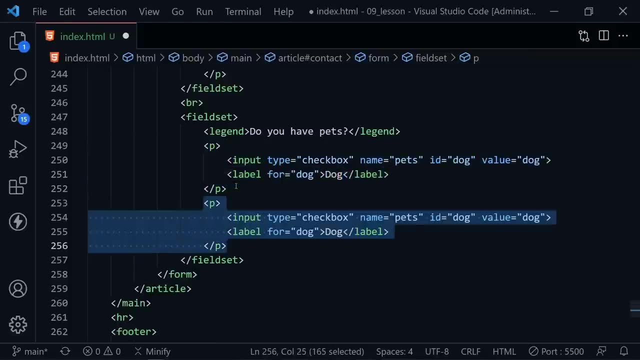 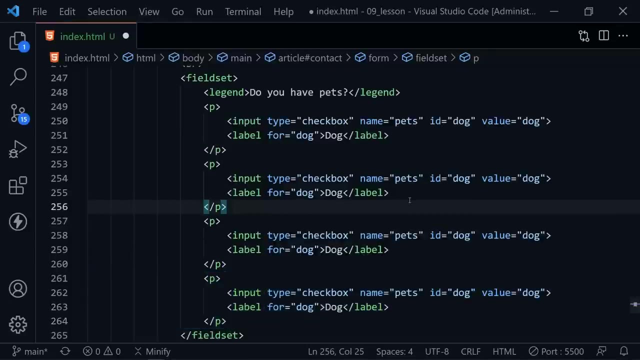 And the label value will be For dog And what we will display on the page Will be dog as well. I'll highlight this. We'll copy this down Three times. So now We'll continue to have the value pets. 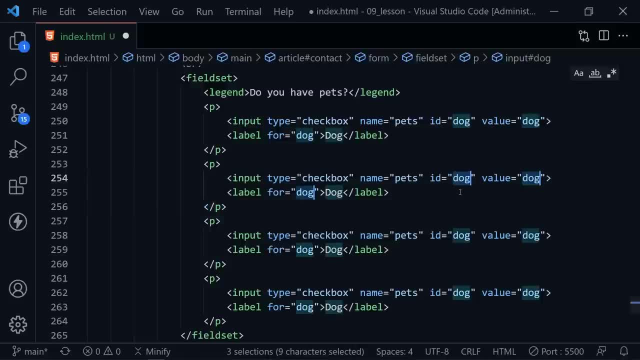 For each one of these inputs, But the next pet Will switch from dog To cat And we'll put cat here on display as well. And then maybe we want a fish. We'll switch this to fish And then finally, We could think about doing: 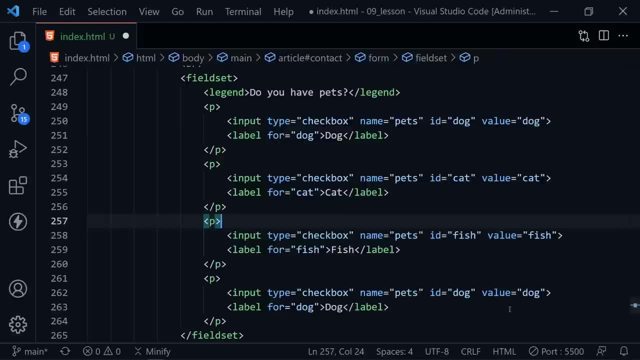 An other as well. But remember, We can't have an id that says other here too, We would be doubling up on that, So that could be a problem. Let's say: And select all three and say Other pet And from there: 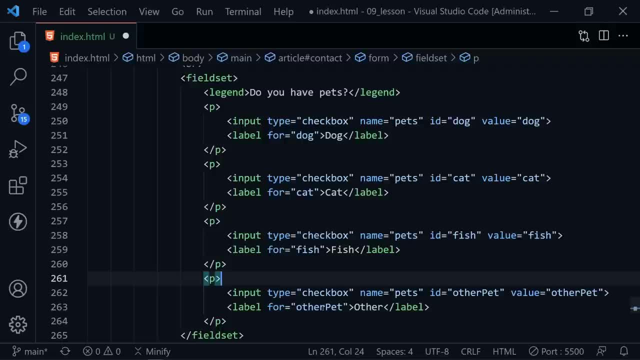 We could say other, Because we just need this to be different. The id specifically Needs to be different Than any other id on the page Or in the form. Now let's save this and look at the page And there will be a difference between the radio buttons. 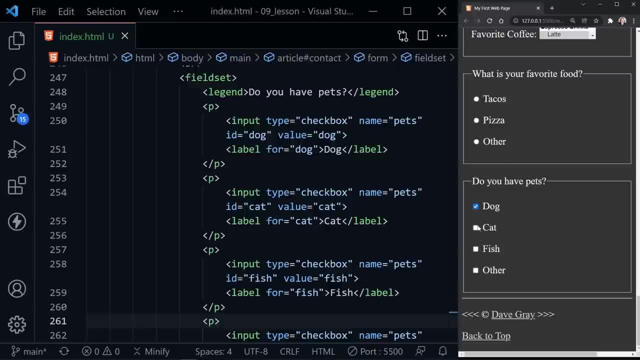 Because when we ask, do you have pets? And we have a checkbox, Maybe we have a dog And a fish And we can select more than one at once. A radio button won't let us do that, But a checkbox will. So maybe we have a dog. 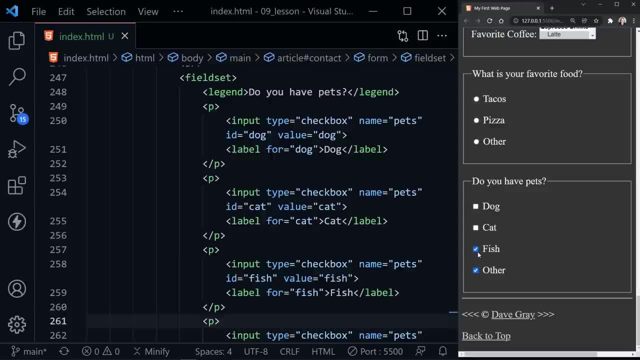 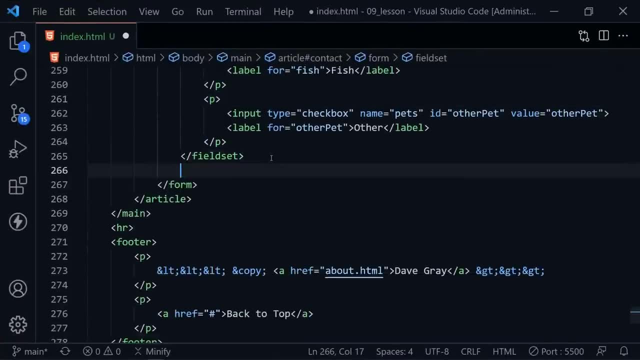 And a frog, So we choose other. You can select as many of these Or as few of these. Now let's go down to our last input type. So we've covered quite a few Today already. Let's add one more field set. 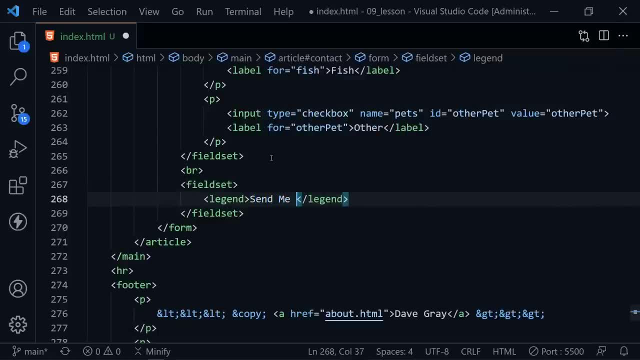 And inside of here, another legend as well, And let's put send me A note. So inside of this field set, We're only going to have one input, But it's definitely different than the others. This one is going to have a label. 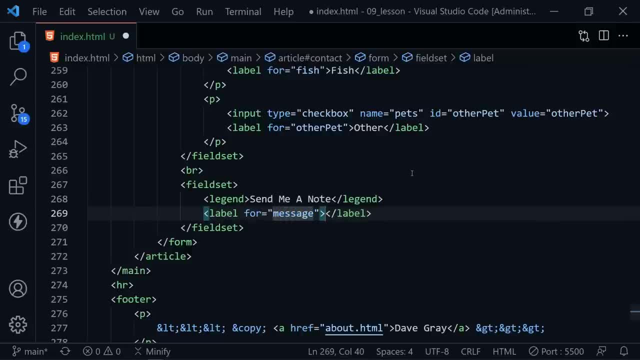 And in the for area We'll just put message, And here we'll put Your message, And now underneath the label, Let's go ahead and add a line break, Just to give it a little space, And then we'll add our input. 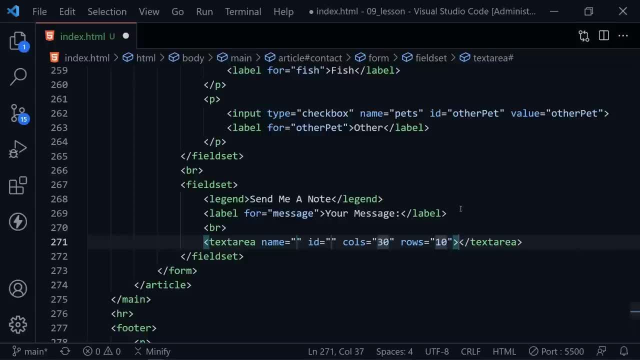 Which is a text area. This should have a name And an ID, And you can also see it's automatically given columns And rows. So for the name value We'll put message. Likewise that should be the same for the ID. 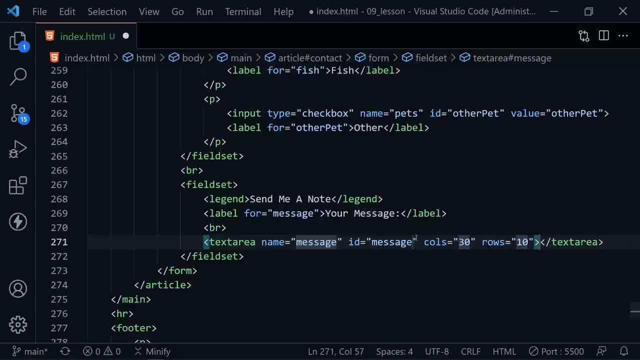 Since it needs to match our for And for the columns And the rows And the defaults here, that Visual Studio Code gave us It's 30 columns, That would be how wide it is, And rows, 10 rows would be how deep it is. 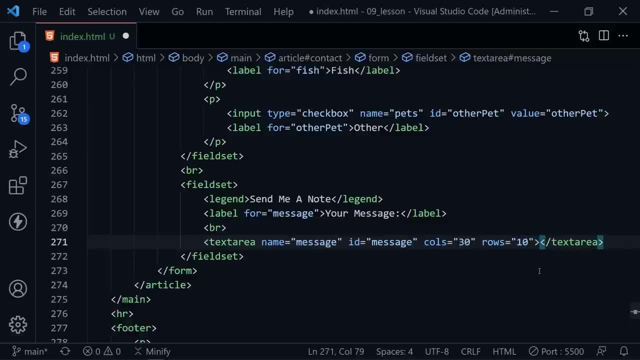 So now inside the text area here We could put a value already. This would be the value Or where the user would type. But I don't really want to do that. I want to leave it blank. But we can add some other attributes. 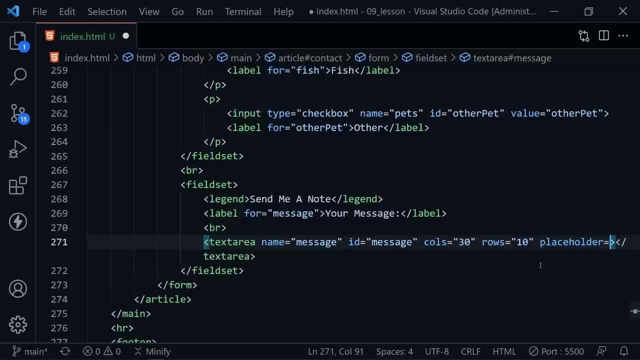 So for those attributes, Or attribute, I should say Let's add a placeholder, Type your message here, And then we'll just leave this blank. But if you were to put it here It would be like a text input Setting the value attribute. 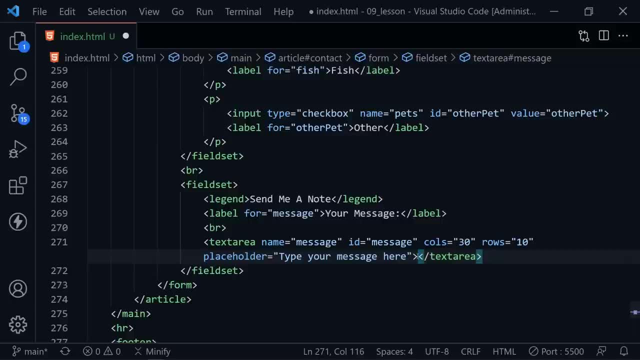 But you don't really do that for a text area. You would just go ahead and type Whatever you wanted to Right there, And it would be the value in the text area. So let's save this. And now let's look back at our form again. 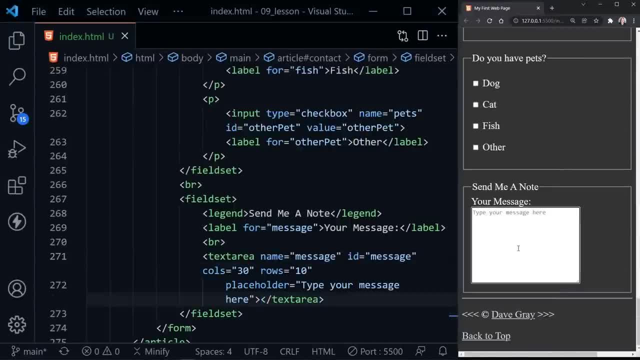 If we scroll down We can see an area Where we're ready to type a message, Which is My message. There we go, So that you commonly see, on a contact us form You might have a Area for the email. 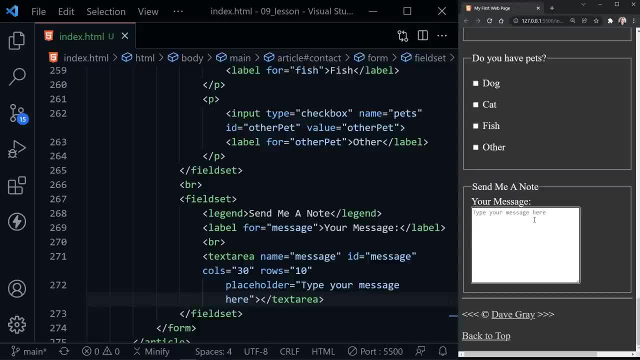 For a different message And so on. But this would be where you would typically type a paragraph, And I just mentioned email. That is another type of input actually, Besides text and passwords. So you could say it would be a type email. 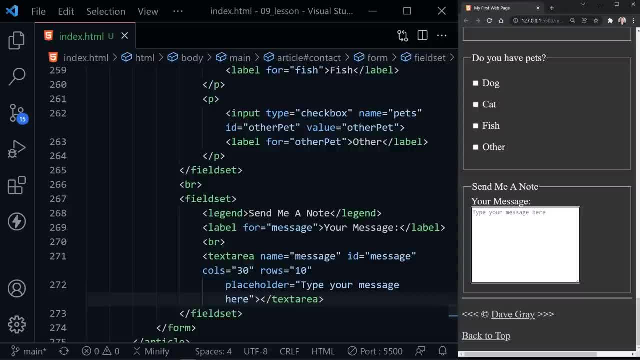 It looks like a text input, But it looks for the at symbol To make sure it's inside of the input as well. So I did not cover all inputs today, But we covered many of them And now we have a full form. 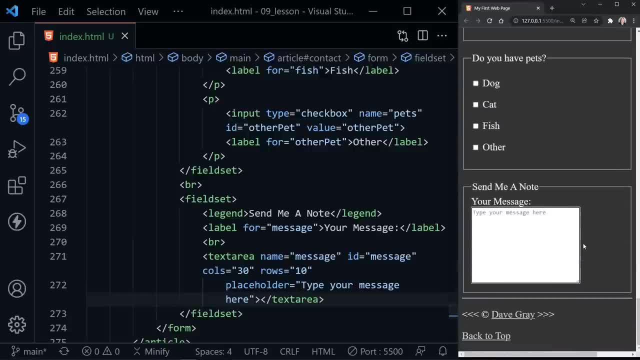 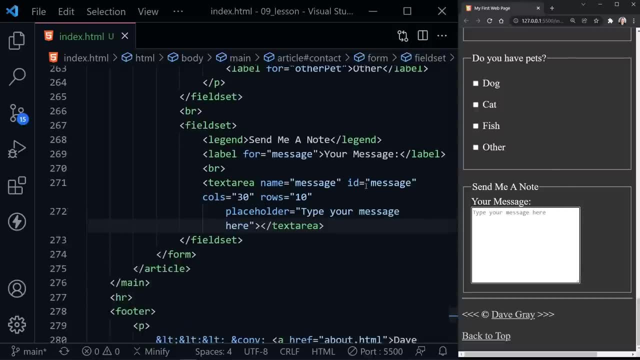 But we're definitely missing something. yet We have no way to submit our form After we fill it out, So we need to add submit button Or buttons at the end. Let's start out with one. So after that final field set, 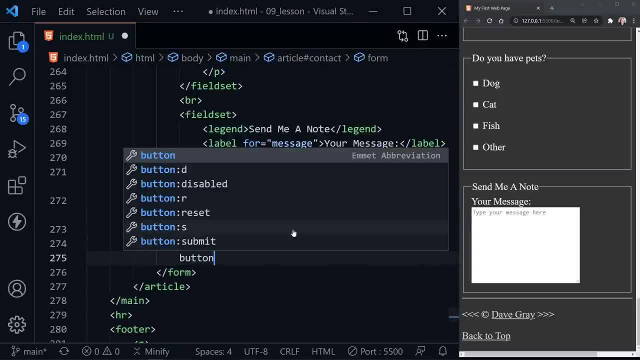 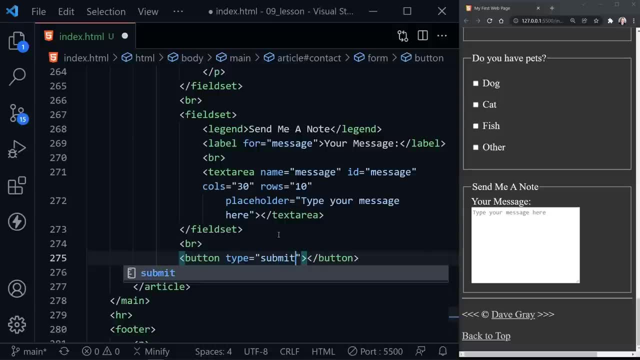 We'll put in another line break, And then let's put in a button element. Now a button element Should have a type. Let's set that equal to submit. Note: you might also see a form That has a type, And here we should put submit. 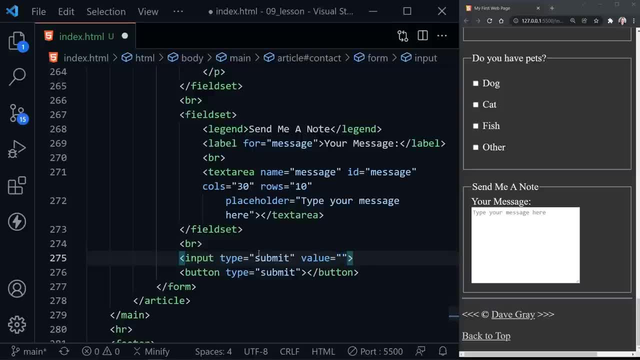 There we go, So you might see an input With a type submit, And that can also create a button. The main difference here Is that it only takes a text value And that's what will show up on the button Inside of a button element. 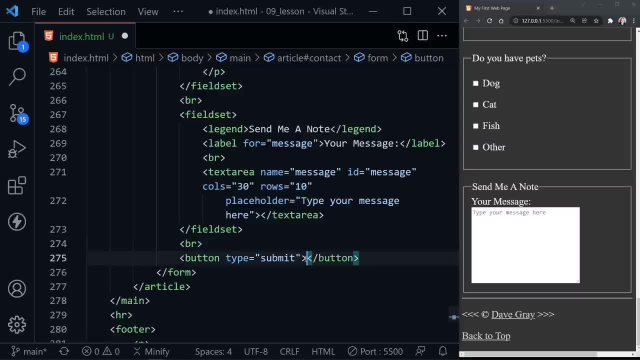 You could actually put more things Than just a text value Inside of the button element. So that is a big difference. I like to use the button elements overall Because once again It's a little more semantic. here We're saying it's a button. 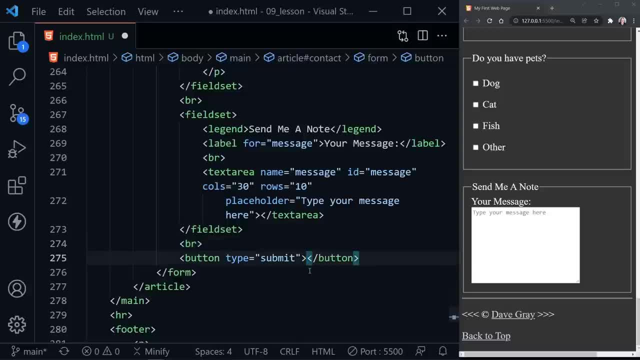 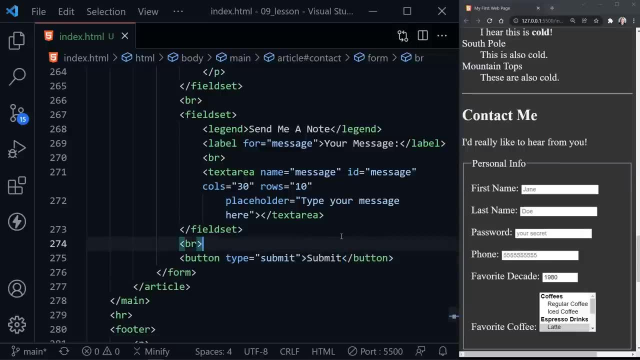 And then we can just set the type to a submit button. So here inside of the button, I'm going to type submit And that's what will show up On the button. So let's go ahead and save. And now, if I scroll down, 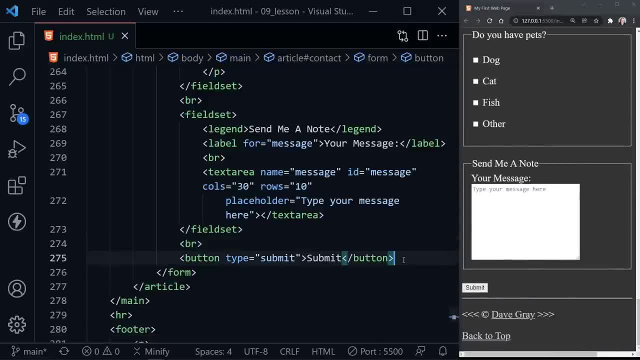 We can see our submit button here. That is ready. So let's go to And let's add it to our form And let's go back and put a type. Set this equal to reset. So if we wanted to reset our form, 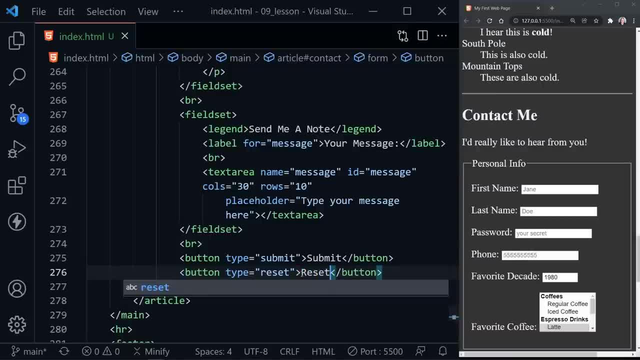 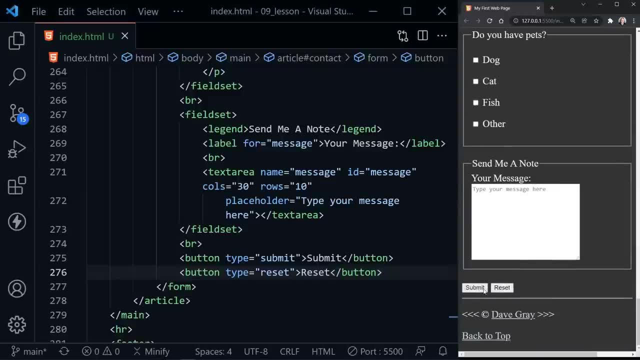 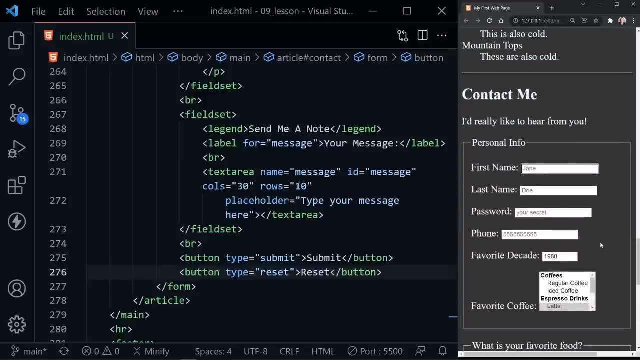 And clear out all of the values. It's fairly handy to have a reset button And every time I save It's going back up. But there we go: Submit and reset And submit. When you submit a page It checks the validation immediately. 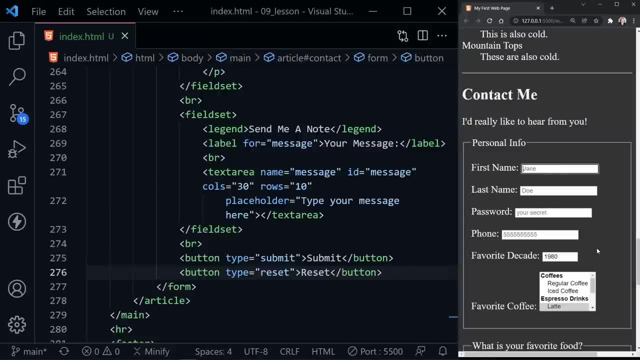 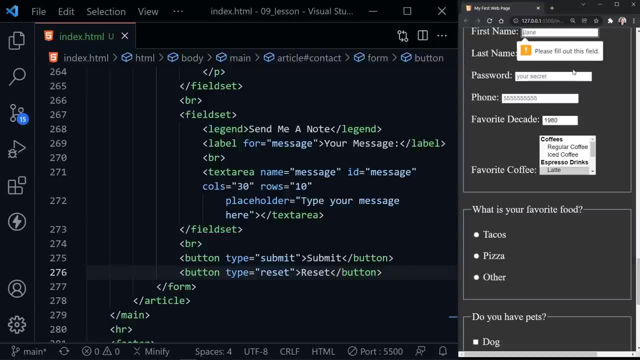 And when I click the submit button, It said I needed to fill this value out Because it's required And we didn't put a value in there, So I'll do that again. It instantly takes us up here And says: please fill out this field. 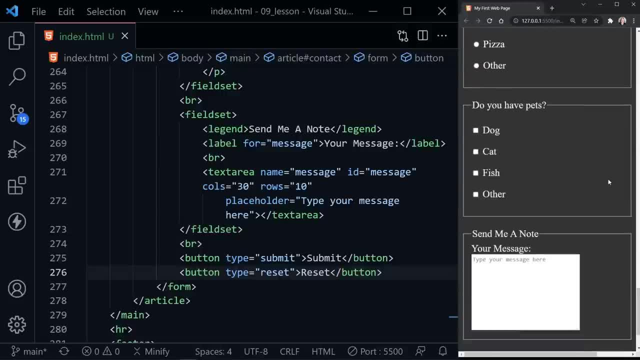 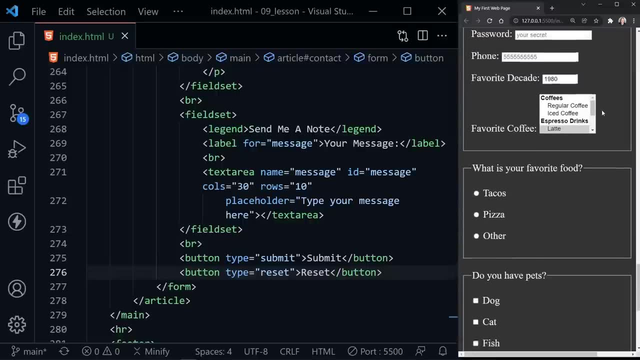 So we've got more than one required. Let me put Dave in the first name, Go back and click submit again. Notice it takes me to last name And says please fill out this field. So it's going to do that for every required field. 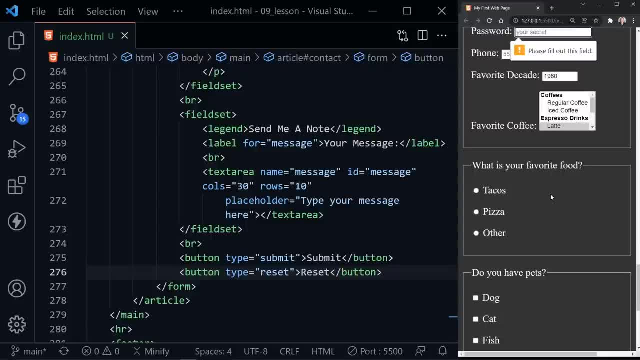 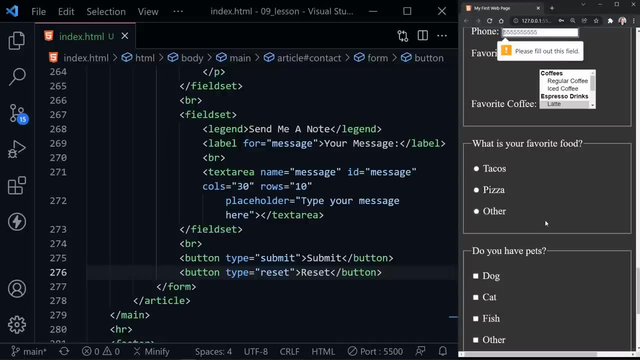 Until they're all filled out. So we can put in Anything in the password field, And I don't think we required anything else. Let's take a look, though Maybe we did. No phone number is required, So 123456789. 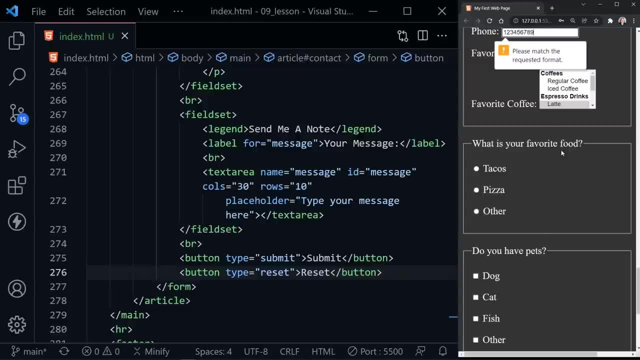 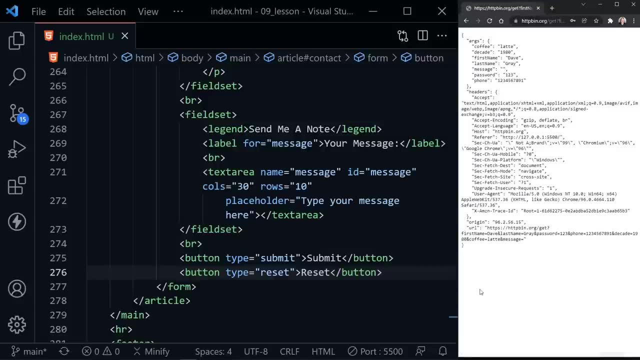 And let's leave it at that. And it says: please match the requested format. It knows we haven't matched yet, So I need one more number. That should be good Now. if I submit, It's submitted. Now let's go ahead and look at this. 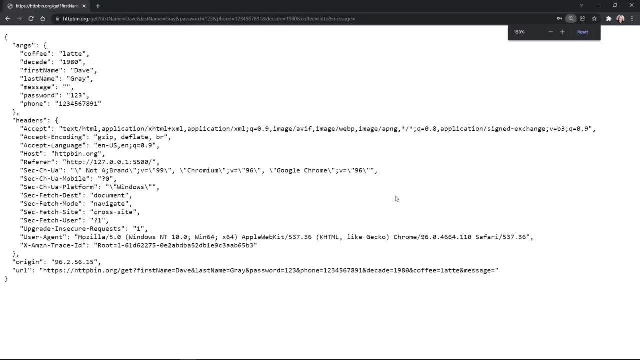 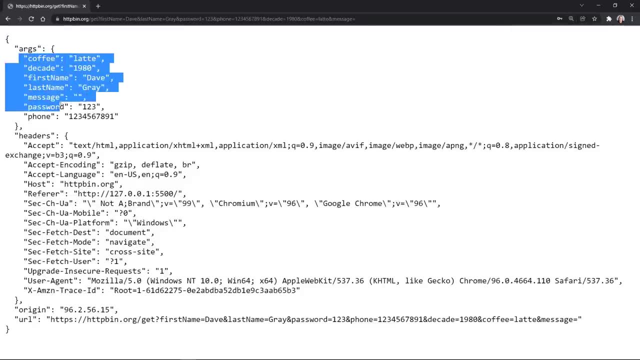 What are we getting from httpbin? And boy, that is bright, But I'm going to make this larger. We see it's labeled as args, Which means arguments, What we're sent with the form. We didn't have everything filled out yet. 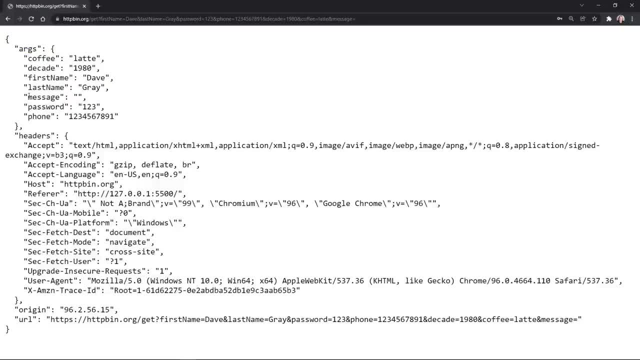 But it did send our default value For coffee and decade as well. We didn't have a message, But it did at least show that it was an empty message And it shows what else we filled out, Including the password. Notice that doesn't mean it's encrypted. 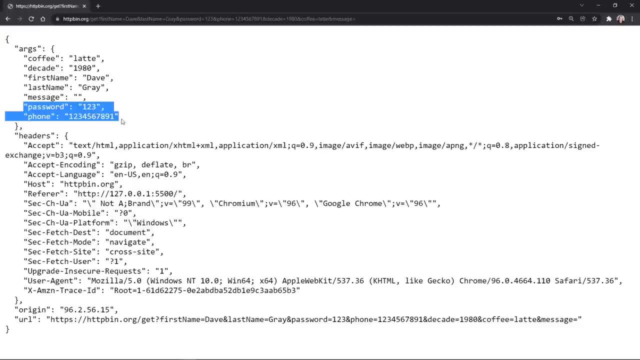 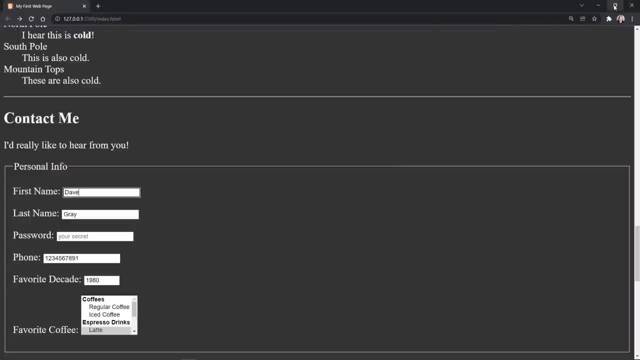 It just didn't show it to us as we entered it, So we're not sending any sensitive information to, But overall That is what we got, So we could fill out the rest of the form And see how all of that looks. 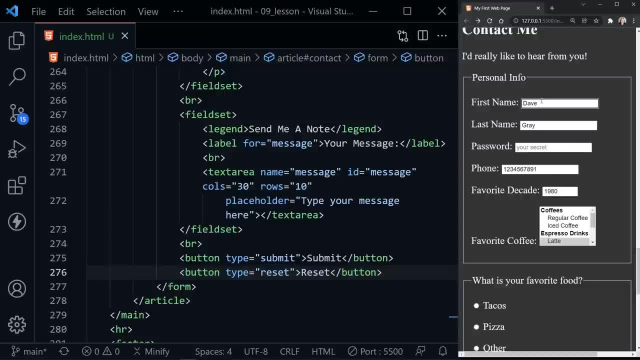 Let's resize the browser again. Boy, that is bright when we look at that information. But notice when we went back, The information is in all of these other fields But it's not in the password field. We would have to re-enter that every time. 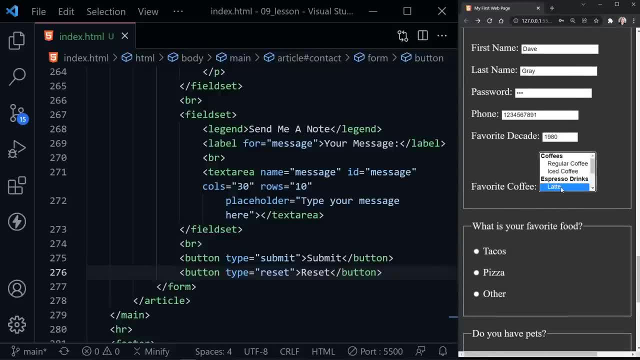 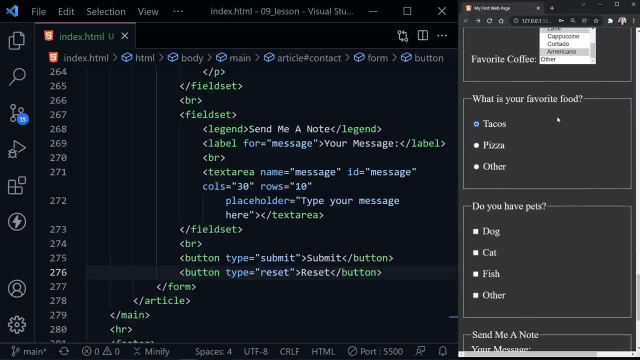 And that's just part of being with the password field. So for favorite coffee, Let's choose a couple. here I'm biased. That's my favorite Tacos is the correct answer here. Do I have pets? Let's go with dog and other. 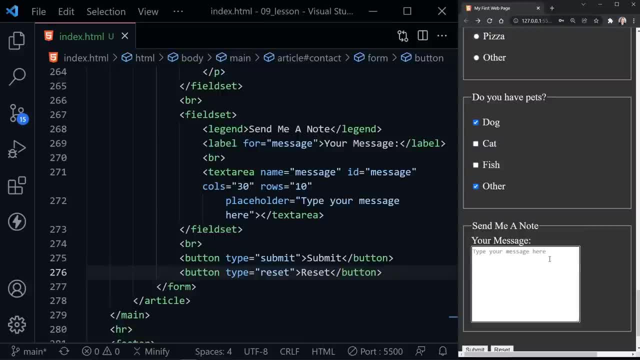 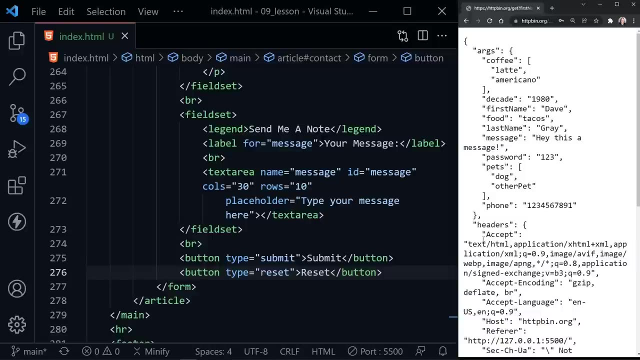 Because, well, I've got two dogs, really, And then we've got your message, So I'll just put: Hey, this is A message, There we go, Let's submit again. It's going to be bright, I know, But okay, nice, it fits on here. 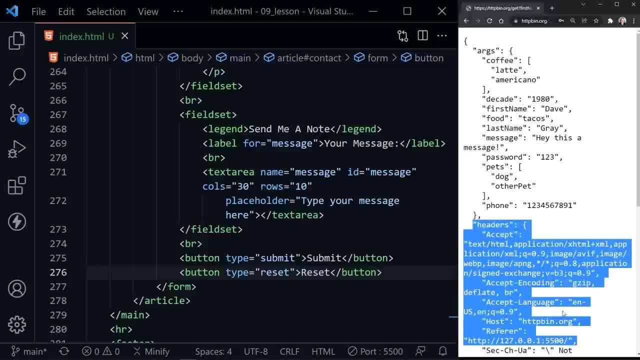 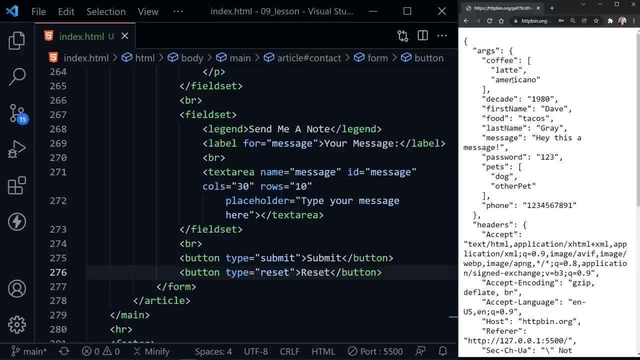 The rest of this down below is headers And just information about The browser. So that's server information, But this is what we're looking at. Notice now. coffee gave us both values. We got the latte and the Americano. We got decade. 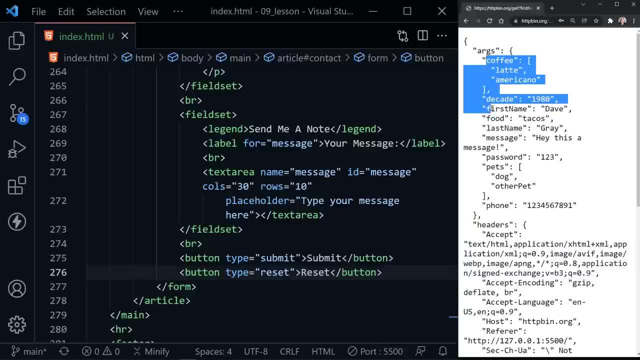 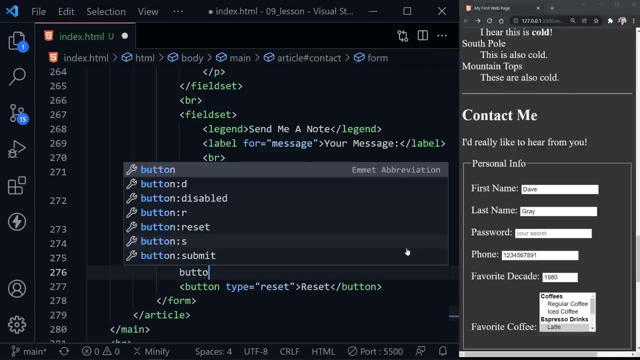 First name, Oh, and the server sorted this in order of fields, So food comes after first name. Before last name There's tacos, Last name And a message and so on. So we got everything we expected to right there And this one. 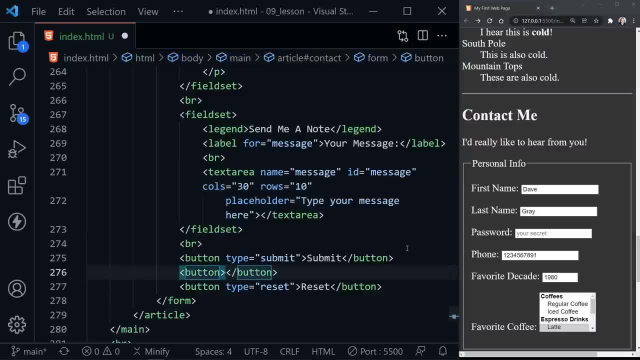 Will allow us to do something that we haven't done before And that is override What we are setting In the actual original form: Action and method. So this will also be type submit And you can have more than one submit button. 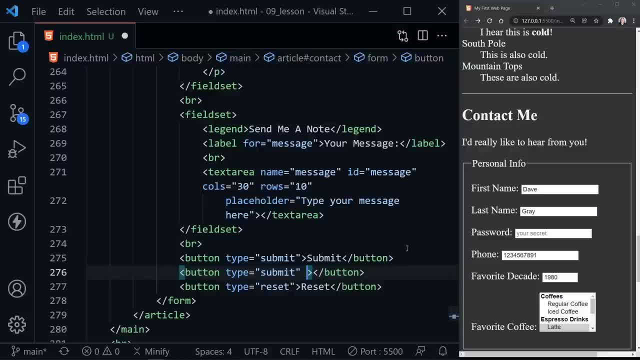 Per form. And now this, instead of just having an action attribute Will have a form action attribute, And here We can provide a different address To send the information to When we press This button. So I'm going to use a very similar address. 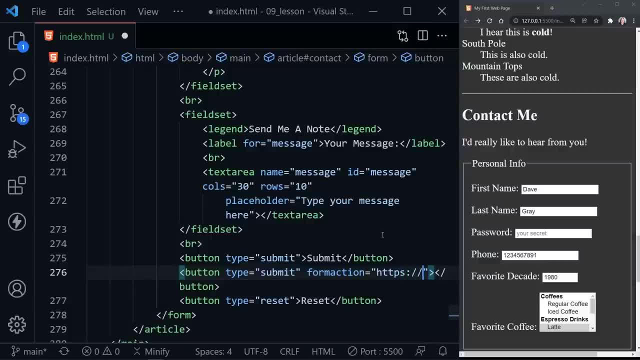 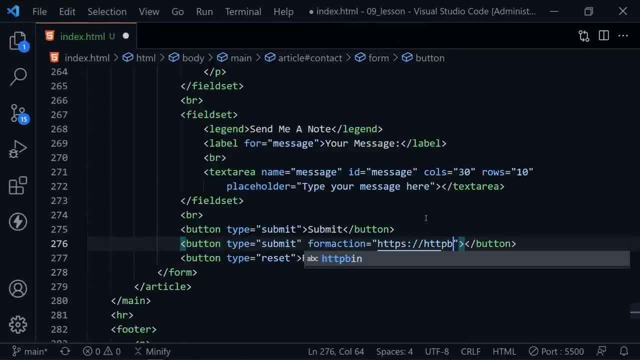 It will be to the same website: HTTPS colon, slash, slash. Let's go ahead and expand Visual studio code, So we have some more room here. There we go. httpbinorg slash post, So we're going to use the post method. 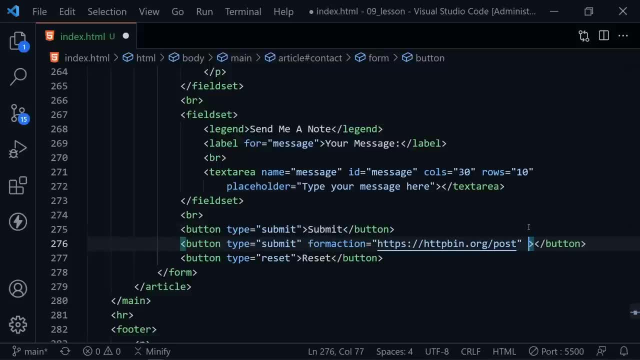 Instead of the get method. And now for the next attribute: Instead of just method, This is form method, And we'll set this equal To post. And so, on the button itself, Instead of submit, I'm going to put post. 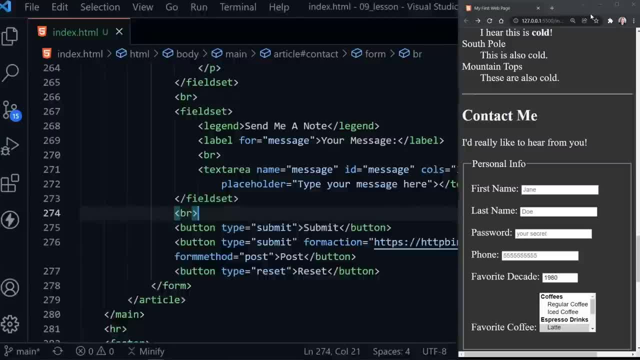 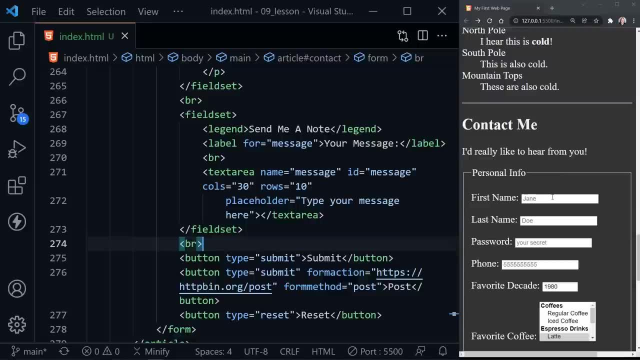 And we can save. And now this will allow us to submit the same information With a post Instead of a submit. Now notice: all the information is cleared out Because we successfully submitted before, So I need to enter in At least the required information again. 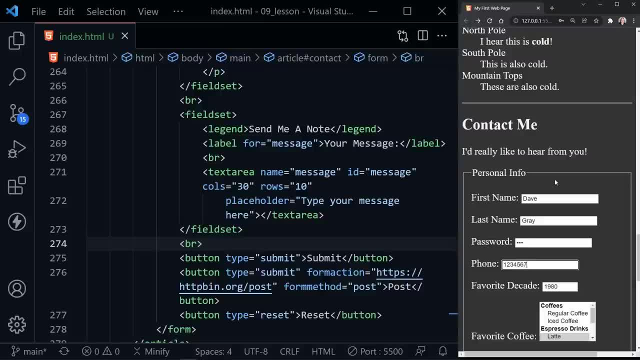 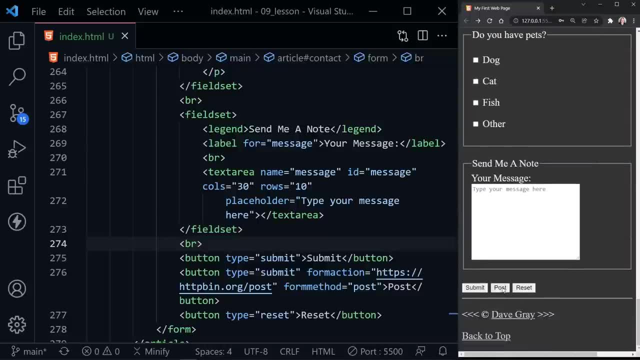 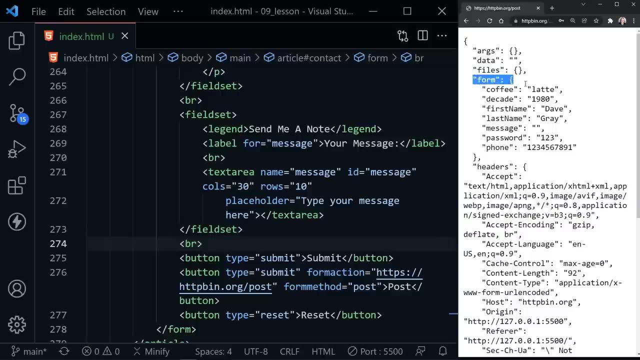 And I believe that was the first four fields: 79. Put a one there Should be good, And now let's go ahead And just press post And see what we get. So we sent it post now To the same website. 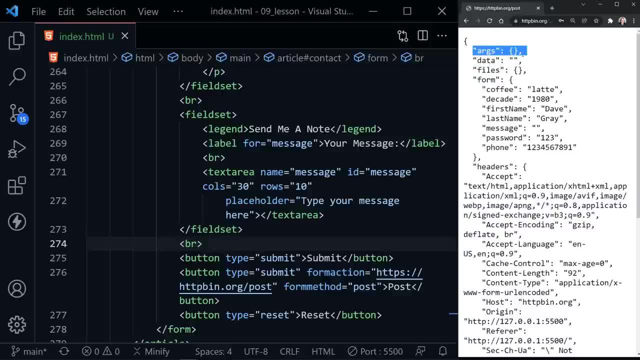 And you can see from the form, Not just args as they were processing With the get request. However, this is, of course, Just for this server. It could be processed differently on a different server. But we have our labels And we have the information from the form. 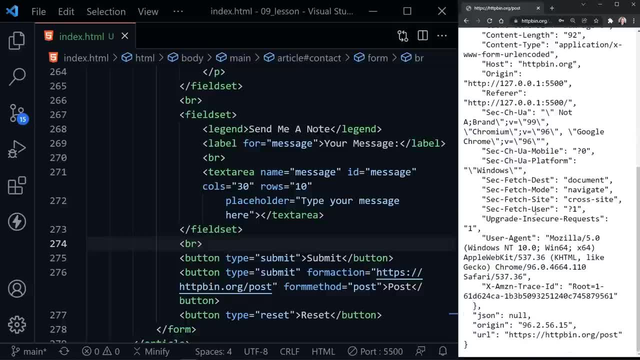 And what we note Is that it says the origin, Where it was sent from, And different things here, And it says the URL at the very bottom Where it was sent to, And that is what we specified. So now let's look at the same thing. 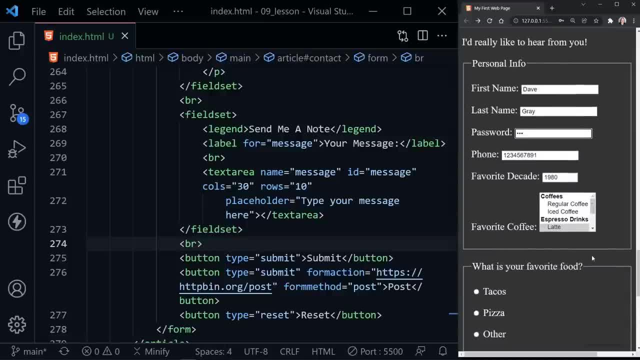 If we are to send this information And I need to put information back inside of the password. I guess it didn't clear out Because it was submitted before. I incorrectly said that It cleared out because we made a change And saved the HTML again. 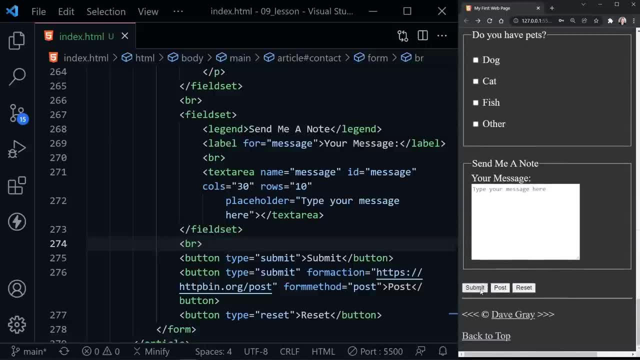 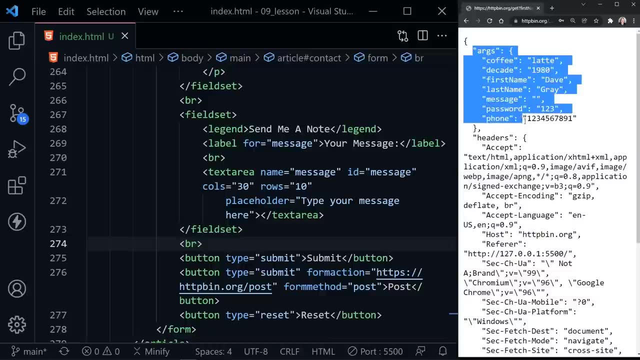 But if we scroll to the bottom now And just submit- And this, remember, is a get request, Not a post request- Now, of course this HTT bin Shows this as args Up here instead of under the form heading. But once again, 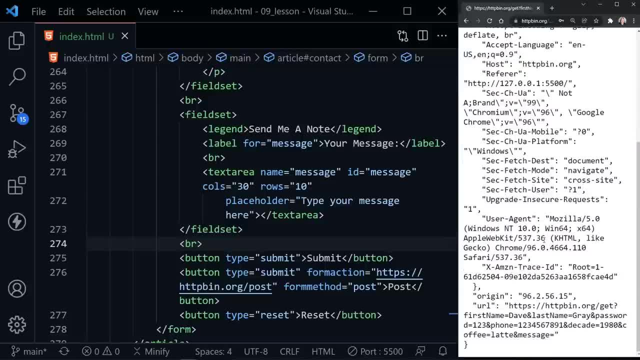 We get all of our information, But what I want to show you Is when I scroll to the bottom, Look at the URL. Now, all of our information Is shown inside the URL, And that is what happens with a get request, Because if we looked up here at this URL, 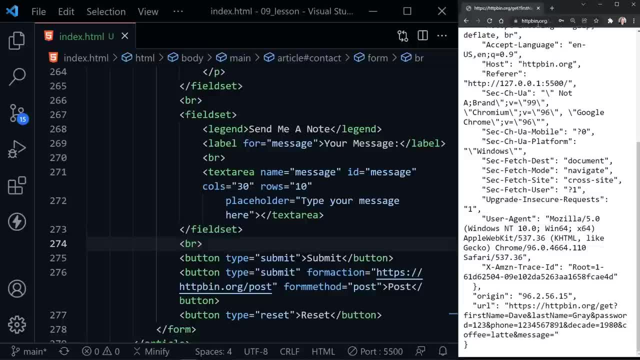 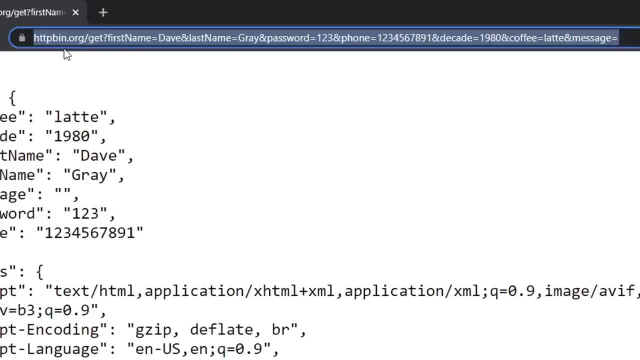 We would see all of the information Inside of it. Matter of fact, I will expand this. It will be bright again, But there is all of our information In the URL And that is what happens when you send a get request. Okay, 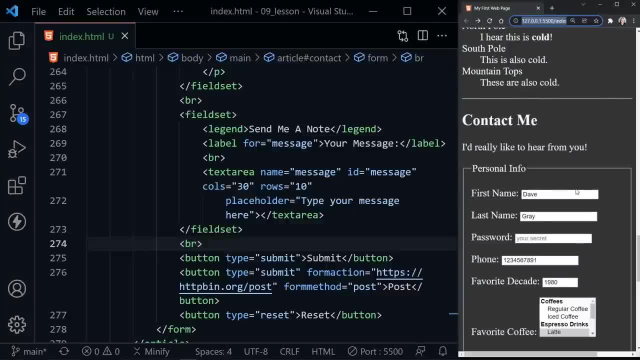 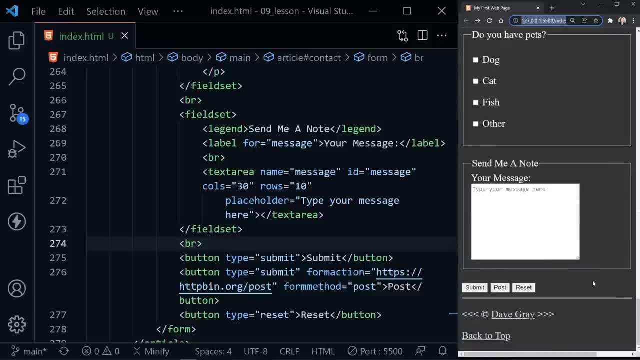 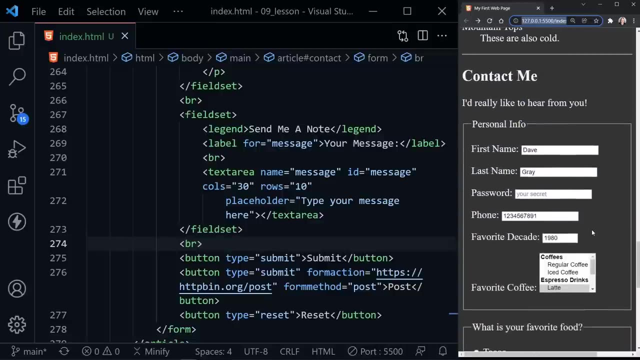 Headed back to our form Resize. So now you have added a full contact form To your HTML page And this is maybe a larger form Than you would often have. But overall We have covered quite a few inputs, But remember to follow the MDN links. 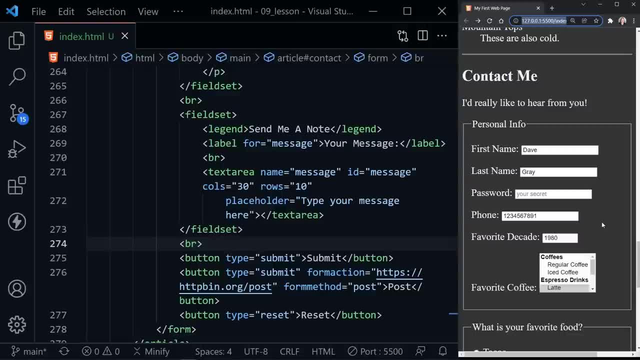 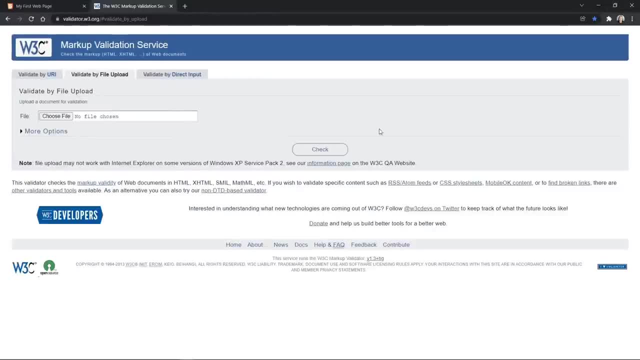 In the description, Because there are even more inputs That I did not have time to cover. Okay, we have reached the end And it is time to validate our page. Let me expand Chrome here, And we have got validate by file upload. 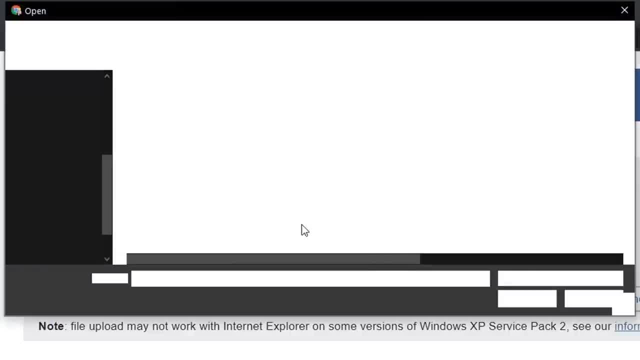 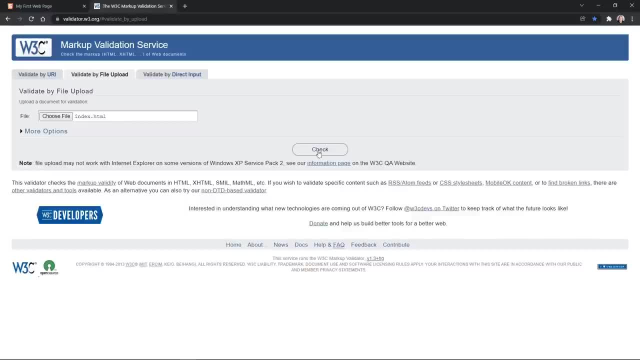 We are going to choose a file And I am going to be in my lesson 9.. And choose the index. You choose the indexhtml You have been working on And then we will click check Just to see if we have any errors. 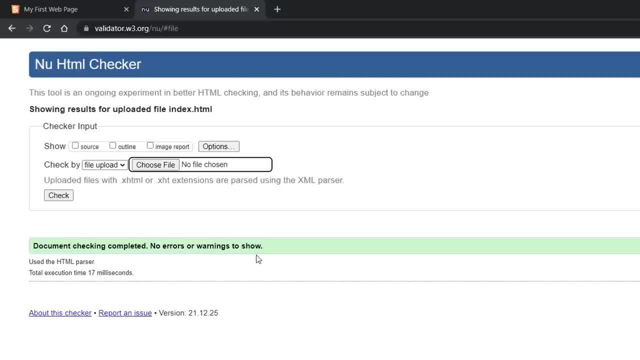 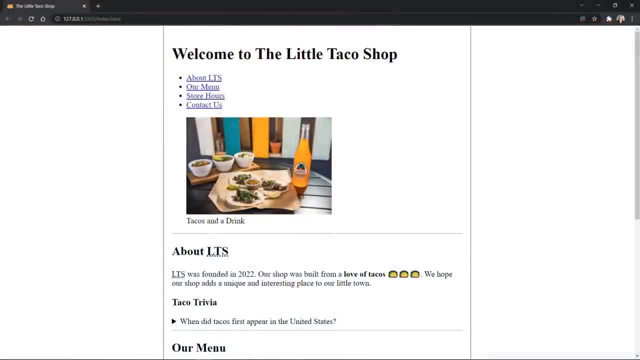 Or if everything validates. So we have got document checking completed. No errors or warnings to show. That is what we want. If you do have errors, It will highlight those. Welcome to your HTML project for beginners. You will be using everything you have learned. 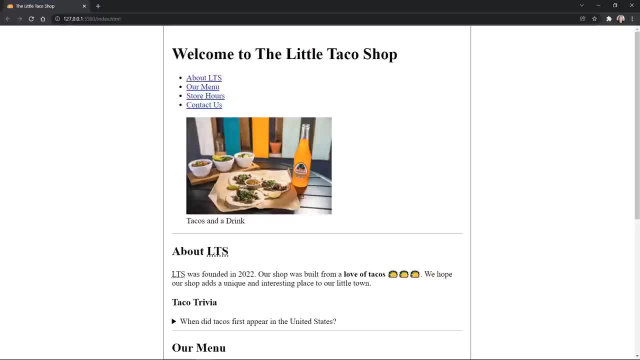 About HTML5.. To build a website for the little taco shop. Let's begin the HTML project. Let's get started by looking at the little taco shop website. So we have got a basic website Here that we created with HTML. It has a nav menu at the top. 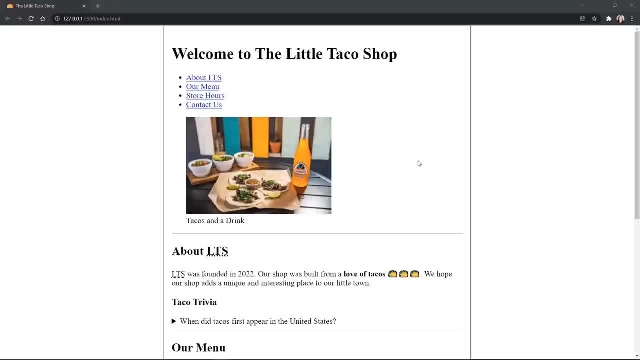 And an image here in the header, And then we have got a description That says about LTS, Which is an abbreviation for little taco shop, And we can see that linked in the nav. So instantly we know that is an anchor link And when we click it 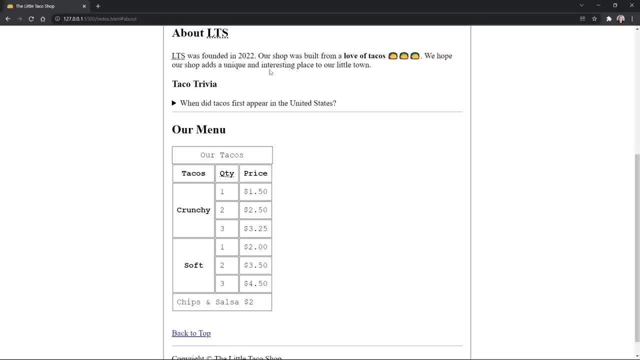 It takes us directly to that part of the page. It has some information About LTS And it even has some emphasis on text here Where it says love of tacos. We can see some taco emojis And there is a link in the directions. 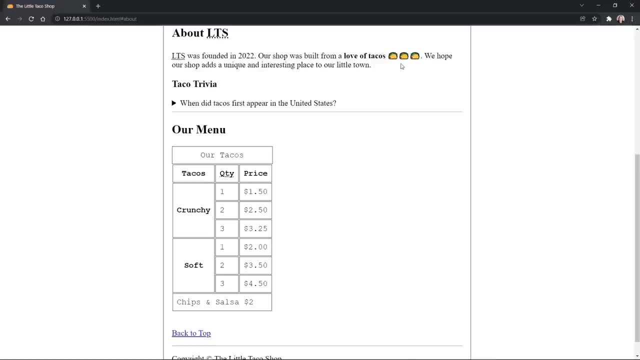 To Emojipedia, Where you can get emojis And just paste them in with your text. Emojis do work in HTML. There is a taco trivia section And you will have to go back in the lessons And remember how we showed something. 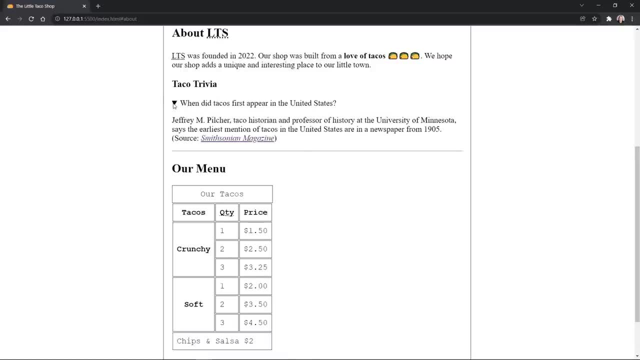 In the HTML And then we are able to click the arrow And it shows more information. This is all done with HTML, Not CSS. Very minimal CSS is applied And available in the stylecss File inside the CSS folder If we scroll back up. 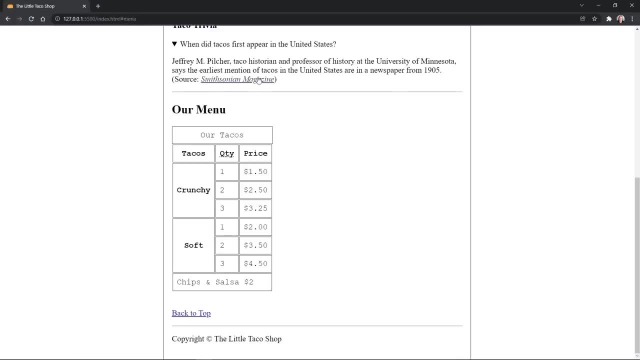 We can see there is also a link to our menu And if we click that It takes us to the part of the page That has the menu, And here the menu is a table. So you will have to go back over your knowledge. 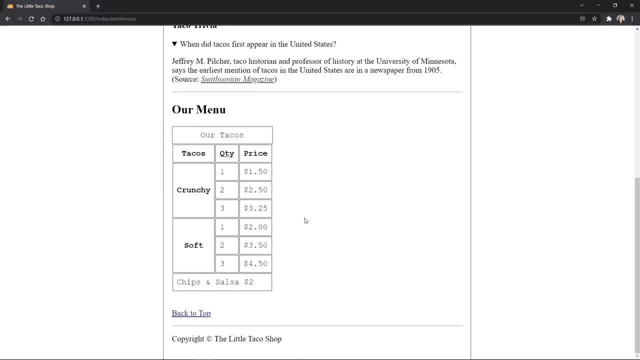 Of HTML tables And how to create this table. Once again, minimal CSS is already available And it will apply to the table As you create it. Of course, there is also a back to the top link And we have got some copyright information. 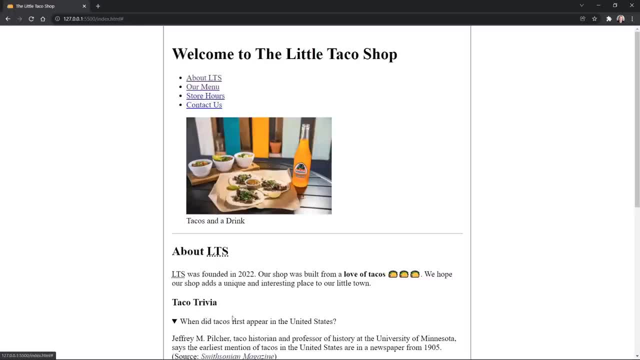 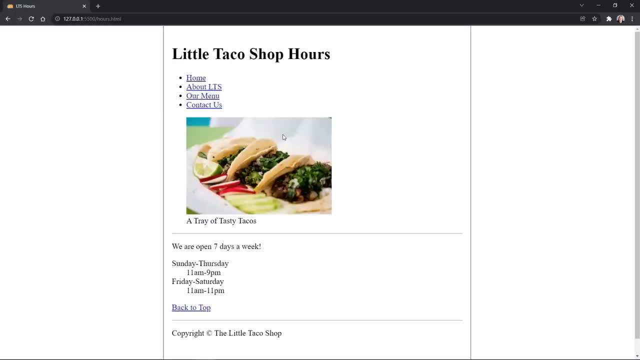 For the copyright sign at the bottom. If we click back to the top, We are back at the top And we need to look at the store hours page And once we click that It navigates to another HTML page. So we have got indexhtml. 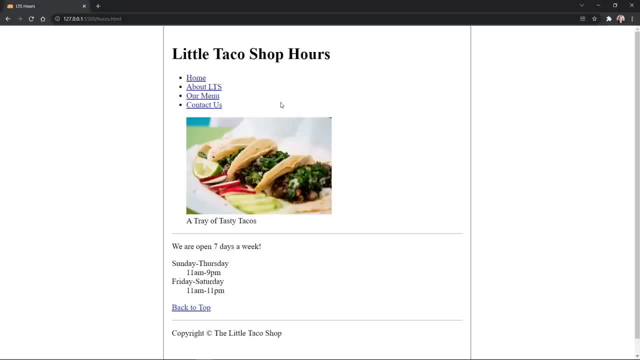 And now the second page Is hourshtml. It also has a navigation menu at the top. As you can see, it is an unordered list And you will need to remember how to create that. And now, Notice this is different. Now we have a link to the home. 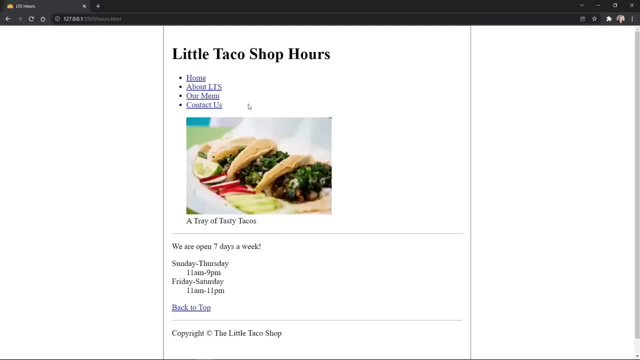 So it is not just the same navigation, It adapts to what page? Of course, And you will have to create that for each page. We have got another image, And once again the image has a caption, And then we have got the hours. 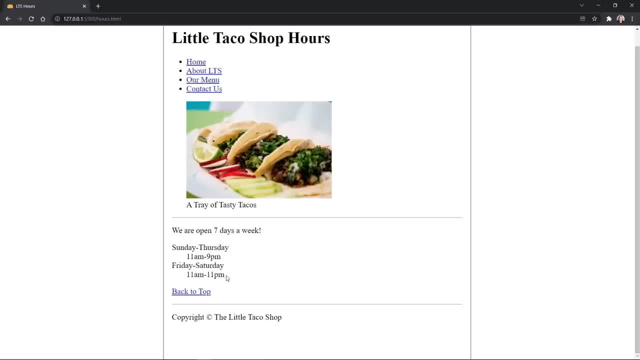 This looks like a list, But you will need to remember what type of list Creates a list that looks like this, Where it says we are open seven days a week, Which is a description, Such as a paragraph, But then this part starting with Sunday: 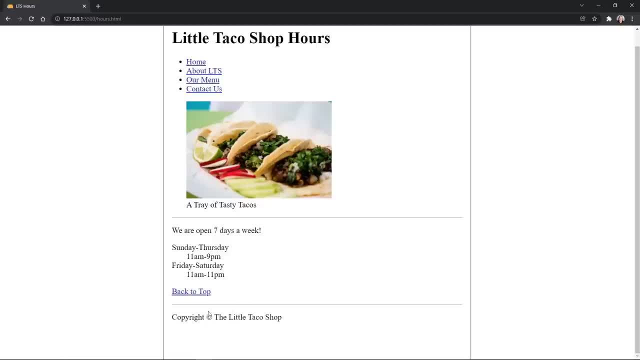 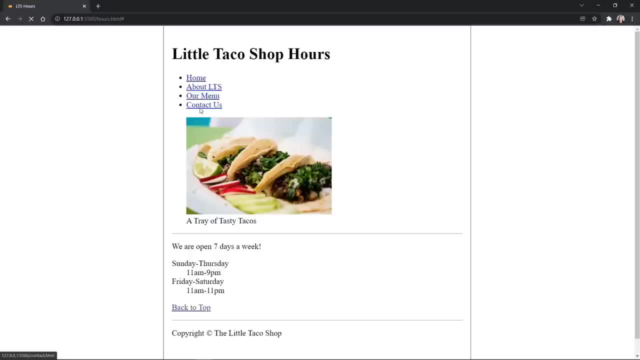 And going through the hours, We have got back to the top again And we have got the same information in the footer. So let's click back to the top And we have our menu. Now let's go to the contact us page. 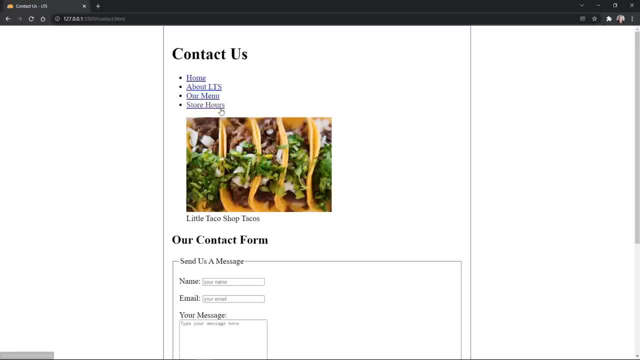 And on the contact us page You can see there is a link now back to the store hours And also links to home And the different parts of the home page. Now that is something to consider too, That we are not just linking to another page. 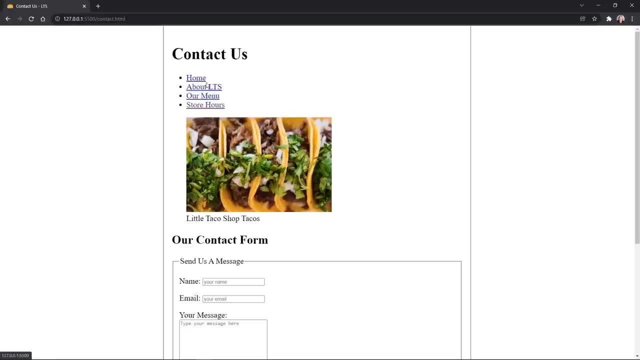 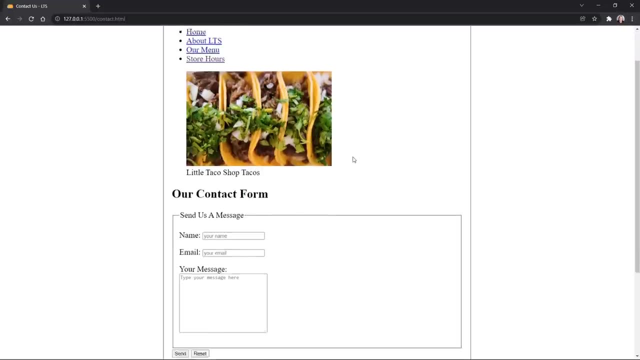 But we are linking to a section Of that home page. Then there is the image Little taco And we have got the contact form And you can go back over the forms tutorial To learn how to create this form And you can submit this form. 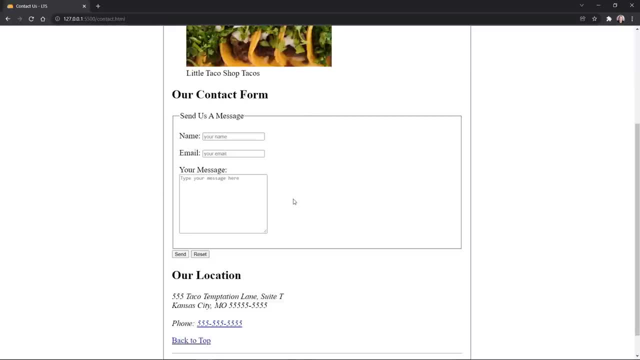 Just like we did in the forms tutorial. We aren't creating the back end That will process the form, But you can set it up to submit to the site We used in the forms tutorial. That will just show the information submitted, And then there is an our location section. 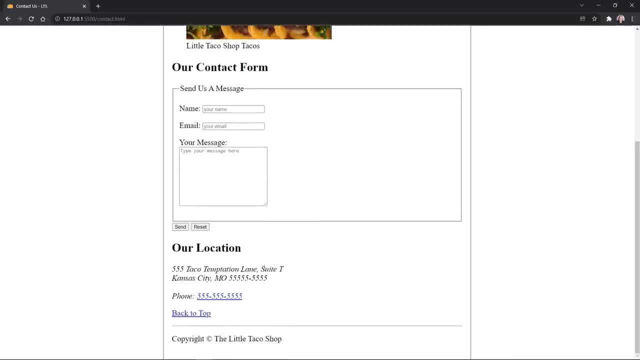 And if you remember the HTML element to use For an address, Then you can click on that For an address- This is what you want to put inside of that- And look The link to the phone number. And if you are on a mobile device, 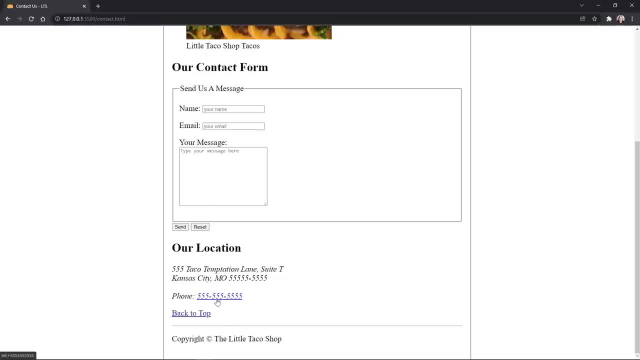 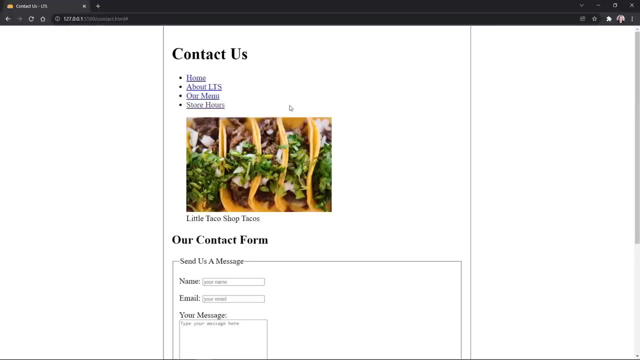 This, of course, is a false or fake number, But this should actually work as a phone number If you create the correct link. And we have got back to the top again, And that pretty much covers the site. But just to reference, Let's go ahead and click the about LTS. 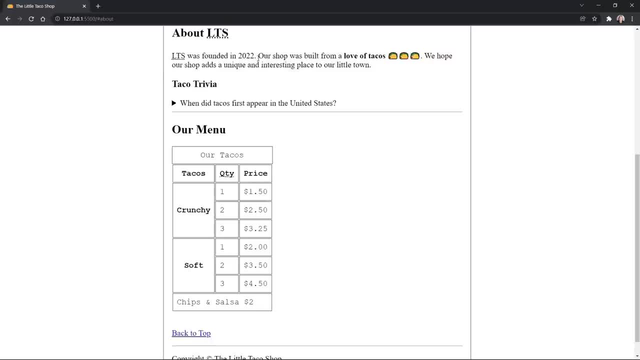 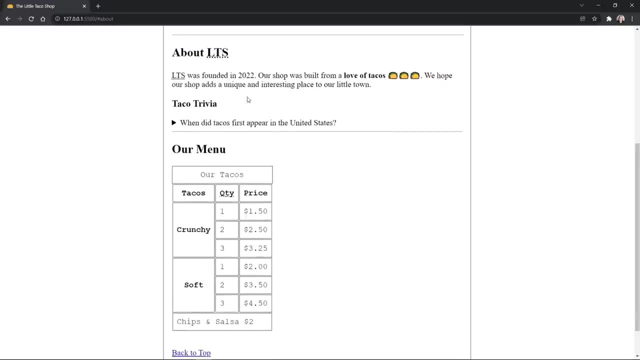 Which will not only take us to the home page, But to the specific part of the page. So you also want To be able to link to that specific part From another page, Not just on the page itself, Such as when we clicked about. 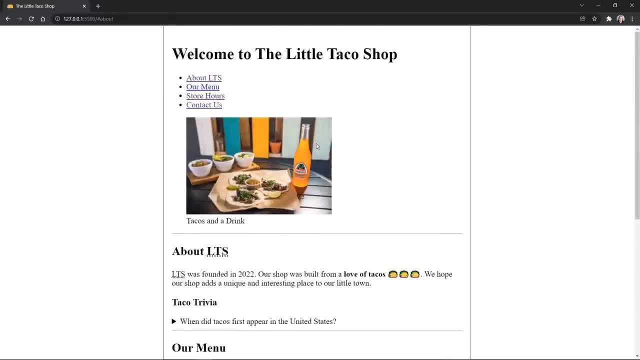 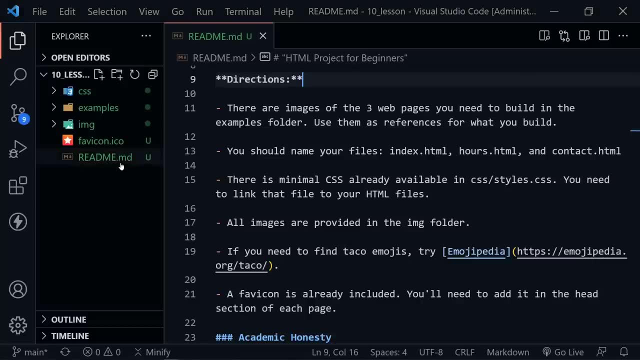 When we were on the home page And it took us directly there, So you can also do that from other pages. Now, as we look at the starter files For this project, Not only is there a readmemd file That has the directions, 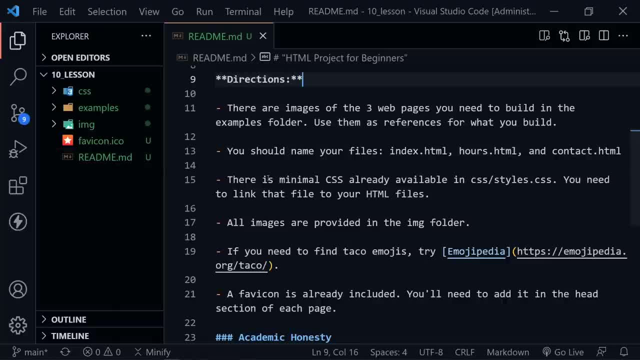 And these directions are in a markdown file. That is what md is, And this is making it very easy to read on GitHub, Where you look at the resources, And so you can also just read them in here Like this, But the other beginner files are already here. 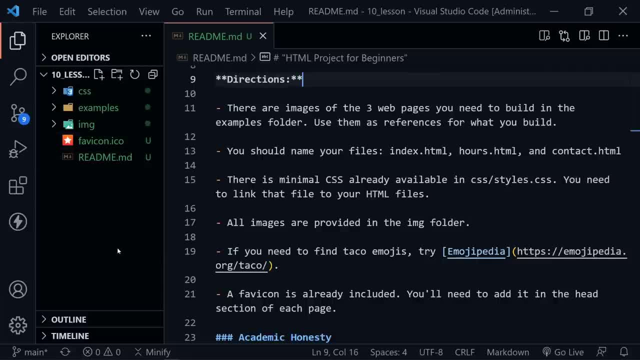 So you have already got a fav icon That you would link to in the head of each page. You have already got some CSS Inside of the CSS folder And you can link to this stylecss In the head of every page As well. 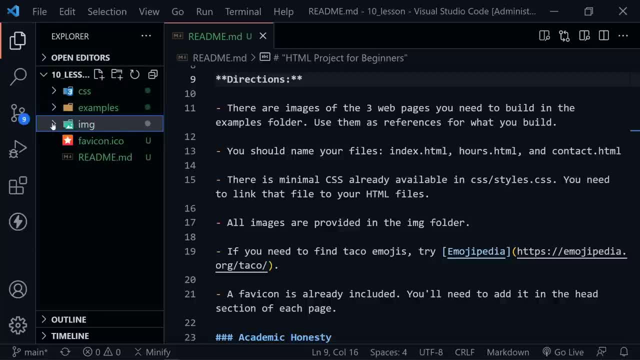 You have got all three images, One for each page, here, And you have got some examples, And these examples are important Because you will want to go back and reference that You don't necessarily have to always go back And pause the video. 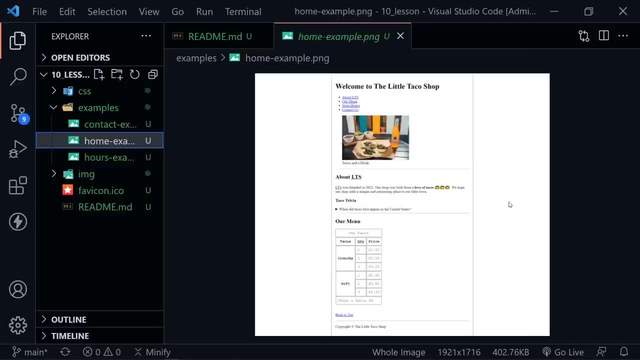 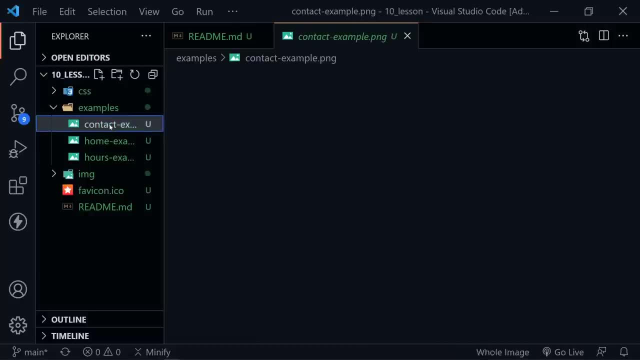 You can just click on the image, And I have made full screen captures Of the entire page So you don't have to scroll. You could zoom in a little if you want to, But you have these to reference. So here is the contact page when it shows up. 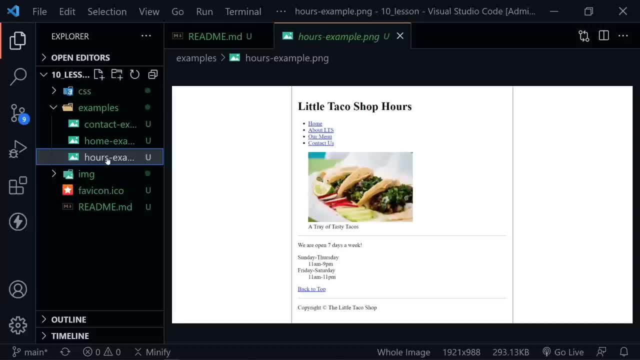 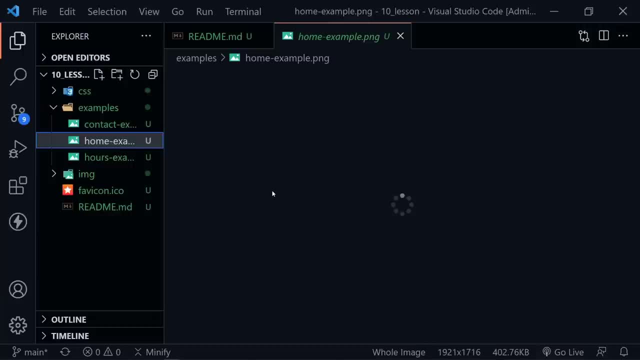 There we go, And there is an hours capture as well. So you have got one for home, One for hours And one for contact, And you can reference these visually To show up inside of Visual Studio Code. Of course, you could open these image files. 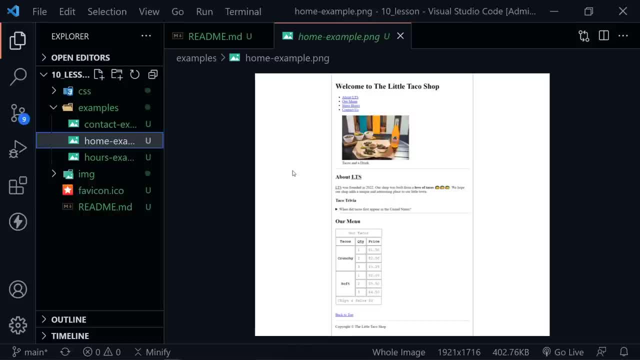 With some other software, If you want to as well, Or directly in the browser, And just keep different tabs open To view each image file. if you want to, That would also work. So there you go. You have got to create three HTML pages here. 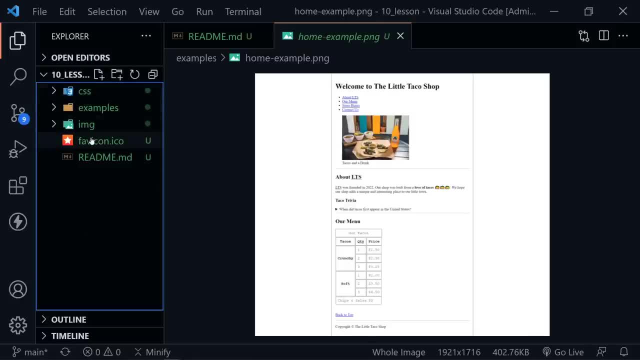 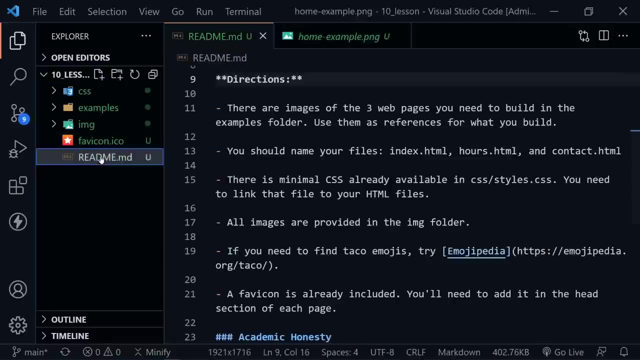 In the root of your tutorial folder And then reference these other files And you have got the examples to look at And you have got the favicon file Already as well. So let me go back to the directions. Let me see if I left anything out. 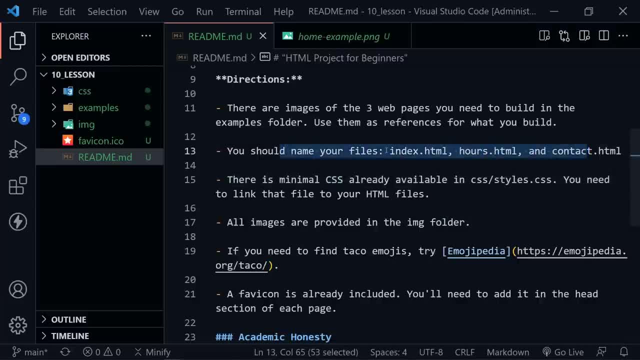 You have got your files all named: Index, hours and contact. We talked about that Minimal CSS available inside of the styles file, Stylescss. All images are provided And if you need taco emojis, Here is a link to that as well. 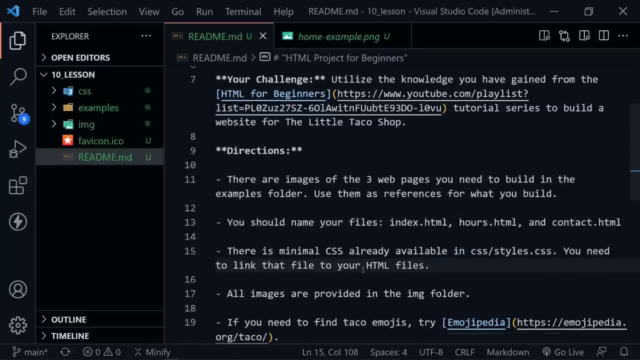 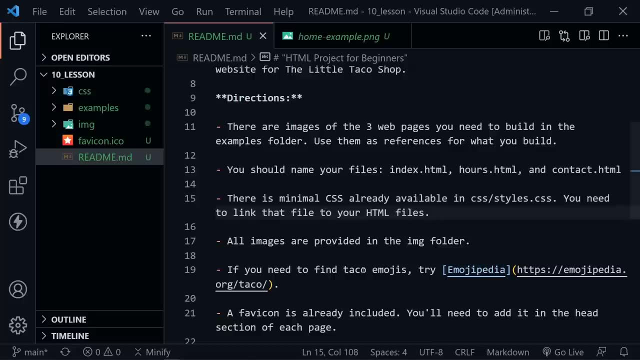 And the favicon is included. So that is everything. Good luck with the challenge. And then, of course, after this, You want to pause the video And look at your ability, And then I will walk through And create these pages with you. 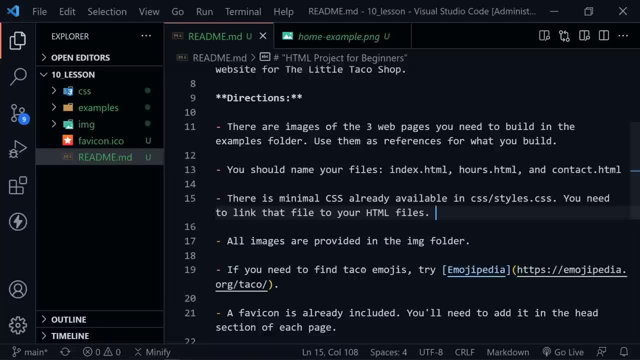 For the solution afterwards. So don't do that now. Pause the video And actually attempt it on your own. That is the best way to get better at something. Try this out for yourself Before you allow me to walk you through it. 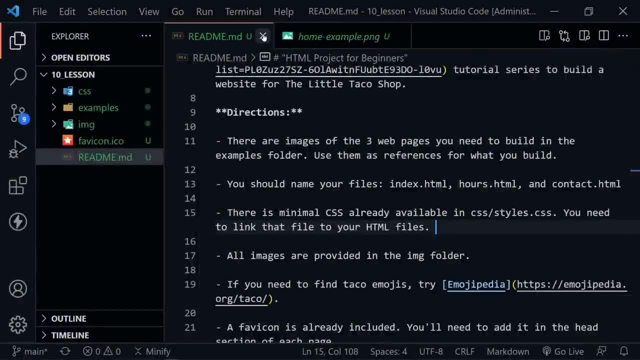 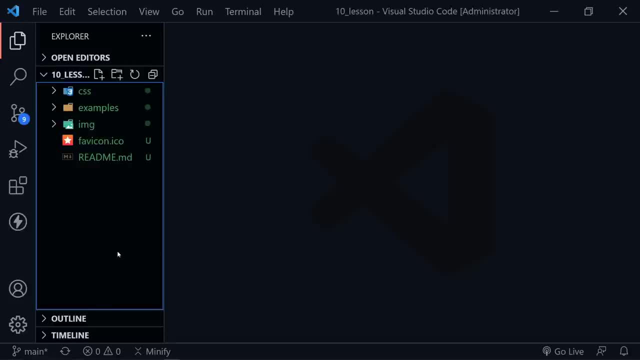 Okay, Let's get started building our project. I will close this readmemd And I will close any image file, Or, as a matter of fact, I will collapse the examples And we are just going to create the three HTML files That we need first. 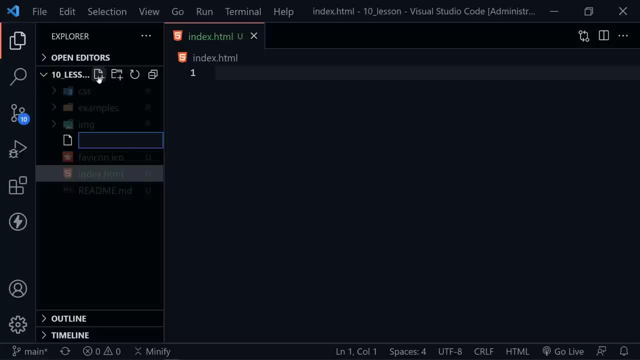 We need indexhtml, And then we also need Contacthtml And, if I remember right, We need ourshtml. Okay, With our three empty files created, Let's go ahead And start on the first one, Which is indexhtml. 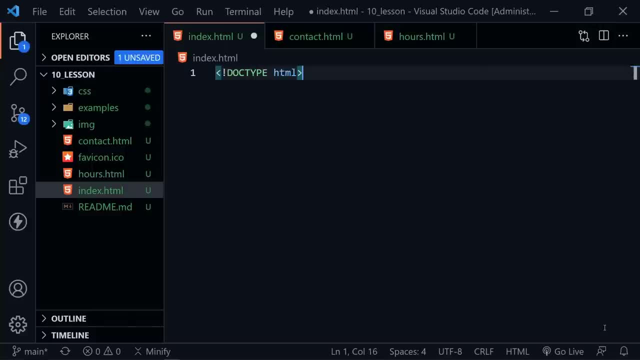 We know every document starts with Type And if I press tab, It adds the HTML From there. we know we need the HTML, I need lower case Or I prefer lower case, And then we need the attribute lang And that equals English. 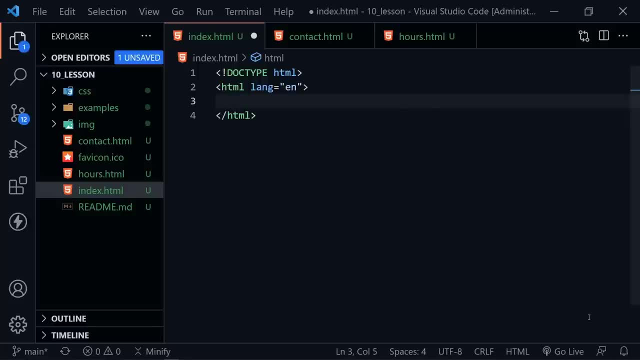 Is what I will put. Of course, you could put something different there. If you want to. We instantly get the closing HTML tag. If you don't, of course, add that as well. From there, let's create the head section And I've got the closing head element. 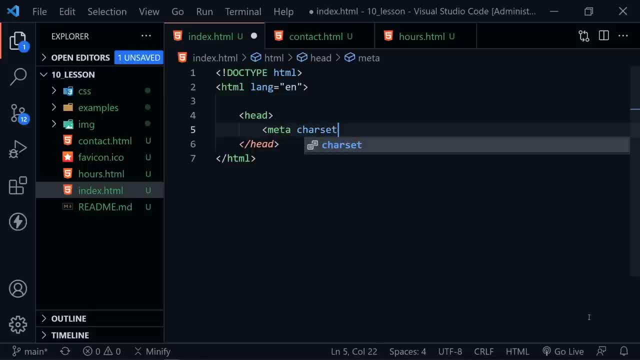 And this will contain several Meta elements. The first one has the character set attribute And we specify UTF-8.. After that, Have another meta And this is going to be Name equals author And of course, this should be your name. 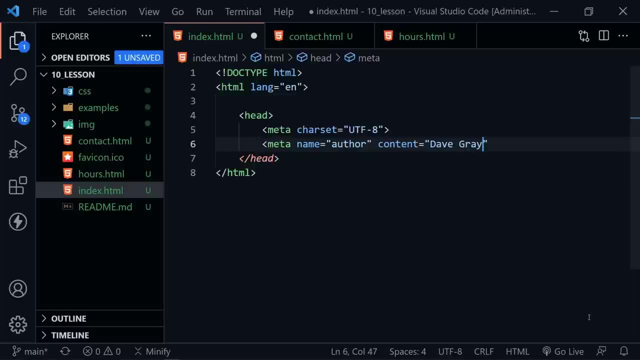 I'll put my name here, So Dave Gray. After that Meta Name equals description And this is where we describe the page. So once again we have a content attribute And I'm going to put The official website For the. 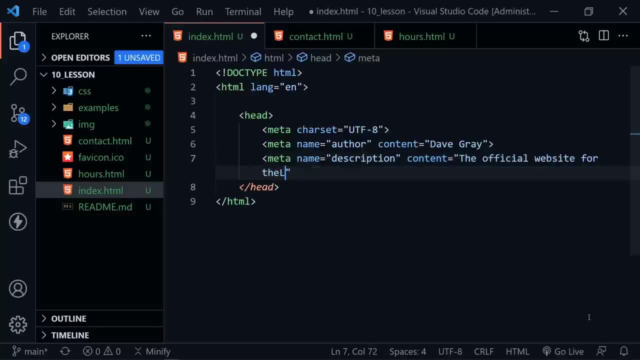 And I need to press Alt Z to wrap the code here. Little Oops, I didn't get a space Little Taco Shop, And I should really put a capital T There as well, Because it's the official name. Okay, so we've got the Little Taco Shop. 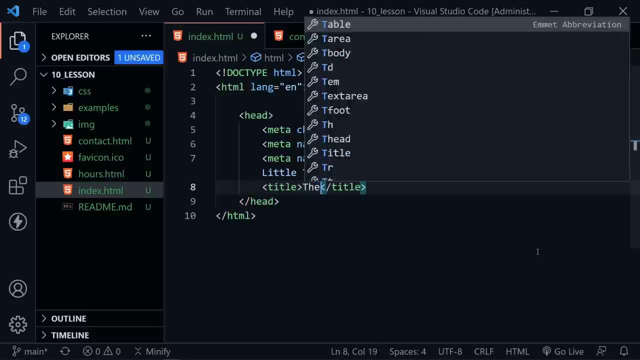 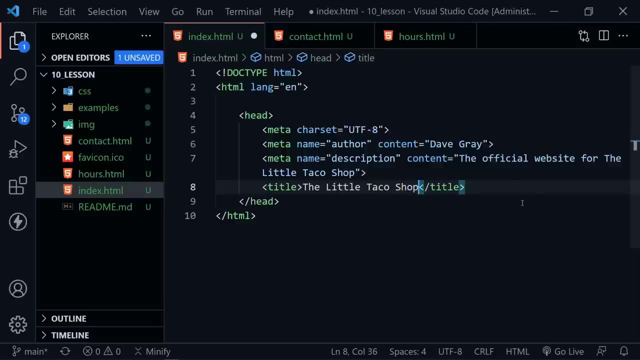 And of course that's what our title was For the page as well. So we want the Little Need to spell this correctly- The Little Taco Shop- In the title as well. After the title Let's add a link, And here we're going to say: 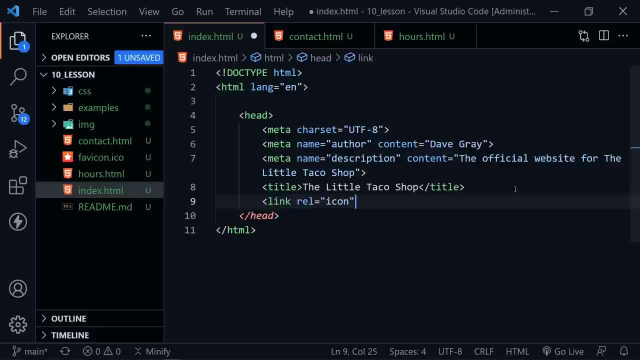 REL, Which is related. It's an icon And the href, And now let's put in that fav icon That we have And after that We can close our link tag And we're finished with the head. So I'm going to press. 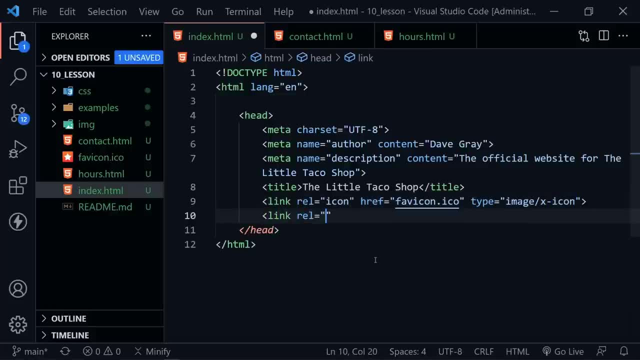 Control S to close, And then we want Style CSS, And after that We can close our link tag And we're finished with the head. So I'm going to press Control S to close, And then we want Style. 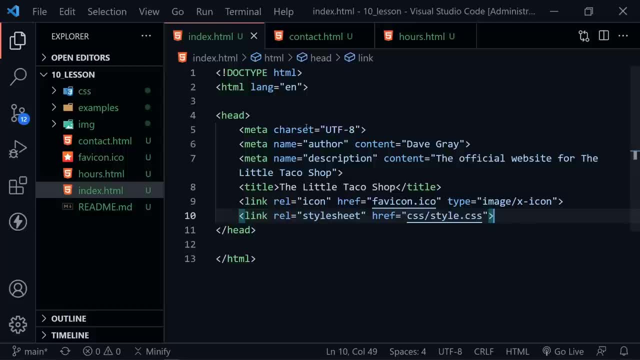 CSS. Now I could copy this much And paste it into the other two pages And just make a few changes, But I'm going to do just a few more things Before I do that. So just underneath the head, We'll start our body element. 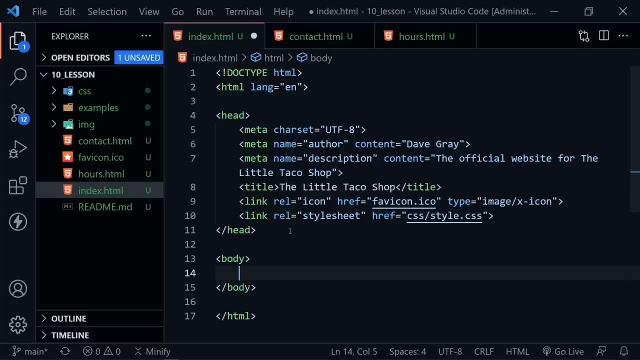 And then in the body element, We'll start with a header element. Inside the header element We're going to have an h1. And we'll say Welcome to The Little. Still not typing that in? There we go, The Little. 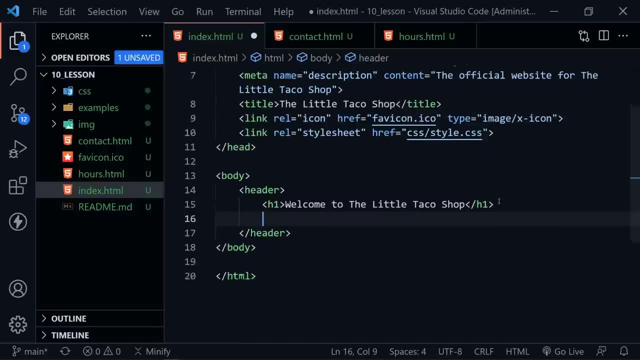 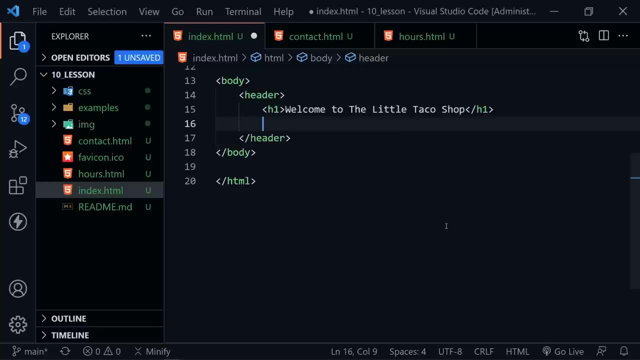 Taco Shop, And that is our h1 heading for the page. Remember, every page should only have one h1 header. I'll scroll up now for some more room, And now we'll start our nav element. This is where our navigation menu will be. 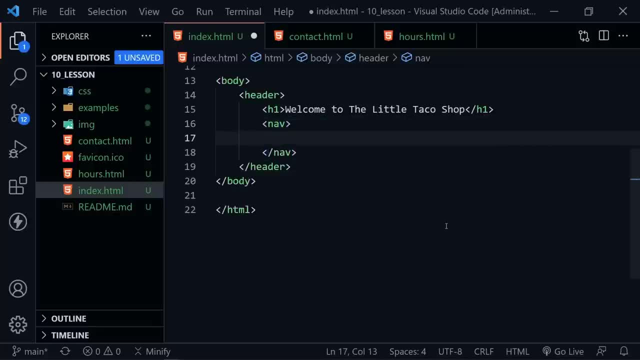 We get that closing element Inside the nav element, We're going to have an unordered list And then each list item Will have a different link. So here we'll start out with. Let me put A line in between. There we go. 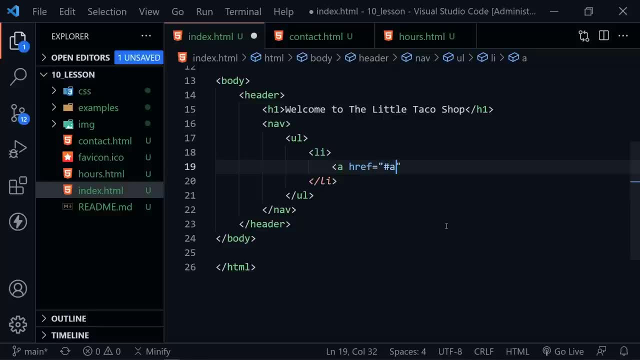 Let's start out with our anchor tag And the href is going to equal Hashtag about. So this is going to link to an about section on this page, So I'll say about, Right there, And then after that Let's go ahead and put an abbreviation element. 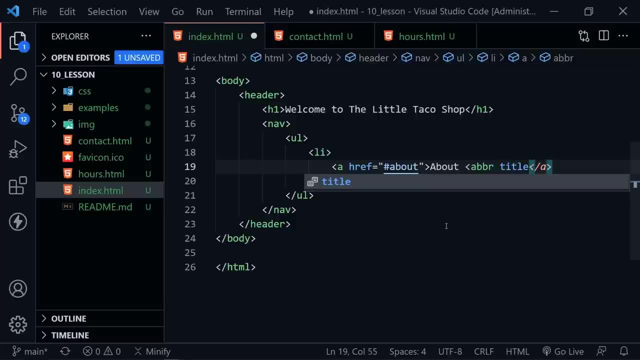 Inside of our link And here we can give a title to this abbreviation And this will be The Little. I spelled it right that time And then we'll close that out And since we're abbreviating, We'll put LTS. 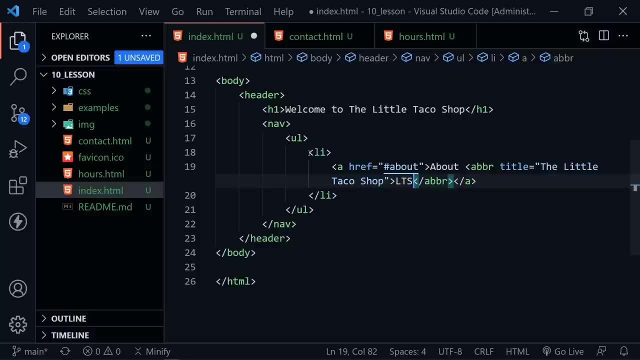 So our link says about LTS And now we can just Copy this link item down, So highlight the full LI And then I press control, alt And the down arrow. It should be the same for you on Windows. It may be a little different on a Mac. 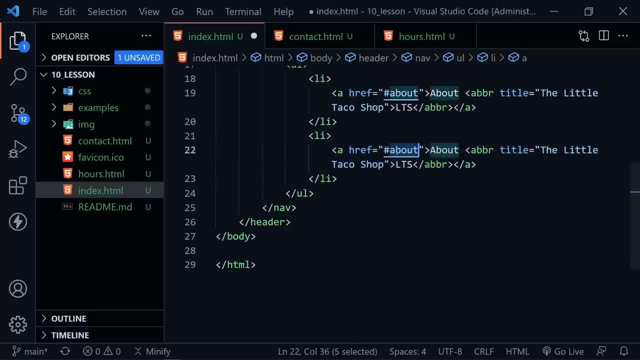 Or Linux. Now, the next link is much easier here, So we'll just say about Menu. I want all lower case again, So no abbreviation for the menu. So it's just About menu, Or I'll put our menu. I think that's what's actually on the page. 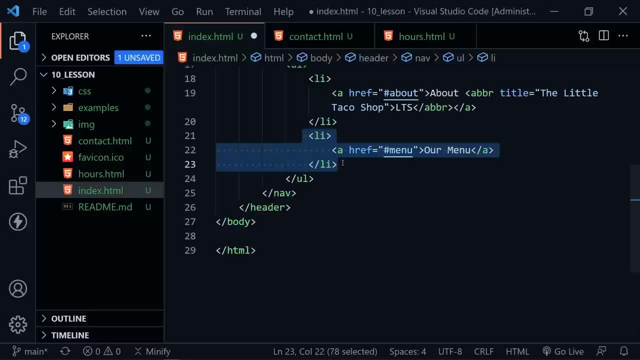 And then from there We can copy this down once again A little easier for the next link, And let's copy it one more time. There we go, Three our menus. Let's change this second menu To HTML, So we're linking directly to another page now. 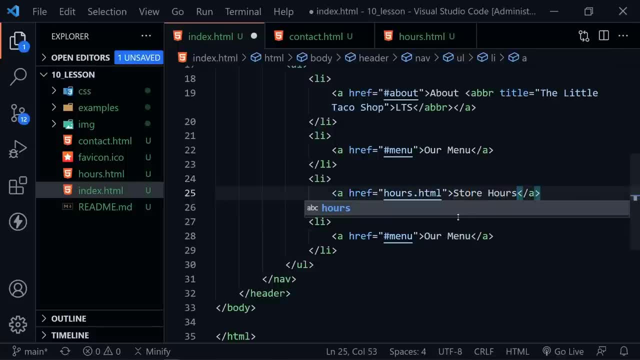 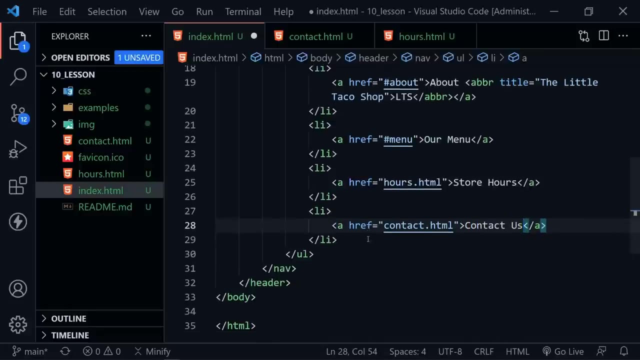 And then we can put Store hours. And then for this last one, We'll remove the hashtag menu And we'll put our contact Dot HTML, And then we'll put contact us here Instead of our menu. Now I'm going to scroll. 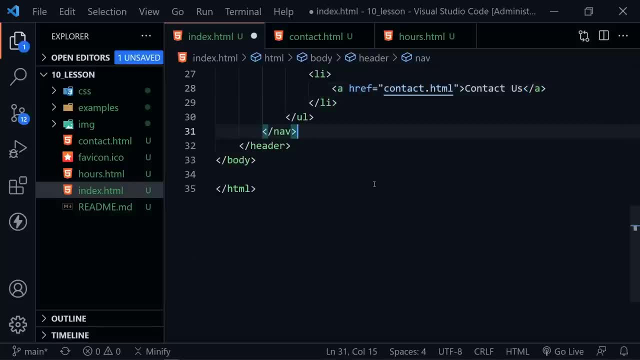 Just a little bit more And while we're still in the header, Out of the nav, But in the header, And then inside this figure, We'll add our image. So here's our image element And we'll give it a source. 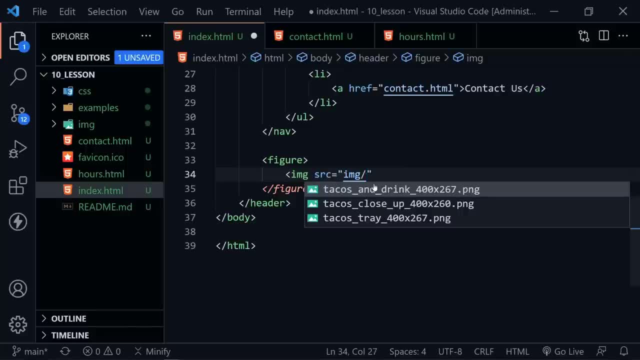 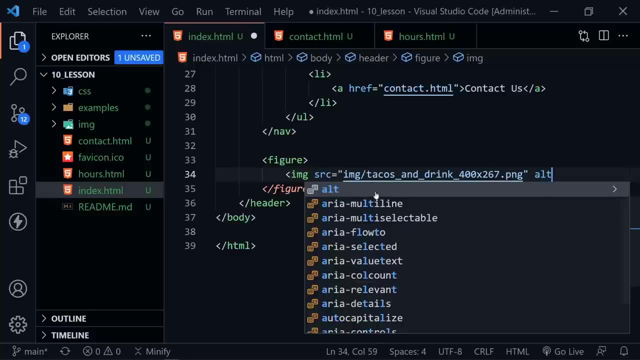 Equal to. And then we want to specify our image folder. And then let's pick our tacos And drink image And once we have that image, We can add some alt text for that That actually says what it is. So we'll put tacos. 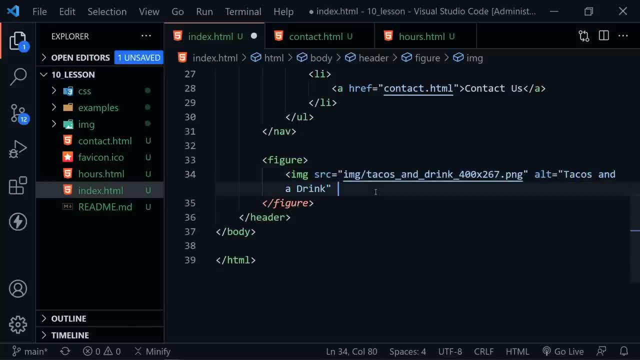 And a drink. Remember. alt text makes our images more accessible. And then we have a title And we'll say: We love tacos. The title does not have to be the same As the alt text. And then let's provide the width. 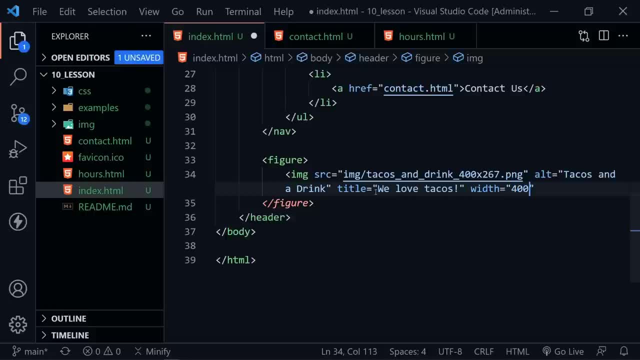 And I notice I saved the width and the height In the image name, So the width is 400.. And then the height Equals 267.. And we can close out our image tag. But we're not quite finished with our figure yet. 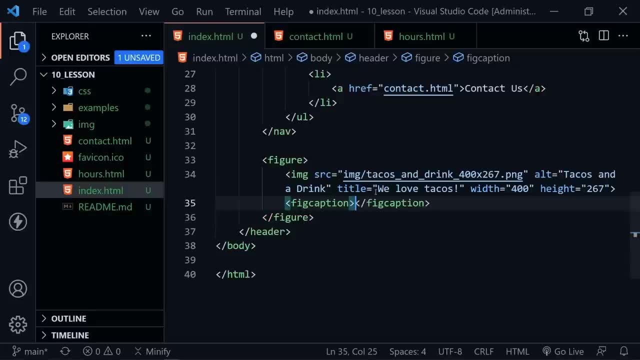 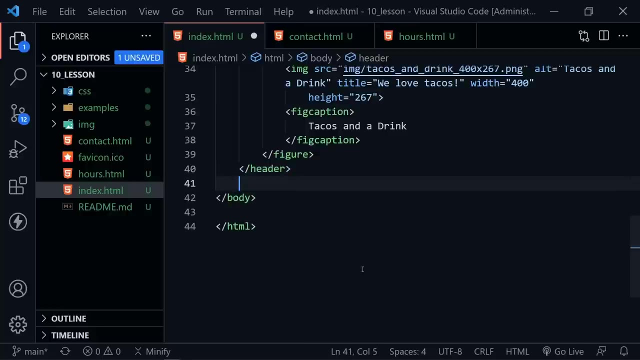 Let's go ahead and add a fig Caption element And inside this, Once again Tacos and a drink As our caption for the image. Okay, Now we've completed the header, So let's once again scroll up for some more room. 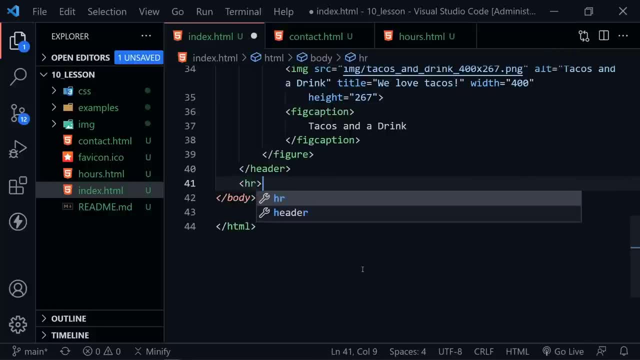 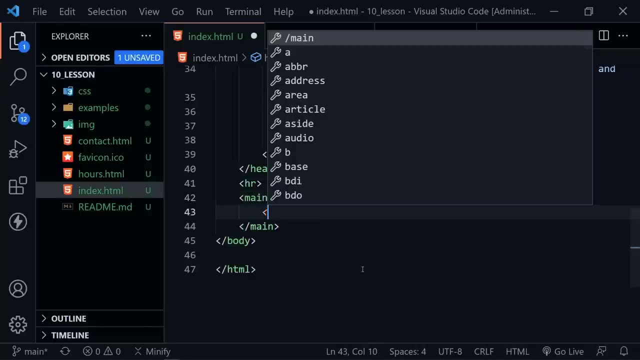 And then, in between the header And the main element, Let's put a horizontal rule And after that Let's put a main element Where the body of our page will be. And so right now, let's leave a comment Saying our content will go here. 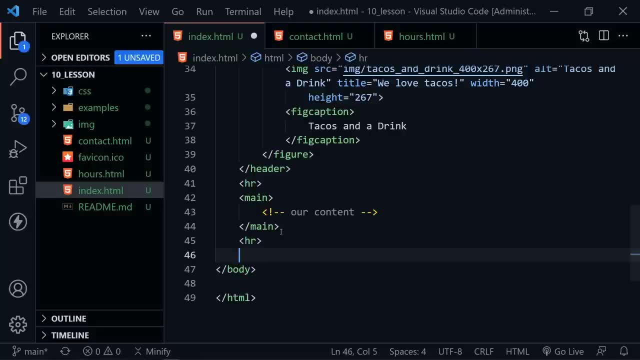 And then after that Another hr, And then we'll have a footer element, And now we need to put something in the footer as well. If you remember from the example, Each footer had a paragraph That said copyright, And now we need to use an html entity. 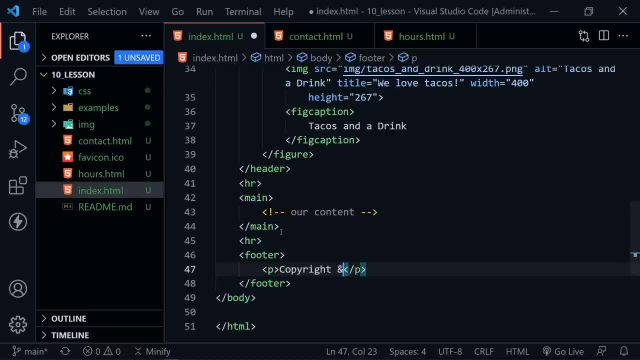 For the copyright symbol, And that is ampersand copy With a semicolon, And then we'll just say: the Little Taco shop, And now we can save this, And now we're really ready to copy all of this code. 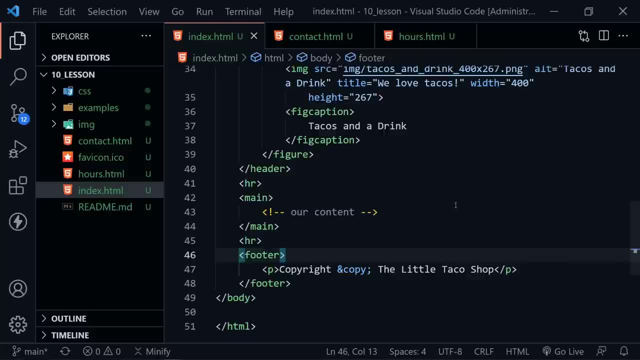 And put it into the other pages as well, And we'll just need to make a few changes. And then, when we add Actual content to each of the pages, That's where it will really differ. So I'm going to press control a. 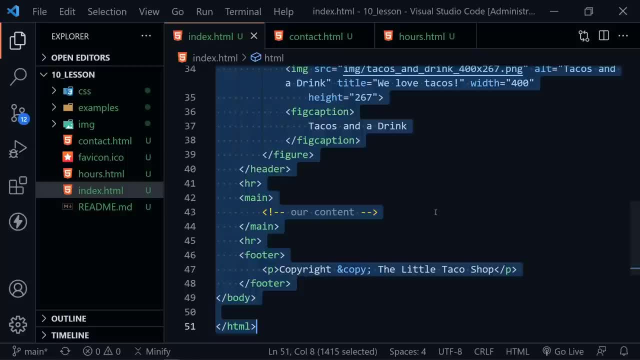 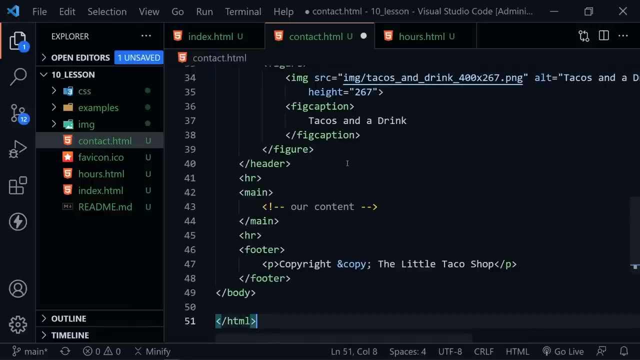 To highlight everything And then control c To copy everything. Go to the contact page And press control v To paste that in Control s to save. Go to the hours page and do the same Control v to paste it all in. 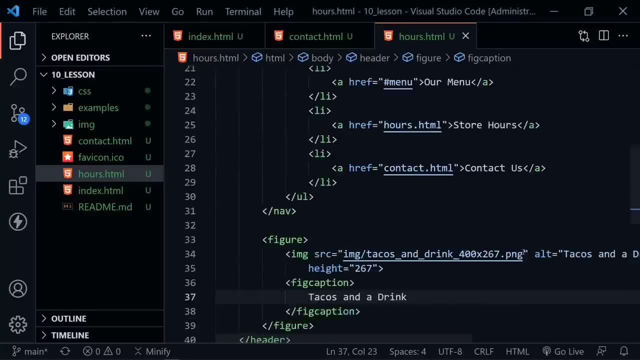 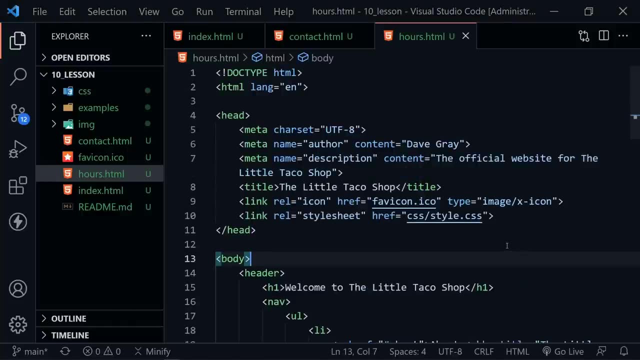 And control s to save. Okay, while we're on the hours page, Let's make the changes here. first, I need to press alt z again In each one of these files To get the code to wrap in each one. So now we can make our changes. 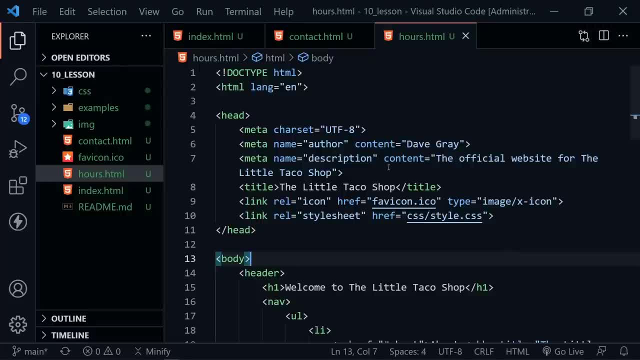 Everything is the same as far as the author And the content, But when we get to description, We'll have a different description. This will be store hours For the little taco shop, And now that we've changed our description, We can also change. 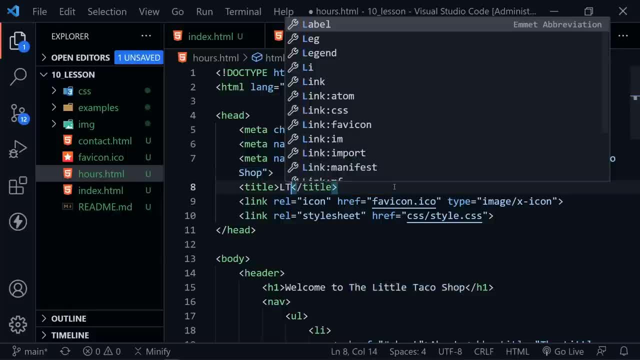 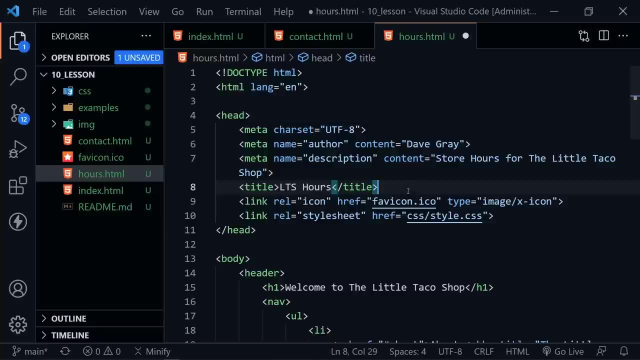 Our title. Instead of the little taco shop here Let's put lts hours. Since it's not the home page, We'll just go ahead and abbreviate As we can assume the owner, employees And even the townspeople In the little town for the little taco shop. 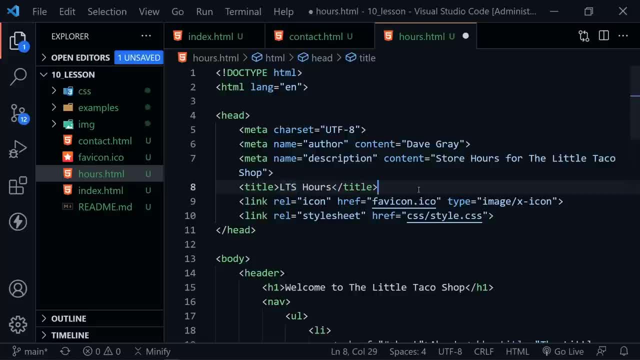 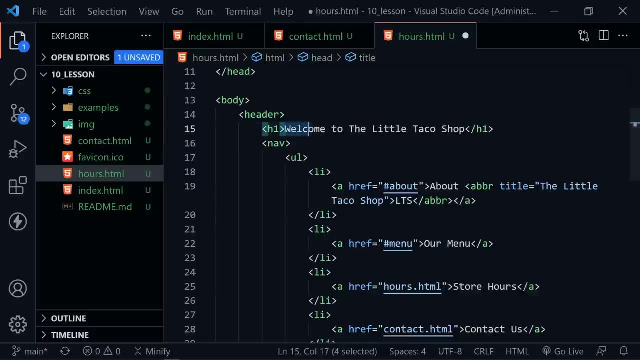 Refer to the little taco shop As lts. Now let's scroll down into the body Where we have our header, And a little bit needs to change here too. So it's not welcome to the little taco shop. here We'll put the little taco shop. 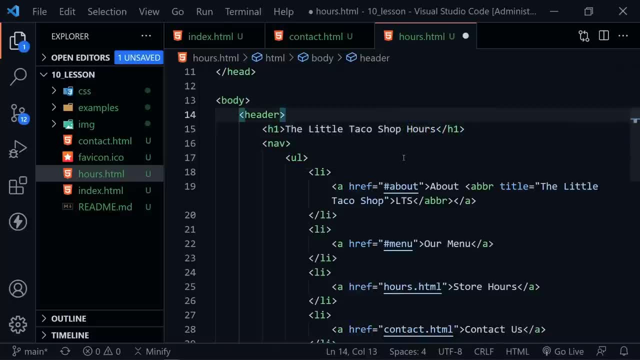 And then hours After that. And now our nav is going to change somewhat too, So it's not just a link To about lts. We need to go to another page And if you remember, We can just go to the slash. 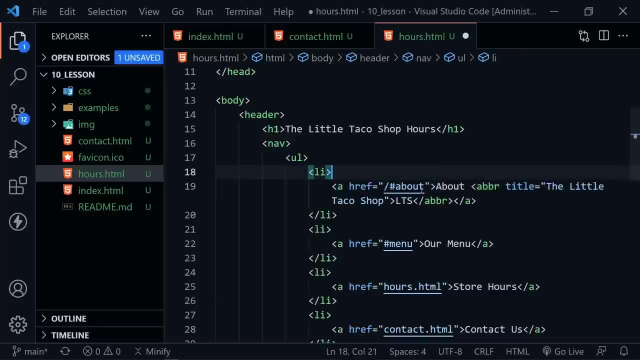 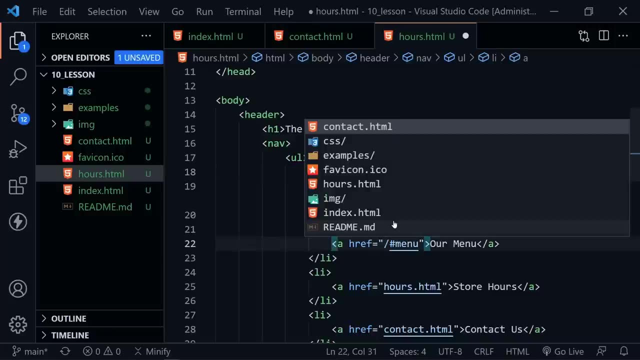 To go to the home page. So here we need slash about To go to the about section Of the little taco shop On the home page. So we'll do the same for the menu, And now We can just eliminate this. 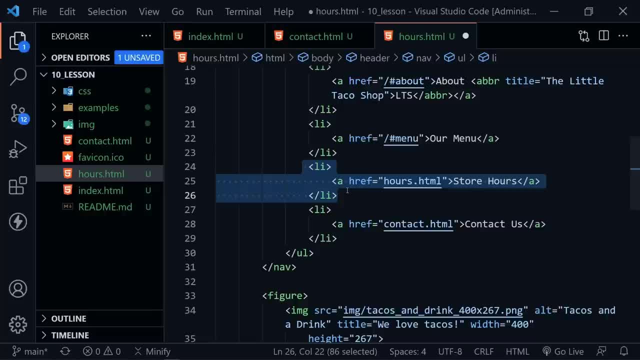 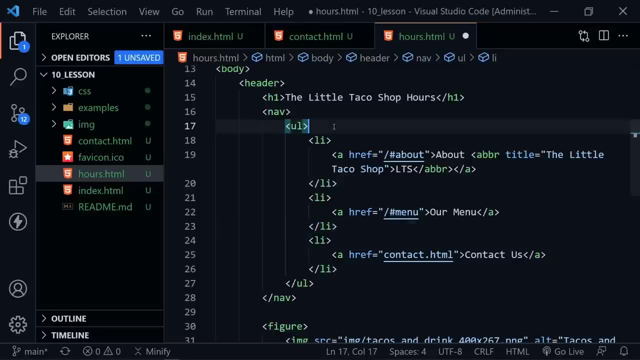 Because we're going to Put in a home link instead. So I'm going to press control x To cut it out And then just backspace out that extra line here, Scroll to the very top And paste in The one that I just cut out. 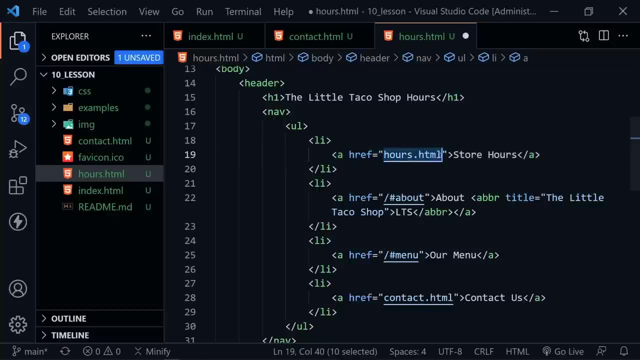 And now we're going to link To just that slash That I was talking about And that will link to the home page. So let's change this store hours To home. Now let's scroll down a little bit further And we need to change out. 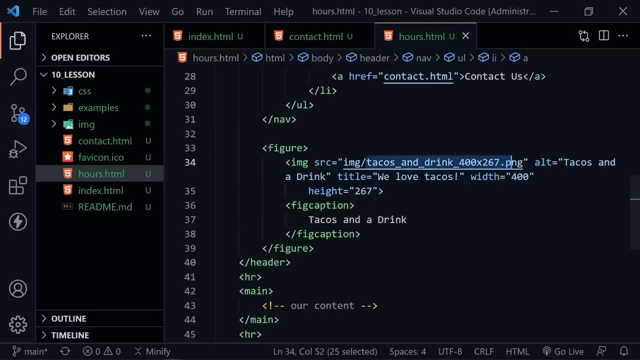 Our image as well. So now we're not going to use the tacos in a drink image. We wouldn't want that on more than one page. So now I want image Slash And we'll choose tacos tray. Now notice, it's also 400 by 267.. 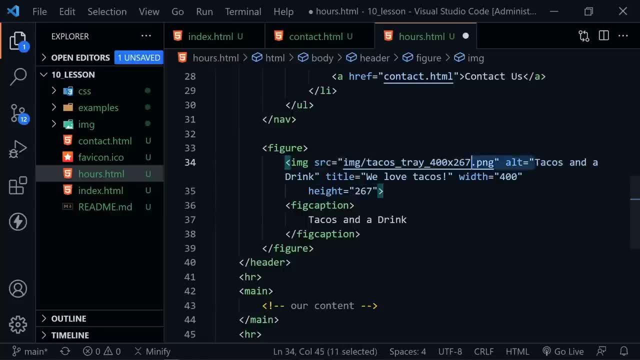 So we don't need to change that. But let's change what It says here for the alt text And we'll say: a Tray of Tasty tacos. And then we can add A tray of tasty tacos For the fig caption as well. 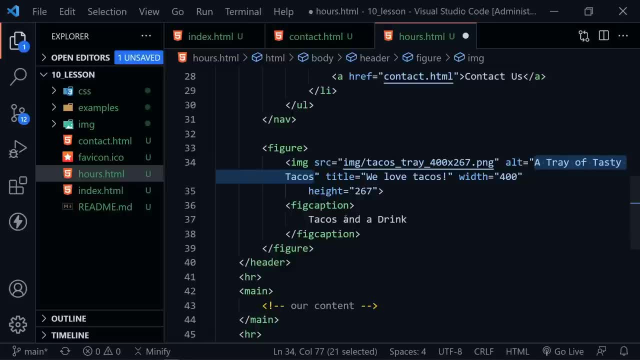 I should have just highlighted that. Copy and paste again Control C Over the fig caption And control V, And we could leave We love tacos for the title here as well, But let's put we love Trays of tacos. 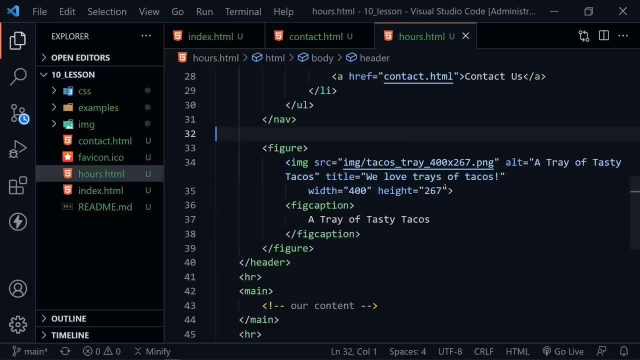 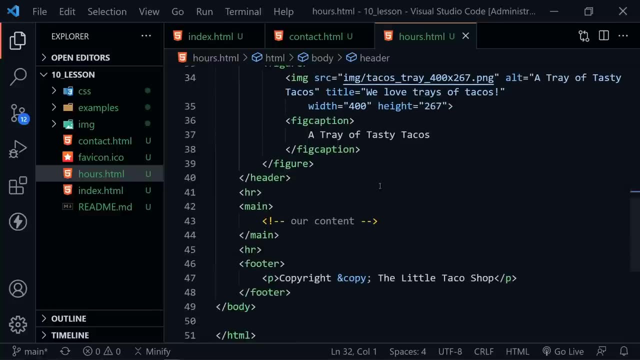 That's some nice title text as well, And remember, the title shows When you put your mouse over the image And if we scroll down, We don't really need to change anything Because the footer stays the same Between all the pages. 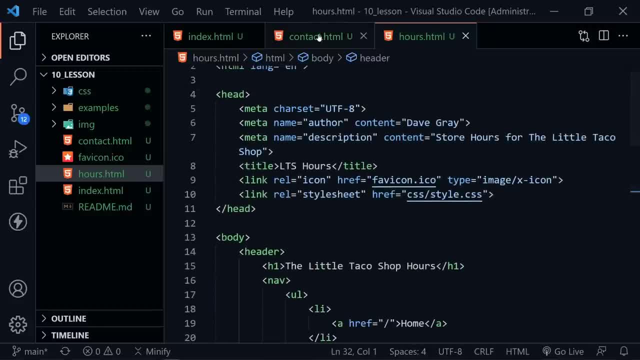 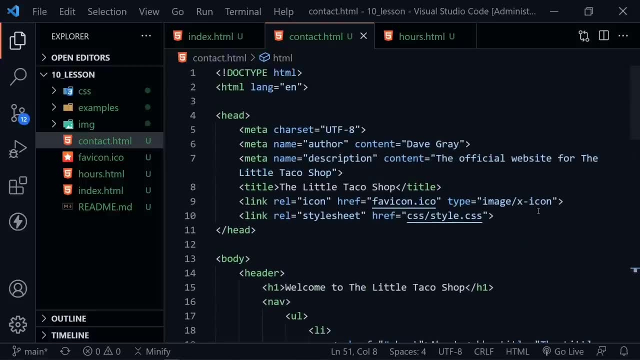 So we're finished with the immediate changes To the hours HTML. Now let's go make those same types of changes To the contact dot HTML. I need to scroll back up to the top first And press alt Z To get the code to wrap. 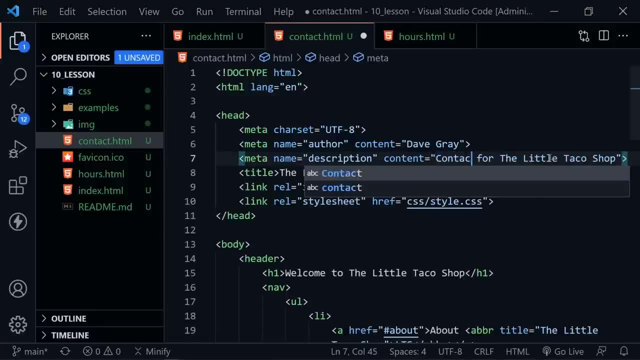 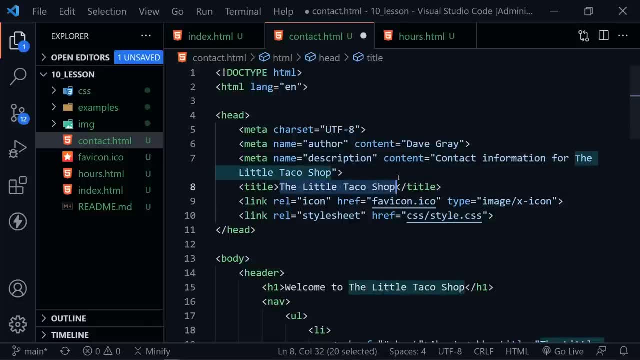 Now we need to change the description again. So let's change this to Contact information For the little taco shop. Let's change the title for the page as well, And here we'll put Contact us, And then let's put a dash. 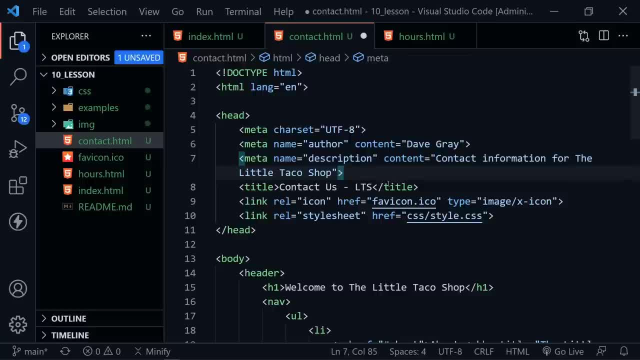 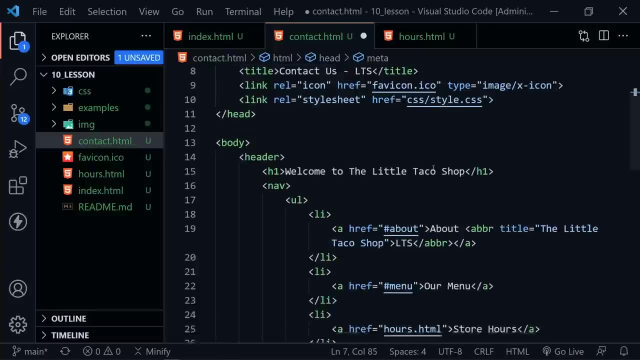 And put LTS. Just because we want the LTS In the title For everything, that's not the home page And we leave everything else the same. So now we can scroll up And this is the contact us page. So let's highlight this H1.. 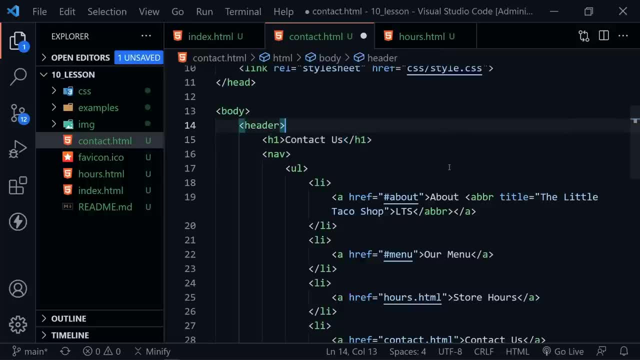 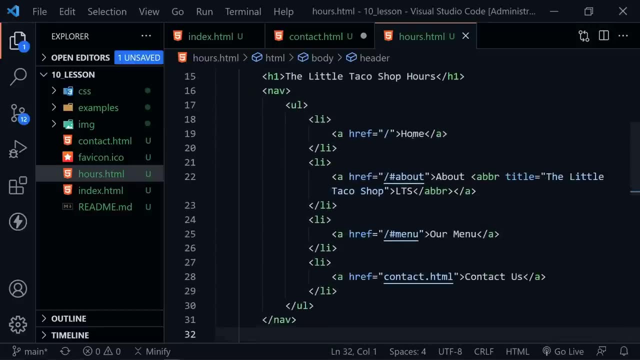 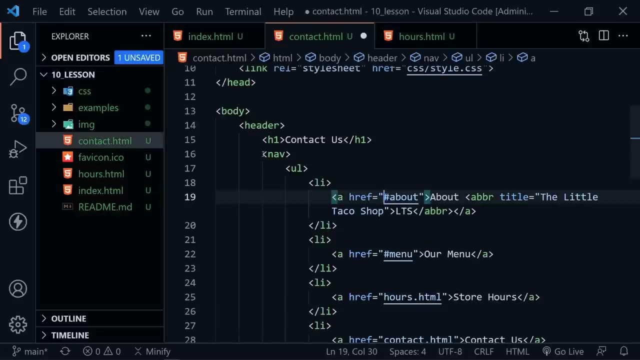 Change this part to contact us. And now for the about. Once again, We did actually go over to the hours And now let's copy This nav And we'll just have to change a little bit Less that way. So copy the nav. 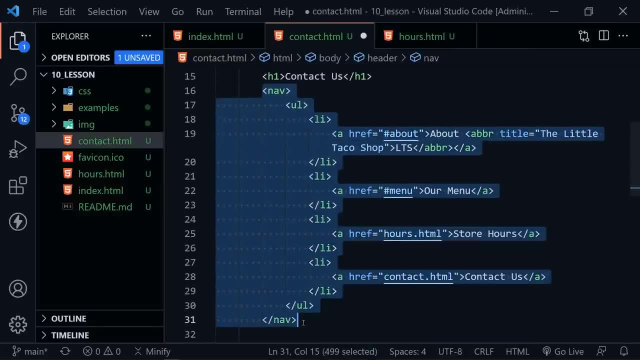 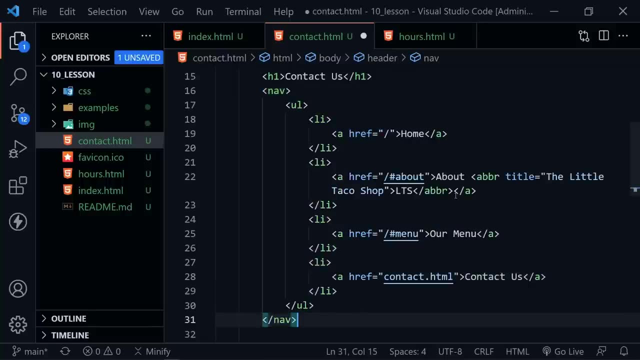 And now we'll highlight the nav that we have in here And paste in the new one From the hours page. So now we have the same home link, We have the same about link, We have the same menu link And we only need to change contact. 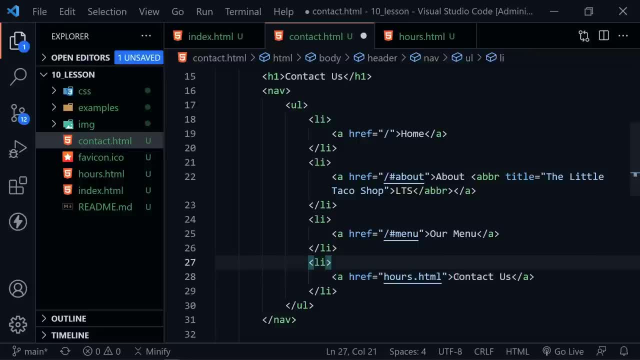 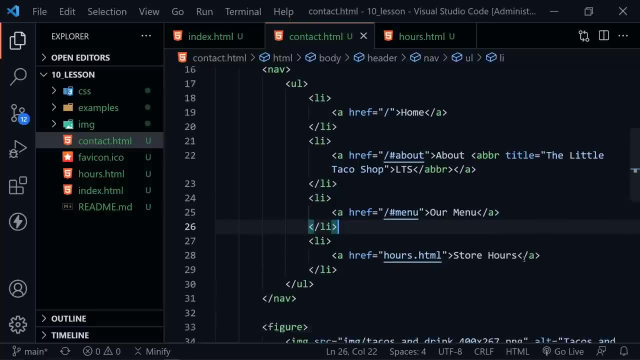 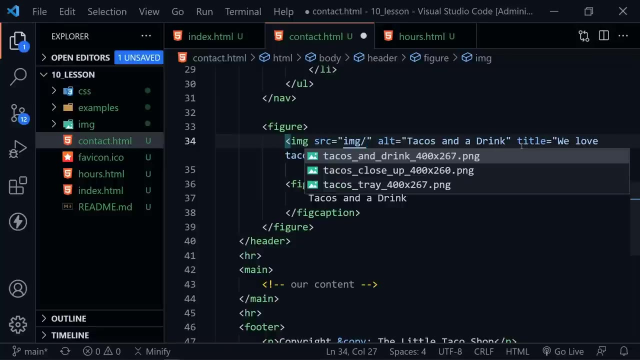 To hours. So we'll link to hours And then we just change this contact us To store hours And let's save that much. Okay, Scrolling down to the figure: We need to change out our image again. This one's just a little different. 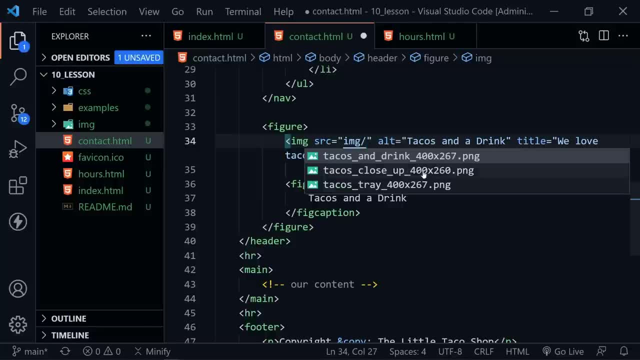 So now we've already had tacos and a drink And the tacos tray. This is tacos close up. Notice the size is a little different: 400 by 260.. So we've got 400 here. We need to change this to 260.. 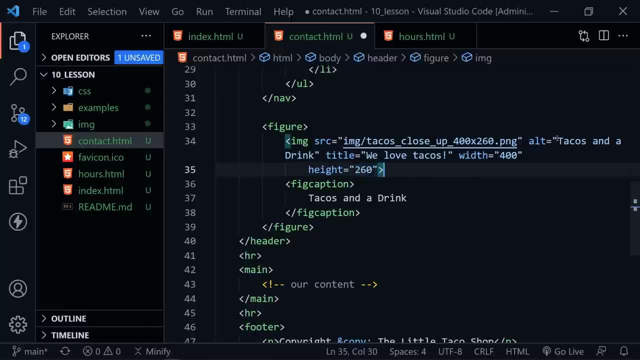 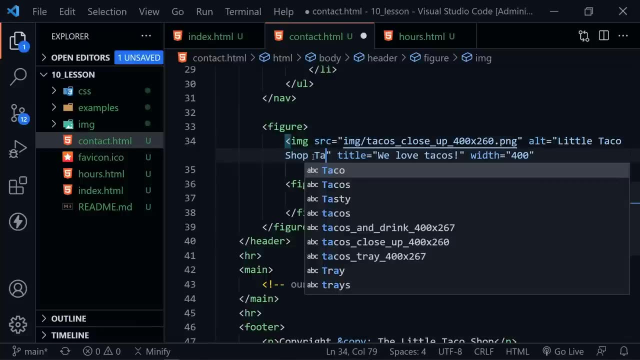 Instead of 267.. Okay, now our alt, Of course, will be a little different as well. This will be little Taco, shop Tacos. And now for the title. Let's put tacos ready to eat, And then we can put. 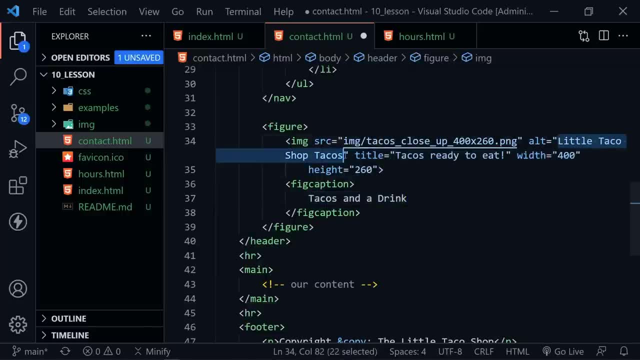 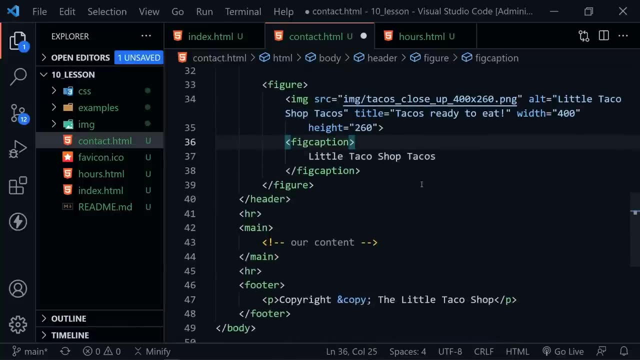 Little taco shop- tacos here too. So I'll once again highlight that alt text And put the same Text in here for the caption That we're showing on the page- And if we scroll down We can see our footer- remains the same here too. 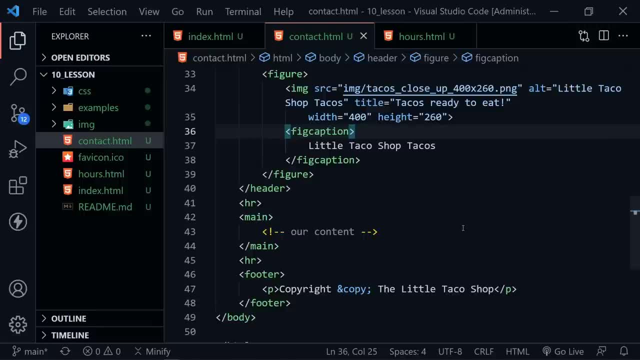 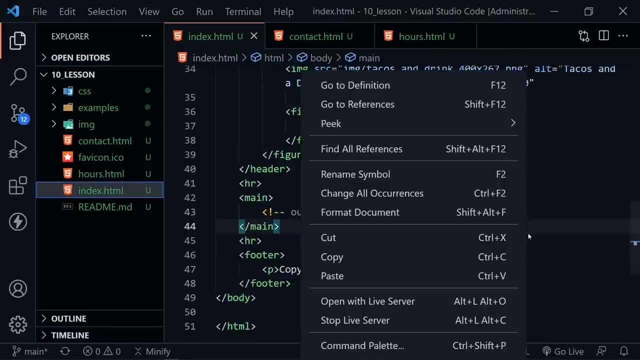 So let's save the page And we're ready to begin working on content For each of the pages. Okay, I'm going back to the index HTML And I'm going to click go live, Or I could right click and choose Open with live server. 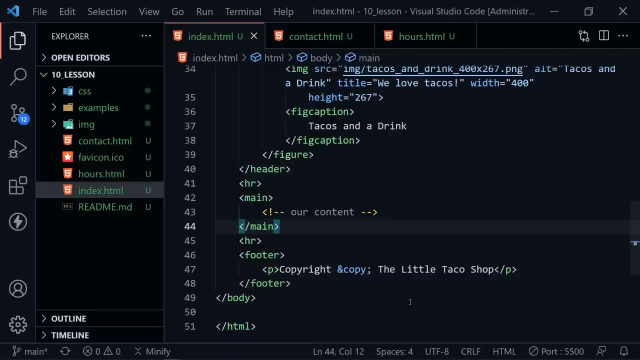 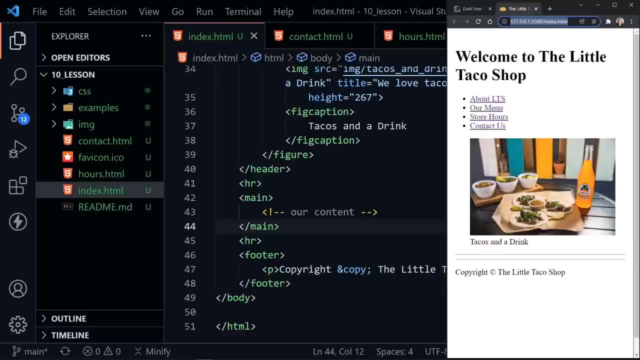 Because we're using the live server extension To view our web page And we can go ahead and start looking at our page. It doesn't have a lot on it, But we have to get started here. We've got our header section. 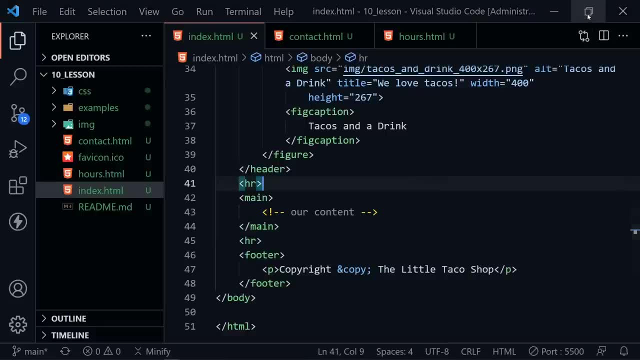 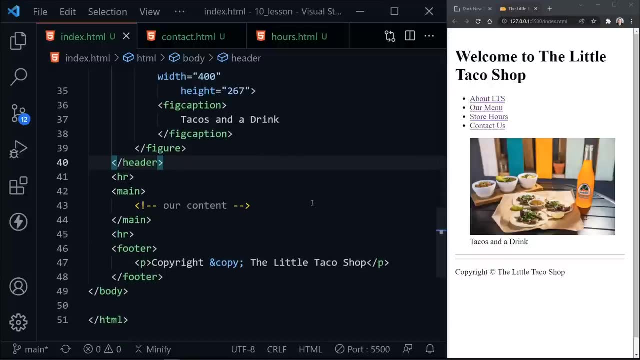 And we've got the menu with the different links. So now I'm going back to the code. I'm going to resize visual studio code And press control B to hide the file tree So I have more room to see the code And we're ready to add content to the page. 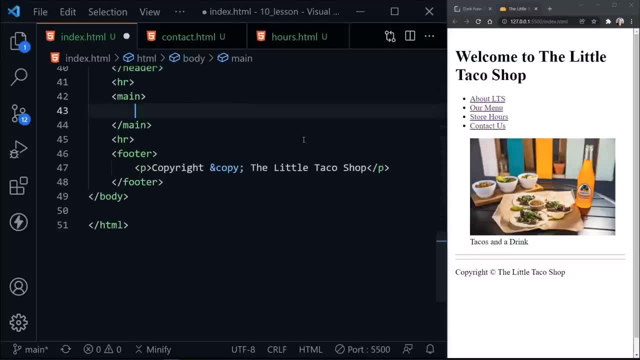 Inside of the main element. I'll delete that And we'll start with an article element. I'm going to give this an ID Equal to about. So our about anchor tag works. Our link works. Now I'll put an H2.. 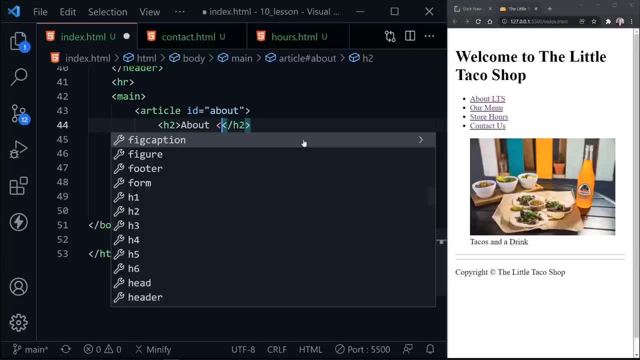 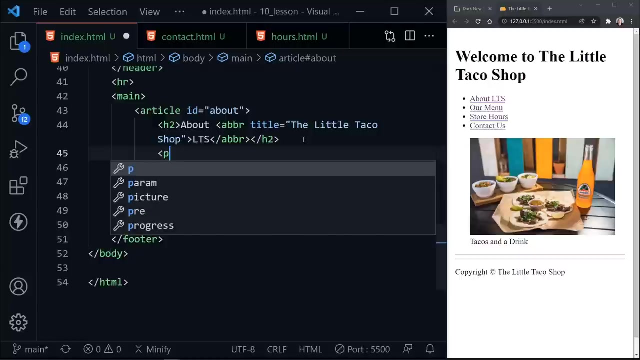 And inside the H2.. I'm going to put about: And then we need that abbreviation With the title value again Of the little taco shop, And now we'll put LTS. There we go, And that completes the header. So now let's put some content. 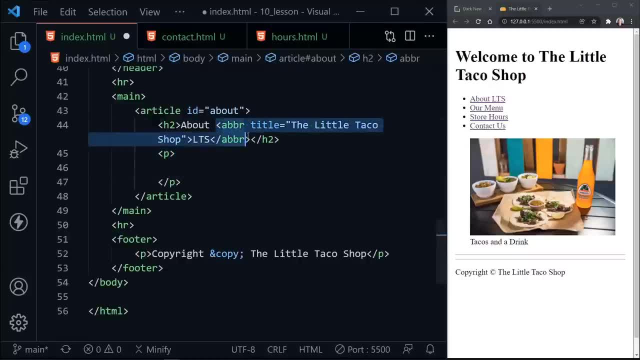 We'll have a paragraph here, Same abbreviation, And start the paragraph with that. So LTS Was founded in And now remember, we can use a time element To give some meaning To the dates and times we put on our page. 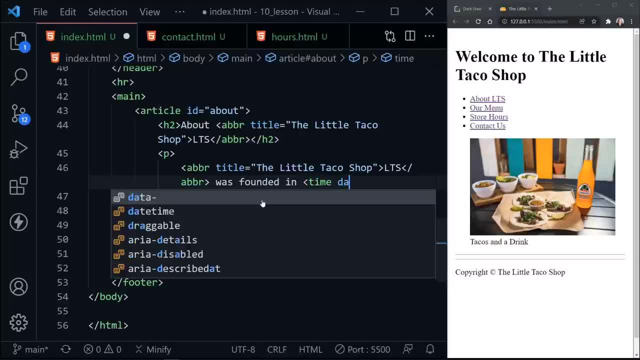 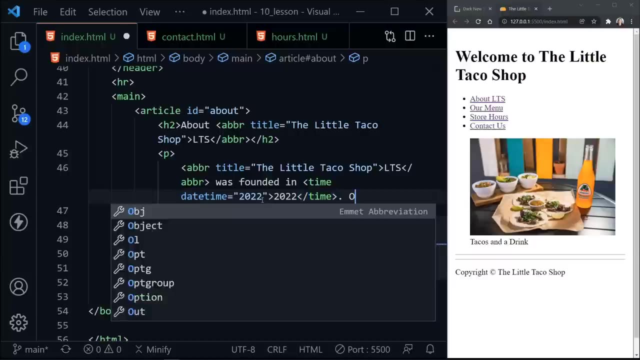 So I'm going to put A time element here With a date time Equal to 2022.. So the little taco shop Is a fairly new location. So Get a period at the end of that sentence And we can put. 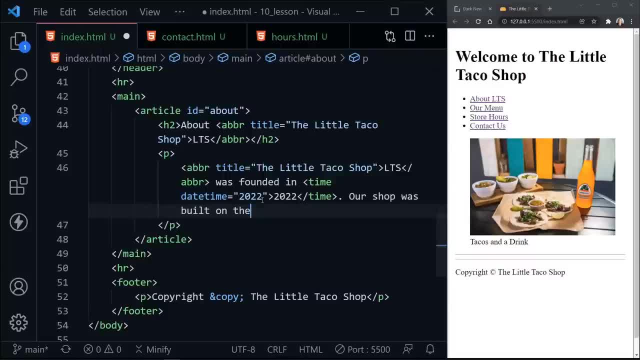 Our shop was built On Or was built from There. we go A love of tacos And now we'll put a period there. We'll say we hope our shop Adds a unique And interesting Place To our little town. 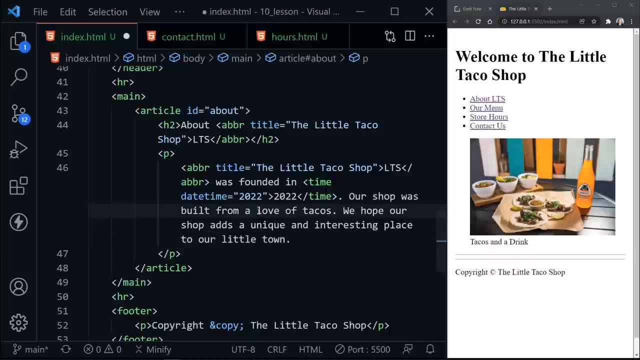 Now let's add Just a little more flavor To our paragraph So we can put a strong element, And then we'll put love of tacos Inside that, So it has some emphasis. And now we also Want to add some taco emojis. 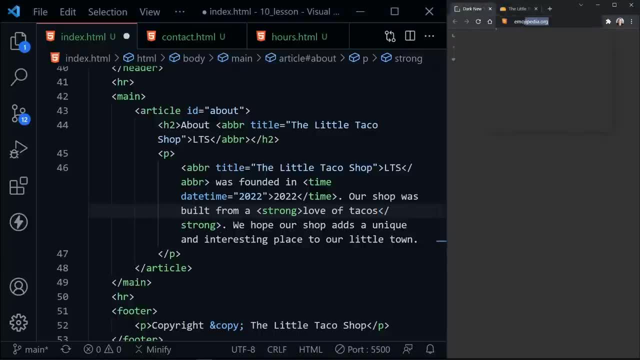 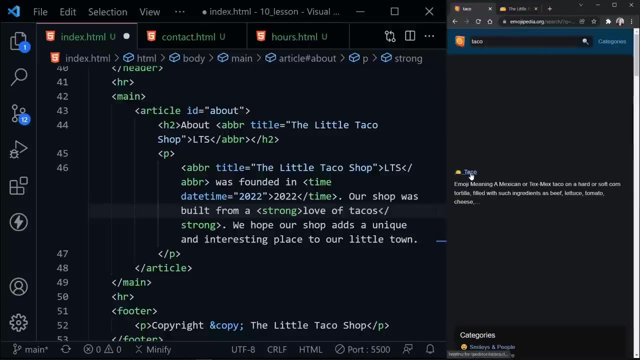 Right after that. So let's go to a new window And I'm going to type in Emojipediaorg And there you can search for emojis. I'm searching for taco And once I find taco I'm going to click that. 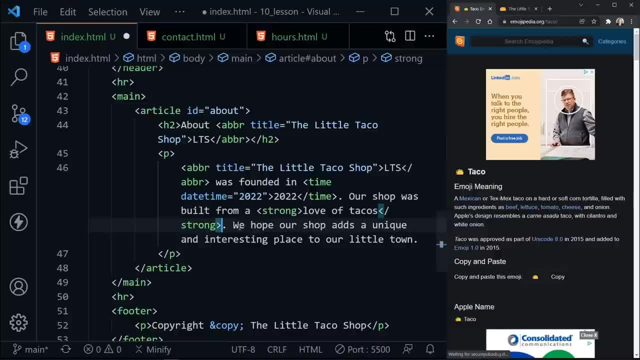 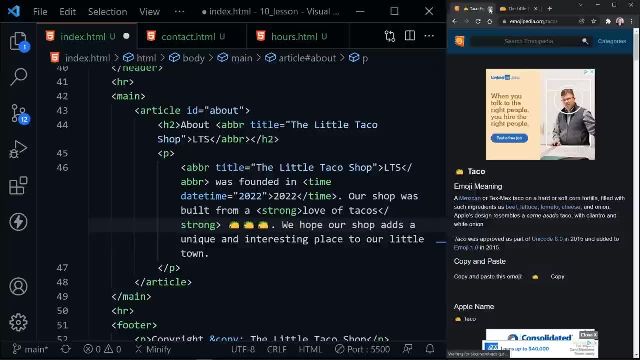 And after I say a love of tacos, I'll put a space And control V, Control V Just pasted in three tacos. So I'm going to close out emojipedia. We no longer need that, But let's save this. 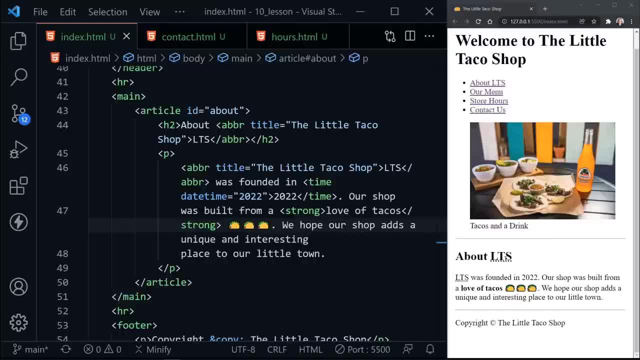 And see what we get on our page. So now, if we look at this, We've got about LTS And there's the abbreviation, And when we mouse over We get little taco shop. And now we've got our paragraph, But right after the paragraph. 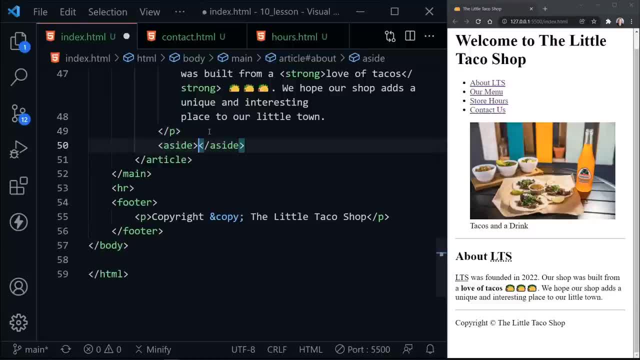 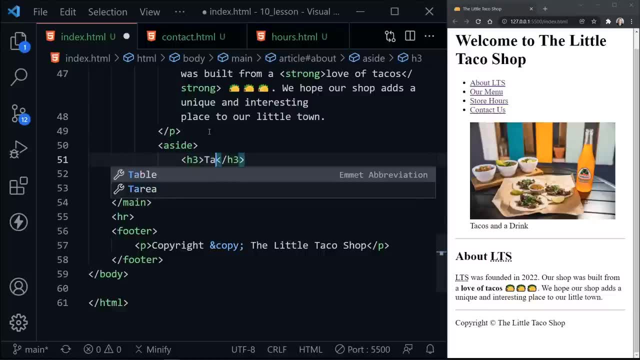 I'm going to use another semantic element Called aside, If you remember that one, And for the aside I'm going to put an H3 header. So we're following that header. hierarchy Put taco trivia. So for taco trivia We're going to have a question. 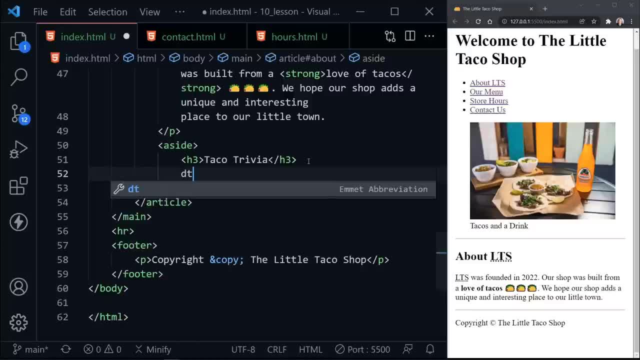 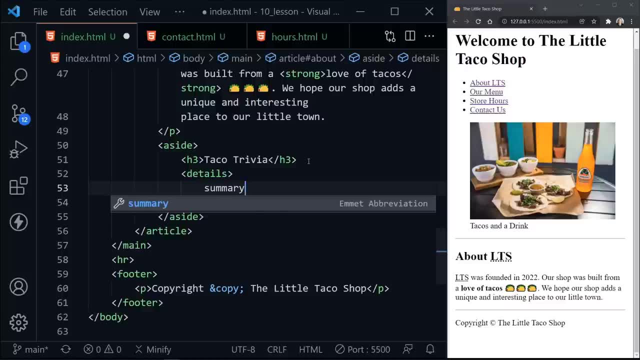 That only shows the answer when you click on it, And for that We need to start out with a details element And then inside the details element We're going to use a summary element. So inside the summary Is where we ask the question. 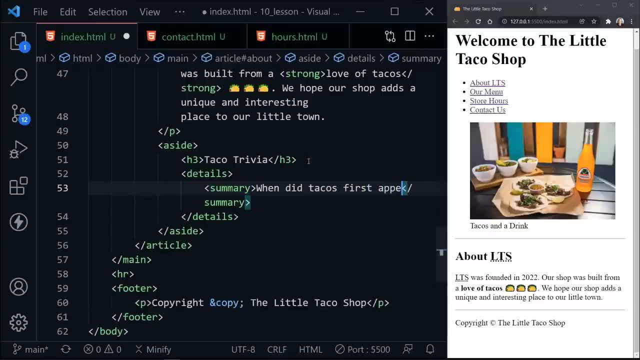 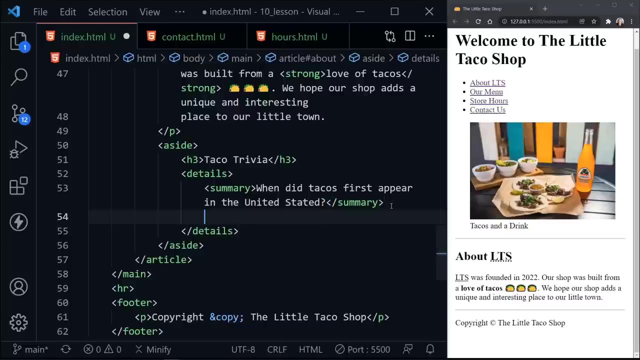 And we can say: When did tacos first appear In the United States? And now the nice thing is, This question will show, But you'll have to click an arrow To see the answer. that is contained within, And that's within. 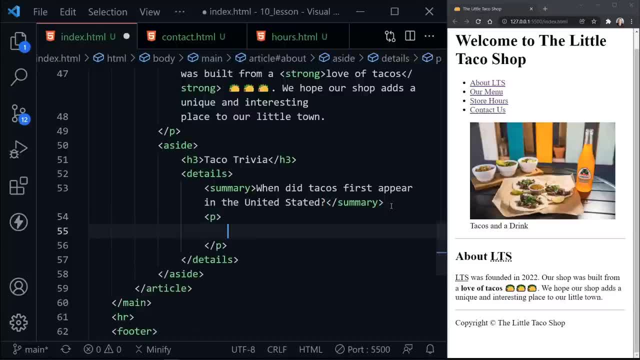 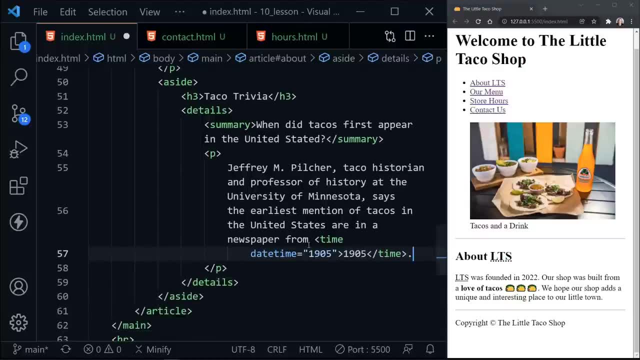 Just the rest of the details here And it's a paragraph. Now I'm going to copy and paste this paragraph in And put it right here And we can save that much And we can see our taco trivia Down here at the bottom. 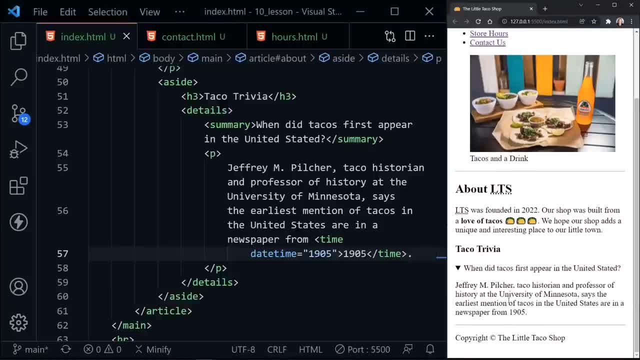 And when we click We see the rest of this, But there's just a little more I would like to add, And it actually has one element in there That was not covered in prior lessons. But remember, There is a wealth of information. 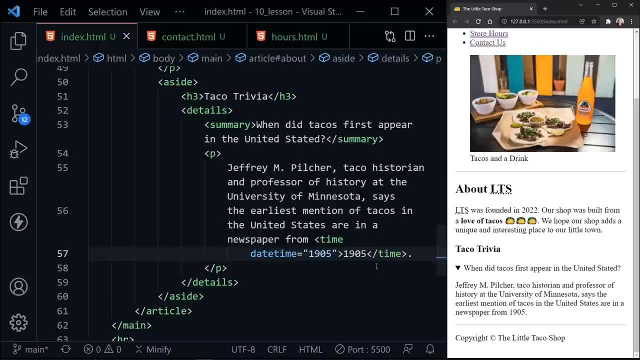 And many different elements That still remain uncovered. I guess They're not used as often, But you can look them up On the Mozilla Developer Network. So I'm going to put in a citation, And there is an element in there Called Cite. 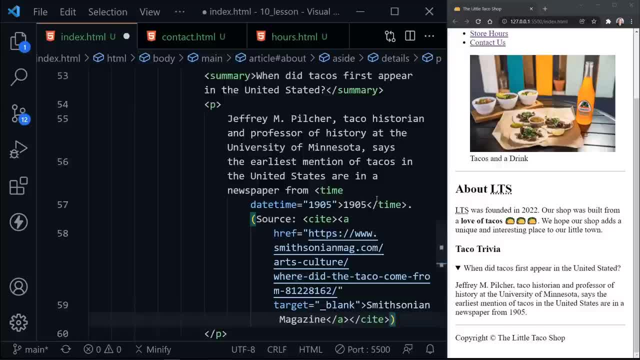 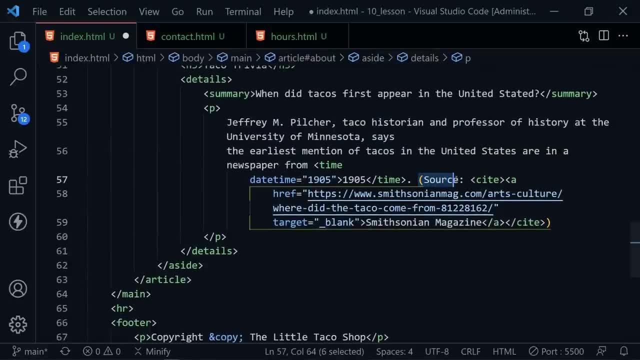 So right after this I'll paste in the citation And here you can see I put the source. Let me expand Visual Studio Code. That's getting a little cramped. You can see I put the source And then I put a cite element. 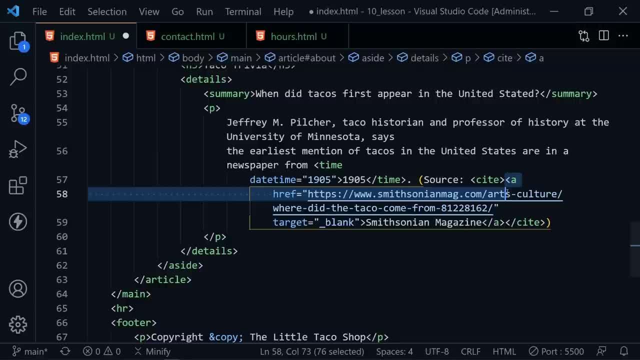 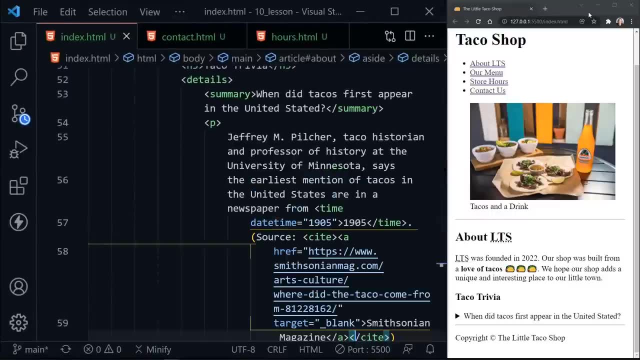 Cite And inside that cite element I put the link to the source. So that is right there And that's Smithsonian Magazine. Let me resize once again. To come back and look at our taco trivia, And when I show the information, 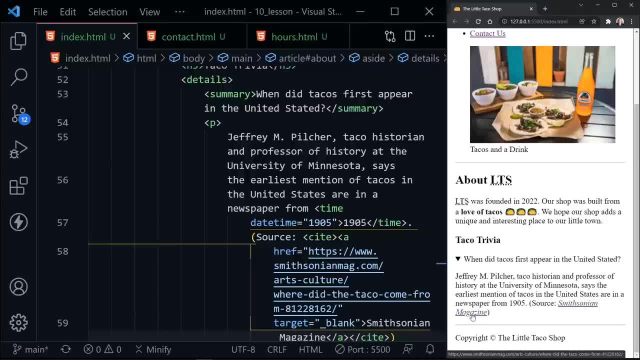 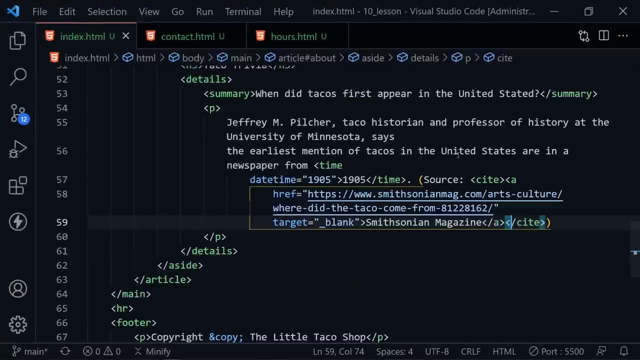 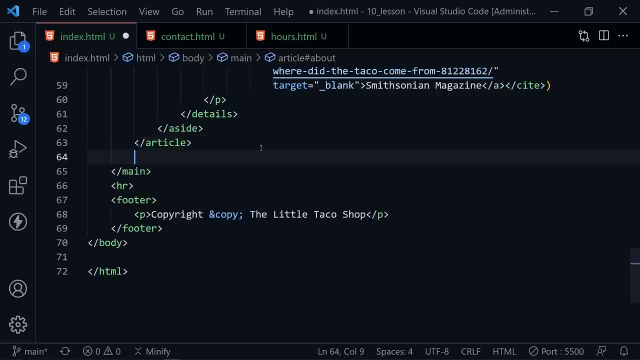 You can see the citation Is put in italics By default With that cite element. Okay, let's resize Visual Studio Code again To get a little more room And scroll up as well. After that aside, We have really completed our first article. 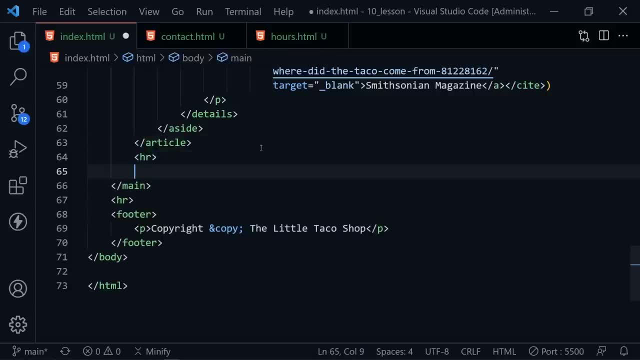 So let's put a horizontal rule in here Which also indicates a topic change At least somewhat In the main area, And put another article Now this article. I didn't add the ID, But it needs the ID Because the ID equals menu. 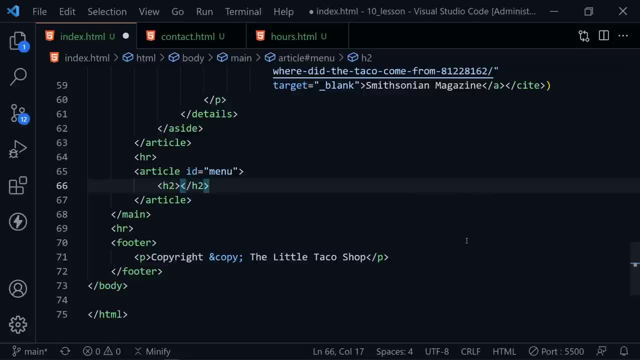 And this is where we will put the little taco shop menu. We'll start with an H2 again To follow the header hierarchy for our page And we'll put our menu for that And then we'll start our table element Inside the table element. 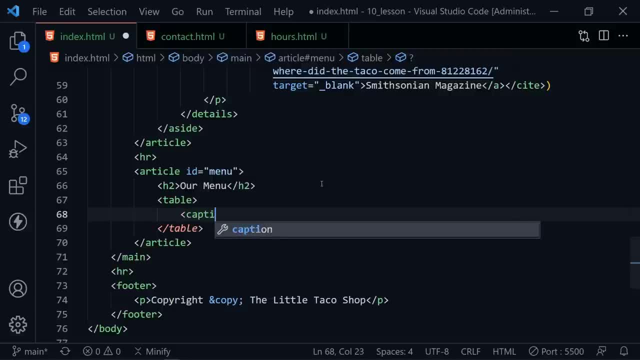 The first thing we're going to add Just immediately. There we go And we'll just put our tacos for the caption. After that, We need a THead Inside. the THead will be a table row And the table row 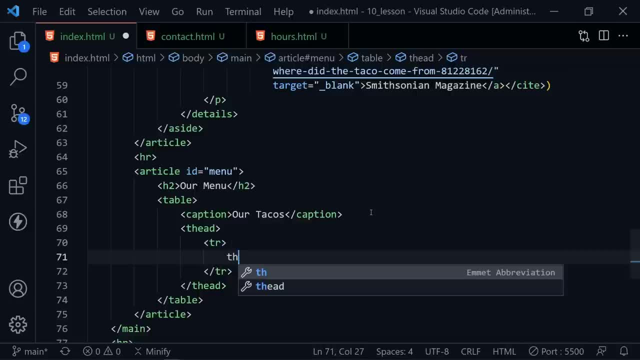 Is going to have our columns And these are our heading columns. So the first one Is tacos. After tacos We're going to have a second TH And this TH is going to have. Well, let me go ahead and type TH again. 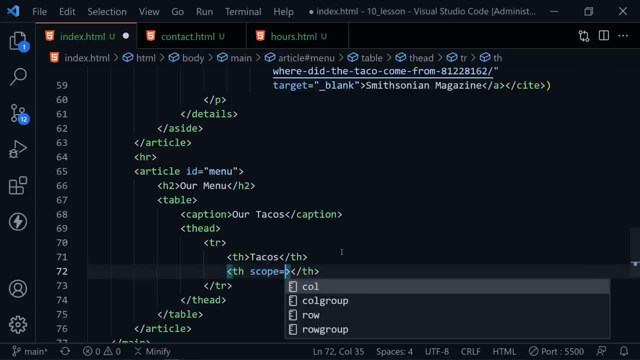 There we go, And then we have a scope, And let's set this scope equal to column, Because it's for the column, And then we need our abbreviation Element once again. So let's type ABBR And then we'll put the title equal to. 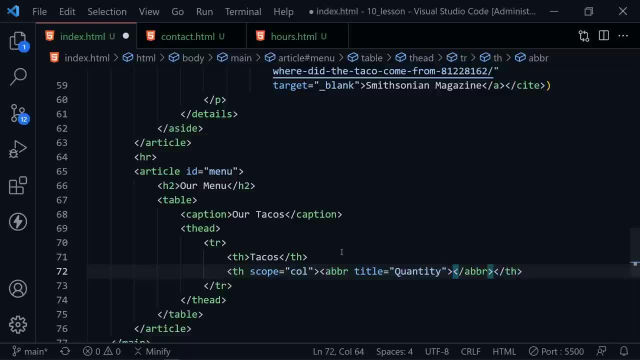 Quantity, And now We can put in the abbreviation for quantity That we want to use, Which is commonly QTY, And then we'll add another TH And it will also have a scope. Let's set this equal to Column as well. 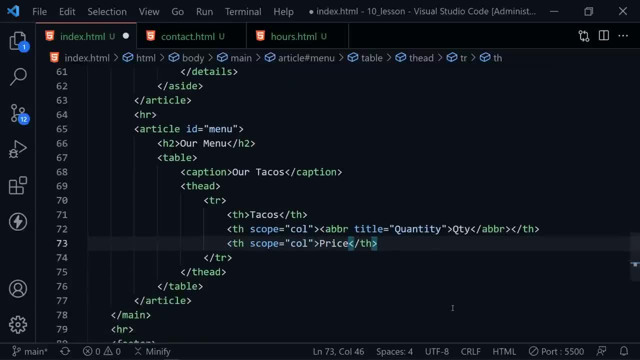 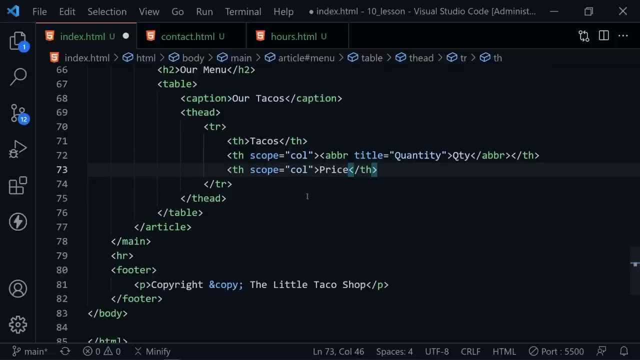 And this will be the price column. Okay, going to scroll up. As you might have realized, When we learned about tables, Tables take up a lot more space As you create them in your code. So we've completed the head And we need more room. 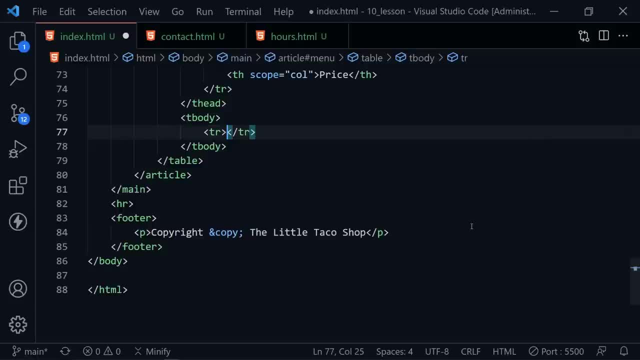 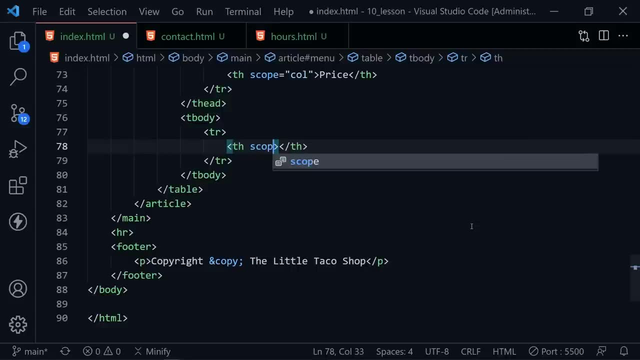 For the body of the table. Let's add a new row, And inside this row We're going to add another heading, But this will have a different scope. So now that we're back there, Let's add a new row, And now that we're ready to put in the value, 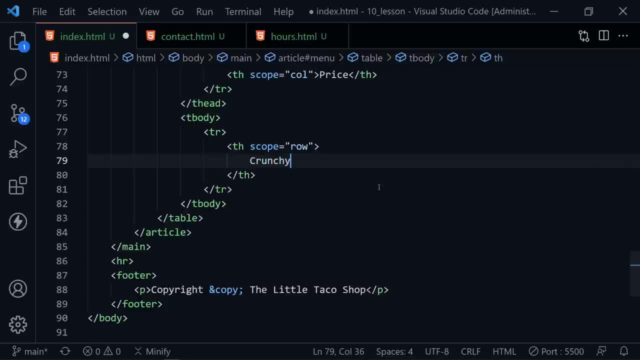 Let's call this crunchy, But I did forget an attribute: This also needs a row span, So this will have a row span Equal to three. Okay, after we've created The scope and the row span With crunchy, We can't forget the values of the other columns. 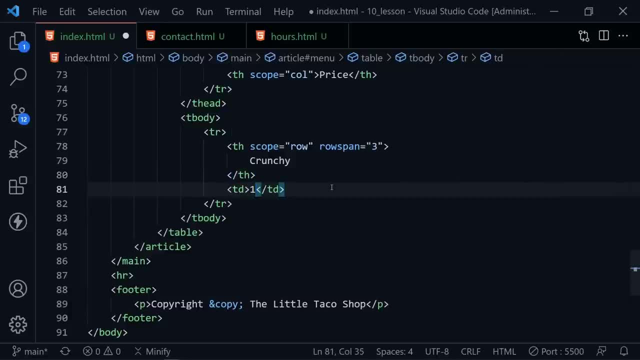 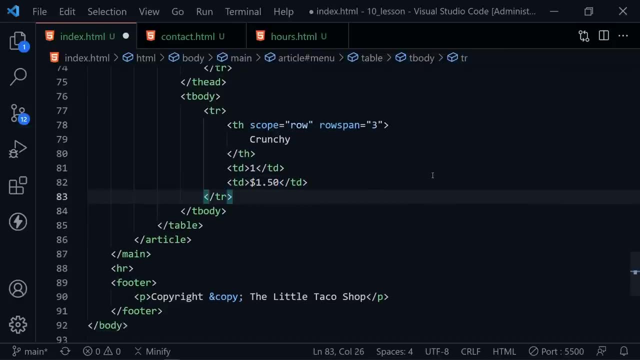 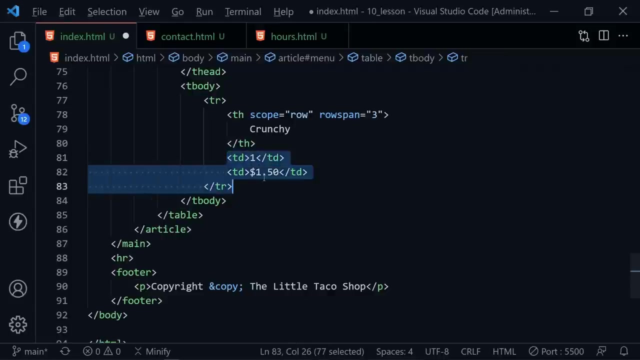 So now we need one For the quantity And for the next one, Which was price 150.. So there's our first row, And now we can create more rows, But what I really want to do Is just take these last three. 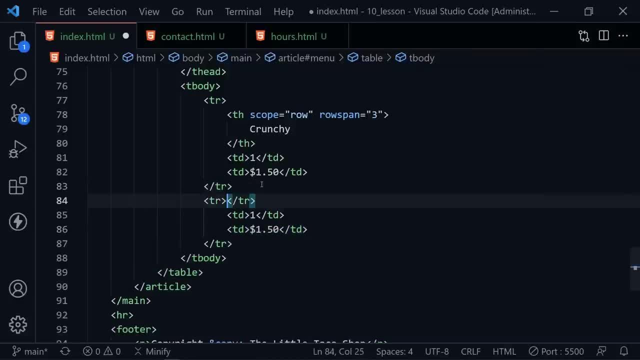 And do shift, alt and the down arrow And then add an opening TR here. Wanted to add a closing TR as well, But we don't need that Because this crunchy Is taking up three rows, So we don't want to add. 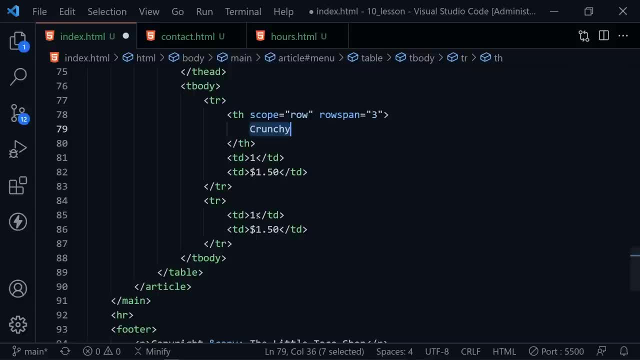 That row down here. We just need the other two rows. So let's turn this one into A quantity of two And two dollars and fifty cents. Now I'll just highlight this row And take it down one more time And we'll have a quantity. 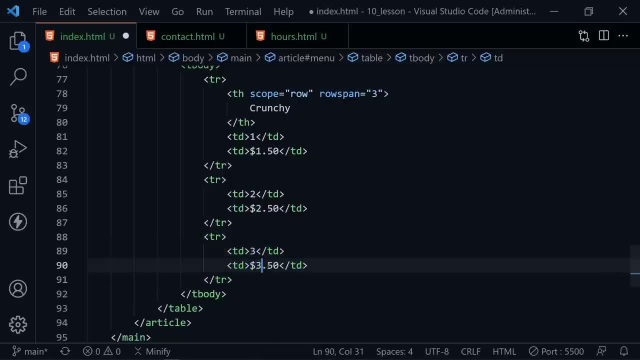 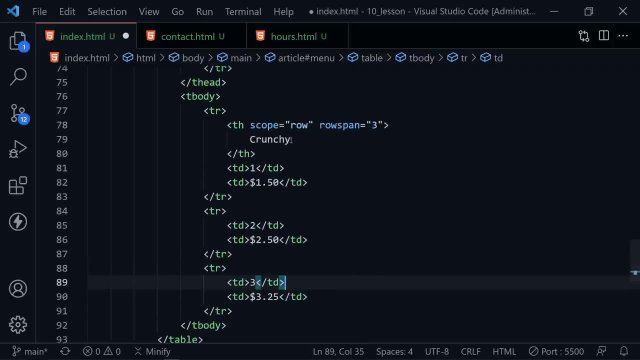 Of three And we'll put three dollars And twenty five cents. So now we've got The feel of this, Where we've got the first one with the title And it's taking up three rows, And then we've got the quantity and the price. 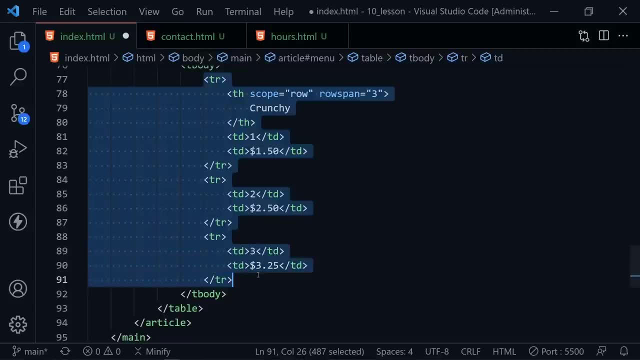 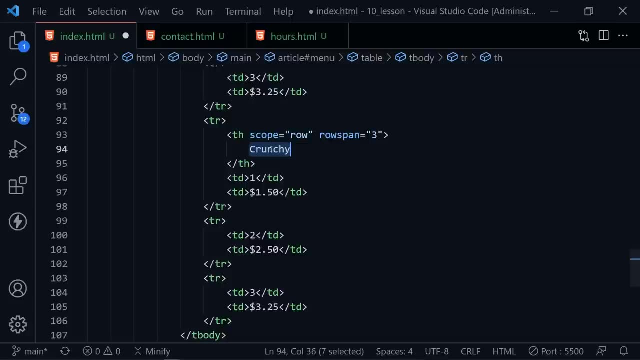 So what I want to do for the next one Is to just highlight These And press shift, alt and the down arrow And, once again, just make changes. So this is going to be soft Instead of crunchy, And now we've still got a quantity of one. But is the price the same? And no, it's not. Soft tacos are a little more expensive. So two dollars, And then, for two soft tacos It's three fifty, And for three soft tacos It is four fifty. Now let's scroll up some more. 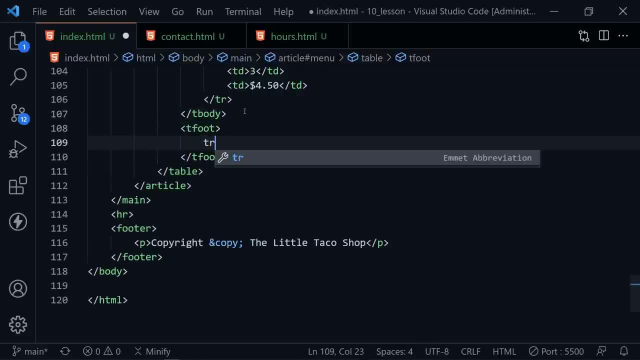 And that's the t foot element. And now inside the t foot We're going to have a table row And then we'll have a data cell, Table data, And it's going to have a call span attribute, So it's going to span all of the columns. 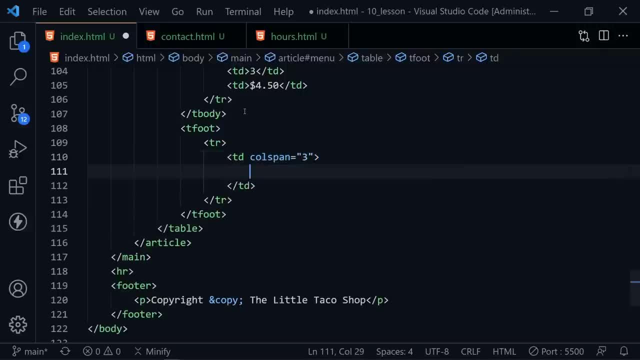 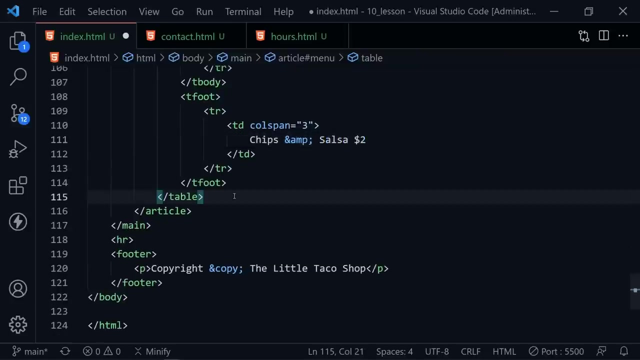 So that's three. And then inside of the table data We'll put chips, And then- and- amp Is for the ampersand, That is another html entity- And then we put salsa- Two dollars- And then we put our table. 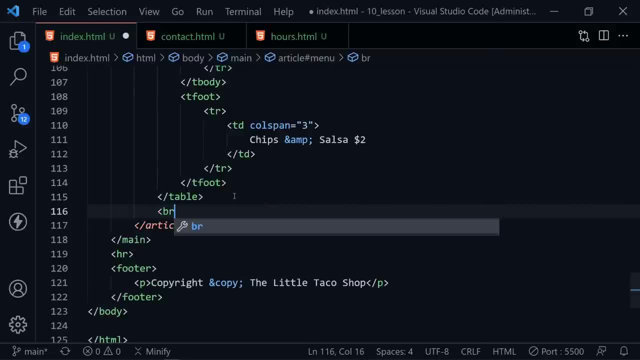 But underneath the table. In this last article, Let's go ahead and put a line break, And after the break Let's put a paragraph And let's go ahead and add our back to top link. So now we'll have an a. 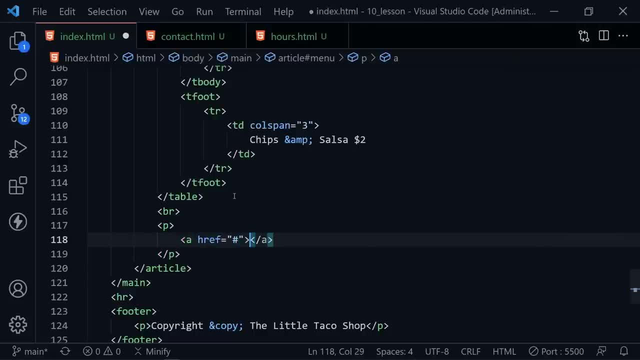 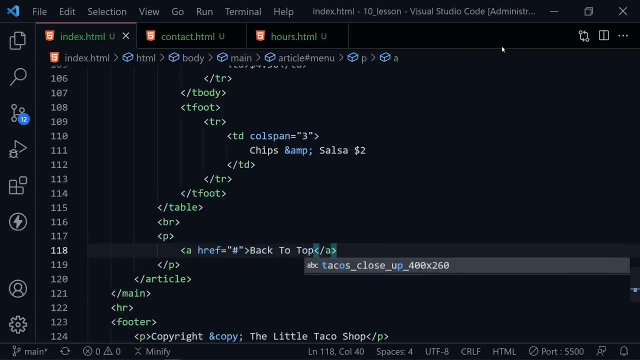 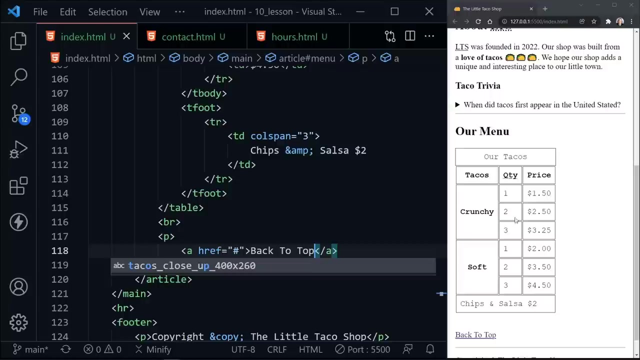 With an href. We'll set this equal to the hashtag, Which should just reload the page. Take us back to the top And we can save. So now let's resize Visual studio code To our content. Yes, we've got the crunchy. that took three rows. 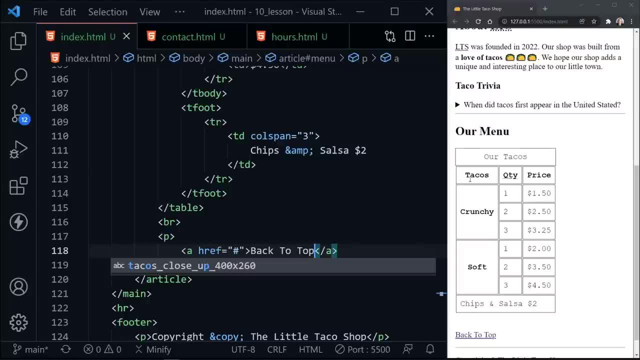 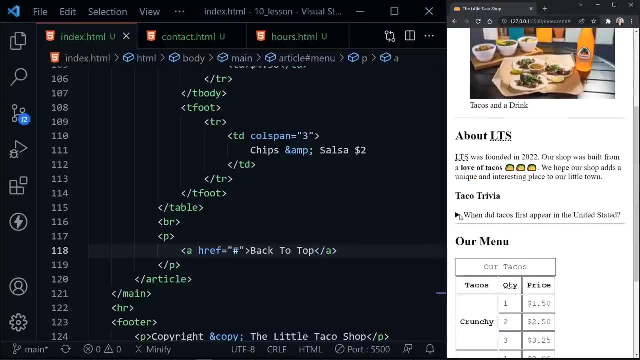 And the soft. that took three rows. There's the table footer. Everything looks like we planned it And our back to top link is here. It takes us back to the top as well- Our taco trivia. Everything is good About the home page. 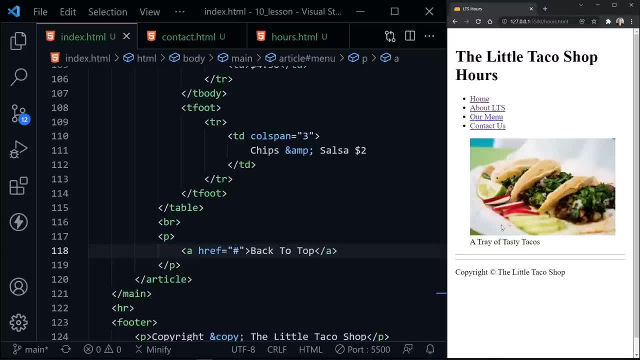 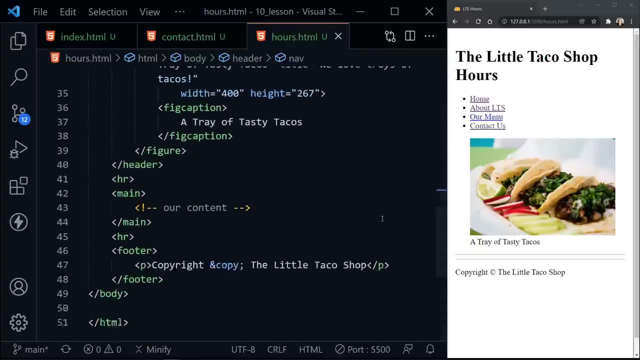 So now let's work on the store hours page. It is a fairly short page And there you can see it displayed to the right, And we'll pull up the code here on the left. Okay, let's scroll down And we've just got a little bit of content. 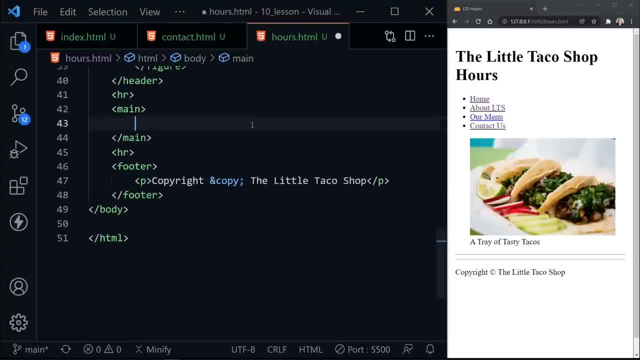 To add in the main area here Of the body, Inside the main element. So we'll start out with a paragraph And inside this paragraph we'll just say We are open Seven days a week, With an exclamation mark. After that we need to add: 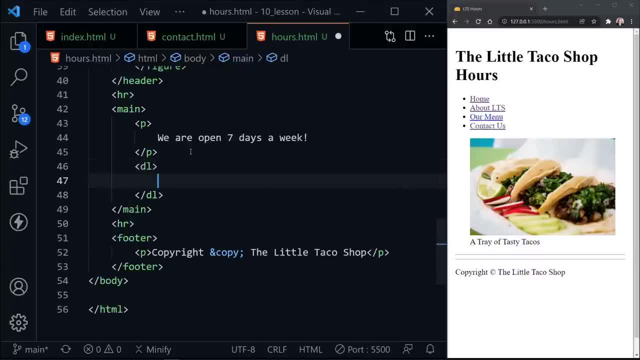 A data list. So it starts out with a dl element. Inside the dl element We'll have a dt And this is where we'll put Sunday-Thursday, So Sunday through Thursday, And then underneath that We'll have a dd element. 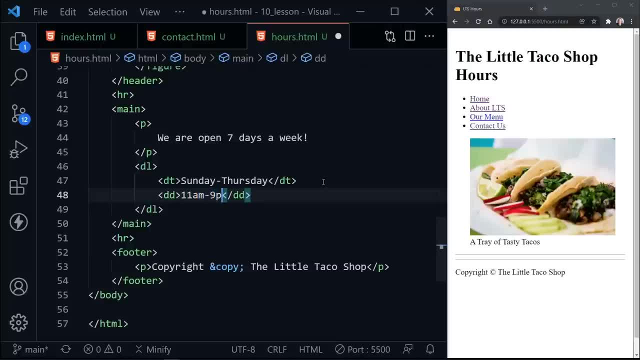 And that's where we'll put our 11am-9pm. So now we can just Copy this down, Because there's only one more that was like it And we can just change the days out. So now this will be. 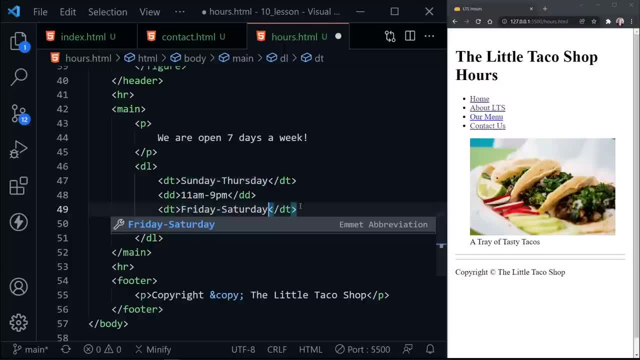 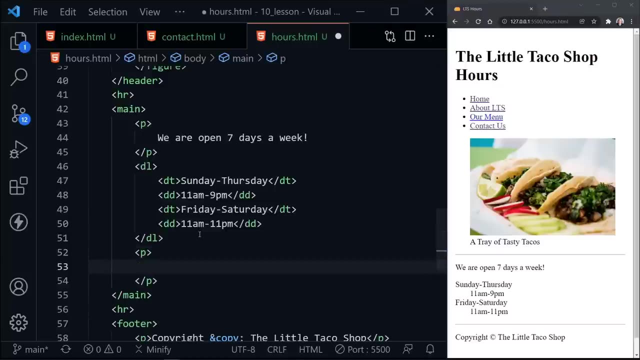 Friday, Saturday, And then the hours are different as well. It's 11am to 11pm, And we can save that. Now We also need to add A back to the top link as well, So here's our paragraph. 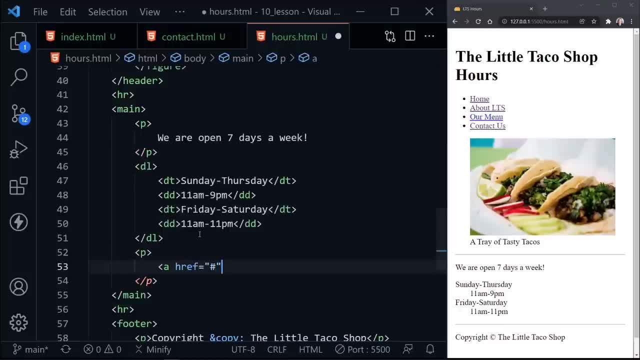 And then we can say A with href Once again equal to the hashtag, And back to top And save once again. And now we can see all of this here on the right. Our back to top really Isn't needed because it's so short. 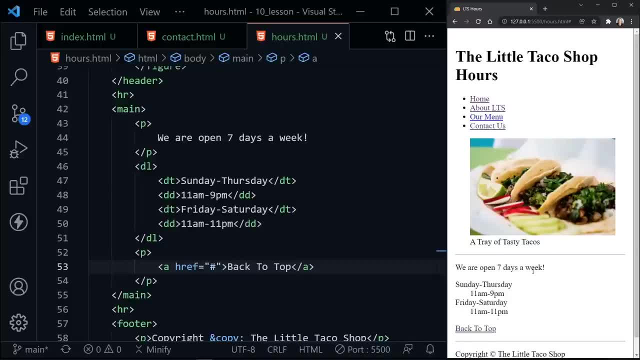 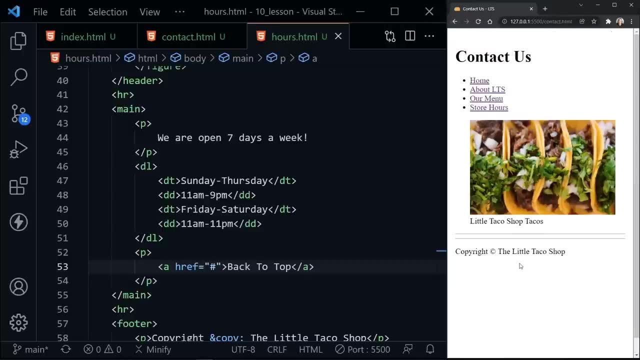 But we're just consistent between each page And that's fine. So let's go over to the menu page, Or not the menu? I'm sorry. We want to go to the contact us page. That's where we are. The menu is on the home page. 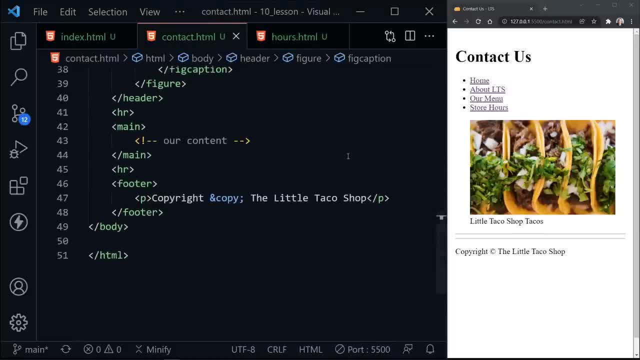 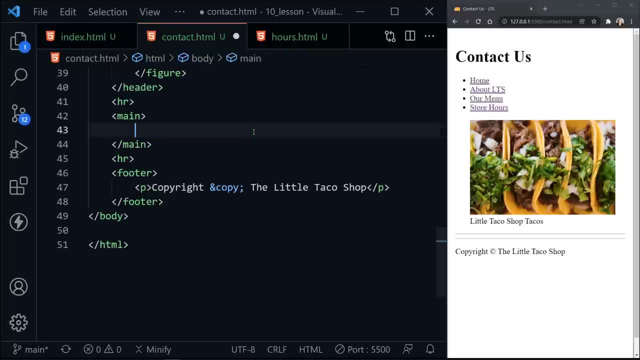 I don't know about you, But I'm starting to get hungry when I look at those. So let's finish up this project So we can go get some tacos. I'm going to scroll up And once again we're going to change out. 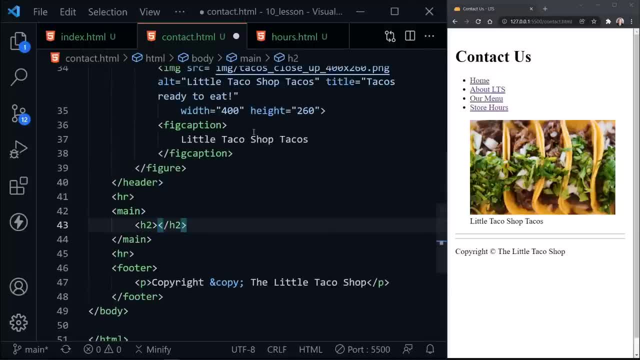 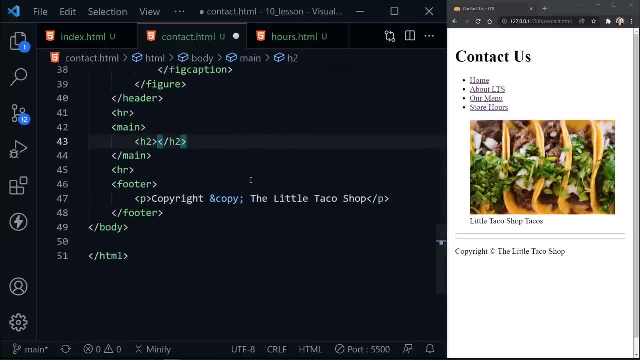 The comment inside of the main element And put in our content. Let's put this up here in the header. I believe if we scroll up There's the h1. So we want an h2 here And this h2 is going to say: 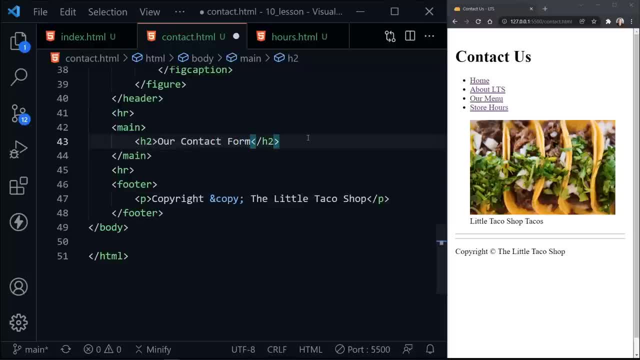 Our contact form. Okay, Now we need to go ahead and create this form. So we'll start with the form element And let's go ahead and give it an action. Well, there we go, Form Tab over and it gives us the action. 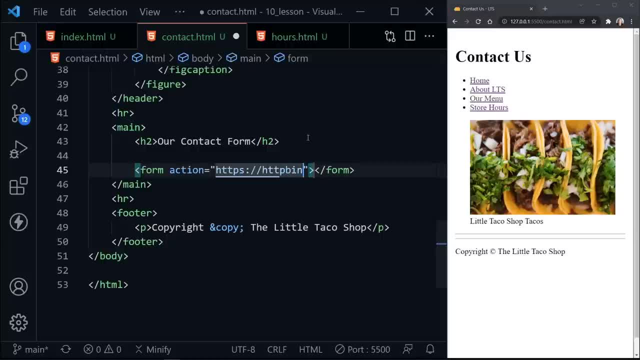 There we go. It's http, binorg, slash, git. So we're going to use a git method When we submit it, And we'll at least be able to see the information On that website. So, as I said, we use the git method. 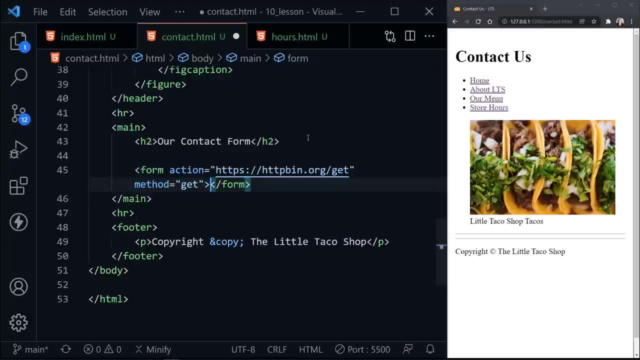 So let's go ahead and apply that attribute as well. Method equals git. After that, I'm going to put some space here in the form And we need a field set element. Now we can put our form Inside the field set element. 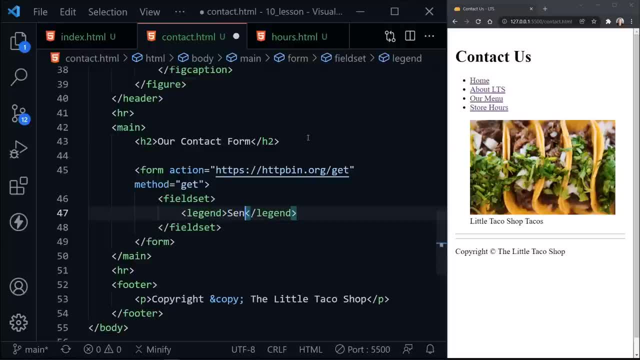 And then we'll have a legend element And here we'll say: send Us a message, And then We can start in with the description Of our form. So we have a paragraph, And then we have a label, And then it has a for. 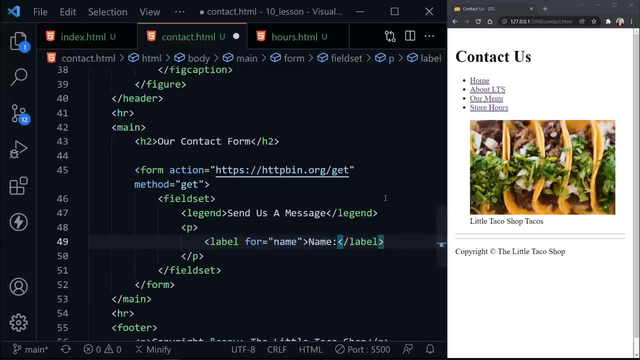 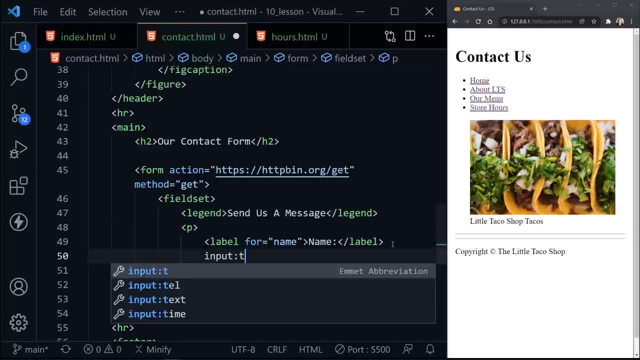 And this will be name. And so then we need to put name inside the label, As we label the input, And now we need that input. So here's the input, Let's give it a type. There we go Text. There it is. 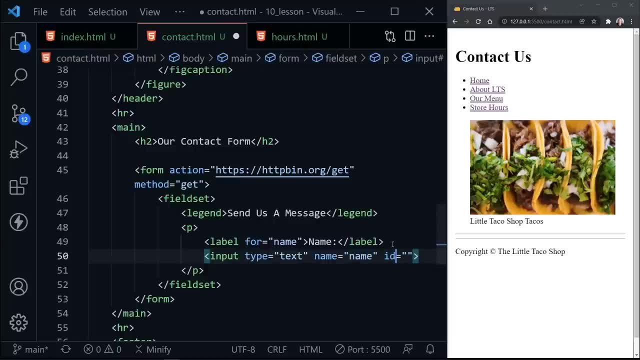 The name, which is name, And the id, which is going to be Name as well. And now I want a placeholder element Here also, And this placeholder Is going to say your name, Giving the user a clue as to what to put in. 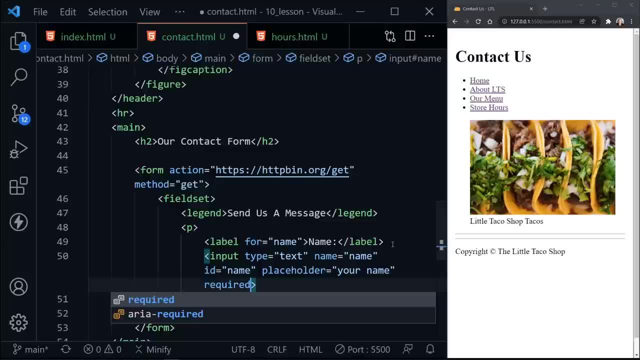 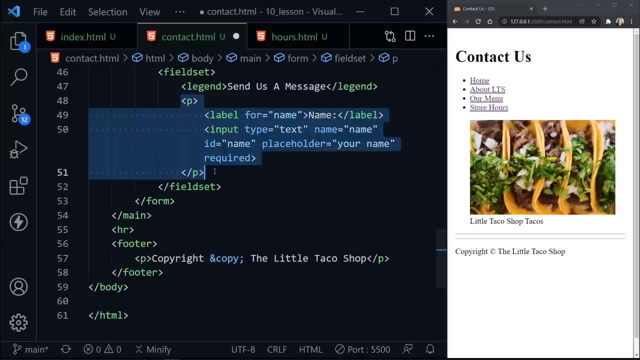 And let's put in required, As we want the user name To be required before they can submit the form. Scroll just a little more For some more room. I'm going to highlight this paragraph now And once again shift alt and the down arrow. 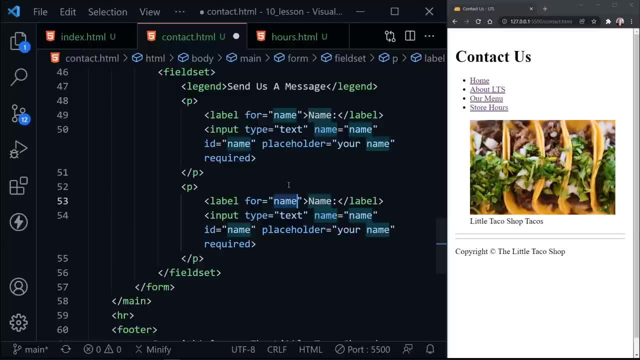 And now I've already got my label and input And I just need to change some of these things. So this will be email And we'll change name here to Email as well, And now this will be an email input. And then for the name: 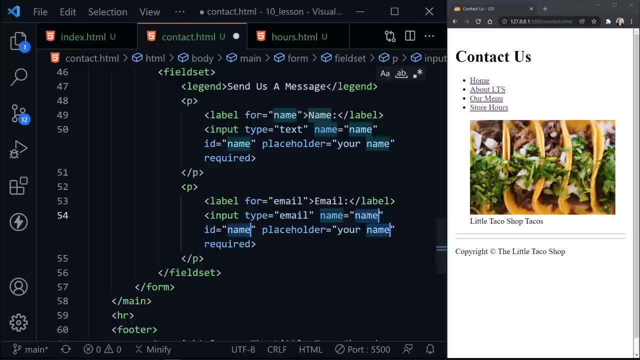 And id. I'm going to press control d For each of those remaining Name words And then I can change them all at once To email. Okay, I'm going to save this much And we see the beginning of our form over here. 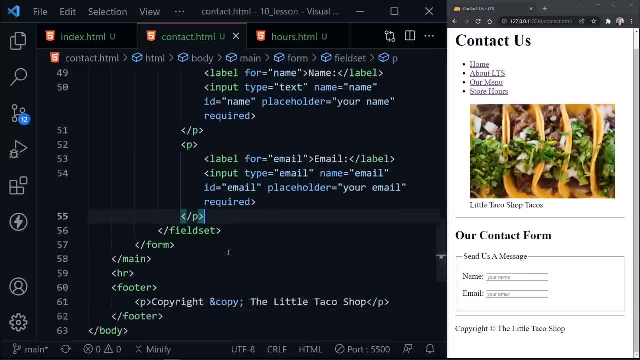 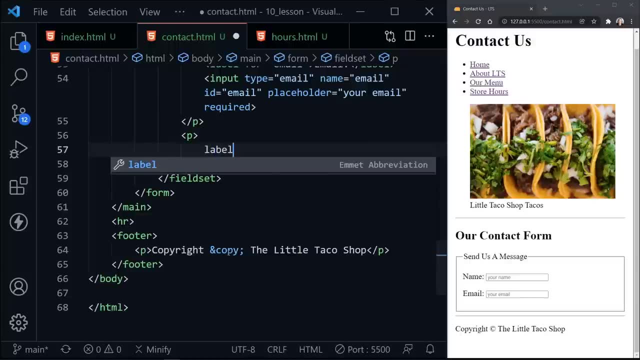 To put in the message. So I think I want to scroll some more for that And then return once again One more paragraph. Inside this paragraph, Let's have a label And now the for here is going to be message. And now inside the label, 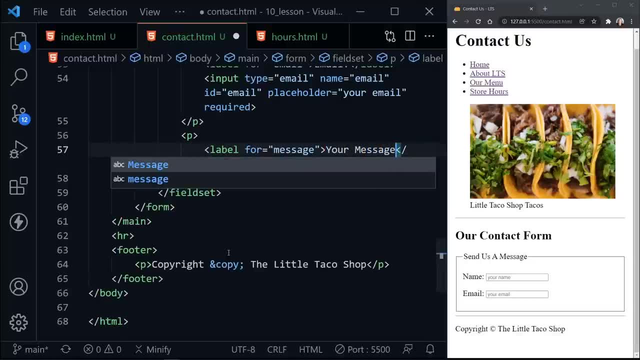 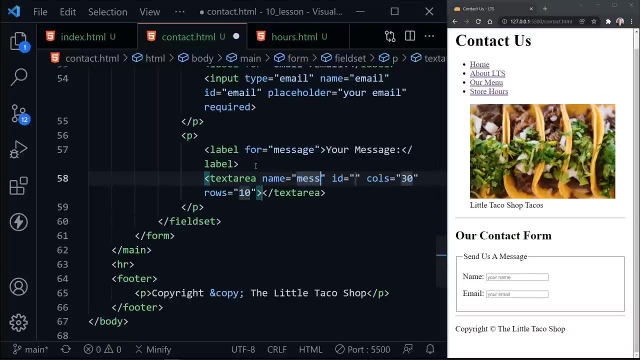 We'll also put: Well, we'll put your message here. That's fine. And then we need a text area Which is a little bit different than a text input. This is going to have the name of message And it should have the id of message. 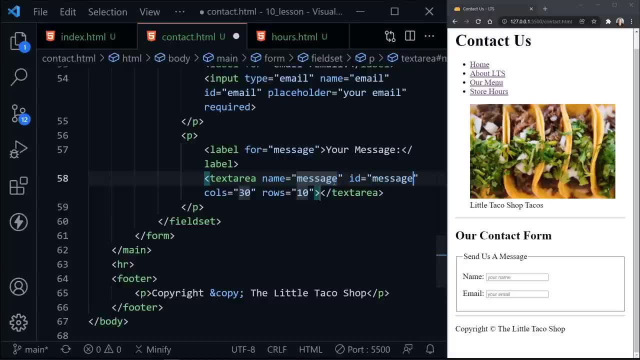 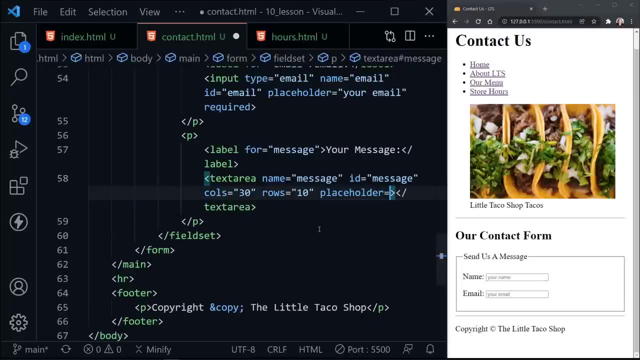 As well Columns 30 and rows 10.. That's fine, That is the default, And then placeholder also. So let's put a placeholder, Let's set that equal to type your Message here And then the actual message, of course. 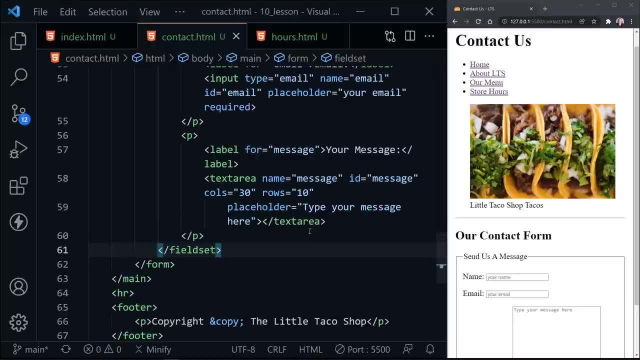 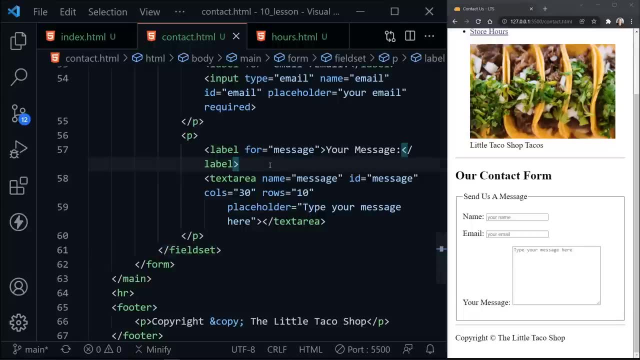 Goes inside the text area. So we'll save that, And now we should see a place they can put their message. Oh, but we can see it looks a little different. This doesn't look quite right. Let's put a break after that. 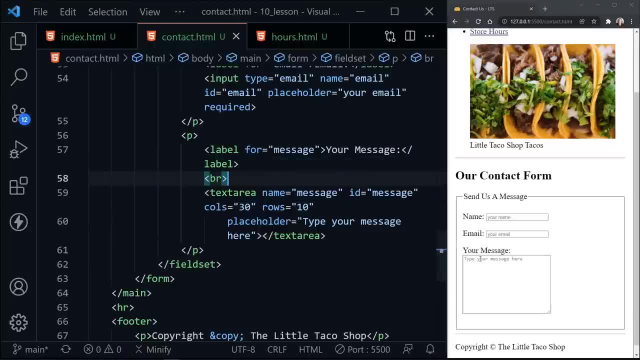 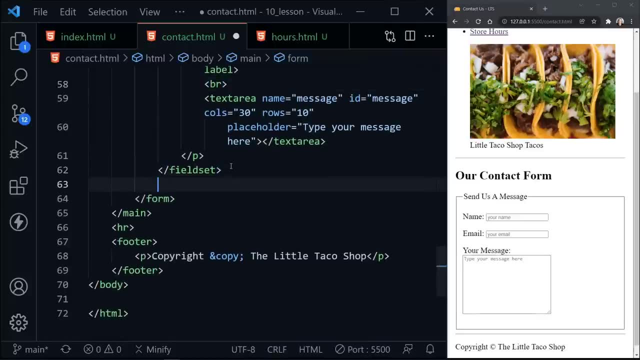 Label, And then it should put the label Up on top of that message box. Now let's scroll a little bit more And after the field set, But important enough, Before the form has ended, We need to put a button, And then inside of this button, 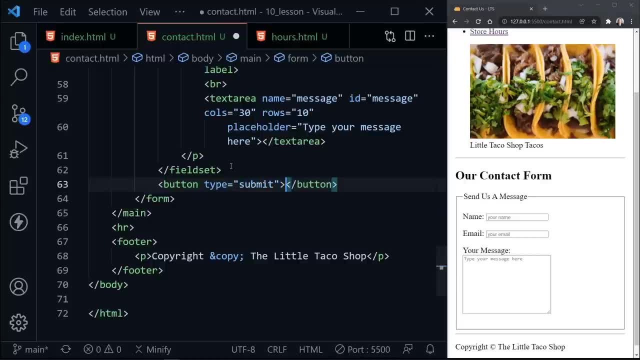 Let's give it an attribute Which is type equals submit, And then let's go ahead and put Send for the button text. I'm going to copy this down: Control, alt and the down arrow, And now this type will be reset. 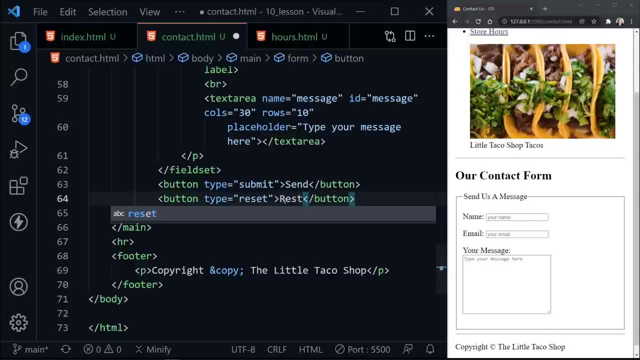 So we have a second button And we can put reset here as well. So now let's save And we should see our buttons That will send or reset the form. And as I look at everything, I've noticed something: We put our form inside the main element. 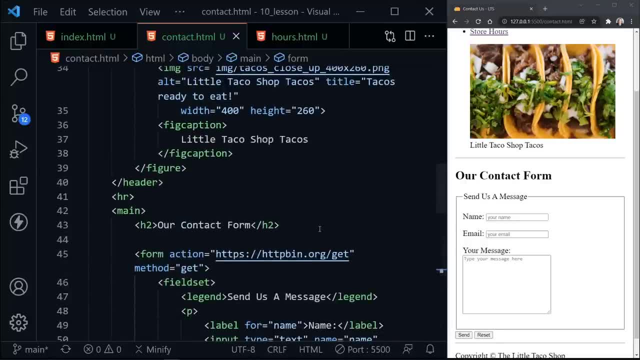 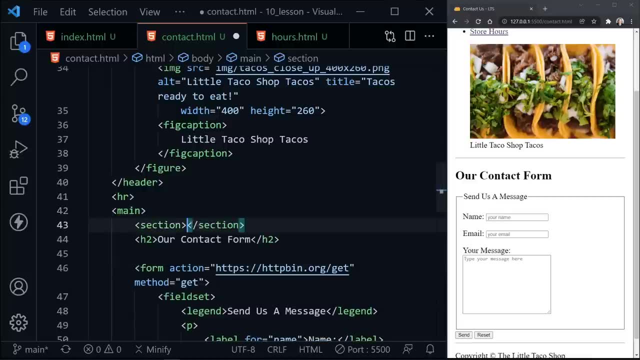 But I wanted to wrap that Inside of a semantic tag As well, Not just the main element, But I wanted to put it inside of a section element. So let's go ahead And put a section element there And we will copy that. 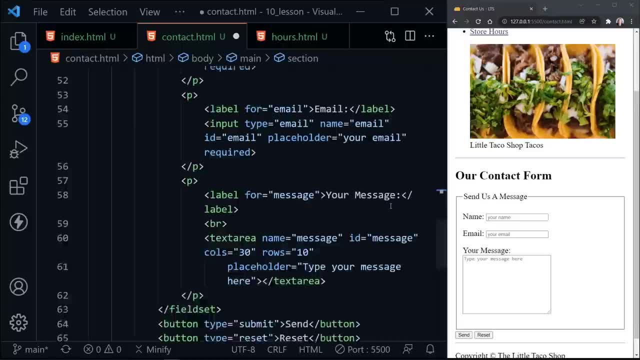 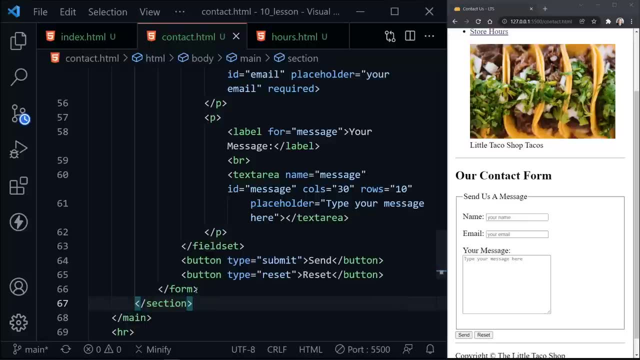 Or cut that actually With control x And scroll all the way down To where the form ends And put the closing section there. Now let's save that. It doesn't make the page look any different, But it holds up the HTML semantics better. 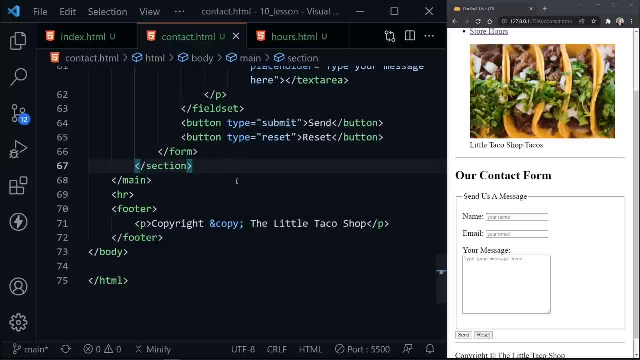 And the main reason we need it Is because the form Is not the only content of the page. So we have another section here, And this section Is the h2 of its own, And here we can put our location, Which goes nicely with a contact us page. 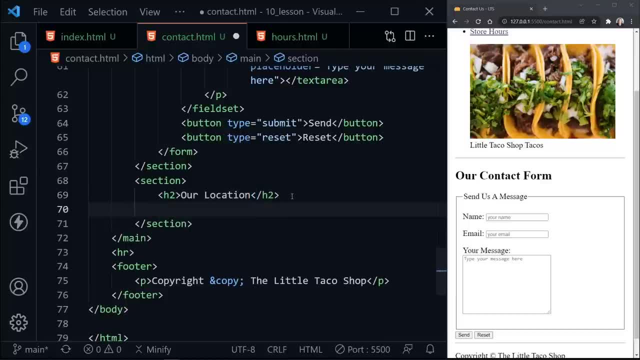 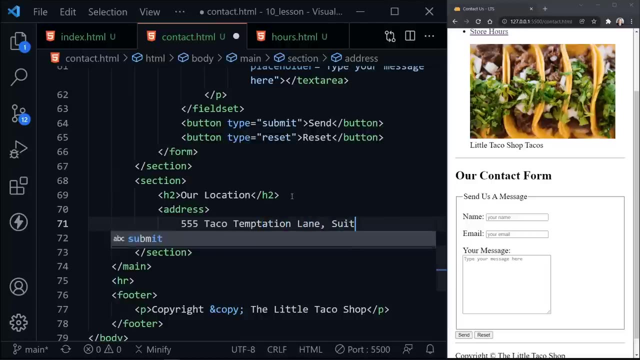 As well. So now we've got the h2 there And we need an address element, Because now we can put our location Inside of this address element. So it's 555.. Taco, Temptation Lane, And then it's at. 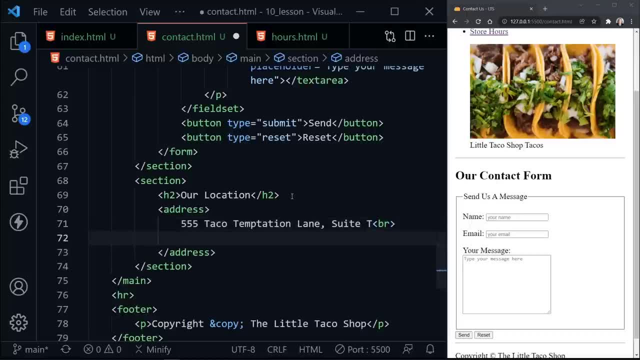 Sweet Tea Line Break, And then Kansas City, Missouri, And then 555.. 55-5555.. Completely fictitious zip code. After that We'll put in a line break And another line break, And then let's put in a phone number. 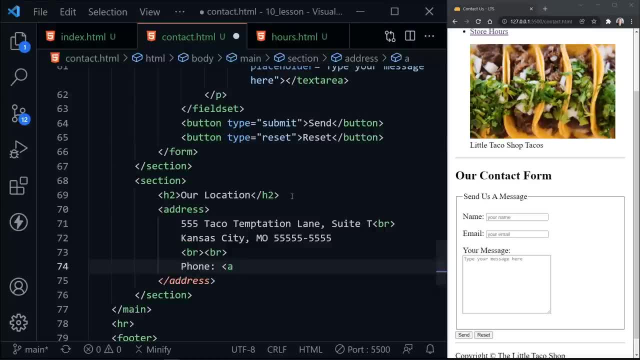 Which is also fictitious, But we want an actual link That will work To make your phone or whatever mobile device Dial the phone number, And we can do that with the tell abbreviation, And then we need A plus And then 555.. 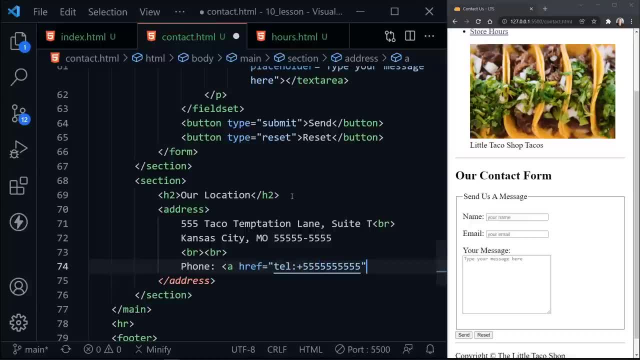 555.. 5555.. There we go, And then we can put the link, So it's 555-555-5555.. And now we've completed the address section. So if we save that And scroll up a little bit, 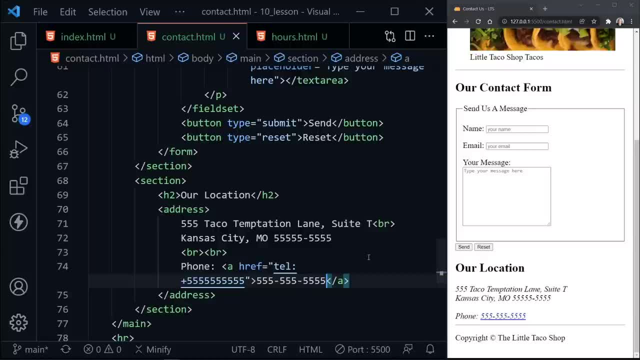 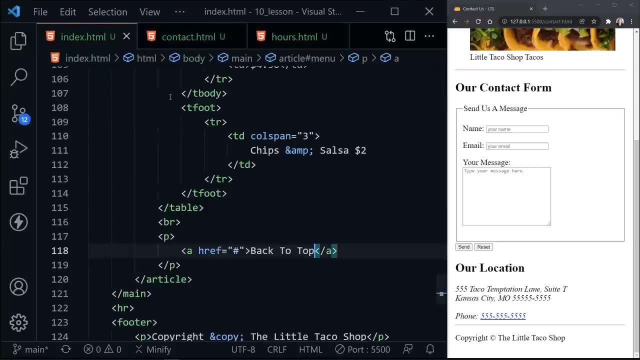 There is the location information And with that, I believe we have completed our website In the three pages. I hope this tutorial has helped And, more than that, I hope you were able to complete much of it on your own. Before watching the tutorial.